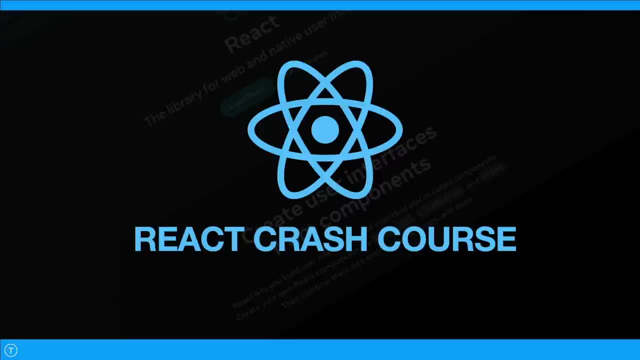 fundamentals. those aren't going to change as far as what we're doing here. So the biggest change to React 19 is that they're adding a compiler which will convert React code into regular JavaScript, potentially doubling performance. So it'll work in a similar way to frameworks like Svelte. Now, 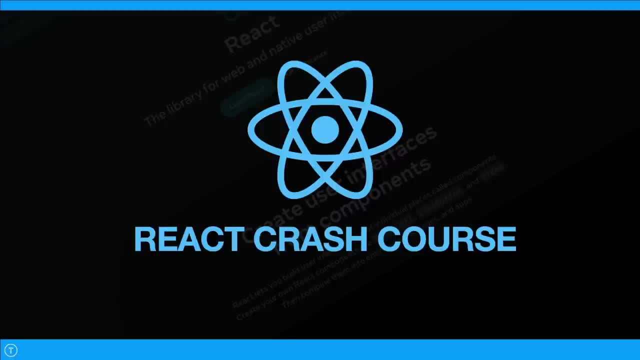 we're going to be using version 18 in this video, as 19 isn't released yet, but all the core concepts that we're going to talk about are the same, so it doesn't matter if you're using 18 or 19.. And I did. 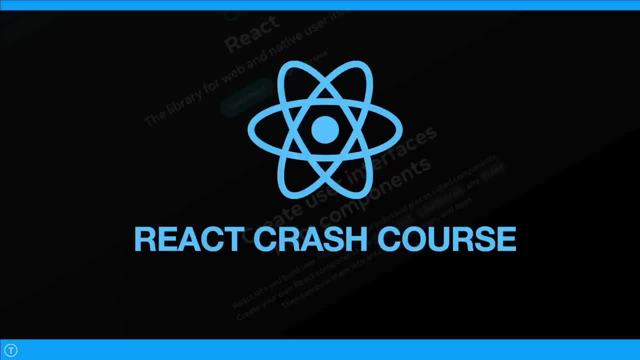 do a video on React 19 a couple weeks ago, and we used the experimental version of React to test out some of the new features, so that might be something that you want to watch after this, if you're interested. All right, so we're going to take a look at some slides and then we'll get. 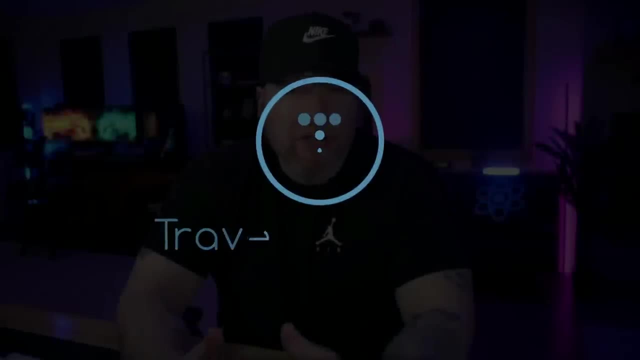 right into learning React. Okay, so, like I said, we're going to spend a little bit of time talking about React 19, and then we'll get right into learning React. So we're going to take a look at some slides and then we'll get right into learning React. 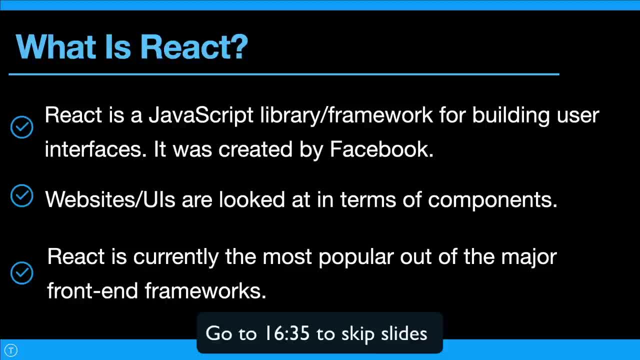 a little bit of time with some slides just to kind of give you an overview of what React is and what it entails. And I'm going to warn you that it may be overwhelming if this is your first introduction to the library, And that's why I like to to be more hands on and jump right in, But it can be helpful to have an overview, just so you understand what React actually is in some of the terms that we'll be using. So what is React? It's a JavaScript library for building user interfaces, And it allows us to build user interfaces. 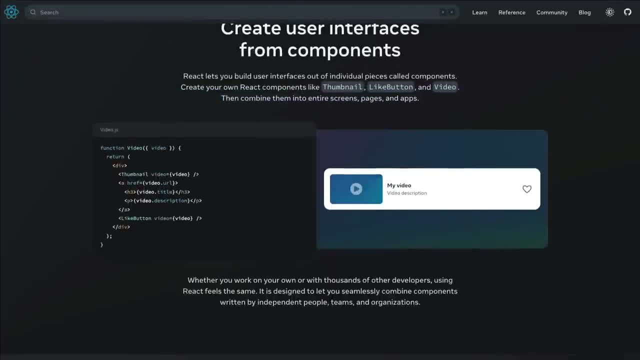 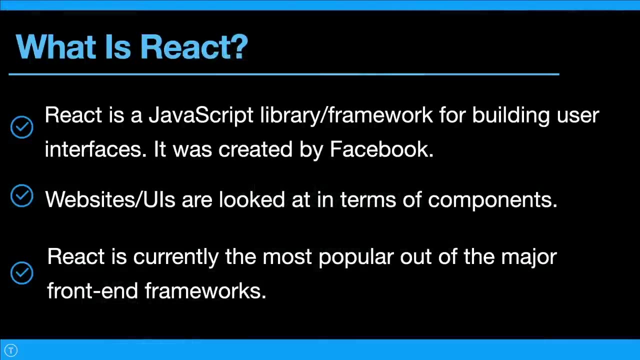 interfaces and front ends of websites and applications using components which I'll talk about soon, And it's maintained. it was created and maintained by Facebook and a community of individual developers and companies. You probably have heard React referred to as a framework. I refer to it as a framework all the time, But it's actually a UI library. 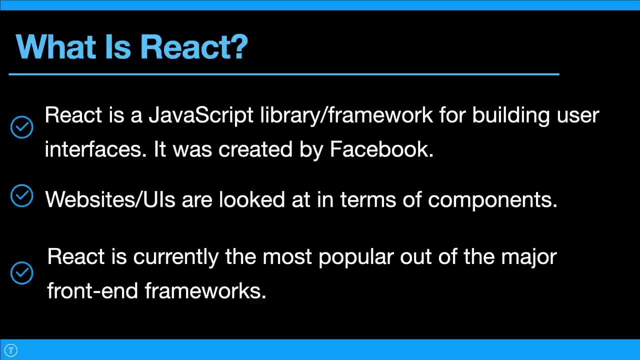 to be specific. And the difference is that a framework is a complete solution. So Angular, for instance, is a full-featured framework because it has an integration. it includes a router, an HTTP client, a state management library and much more. And the reason 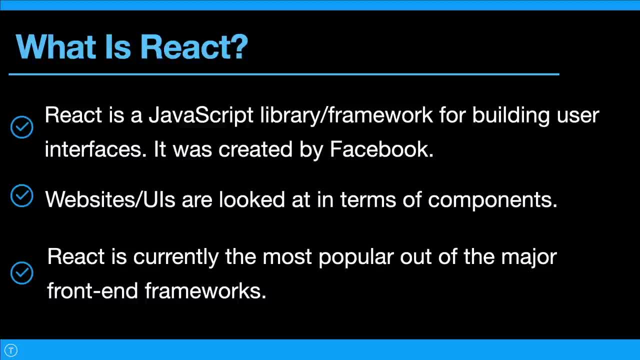 that React is often referred to as a framework is because it operates like one and it's in direct competition with frameworks like Angular, And, in fact, it's actually the most popular out of the major front-end frameworks, which are React, Vuejs, Angular and Svelte, And it's often used. 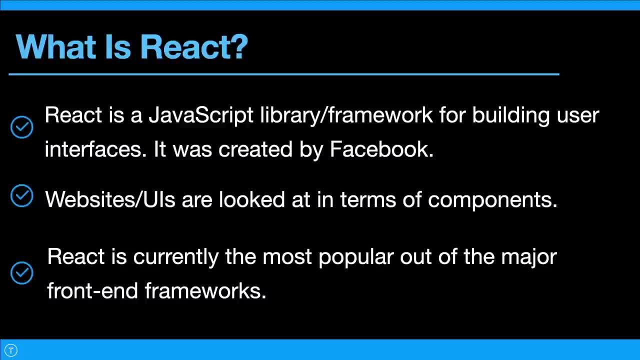 with other libraries, such as React Router, to create a full-featured solution. And also the ecosystem of React is huge, so it can be used for a wide variety of applications, such as single-page apps, server-side rendered applications and static websites, which I'll talk more about those. 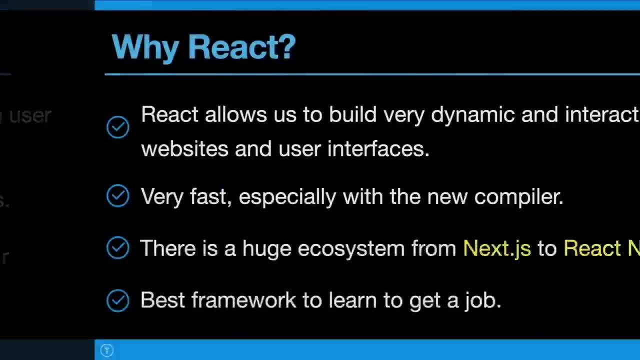 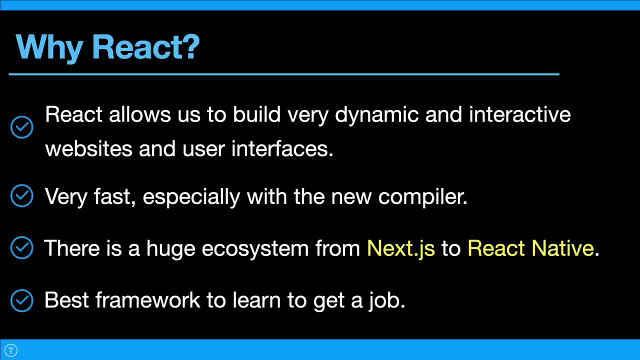 in a few minutes as well. All right, so why React Now? back in the day, the web was very static. You would click on a link and it would take you to another page. The entire page would refresh. this was the state of the web for a long time. Then came along AJAX, and this allowed us to make 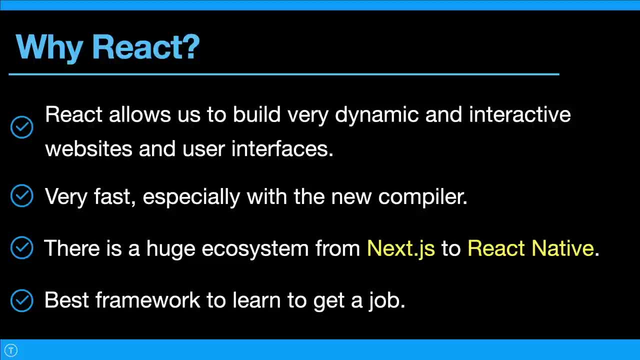 requests to the server and get data without having to refresh the page. And this was kind of a game changer in terms of the user interfaces, So it allowed us to build single-page applications where we can have a very dynamic user experience. But as this type of application and interface 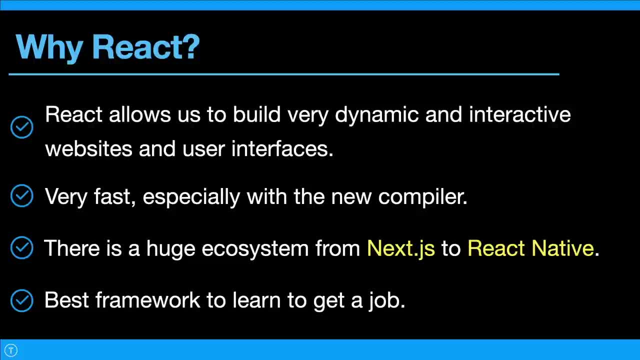 grows, it can become very hard to maintain, And this is where React and front-end frameworks come in. We can build dynamic UIs in a way that's easy to maintain and scale, And if you've ever tried to build a large-scale UI with vanilla JavaScript, you know. 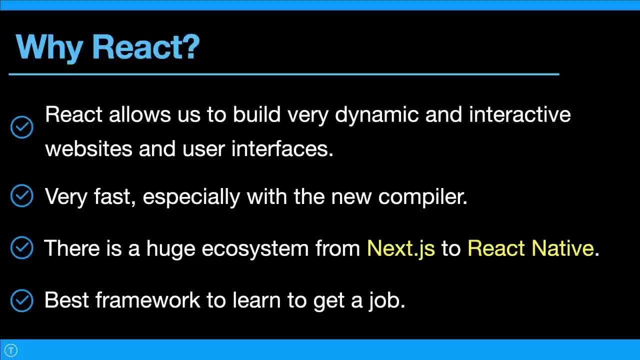 that it's quite a task and the code gets very unorganized and messy unless you build your own framework or something like that. So React and these other frameworks make this much easier. Now, traditionally, just to talk about how it works kind of under the hood, React used something: 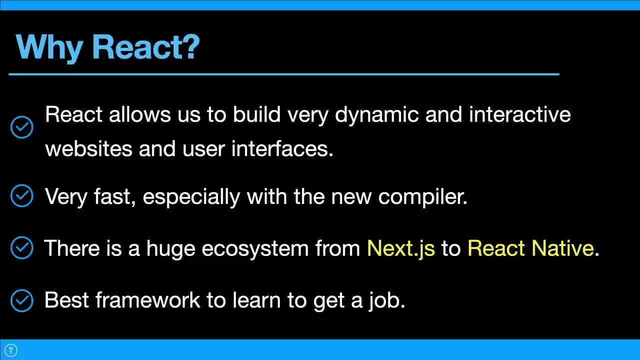 called the virtual network, And this is where you can build your own virtual network and you can use the virtual DOM, The DOM meaning the document object model, which you should be familiar with. If you're not, I would definitely recommend learning more vanilla JavaScript first, But the virtual 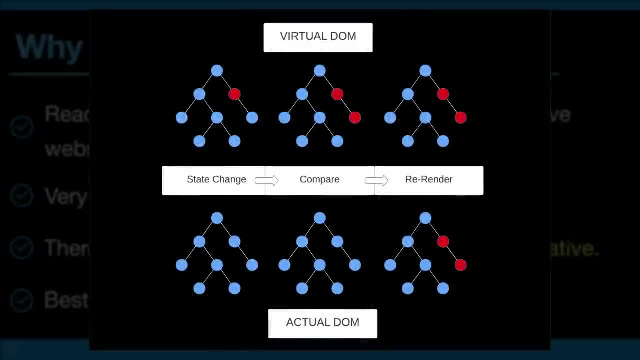 DOM is a lightweight copy of the actual DOM, And when the state of a component changes, the virtual DOM changes first, and then React will compare the two- the virtual DOM and the actual DOM- and it will update the parts that need to be updated. So this is traditionally how React works. That's how 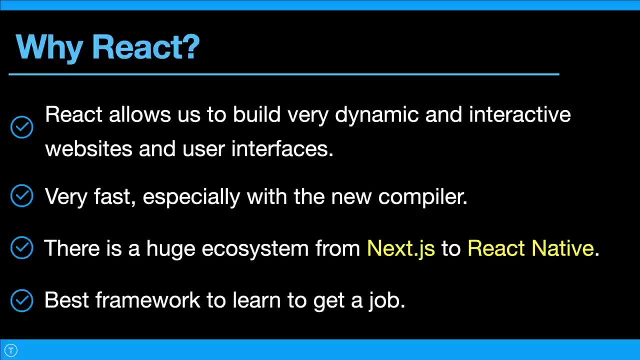 version 18 works- that we're using now, But with the upcoming version 19, React will have a compiler that, to my understanding, will replace the virtual DOM and it'll make things faster And it will also automate some of the tedious tasks. 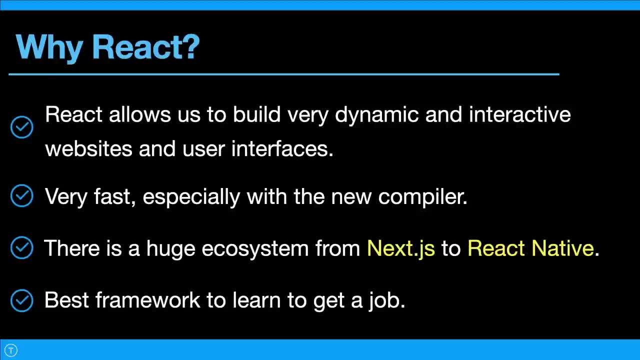 making React easier to work with overall. Now, most of the reasons to use React also apply to the other front-end frameworks as well, And if you ask me specifically why React over the other ones, I would probably say jobs. There's definitely a lot more React jobs. 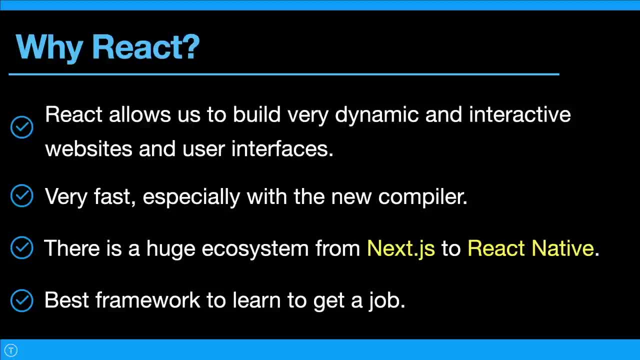 than the others. Also, the ecosystem is huge. when it comes to meta SSR frameworks like Nextjs and Remix. You have React Native for mobile development. It's definitely the most popular. Now I'm going to be 100% transparent with you guys: The reason that I use React and the reason 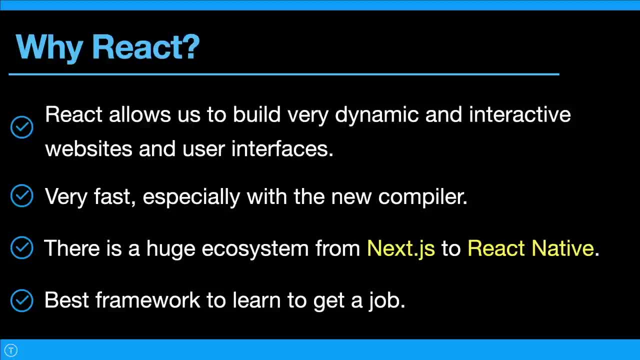 that I do most of my courses and videos on React is because of its popularity To me. Vuejs and Svelte do a lot of things in a much more straightforward way. If you're not caring about jobs, maybe you're a freelancer, or maybe you're just trying to. 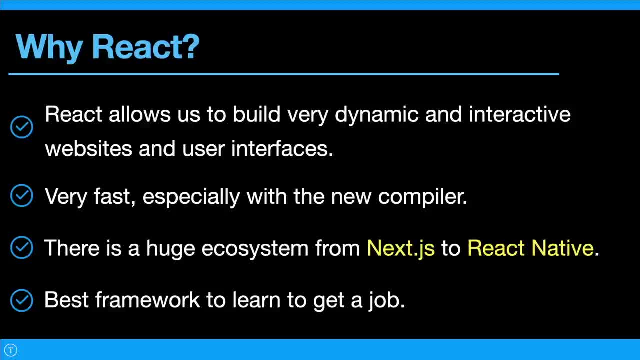 build your own products. I would definitely look into other frameworks as well, especially Svelte and Vue, because, again, I think React just overcomplicates a lot of stuff. Don't get me wrong: It's a great framework, but if we're just looking strictly at how we write our code using these frameworks. it's not going to be a great framework If we're just looking strictly at how we write our code using these frameworks. it's not going to be a great framework If we're just looking strictly at how we write our code using these frameworks. I think that Svelte and Vue are 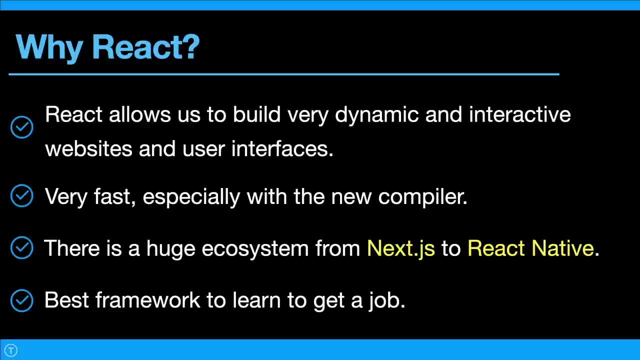 easier With that said, that is just my opinion, so take that with a grain of salt. Also, these frameworks basically do the same thing and once you learn one, if you learn React now and then you want to jump to Vue. it's going to be easy. It's just syntax that changes The. 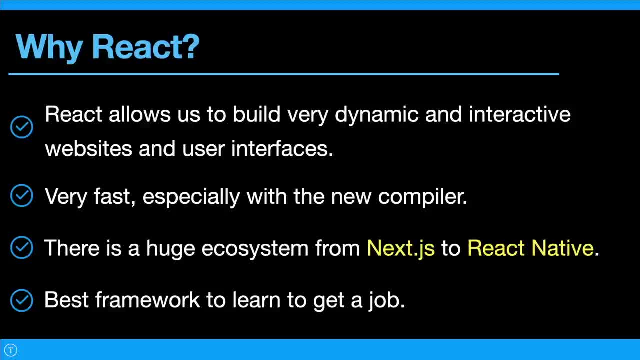 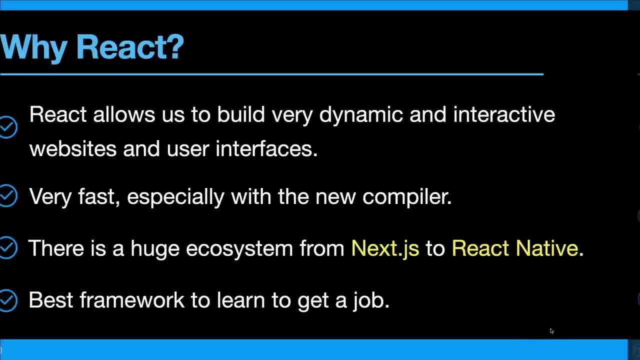 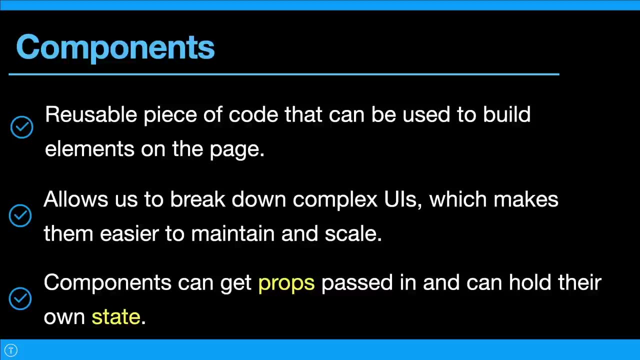 core of what you're actually doing is the same: You're still writing components, You're still writing your own syntax, All right. so, speaking of components, components are the core concept of not just React but any front-end framework, And a component is a reusable piece of code that 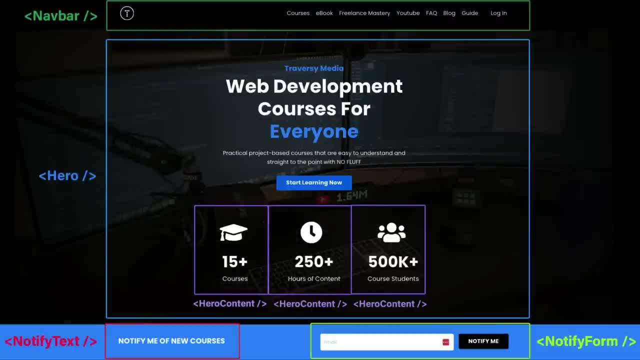 can be used to build elements on a page. Components can kind of be thought of as custom HTML elements, And components can be broken down into smaller ones. This is called composition, And this is a great way to build UIs, because it allows you to break down complex interfaces. 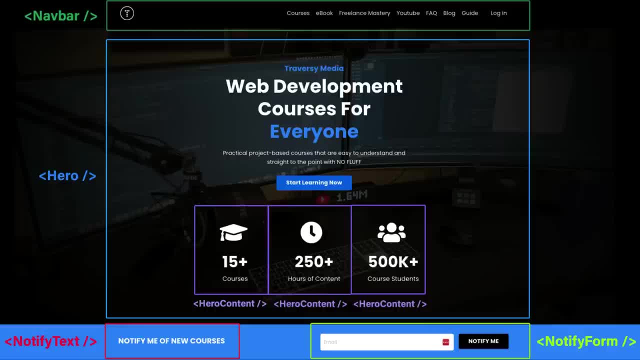 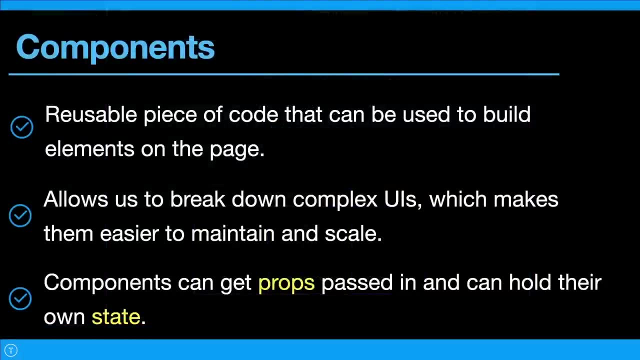 into smaller ones, And this is a great way to build UIs because it allows you to break down smaller, more manageable pieces, And this makes your code easier to maintain and scale. And components can be either classes or functions. However, classes are kind of the older way of. 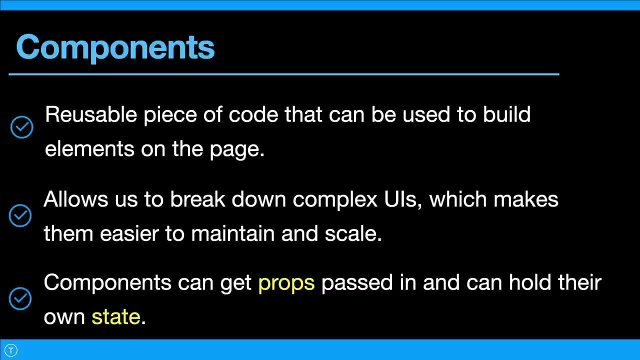 doing things in React. Nowadays you're not really going to see class-based components. They're all functional. We will be using functional components in this course and in any other course I do. Components can also take in props, which are basically like arguments or 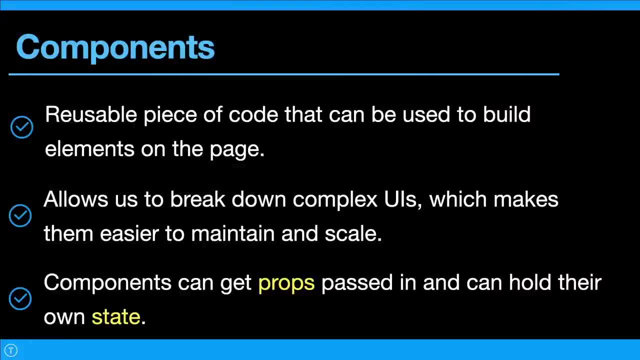 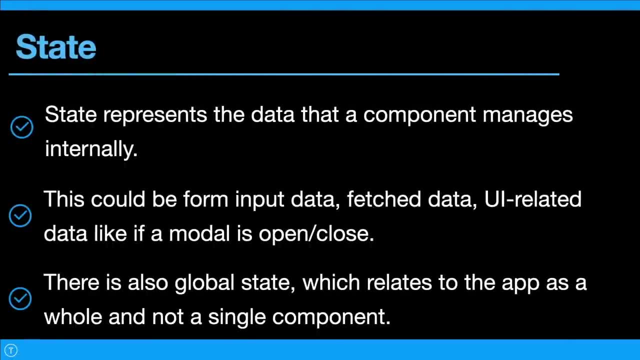 attributes And they can also hold components in a way that they're not going to be able to hold their own state or their own data. Now, state is another thing that you're going to have to wrap your head around when working in the front end. State represents the data that a component 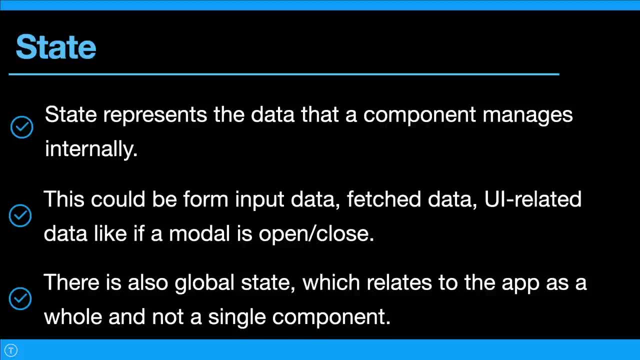 manages internally. It allows components to store and manage their own data, which can change over time And it'll change in response to user interactions or other factors. Now, state is typically used for data that's expected to change, such as user input, fetch data from APIs. 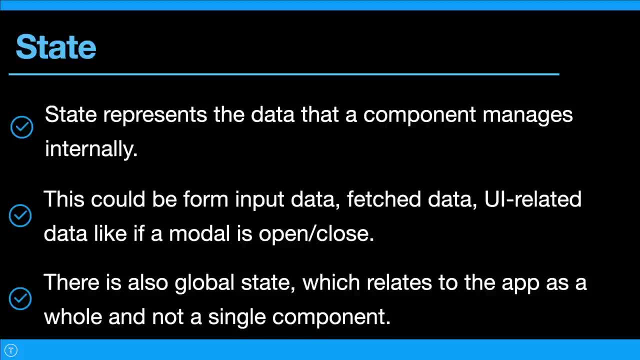 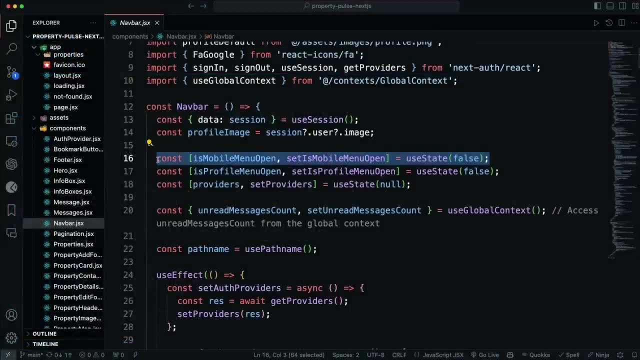 or UI-related data, like whether a modal is open or closed, And to define state in a functional component, you can use a hook, And I'll talk more about hooks in a second. You'll use the use state hook, which is a built-in React hook, And this will return an array with two elements: the current. 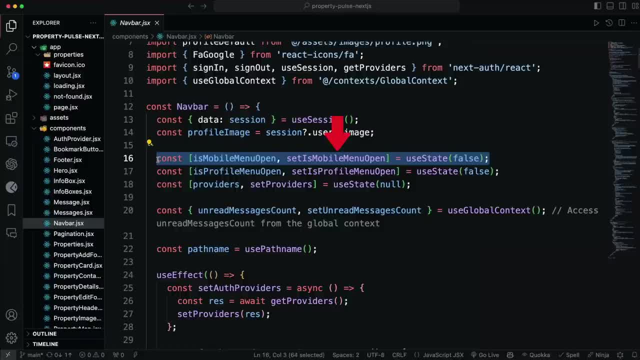 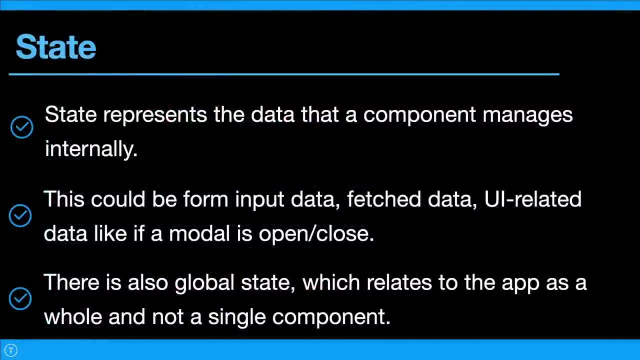 state value and the function to update that state. And again, we're going to get into this. I know that just hearing me say this doesn't tell you much. We will get into examples Now. there's also something called global state, which relates to the app as a whole and not just 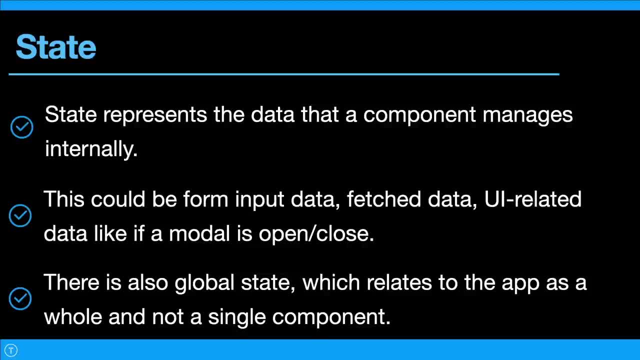 a single component. So this would be something like the data that you fetch from your database. You probably want to share that with multiple components. So there's ways to handle this, everything from just keeping your global state in your main component and passing it down to. 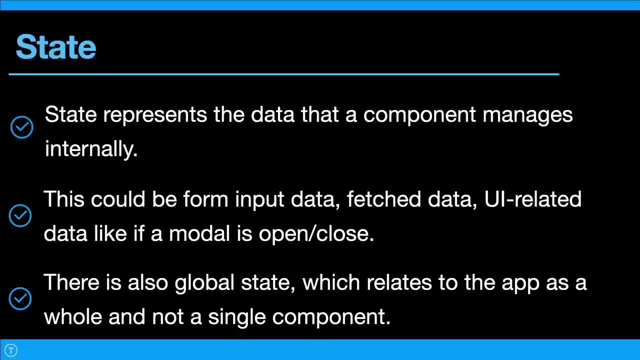 child components to the React context API, which is beyond the scope of this tutorial, but it is an option within React. You can also use a third-party state management system like Redux. Okay, now, we're not going to get into context or Redux, but we will look at some global state. 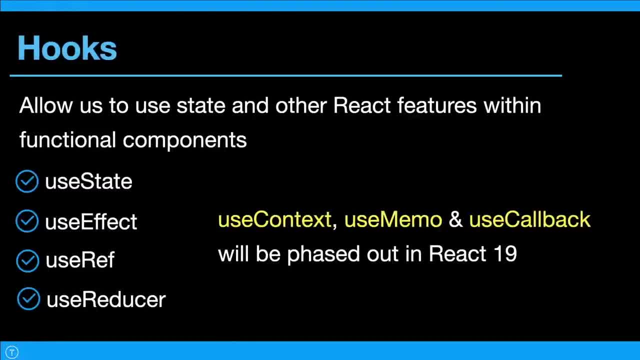 later on. Now, if you've never used React before, hooks can be really intimidating. They're also difficult to explain, so bear with me. Once we start using them, it'll be more clear Now. React hooks are functions that enable functional components to use state and other React features. 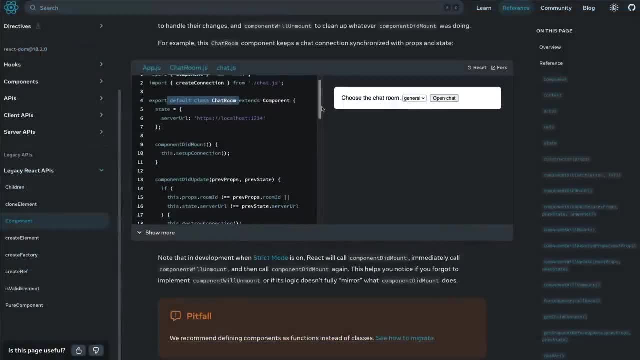 without writing a class, Because, like I said, if you're using React, you're going to have to use a class. So, if you're using React, you're going to have to use a class. So if you're using React, React components used to be classes and they used to have something called lifecycle methods. 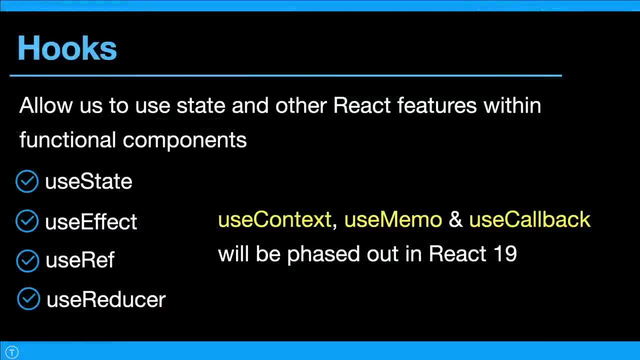 which were methods that ran at specific times during the component rendering process, And functional components don't have lifecycle methods because they're not a class, So hooks allow us to do the same stuff that we could do within class components, such as set state. 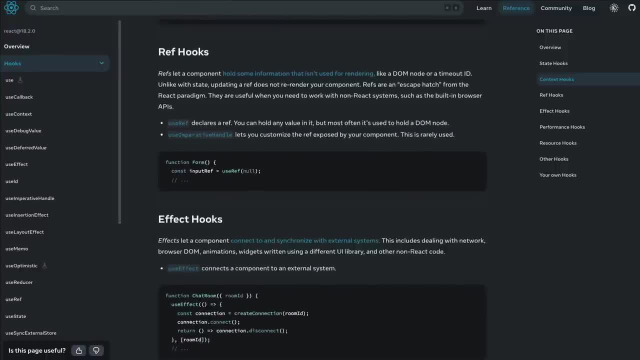 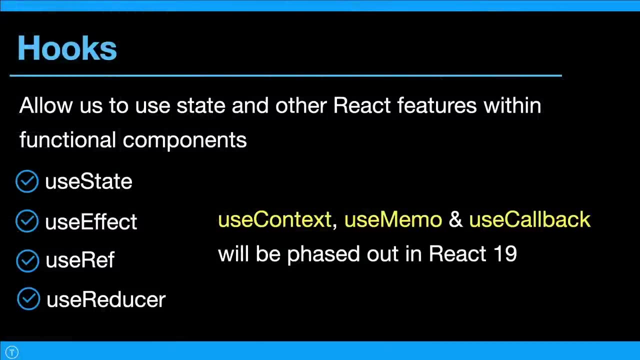 such as perform effects like data fetching on load, things like that. And basically right now, at this point in your learning, the two main hooks that you need to know are use state and use effect. The others aren't really essential for you to know, at least right now. In fact, three of them are being phased out in React. 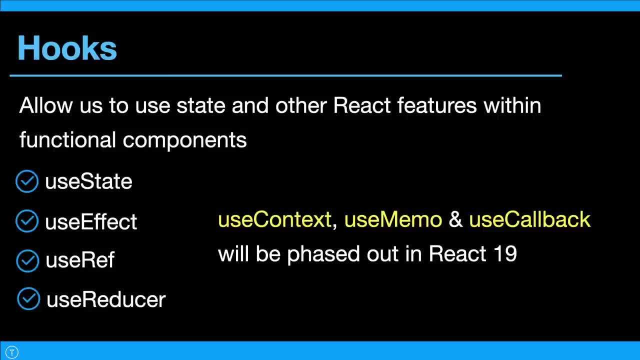 19.. As you can see, all hooks start with the word use, So you can also create your own custom hooks to use within your components, And that's not something you need to know right now, But just know that you can create a hook that basically does anything. All right, so I just want to give. 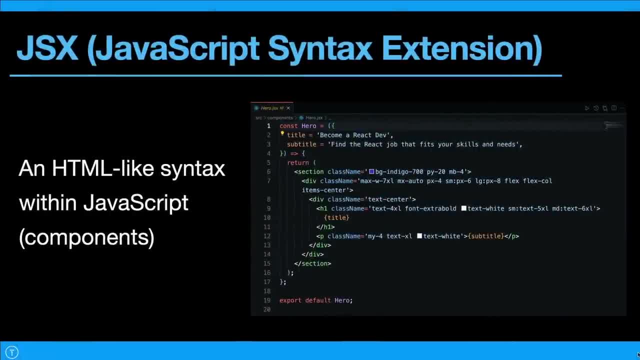 you a full picture of what a component does. So I'm going to go ahead and start with this. So I'm looks like. So we know that it can have state associated with it, which is just data, and it can also take in props. Now the other part of a component is the output, and the output is JSX. 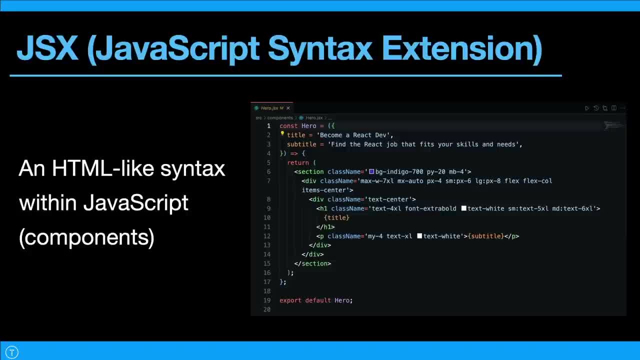 or JavaScript Syntax Extension, and this is basically HTML or an HTML-like syntax within your JavaScript. that and that's what is actually returned from a React component. So this is actually an example. right here you can see, there's it's a function called hero. it's taking 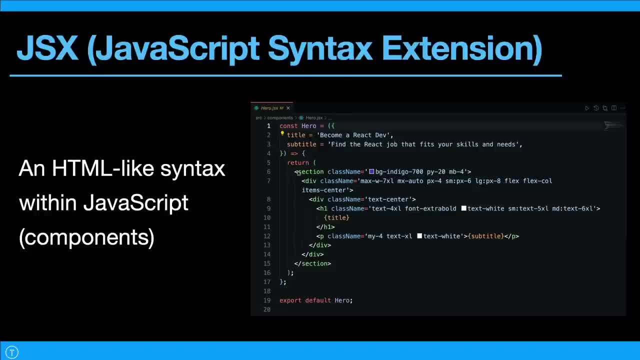 in some props, a title and subtitle with a default, and then it's returning what looks like HTML, but this is actually JSX. Okay, what's great about JSX is that it's dynamic. it's basically what HTML would be if it were a programming language. You can see right here we're outputting title. 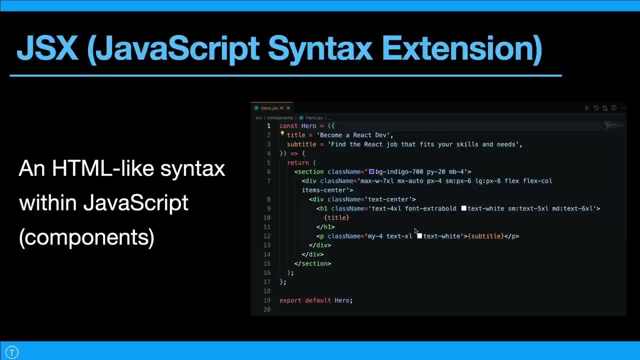 and subtitle, which are coming from these props. All right, you can also have expression. you can have loops, conditionals. you can basically do anything within your JSX, All right. so there are some differences when it comes to HTML, as you can see. you can't use class, because that's a 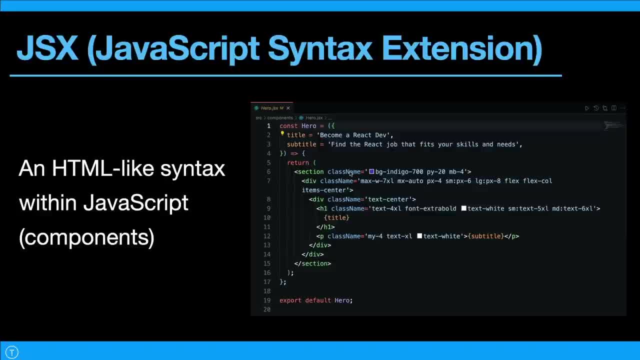 reserved word in JavaScript. so instead we use class name also, for if you, let's say, you have a label with a for attribute, that's going to be changed to HTML for. So there are some slight differences, but for the most part it's just HTML. All right now. I was a little hesitant to even 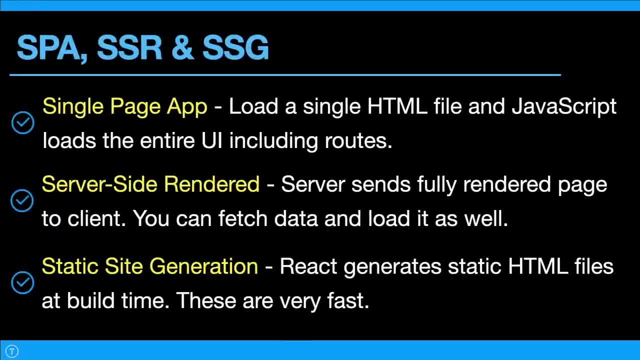 add this page because I think it might confuse some people, so if you don't understand it, that's fine. don't worry about it at the moment. So there's different types of applications and websites you can build using React. So what we're going to be doing today is a spa or a single page. 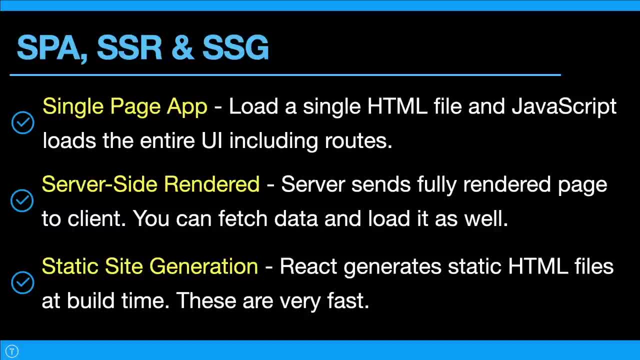 application, and this is what these frameworks were initially created for. So, basically, it loads a single HTML file and index HTML in the browser, and then it it loads a JavaScript bundle that includes your entire UI, your entire application, basically, And this allows our interface to be. 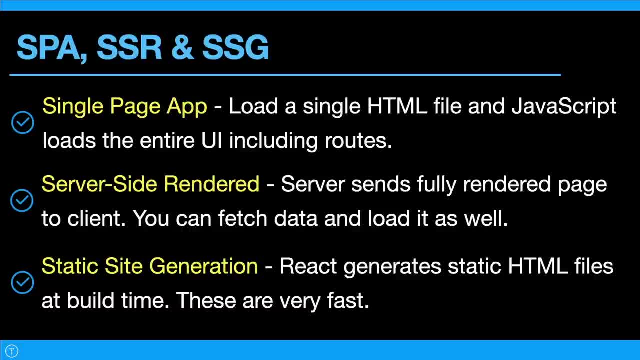 very interactive and even if you go to a specific page- like, let's say you click on a link and go to slash about, it's not actually loading the about page on the server. the JavaScript is loading that content for you. So spars are, like I said, great for really fast, dynamic interfaces, but it can 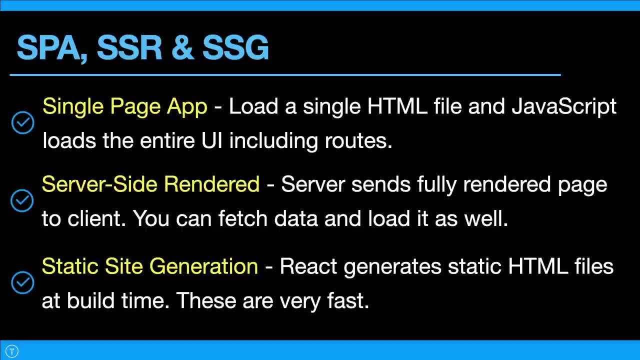 have some issues when it comes to initial page load times, As well as SEO, since the content comes from JavaScript. So the solution for that is to create a server side rendered app, which you can do with a framework like Nextjs or Remix. Now these 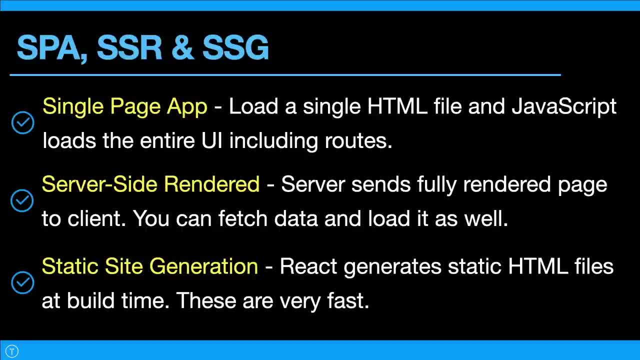 frameworks still. they still use React. You can kind of think of it as a wrapper around React- and instead of everything being bundled in the JavaScript, the initial page load is rendered on the server. So this is good for SEO. It's also good for the. you know the initial page load time. 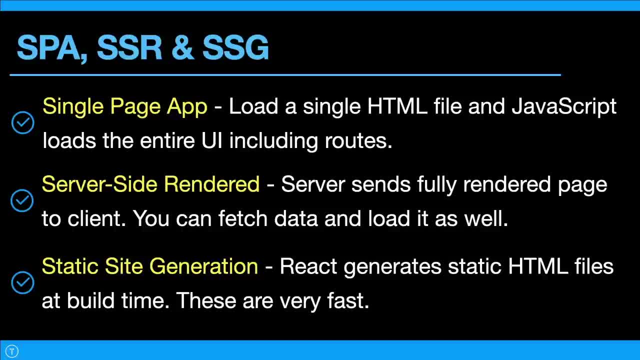 Now an SSR or a server side rendered app is a little more difficult to deploy because you do need a server. A single page app you can pretty much deploy to any any type of host SSRs you you use something like Vercel or Netlify or something like that. Now the third option is: 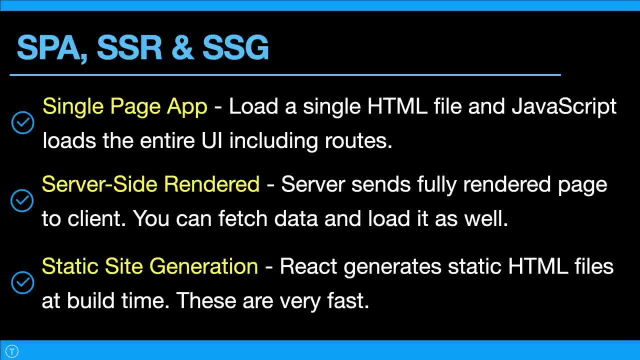 static site generation. So a static site is where the server generates a bunch of HTML files at build time. So we have frameworks like Gatsby and Astro that can do this, And those frameworks also use React. So I know that this can get complicated because there's just so many. 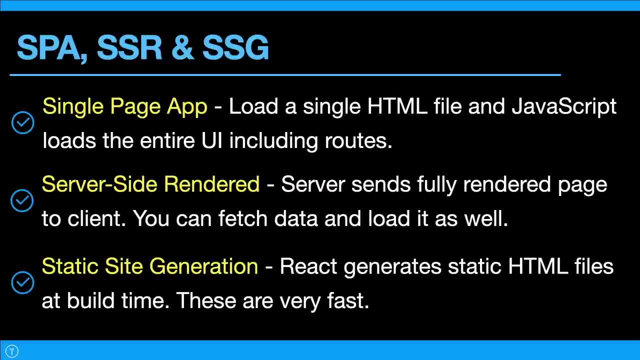 damn frameworks, But just know that they're all using React. So what you learn today still applies: whether you're using Gatsby, whether you're using Nextjs, Astro, you can actually use React or Vue or Svelte components. But yeah, what you're learning today is basically the core. 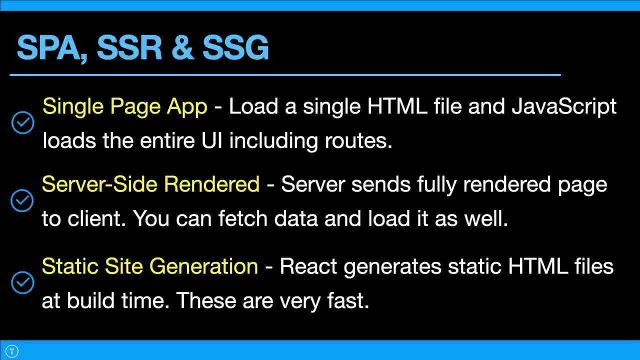 of all this other stuff. So don't worry about learning this other stuff right now. Just know that it is available And just know that if you're confused, that's completely normal. You should be. It's JavaScript. You're always going to be confused And I just realized this is React. 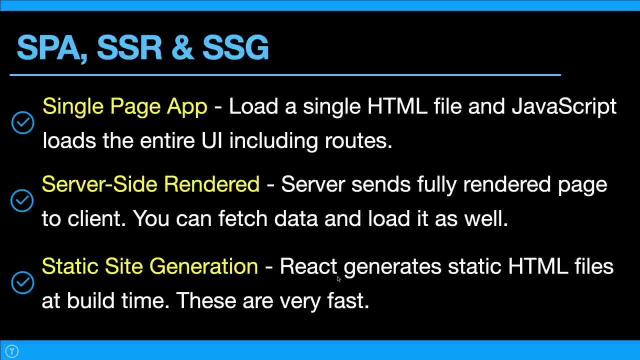 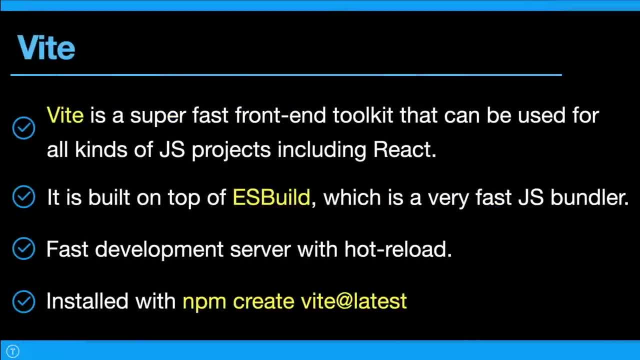 generate static HTML. That's not really accurate. It would be the, the meta framework, like Gatsby, that is generating it, not React itself. Now there's a few ways to get started with React. We're going to be using a tool called Vite, along with the React. 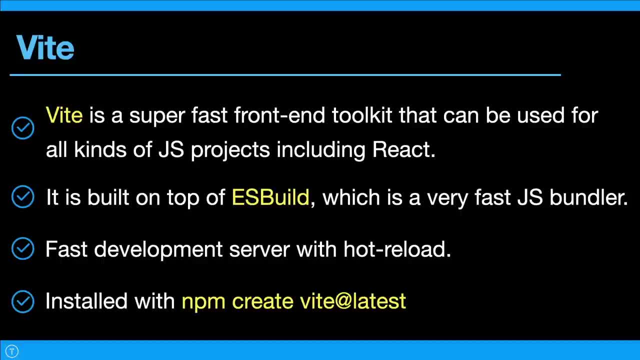 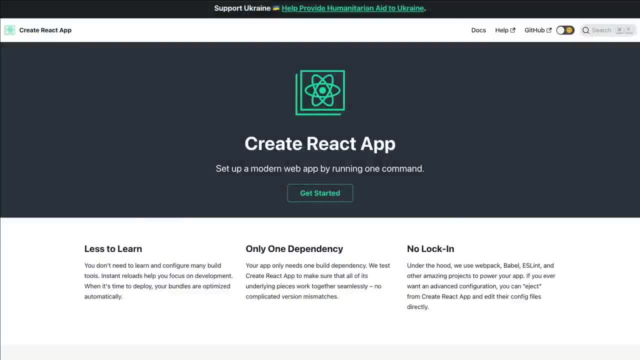 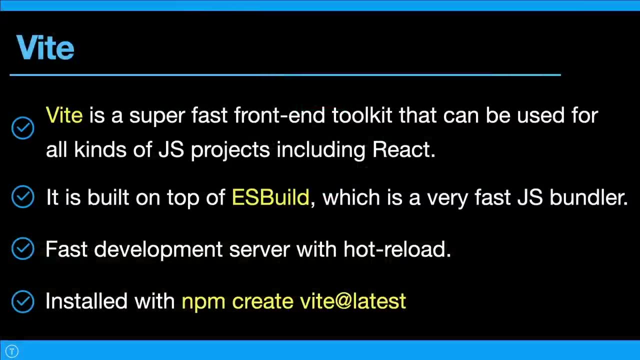 plugin And getting set up is as easy as running this npm command. Now, create React app was the most popular option to build a spa with React And it's been around for a long time, But it's no longer recommended. It's a bit bloated, It's slower And, as far as I know, it's not supported anymore. 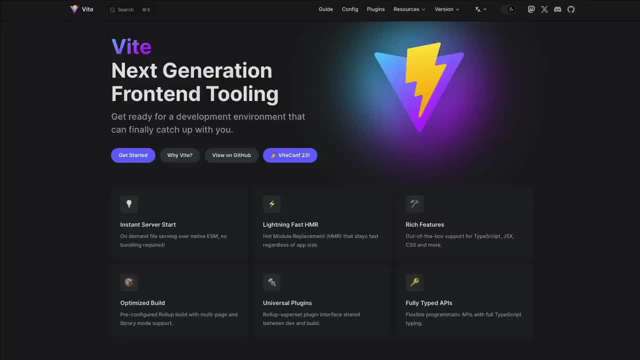 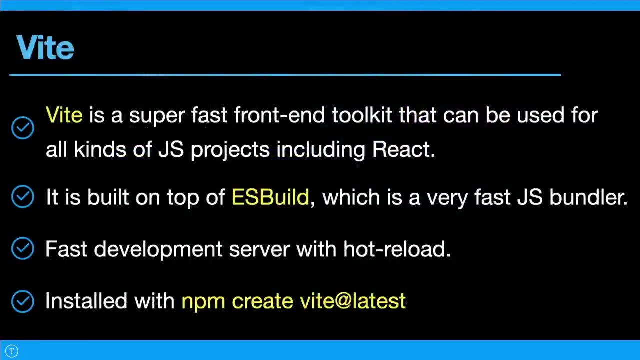 So Vite is a newer solution that's faster, It has a better developer experience. It's built on top of something called ESBuild, which is a very popular software- And it's a very popular software- fast JavaScript bundler, And it also has a built in development server with hot module. 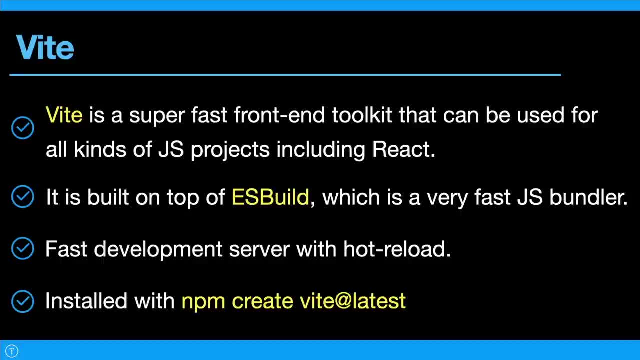 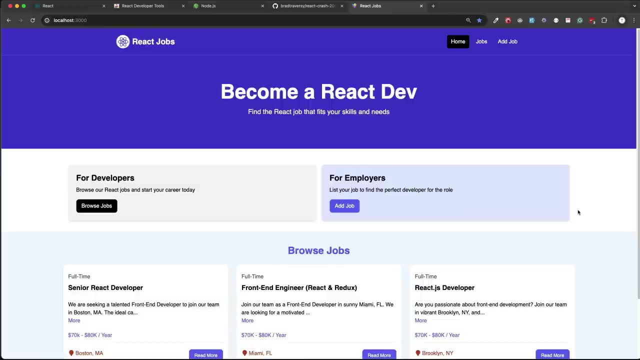 replacement. So it's a great solution for building spas with react and other frameworks as well. So that's it. Let's jump in and let's get our hands dirty. learning react, All right guys. So real quick. I just want to explain how my crash courses go if you're new to them. So basically the point. 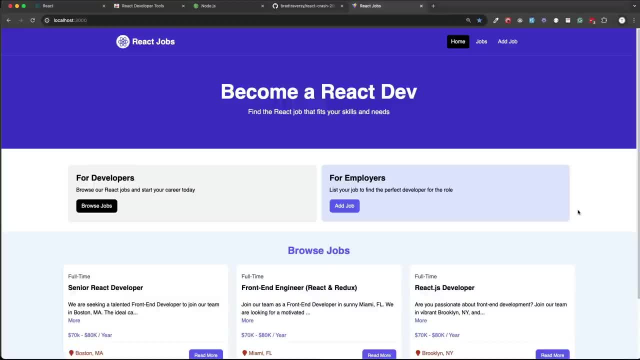 of this is to teach you how to get up and running with react in this case, And we want to go over all the fundamentals. But I also want to create a project and end up with something that you can have, that you built by the end of it. So this is what we're going to create: this react jobs website And. 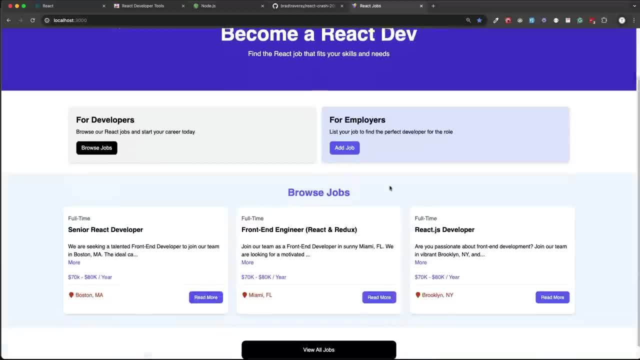 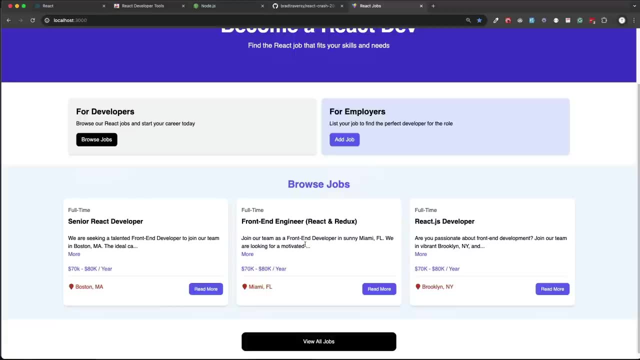 it's just a job listings front end. Now, as far as the data itself, it's going to be coming from a mock back end that we're going to create with JSON server. It's really simple Basically, we just create a JSON file with some data and we can then send, get, get requests put post. 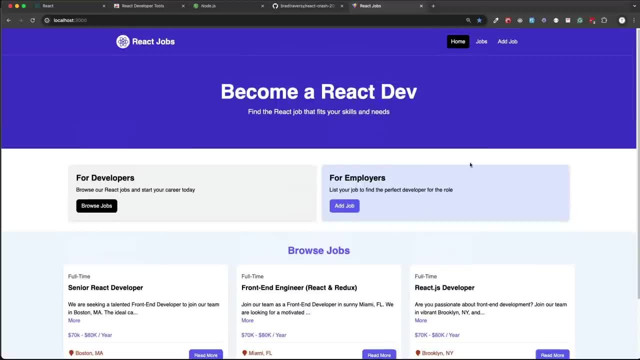 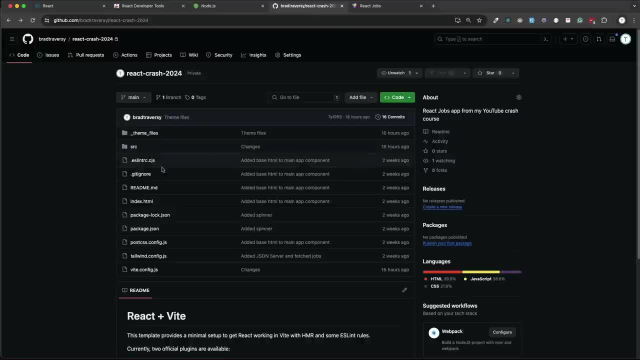 and we're going to add crud functionality, All right. So as far as the template here, the design, this is a tailwind theme that I created And in the repository you'll have your source folder with you know all your components and react stuff And then this theme files- underscore theme files- is 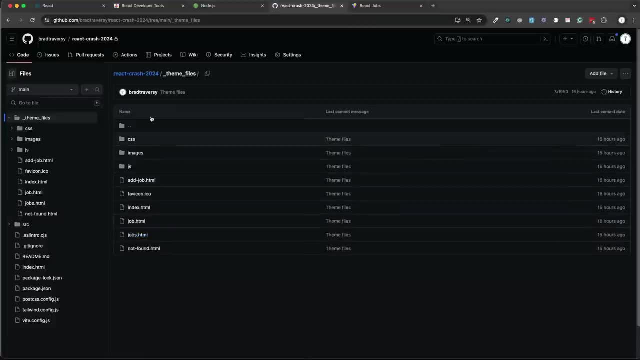 going to be just the HTML files, basically just a theme. It's not going to actually fetch data or anything like that. It'll all be hard coded, but it'll have all the code And then we're going to have all the classes and all the stuff that we need for styling. So we'll be copying some of that as. 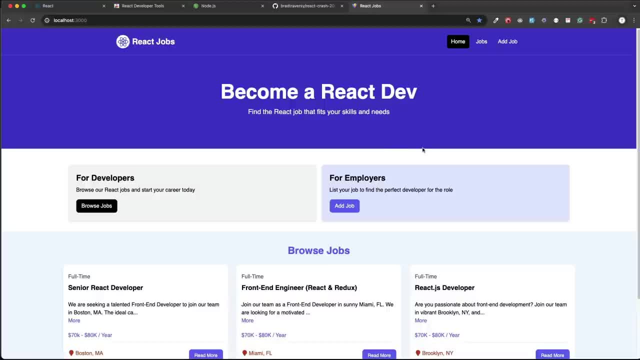 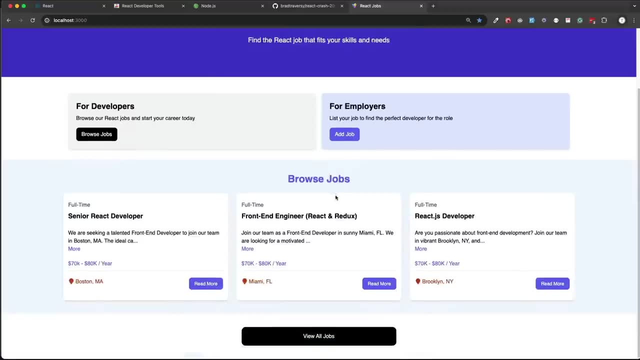 we go along because I like it to look decent. Now, just to quickly go over this, the home page. we have a hero component, nav bar component, some boxes, and then we're going to fetch our jobs and list three of them on the home page. We can toggle the description here. just to give you an example of 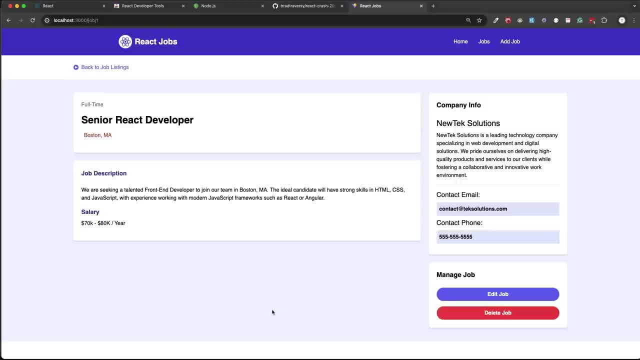 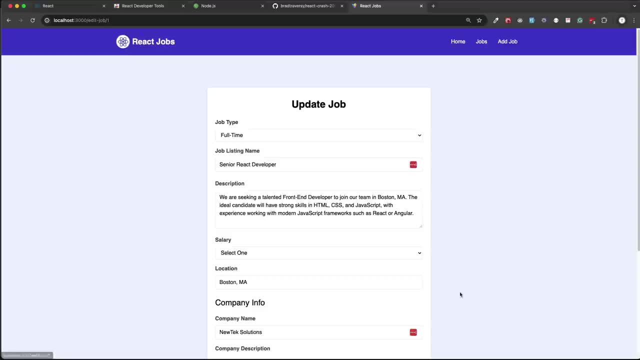 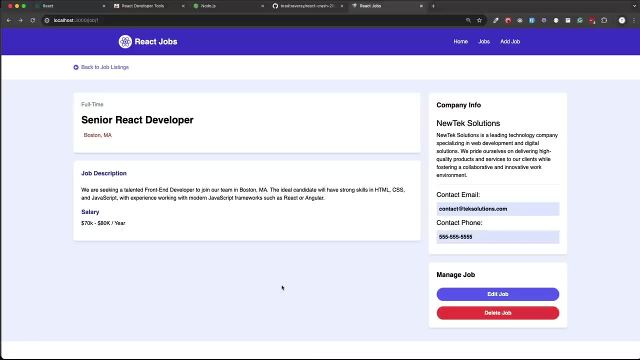 state, component state, And then, if you click read more, it'll take you to the page, the details page, all the info, the company info. there's buttons to edit and delete the jobs. Now, we're not going to get into authentication. That's something that would be separate from this crash course. I do have videos. 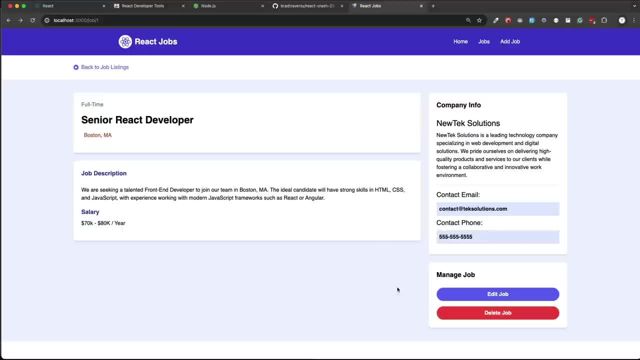 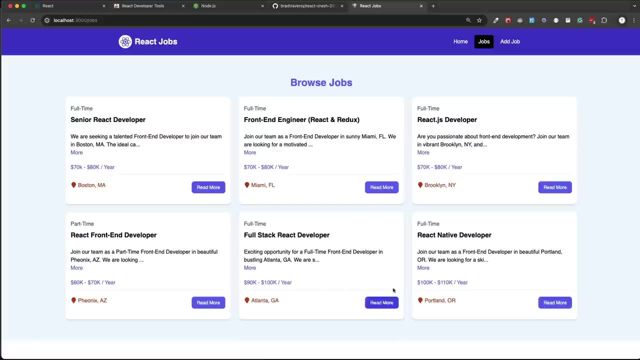 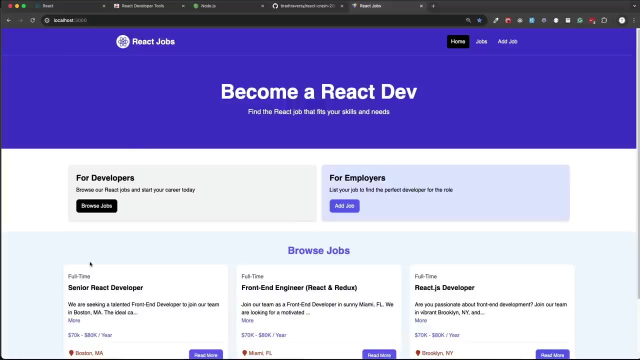 with all different types of authentication and react, but we'll have full CRUD functionality. We have our ad page here to add a job. We have our jobs page, which will show all the jobs, again having this little toggle here. So it's a pretty simple project, but I think that it's. it's a, it's a good. 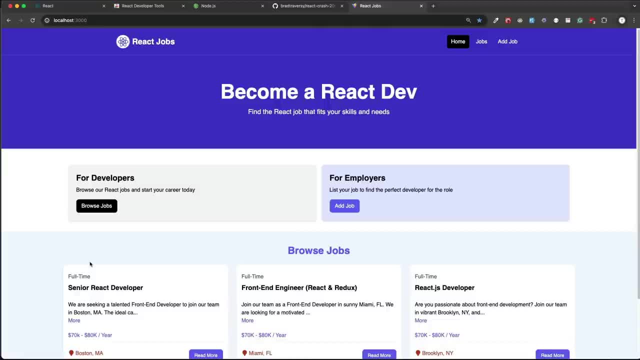 one to just kind of break you into react and how everything works as far as components, props, events, things like that. All right, So yeah, that's, we'll be building. the repository link will be in the description And, as far as what you need, you're just going to have to have no JS installed. 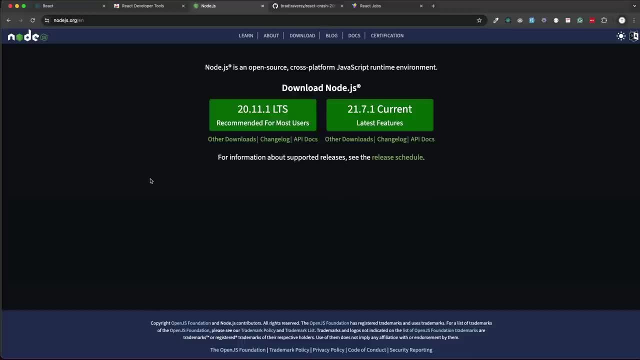 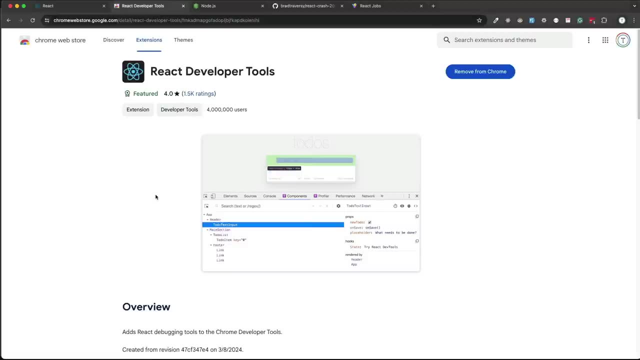 because we're using V and we're using the node package manager to set that up. So NPM comes with no JS, So just download that. if you don't already have it, I would suggest installing the react developer tools in your browser. We'll probably use those at some point, But if you're 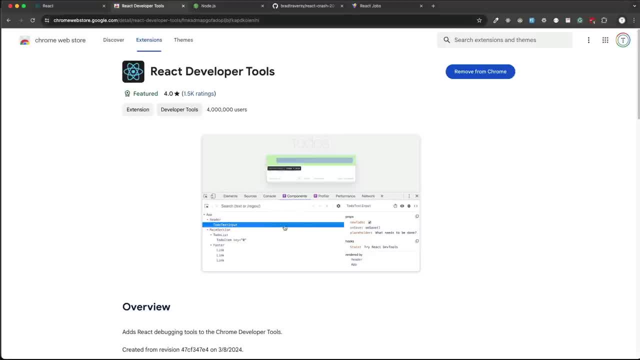 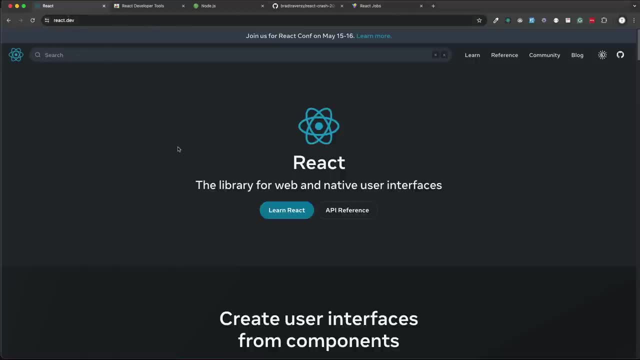 going to have to do that at some point. you can see the components through, you know, through your browser, and see any props and state and things like that, So it's helpful. And then react dot dev is the new react Web site and this is where you can find all the documentation, So you might want. 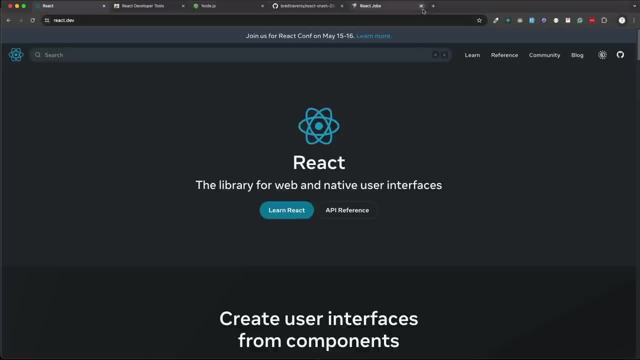 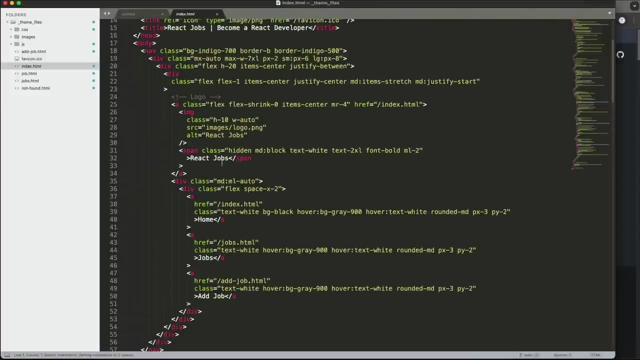 to just use that kind of as a supplement to the crash course. All right, So we can close this stuff up here. I'm just going to keep the reactive Web site open and I do have in sublime text. I have the theme files. We need to copy something from here, you know, to get the HTML and the classes. We'll go ahead. 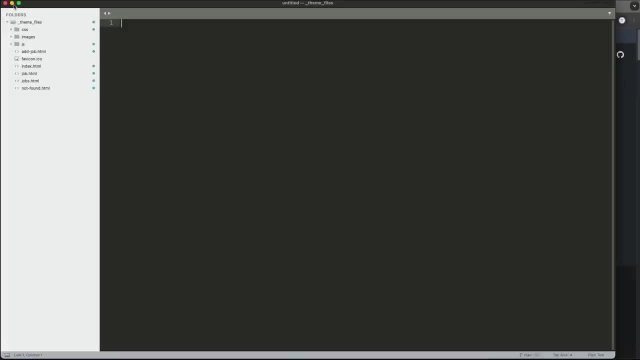 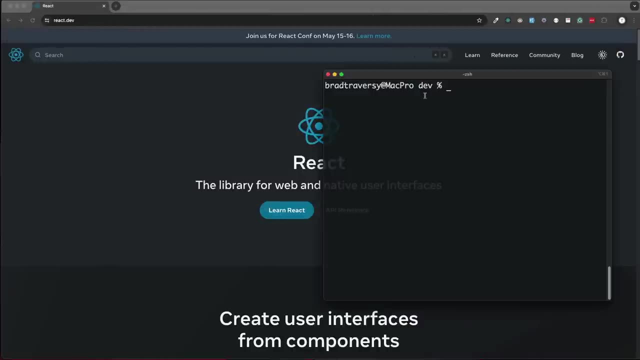 and just grab that. So maybe just open the theme files up somewhere. All right, So we're going to start off by opening the terminal and just go to wherever you want to create your project folder. I have a folder called Dev that I'm going to use, and then we're going to run NPM, create, again make. 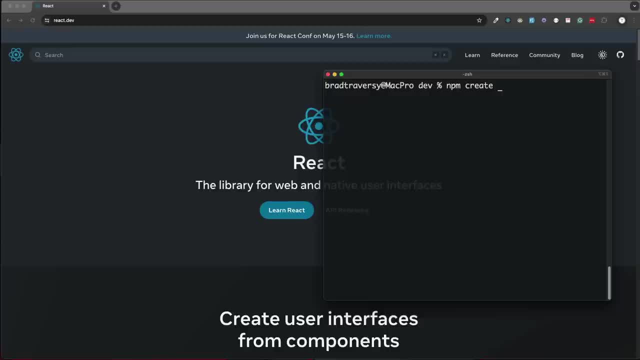 sure you have no JS installed, or NPM won't work. So we're going to say: create V at latest and then just whatever you want to call the folder. I'm going to call it react crash dash 2024, but you might want to call it like react jobs or something like that. I'm just naming it this for for you guys. 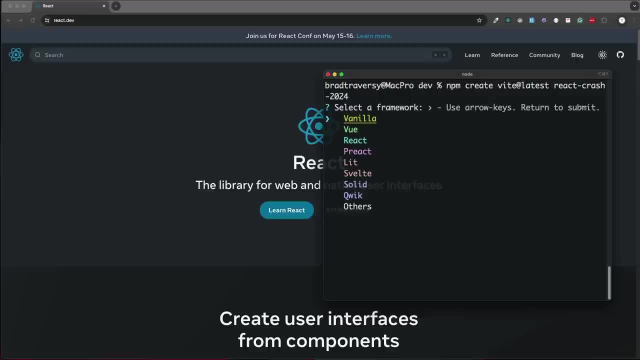 for the repo And then, as you can see, you can use vanilla, JavaScript, view, react and other frameworks. we're going to go ahead and choose react and you can choose to use TypeScript if you want. I'm going to go with just regular JavaScript and that's it. That creates basically a boilerplate app for us. 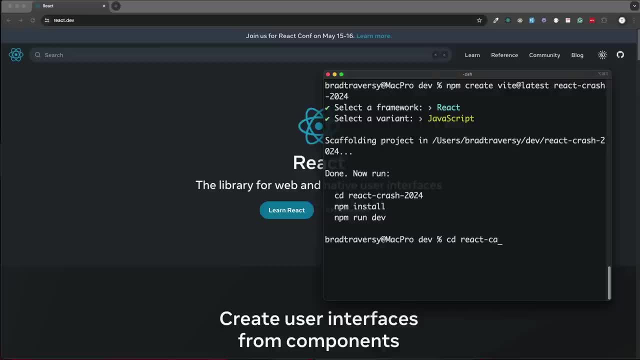 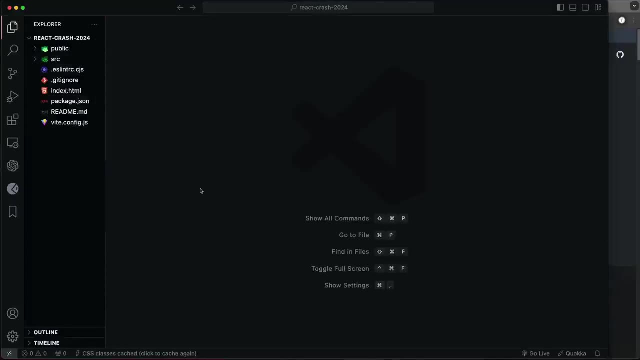 So we can see D into the that folder that we just created. And then from here I'm going to go ahead and open up Visual Studio code with code dot, And if you're using something else, that's fine. just you know, open. open the folder in your, in your text editor or ID. So let's just take a look at the file. 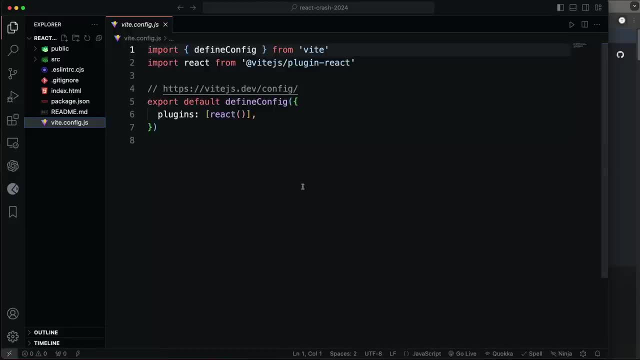 structure real quick. So there's a V config file and this is for any configurations for your dev. as you can see, we're bringing in the react plug in and using it here, passing it into this array. That's because we chose react when we were asked the questions. One thing I like to do is change. 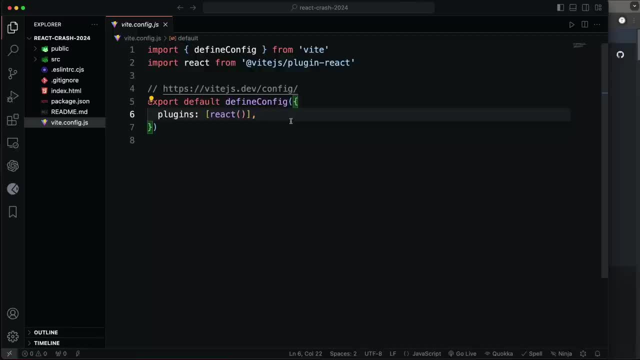 the port because by default it's. I believe it's five, one, seven, three. I prefer to use 3000 for front end stuff. So what we can do is add in a server object and then in that server object we can say port and then whatever you want. So I'm going to use three thousand. So now, if I open up, 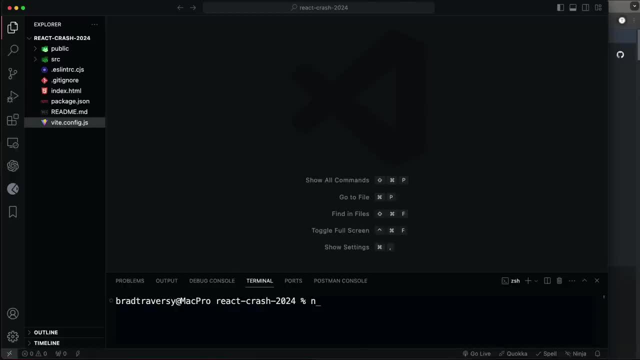 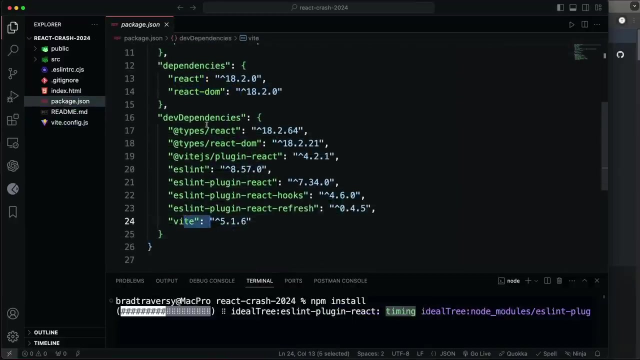 and open up my terminal within VS code, my integrated terminal, and run first of all NPM install because, as you can see, there is no node modules folder, So we need to install the dependencies which are react, react, Dom and Vite, And then we have some plug ins for ES lint as well as some types. 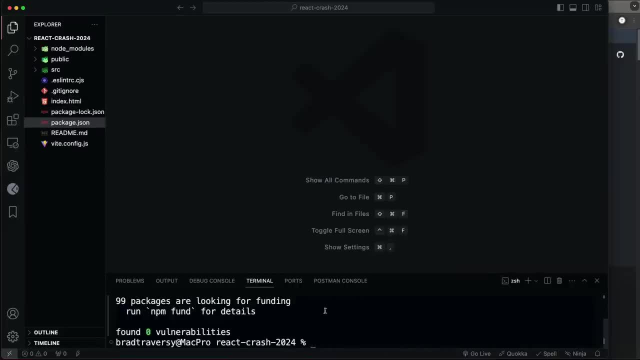 for TypeScript. All right. So once we do that, as you can see in the package, Jason, there's a dev script so we can run NPM, run dev, And for me it's going to open on three thousand because I change that value in. 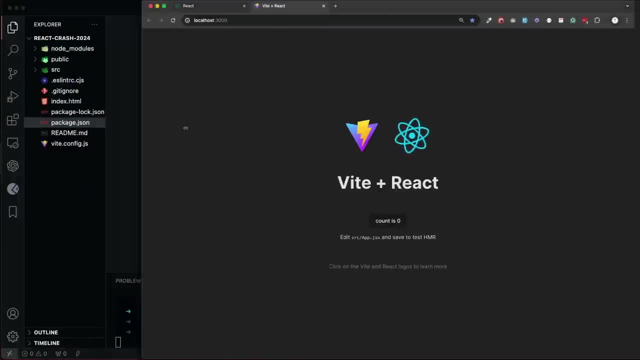 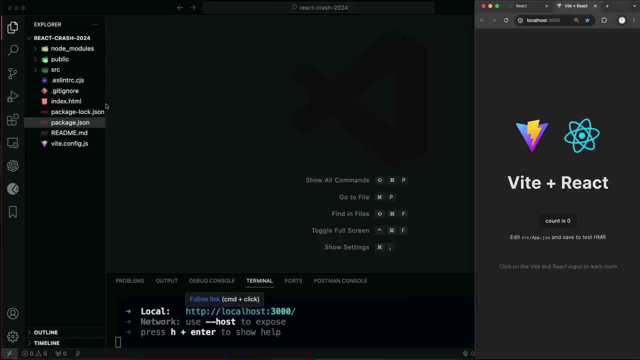 the config. So let's open that up and you should see a page like this, just a landing page, All right. So now we have the dev server running. Let's just talk about the structure here for a minute. So the index HTML: remember, this is a single page application and this file is the. 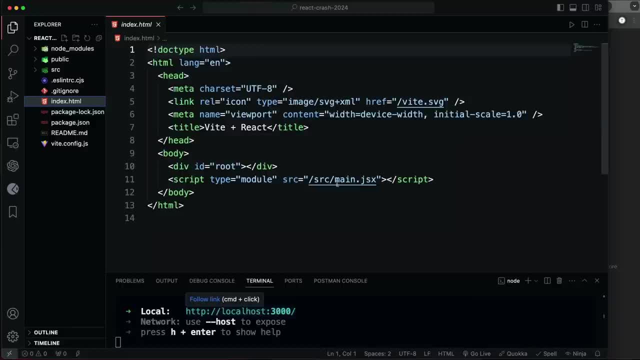 single page, because this loads in the browser and then everything else loads through JavaScript And, as you can see, here we're actually including the main dot JSX file in the source folder, including that as a module, which is really cool. It's different than how you know. 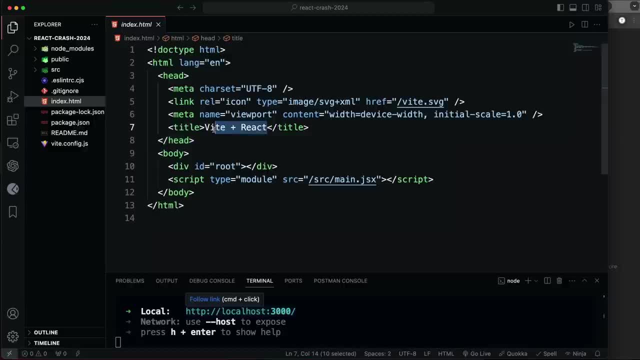 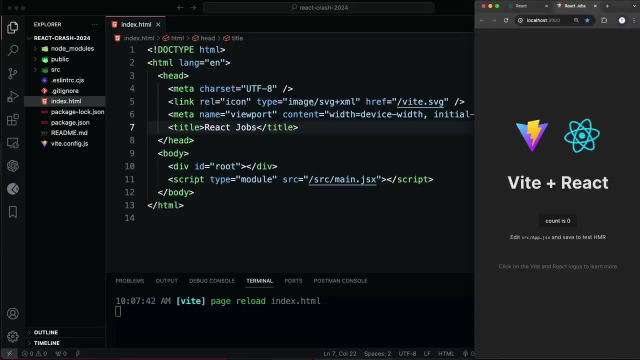 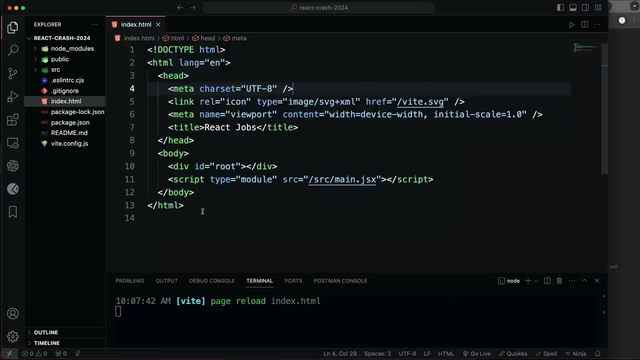 create react app works with Web pack. So here I'm just going to change the title to react jobs, and that should change. as soon as I save it, You can see up here and then the way that this works. if you're not familiar with front end frameworks, they all pretty much do this: cut the same type. 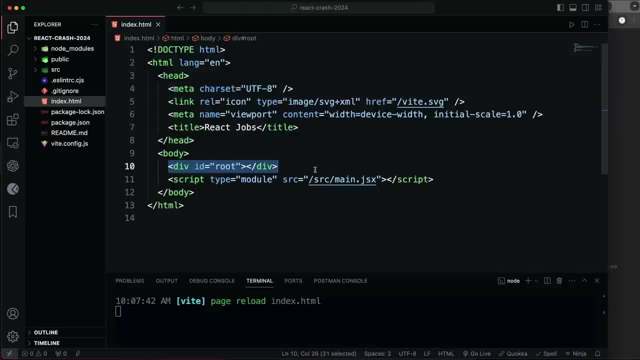 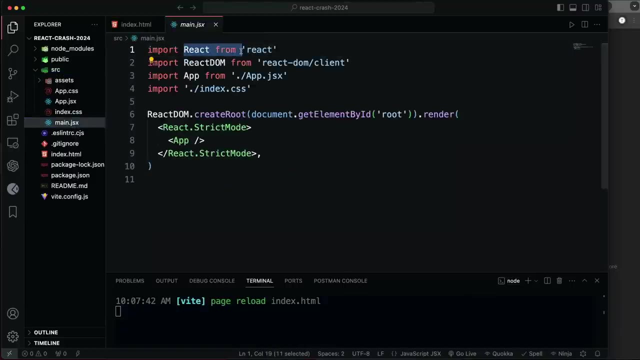 thing. We have a div, or I should say, single page applications do the same thing. There's a div and it has an idea of root. If we go into the source folder, this is our, our react application, and the entry point is this main dot JSX file. And here we're bringing in react, react Dom, which is the 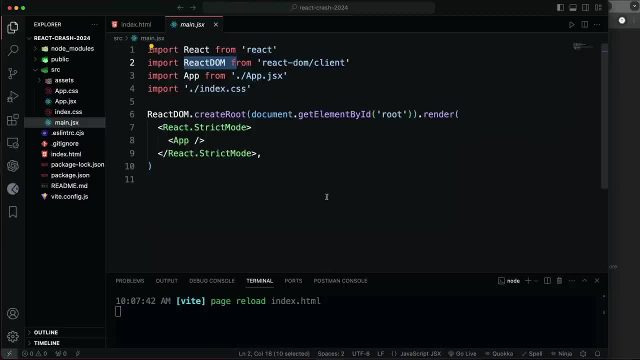 library that allows it to work with the document object model of the browser And then on that react Dom object. we have a create root and that gets passed in An element and, as you can see, we're, we're selecting that root element by ID and then we're. 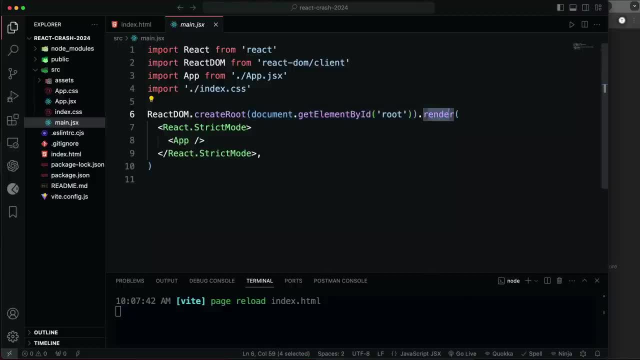 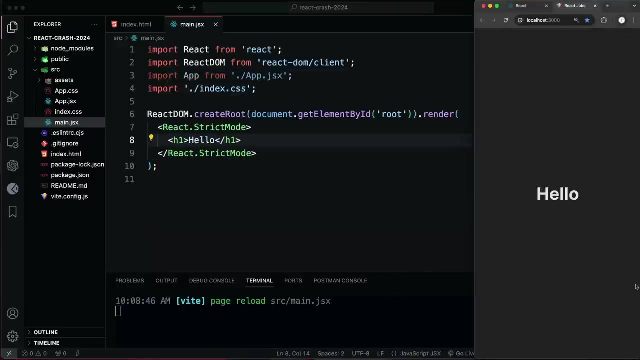 calling this render method and you can render whatever you want as your application. In this case, we have this app component, which comes from this app dot JSX file. Now I could change this to anything I want if I put an H1 here and say hello and I save that. As you can see, that's what's. 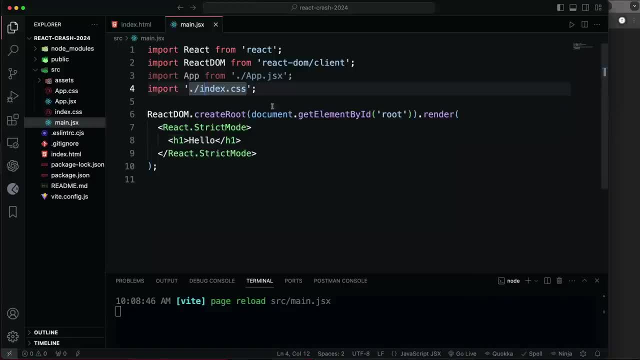 rendering as my application and it's styled because of this Index dot CSS. So I want to just clean this up a bit. I'm just going to undo that and put the app back, And then you also have this strict mode, which is a wrapper component that'll check for. 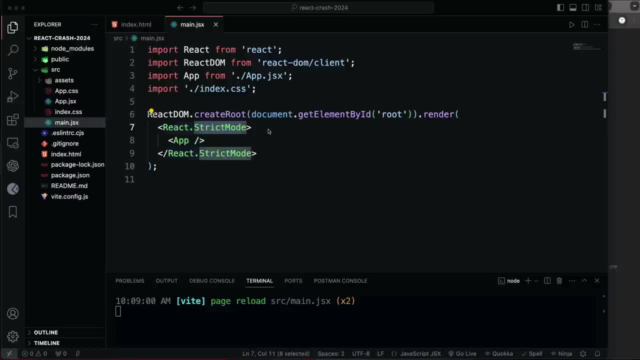 potential problems in your app. So it'll check for things like deprecated and unsafe lifecycle methods, legacy context, API usage, things like that. So what I want to do is is a little bit of cleanup. So, as far as the CSS, you can see, it comes with two CSS. 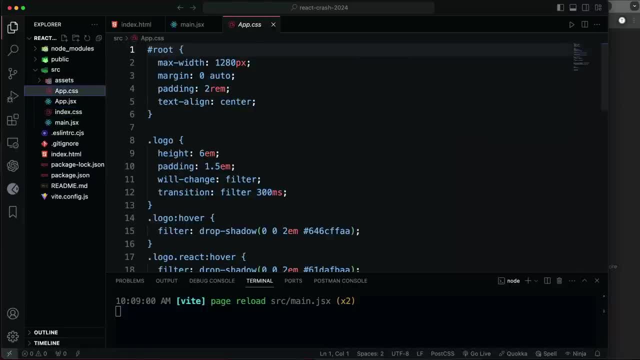 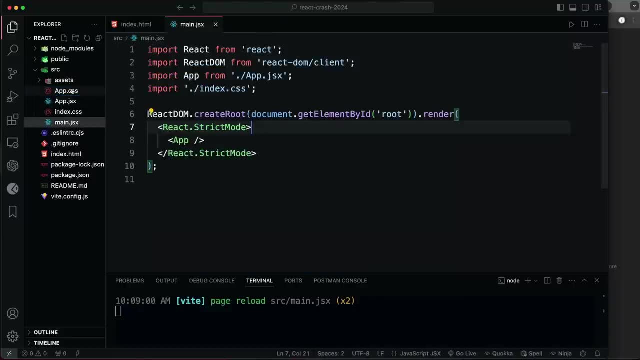 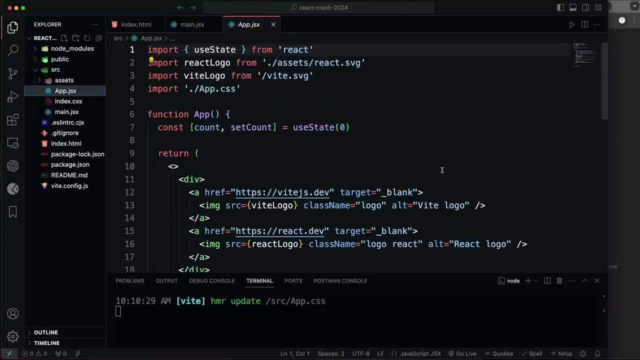 files: index dot CSS and app dot CSS. We're going to be using tailwind, So we need to install that and set it up. I'm just going to keep the index CSS, So let's delete the app CSS and the app dot. JSX is our main component And basically this is all the stuff you see right now on the home page. 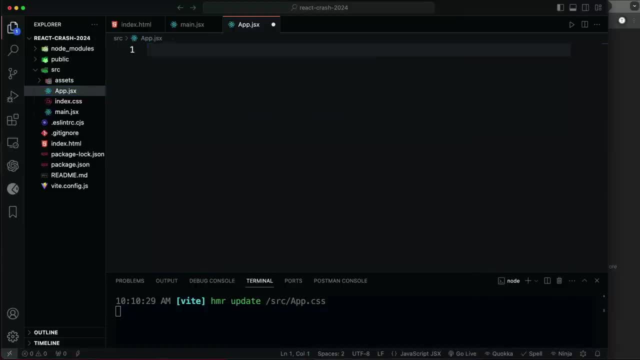 So what I'm going to do is completely wipe that away and just create basically an empty component. Now, components can their functions, So you can do a regular function- So, for instance, we could do function app- or you can do an arrow function, So a const app, and then use an arrow and you can type it out if you want. But I would 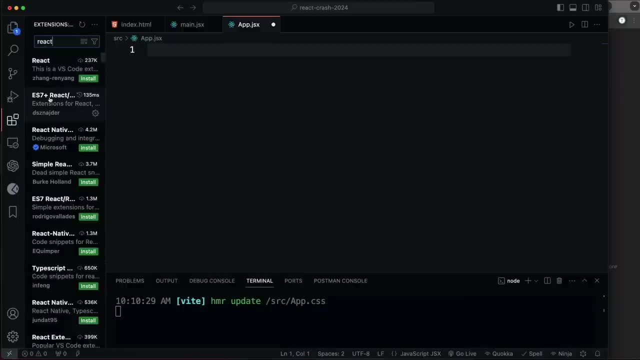 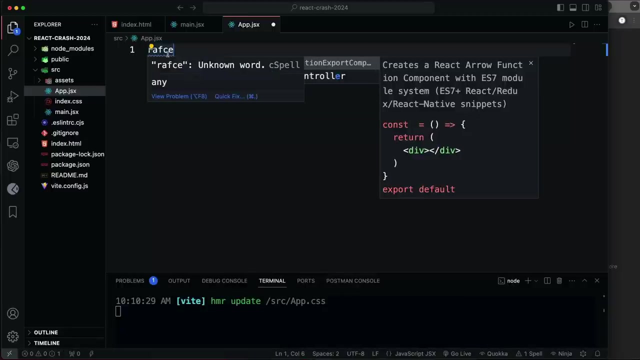 suggest using this extension here. This is called ES7, react redux, react native snippets, And this gives you easy snippets that you can use to generate components. So what I like to do is r, a, f, c, e, which is react arrow function component, and then 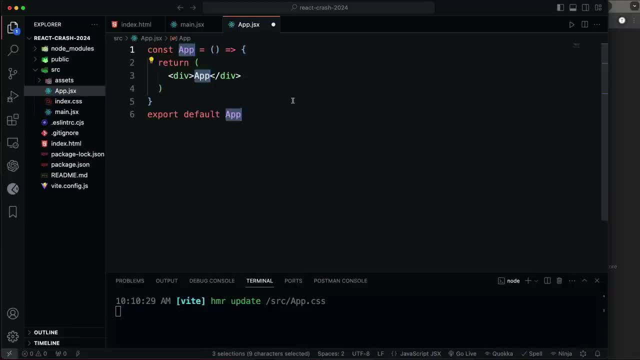 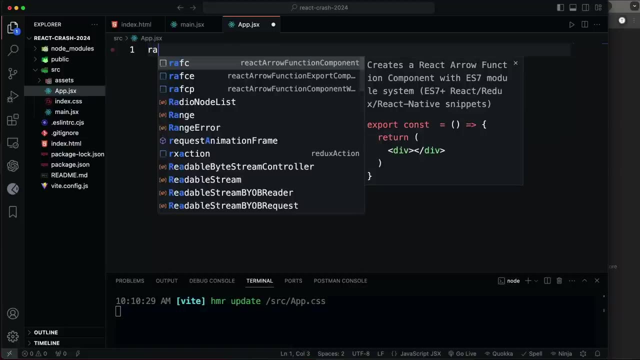 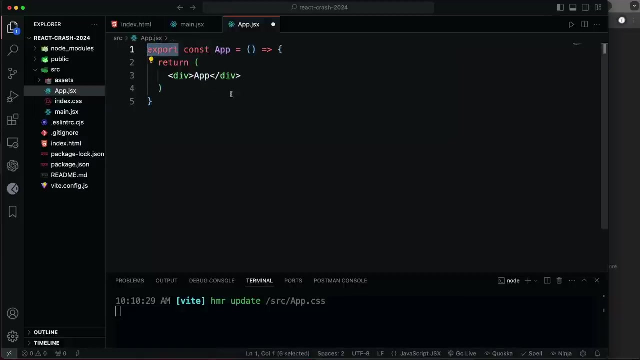 export, which will be at the bottom. So you see, if I hit tab or enter, it gives me an arrow function and has the export at the bottom. Now there's other snippets like r, a. if we do r a, f, c, it does do an arrow function. That's what the a is, But the export is here as opposed to the bottom, And 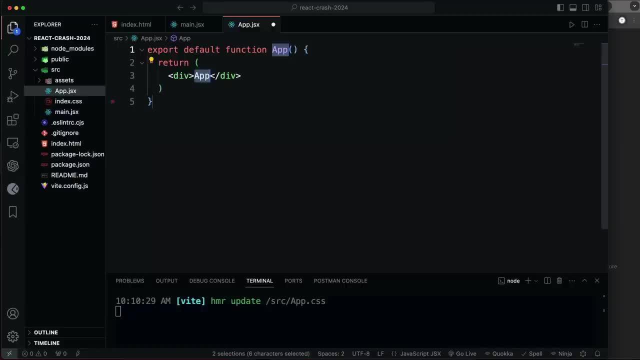 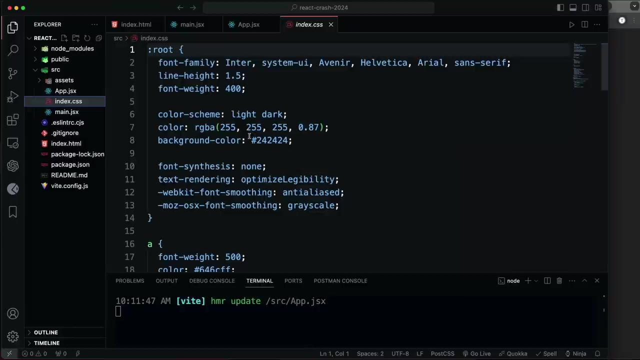 then for the regular function, I believe is r, f, c. So now you can see it's using the regular function syntax, So you can use any of these, but I'll be doing r, a, f, c, e. So if I save that now, we should just see app. Now I want to get rid of all the CSS And, as you can, 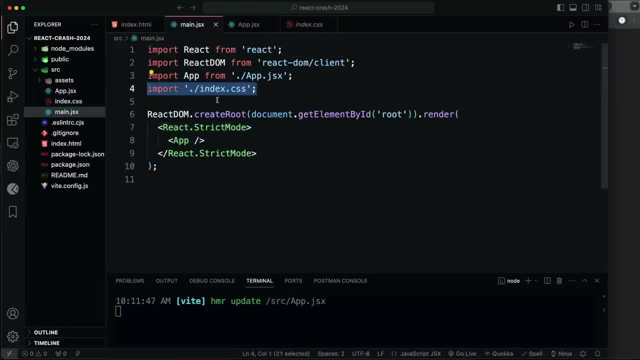 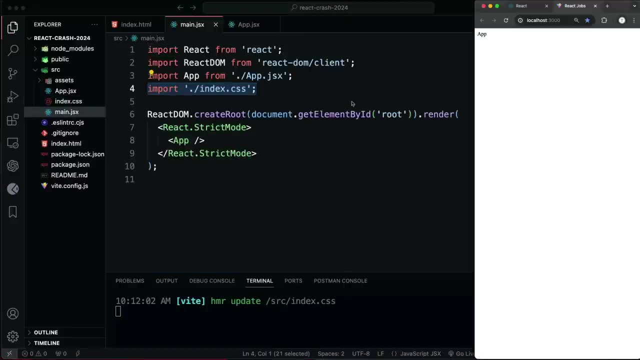 see in the main, dot j s x. it is including the CSS file and I'm going to keep that, But let's just get rid of everything in that file for now. OK, So now we just have just an unstyled website, So yeah, 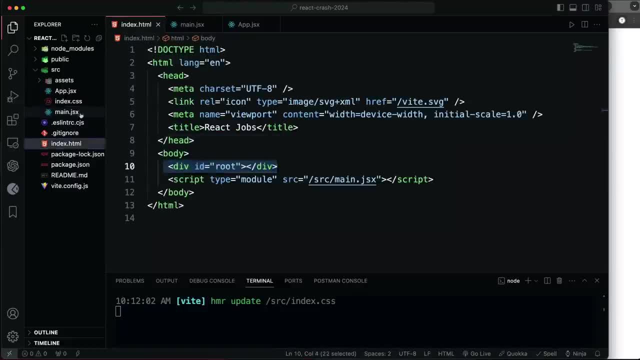 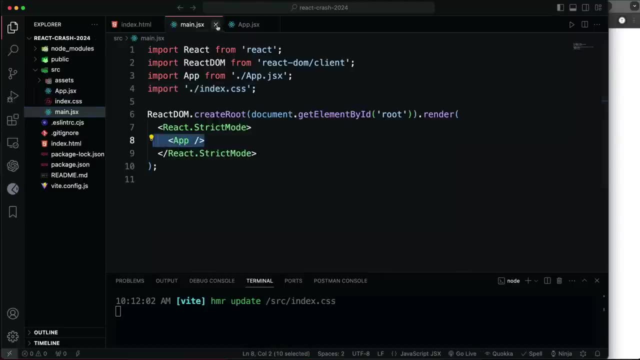 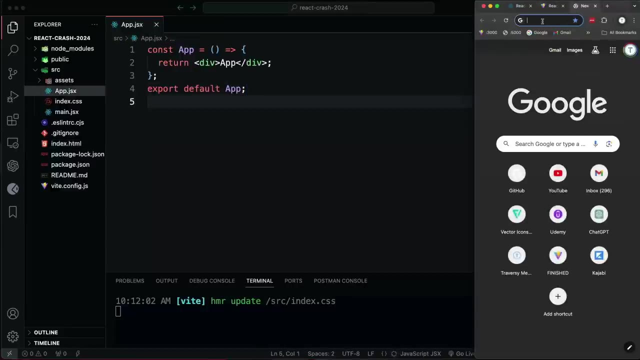 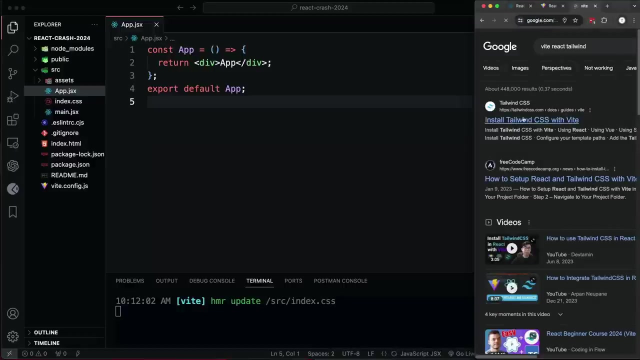 that's pretty much how this works. We have this div with the idea of root and then we're inserting our app into that using this render method. All right, Now let's let's get tailwind set up, And there's some steps we can follow. if you just Google, let's say, Viet Viet react, tailwind. So right here. 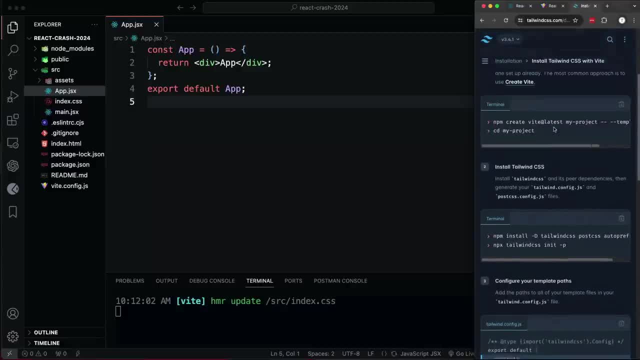 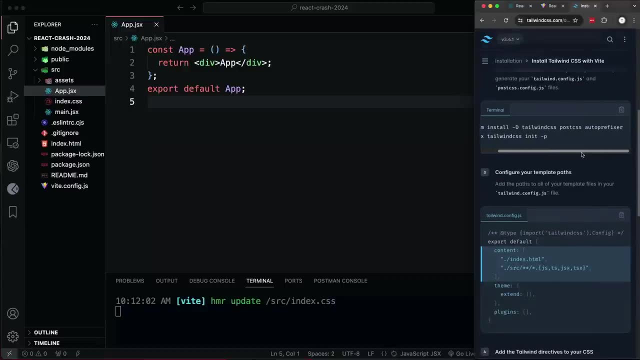 install tailwind CSS with Viet. So basically, we need to install. Let's see, we already did this, created the Viet projects. Now we just need to install tailwind Post CSS and auto prefixer. So I'm just going to grab that And then I'm going to open up a new. 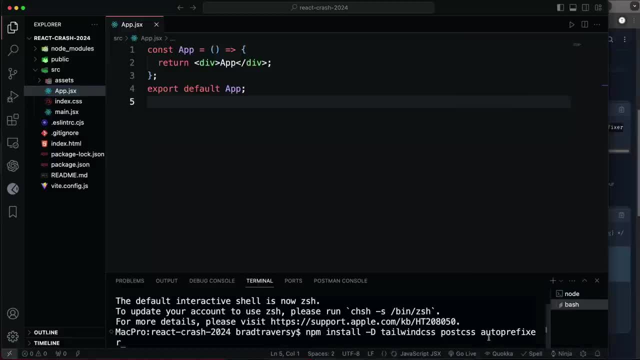 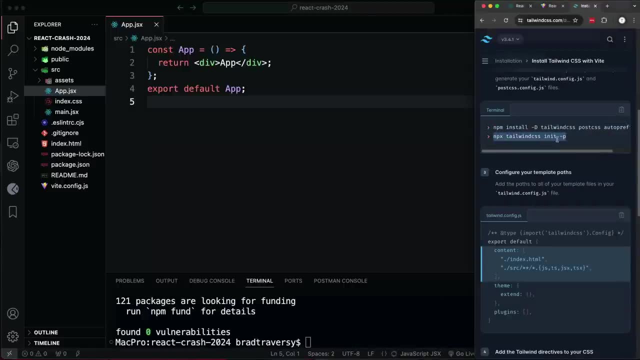 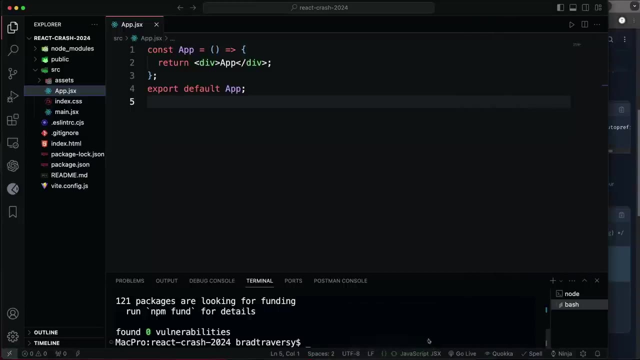 console. I'm going to just let that one run the server And we'll go ahead and run that. And then we want to initialize tailwind with dash p. So this: this will create a tailwind config file and the dash p will create a post CSS config file. So let's go ahead and run that. And now you can see. 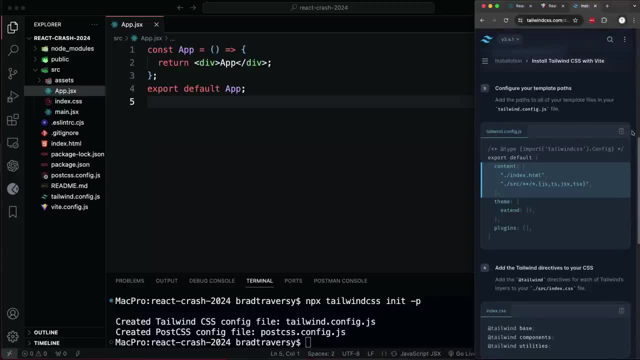 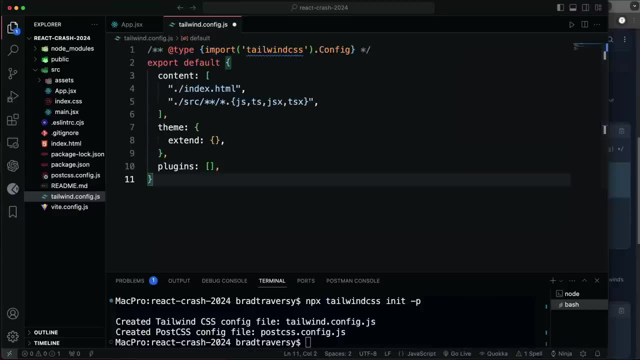 then the tailwind config. we want to have this, So I'm just going to copy that whole thing, go to tailwind config and just paste that in, All right, So basically it's going to watch anything that has a JSTS, JSX or TSS extension. It's going to look for tailwind classes in any of those files in the 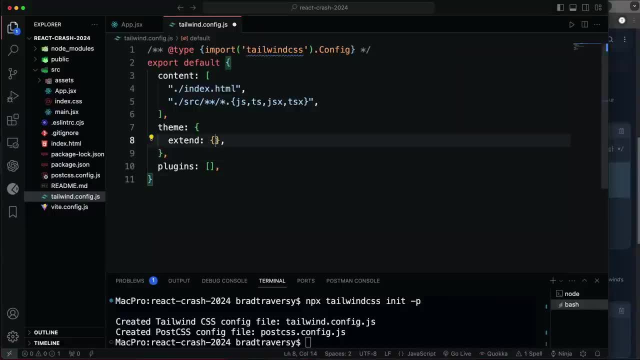 source folder. Now there is a couple of things I want to add here. So in extend I'm going to say font family and I want to use the Roboto font, So I'm going to say sans, and then in an array we can pass in Roboto or whatever font you want to use. 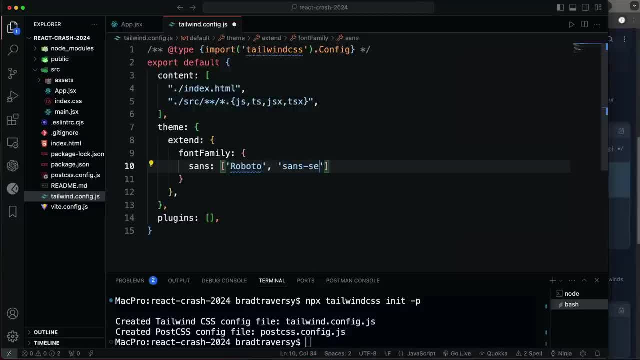 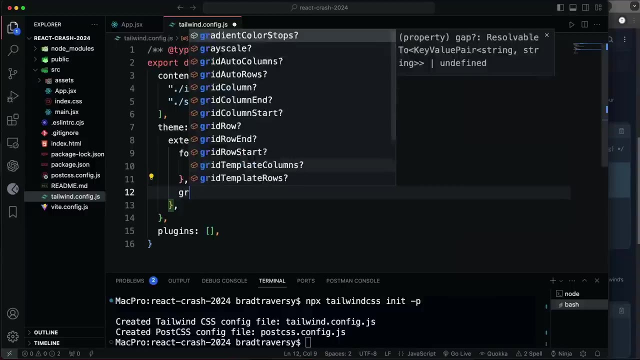 and then sans serif, So it just allows you to pass in a font stack. And then also, I want to have a certain grid class for the details page. that's 70- 30. Basically, the left column will be 70, the right will be 30. So I'm going to say grid, grid, template columns. 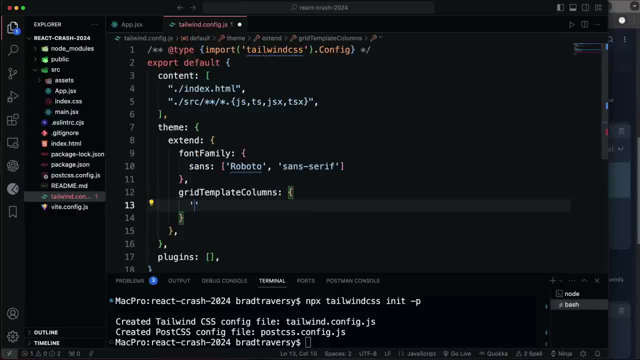 And then we're going to just pass in here a string and say 70 dash 30. So that'll be the class. And then we want here 70 percent space and then 28 percent. We'll leave a little bit of room there. 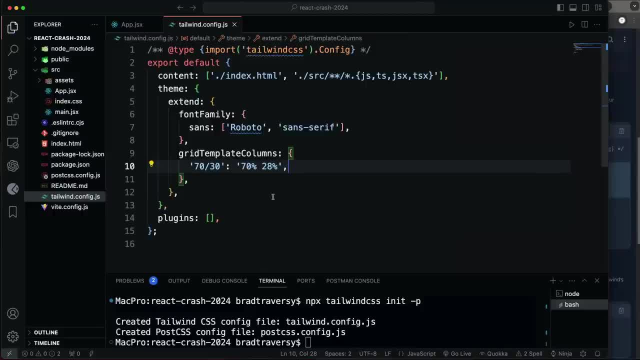 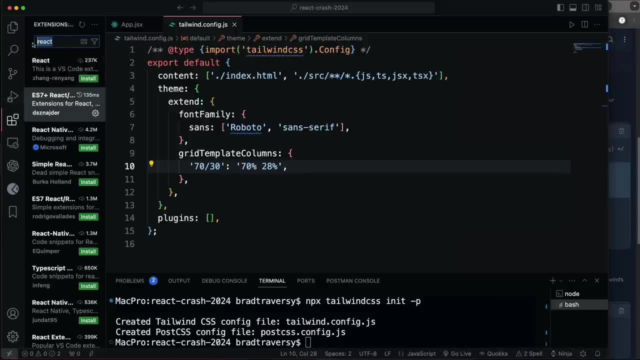 OK, So that's going to allow us to add a class later on that we need. Now my spell check is showing these blue squiggly lines, So I'm just going to disable that extension. OK, So that's going to allow us to add a class later on that we need. Now my spell check is showing these blue squiggly lines, So I'm just going to disable that extension. 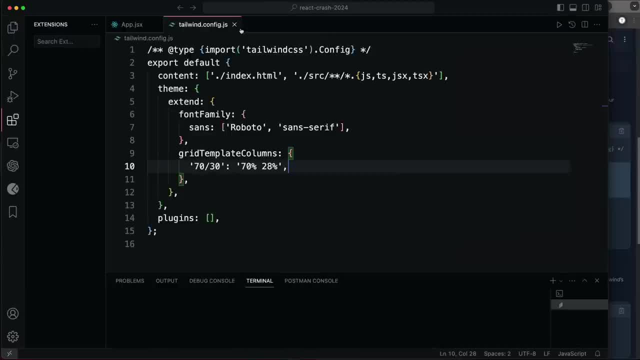 OK, So that's going to allow us to add a class later on that we need. Now my spell check is showing these blue squiggly lines, So I'm just going to disable that extension Just to get rid of those, because that could be a little confusing. 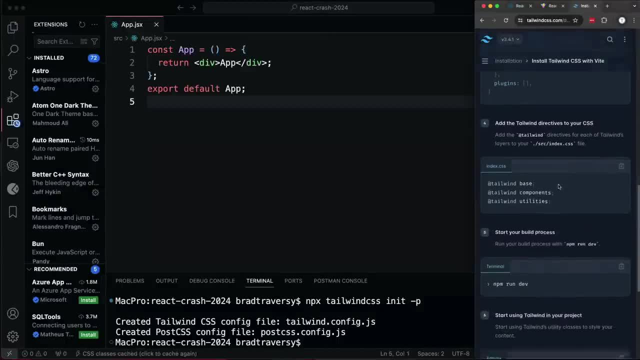 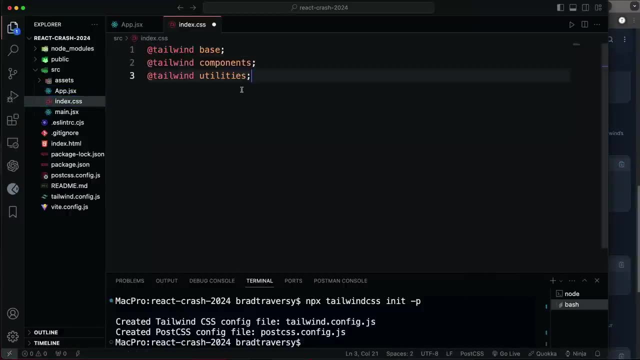 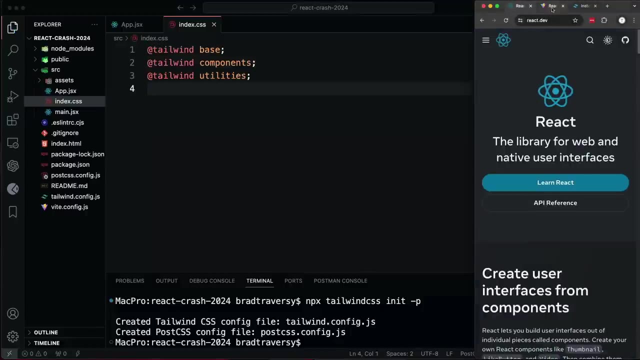 OK, So that's the tailwind config. Now we just need to go to our index CSS and add these three lines which is going to load tailwind. So right here, index CSS, add those, save it and then we should be all set. So if we go back to our application should see you might have to reload. 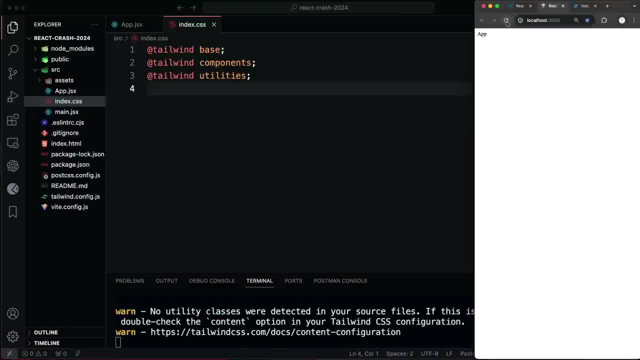 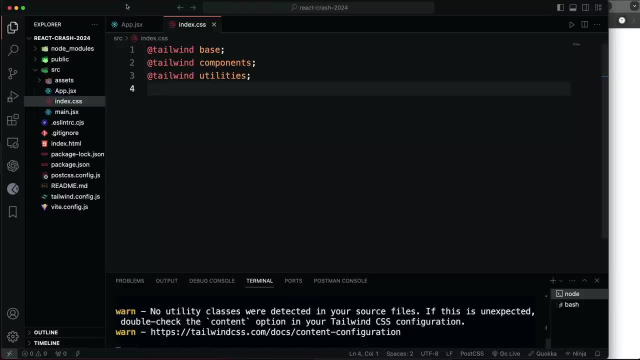 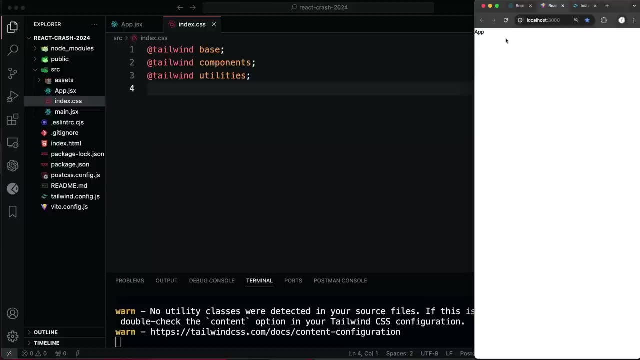 Let's just stop the server and run it again. Let's just stop the server and run it again. The utility classes were detected. Oh, we don't have any tailwind classes, but that's the only reason it's saying this. But you can see the font has changed and there's no margin or padding, so tailwind is being included. 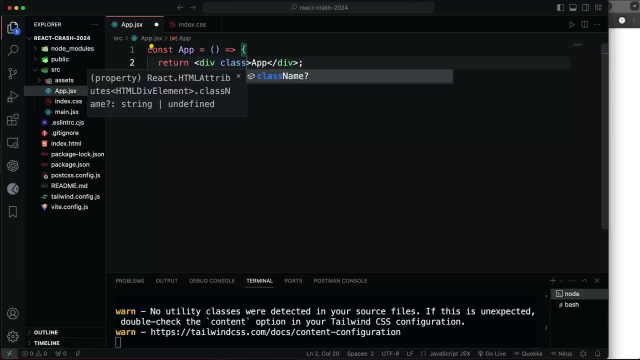 In fact we can go to our app component. In fact we can go to our app component And remember, with JSX we can't use class, we use CLASS name. So let's say CLASS name and we'll do text dash 5XL, 767, 00etta. això las unsungas. 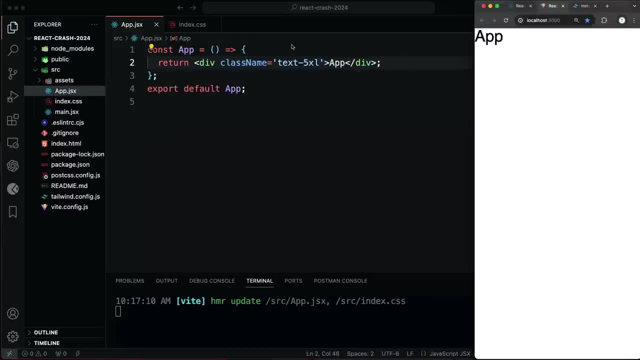 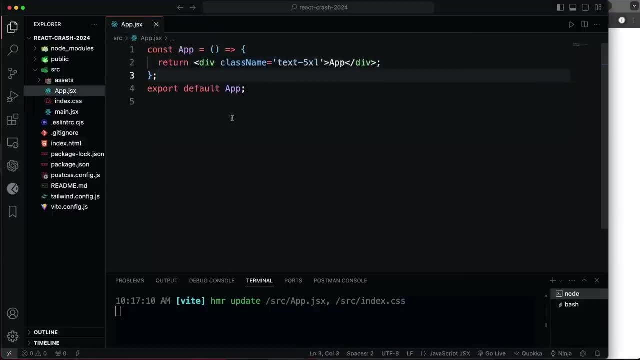 class, And there we go. So Tailwind is now working. So let's close that up And I'll just put this here. close that, All right. So we're going to talk a little bit about JSX. So every React component is going to return JSX. That's what. this is right here, which is an 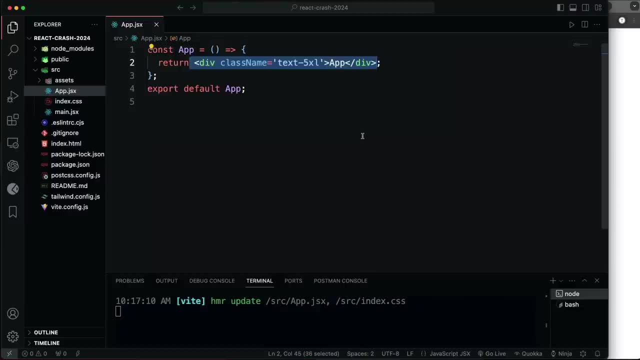 HTML-like syntax And I'm going to give you some examples of some things you can do here because it is dynamic. But one rule that you have to remember is that you can only return a single element. You can have as much stuff in that element as you want, like inside this div. 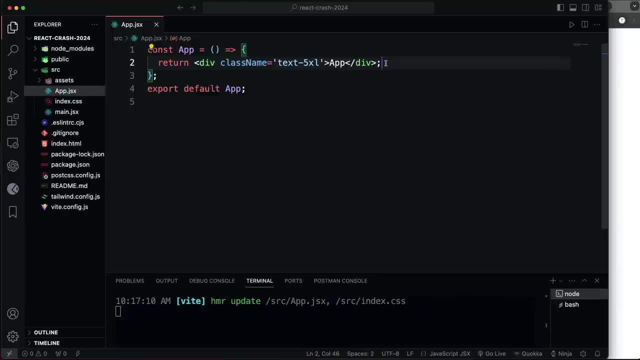 but it can only return one. So if I try to, for instance- and you can put parentheses around this as well, Oops, Parentheses, and put it on multiple lines, But if I were to add a paragraph here like that, you'll see I'm already getting an error in VS Code. It says JSX expressions. 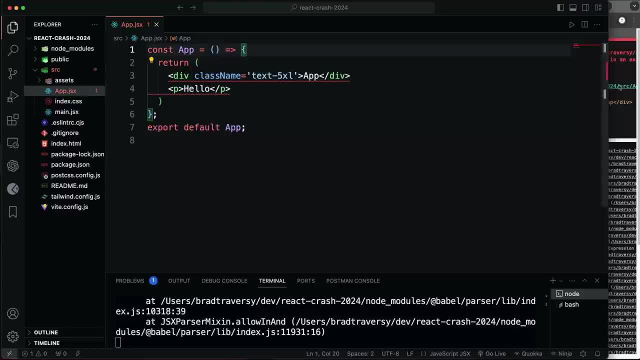 must have one parent element. So if I were to add a paragraph here like that, you'll see I'm returning a div and a paragraph. Now, if I wanted this div and this paragraph, then I could simply wrap it in a single element. So I could say: div- Oops, I hate when it does this. So I could say: 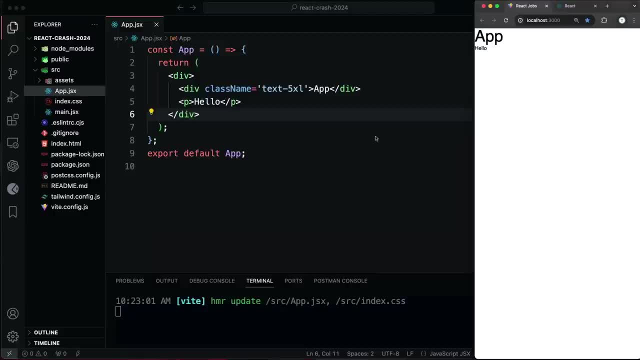 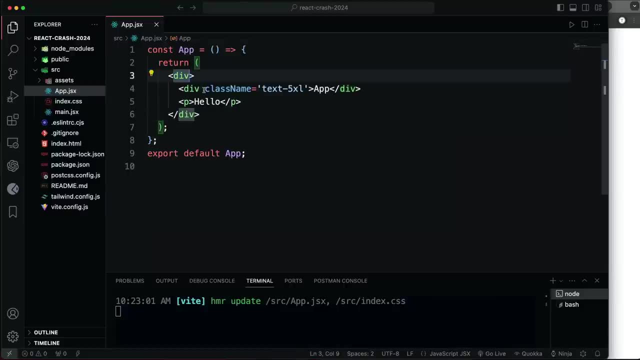 div and then end that here, And that's absolutely fine. Okay, So just remember that it has to be wrapped in a single element. Now, you might not want an actual div here, So what you can do is use what's called a fragment, and it's just an empty HTML tag, So just like this. So if I do that, 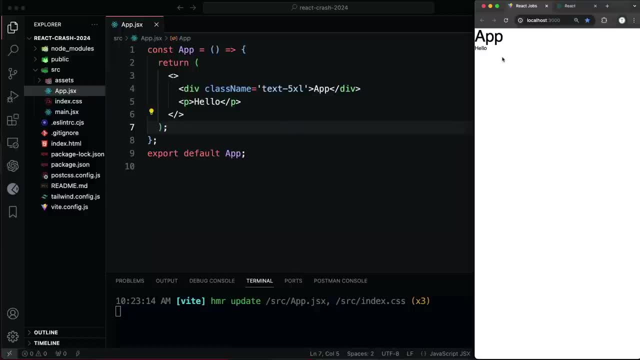 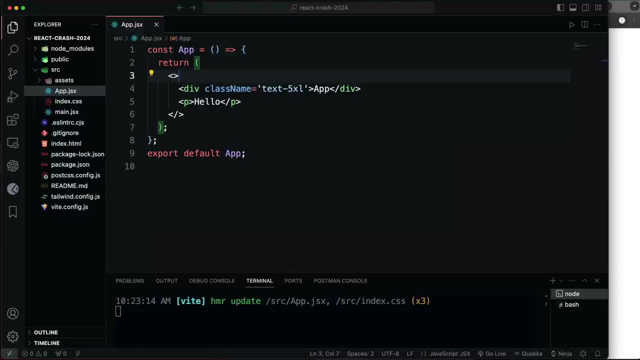 you can see that still works. but now it doesn't have a surrounding div in the actual DOM. All right, So just remember that. Now, to give you kind of a little JSX crash course, let's say we want to put a dynamic variable here, So above the return I can just write JavaScript. 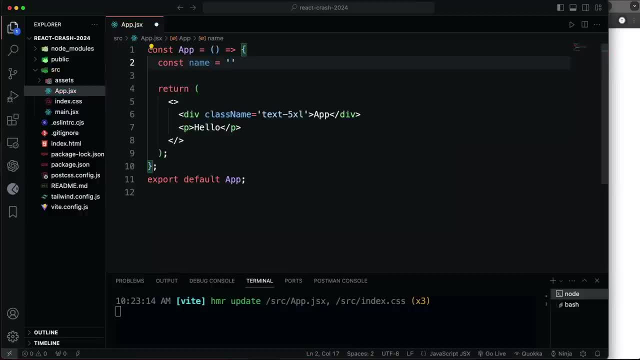 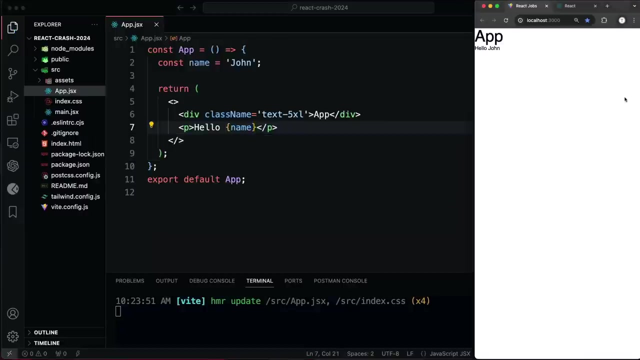 So, for instance, I'll create a variable called name And this isn't part of the project, It's just to Give you some examples. So we'll do name And then I can put that value anywhere within my JSX, wrapped in curly braces. So I could say hello and then curly braces, name, And you see I get. 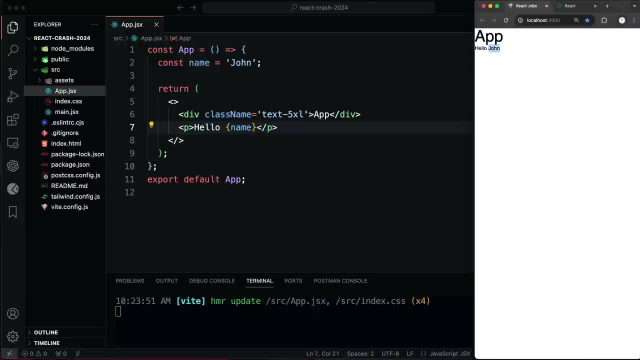 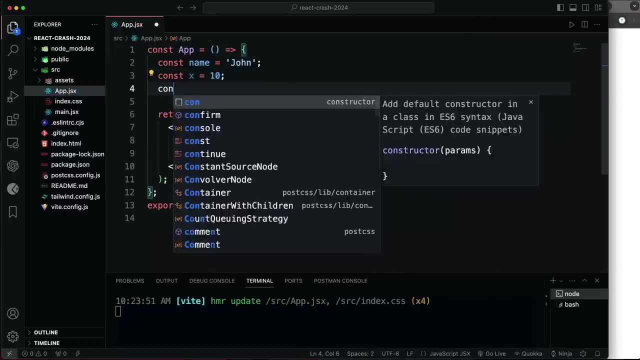 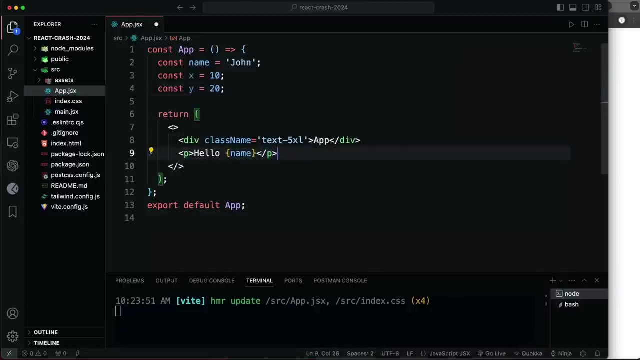 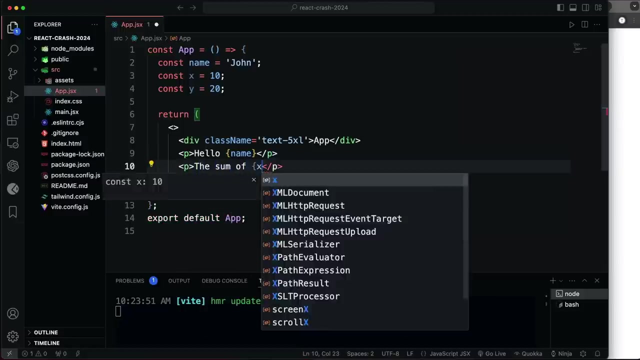 hello John. And it doesn't have to be just a single variable, It could be an expression. So, for example, I could say: const x equals 10 and const y equals 20.. And then I could say: let's go under that. We'll put another paragraph and I'll say the sum of and we'll put in x and y. 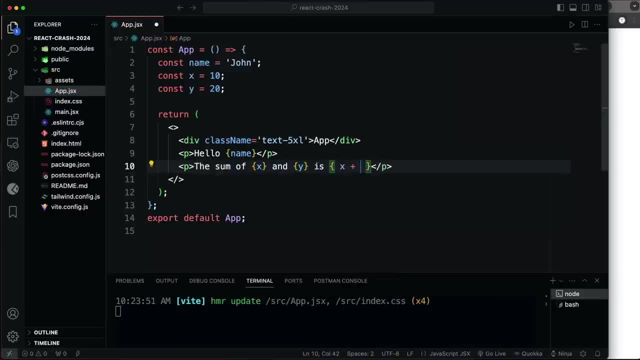 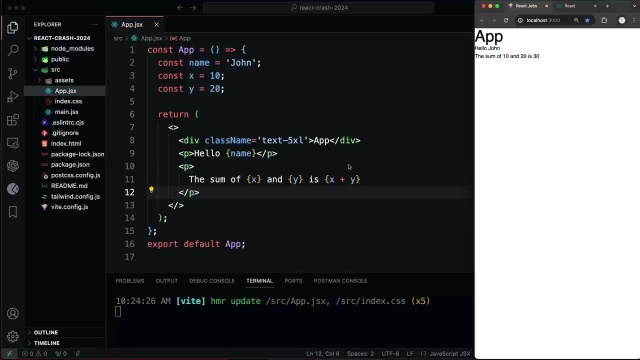 is, and then I could do an expression. I could say x plus y, And if I save that I get the sum of 10 and 20 is 30. So basically you could put whatever you want in these curly braces. Now we can also. 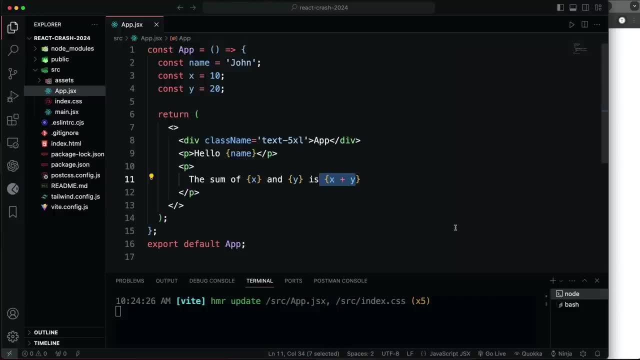 use loops and we can render There's something called a list. So let's add up here, let's say const names, and say: and we'll make this an array and we'll just put some names in here, So Brad, Mary, Joe and Sarah, So we get. 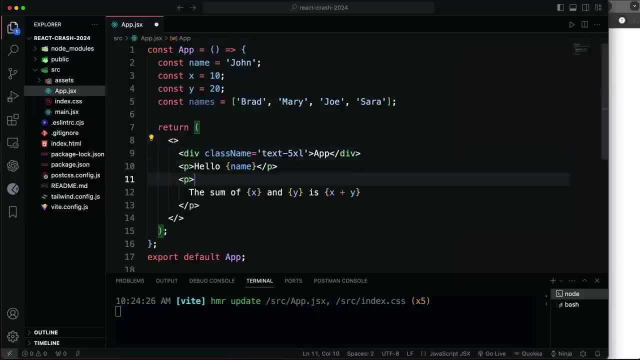 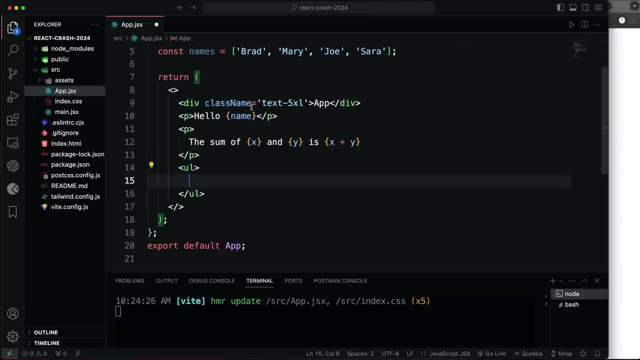 some names And let's say, I want to loop over these and output them in the browser So we can create a list by. Let's put this in a UL, And it doesn't have to be a UL, It could be anything. 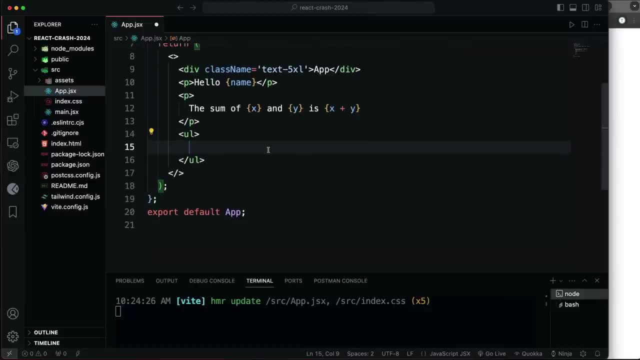 But I basically want to. I want a list item that has these names inside. So what we can do is open up some curly braces, take our names array and then we use map, which is just the vanilla JavaScript high-order array method That. 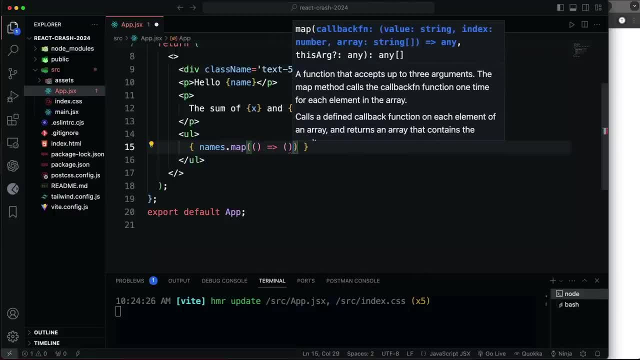 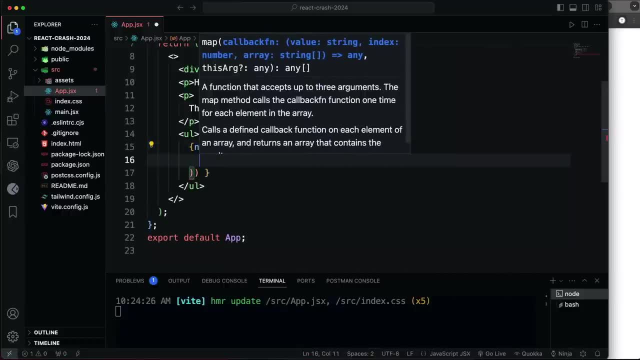 takes in a function, but we're going to return some JSX for each one, So we'll say map and then name, And then in here we can have whatever we'd like. I'm going to use a list item and then we should. 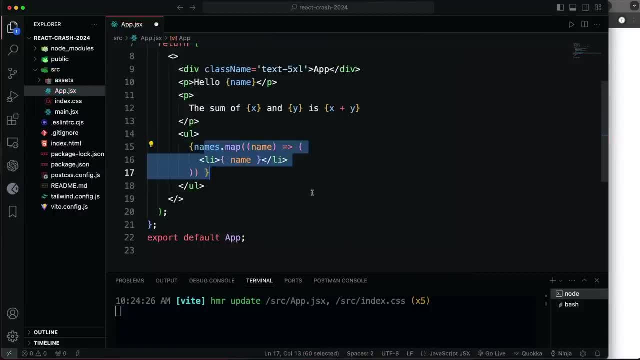 have access to each name, So this creates what we call a list. If we check it out now, you'll see the names are all on a list. All right. Now, if I open up my console, we're going to see an error or a warning. 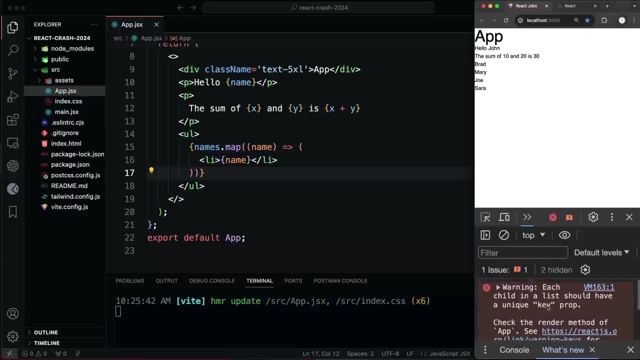 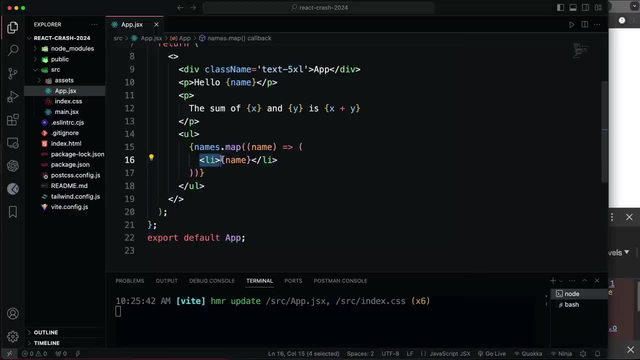 And let's see It says- Let me just reload this: Okay. So it says each child in a list should have a unique key prop. So when you create a list, whatever this element is inside the map has to have a unique key prop. So we'll say key. 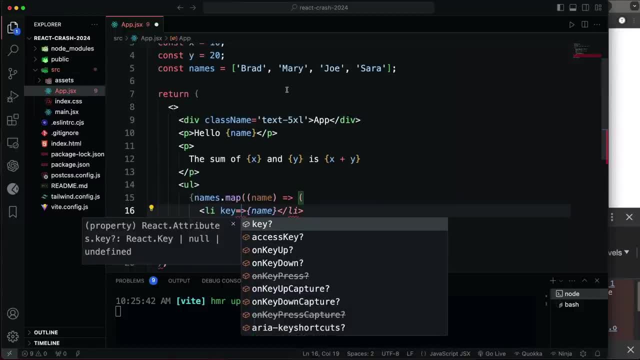 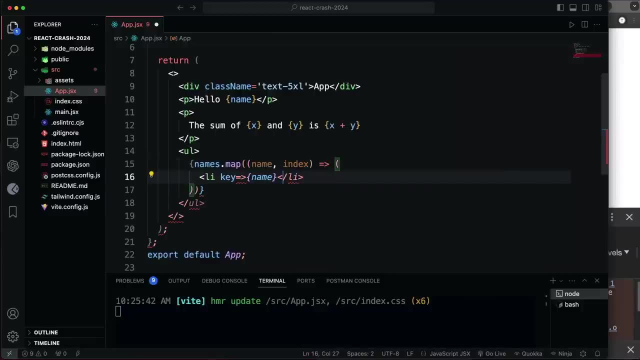 if we had an ID in this array, like if it was objects with IDs, we could use that. But since we don't, what we can do is get the index by passing in a second argument here, And then for the key we'll say: that's going to equal, And if you're going to set this to something dynamic, 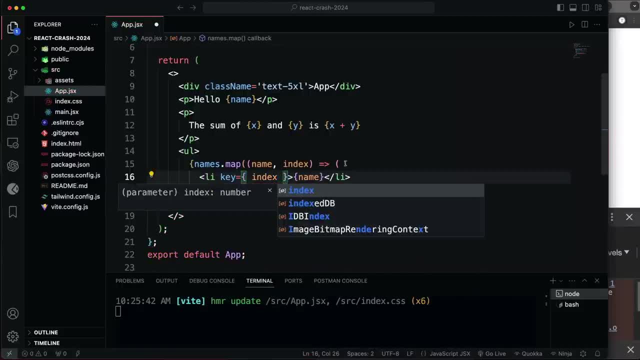 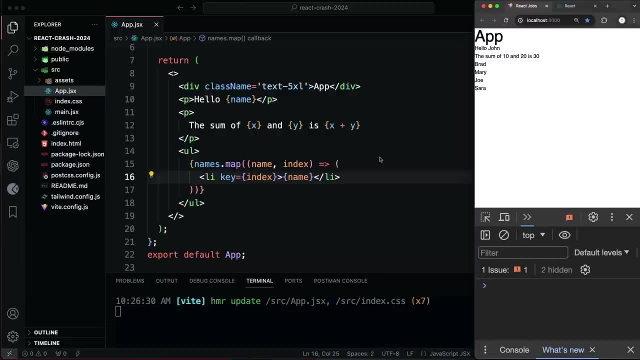 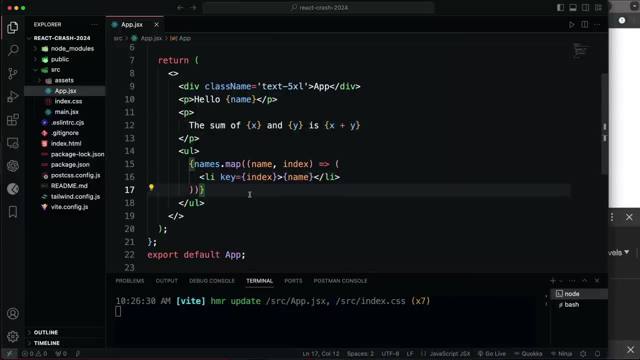 then you use curly braces So we'll say key equals index And then if we reload that, that error goes away. So that's a list. Now we can also use conditionals within JSX. Now I can't. I can't use like an if statement in here in in curly braces, like I can't do this. 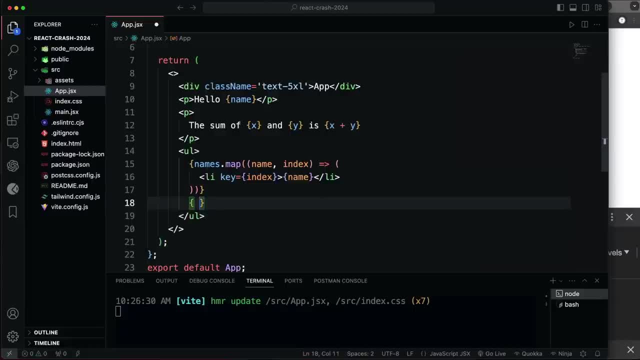 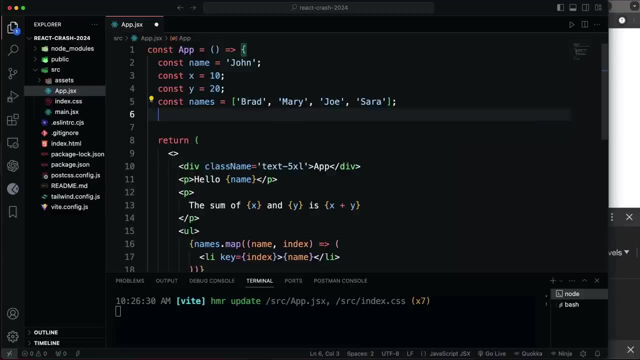 if something, because it has to be basically a one line expression. One thing you could do is you could have different returns. So let's say we have, let's say, logged in and set that to true right, And then you might do something like if logged in. So I'm doing this. 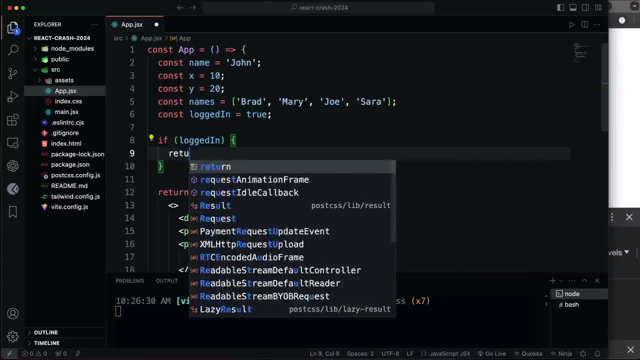 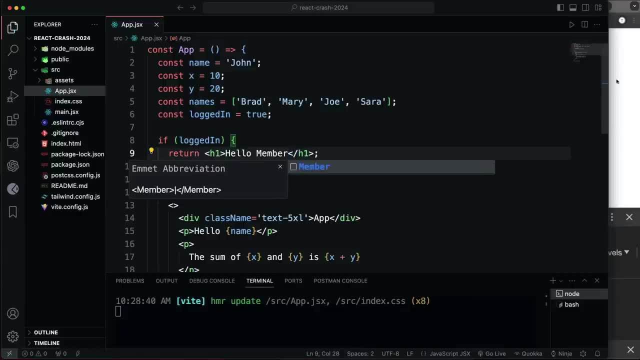 above the return. So if logged in then I could return. I don't know. we'll just say h1, and then hello member. So if I did that then I see hello member and none of this is going to render. But 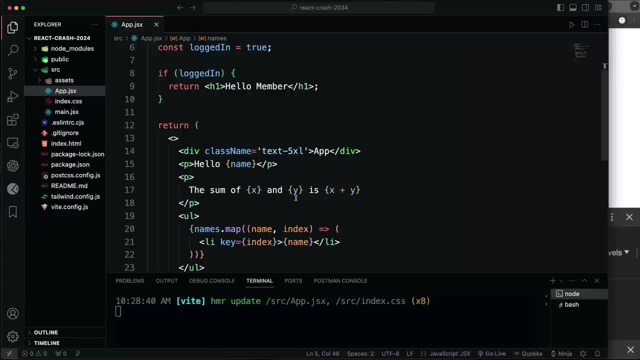 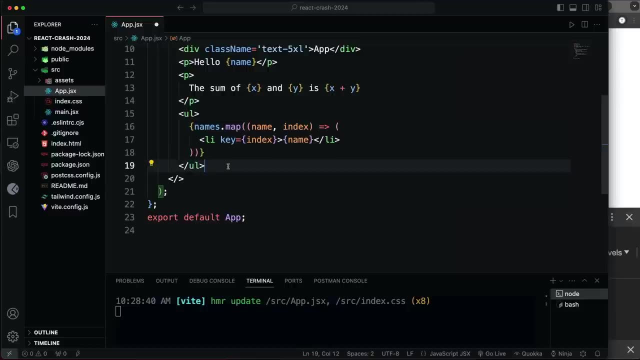 usually you're going to want to have the conditional somewhere in here, So in that case what we could do is get rid of that. let's go underneath the URL And we could use a ternary. we can say: if logged. 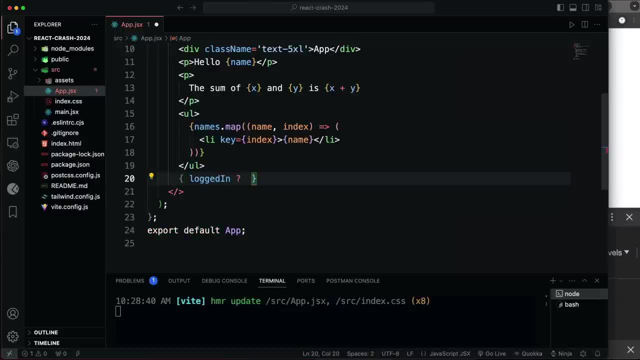 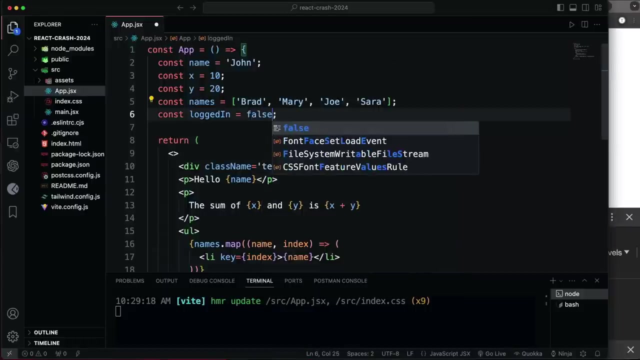 in, then let's show an h1, and we'll say hello member else. then we'll show we'll say hello guest. So now if we take a look it says hello member and if I change logged in to false it says Hello guest. Now let's say you don't want to. 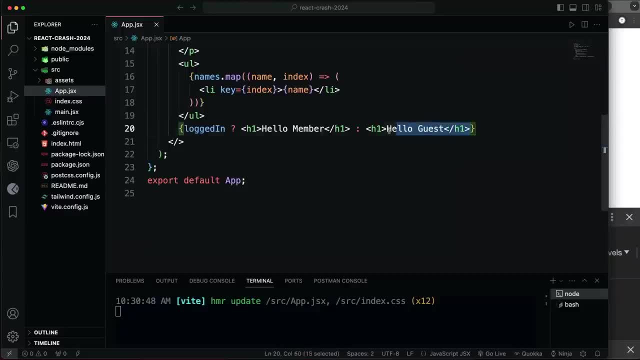 show Hello guest. you just want to show Hello member if they're logged in. So a couple things you could do. you could just put an empty string here, So now it doesn't show anything. Or you could get rid of this- the colon here- And instead of using a ternary you could just use a double. 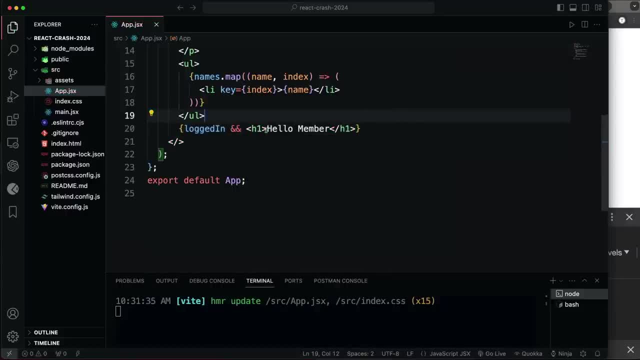 ampersand. So basically this is going to return this. if this is true, So right now it doesn't show anything. But if I change it to false, it says: Hello guest. Now let's say you don't want. 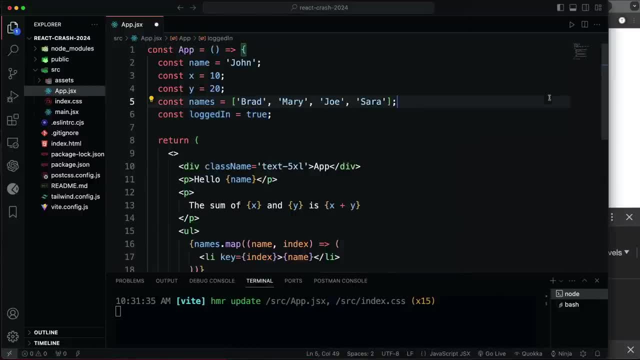 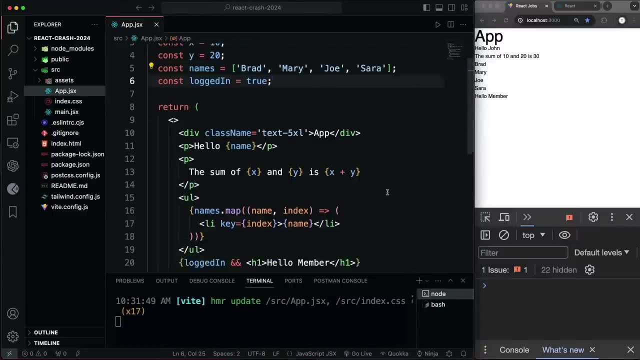 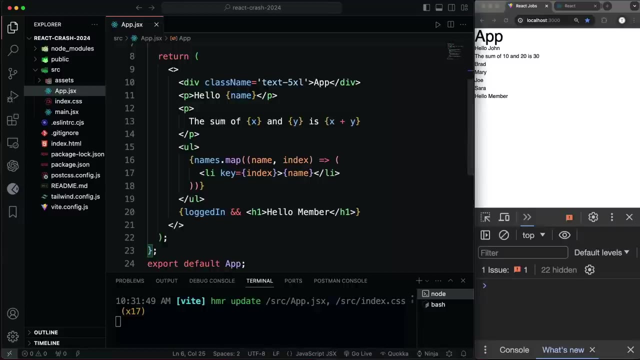 anything. But if I change logged in to true, I should probably just make this smaller. So if I change logged into true now it says: Hello member. Okay, so you can do all kinds of dynamic stuff in here And I like to say that JSX is what HTML would be if it were a programming. 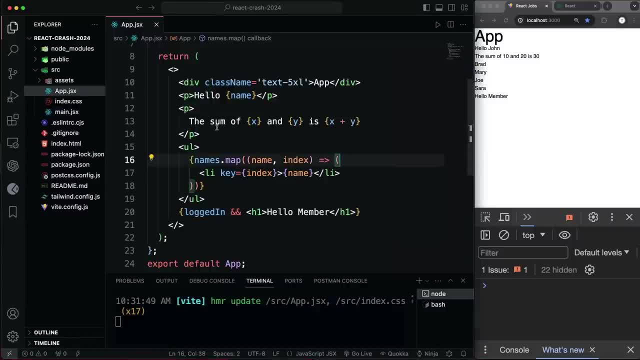 language and it had logic. Now for styling. there's a couple ways you can do this. So, obviously, you can have your CSS file and you can add class class names. okay, remember, you don't want to use class, you want to use class name. But if you want to put inline, 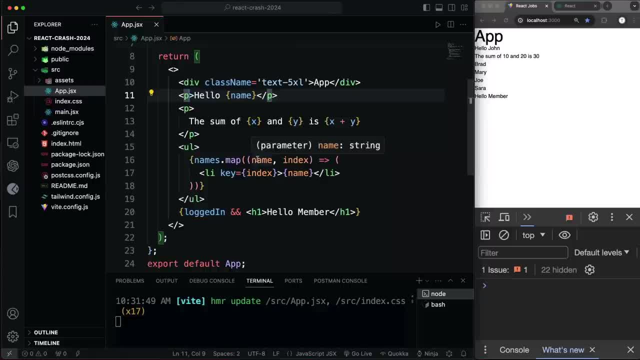 style. you can actually do that within your JavaScript, within your JSX. So let's say, for I don't know, I guess this, this, Hello john, right here, let's add style. Now we're going to pass in here double curly braces. if you're adding inline style like this: 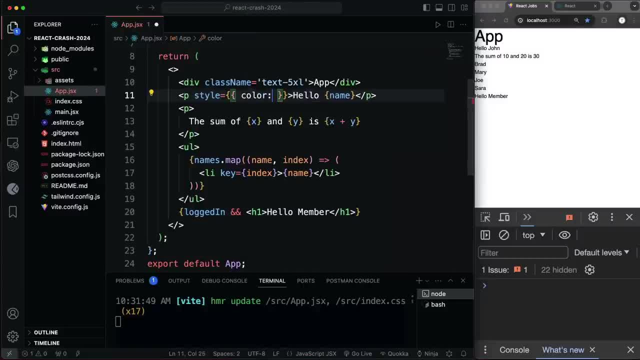 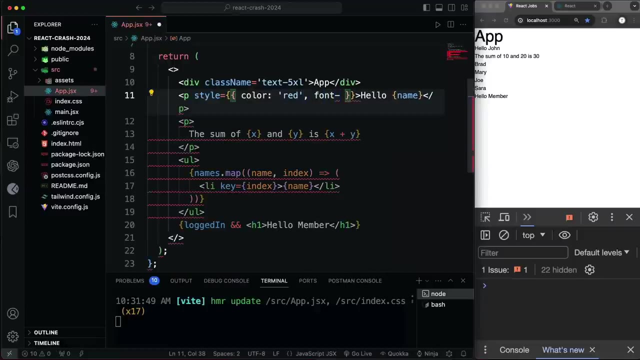 And let's say we want to change the color. So we would say color colon and then a string of red. So it's not quite CSS, but you have the same properties. But one difference is you're not going to have for like font size, like let's put a comma here. you're not going to do font dash size. 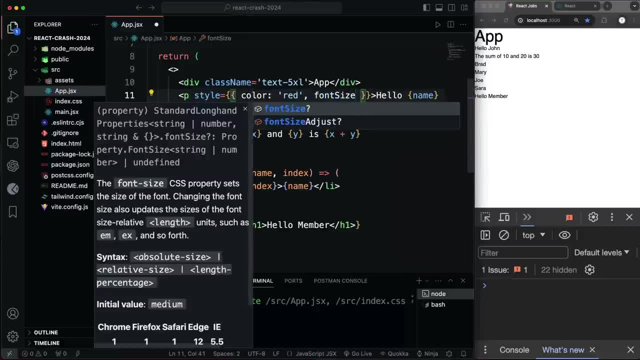 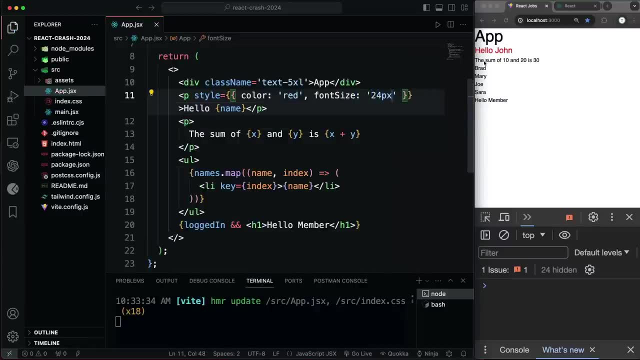 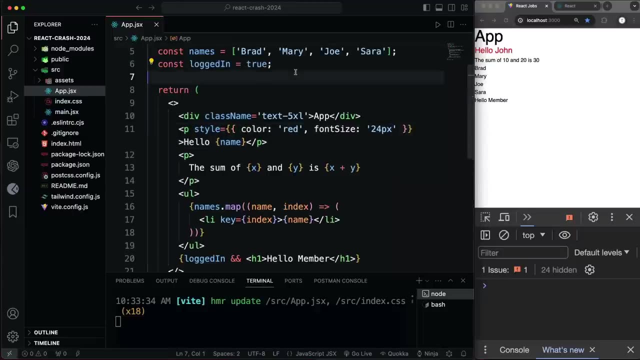 like you wouldn't. CSS. you're going to do font size like that And we'll change that to, let's say, 24 pixels. Alright, so if I save that now, you'll see that that style differently. Now you can also put this stuff in a variable if you wanted to. So up here, let's say: 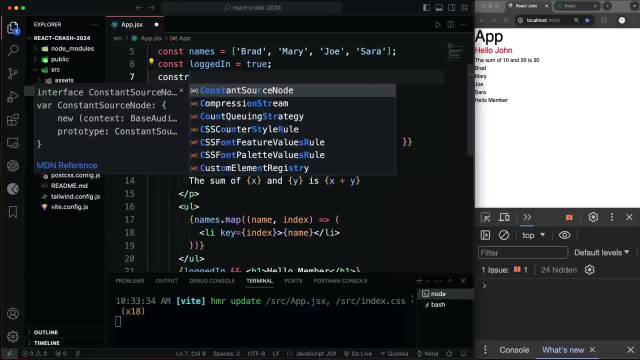 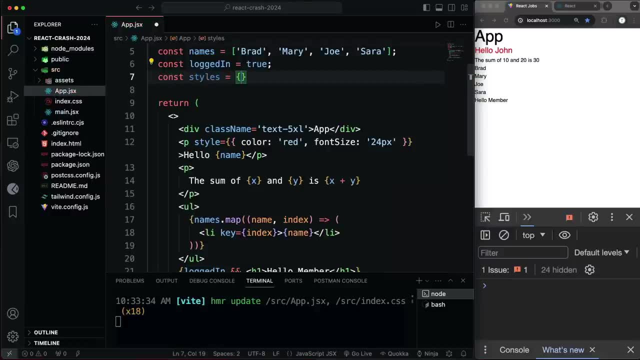 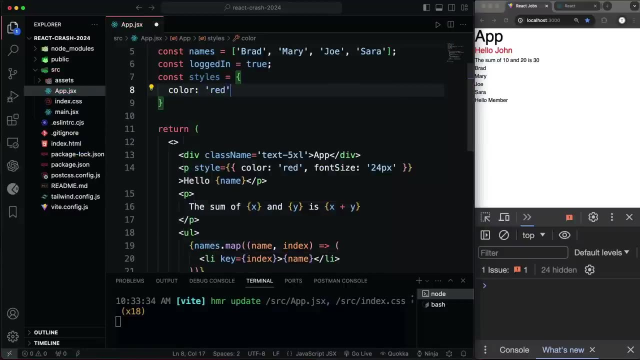 we want to do const And let's call this. we'll just call it styles, const, styles, And we're going to set that to an object that has color color red. so make sure you put it quotes, because it's a string, and then font size And for that 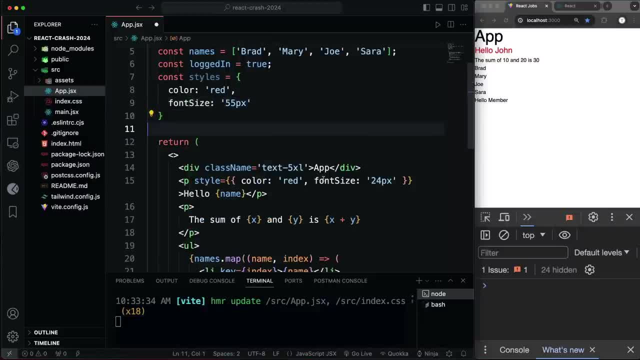 we'll say, let's say, 55 pixels, And then what you can do is, instead of setting this, you could just simply set it to. In this case, you would do single brackets or curly braces and then just add in styles. Okay, so now it's using this, but we're not going to need to do anything like this, because we're 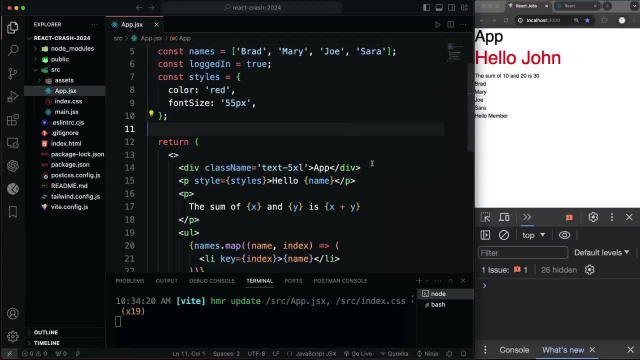 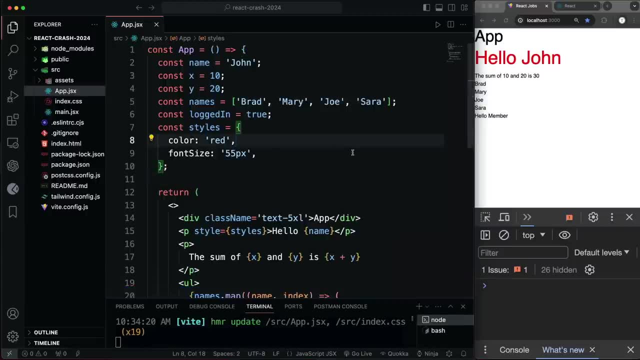 using tailwind. So all we have to do is add classes, Alright. so none of this has to do with the project. I just wanted to kind of give you a little intro, a little crash course to JSX. So what I'm going to do is just get rid of all of it and RAFCE once again and just clear all that. 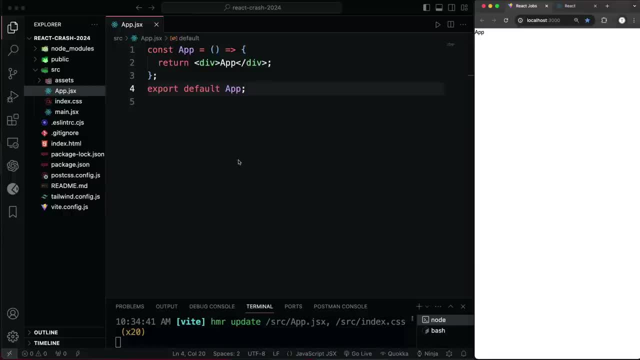 So we can close this up for now. So we want to start our project, And the way that I want to do this is just start off by copying the entire homepage and putting it into our app, our main app component, and then break it up into smaller components. So let's do that. I'm going to go to 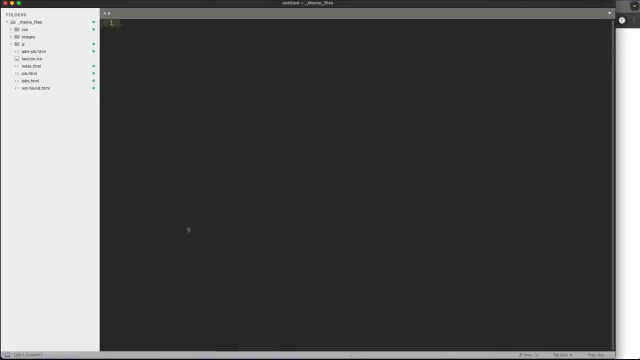 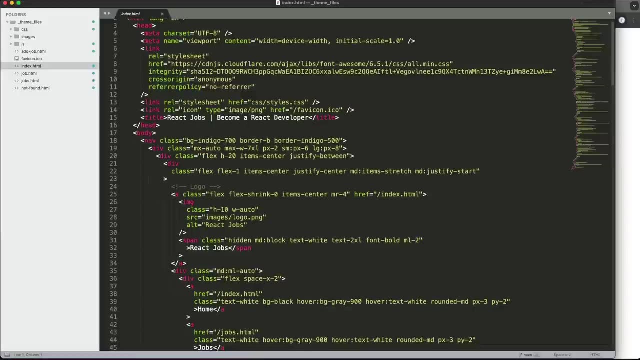 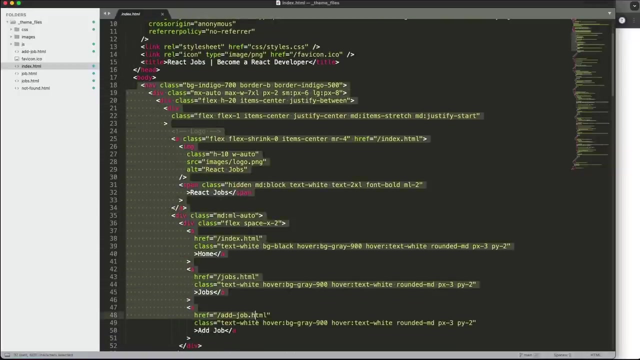 Sublime Text, because that's where I have my theme files And we're going to go to index HTML. Okay, so just open that up Now. we don't need the head stuff. that's already in the, the single page, the index html, so let's grab everything that's in the body. so from this nav, 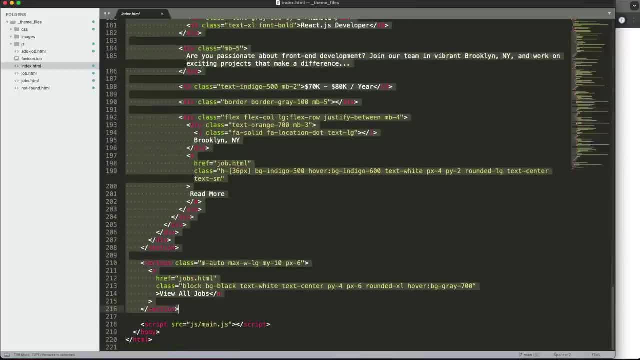 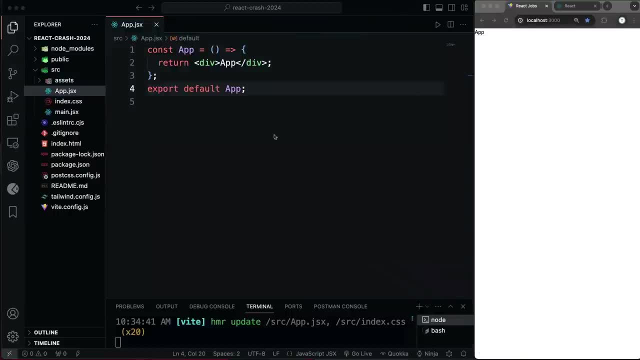 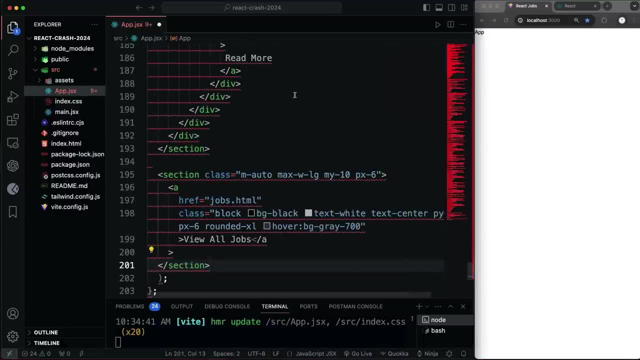 and then we want to go down to, uh, the last section. we don't, we don't want the uh, the script there, so just just grab this and then we're going to put this as the return. so let's return some parentheses and then paste all that stuff in now. i'm sorry we can't do that because, remember it- 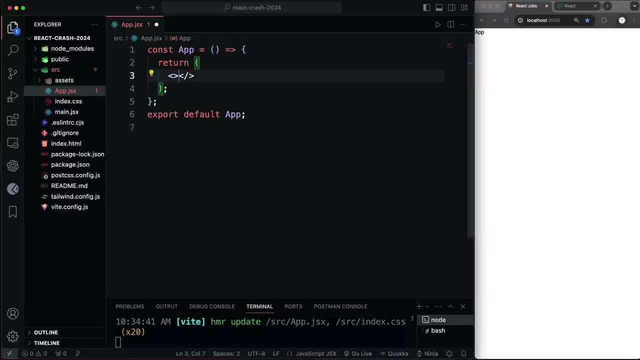 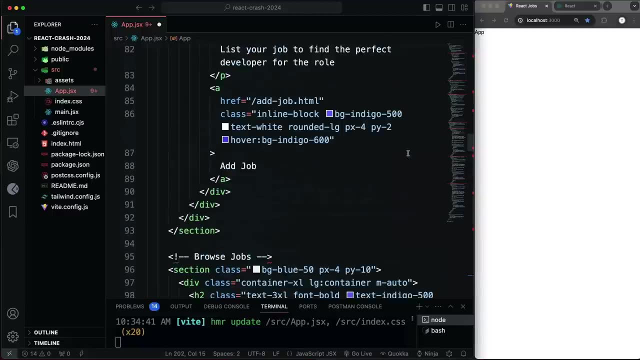 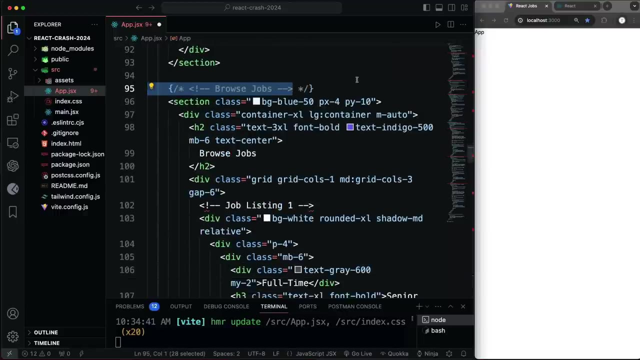 has to be inside of a parent. so what we can do is use a fragment and then paste everything in that fragment. now, remember we don't want to use class. it will work well. one thing that's not going to work is the comments here. so you either have to comment it out with jsx syntax like this, or just 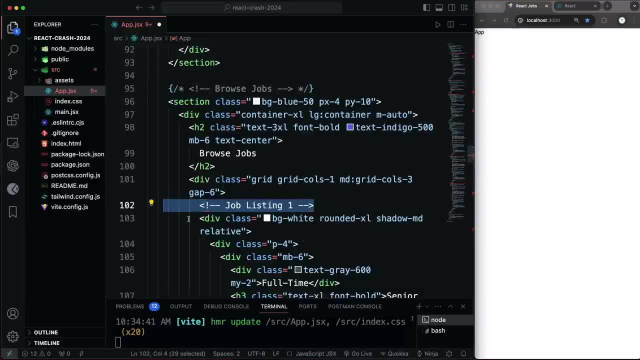 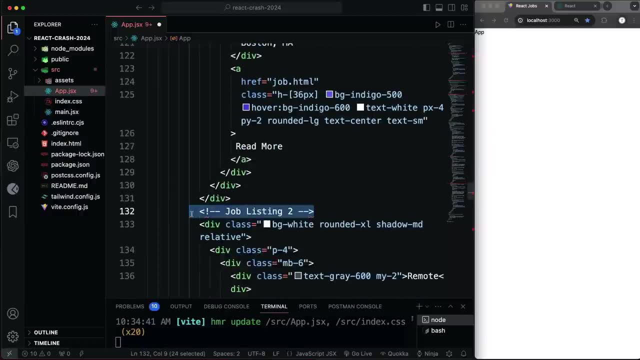 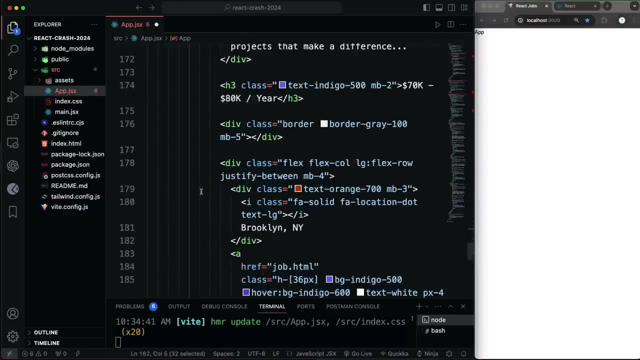 get rid of the comments. i'm just gonna, i'm gonna get rid of. well, i guess i'll keep them, we'll just comment these out. so yeah, you definitely want to either delete or comment them out because you're going to get an error. so, job listing 3 and i just put the comments in just to kind of break everything up. is that all? 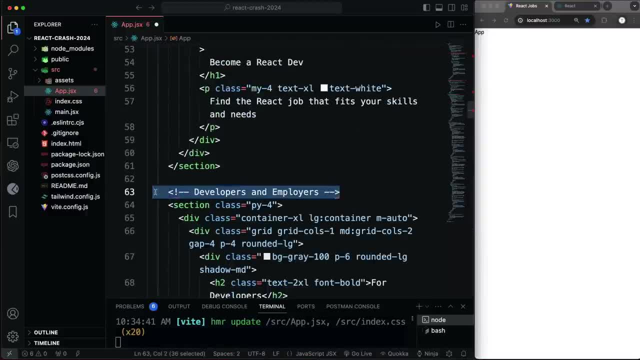 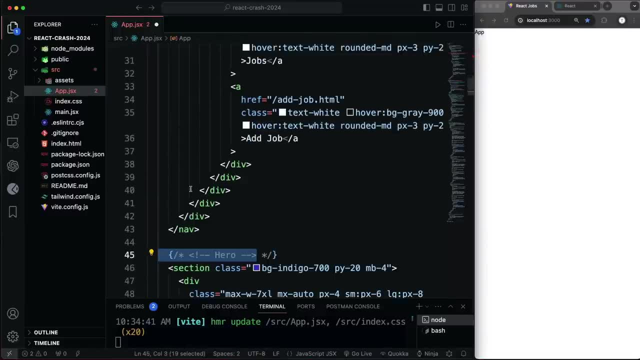 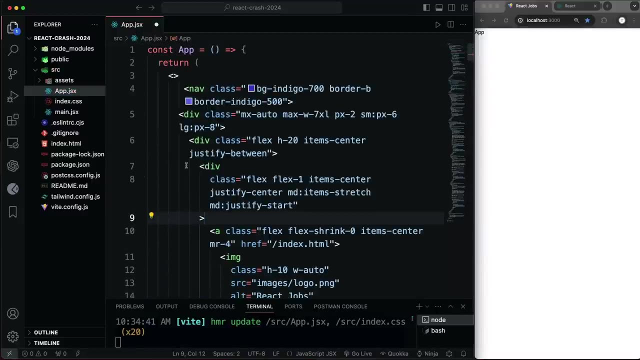 of them. let's see this one here: developers and employers hero. and to comment it out, i'm just highlighting and doing command forward slash or control forward slash logo. we don't need that comment, okay, all right. so now if i save that, you'll see it actually does work. 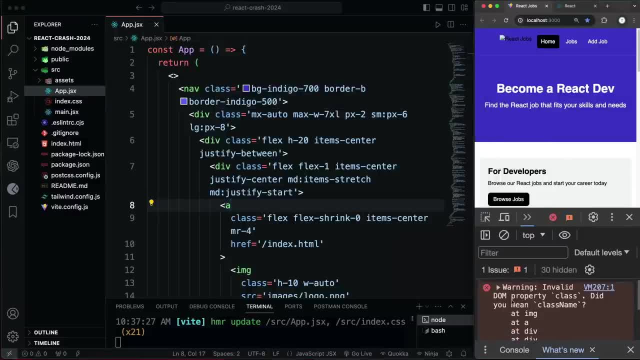 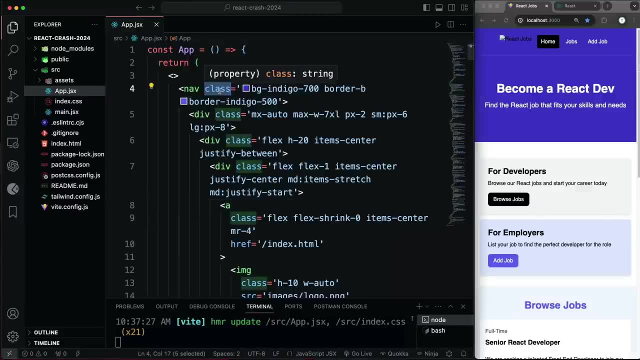 but if i were to open up the console, it's going to tell me invalid dom property class- did you mean class name? so it's telling us to change these. so what we can do is just highlight the first one and we can do a command or control, shift l that will select all of them and then we're going to 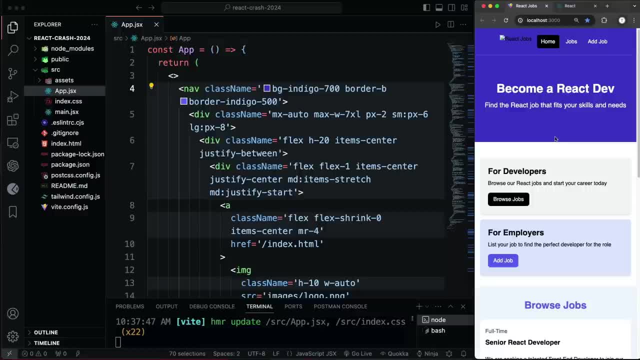 change it to class name, save it and then that should. if we reload, that will get rid of the the warning. okay, so now we have our entire module that we're going to be using, so just do this. so create the class name makes it easy to set up the tab. so if you're looking to change the class name, 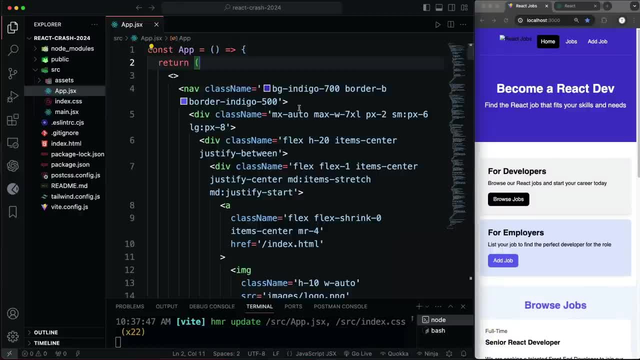 have our entire page inside of this, the app component, which obviously isn't what we want. we want to break everything up into components, so let's start off. we'll just go from top to bottom. we'll start with the navbar, so that's this entire nav tag and everything in it. so what we'll do is: 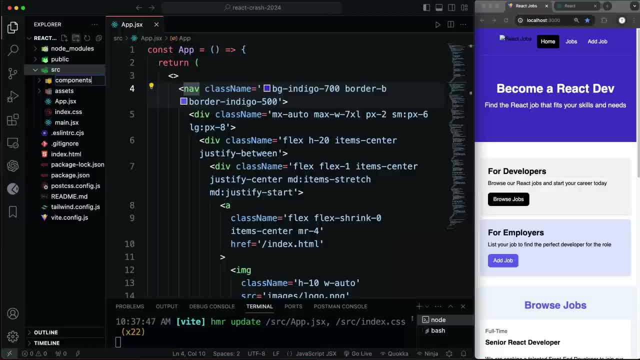 in the source folder we're going to create a new folder called components, and in components i'm going to create a file called navbarjsa. now a component can have a js or a jsx extension, and if you're using typescript, it can be ts or tsx. i prefer jsx, so we're just going to do that, and 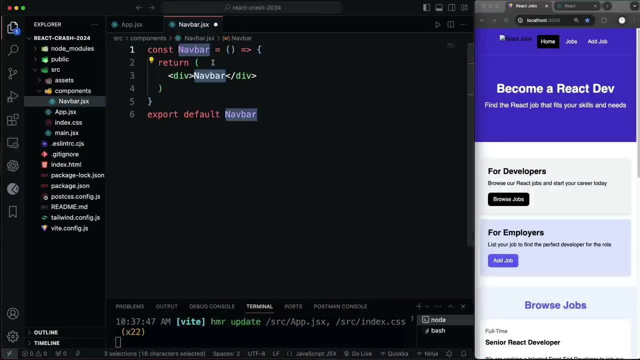 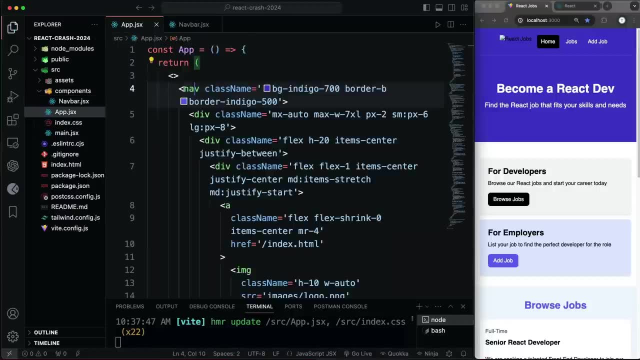 we'll do r-a-f-c-e again and it's going to call it navbar because that's the name of the file. that's fine, so i'll save that now to bring that in and use it into our main component. we're going to go up to the top here and say: import now. 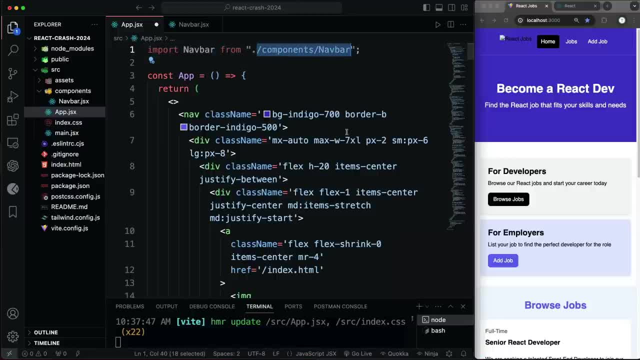 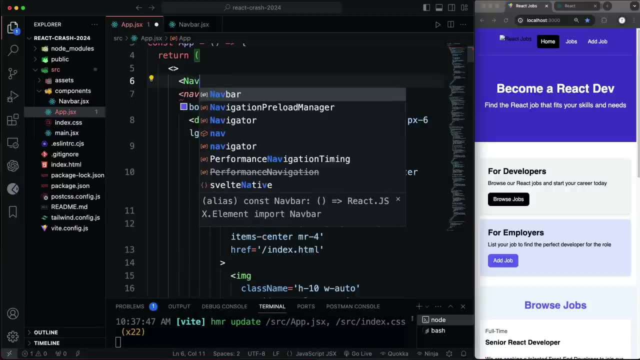 and we're going to go into the navbar from dot slash, components, navbar, and then we can put that anywhere in here we want. let's just go right above the actual nav tag and say navbar, just like a, an html tag, and there it is. so now we're importing and using. 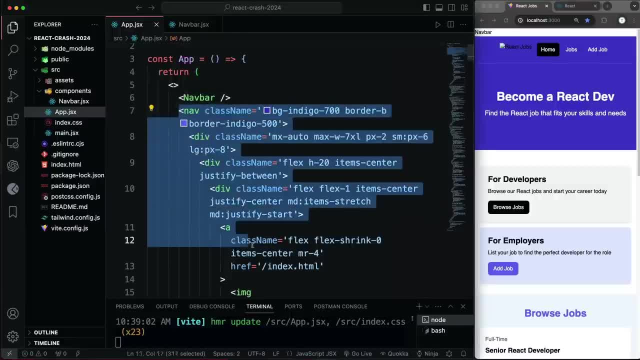 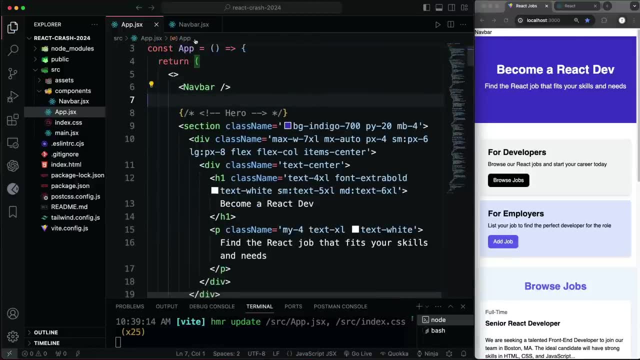 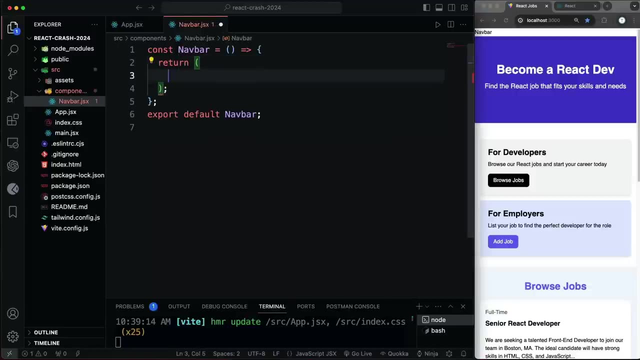 that component. so let's take the, the entire nav tag and everything in it and let's cut that. if we save it, you can see now it's gone and i'm going to go into the navbar and i want to put that as the return. so we'll put some parentheses and then paste that in, save it and 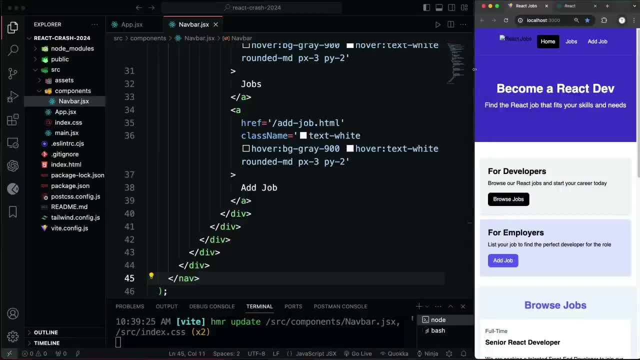 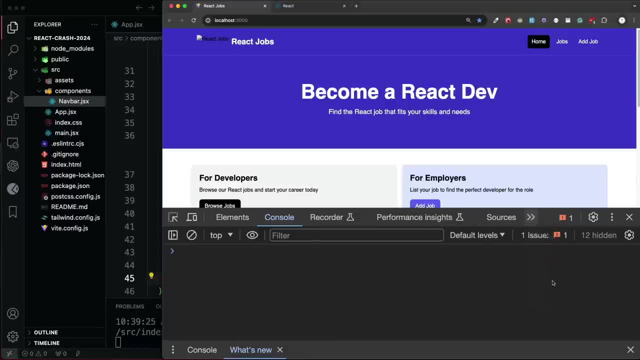 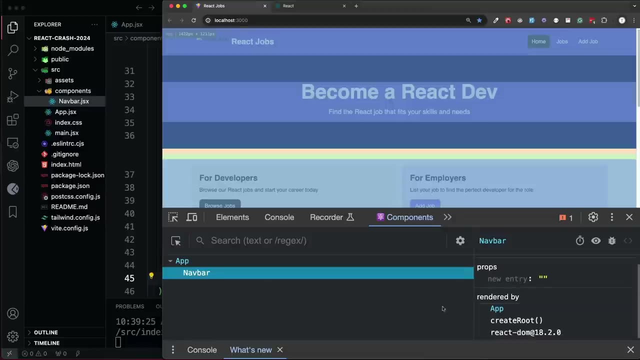 now it's back, okay, but it's in its own component. and if we were to use the react dev tools? so if you open up your tools down here and you go to components, you can see we have our navbar component and it will show you any props or state which obviously right now we don't have any, but that's. 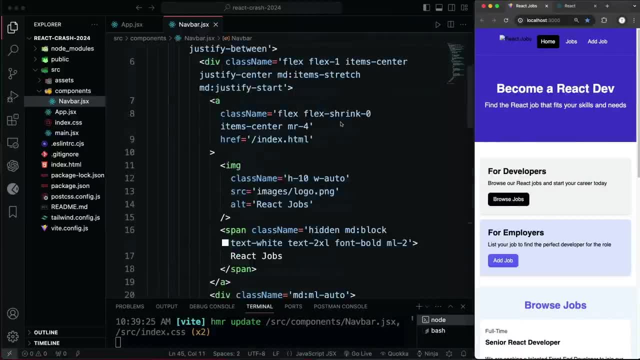 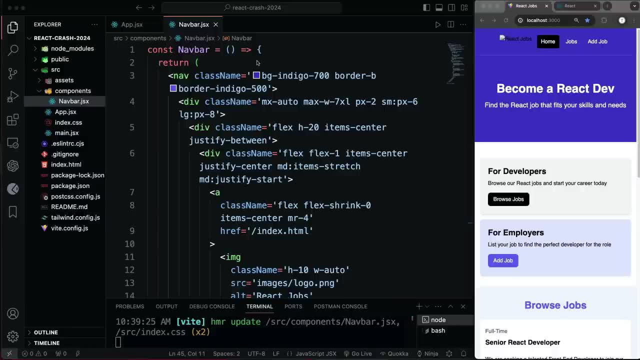 a separate component, a ui component. so now let's- uh, let's- do some stuff here. you notice that the image isn't showing the logo, so, first thing, we need to bring it into our file structure and i'm going to put it in the assets folder. right now there's just this react svg, which we can- just we can- get rid of that. 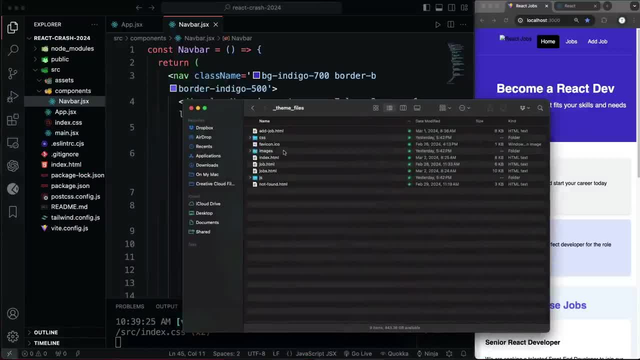 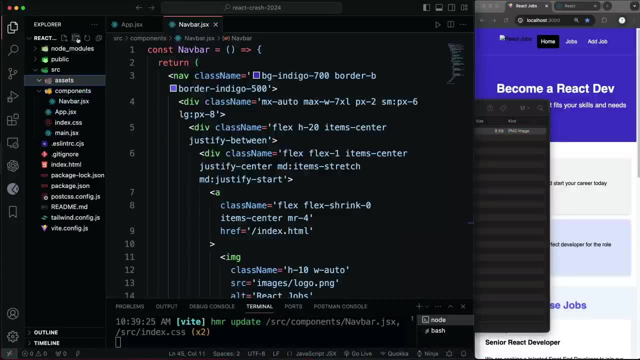 and let's bring over. so if you go in your theme files and you go to images, you'll have the logo png. so i'm going to bring that. actually, let's create, let's create a folder called images in the assets folder and then we'll bring the logo into that. 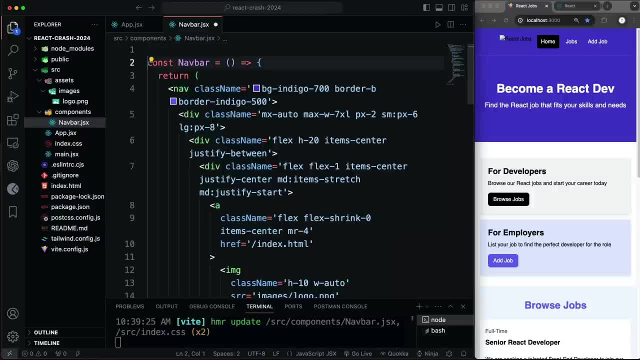 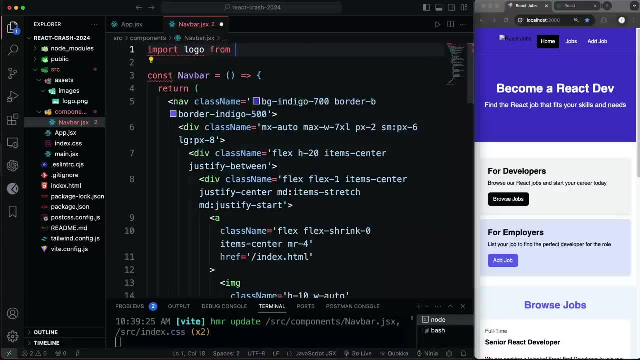 all right, and then what we can do is bring that image in to our navbar so we can say import, let's say import logo from, and then we need to navigate. let's see we're in components. so we want to go up one level into assets and then into images, and then 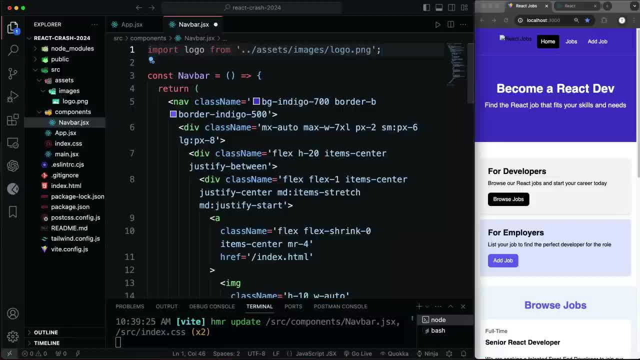 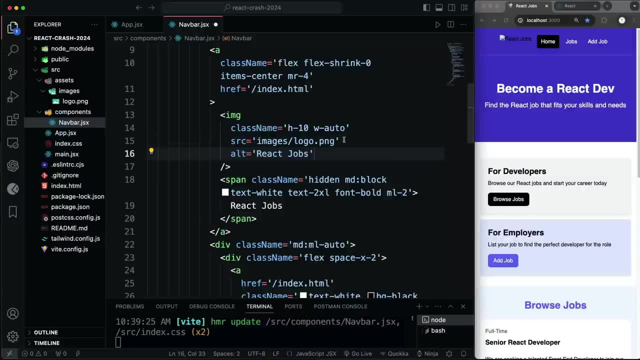 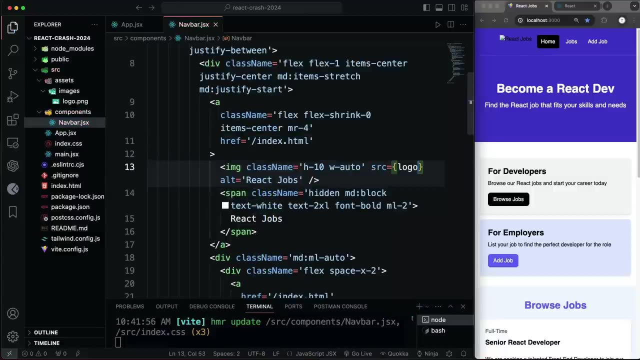 logo dot png. okay, so we're going to bring that file in and then we can go down to the image where we have the logo, which is right here, and let's replace the source. we're going to make it dynamic, so we need our curly braces and then we can say logo. and there we go. so now the logo shows. 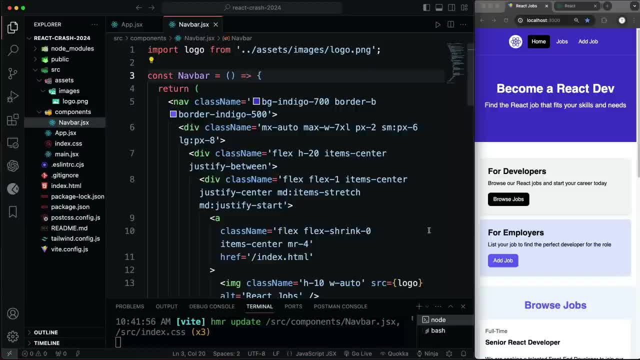 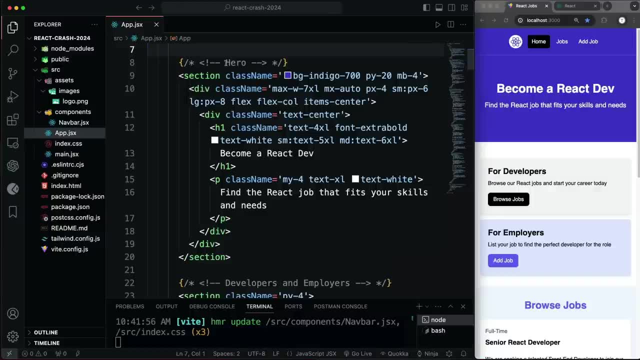 so now the navbar is its own component. we'll come back to this later when we deal with the, the routes and links and that stuff. but now let's deal with the hero. so the hero is not Kosten hero. is this section right here? so i'm going to just get rid of that comment and then i'm going 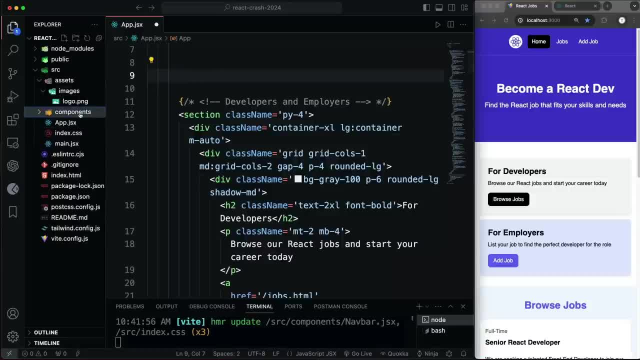 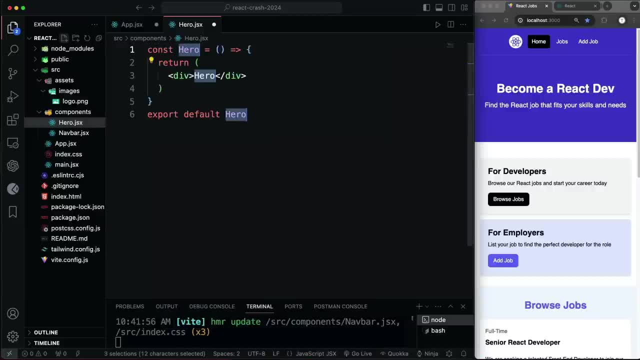 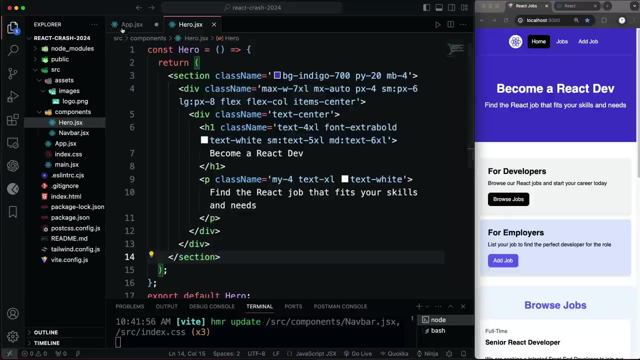 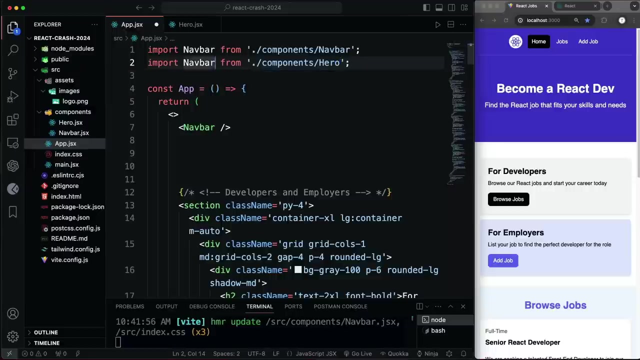 to cut this entire section and then, in components, let's create a file called herojsx and we'll do rafce and let's get rid of that, and then i'm going to paste in that section, save it, and then let's go to our appjs and do the same thing. we'll bring in hero, hero and then we can embed it like that. 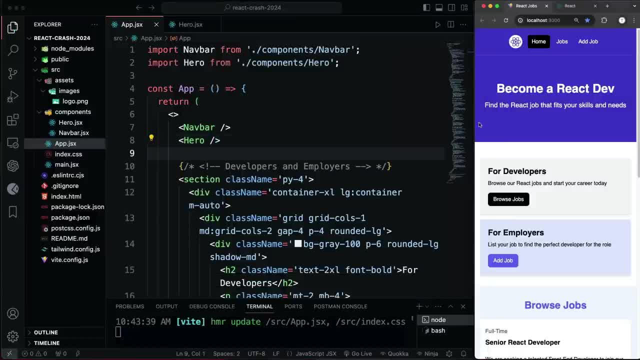 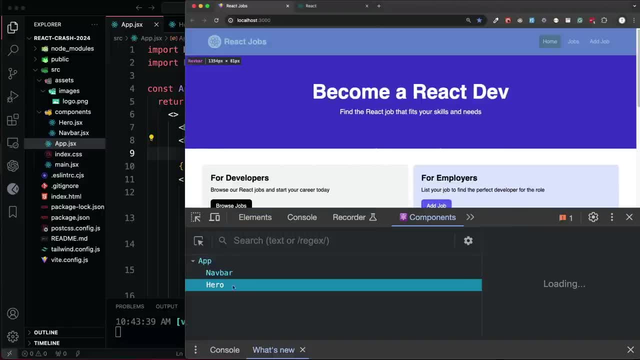 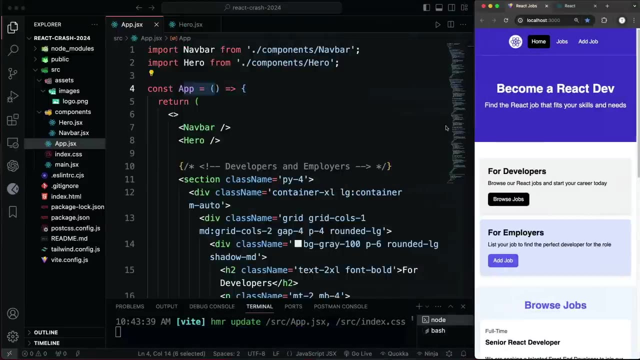 okay, save, and we still get the same thing. but now the hero is in its own component. in fact, if we look at the dev tools again, if we go to components, you'll see we have navbar and we have hero. now i want to go over props because, remember, i said we can pass in props to a component, which are basically attributes. 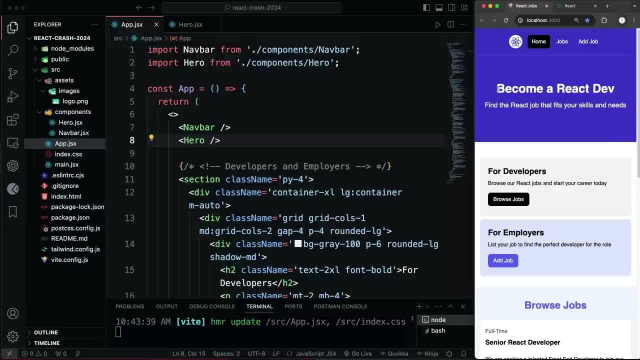 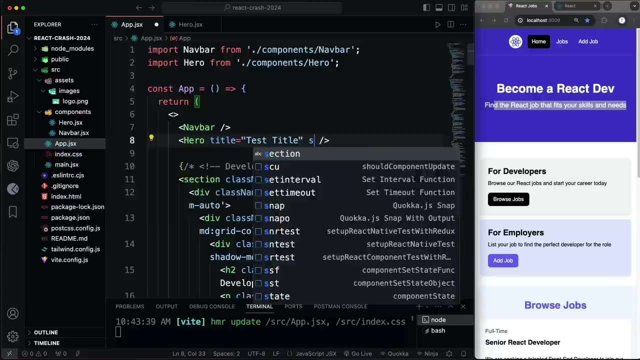 so let's say we want to be able to pass in two things: we want to pass in the title, which would be this, and the subtitle, which would be the smaller text, so we can pass it in. let's say title, and for now i'll just say test title, and then let's pass in subtitle and i'll say this is the. 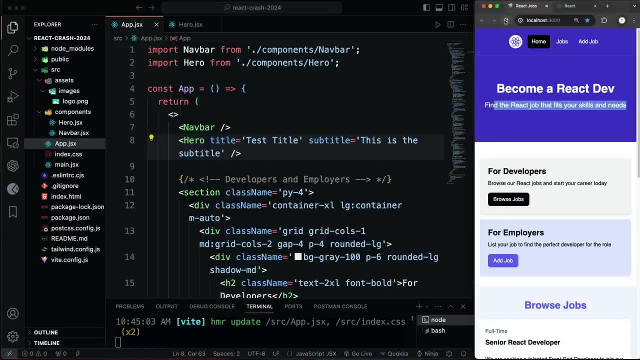 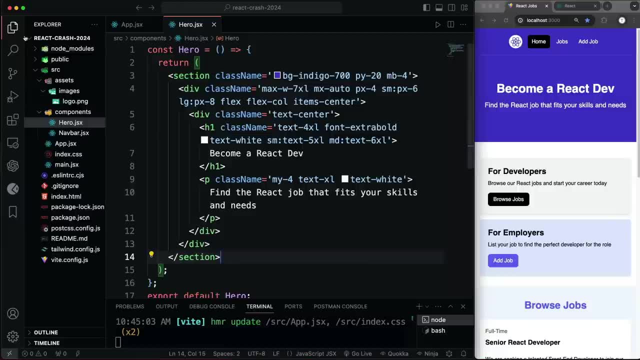 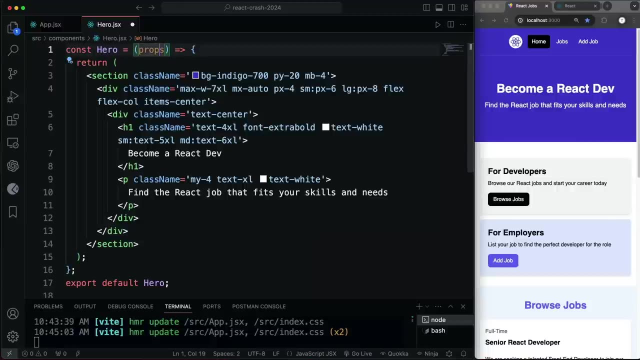 subtitle. okay. so by doing that nothing happens, right? so i mean, i'm just passing it in, i'm not using it in any way. so let's go into the hero, close that up for now, and then what happens is that props. it'll get passed in here and you can call this anything. i'm going to call it props for now, but in a 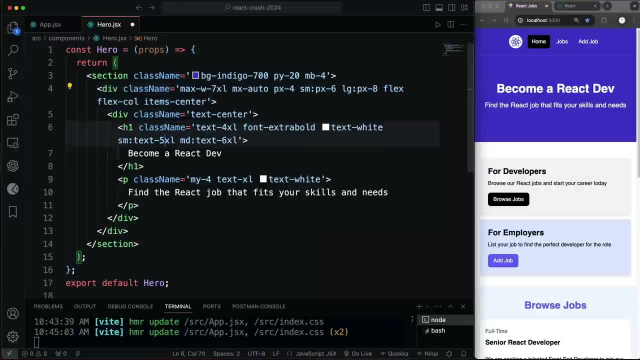 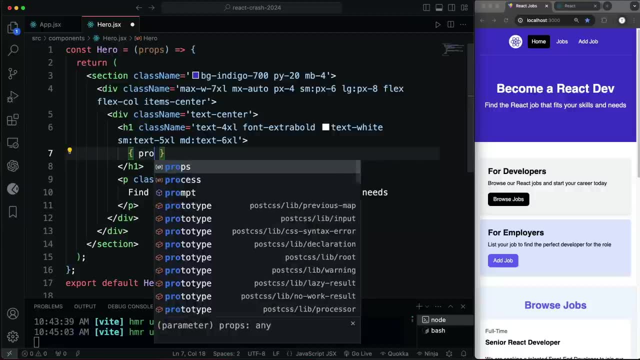 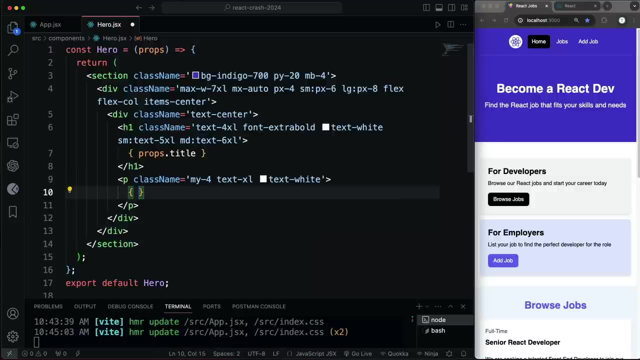 minute i'm going to show you how we can destructure it as well. so we want to put the title here instead of this hard-coded content. so what we would do is open up our curly braces. we can say props dot- title and then, here for this one, we'll say props, props dot subtitle. 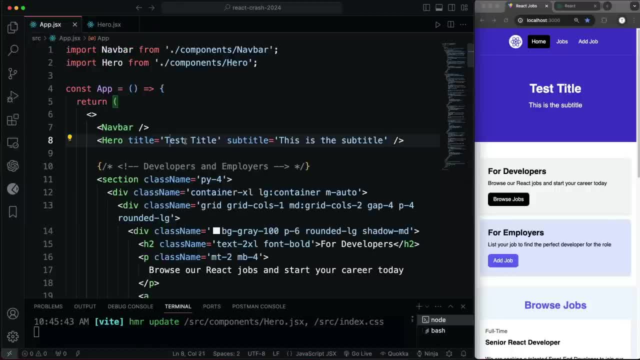 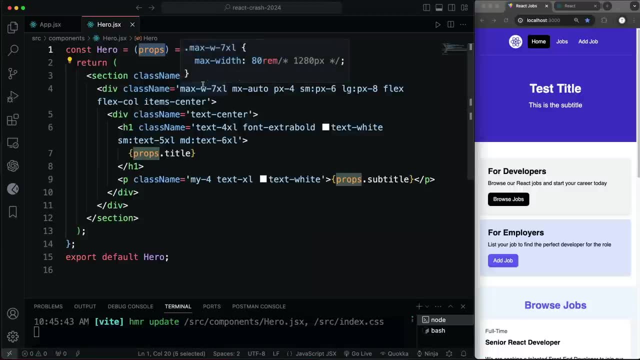 and if i save that now, whatever i'm passing in is going to get displayed as the title and subtitle. now, usually what you'll do is destructure this, so instead of just props, we could add some curly braces in here and then destructure the title and the subtitle like that. 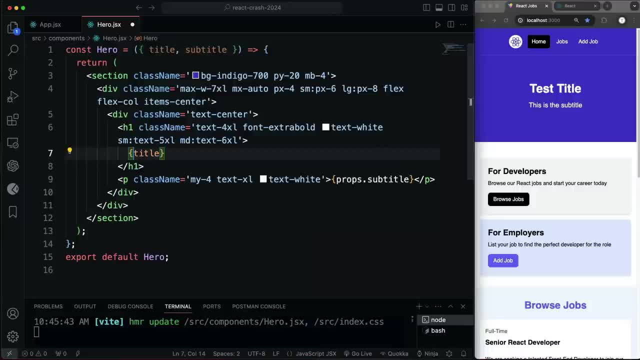 then wherever we use this, we don't have to do props dot, we can just do title, and then here we can just do subtitle and that still works. now you can also have default props. so all we have to do is up here, let's say, for the default we want. 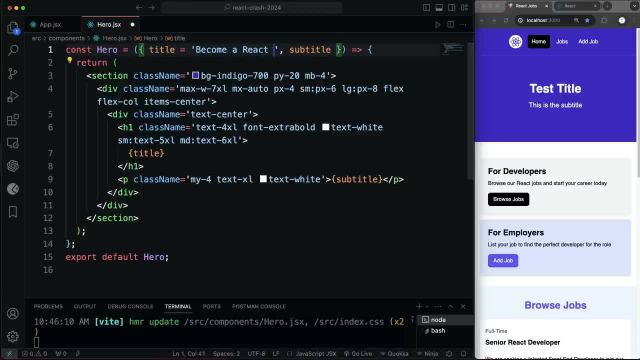 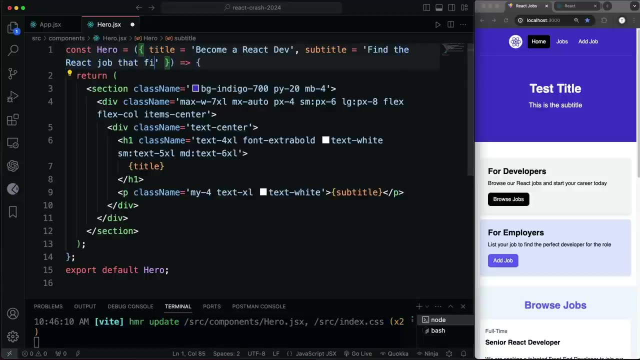 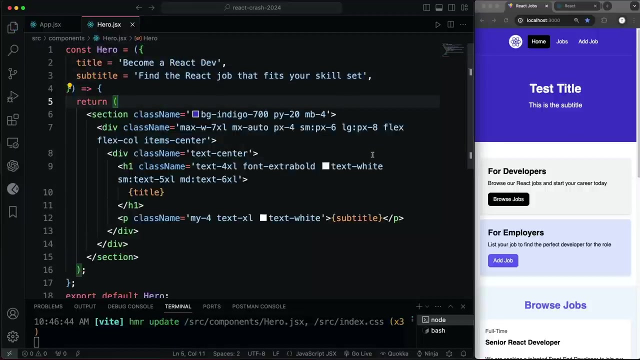 what we had become a react dev and then for the subtitle set that: uh, what was it find? find the react job that fits your skill set. okay, so if i save that, nothing happens because we're passing in the title and subtitle. whatever we pass in is going to override. 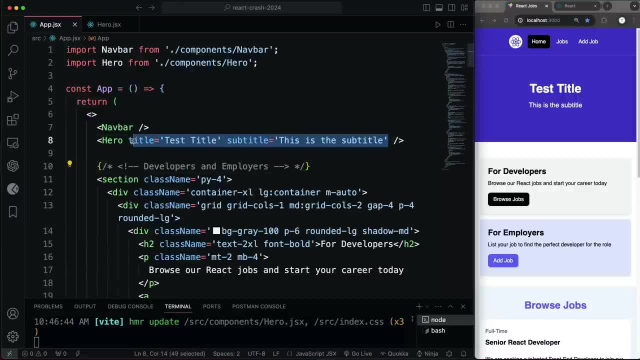 the default props. so let's get rid of these, put it back to just hero. and now we have our default prop content showing. now we can also have wrapper components. so, in addition to just being able to do this with the self-closing tag, we could do something like, let's say, we had a card component. 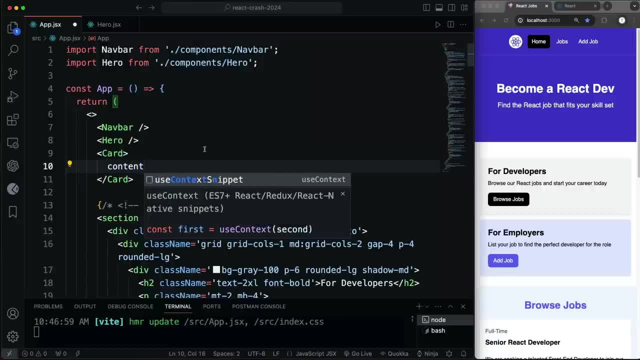 and then you want to put you know whatever content inside of it. so let's do that for these two cards here all right now, instead of of bringing in the card component that we're going to create into this file and having all that content here. i want to keep this active, so i'm going to go ahead and 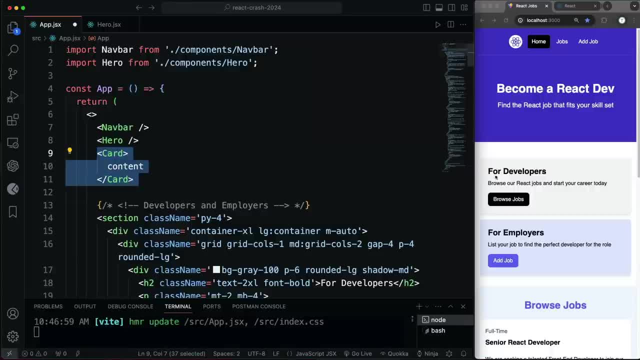 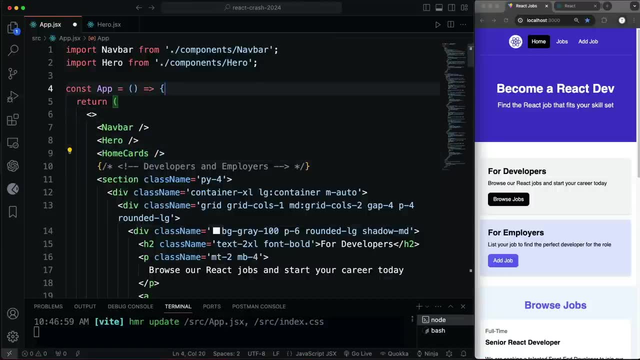 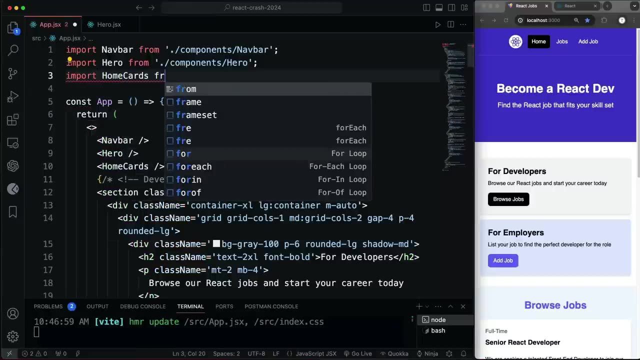 keep this app file clean. so what we'll do is create a component to hold all of our cards and we'll call that home cards. i know we didn't create this yet, but let's just embed it here and then bring it in. we'll say: import home cards from, and it's going to be in components: slash home cards. 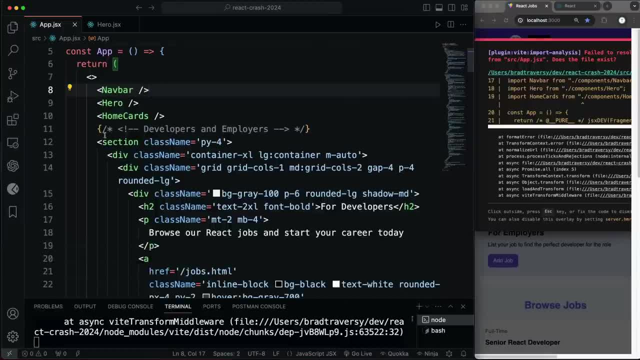 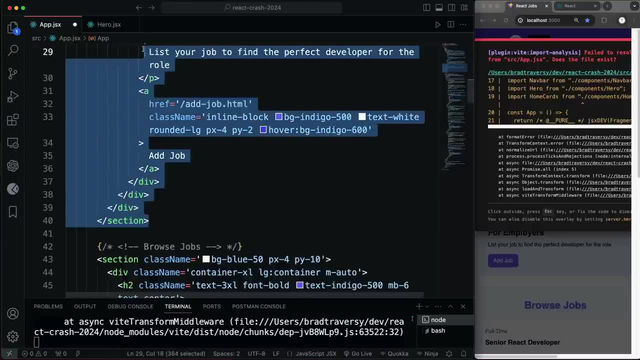 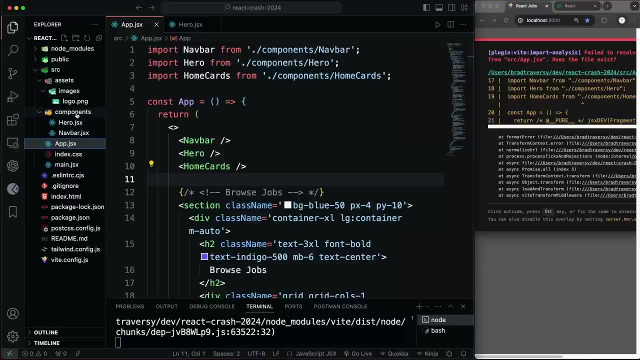 okay, and i know we haven't created it yet. that's why we have an error, but let's go ahead, we can get rid of that comment. and then let's copy this entire section, which ends right here. okay, so we're going to- not we're going to- cut that and let's go into components, right, and then 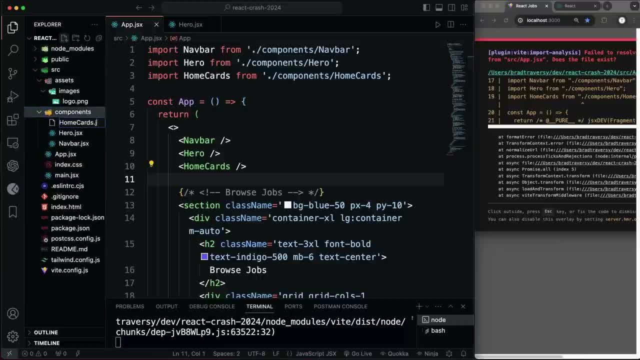 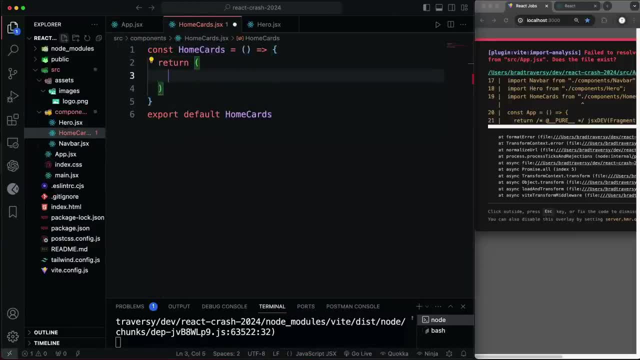 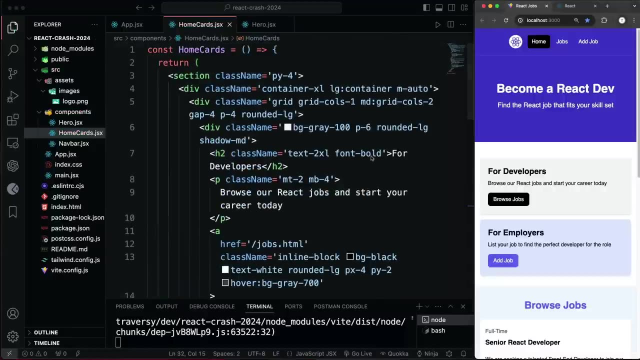 components. we're going to create a new file called homecardsjsx- r-a-f-c-e, and then let's do get rid of this, and then we'll paste in that section, and then it should should. yeah, there we go, so it's working again. so now this right here is its own component, called. 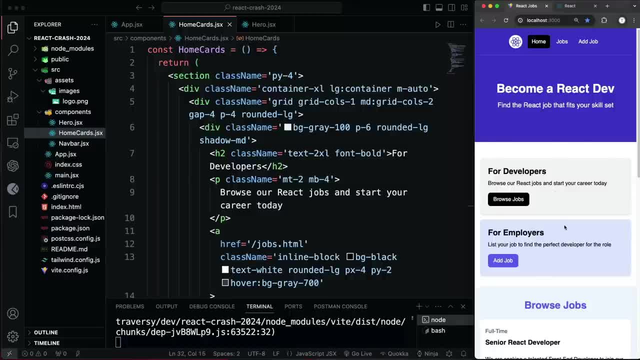 home cards, but what i want to do is have each one of these be a card component that we can wrap the content in. so whatever content we wrap will have this background color and i also want to pass in that background color as a prop or pass in the class as a prop. so let's create another component. 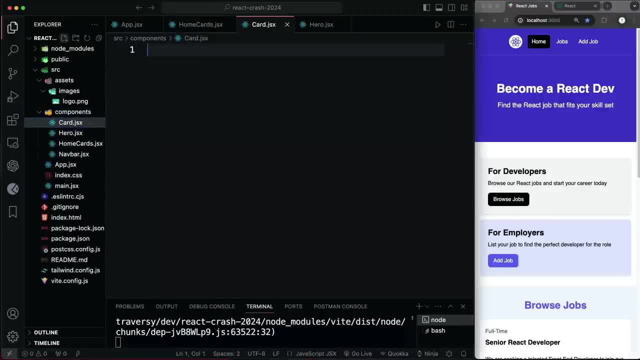 called cardjsx r-a-f-c-e. okay, now this card component is going to take in as a prop. it's going to take in we're going to destructure. it's going to take in children. so children is what we use for whatever we wrap. so if we pass in like an h1 into the card component, we wrap the card. 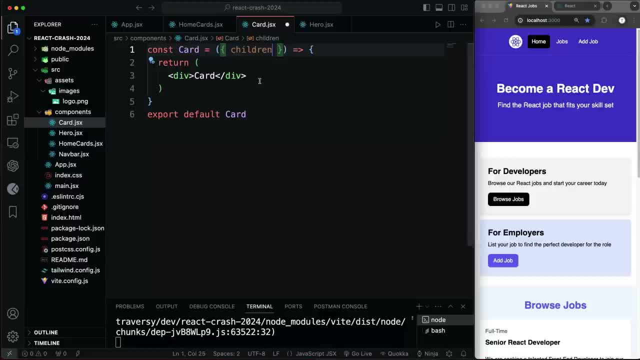 or wrap the h1 in the card, then this would be that h1, so that, children, we just want to display that um in the return. now i do want to have the, the card styling like the background and the, the shadow and all that. so let's um, let's make this a div that we return, but let's add some classes. 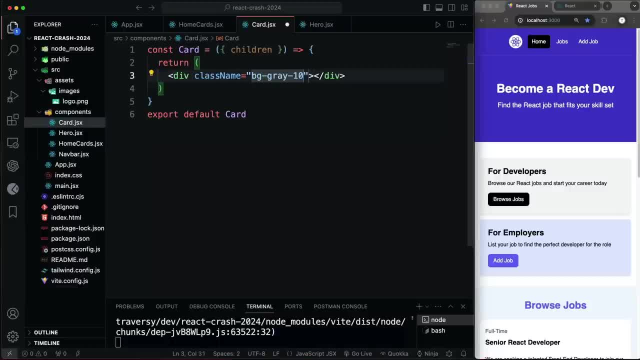 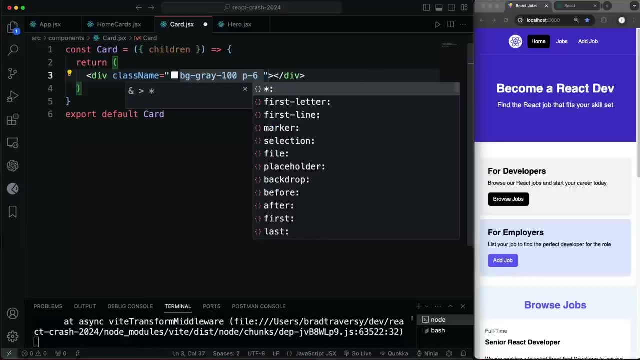 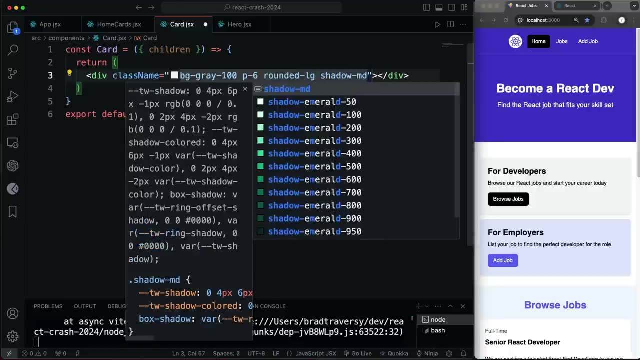 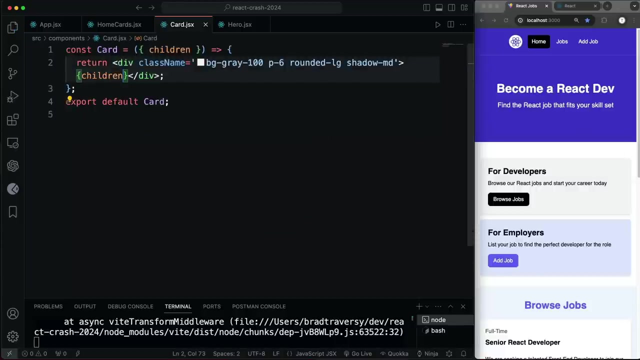 so we'll say: bg dash, gray dash 100, let's do padding dash six, let's do rounded dash lg and let's do shadow dash md. all right, so we'll do that. and then in here is where we want to output the children, which is going to be whatever it is we wrap. so i'll save that. and now let's go into 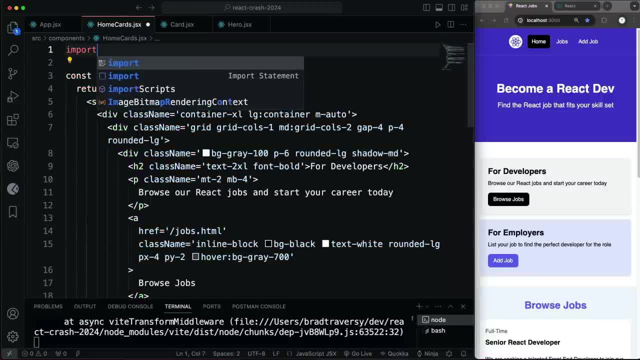 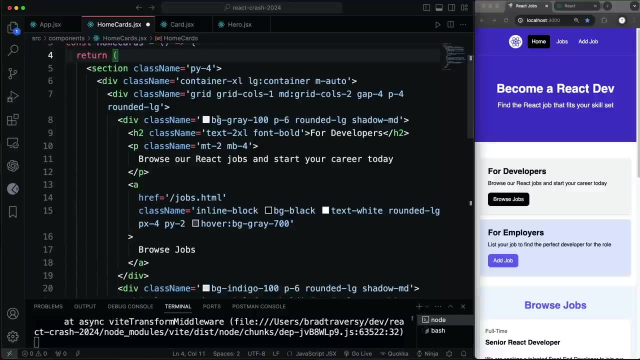 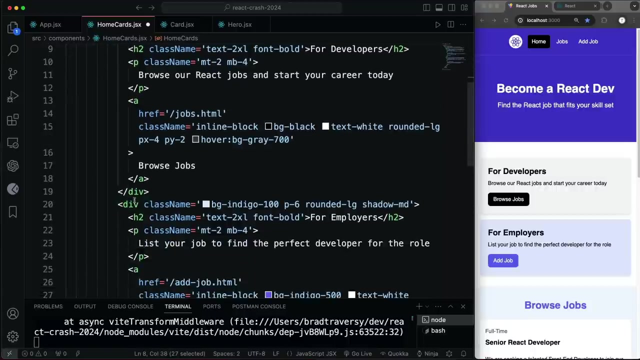 home cards and let's import cards- oops, cards from dot slash, not cards, just card, singular, okay. and then let's see where we have. so we have the grid class, and then these right here, right so, this bg gray and then this bg indigo, these are these two. so i want to take everything. 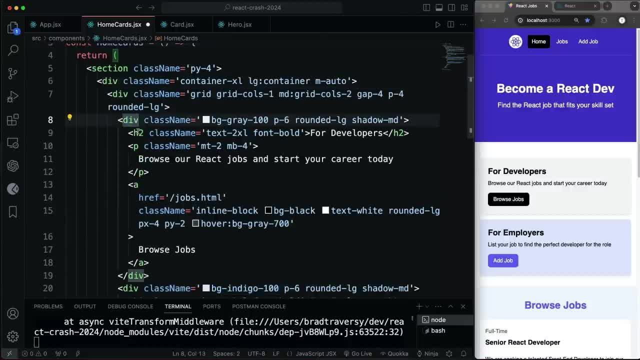 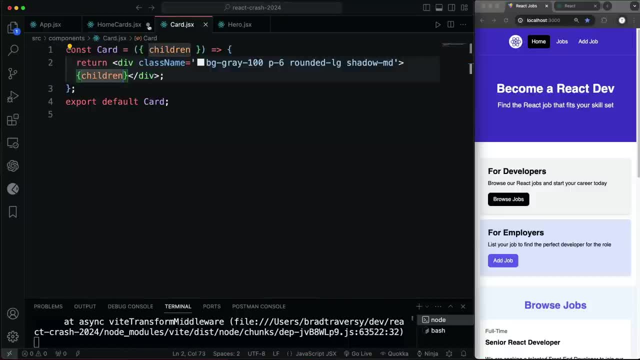 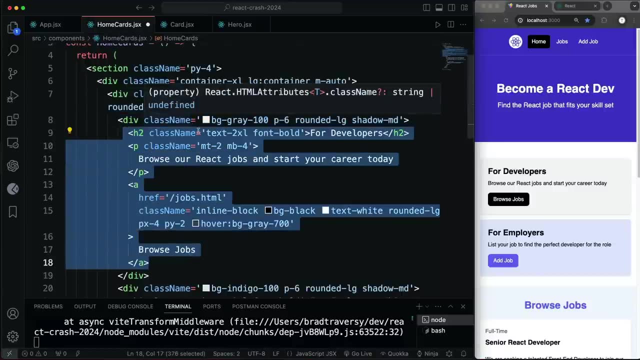 that's in the bg gray div, right here, right this h2 and all this, actually, you know what. let's just take the whole thing, or wait a minute. no, we'll take everything in it. so the h2, the paragraph and the link, i'm going to grab that and i'm going to copy it and then i'm going to cut. 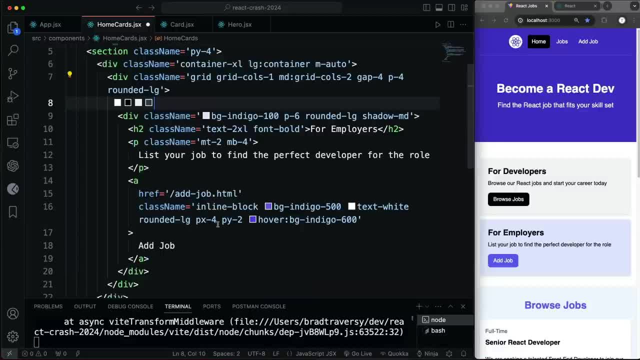 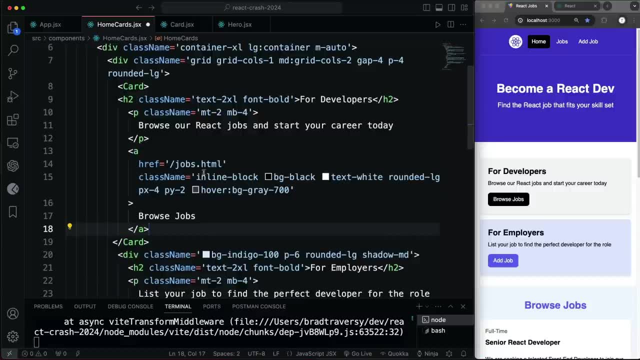 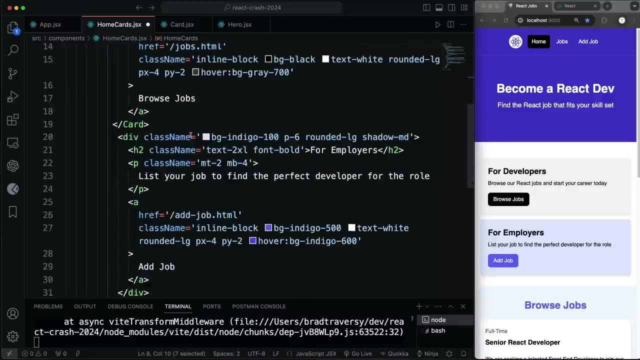 or not cut, but just delete this entire div, and then this is where i want to put the card and i want to wrap this stuff. okay, so this card now is basically just taking the place of the div, this bg gray div, and then let's do the same thing here. we'll take the h2, the paragraph and the link. 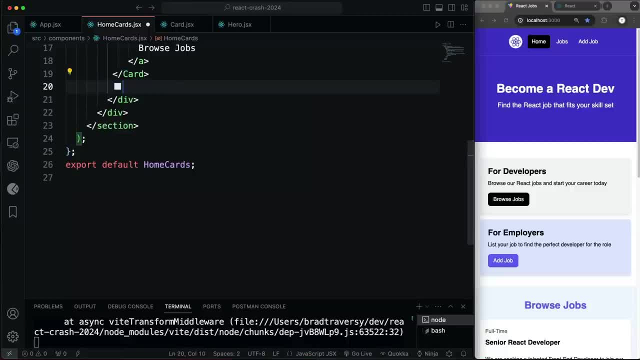 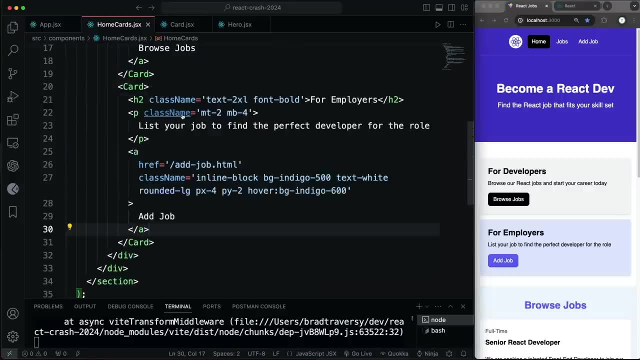 we'll cut that and then we'll replace this div with another card, because you can have as many of the of the same component as you want. then we'll paste that in now. if i save, you'll notice that they're both. they both have a gray background because that's. 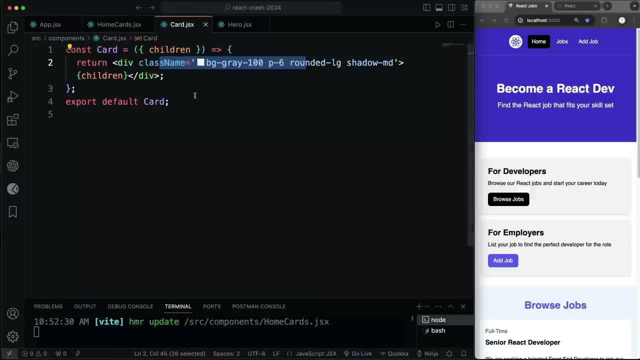 what we're using in the card wrapper component. but what i want to be able to do is pass in a class like this so i can change the background color. so let's add another prop here. so, in addition, that it'll take in bg and i want to set a default of the bg dash gray, dash 100. so that's what it. 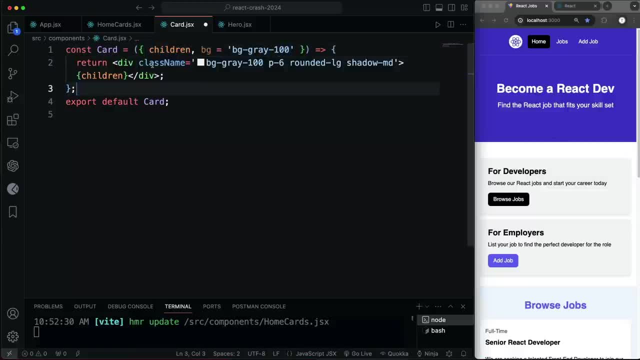 will be if you don't pass in a bg. all right now here. we want to make this class name dynamic. so instead of hard coding the b- this right here- we want it to be this variable. so how do we do that? well, we have to, instead of just using quotes. we have to. it's going to be dynamic, so we need to use. 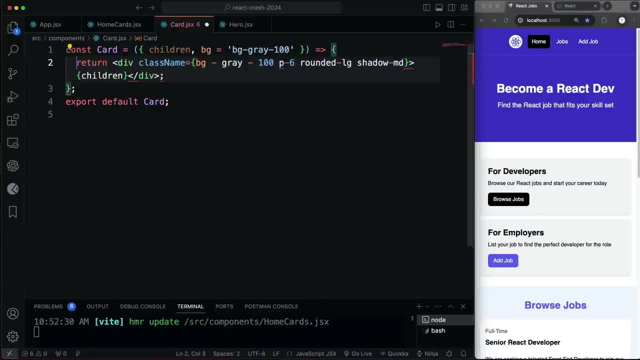 curly braces. so let's do that. and then let's get rid of where's my cursor. let's get rid of this right here, bg gray, and then we're going to put some back ticks in here. so here and then here. okay, so right now it's just it has these hard-coded classes, but since we're 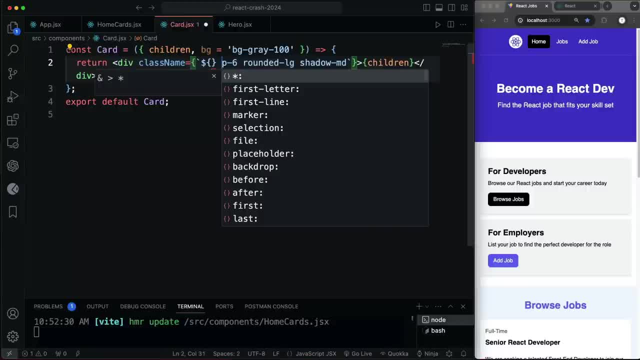 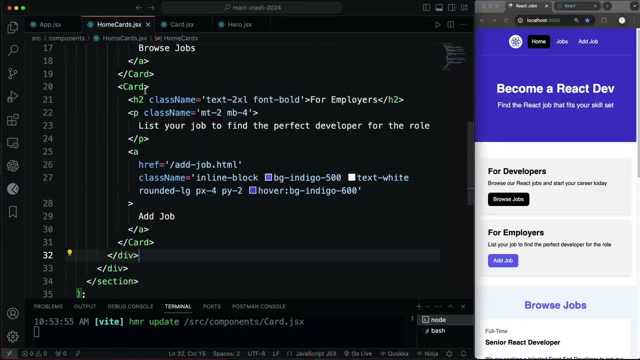 using a template, literal. now i can put a variable in here. so i'm just going to do that and then put the bg variable here, which by default will be this, but i can also pass in a new one. so if i save that now, you'll see that's still gray. but if i were to go to the second card here and then pass in bg, 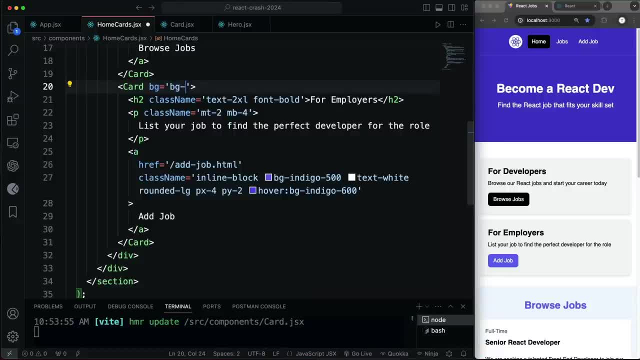 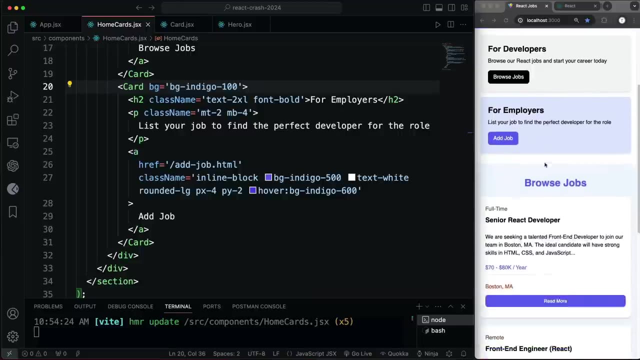 and set that to, let's say, bg dash, indigo dash 100 and save. now i've changed that so you can use props to not only change the content but to also change the styling. so now we've come to the browse jobs and now we want to start to work with data a little bit now. 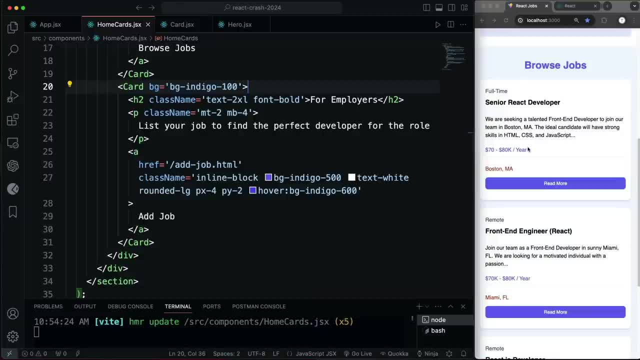 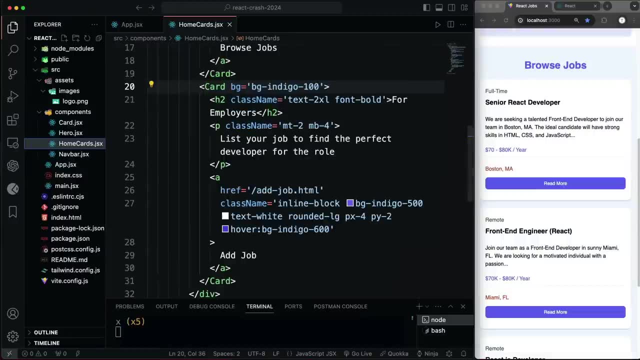 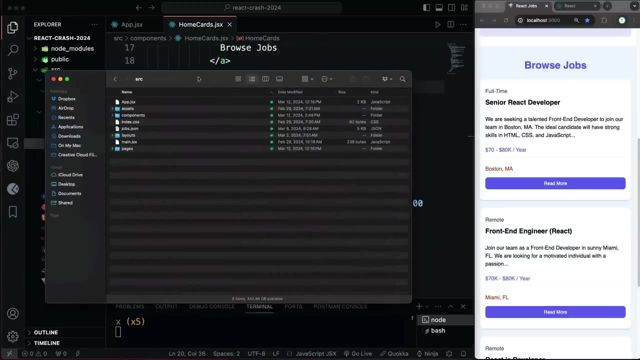 we don't have a back end yet, so we're not going to be fetching these jobs just yet. what we'll do for now is just use a json file. so let's just open up the. so from the repository. in the source folder there's a jobsjson file, so i want you to take that and bring that over to your. 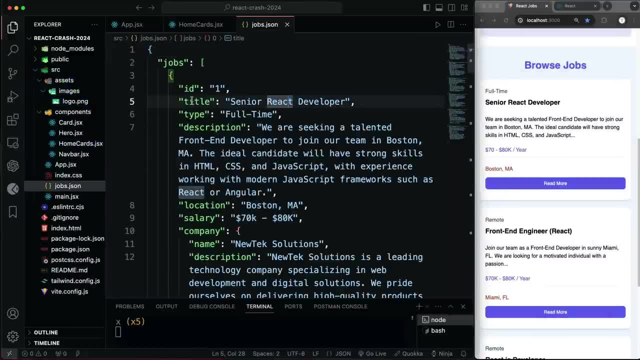 source folder. now, at the moment, this is an object that has a job, a named jobs, array inside of it, and the reason for that is because, with json server, which we're going to use later, that's how you need to format it, but for now, what i want you to do is just just have the array, so we can get rid of this. 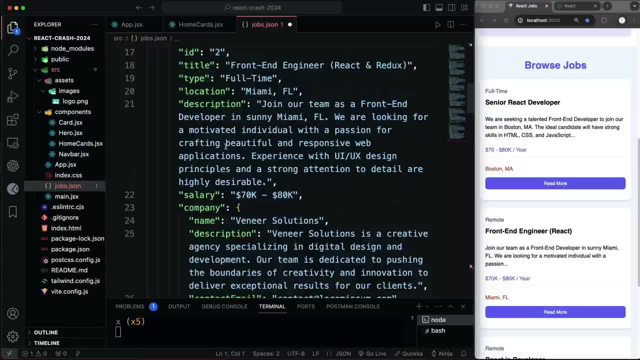 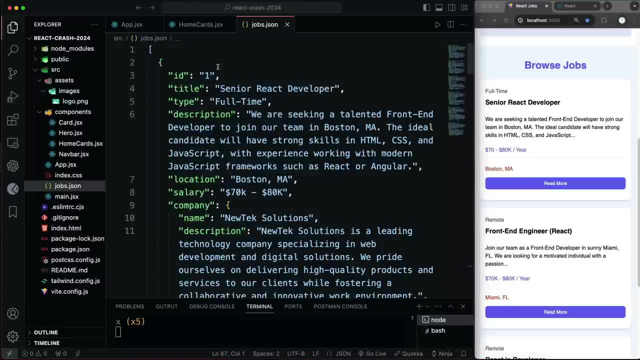 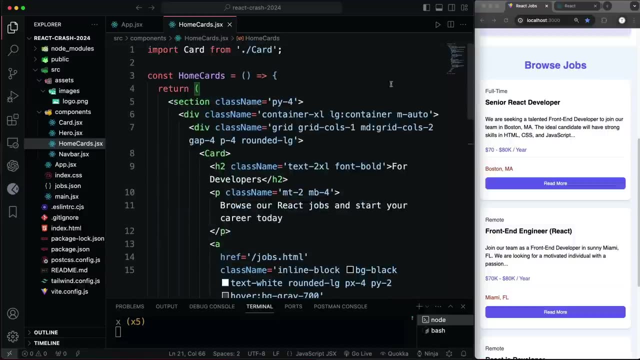 the curly brace and then the jobs. so it just starts with the bracket and then down at the bottom, just get rid of that curly brace, okay, so now we just have an array of jobs and we can bring this into the files, where we file where we need it now we could bring it into, you know, into the 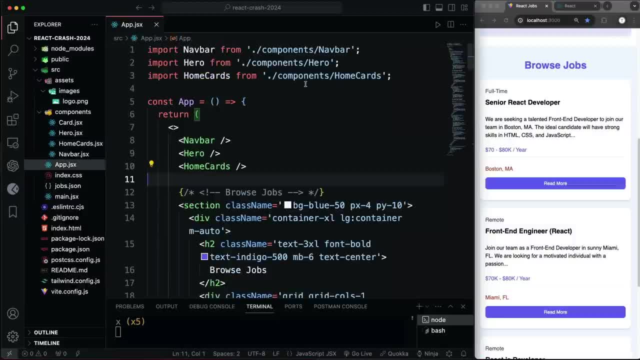 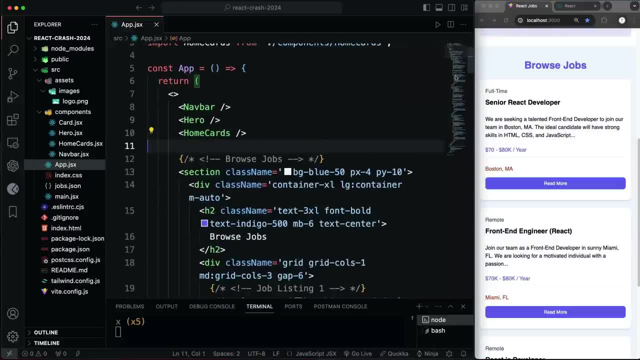 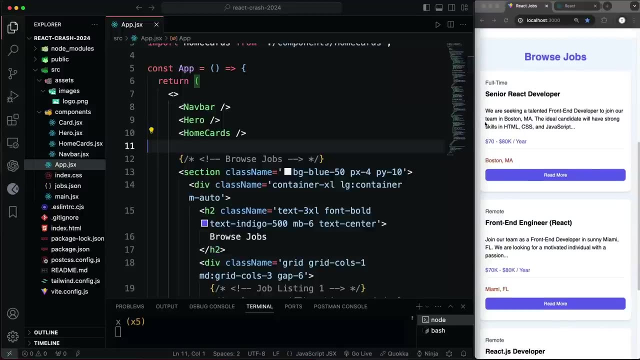 we can close home cards, but we could bring the data into the app component and then we could use it here. but, like i said, i want to keep this app component clean, so why don't we put the listings into its own component and then we'll have a single listing component, which will be you know. 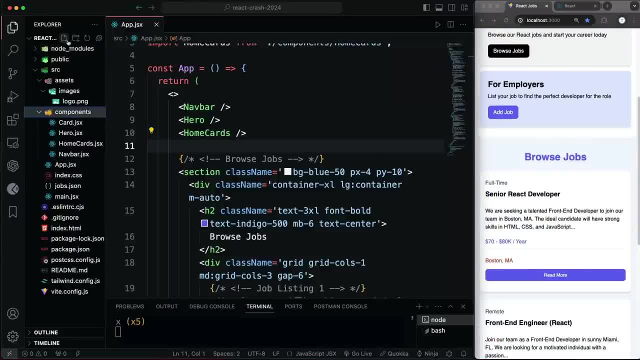 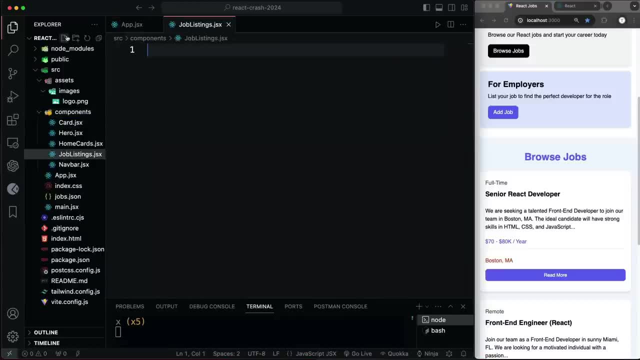 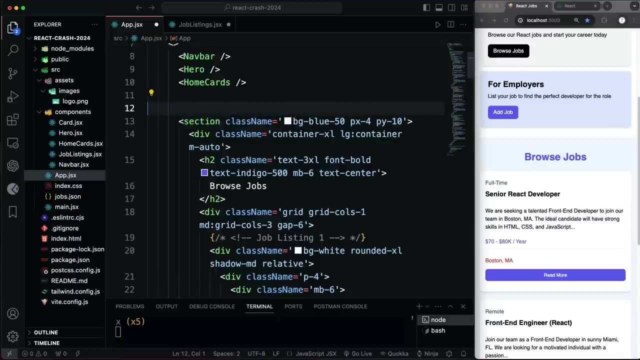 this, this block. so in components let's create a new file and we'll create a new file and we'll call this job listings dot jsx and let's do rafce, and then let's grab from the app this entire section under browse jobs. we can get rid of that comment and then this section see. so this ends. 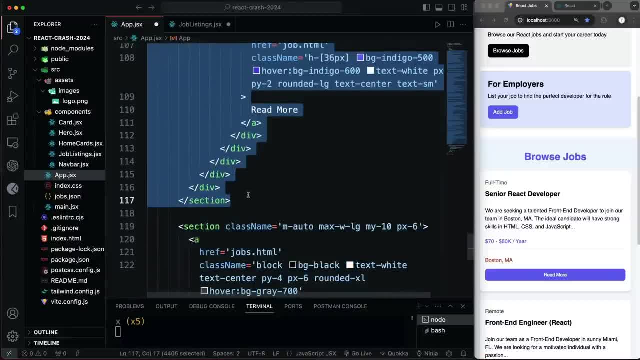 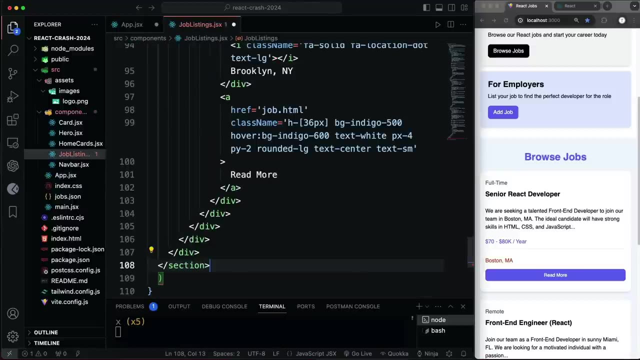 right here. actually, let's see, do we want the? uh, we'll put the. we'll put the other section with the, the view all button, in its own component. so let's just take this one section, cut it and then, in the job listings, get rid of that, paste this in, save it. let's go back to app. let's import. 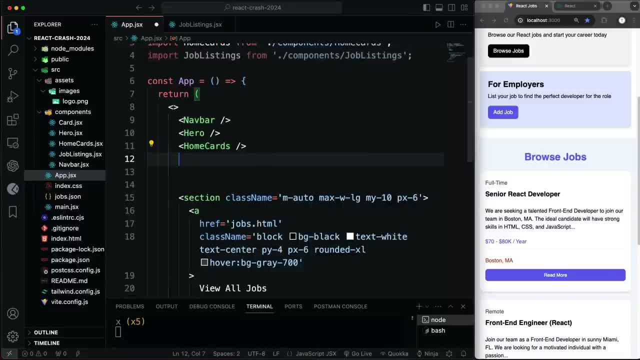 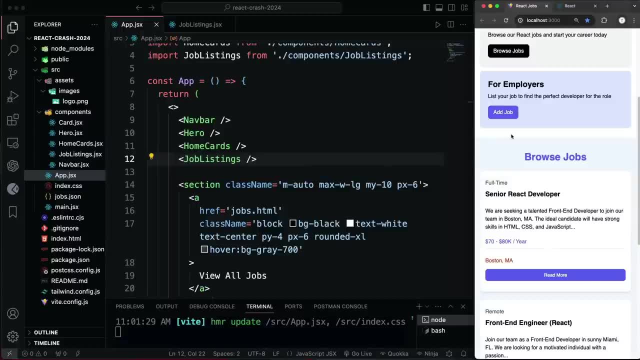 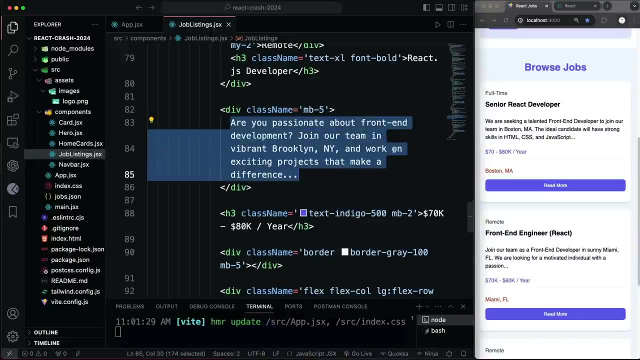 job listings and then let's add it here. so job listings, so you can see how we're cleaning this file up. now it's going to look the same, right, except now this is in its own component. now i want this data because right now, if we look at this, the data is just hard coded in the html. i 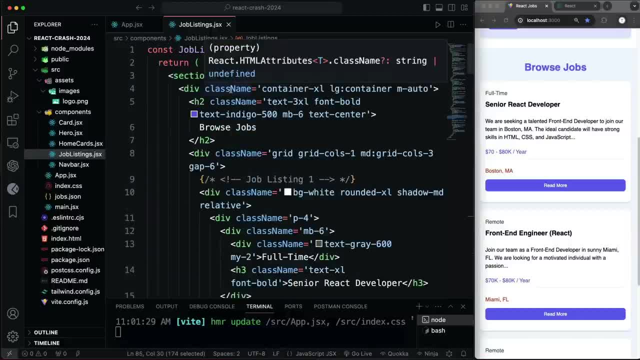 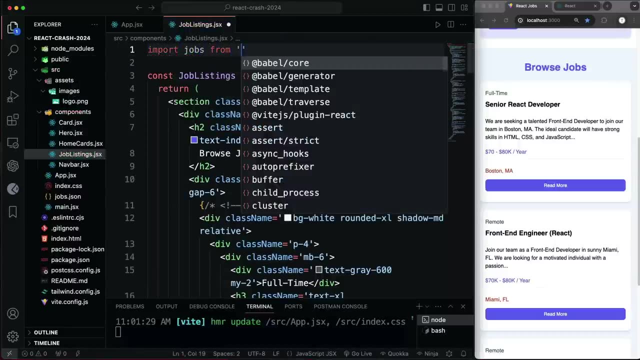 want it to come from that json file. like i said, ultimately it's going to come from json server, which is a mock back end, but for now we'll just bring in the data directly. so we can do that by just saying: import jobs from and we want to go, let's see up one level into, and then we want jobs. 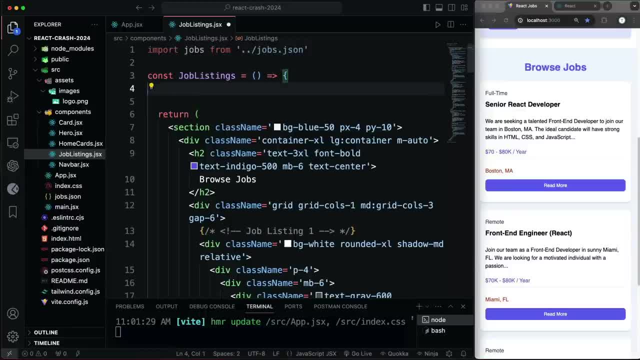 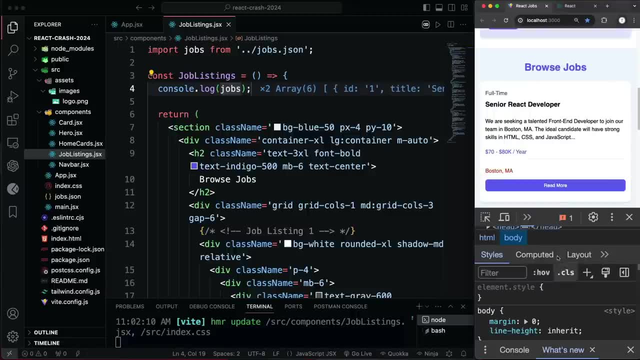 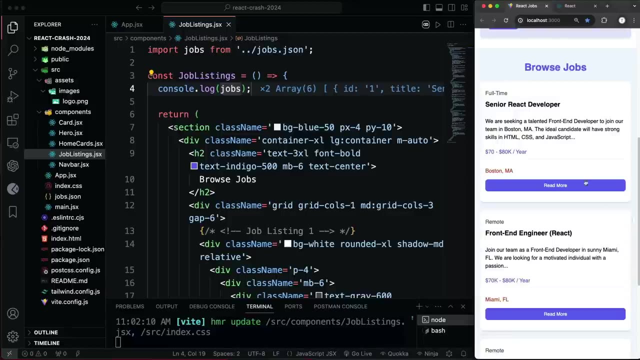 dot json. and just to make sure that we're getting that, we can just do a quick console log of jobs and then if we check out console see we have an array of jobs all right now we want to show those jobs here. so what we'll do, and this right here: 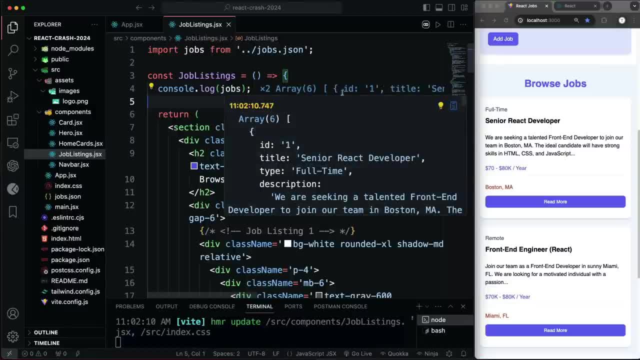 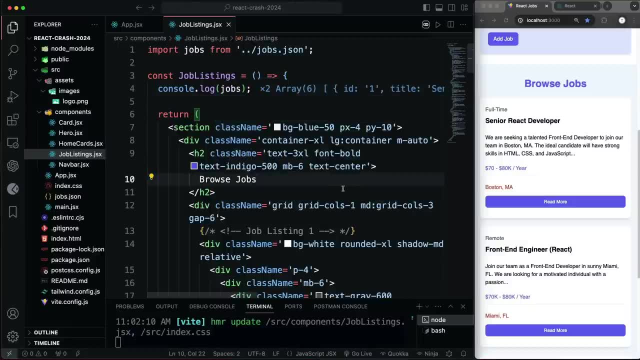 that you're seeing the log in my browser. this is the the console ninja extension, not the browser. my editor. this is from the console ninja extension, if you want to check that out, it's pretty cool. so let's see. we want to create a list. remember i showed you a little while ago that if you have an array, 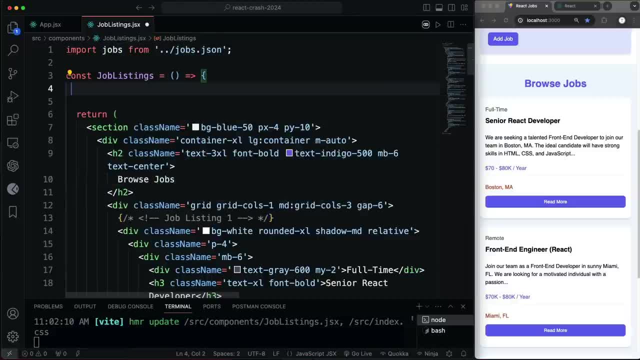 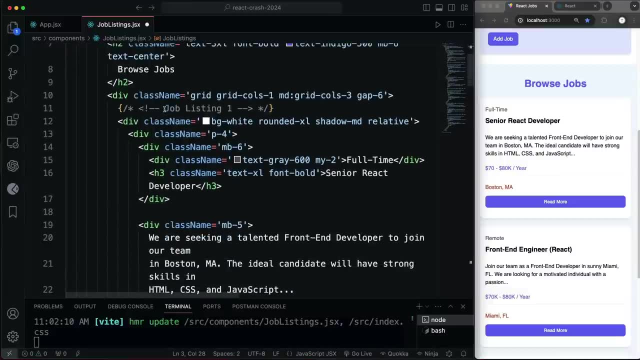 which is is what this is- jobs. you can loop through it and create a list using the map method. so let's figure out where we need to do this. so we have the grid here, so why don't we, inside of the grid, create a list that will have a div like this, with the bg white rounded xl around all the jobs. okay, just like we. 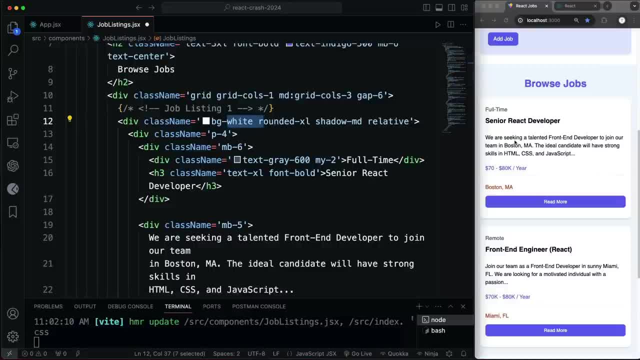 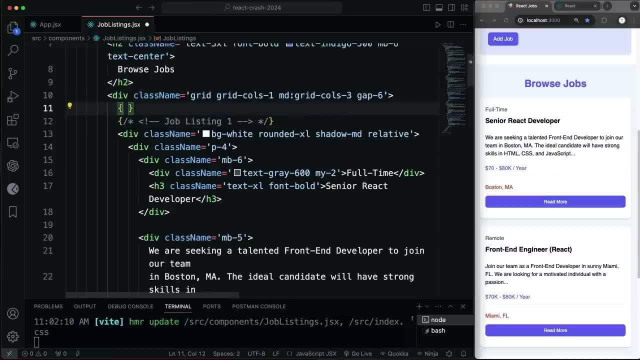 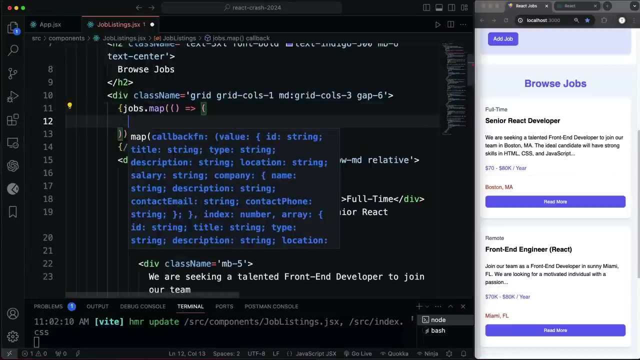 see here same thing, but we'll be using the actual data from the file. so i'm going to go right above where it says job listing 1, and let's take, let's say jobs dot map and then that's going to take in a function and we're going to return some jsx from that and the j and that's going to take job. 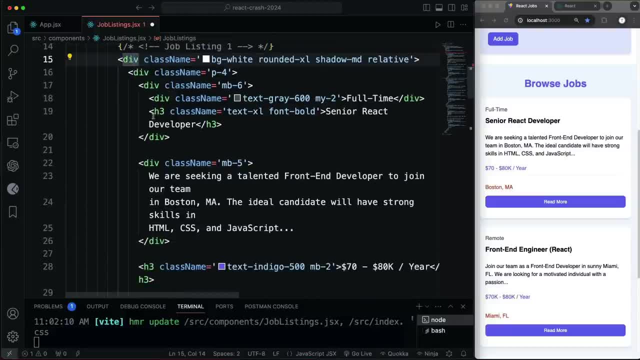 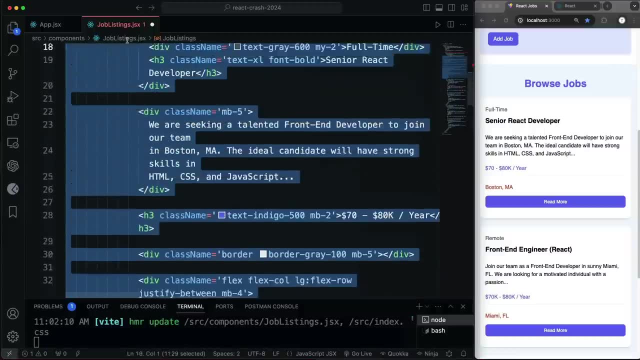 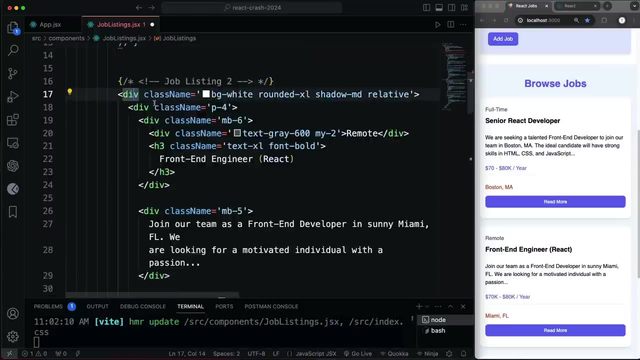 and then the jsx that i want is one of these divs, one of these boxes. so this div which ends right here, i'm going to grab that and i'm going to cut that. okay, we don't need that. we don't need these other listings now. 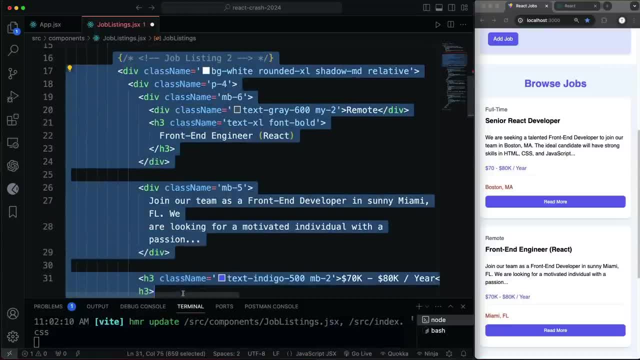 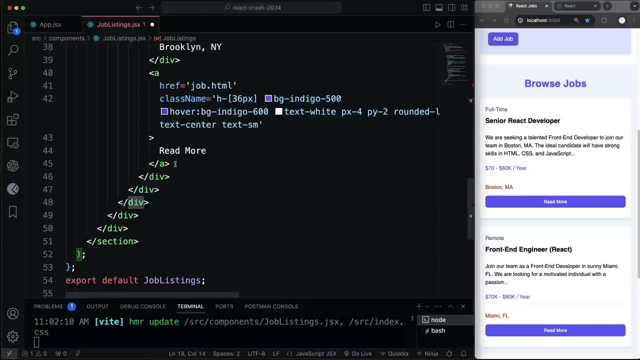 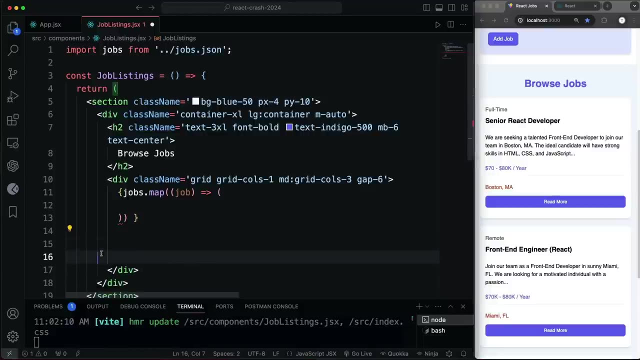 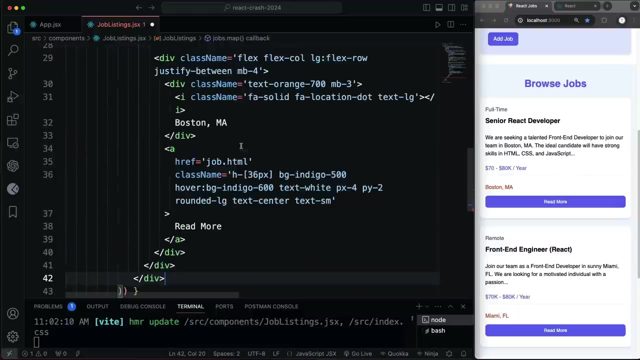 so let's get rid of job listing 2 and job listing 3, which ends right here. make sure, just make sure, you get rid of the right divs, all right, so we're just, we're really cleaning this up as well, and then inside here, right inside, the function is where i want to paste in that single div. now, if 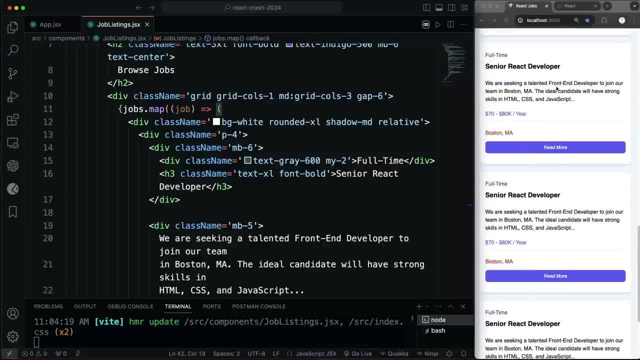 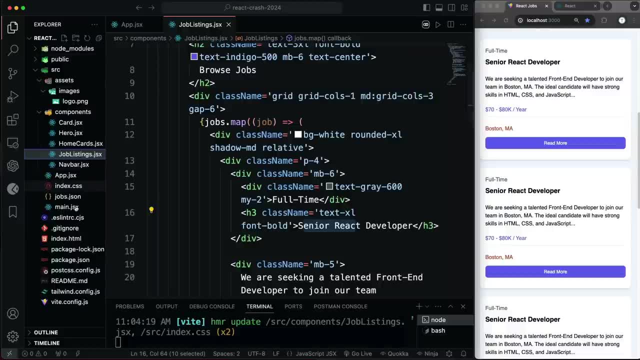 i save this, you'll see it's going to show it a bunch of times. it's showing the same data, because that data is hard coded, but it's showing what? 10, because that's what i have in the json file. so if we look here, we have 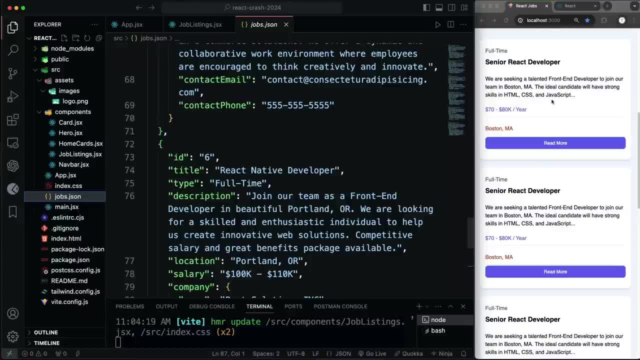 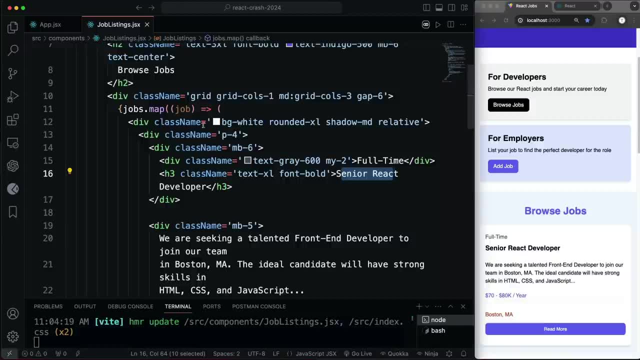 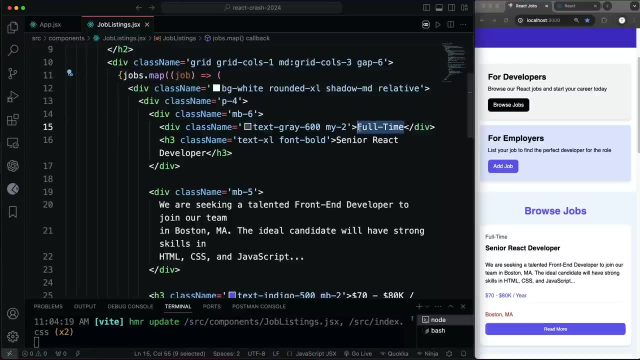 oh no, it's six. yeah, id one through six, so it's showing me six boxes, but it's all the same data. so all we have to do now is replace the hard coded data with the data from each job which we're getting right here. so, for where it says full time, let's change that to job dot and then 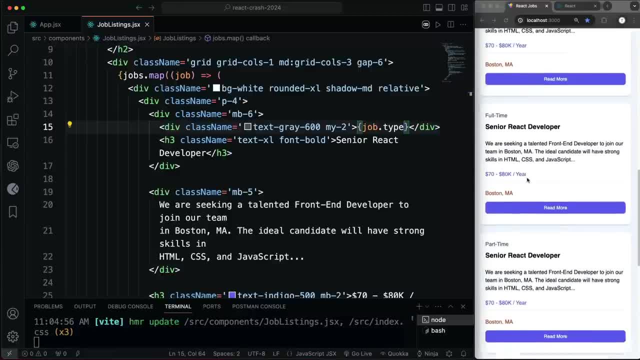 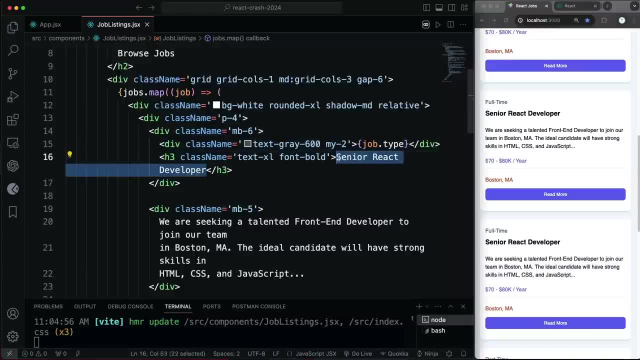 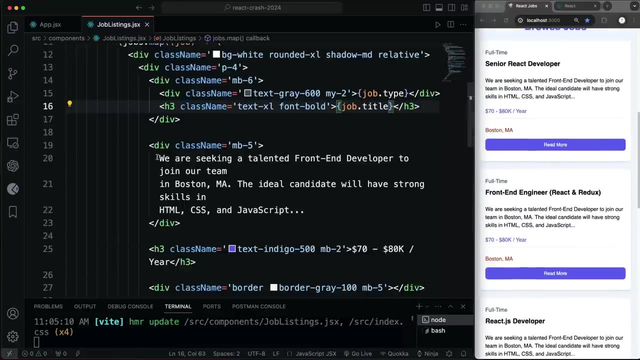 type. so now those should be a little different. full time- this one says part time. okay, so for the this right here the hard coded title. let's get rid of that and let's say job dot title. now all the titles are different. then we have the description. let's get rid of that and say job, job dot. 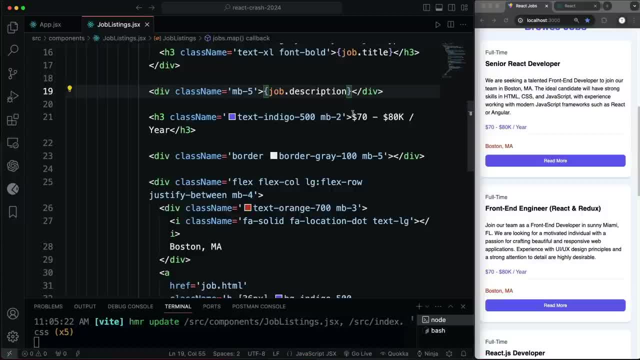 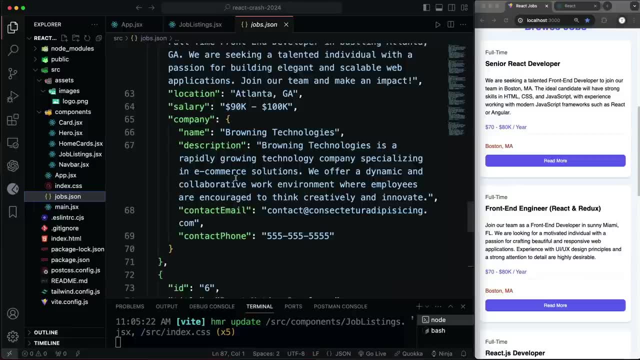 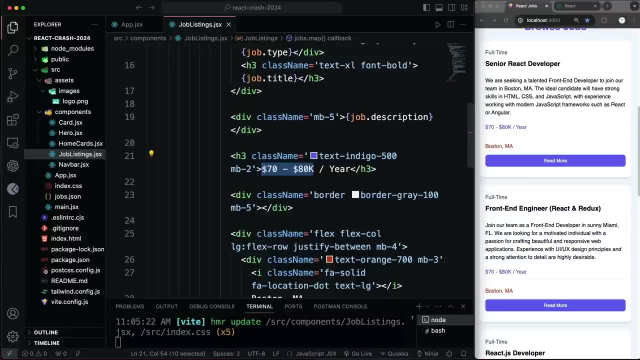 description. okay, now those are different. then we have the salary. so this right here, let me see how those salaries formatted, do they have? okay, so it's just the whatever k to whatever k. so the slash year will leave there, but we'll replace this with job dot salary. 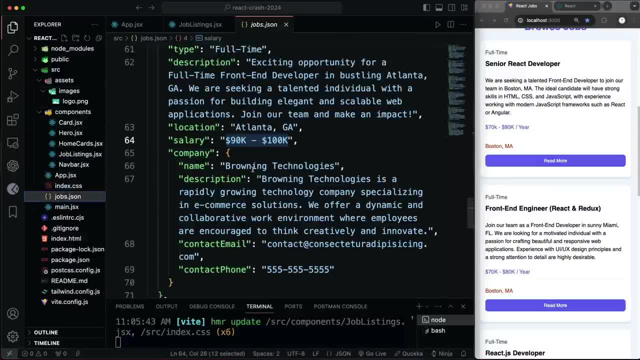 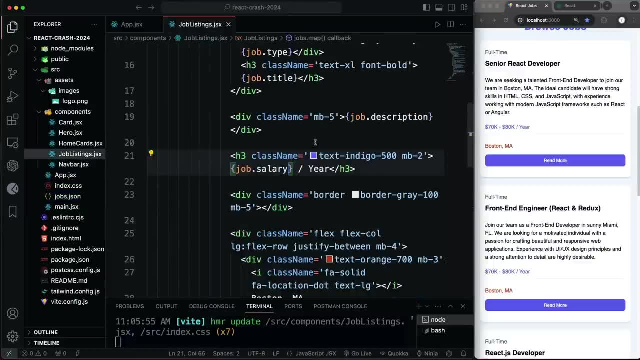 uh, that should be a big k. let me just fix this, all right. so let's see what else do we have here, the location. um, and, by the way you see, this is the job dot salary. so let's see what else do we have here, the location. 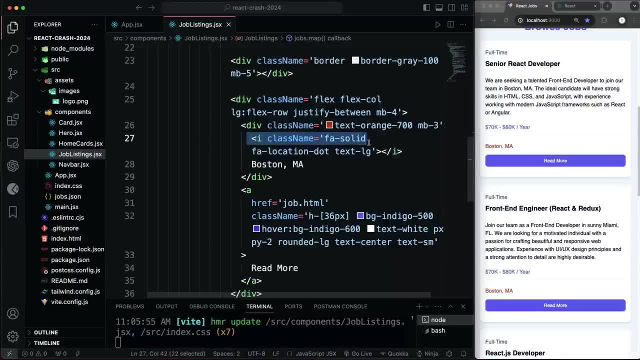 and, by the way you see, we do have the font awesome i tag here. we don't. we're not using the font awesome cdn, so it's not showing up the little map marker. but i'm going to show you an extension that we can use, called react icons, where you can basically bring in your font awesome icons. 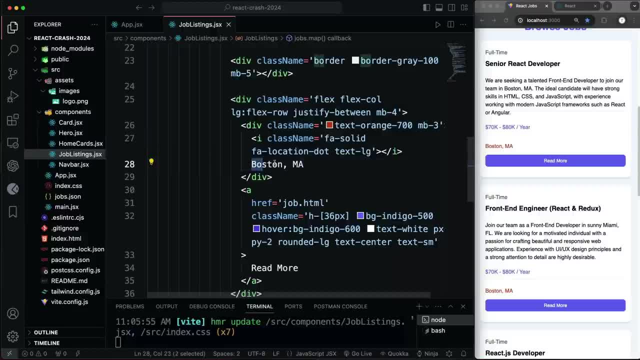 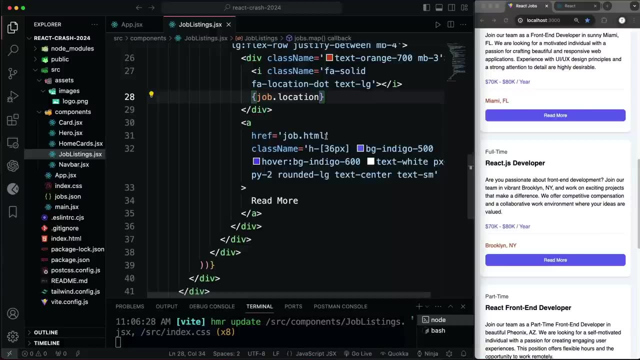 as a component, but we'll do that in a minute. let's change this to job dot location and now you can see that the locations are different. and then, finally, the link here is going to job dot html, which obviously isn't correct. ultimately, we want to be able to go to our website slash. 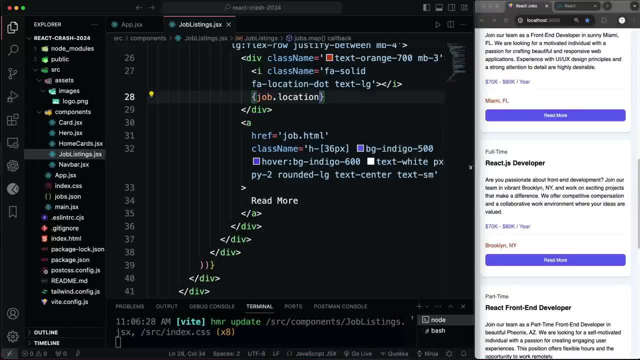 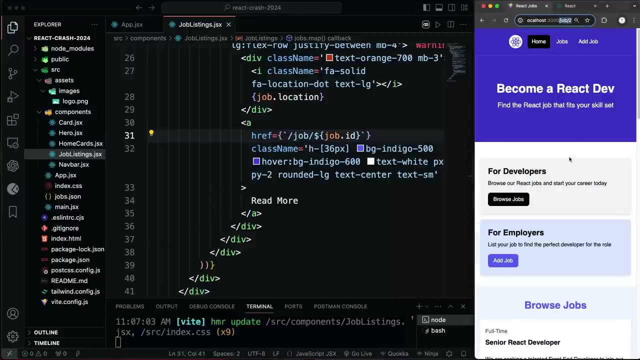 and then jobs and then slash whatever that job id is. so let's change this to template literal so we'll put in some back ticks and we'll say slash, job, slash, and then we want the id, so job dot id, like that. okay, so if i click it it's going to go to job slash two in this case. 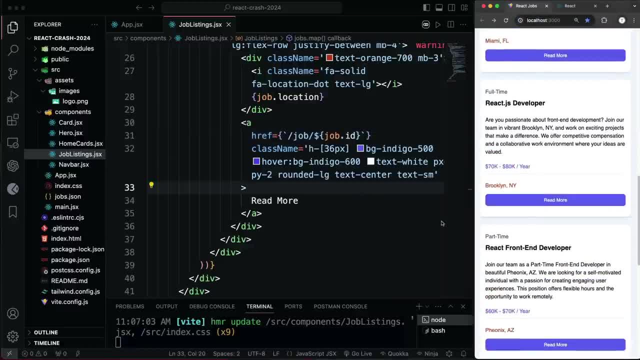 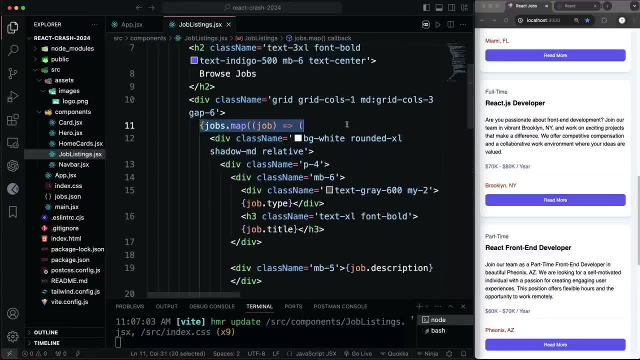 which doesn't exist yet, but that's fine. now, another thing i'd like to do is to make this an actual component, because right now in our job listings- yes, we have a list, but we're just outputting a bunch of html. let's make this into a single component that we can then show for every. 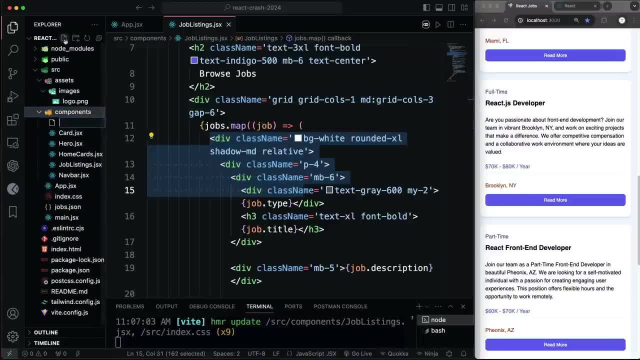 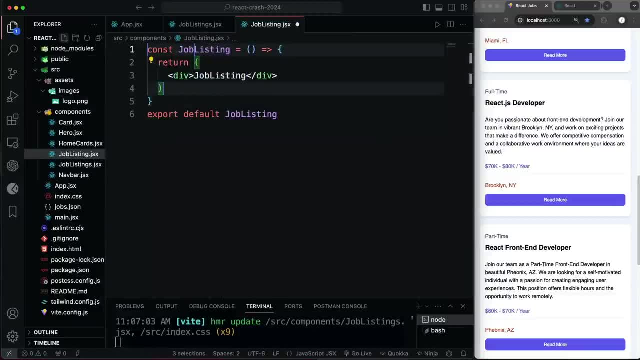 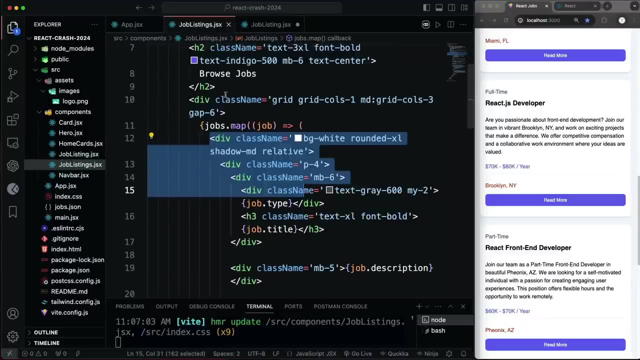 job. so in components let's create a new file called job listing, singular dot, jsx, rafce, and then that's going to take in as a prop. we'll destructure and that's going to take in a job, and then what we can do is in the job listings. 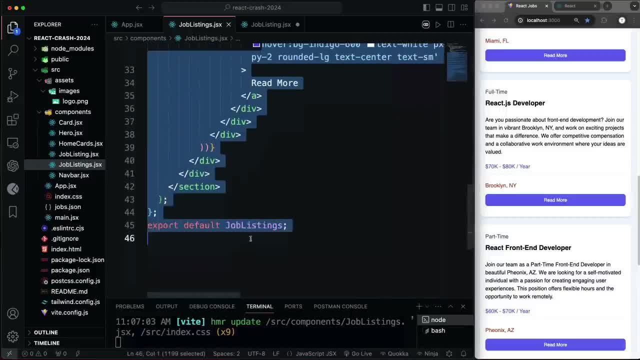 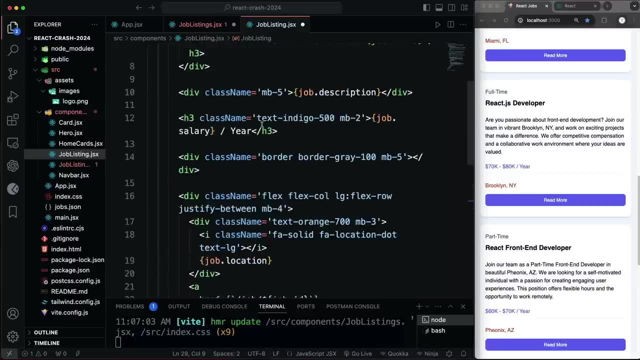 within the map, this div we're going to grab that ends right here we're going to cut it and then here we want to paste that in and basically it's going to get passed in that job prop and then we'll use it in the job listings and then we're going to take in a job. 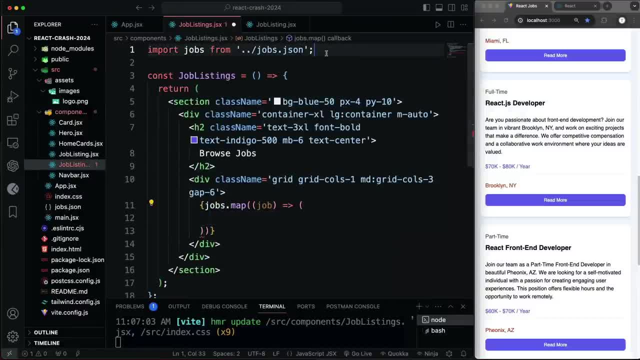 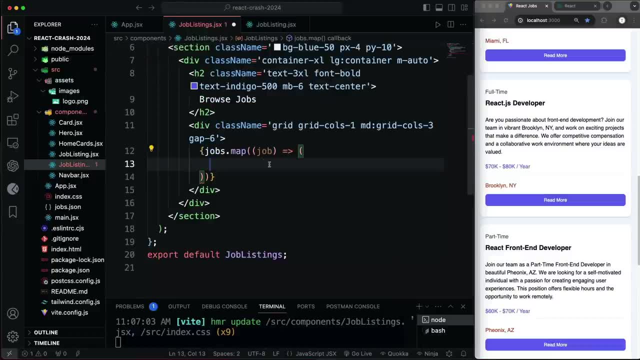 in all these different areas. so now in job listings we can simply import job listing, the singular, and then what we want to render for each job is going to be job listing and it's going to get passed in a job prop. okay, now remember, when you have a list it also has to. 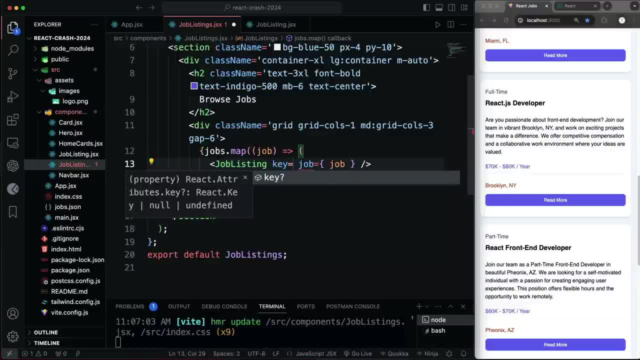 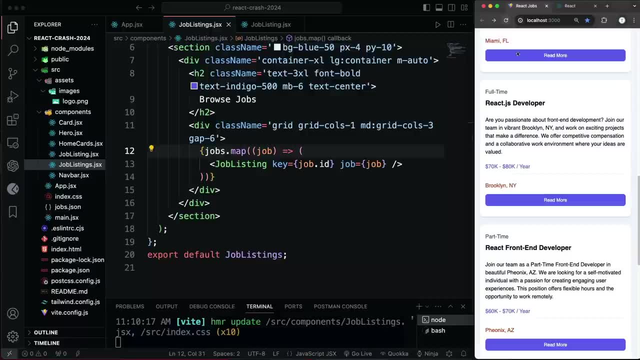 have a key or you're going to get that, that error. so let's say key equals and i'm going to set that to the jobs id because that's going to be unique. remember, it has to be a unique value. so if i save and reload, you can see that it's still. it's working. 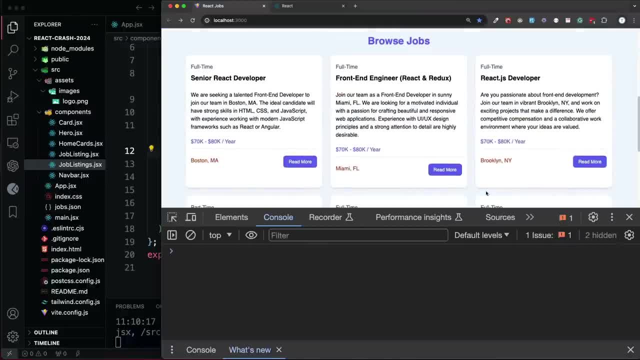 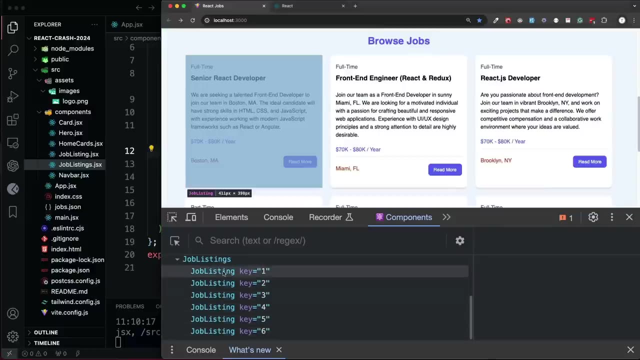 okay, and if we look at the dev tools here, if we go to components, you can see all of our. you can see our tree of components. navbar hero in the home cards we have two card components. in job listings we have six job listing components. all right, and if we look at that, you'll see over here. 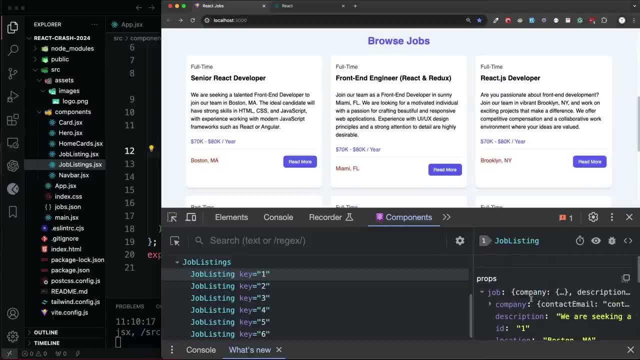 the props, which is all the job data, so you can see how the job listings are going to be, how this ui is nice and organized. now right, everything is in ui components and it's easy to manage. so if you were using just vanilla javascript, you would have this giant monolithic. 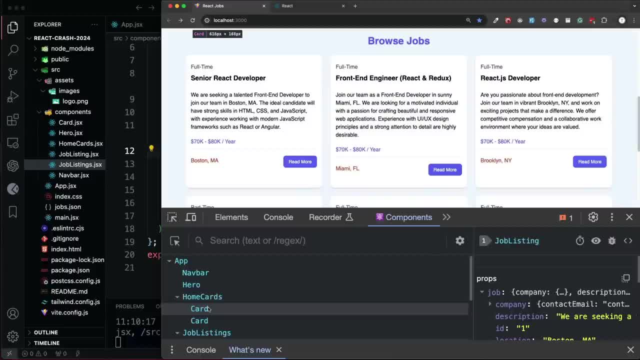 file where you're just selecting all these elements using whatever query selector, and then you'd have to just create all these different functions and it's just. it gets very messy. but with react, or not just react, but any front-end framework, you have everything nice and neat for. 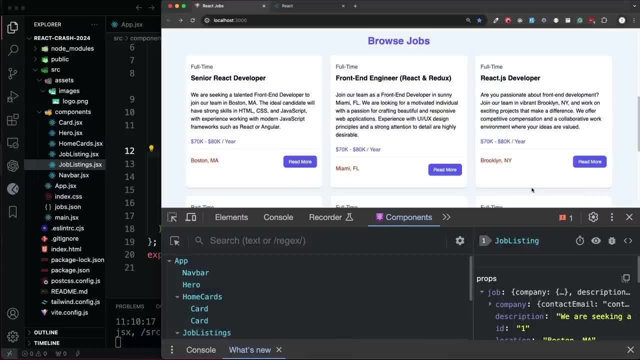 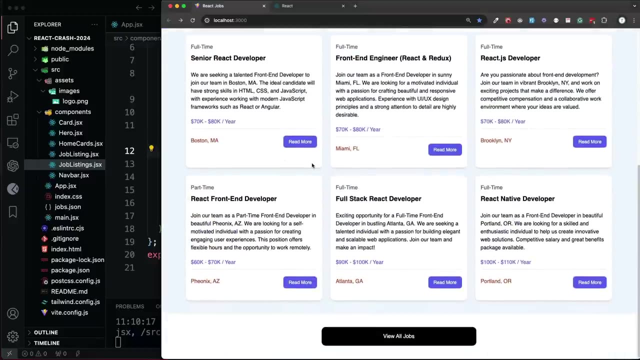 you ui okay and it might seem like more work at first, but as you your application scales, you'll be, you'll learn to appreciate it all right. so on the home page, i actually don't want to show all of these, i only want to show three. but i also want to use the same job listings component when we get to the 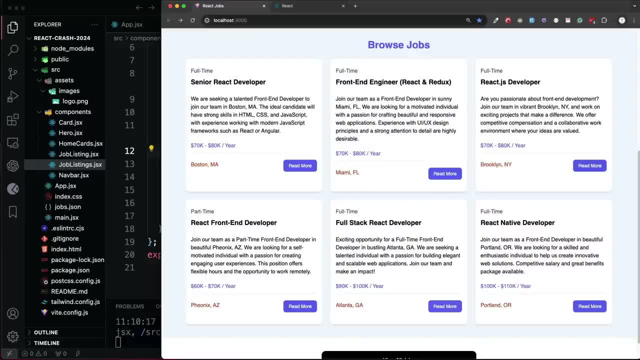 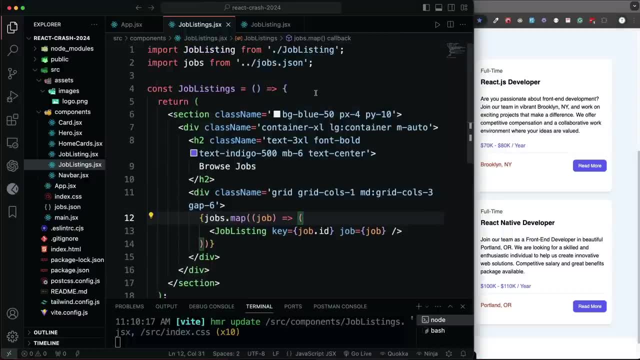 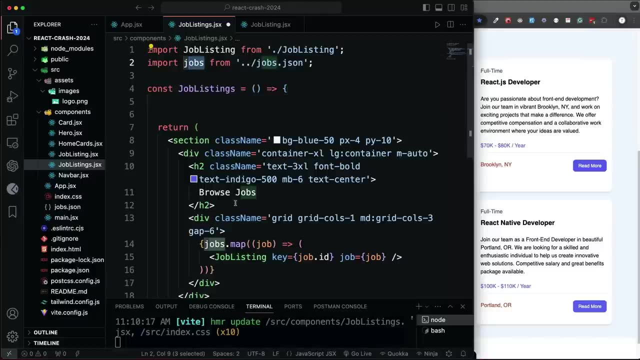 jobs page. so i'm trying to think of how- how i want to do it right now. i think i'm going to do it right now. let's just go to job listings and what we can do is, uh, let's see, instead of just using jobs directly down here and looping through, let's do this. let's say, const recent jobs and let's 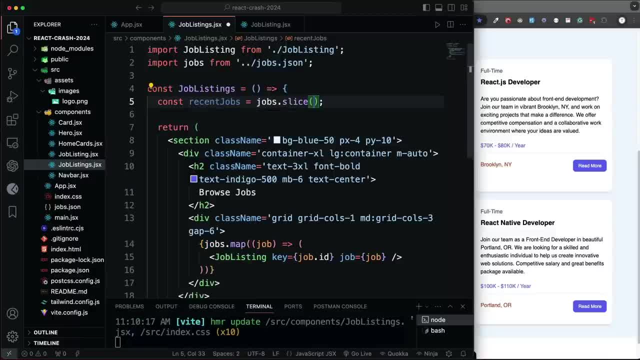 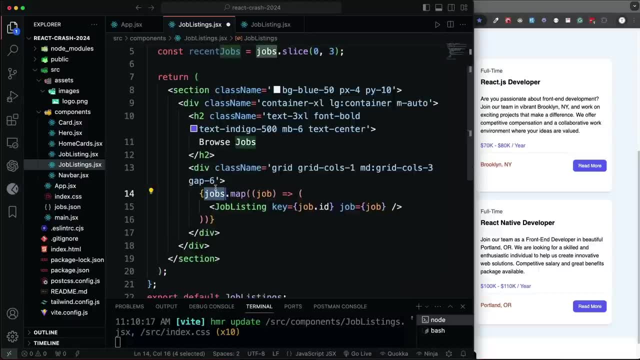 set that to the jobs array, and then we're going to use slice and we'll say: we want to get from zero to three, so we only want the first three, and then we'll replace this with recent jobs. so now it's only going to loop over those three. save that and there we go. 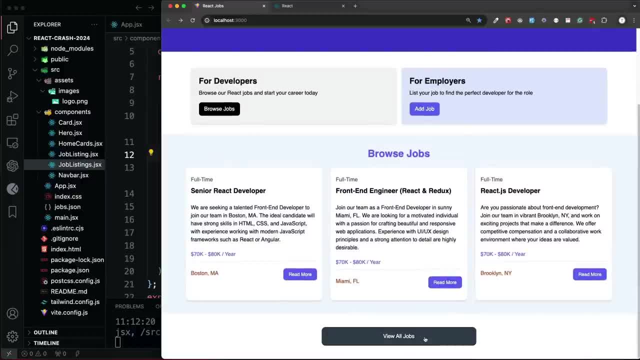 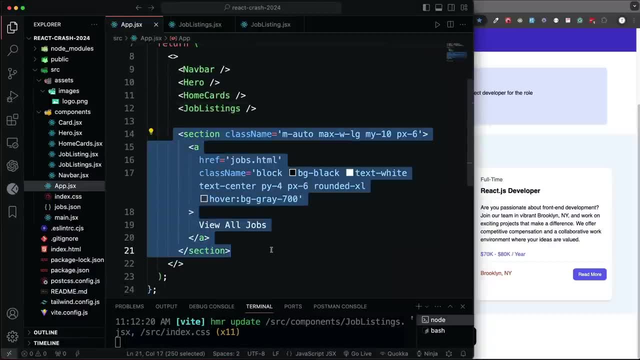 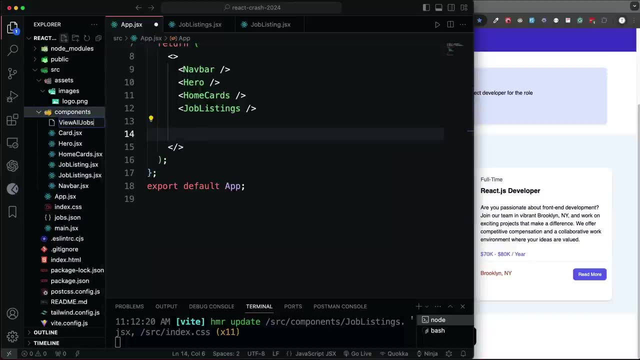 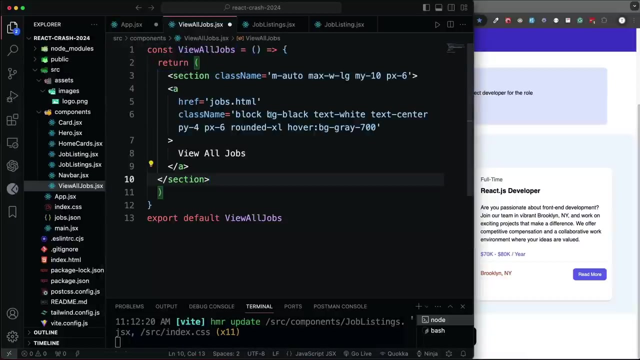 all right. so this final thing, this button: if we look in our app js, that's the last thing we have, so let's put that in its own component, so we'll cut that section. and then in components let's create view all jobsjsx- r-a-f-c-e and we'll replace this with that section. 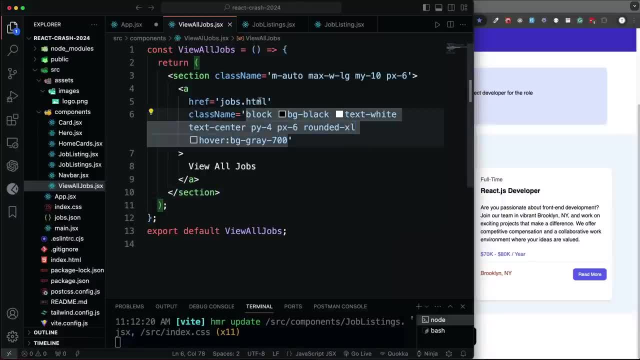 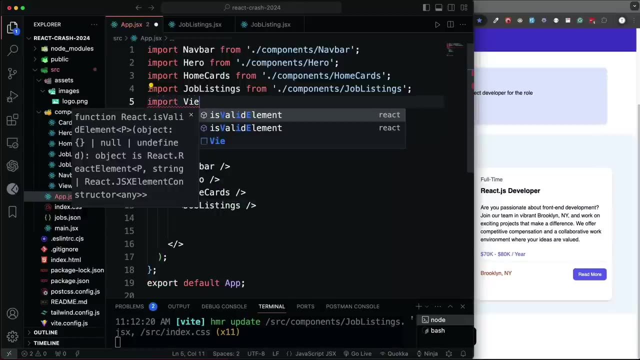 okay, and for the link here, let's change that to just slash jobs, because when we start to use the router, that's what it'll be and then in the app file we can just bring that in. so import view- um, what i call it- yeah, view all jobs. why isn't it coming up? 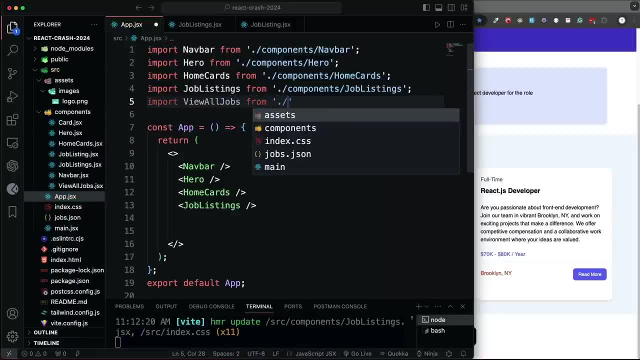 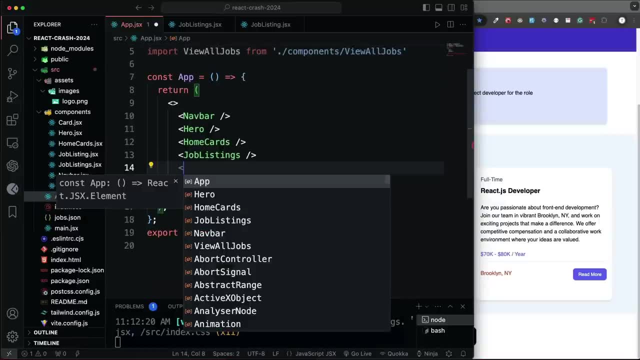 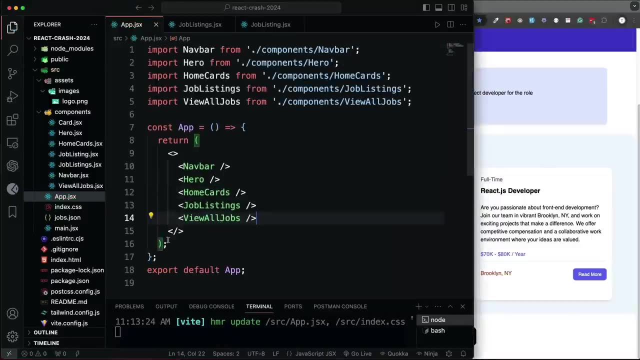 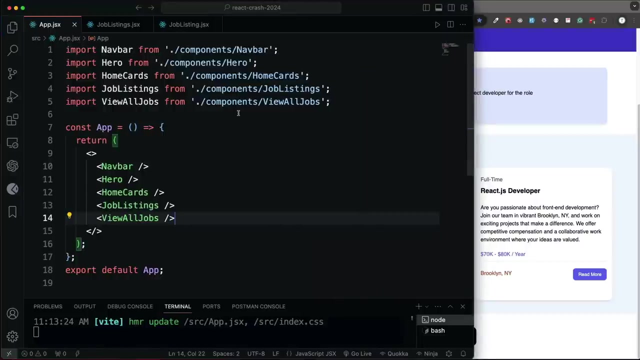 dot, slash, slash, view all jobs and then embed it here, save it and there we go. so now our app file is nice and neat. so what i'd like to do next is get into state a little bit and the use state hook. so remember there's two types of state. you have component state, which relates to a single component, so one. 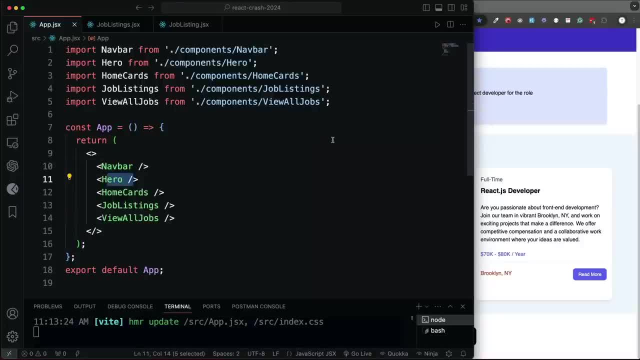 of these right now: bar hero- and then you have app level or global state, and then you have the global state which you can- it relates to the entire app and you can pass down to components. so what i want to look at now is is is component state, and i want to go into the job listing 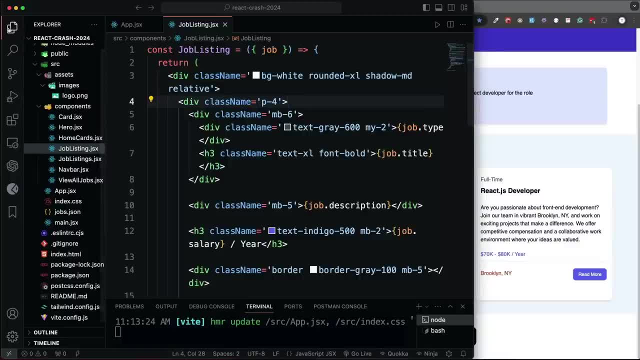 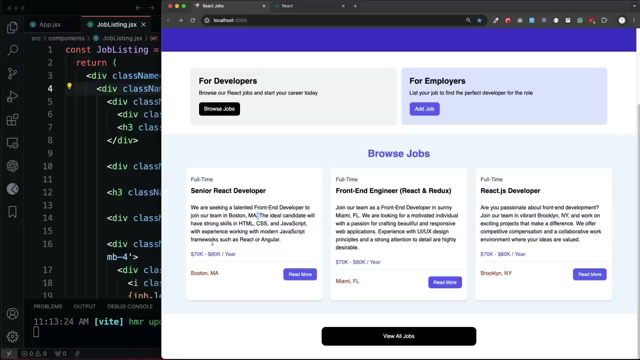 component. so this right here, and basically i want to be able to toggle this description from being short where it ends around here, and then we can have a button that says show more, that we click and it'll show them, and then we can go into the job listing component and we can go into the job. 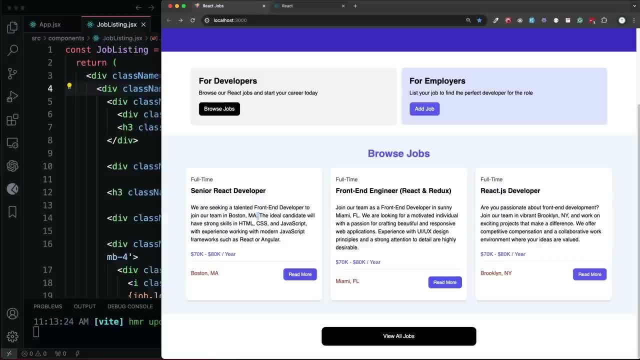 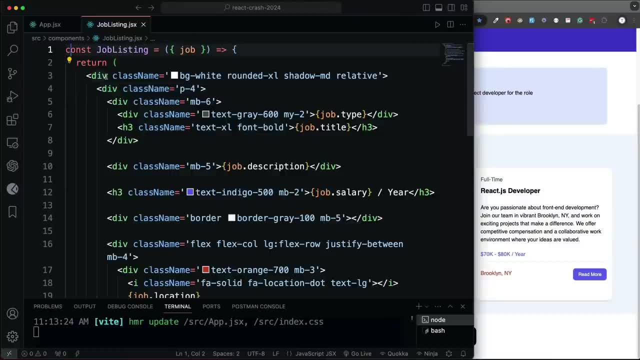 listing component and it'll show the rest. so basically, we'll have a piece of state called show full description. okay, and we can change that based on if we click that button. so let's come up here. and if you're going to add state, you need to use the use state hook. so we're going to import use. 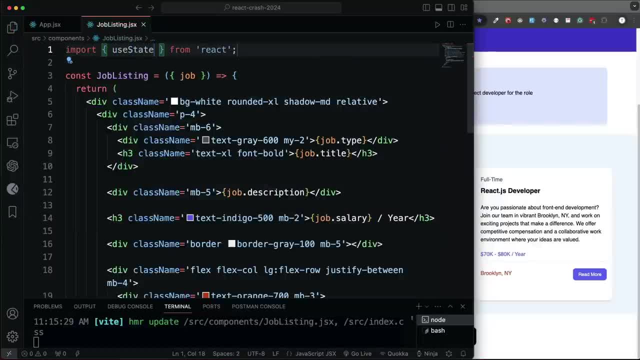 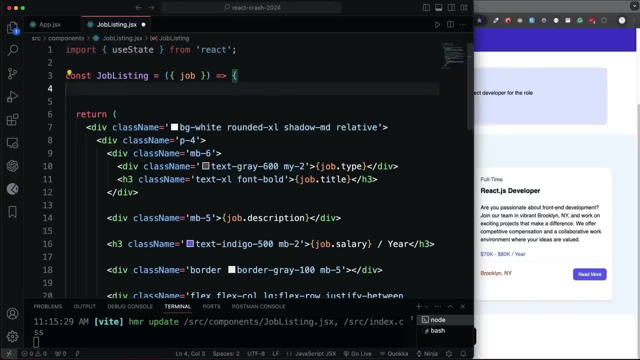 state and that's going to be from react. okay, now, the way this works as i briefly showed you in the slides, we're going to come above the return, the output, and we're going to have an error or some brackets here and we want to set that to use state. okay, now, this is going to pertain to the 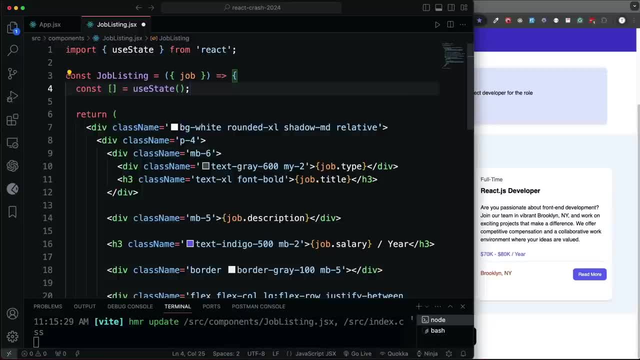 the show full description, and it's going to be a true or false value and in here you want to put whatever you want as the default. so i'm going to say false, i don't want it to show. uh flask false, i don't want it to show by default. and then in here we have two things: the name of the state, 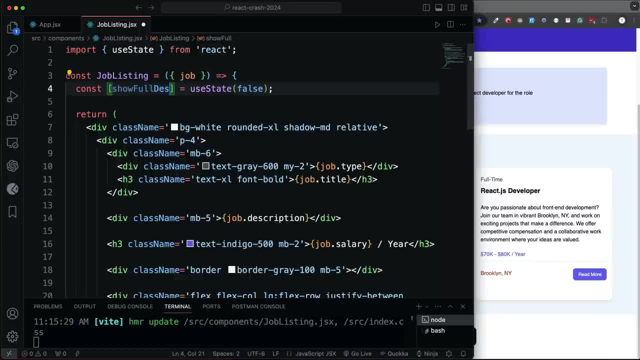 itself, which i'm going to call show full description. And then the second is going to be the name of the function that we call to change that state, And it's going to be whatever this is with just set in front of it. So, in this case, 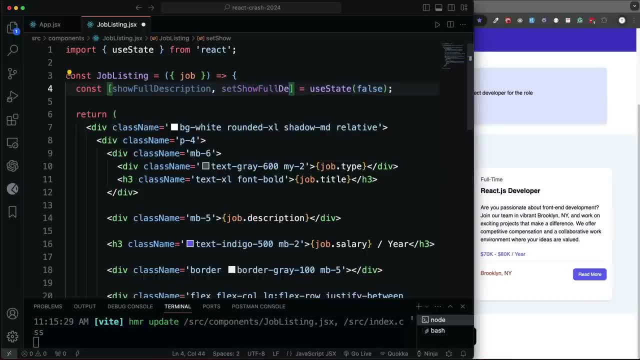 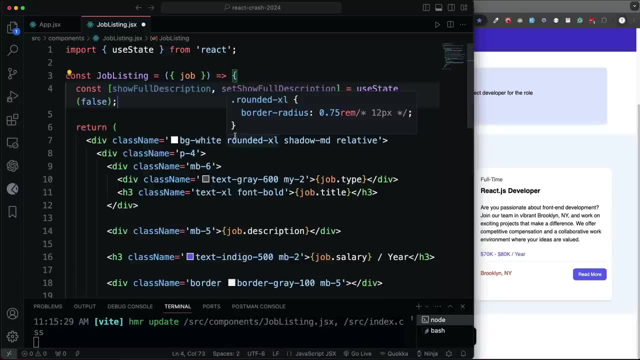 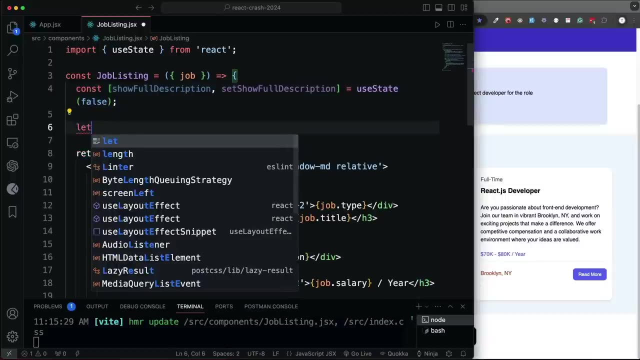 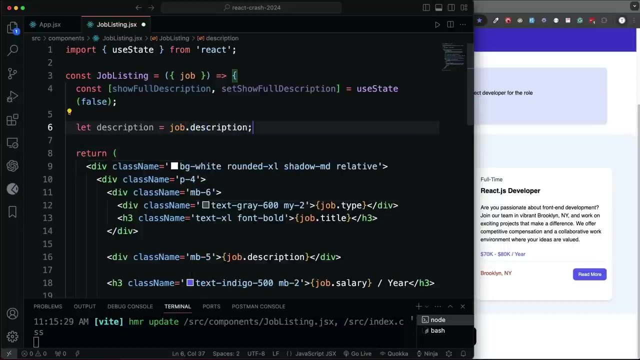 it would be set show full description in camel case. All right, so now let's get the description. So I'm going to go right above the return here And I'm going to say let description. and I'm going to set that to the job dot description, That's you know the job that's being passed in for each. 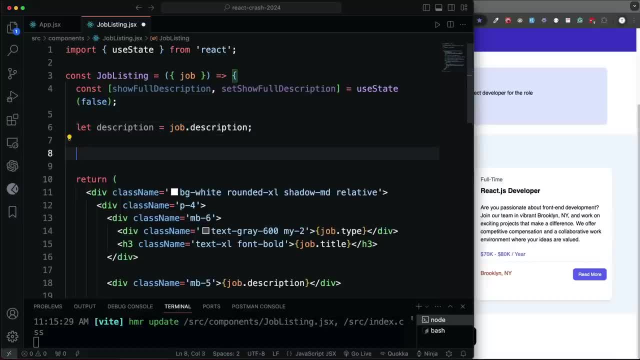 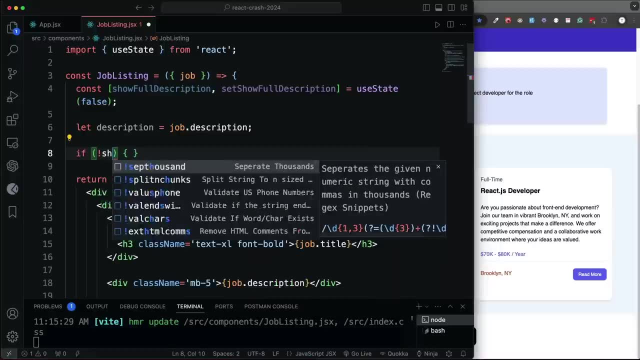 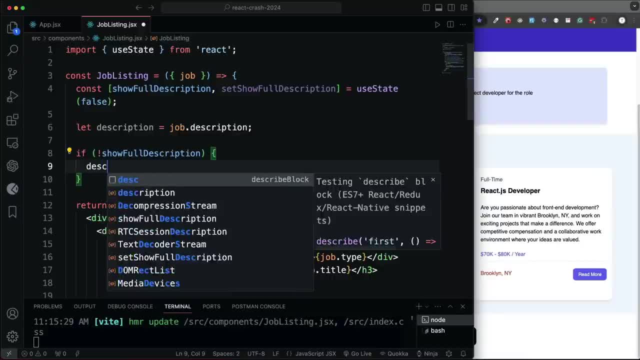 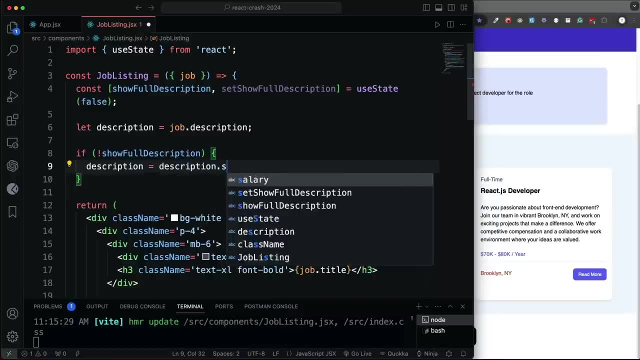 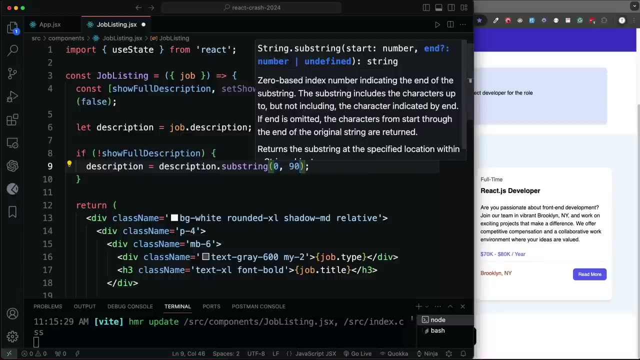 basically just cut off some of it. So we'll take that description And we'll set it equal to whatever that, just whatever that description is, except I'm going to use the substring method to cut it a little bit, So we'll say zero to 90. And then I want to add on to it in ellipses: 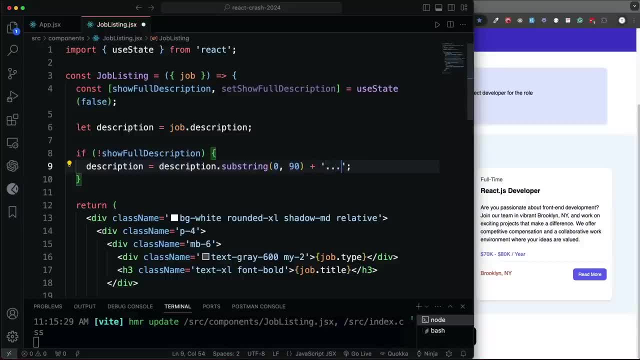 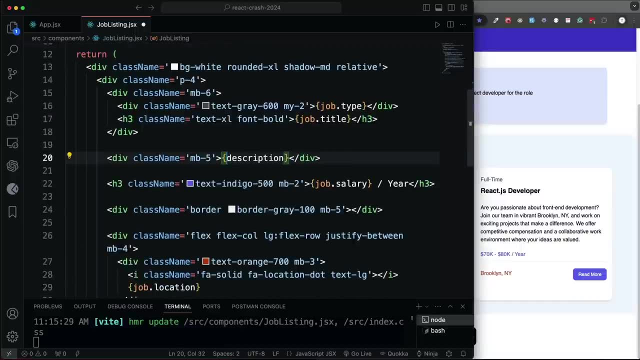 the three dots. So I'm going to concatenate three dots onto it And then what we can do is just replace job dot description. So now, if I save that, you can see that they all got shorter and they have the little ellipses on. 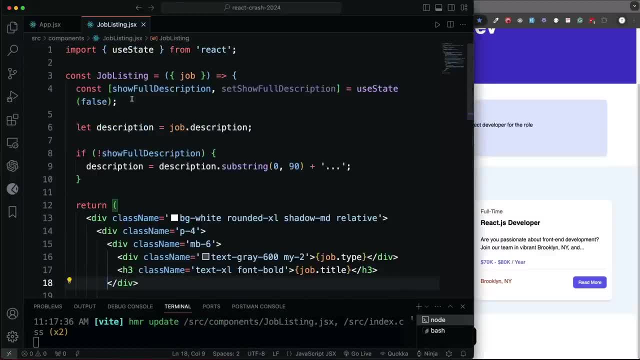 the end, All right. so just to kind of reiterate, I haven't done anything with this state yet. All we've done is take the job description And if the value of show full description is false, which it is by default, then it's going to cut off. Okay, it's going to cut off after 90 characters and add: 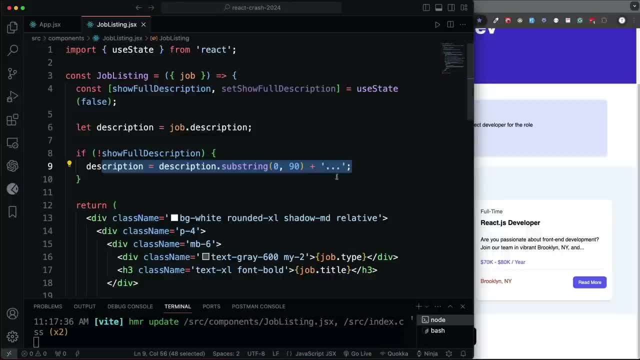 the ellipses. So now, if I save that, you can see that they all got shorter and they have the little buttons. So now we want to have a little button that we can click- and this is going to get us into events as well- But we want to be able to click that and show the full description So we can call. 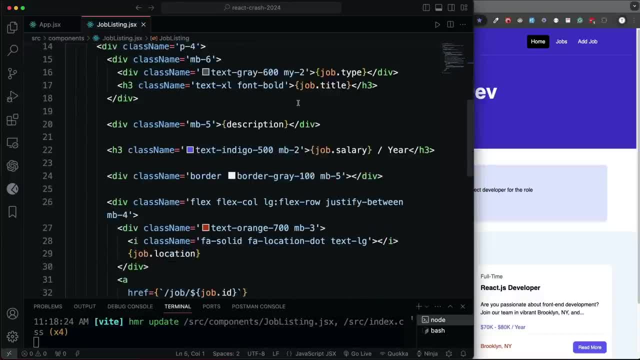 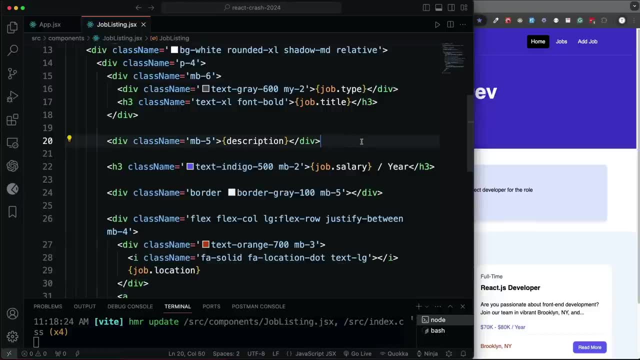 this to change that, And so let's go down here and let's add that button. So I'm going to put it, I'm going to go right under the description, which is right here, Okay, and then we're going to add a. 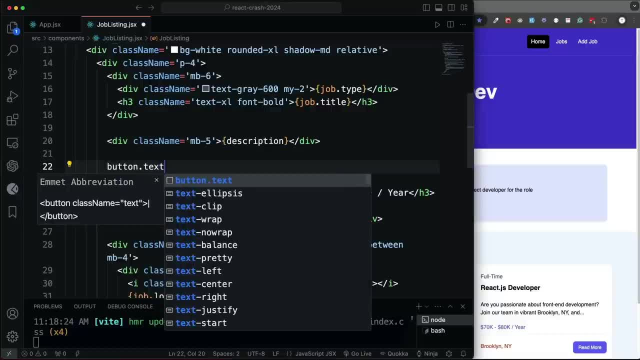 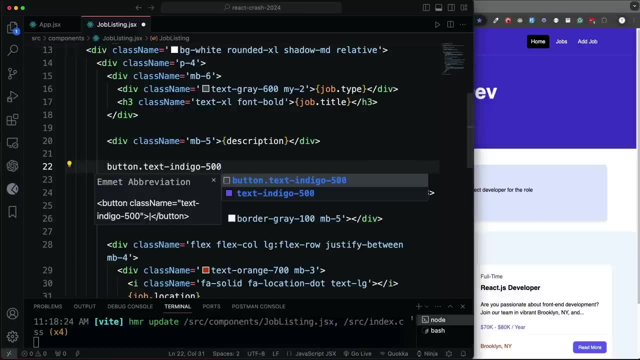 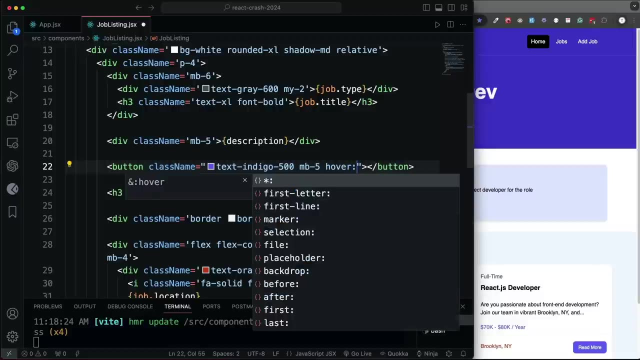 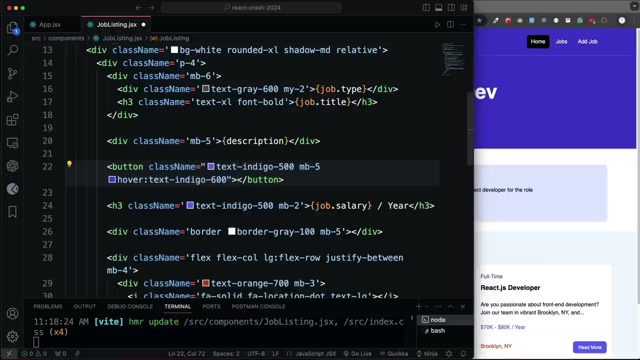 button And I'm going to add some classes to this. Let's do text dash indigo, Text indigo 500. And let's do margin bottom five. And then I'm also going to add in on hover. then we want text dash indigo, dash 600. And then in the button text. So this I want, this is going. 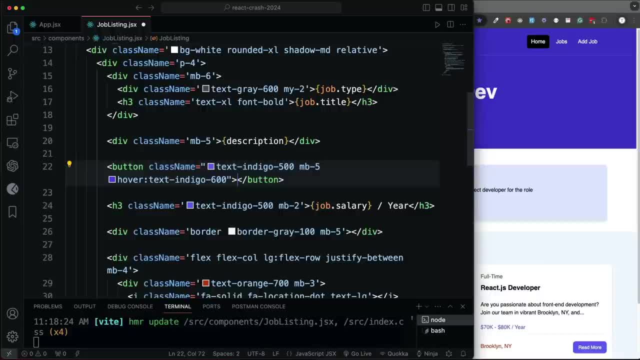 to depend on the state. Okay, so this is where we show something different, based on the state. Well, we've already done that with, you know, cutting it off short, But I'm going to have a conditional in here, ternary, And I'm going to say: if showed, if show, full description is true. 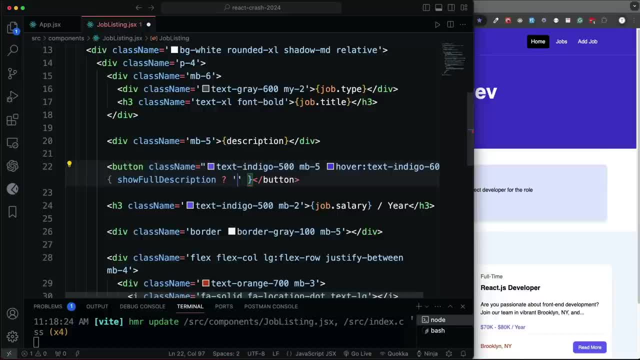 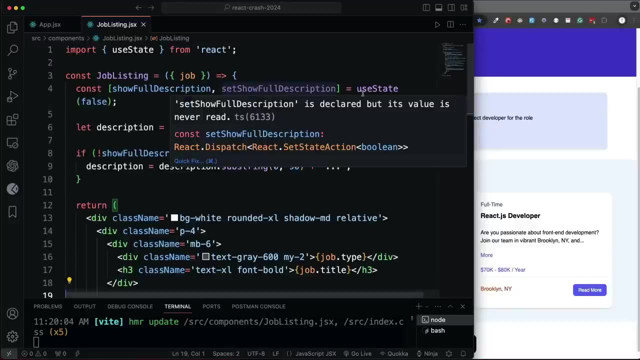 then I want this: I want this text to say less else than I want it to say more. Okay, so if we save that, check it out So it says more, because set set show full description is false. If I make it true by default, it's going to show all the text and then this is going to: 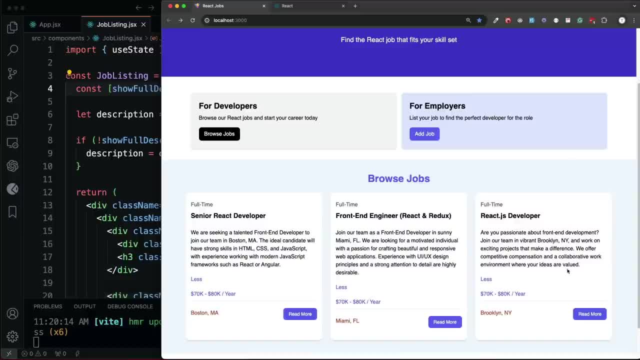 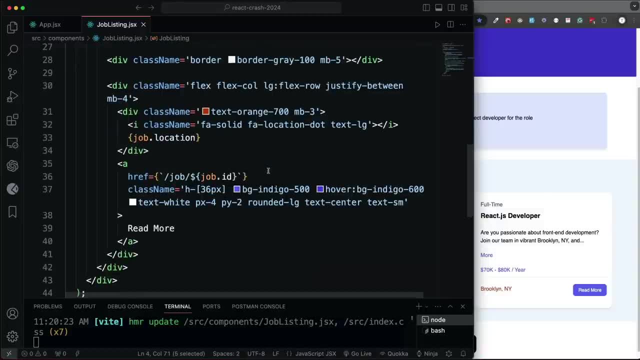 say less So you can see just the value of that state changes my component, So I'm going to put it back to false And then let's make an event. So when we click that, we then set that state to just the opposite. if it's true it'll be set to false, if it's false it'll be set to true. So to do that. 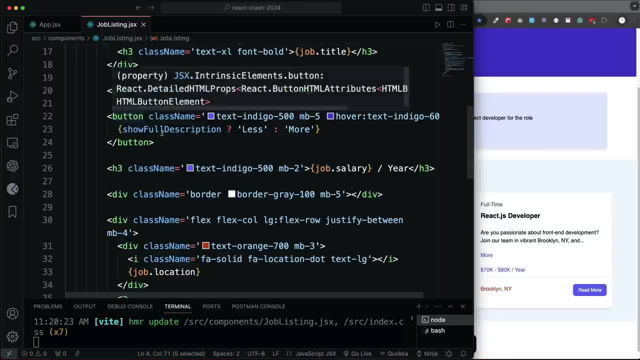 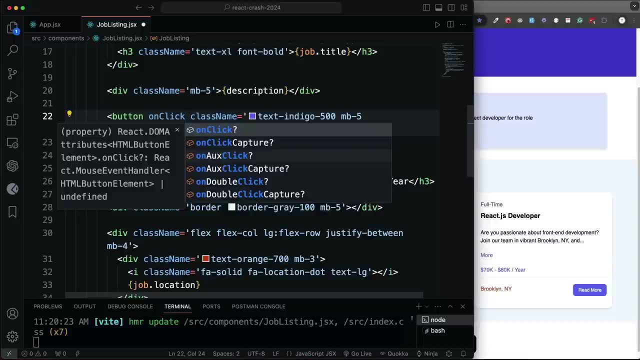 let's go to the button And let's add: Just put it right here. we're going to say on click. So when want to add an event, it's going to be on click. you have um on submit and it's going to be camel. 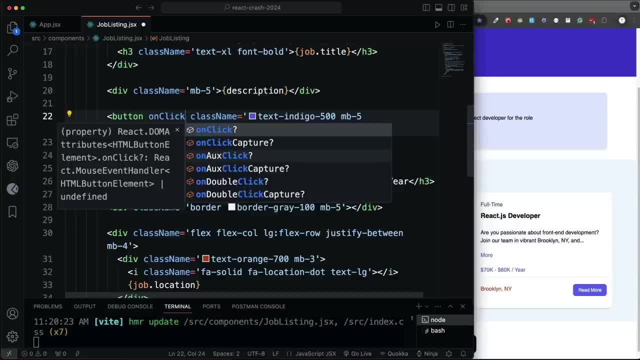 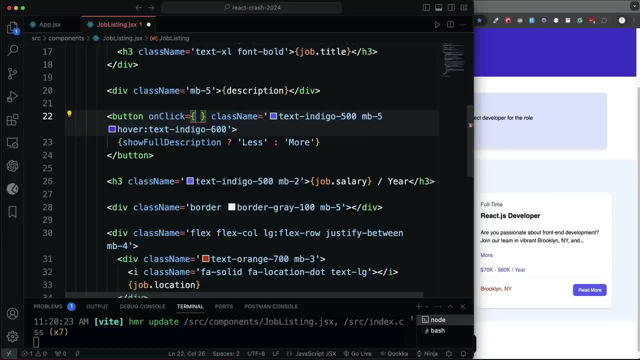 case like this, not like vanilla javascript, where it's all lowercase, so on click. what do we want to do? we want to basically just call that set full, uh, set show full description. now, you don't want to just do set full description here, because that'll actually call it without even clicking. 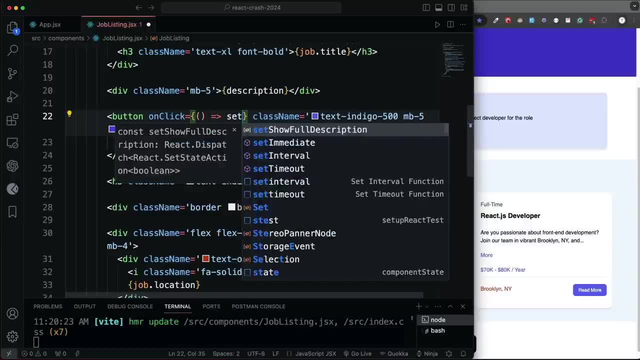 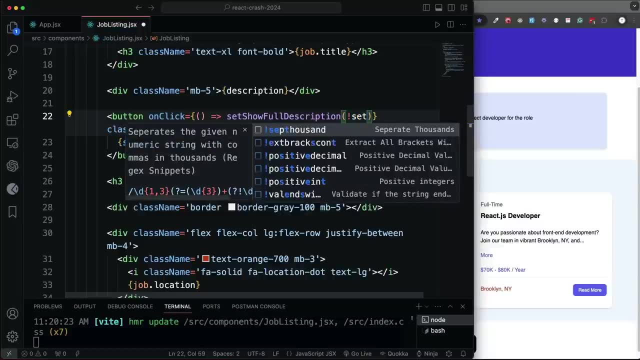 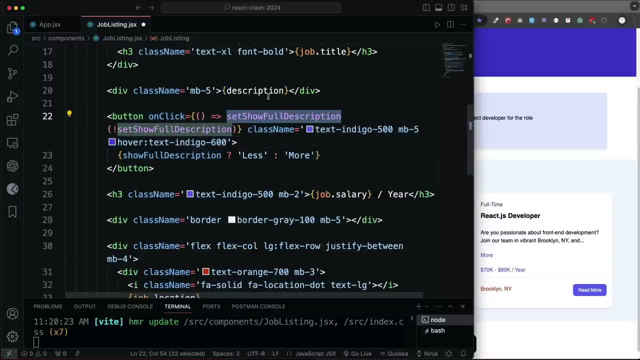 on it. you want to run a function and then call set, show full description. now you could do this. you could say: just set it to not whatever. set full description is okay, because when you call one of these methods, whether it's set show full description or or set, i don't know- set anything. 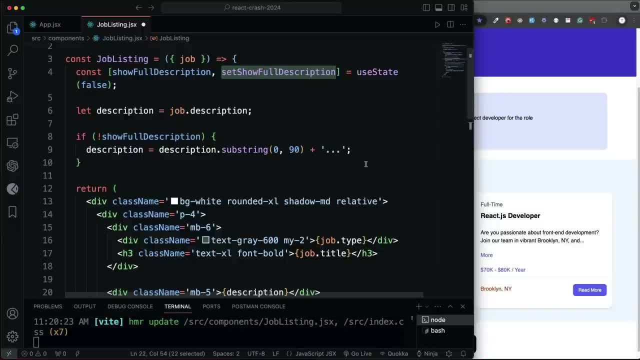 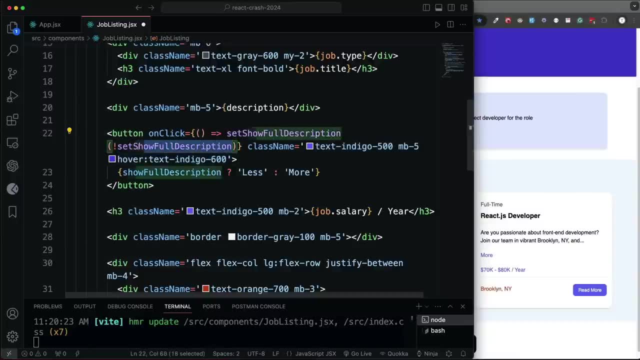 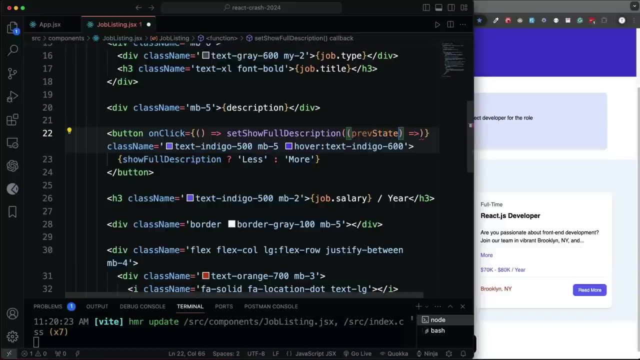 whatever you you have for your state, it can take in a couple different things. it can take in a straight value, so in this case we're just setting it to the opposite. or it can take in a function. so if you pass a function in, you actually get here whatever the previous state is and you can call this whatever pre. 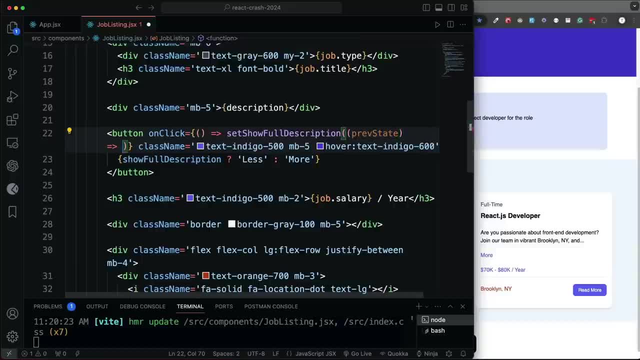 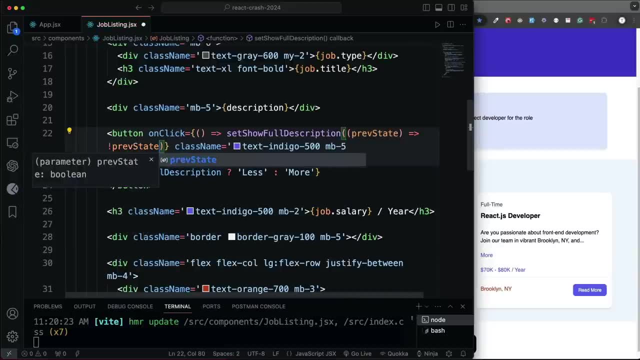 pre state and what we want to do is then set it to the opposite of whatever the pre state is. so if it's true, set it to false. if it's false, set it to true. um, because you, you can do it the way i just showed you, just passing in the not set full description, but you can. 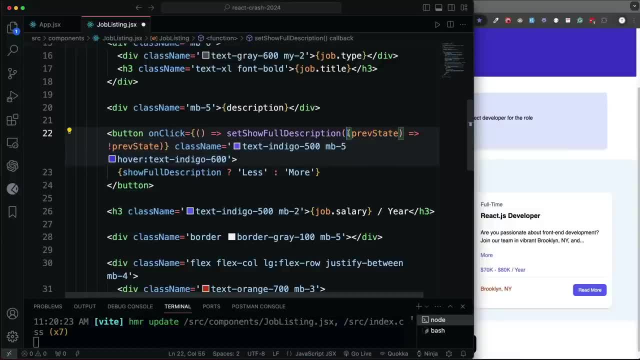 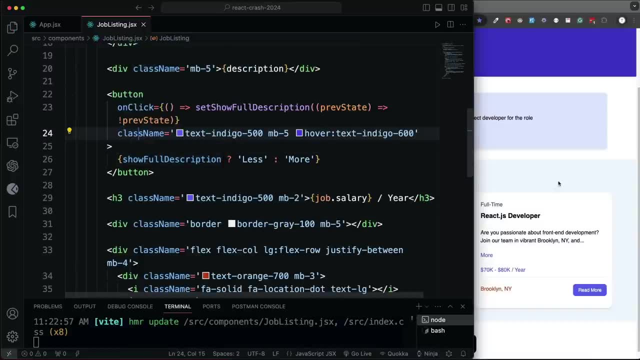 run a function and then set it to the opposite of whatever the pre state is. so, if it's true, run into some issues. so this is a better way of doing it: passing in the function, getting the previous state and then setting it to whatever the opposite of that previous state. so we'll save that. 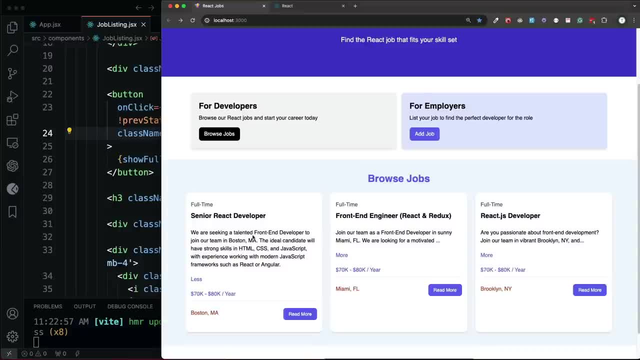 and then let's come over here, let's click more, and now we see the whole thing and of course, it's only the component where that we click that we're talking about. okay, these ones stay the same. if i click less, then it'll show less, all right, so this is. i know we don't have a lot of. 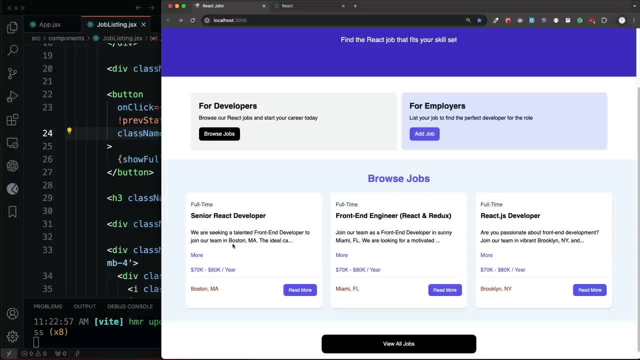 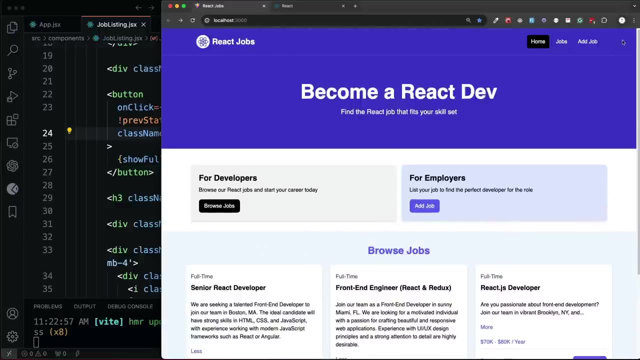 this type of stuff in this project. but that's the beauty of using a front-end framework is the ability to add this, this kind of dynamic stuff. okay, and you can picture using this for, like a modal, you have the open and closed state. if you have a menu, a hamburger menu, you have maybe menu. 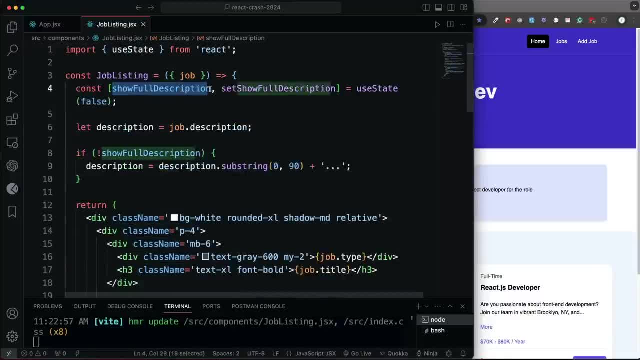 you could have menu open, like right here. you could have menu open and set menu open or something like that. so hopefully this gives you just kind of a a good picture of what component state is and what you can do with it. now we're close to our home page being. 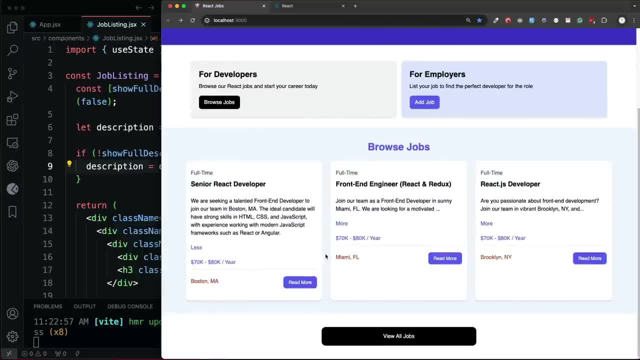 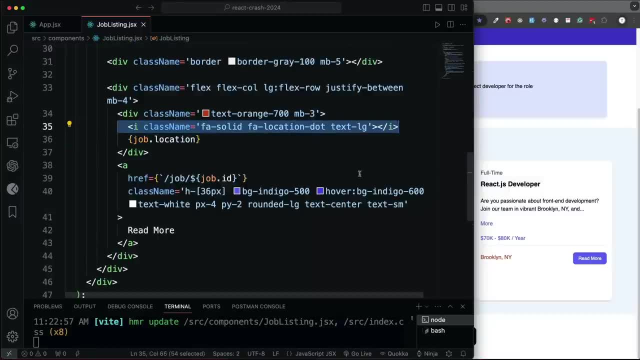 done. so let's take care of the icon, because right now we have that in our job listing component. we have that i tag which isn't showing anything because we don't have the font awesome, cdn. but i don't want to use the cdn, i want to use a separate package for that. so this will kind of 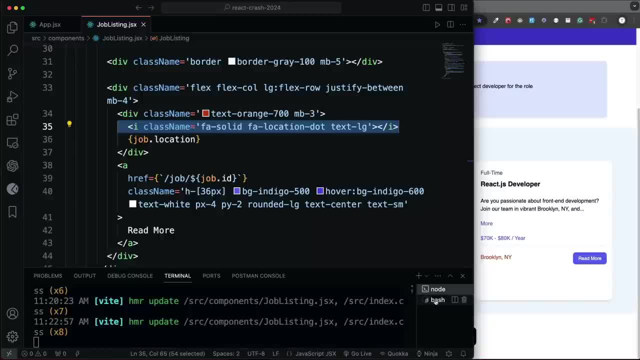 give you a little bit of experience in using additional packages. so i'm going to go to my terminal here, the one that's not running the server, and we're going to say: npm, install, react dash icons, and this will allow you to work with not only font awesome, but material icons and some of 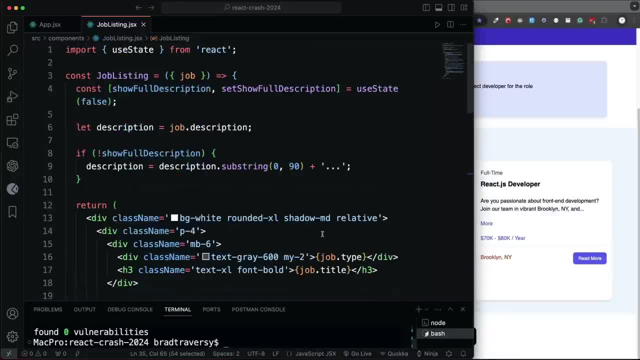 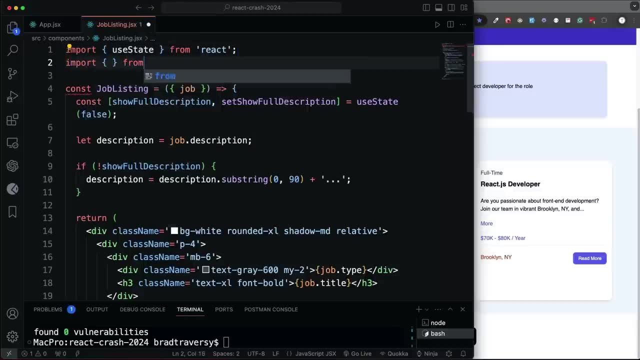 the other packages as well. so now that we have that installed, we can go to any component we want. so in job listing let's import and we can get from react icons. but since we're using font awesome, it's going to say: typical fonts do not use that. sameosely, we're going to use the font awesome. 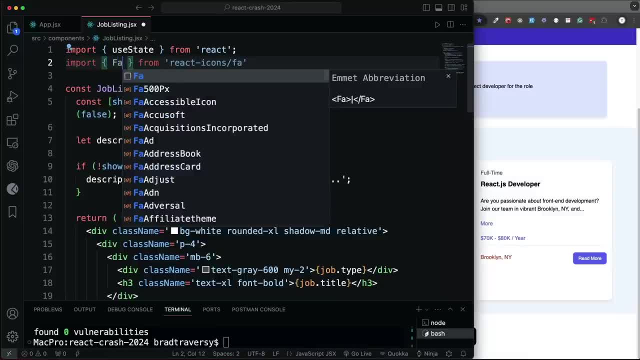 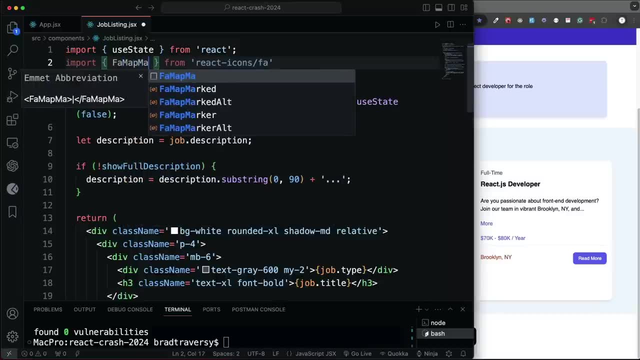 icons this time, because they're the same same as the font awesome, and these armed icons here are simply the format icons, so they're the macro icons that are included in the layout and these are basically the adjacent icons that you can differentiate between these macs that are available. 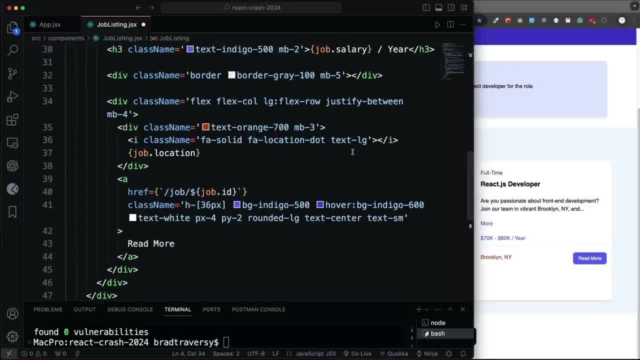 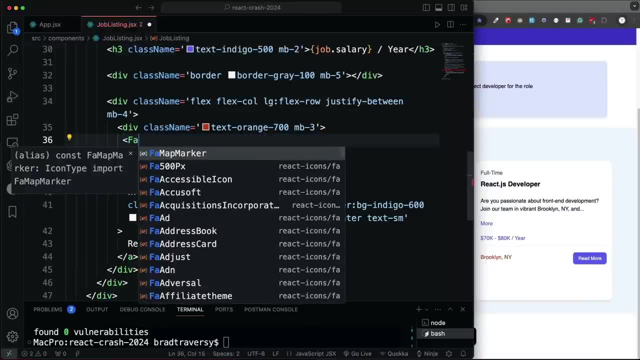 for in theiano functions. so you can see, i have some of the components here that this has cut out. i don't want that. oh, do i want this? i want this sub anger and then, following the storm map marker, which is a component. so basically the icon itself is a component. 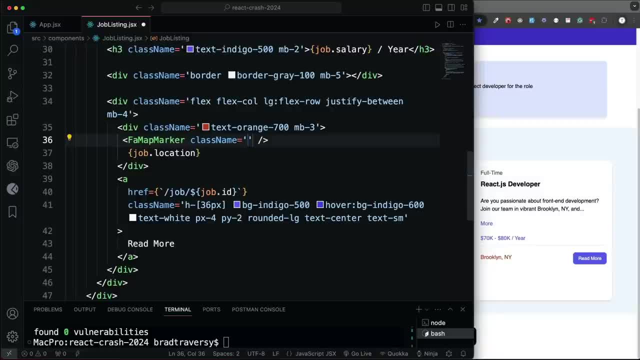 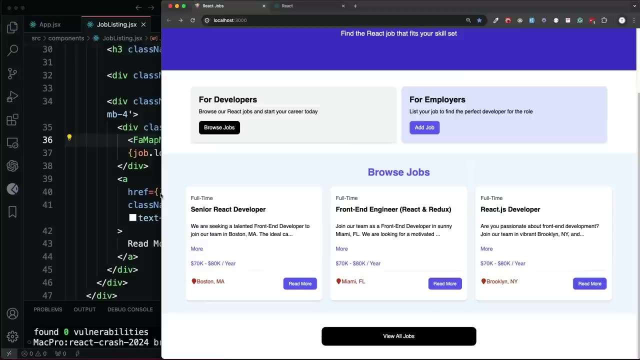 and I'm just going to add some classes to this. I want it to be in line side by side with the location text LG and then a little margin bottom. so let's save that. and now you can see we have our little icon. let's actually put some. 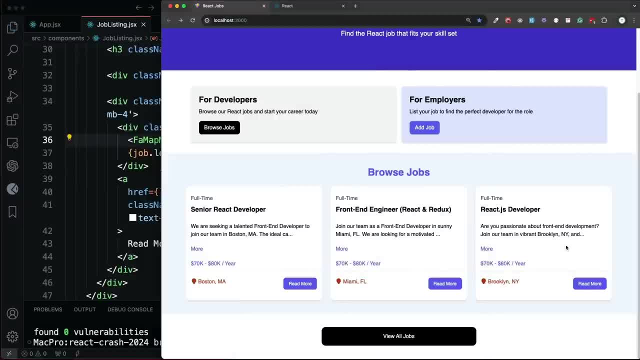 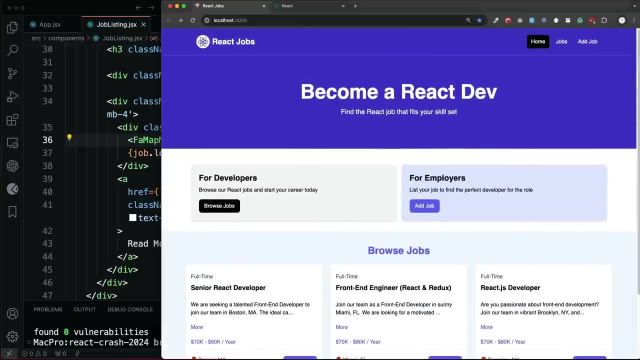 margin on the right as well, say: mr1, push that over a little bit. so now, anywhere you want icons, you can bring it in from react icons. so I think now we're to the point where we want to start to add additional pages. right, we want the jobs. 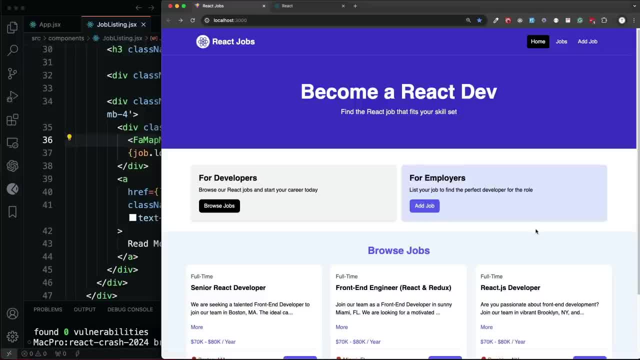 page, the add job page. so we can't do that with, just react. so this is- this is where you know what I talked about earlier: a library versus a framework. being a library, it doesn't have a way to add separate pages, so we're going to use 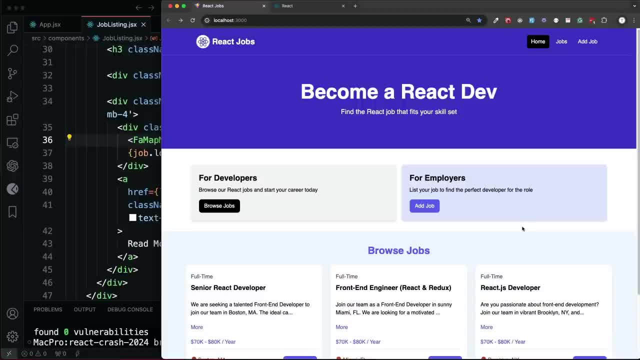 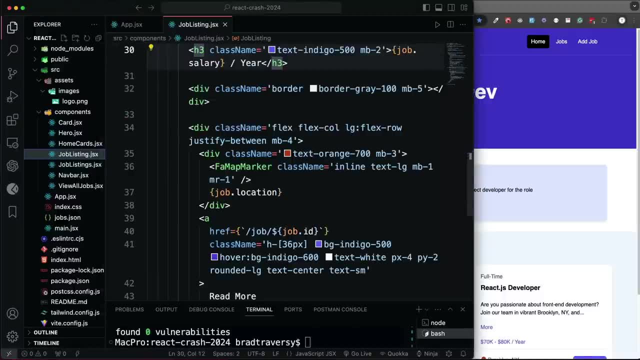 react router, which is the basically the most common way to add a page. so we're going to use react router, which is the basically the official router for react, but it is a separate package so we need to install it. so let's go to, let's go to the terminal again and we're going to 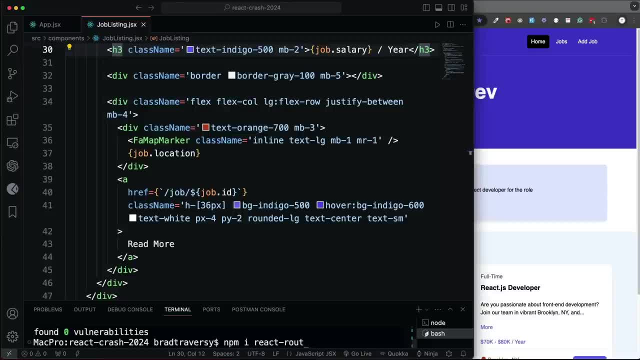 npm install and the name of this package is a react router, dash Dom. okay, make sure you add the dash Dom. so we're going to install that, and the way that you set this up has changed a lot over time. in fact, there's been at least two times where I've created a react course and 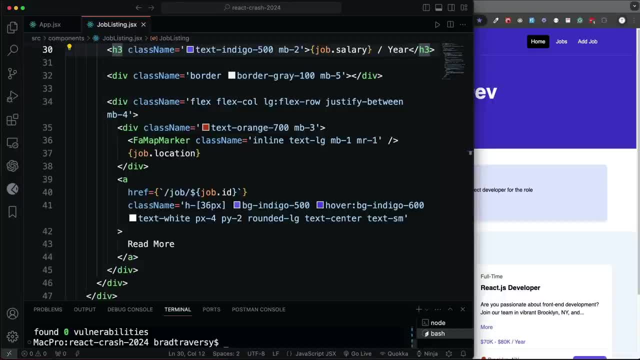 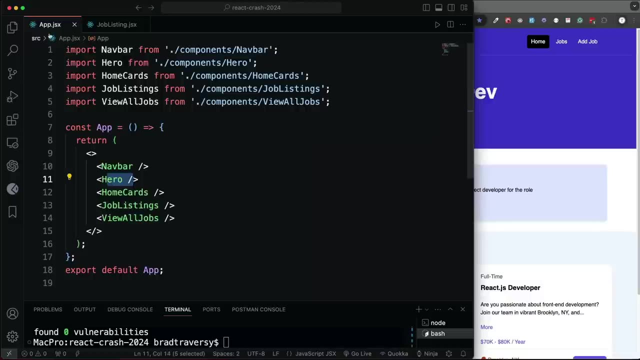 then, not too long later, they changed it up on how to use this and it can be a little. the boilerplate can be a little overwhelming for beginners, so just bear with me. so we're going to put all the routing stuff in the main app file, so in 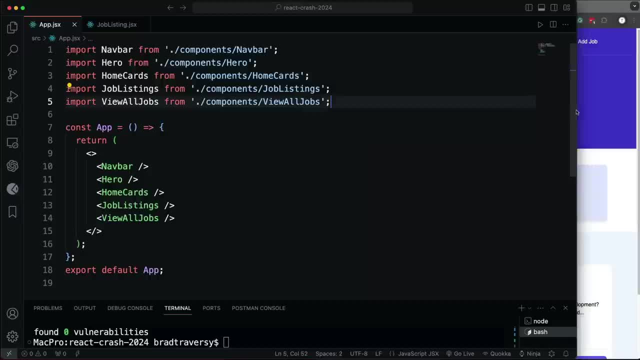 the app jsx and react router is. it's actually a pretty big package, it's it's. it's built the remix framework, which is a server-side rendering framework for react. it's built on top of react router. so there's a lot that you can do where. 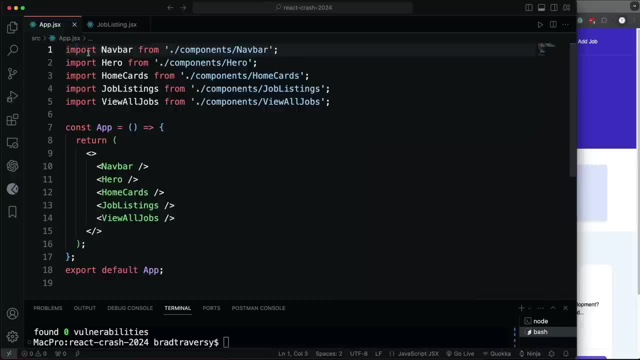 we're going to get into some stuff like data loaders, that react router offers. we're going to do that later on, so just just be aware that it is. there's a lot to it and it can be a little overwhelming, but I'm going to show you exactly how to. 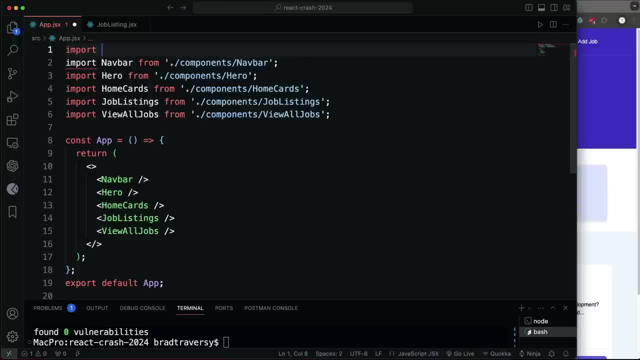 create routes and you know. so you can have multiple pages. so let's import a few things from react router Dom. again, make sure you use the dash Dom at the end. so we're going to bring in the route component. we're going to bring in create browser router, create. it's called create. 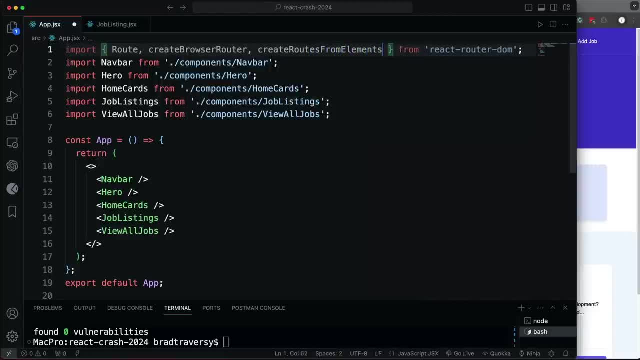 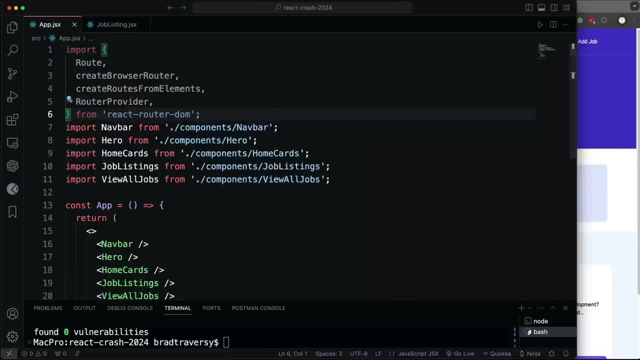 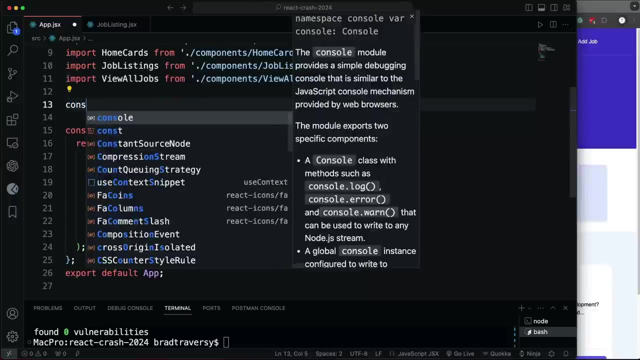 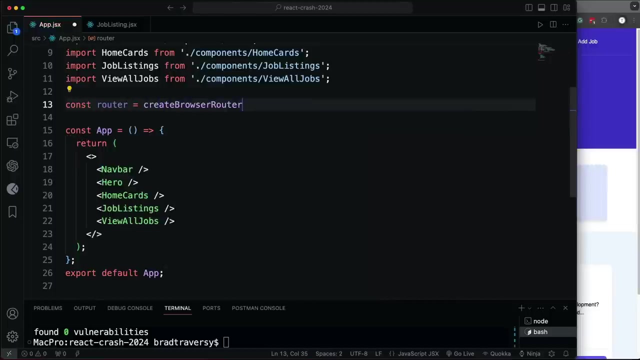 routes from elements and also the router provider. okay, so we want to bring in those things now. the way that this will work is of the the return in the main app component. we're going to create a variable called router and we're going to set that to create browser router, which does just that. it'll create our 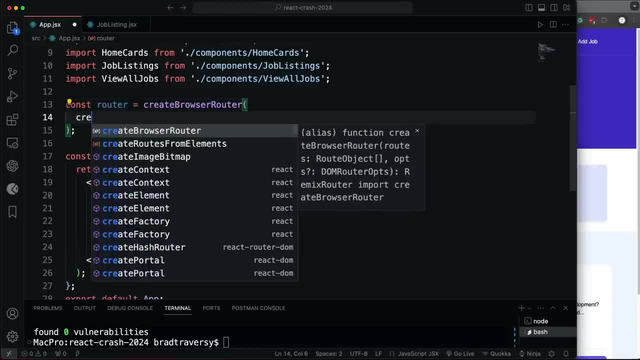 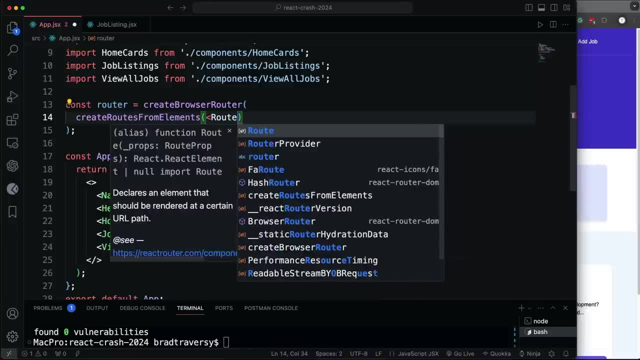 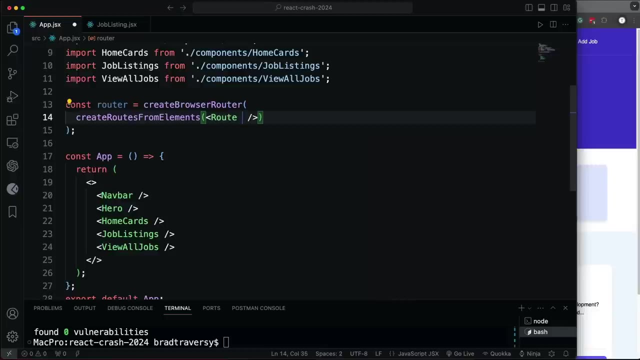 router and inside that we're going to then use, create routes from elements and inside that is where we can use our route component. so we're gonna put in route and then you can put in a path. this is going to be for the home page, so we'll just- we can actually just put in index and then 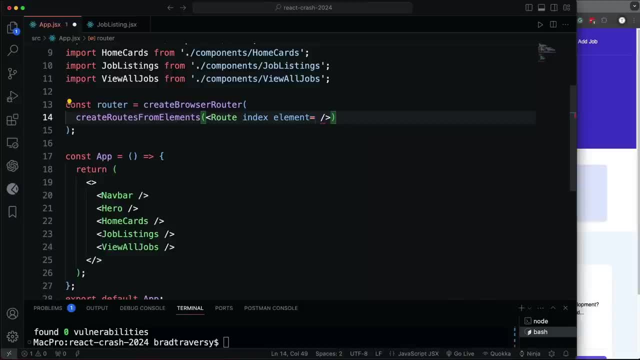 you can have an element represent that route. so for now I'll just- I'm just going to put in in H1 because you can do anything, just to show you. we'll just say: my app, okay. now this isn't going to do anything just yet, because we haven't- um, we haven't implemented the provider. okay, the provider. 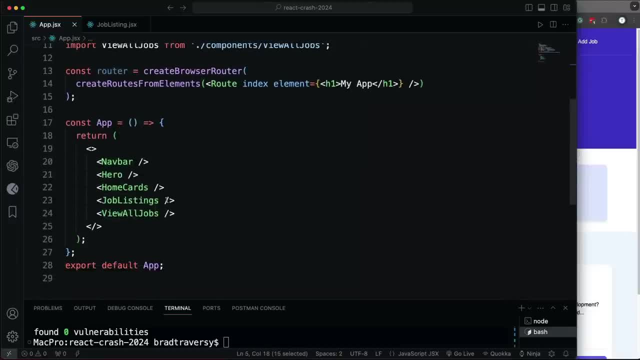 is what provides the router and that's gonna go in. put the browser in and she can use it and that's going to job you that to go down here. so we're actually going to change this up and not embed these components in here, because we're going to have separate pages, so we can actually get rid of all this and all we're. 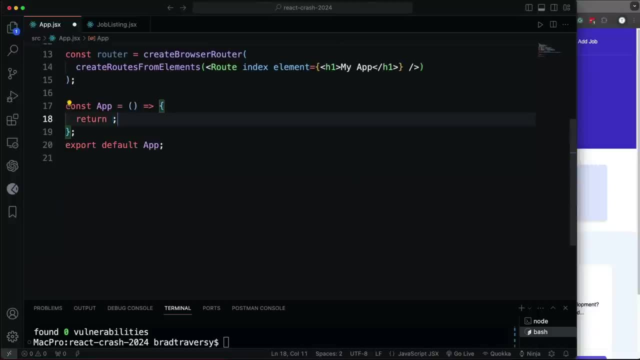 going to return is going to be the router provider. so we're going to say router provider and don't worry, we're still going to use those components, they're just going to be used in a different way. so let's say router provider and then that'll take in the router that we just created above. 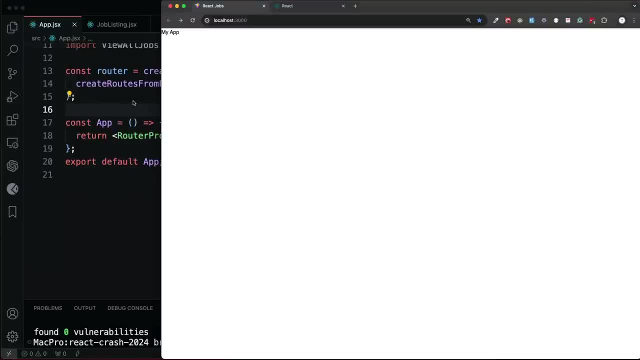 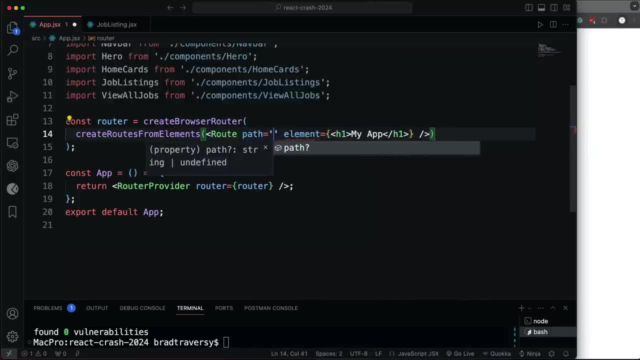 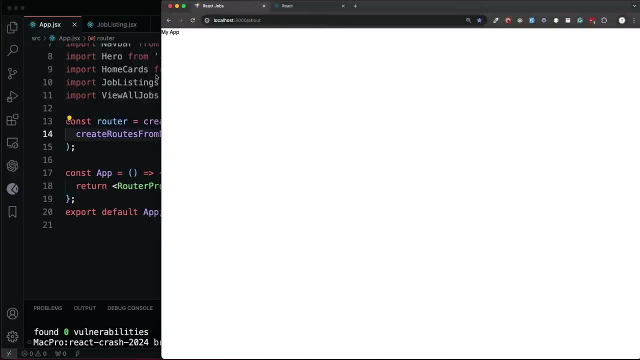 so if i save that now you can see we have my app and that pertains to the home page route. now if i were to set this, let's say, path equals, slash about right, and then i go to slash about, then that's going to show that element, okay. so this does exactly what it says: it creates a route. 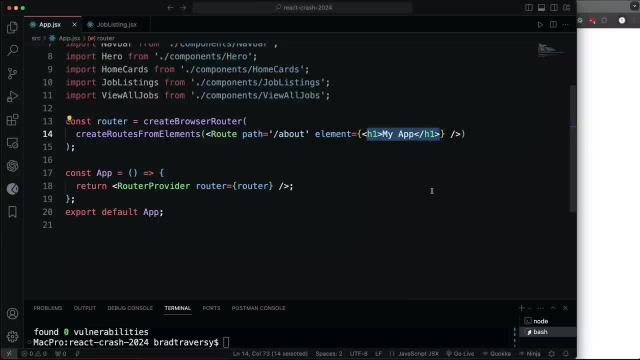 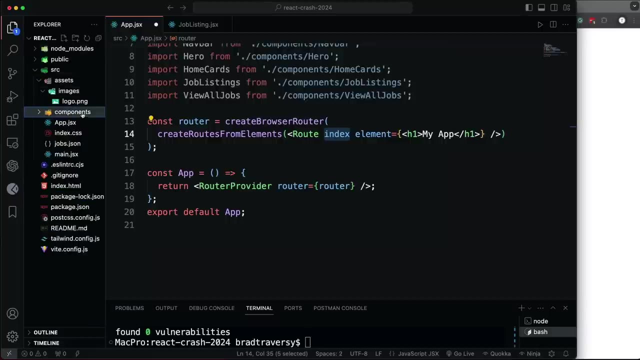 with a path and it creates that from an element which, in this case, is h1. now i want to show a page for my, for my, index. let's put that back to index. so what? what i do is create a separate folder, because your pages are components. they're still react components, but i don't want to put them in. 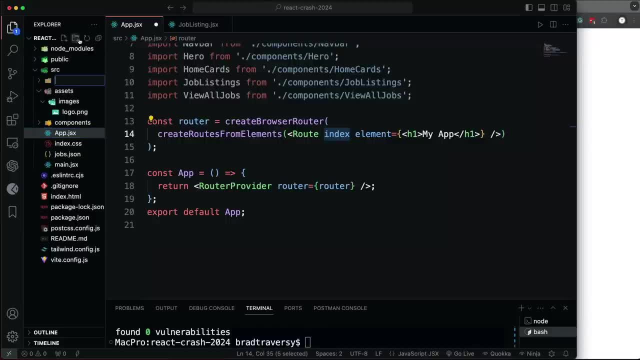 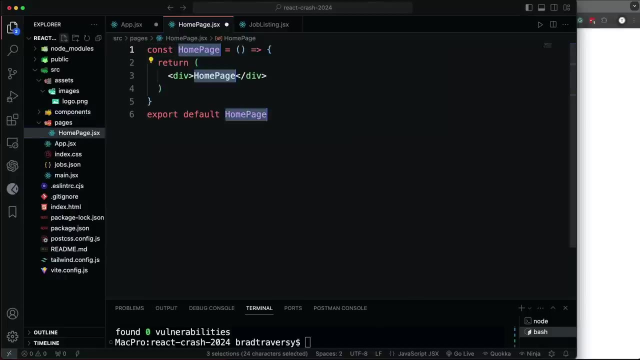 the same folder as my regular ui components. so let's create a folder called pages. you might see it called screens sometimes, but we're going to call it pages. and then we're going to create a home page dot jsx file and, just like a regular react component, we'll do rafce and on the home page 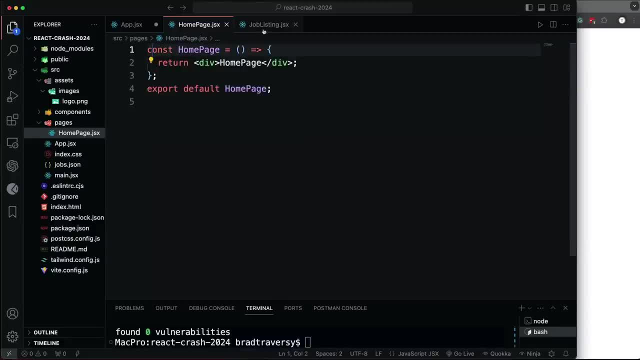 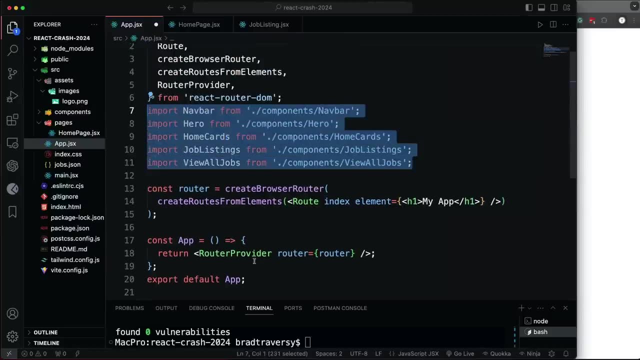 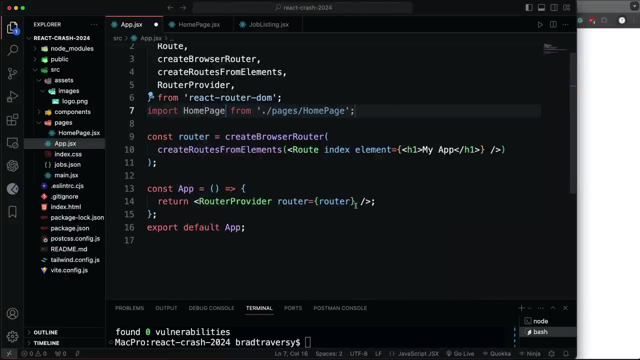 we want to bring in. actually, let's just save this for now and go back to appjsx and we no longer need to bring this stuff in here because we're not using it in our main app file. so we can get rid of that. but we do want to bring in our pages that we're going to use, so we'll bring in home page. 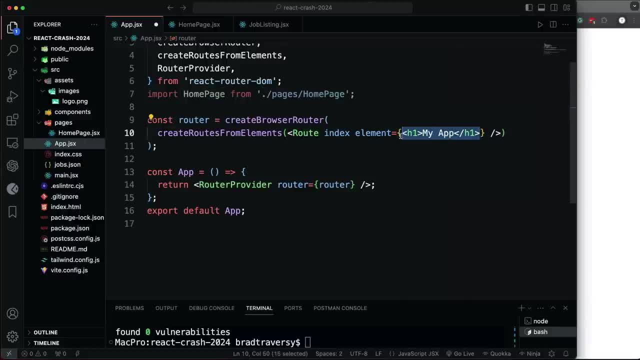 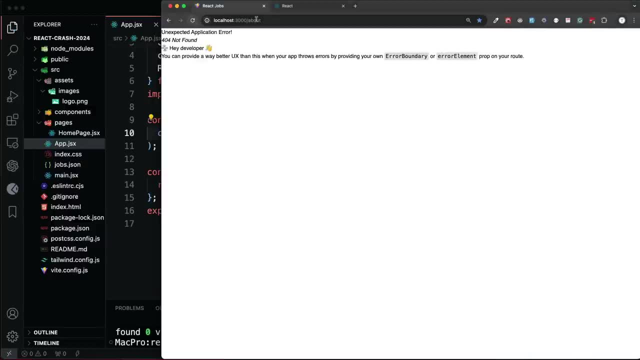 make sure it's from pages and not components, and then here we're going to render the home page okay. so now, if i save, that and we go about, doesn't exist, and i'll show you how we can create a custom 404 page as well. but if we go to the home page, then we see the text: home page. 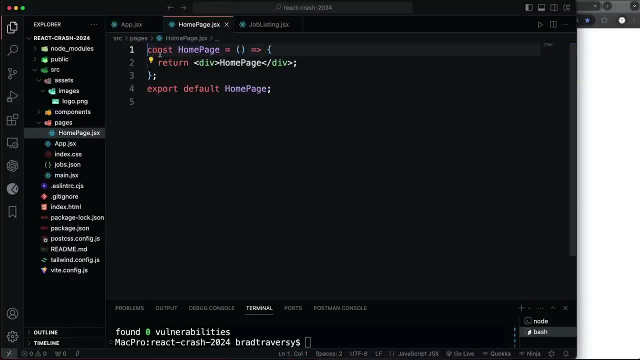 okay, now in the home page, this is where i want to bring in um, not the navbar, because the navbar i want to show on all pages and we don't want to have to bring it into every single page. so we're going to create something called the layout. but let's say: 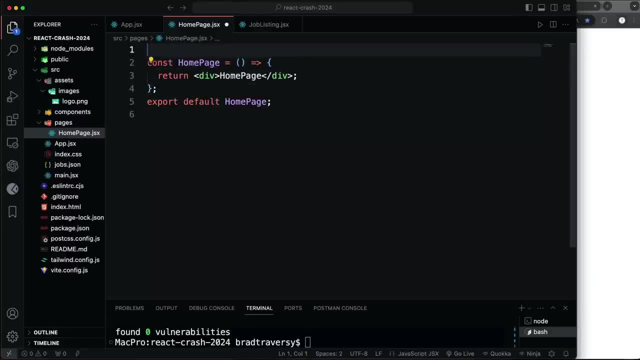 the hero component, for example, that i only want on the home page so that i would import, let's say, import hero from, and then let's see, we're going to go up one level into components, and then hero, and then let's- uh, we'll make this a fragment. 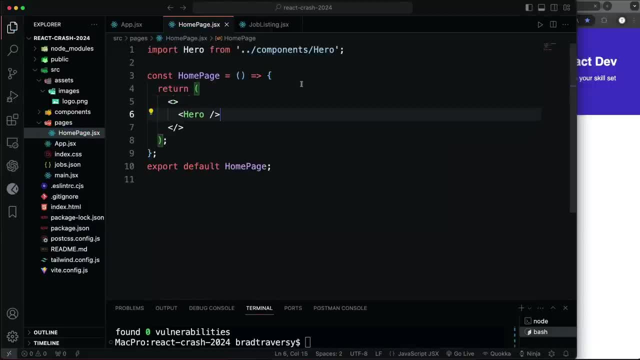 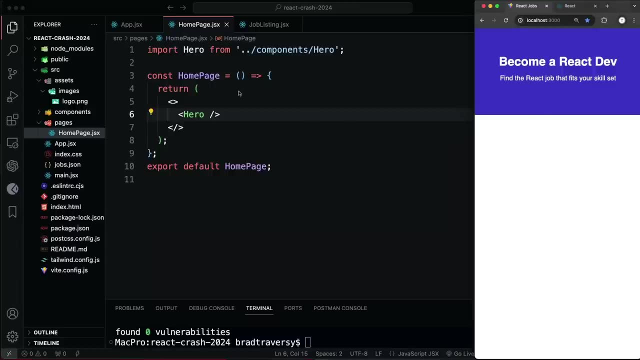 and then we'll put our hero component, save that and now the hero component shows: all right now, like i said, for the navbar and things like footers, that's stuff you want to show on every page. so this is where layouts come in. so we're going to create. 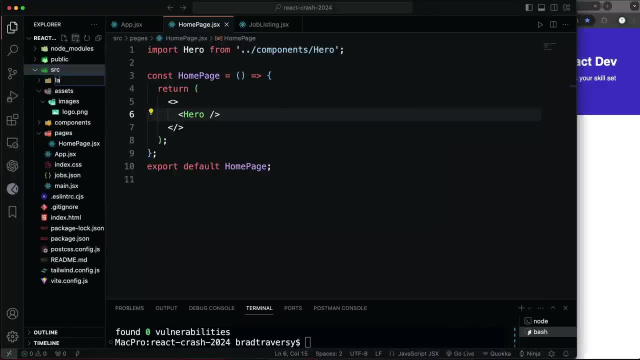 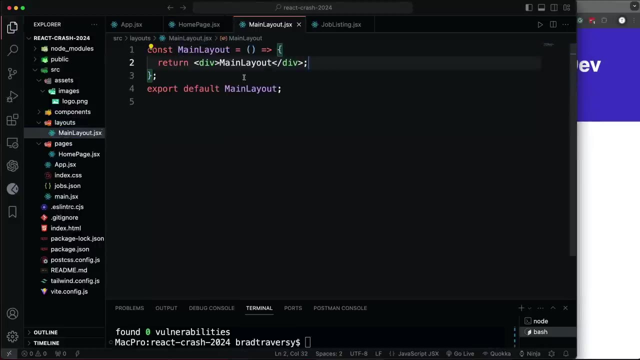 another folder in the source folder called layouts, and you can have multiple layouts. this particular project will only have one, but you can have multiple. but let's call this main layoutjsx. and again, this will be a react component. now, before we do anything here, i just want to show you how to actually use the layout so we can bring it into our main appjsx. 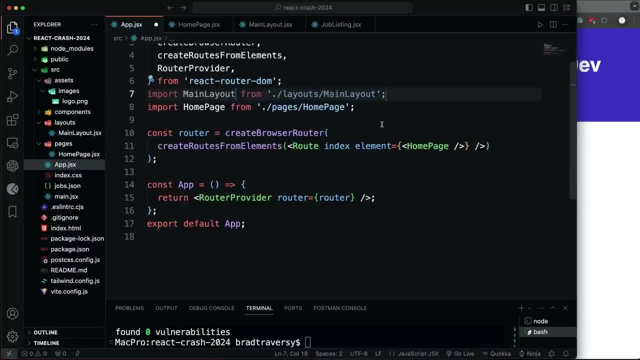 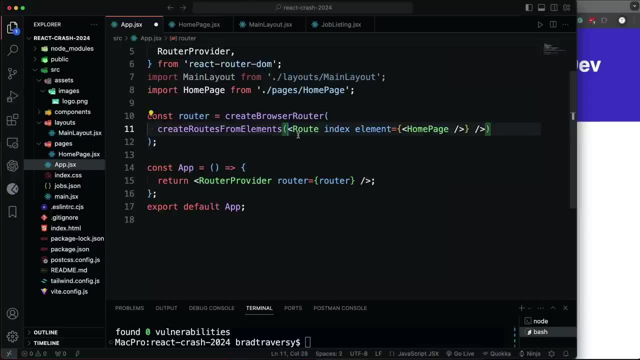 let's say import main layout and then what we need to do is just create a parent route to the rest of our routes. so let's go right here and say route and say path, and set that to slash, and then the element is going to be set to the main layout, okay, and then we're going to 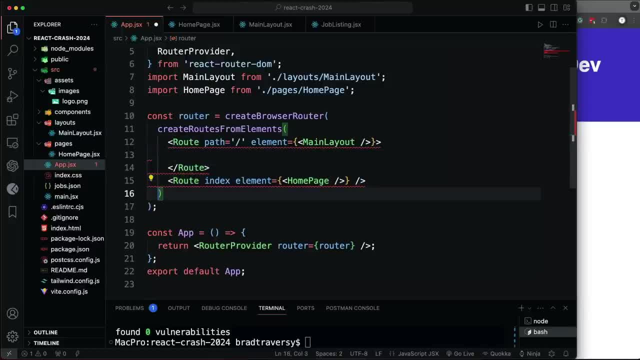 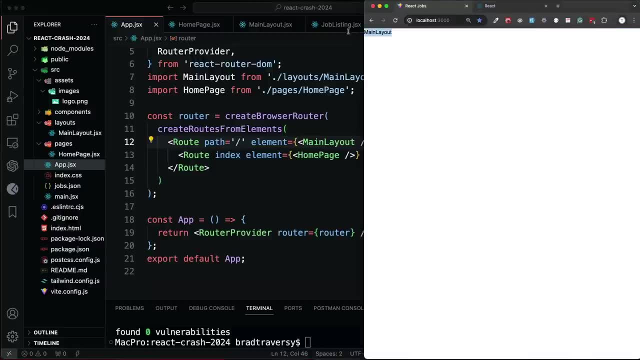 surround this. this parentheses should be here, and then we're going to move that in here. okay, so basically, if I save that, you'll see main layout. so now this is being applied. we don't see the home page anymore, and I'll show you how we can get. 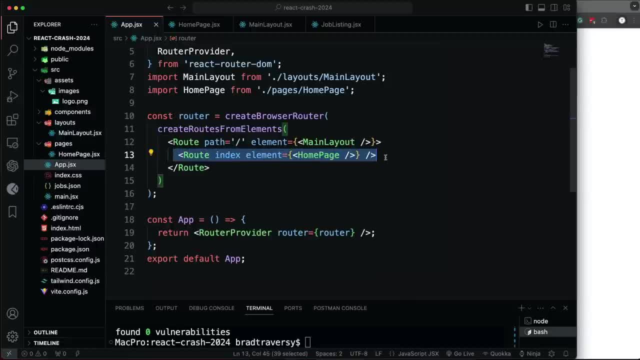 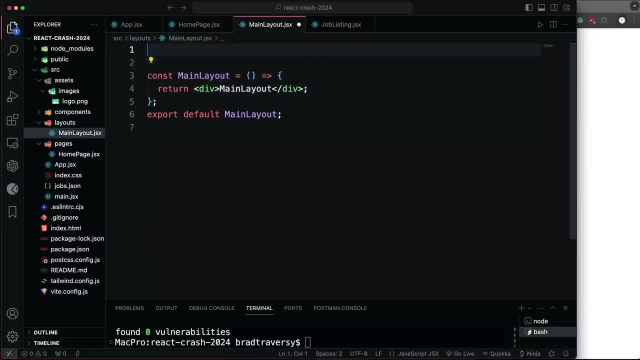 that back in a second. but basically anything, any routes we put in here are then going to use this layout. so in the main layout, whatever route you're on that, that content, that page is going to come through the outlet. so we're going to import outlet from. 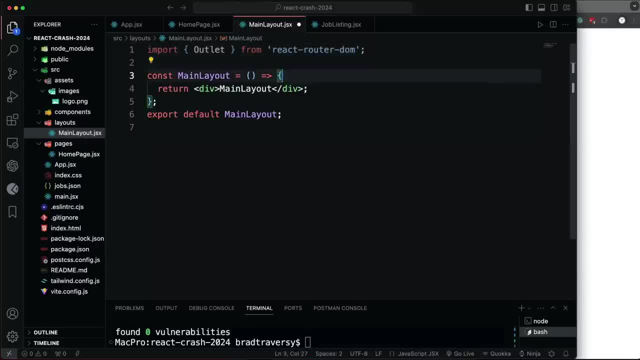 you react: router, Dom, and then down here. let's make that just a fragment and then get rid of the text and we want to output here. we want to say outlet: okay, it's like it's an actual component. now, if I save that, we're seeing the the hero. 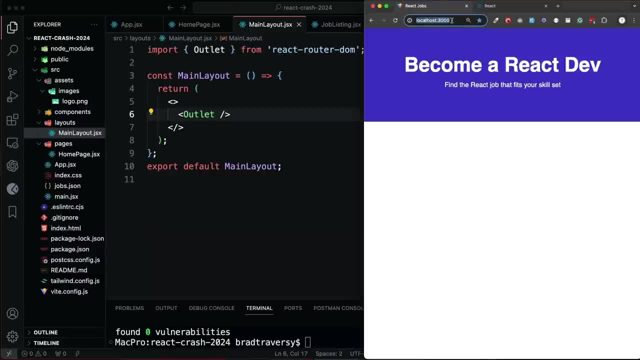 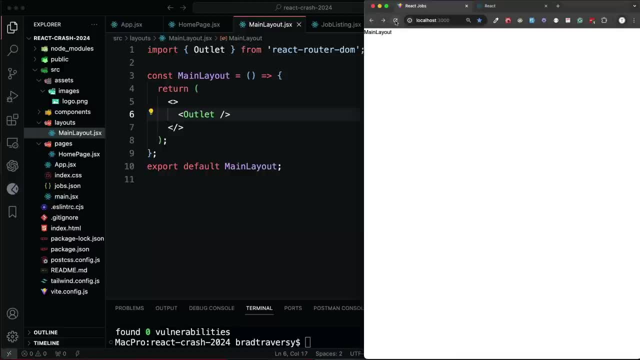 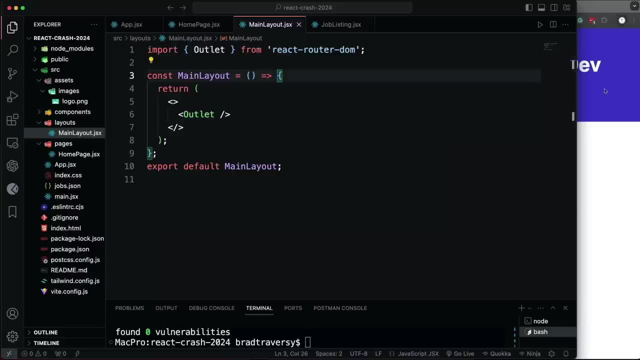 again because we're on the home page, right, we have no other routes. so if I were to go to slash about, we're just going to see this 404 private data in sozial data to take that we can update if I got the highest level successfully this timeline that we just made last night. okay, but before that, 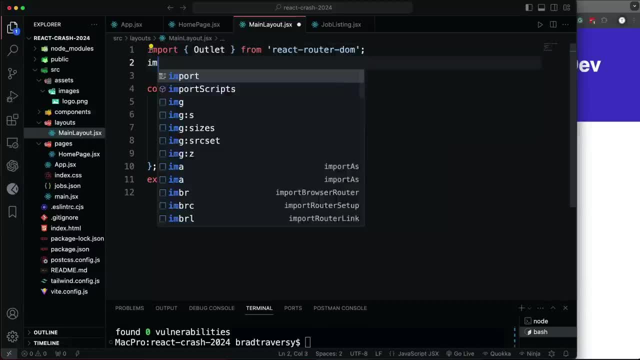 I need to take a copy of this. so if I wanted to take a screenshot, it brings that meaning. all right, just Escape and then run this. I'm going to do Zahl, ok, Ok, coming right out of the state. so I'm just going to And there we go. So now any page we're on is going to have the navbar. 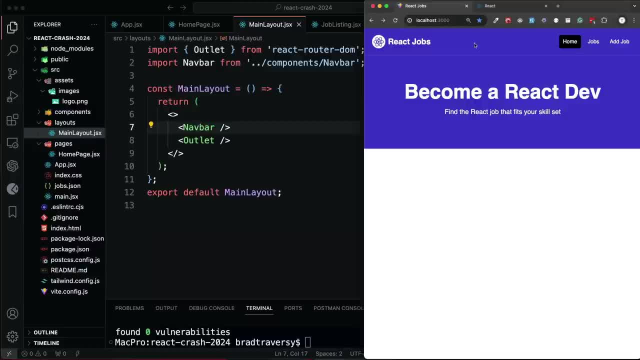 And of course, this is much better than doing. you know the vanilla way of having separate HTML pages, where you have your separate header or your separate navbar code HTML on every page. So now that we've done that, let's see the next thing. Let's finish up the home page Basically. 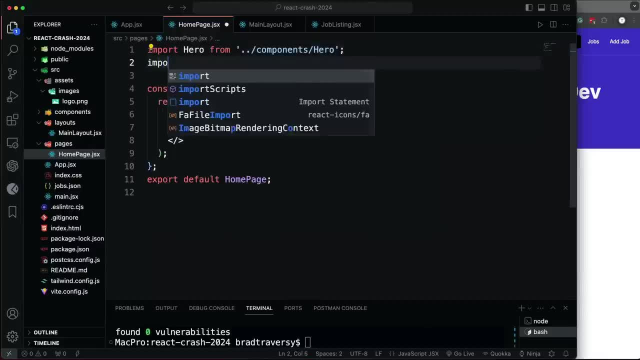 we're just going to bring in the rest of our components that we had in the main app file. So what else? we have the hero, we have the home cards. So I'm going to bring that in from components slash home cards and we'll put that right here. 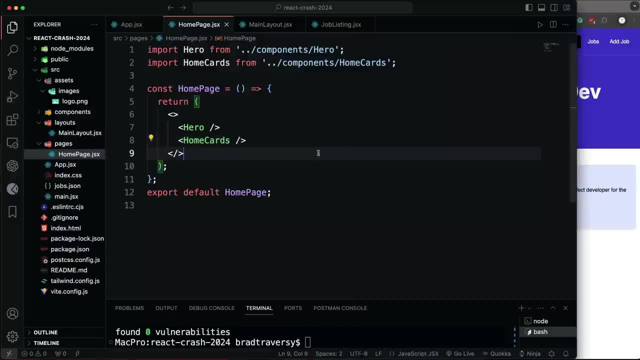 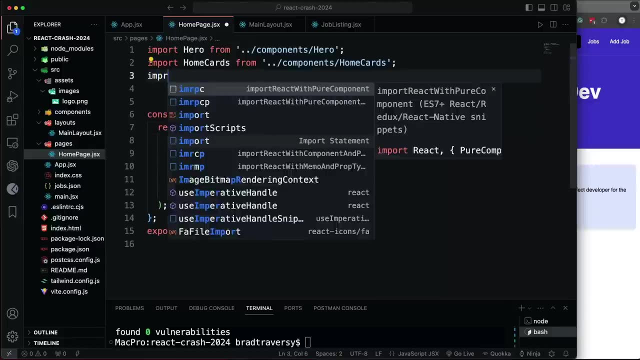 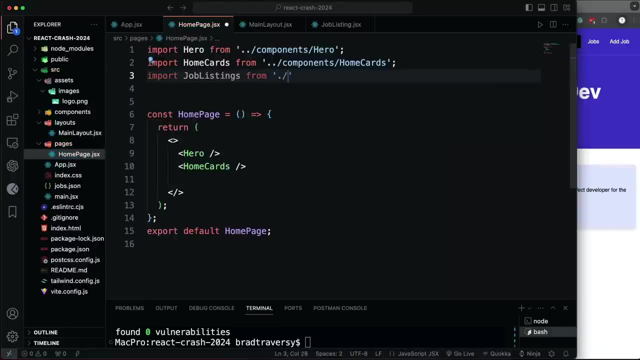 Okay, so now those are showing there. What else do we need? the job listings- import job listings plural dot, dot, slash components job listings- put that here. So instead of just putting this stuff in the main app component, we're putting it in the home page. 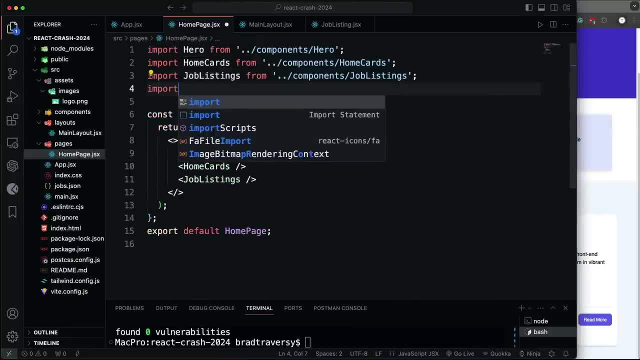 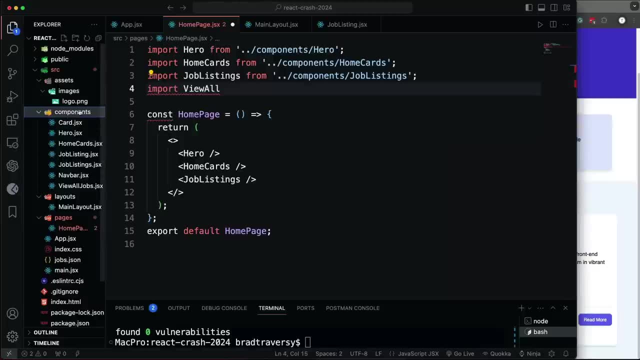 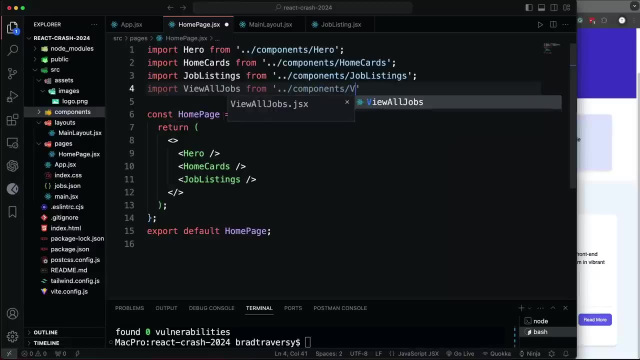 Okay then the last thing I think was the view all, So view, was it? view all listings, view all jobs- All right, we'll put that here And there we go. So we have this which goes to slash jobs, which doesn't exist yet. 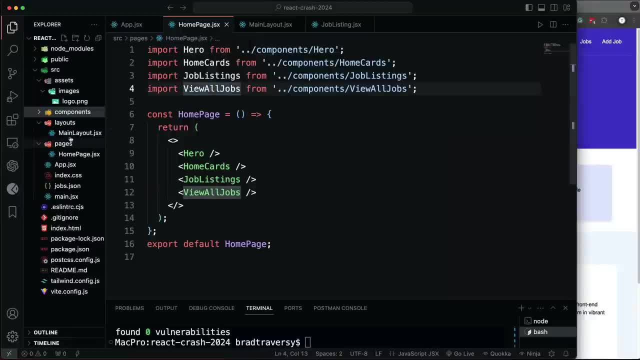 So let's do that. Next let's create the jobs page And the jobs route. So that's kind of the workflow from now on is you create a new page and then you go to the app file and add the route. So let's create a file in pages called jobs page. dot j s x. 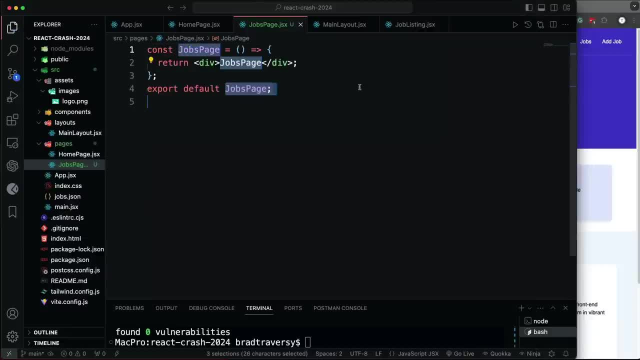 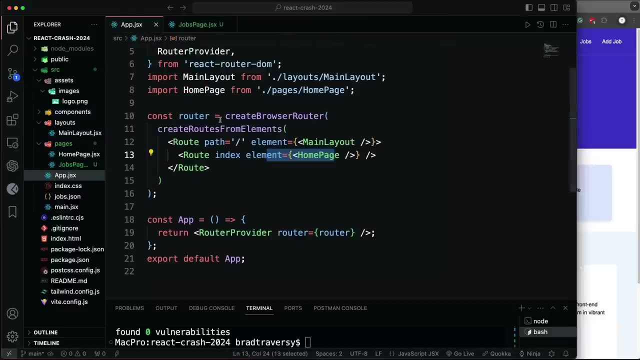 I'll say r, a, f, c, e, jobs page. just save that for now, And then let's add the route. we can close this other stuff up. Let's add the route into app j, s, x, So we need to bring in jobs page And then 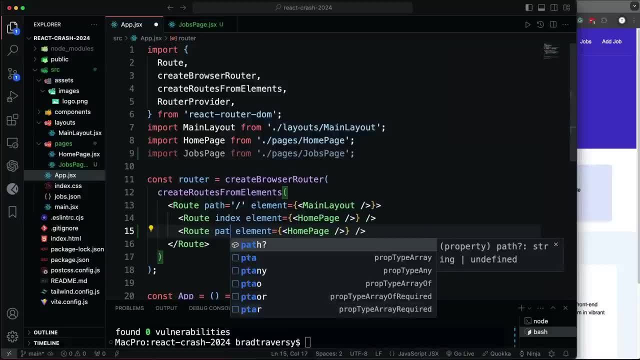 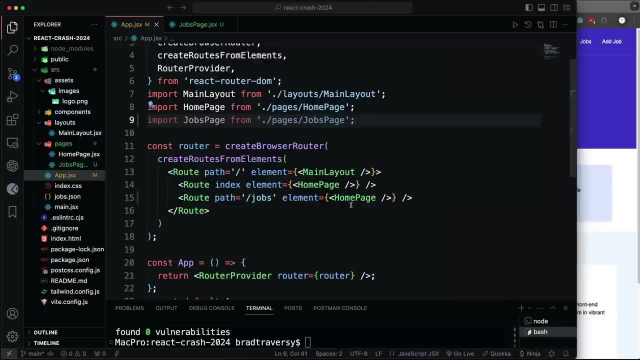 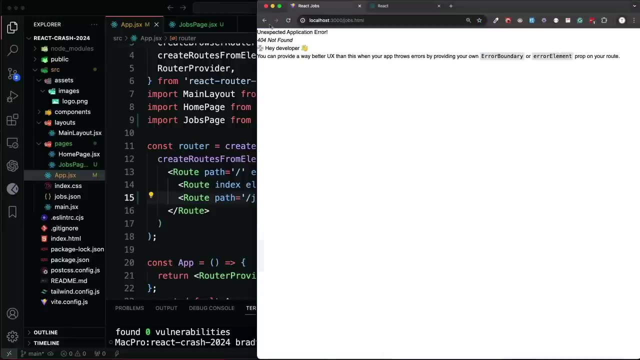 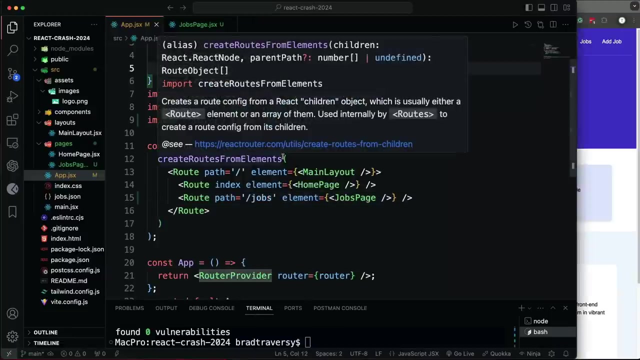 we can just copy this down. except now we're going to change index to path And we're going to set that to slash jobs And change this, the element to jobs page. So now if we click on jobs, oh, this is still going to jobs HTML. And that's another thing I want to get to his links. 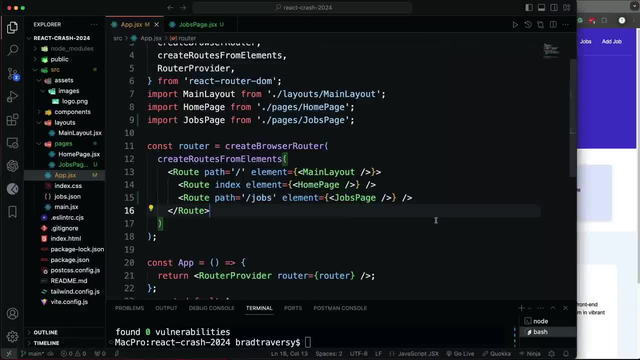 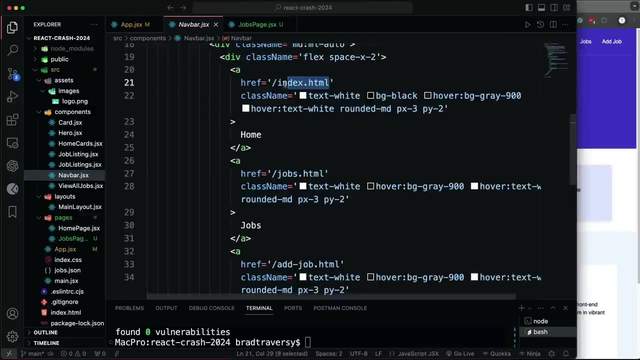 because it works a little bit different. We don't use a tags, we use the link tags, So but we can use the a tag, it will work. So just want to real quick go into the nav bar, So components, nav bar, and just change- Let's see this index HTML, change that to slash. 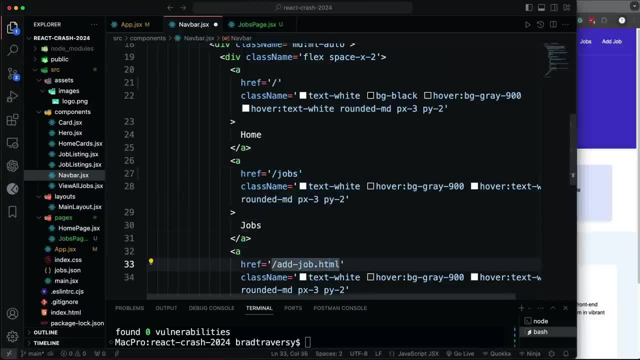 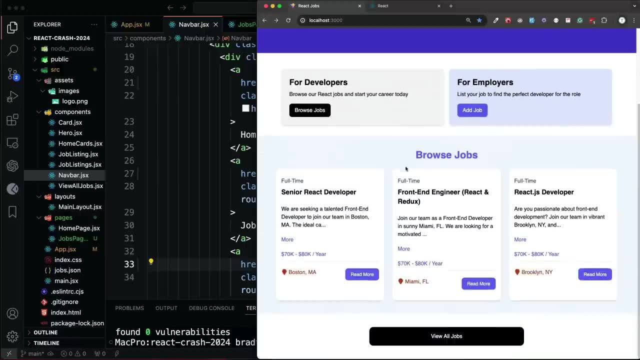 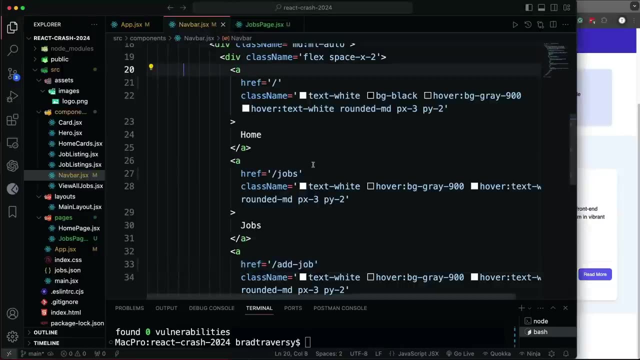 change this to slash jobs and change this to slash job. Alright, so now if I click jobs, it takes me to the jobs page, right. Also, this button down here goes to slash jobs as well. So now let's get into the link tag. 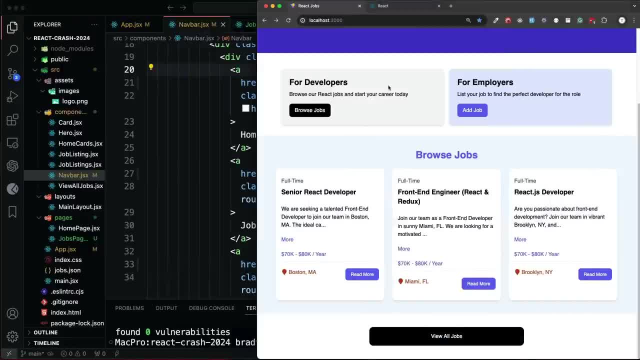 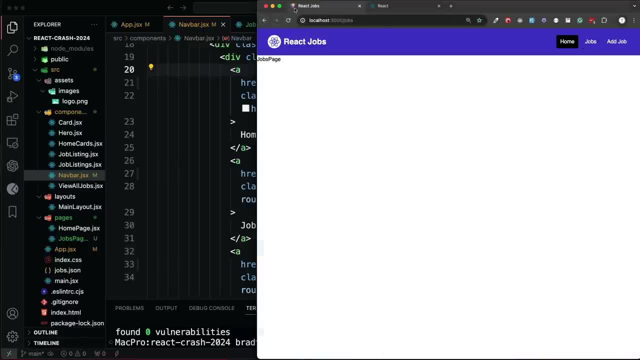 because we don't want to use a tags because it does a complete page refresh. Okay, so if I click wait, So if I click that, if you look up here in the in the tab, it shows the little little loader. real quick, right. 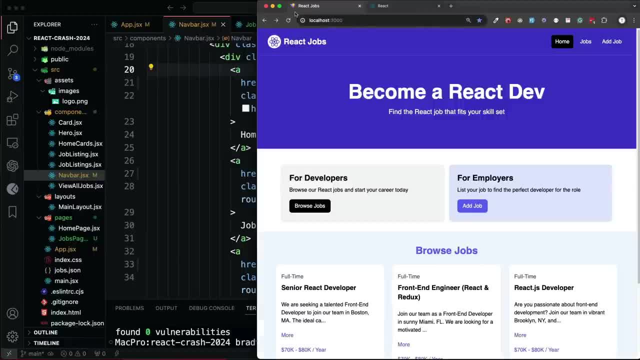 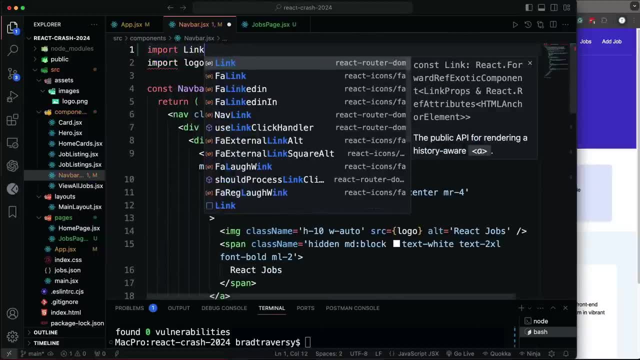 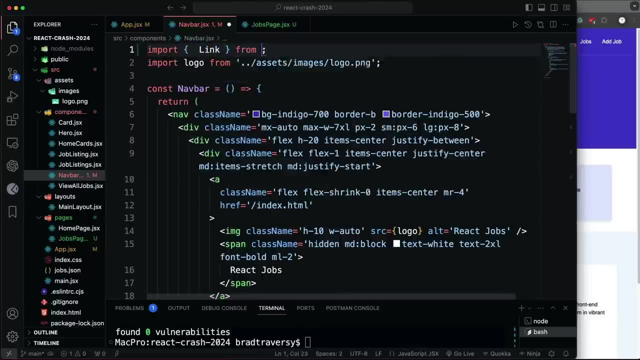 So by using the link tag it doesn't do an actual refresh. So in the nav bar let's import link. actually it's going to be in curly braces. So we want to import link from react router DOM And then we're going to change any a tag we have, such as this one. 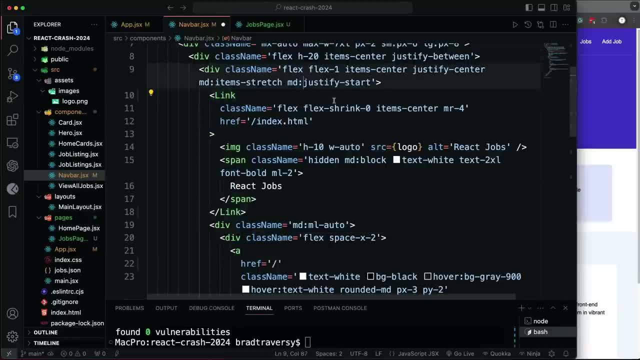 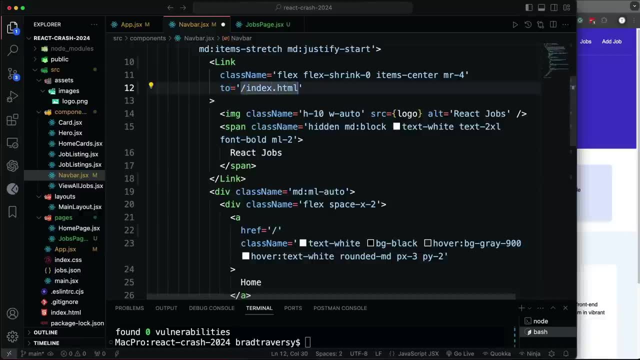 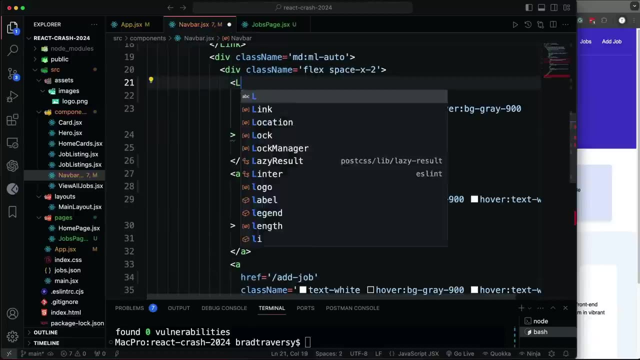 which goes around the logo. we're going to change it to link. And then the href. we're actually going to change it to two, And then let's make this just slash which is the homepage. Alright, so that one and then we have this one. change that to link. 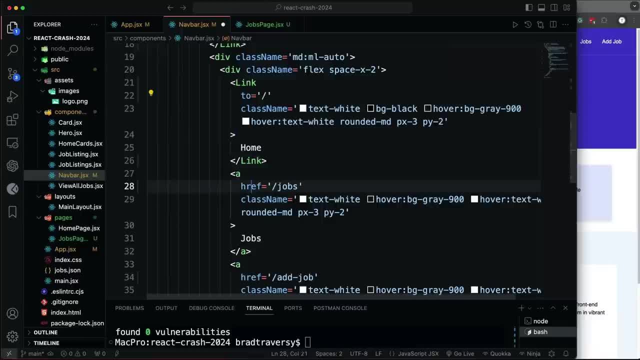 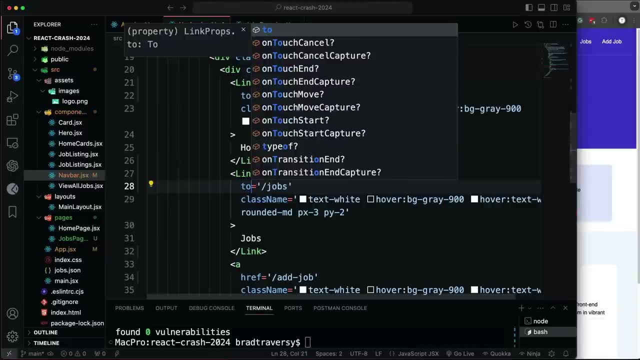 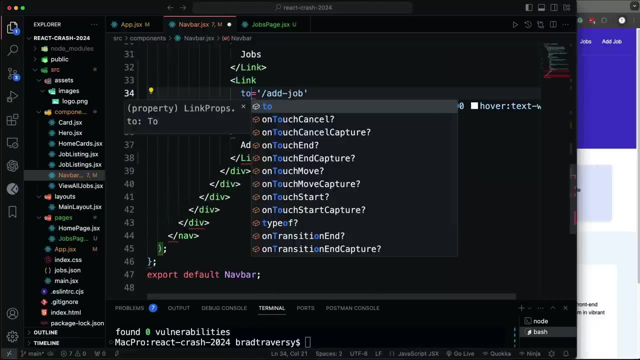 change this to two. Same thing here. link. make sure the ending tag changes as well To: and this one, Unknown Speaker 31. Alright, so now let's save that. And now we're just going to reload this page. If I click there, you can see it goes to the home. 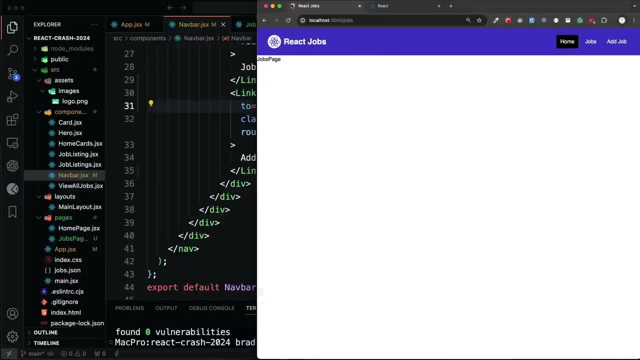 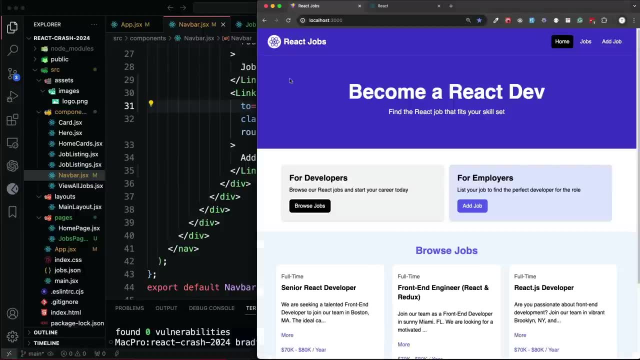 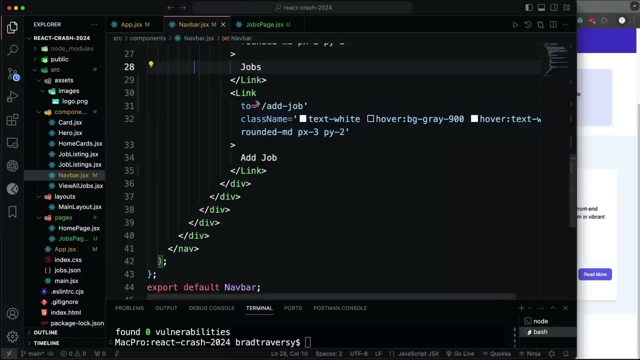 And as I as a link and change pages, you see there's no refresh loader thing in the in the title. It's very fast, right, Because it's all, it's all in the client And we want to change the link down here and the links for all these buttons to use the link tags. So let's go to see. 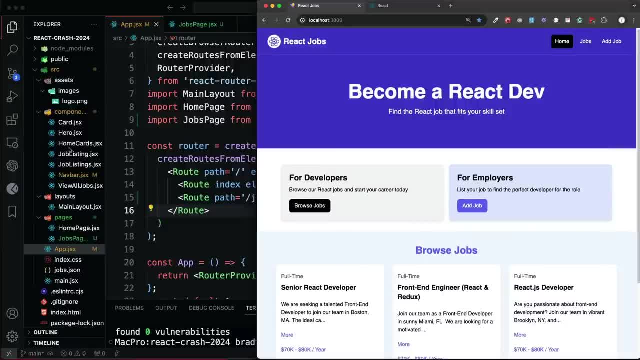 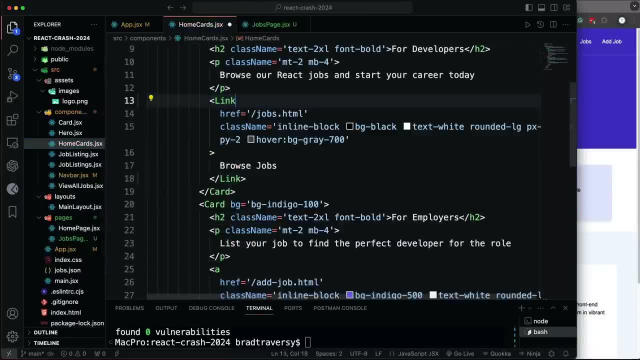 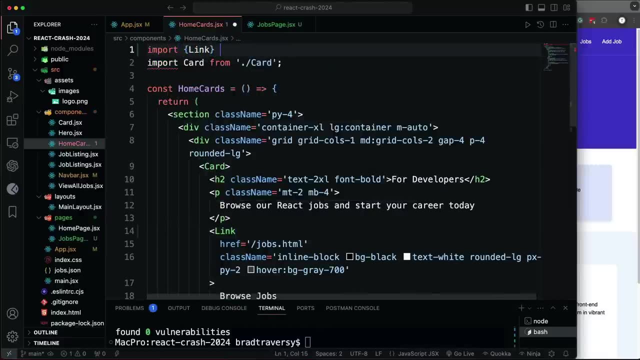 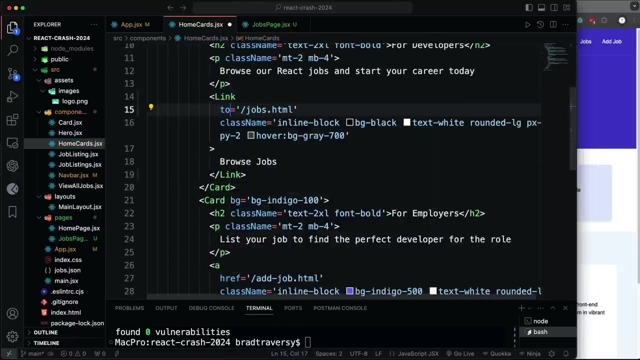 what's next? we'll go to the um. where is it? home cards, yeah, this home cards change that. actually, we need to bring it in. so, up top of home cards, let's import link, okay, and then this is going to be two and it's going to go to slash jobs and then this one. 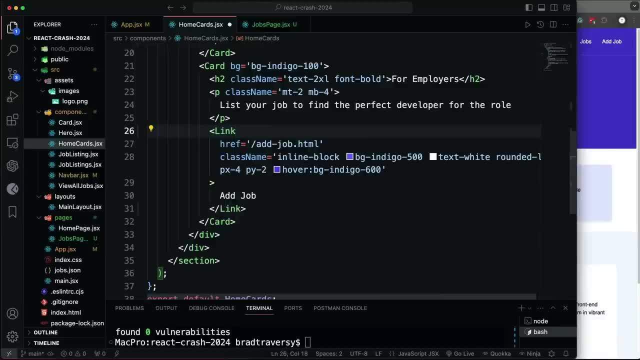 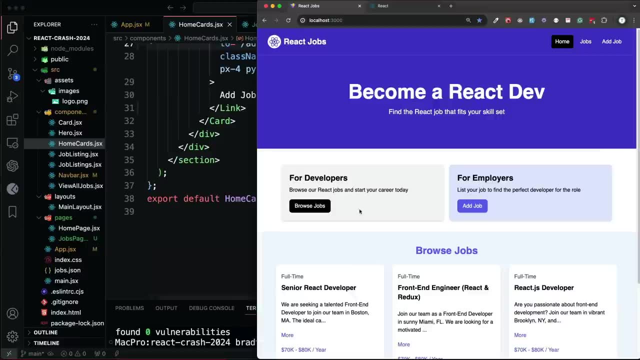 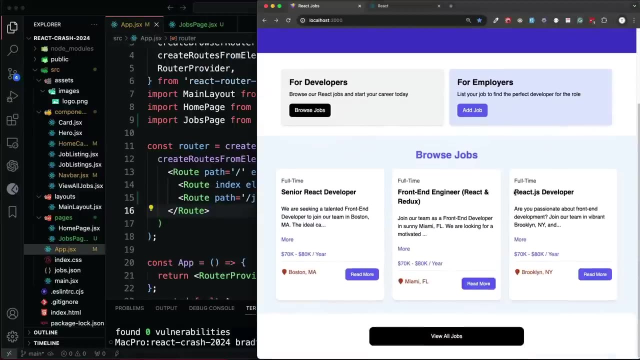 the add job. let's change that to link, change that to two and change that to just slash add job. all right, so that should work. this does. that route doesn't exist yet, but it will. then we have the the job listing component, so let's go into that job listing and let's bring in 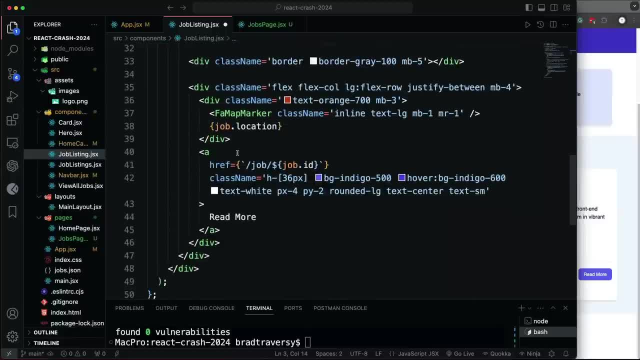 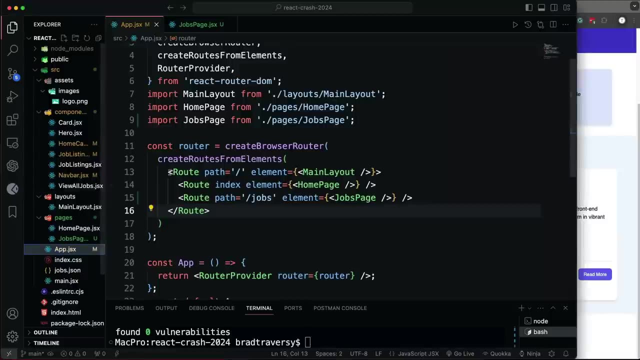 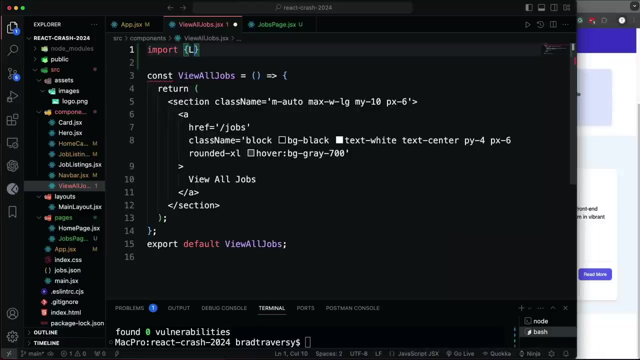 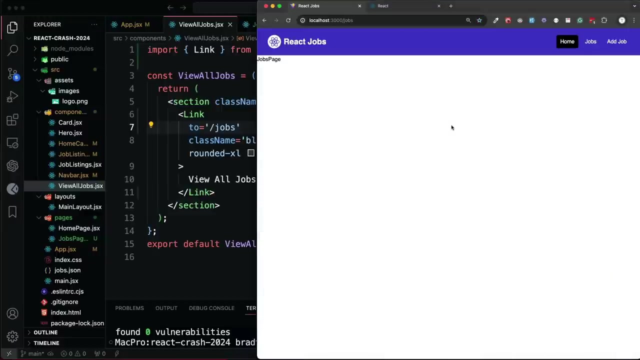 link and then the a tag which is right here, link to: okay, and then is that it. I think, yeah, I think that's it. did we do this one now? view all jobs. I want to do that as well. okay, and then change this and this. all right, cool. now a couple things I want to do before we. 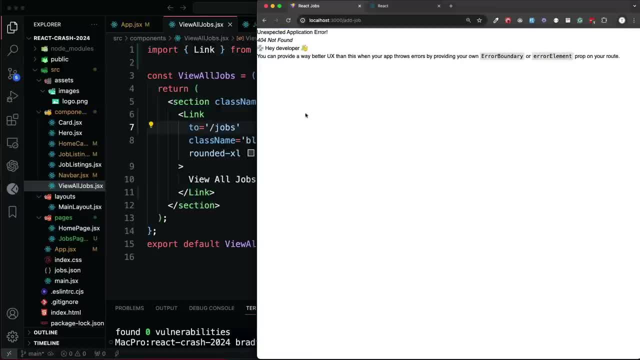 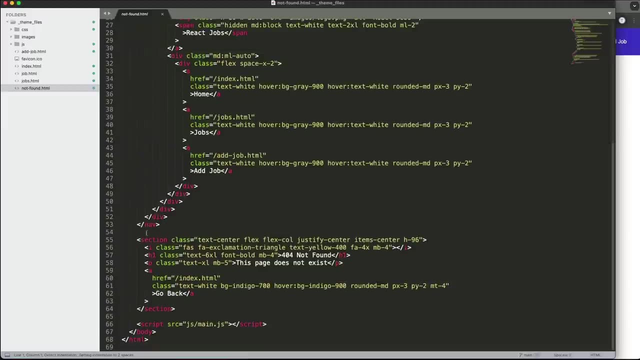 get to the jobs page. so one thing: I want to have a custom 404, because obviously this doesn't look very good. so what we'll do is go into the theme files, and I believe I have not found. yeah, right here, not found. so all we want here is: 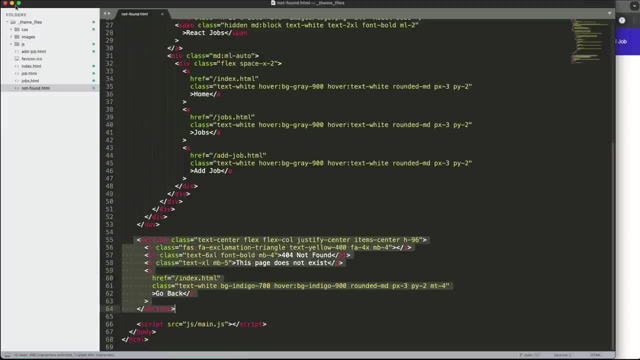 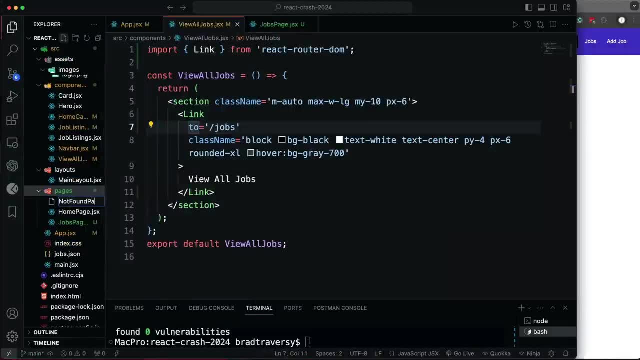 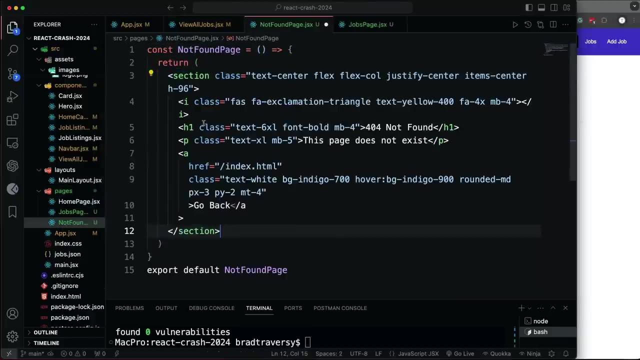 this, this set of files, and then we're going to go into the theme files and then go into this section. so I'm going to grab that and then let's create a new page. so in pages we'll say not found page- jsx and rafce, and then I'm just going to paste in that section. be sure to change. 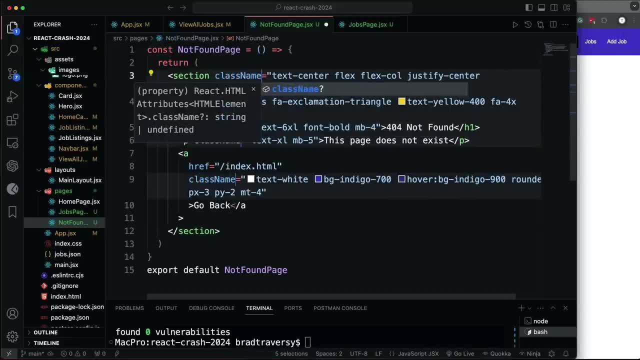 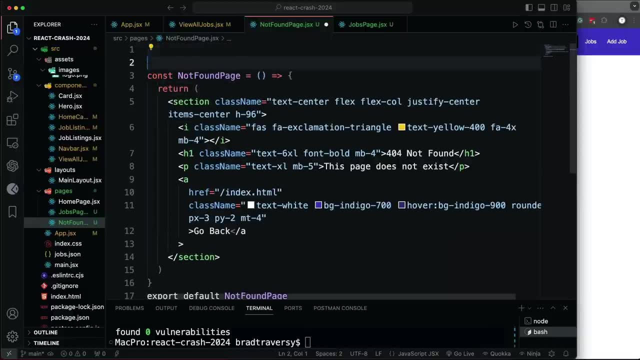 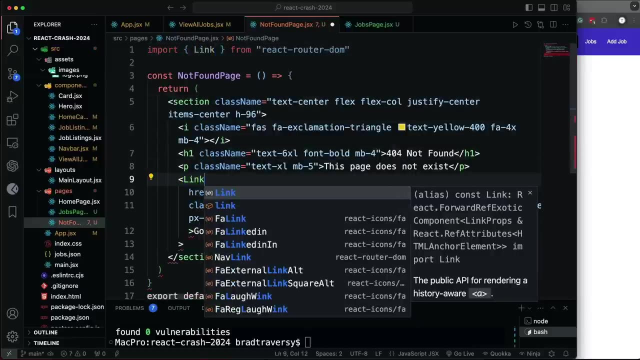 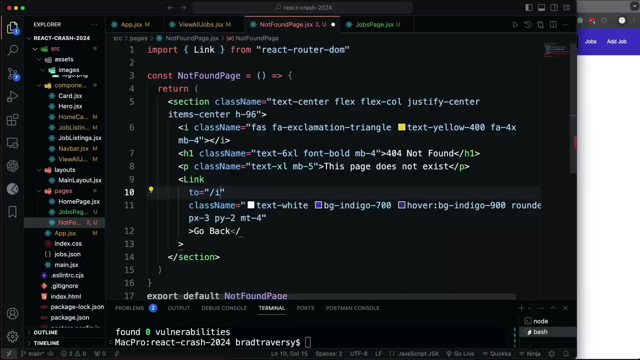 all the instances of class to class name and let's see we're going to bring in link into this file. but well, so let's import link and then change this a tag to link and change the href to two and change this to just slash, just slash. 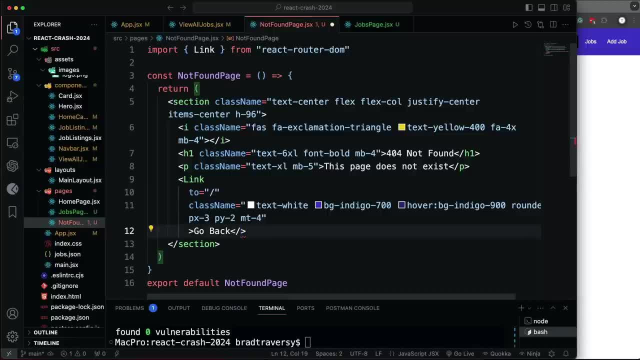 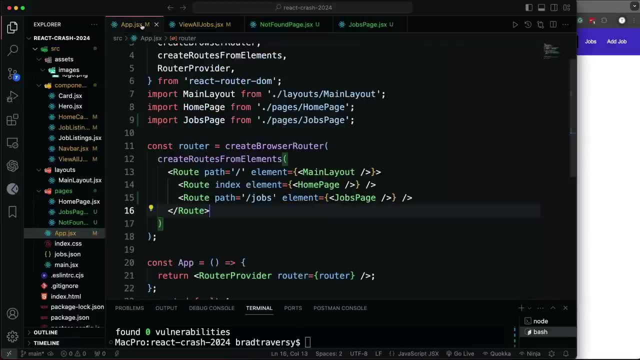 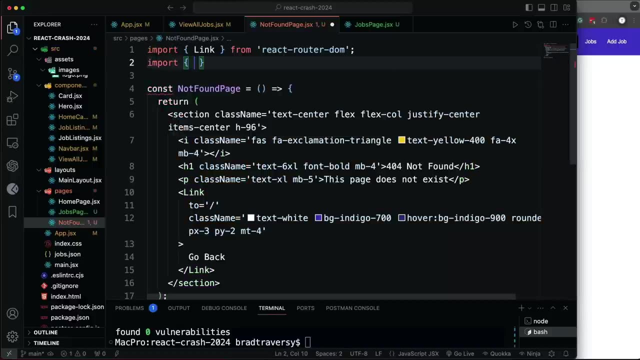 uh, why is this? all right, there we go. so now let's go to actually. do we have an icon? yeah, we do have an icon here, so i'm also going to bring in f a exclamation triangle from react icons, and then let's replace this. this i tag right here: 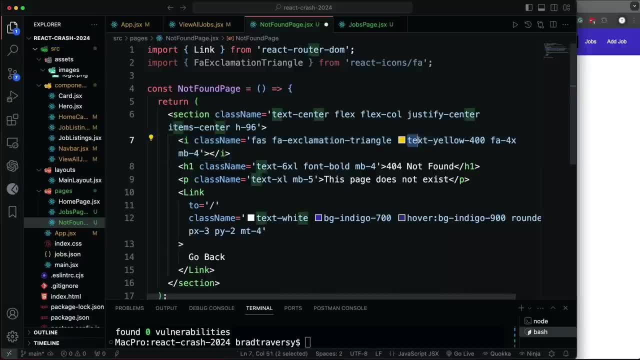 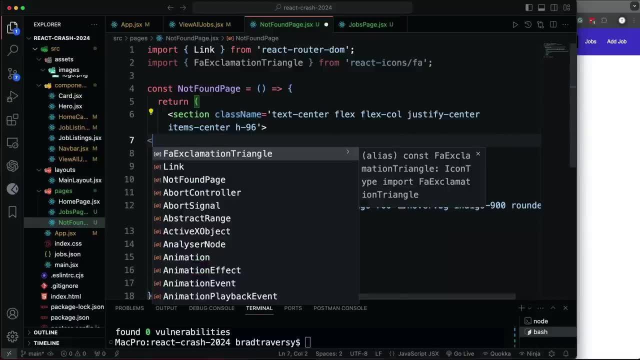 i'm just going to copy these classes, yeah, and then we'll get rid of the i tag, and then let's put in f a exclamation triangle and then class name, and then we'll get rid of the i tag and then let's put in f a exclamation triangle. 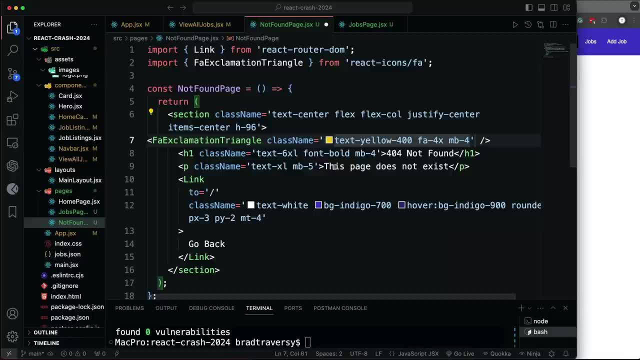 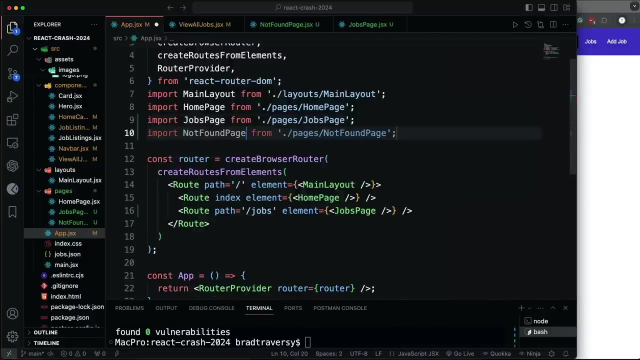 paste in. we're going to have text yellow and then, um, actually we don't need this fa class right here. we're going to get rid of that. let's add text dash 6xl. okay, now to make this show on pages that aren't found. we're going to go back to the main app component and let's import the not found page. 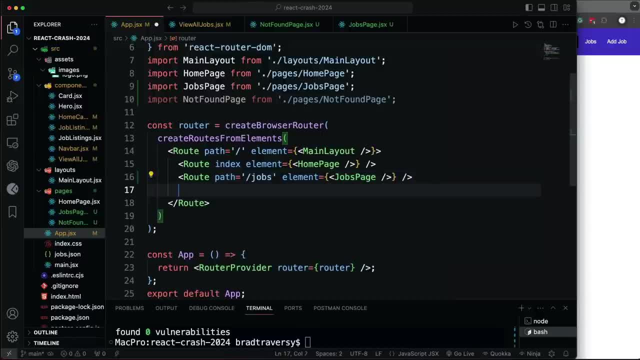 and then what we can do is add a new route. actually, we'll just copy that down and we're going to set this to the not found page and for the, for the path, we're just going to put in an asterisk. so this should be like a catch-all. so home should work, jobs works if i go to add job. 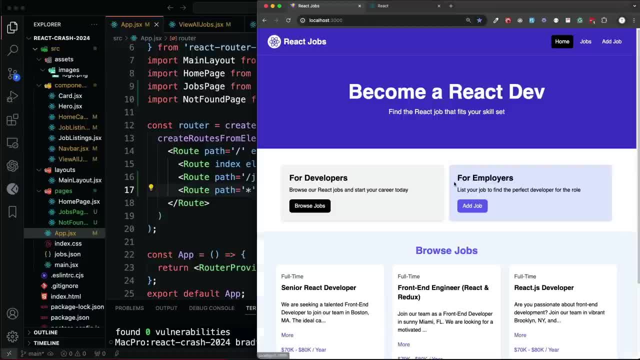 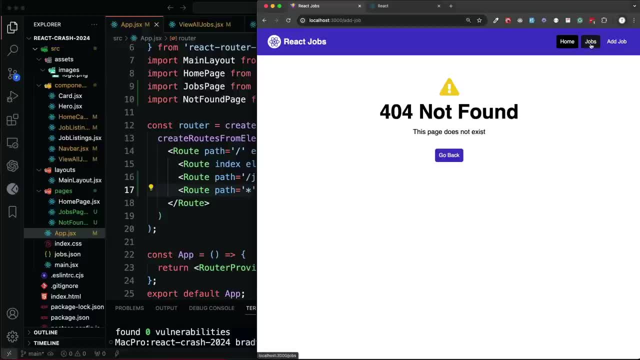 we get 404 not found, okay. so any page that's not found, you're going to get that, which looks a lot better. now the next thing i want to do is is the active link. so i'm going to go to the active link. so right now you can see if i go to jobs. the home is still active. so if we open up the nav bar, 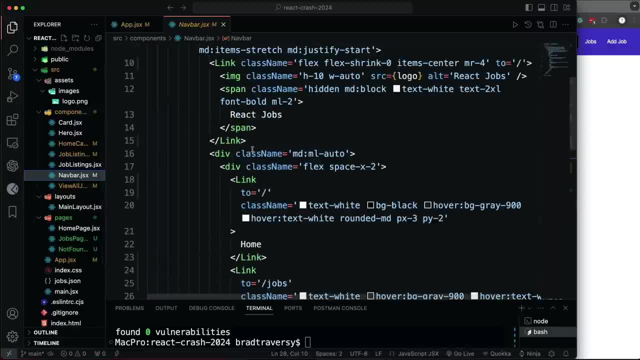 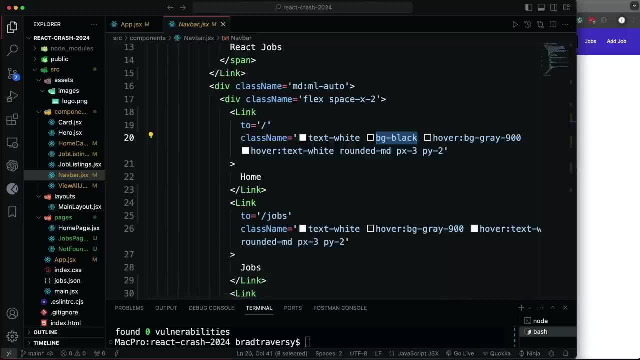 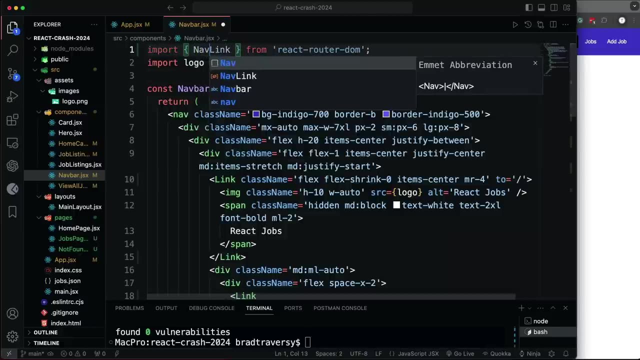 right here you'll see that the home link has a class of bg black. so basically we want to show that bg black on whatever the the active page is. now we can do that by bringing in something called nav link instead of link, which works. it works in a very similar way, except it adds a class, that's. 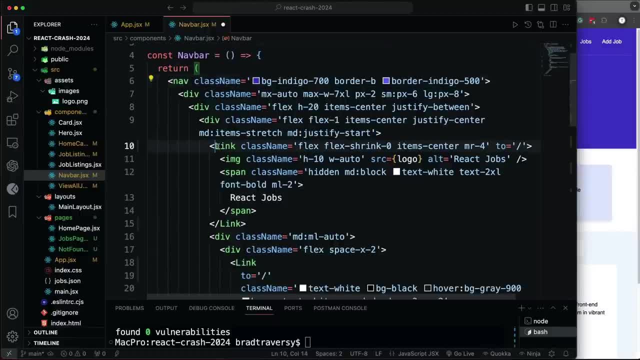 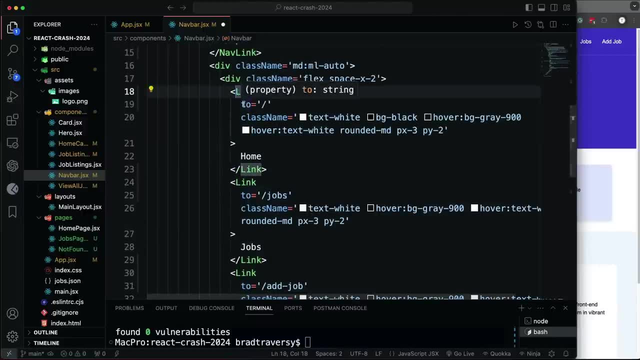 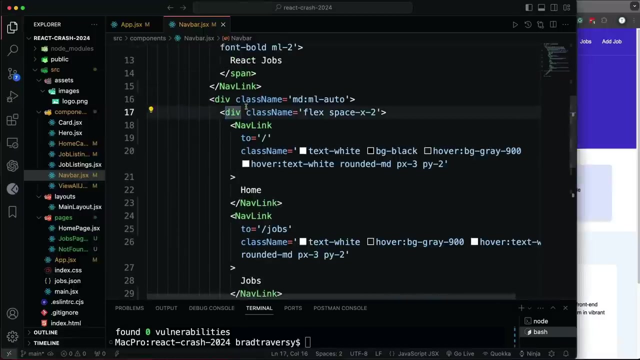 a class to the active link and we can change all the instances of link to nav link and it'll work the same way. so, right here, here, here and then here, all right. so if we do that, then this should still work the same way. so what we're going to do is go to the home link, which is right here, and 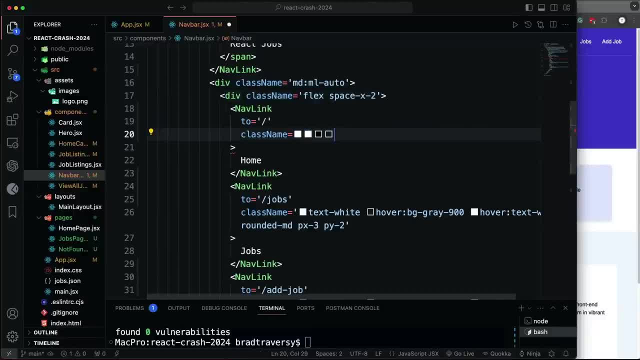 for the class name. let's just delete all this for now and and put some curly braces in here, and what we can do is actually pass in an arrow like this, and then in these parentheses we're going to pass in, uh, some curly braces, and then put is active, and then we can test this. so this will be a true or false if 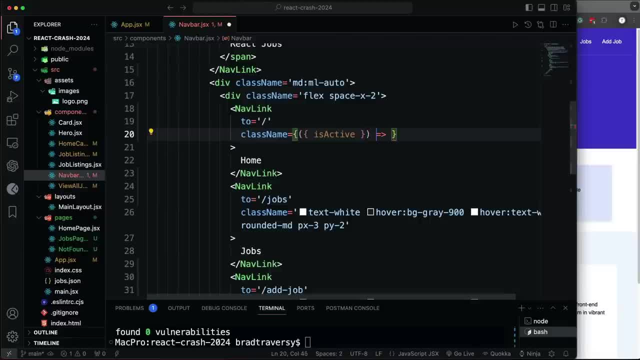 the link is active, if we're on that page, then this will be true. so then for the class name we'll have a ternary and we'll say if is active. so if this link or this page is active, then show a class, else should have another class. and i'm going to just copy all these right here and i'm going to 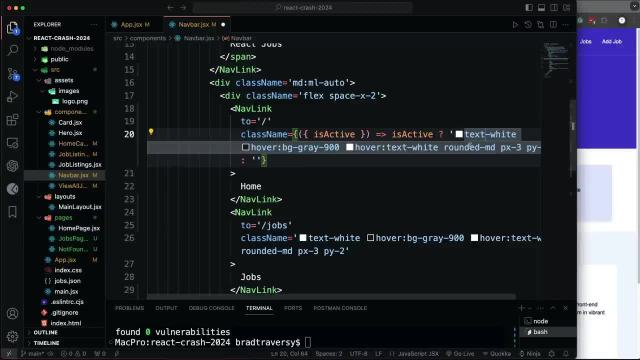 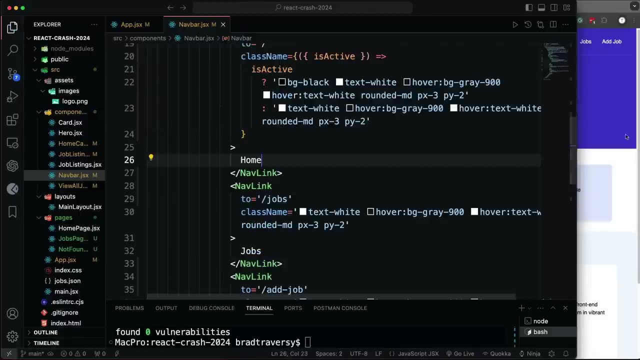 put that in the first one, but i'm also going to add in here bg dash black. okay, and then for the else, this one, i'm just going to put it in without the bg black. so now, if i save that so you can see it has a black background, if i go to jobs it doesn't. 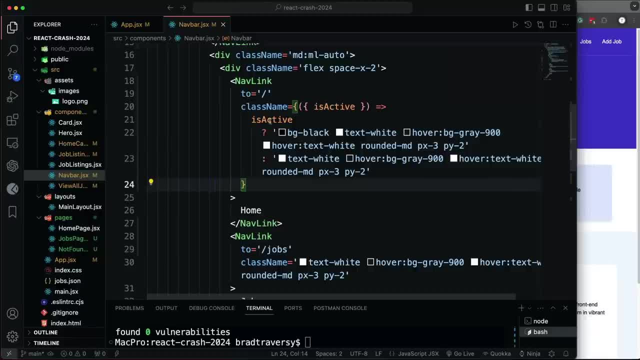 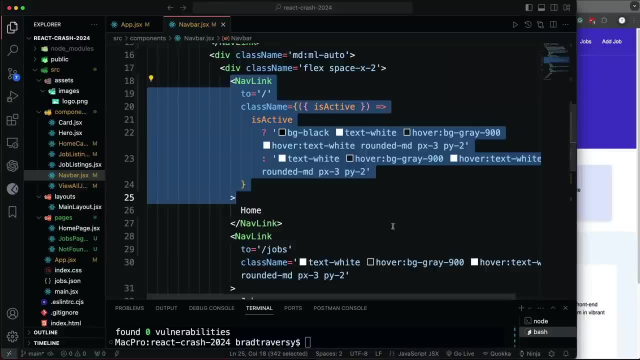 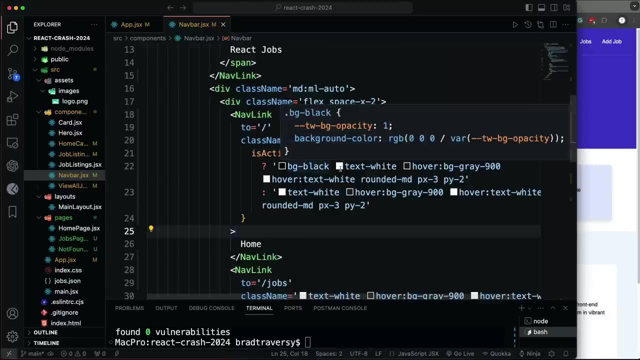 and we want to do that for all of these. so what we can do is just copy the first nav link. actually, you know, a cleaner way to do this would be, um, to put this in a function up here and then just add it. yeah, why don't we do that? that makes more sense. so let's grab the function. so this, the 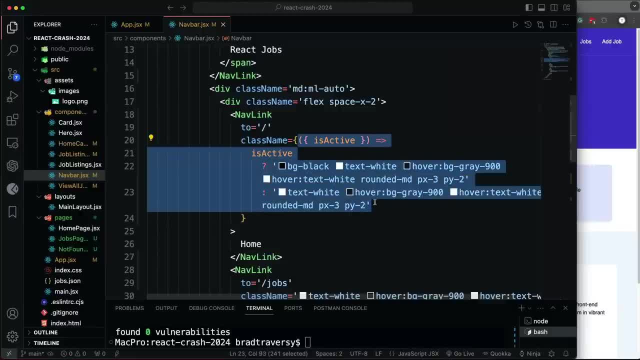 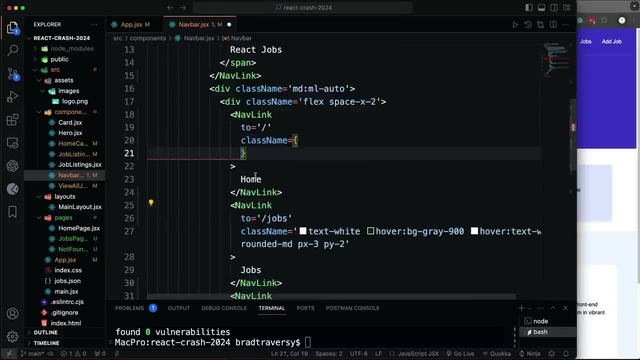 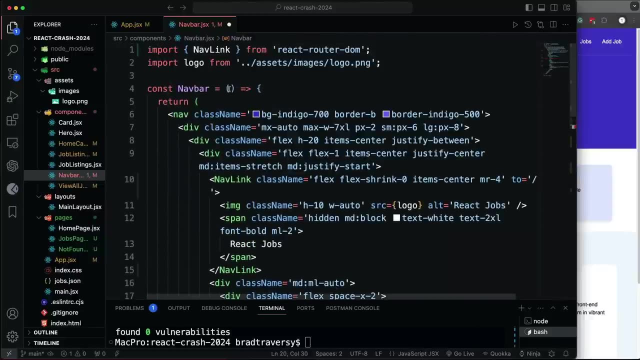 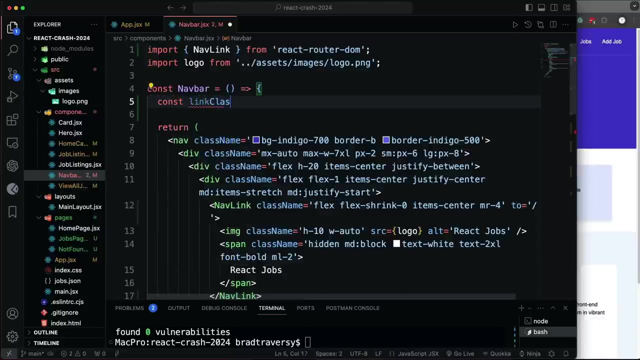 and then the arrow. so basically to this: and let's cut it so that all you have now, oops, so that all you have now is just the curly braces. and then we'll go up here and we want to go within the component and let's say const, we'll call this link class and then set that and then paste that in. 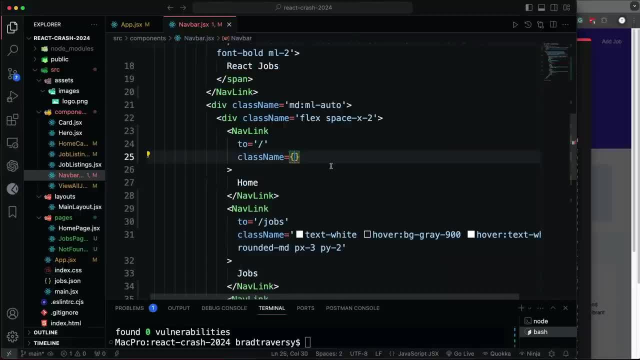 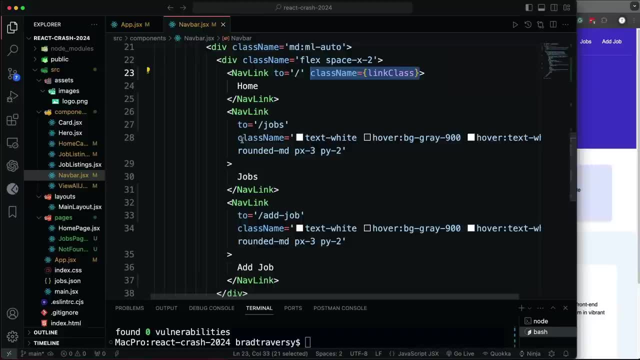 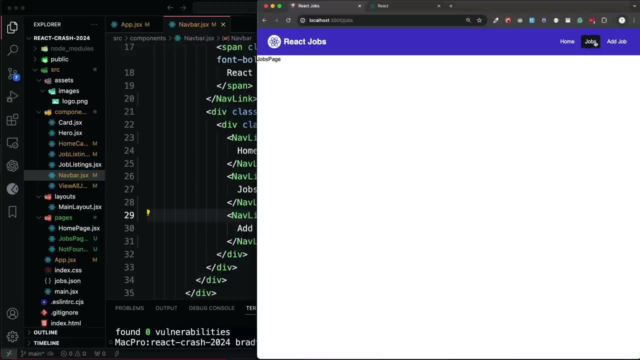 okay. so now what we can do is just simply add for class name, we can just add the link class and we can do that for all of these. so we'll take that, do it for that one and for this one. and now, if i go to jobs, now that's highlighted, okay, add job. i mean it still does the active. 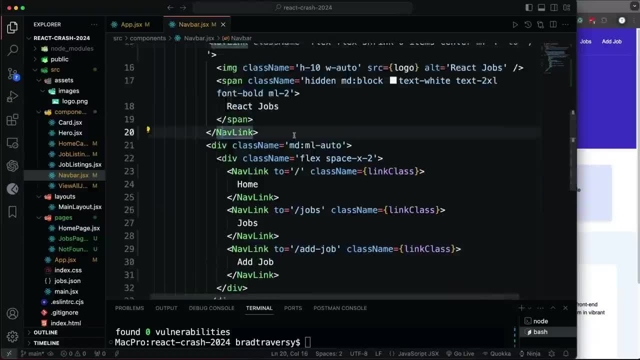 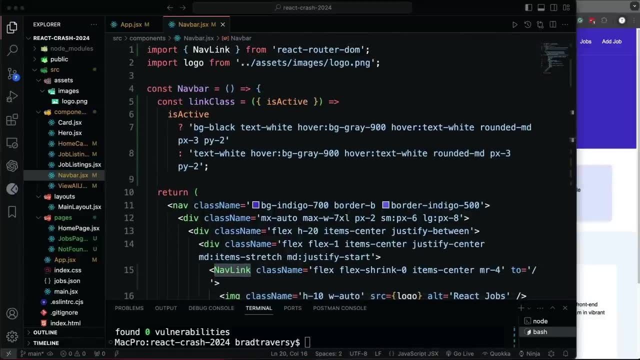 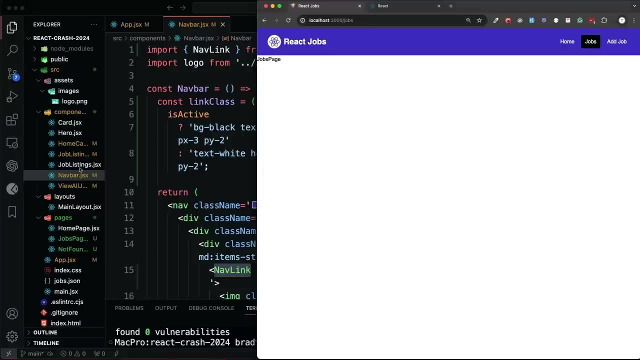 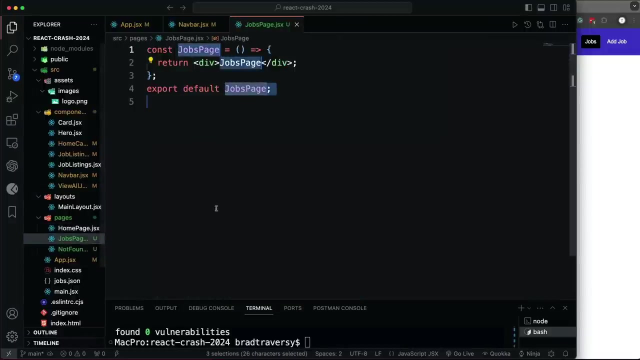 link, but it doesn't exist. so you can see, we make this, you know, dynamic by using nav link. so let's do the job. uh, the jobs page, which is going to be really easy, because i want to reuse the job listings component. so let's, uh, let's do this, let's go into jobs page. 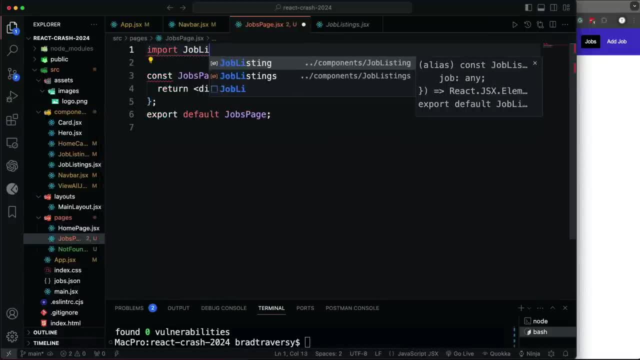 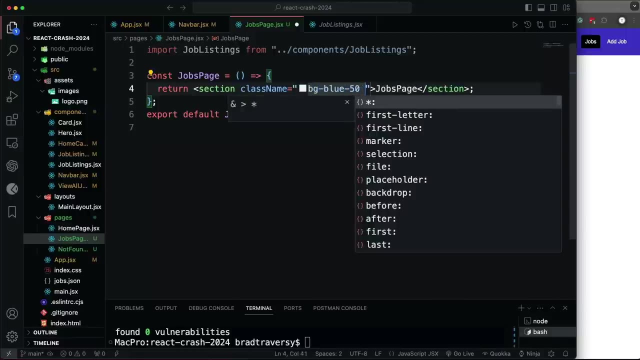 and let's bring in job listings. and then let's see, i'm just going to make this a section and give it a class name of bg, dash, blue, dash 50 and px4 and py6, and then all i'm going to have in here is the job listings. 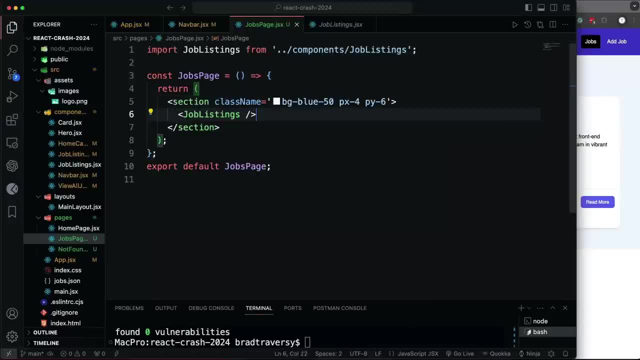 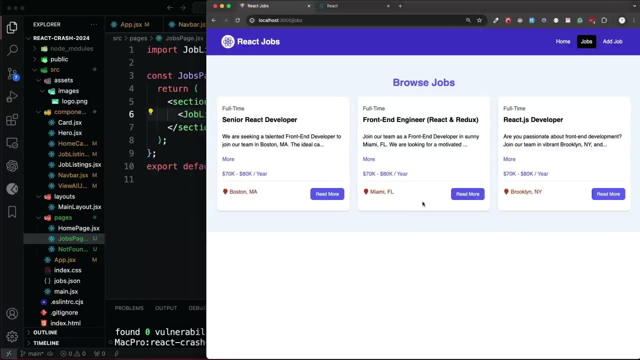 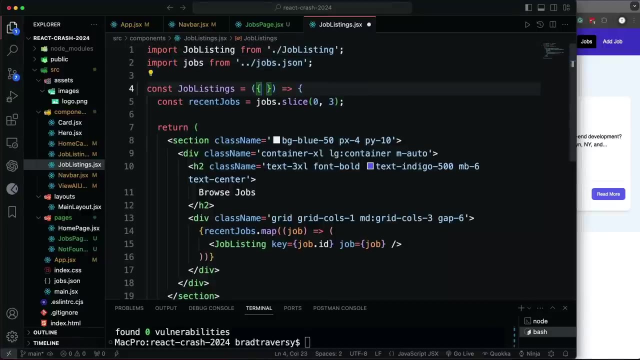 component. so let's add that. okay, so the issue here is that we're only seeing three and we want to show all of the listings. so let's do this. let's pass in a prop into job listings and then we're going to set it to false by default, and then let's- let's change this. 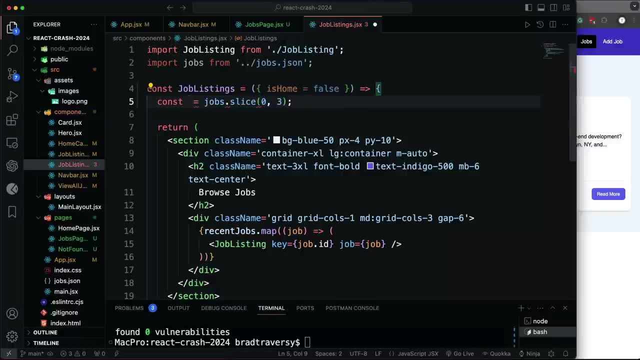 variable. let's: um, yeah, because instead of recent jobs, we'll call it job listings, and then we're going to say, if is home, then we want to set that to job slice, just like we have it else. then we want to set it to just jobs, which is coming from the file, which is going to be all of. 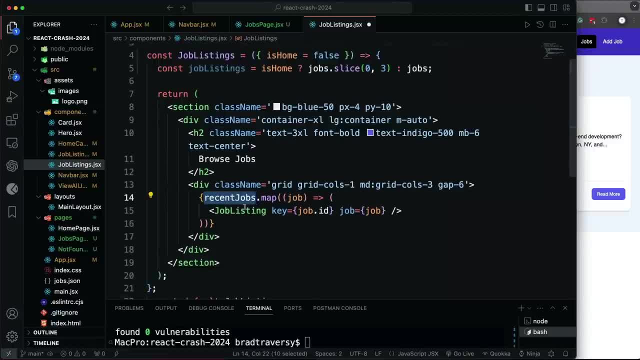 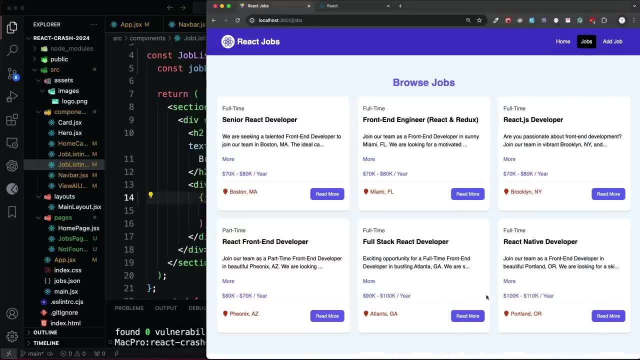 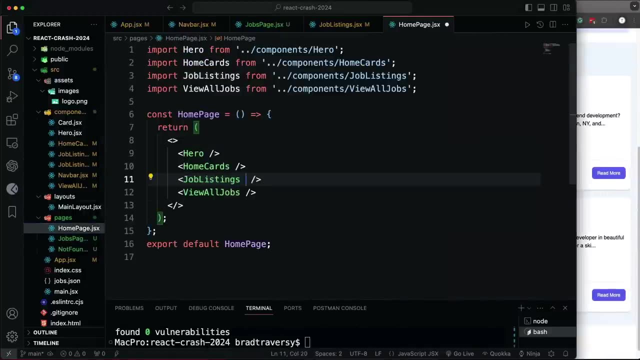 the jobs and then down here, instead of creating a list with recent jobs, we'll create it with job listings. so now, if i save that, you'll see now it shows all six. now on the home page it shows all six. however, let's go to our home page and let's pass in that prop of is home and we'll set that. 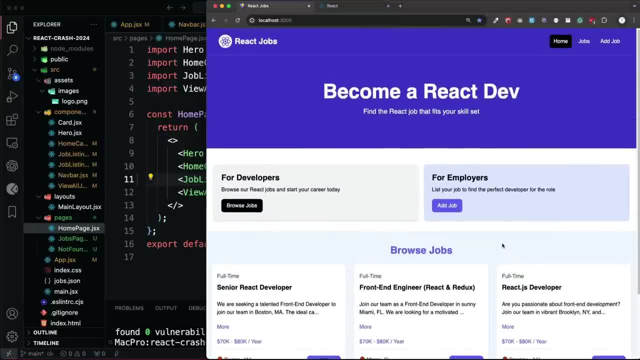 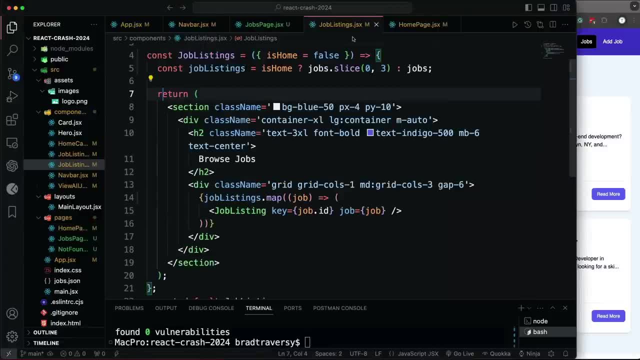 to true. so now, if i save, now, we only see the three on the home page. so let's go to our home page. and let's go to our home page so that takes care of that. we could even change the title based on if it's home or not. so let's say, let's say this: if is home, then let's show um. 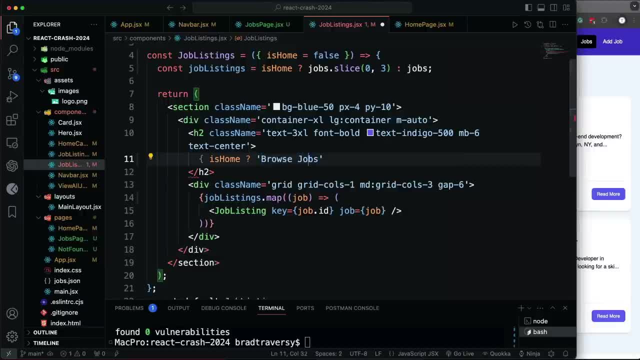 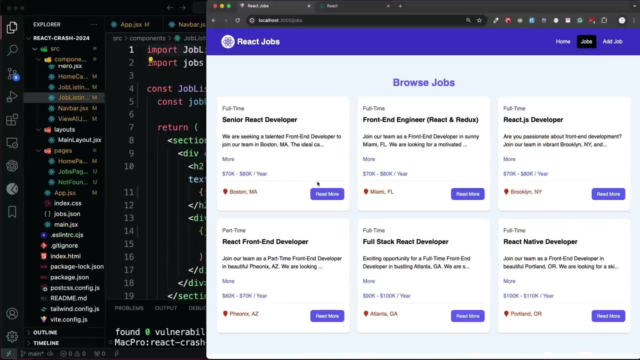 browse. no, we'll do recent. yeah, if it's home, we'll say recent jobs. else we'll say all jobs or browse jobs, yeah, browse jobs. so browse jobs, recent jobs. before we get into the single page: right, if we click on this, we go to job slash and then the id. before we do that, let's switch from just bringing in a json file to 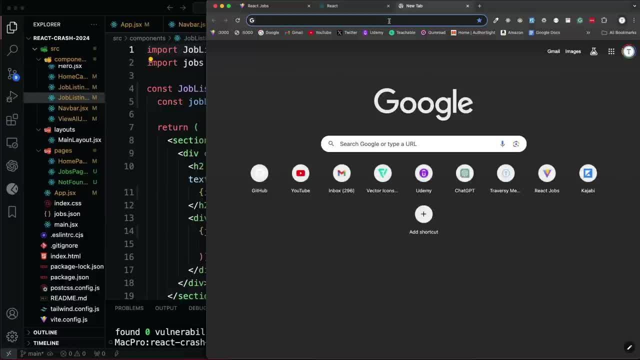 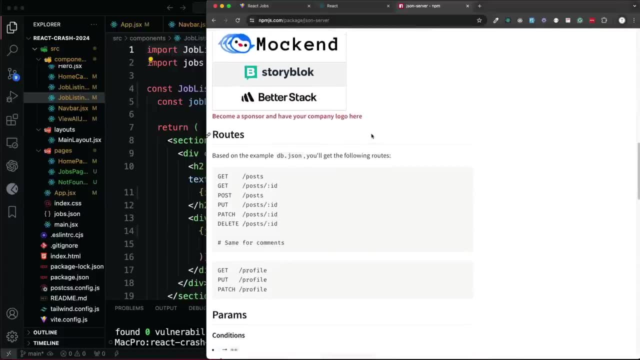 actually fetching data from a back end, and to do this we're going to use something called json server, which is a fantastic library that basically lets you create a mock api and you can send, get, post, put, patch, delete requests, so you can create crud functionality. it can be any resource you want, because all you have. 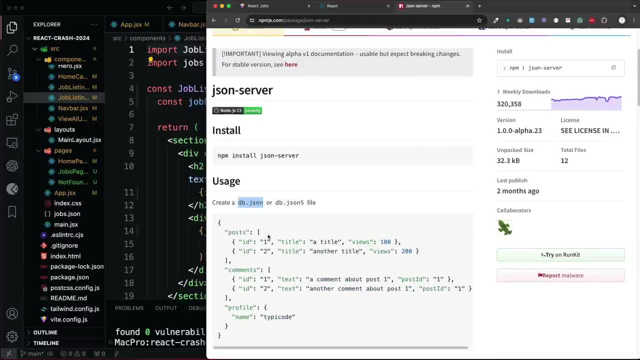 to do is create a json file, which we already have, and you can put any type of resource you want in it, so we can use our existing json file. we just have to basically put back what we changed, which was make it an object that has a jobs, a named jobs array, and then we can install json server. 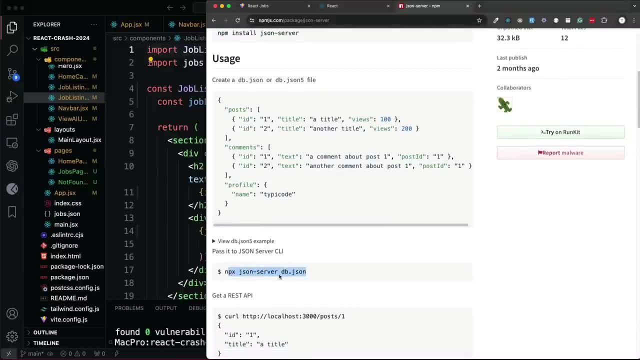 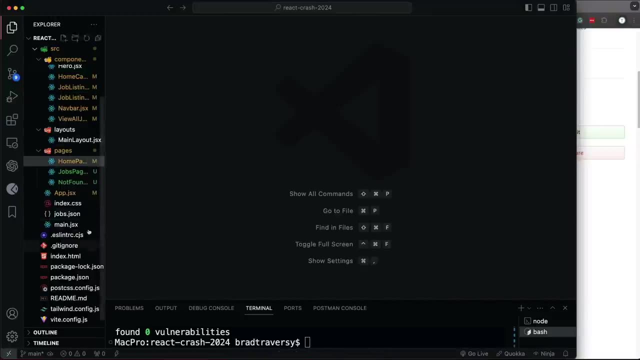 and then we can simply run it like this, so we can create an npm script to run the server, which will run on a separate port than our front-end react app. all right, so let's do that. let's uh, for now just close all this stuff up, and then the json file, the jobsjson file. we're going to go ahead. 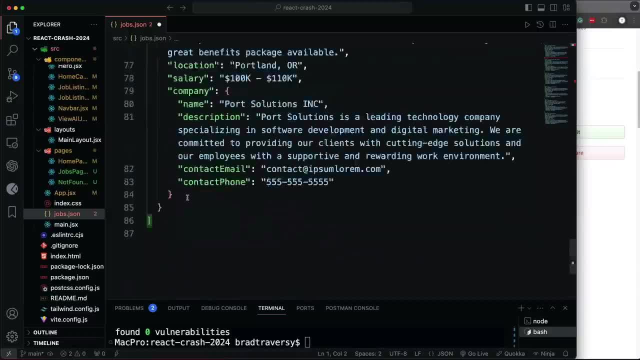 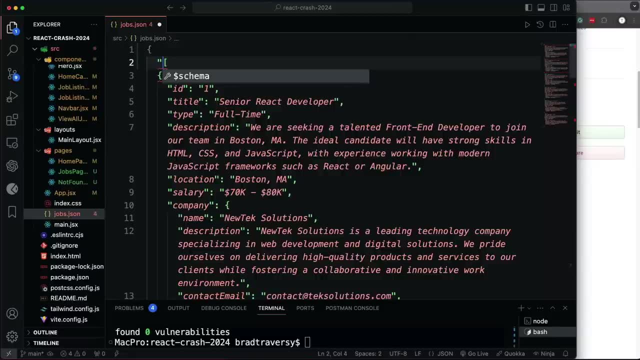 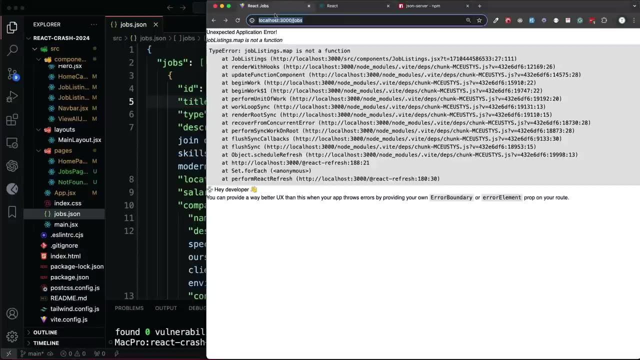 and just put opening curly brace here and then a closing one at the end, and then we want to just name this array. so we're going to put double quotes, call this jobs and then set that to that array. now that's going to break our application. so if we go back you can see it's broken because it's. 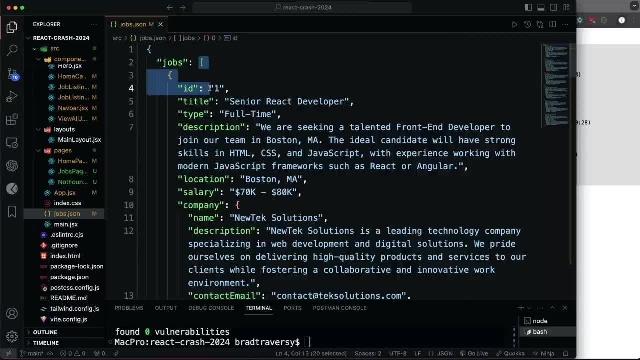 just looking at the jobs file and it's looking for an array, not an object with an array in that object. so that's fine, and don't worry about it being broken for now. we're going to fix it. but let's come down and let's install json server. so i'm going to install as a dev dependency json. uh, json dash, right i. 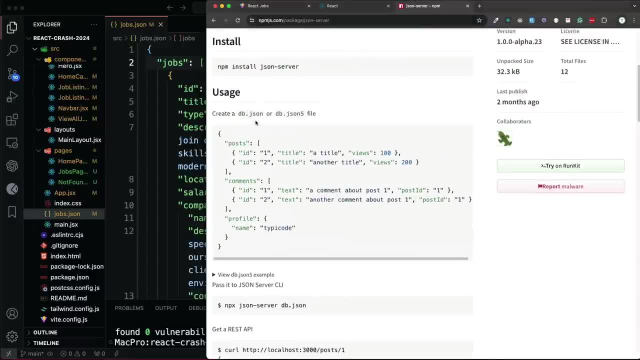 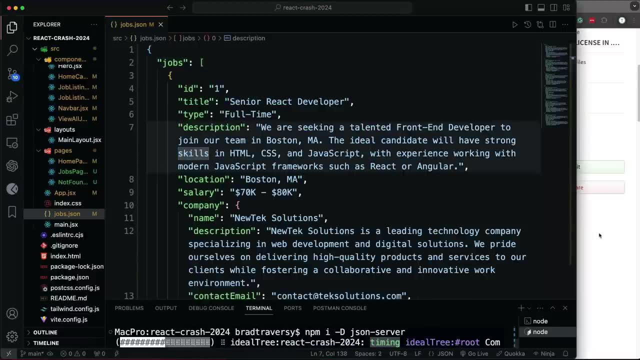 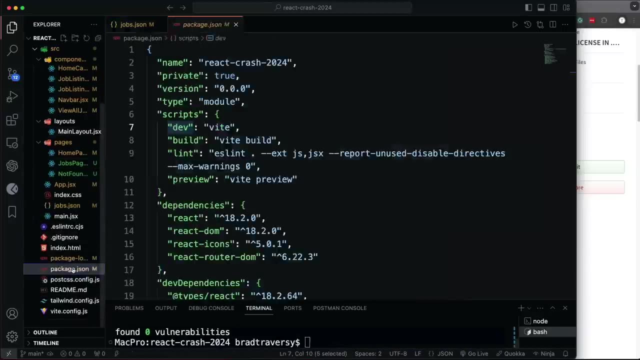 believe it's. i've done this so many times, i don't know why, i don't remember. yeah, it's json dash server, okay, and then as far as the the command to run json server, we're going to put that in our packagejson file, so let's go here and then let's add in. 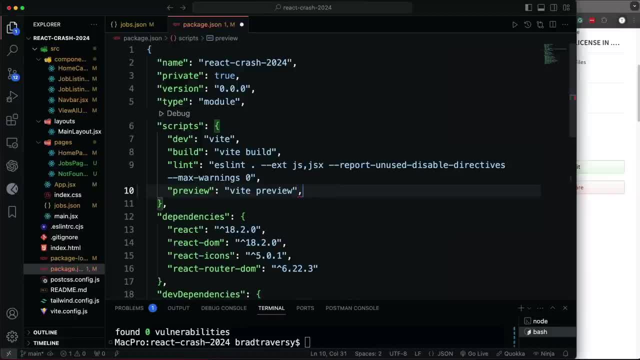 yeah, we're going to add in a server. we'll put this at the bottom here, just put a comma and then we'll call this server and what we want to run here is going to be json dash server and we want to dash dash. watch in the source file. 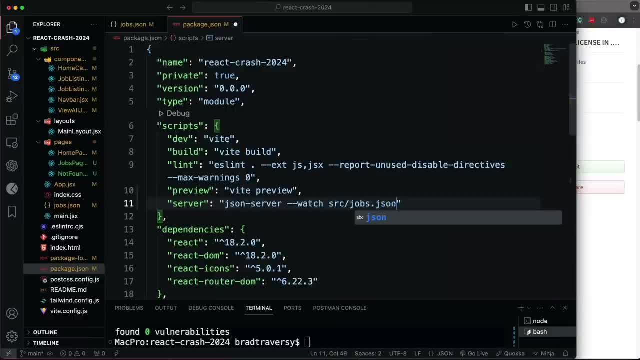 folder, the jobs dot json file and then dash, dash, port. now i i have something running on port 5000 on this machine. that's usually what i would use, so i'm going to use 8000 for the server, but feel free to use whatever port you want. i think it's. i think it's 5000 by default, i'm not sure. 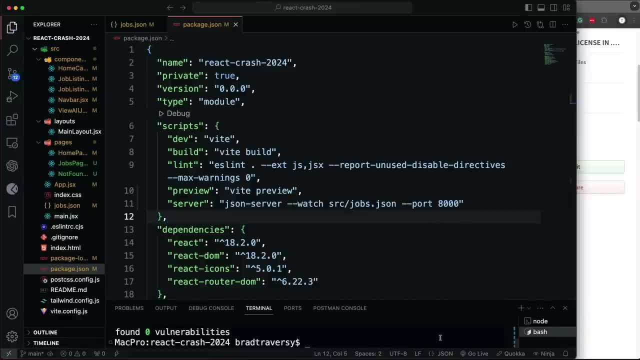 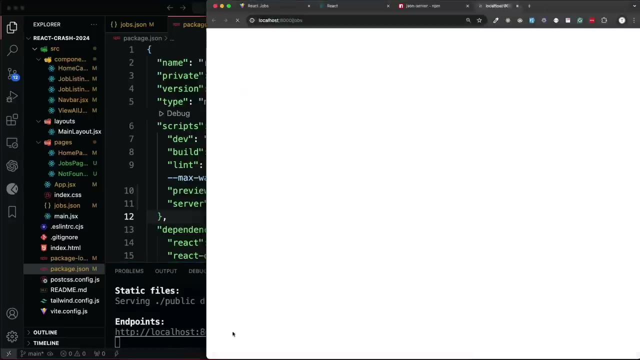 but let's go ahead and save that and then i'm going to run. so i already have my react dev server running in this terminal, so i'm going to go into this one and do npm run server and, as you can see, we have an endpoint of localhost, 8000 jobs, and if i go to 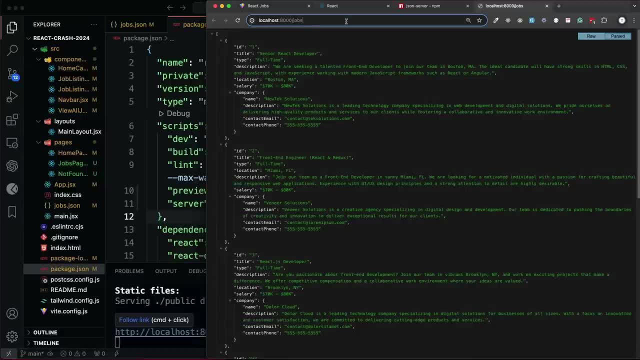 that in the browser i'm now seeing my data. i can even go to job slash and then the id and i get the single post. so it's it's just like if we built a rest api with express or django or anything else. we can also make post requests and add one. 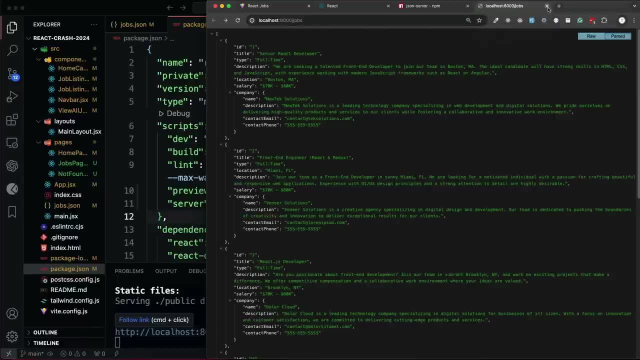 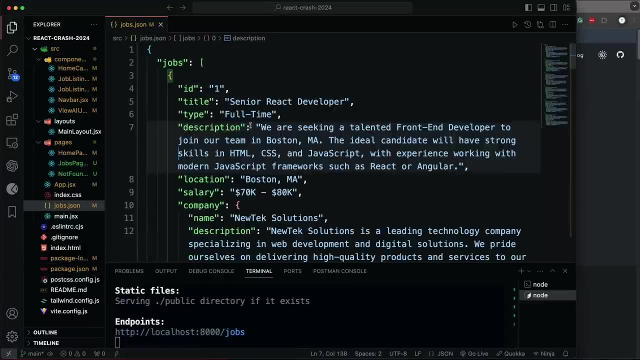 and it'll get added to the actual json file. we can edit it, we can send a put request, we can send a delete request. so we essentially now have a back end, all right. so so where i want to fetch this data is going to be from the job listings component. 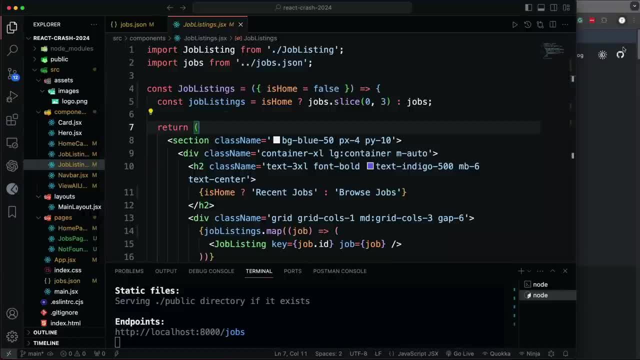 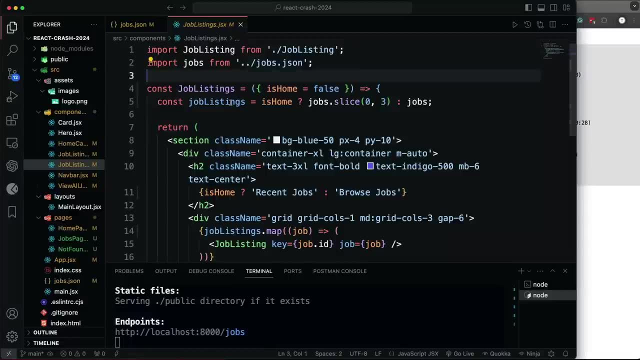 because that's where that's the only place in this application where we need the jobs, because we're using this component on both- though we can't see it now- but we're using it on the home page and on the jobs page. so let's, uh, let's. 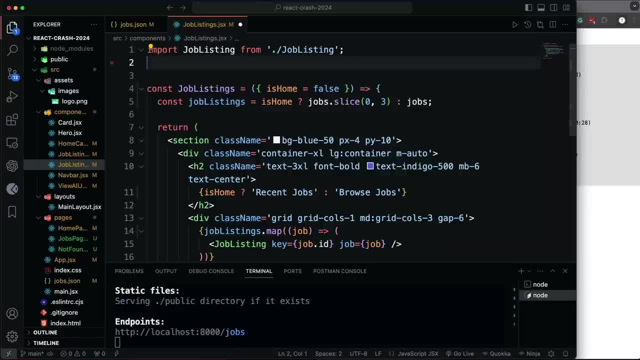 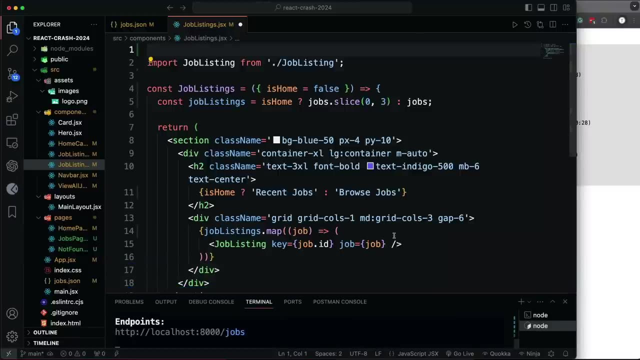 change this up a little bit. we're no longer going to just bring in the jobs file. we're going to make a request and we're going to do that inside of a use effect hook, because what the use effect hook does is it allows our components to to have side effects, and we want. 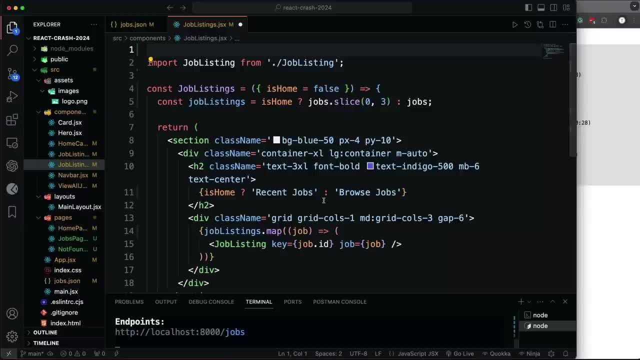 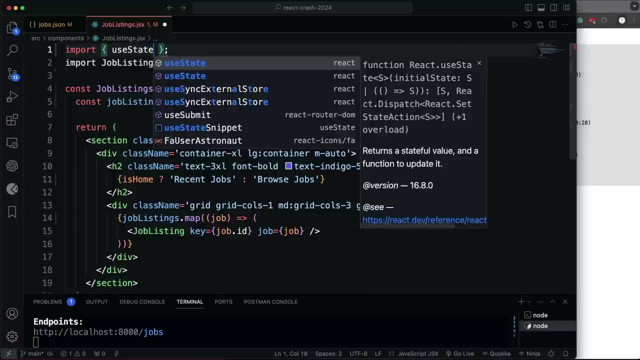 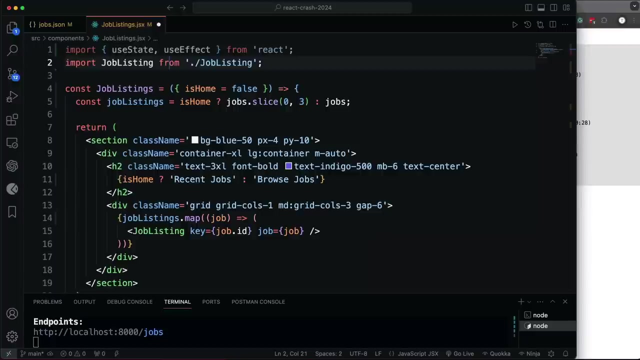 a side effect of fetching data when the component renders. and when we get those, those jobs from the api, we want to put them in state, so we will also want to bring in use state. so let's import. we're going to import use state and use effect from react and as far as the uh, 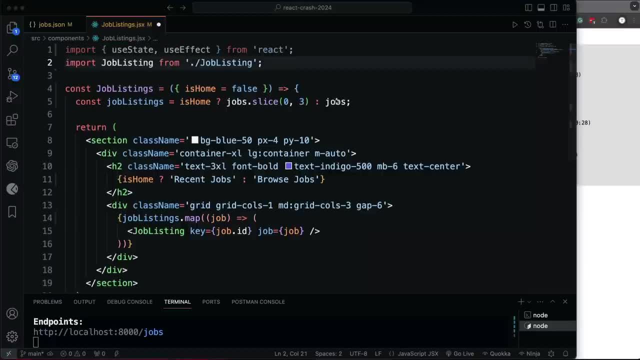 let's see, let's- um, yeah, let's add the state. we no longer need this because we're not dealing with. um, yeah, we'll just get rid of that. and then let's create our state. so, just like we did with the show details in the job listing component, we're gonna add a piece of state here for our jobs. 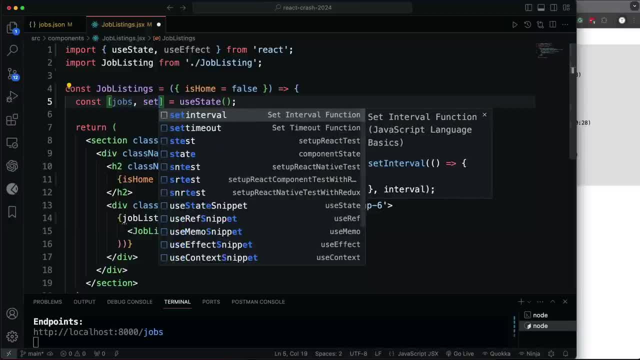 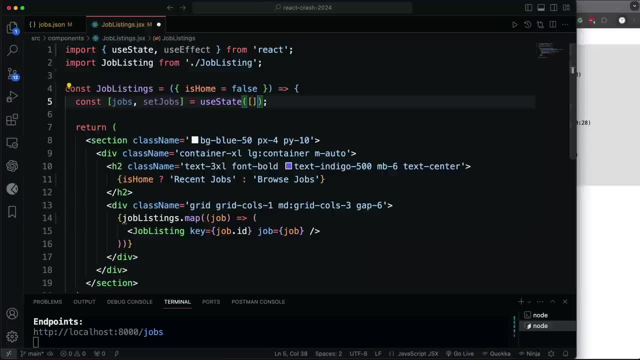 so remember this takes two things: the name of the state and then the name of the function to update this state. so jobs and set jobs, and then the default value we want for jobs goes in here, which is going to be just an empty array. because it's going to be an empty array. 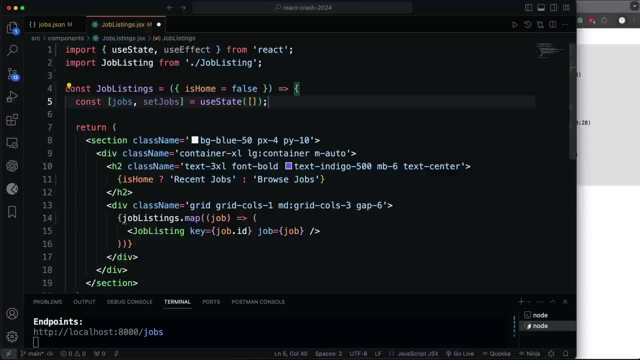 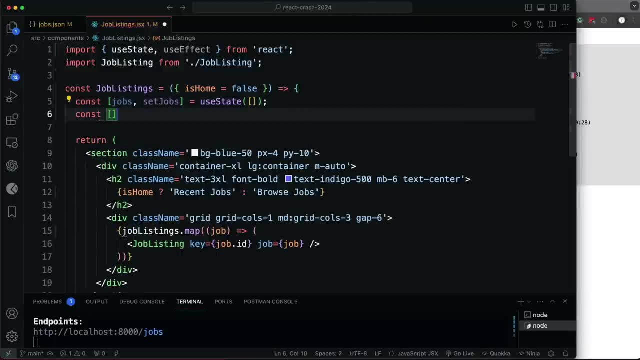 we'll make the request when the component loads through the use effect and then we'll fill this with the response from the API. Now I'm also going to have a piece of state for the loading, So loading and then set loading, So that way we can show a spinner or something when it's 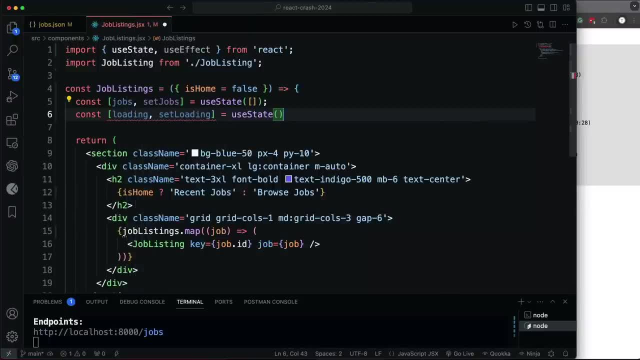 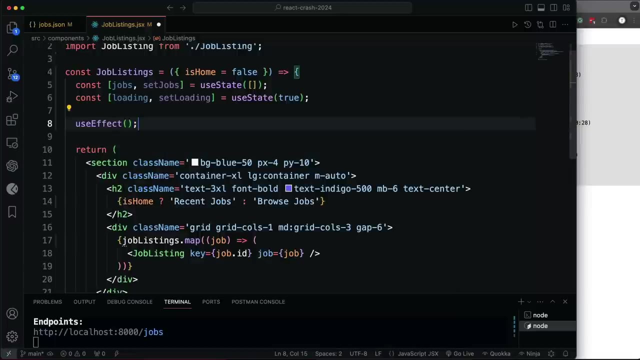 actually fetching And I'm going to set that to use state And as a default I'm going to pass in true And then, once we do the fetching and it's done, then we'll change it to false. So now let's add our use effect. So we're going to say use effect. Now, the way this works is it? 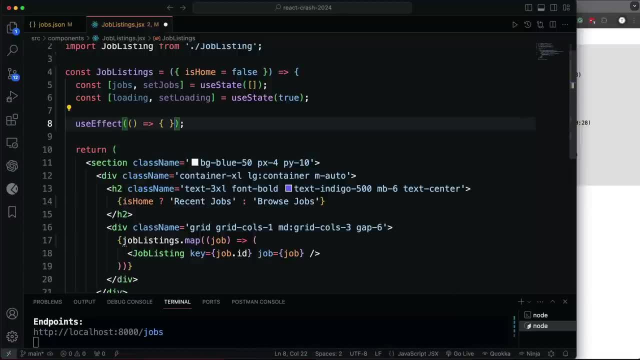 takes in two things: it takes in a function And then it takes in a dependency array. So if you put something in here- like, let's say, we had a variable called name or something like that- if we put name in here, then every time that name changes this use effect will run. Now. 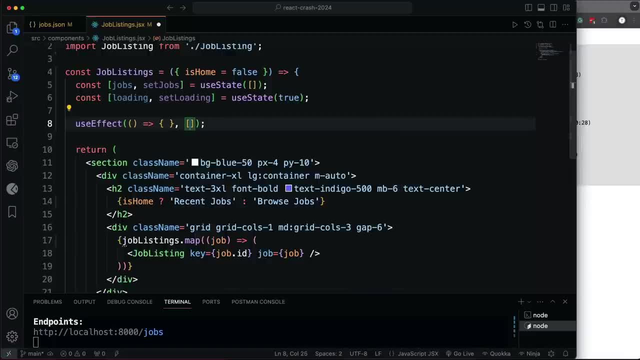 you want to have an empty array. even if you don't have anything, you know any variables you want to put in here, Because if you don't, it's going to just be a never ending loop. So you want to have this. 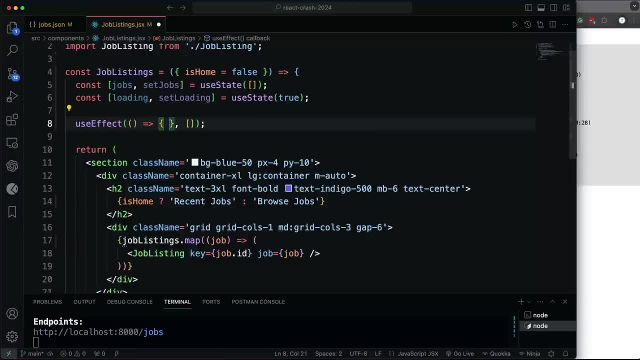 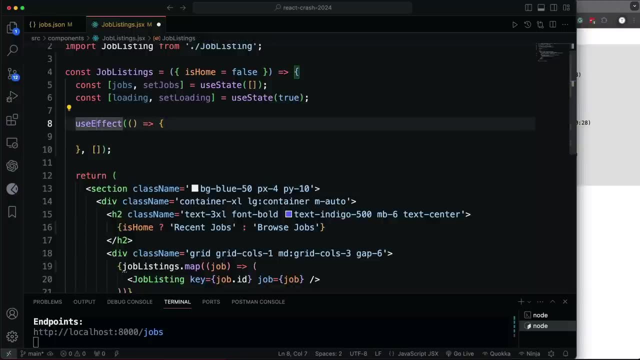 empty array in there in most cases, And then in this function, here I want to do our fetching And I want to use a sink await. However, you can't do this. you can't say a sink right, I can't do that, And then in here say await fetch, I can't do that. So 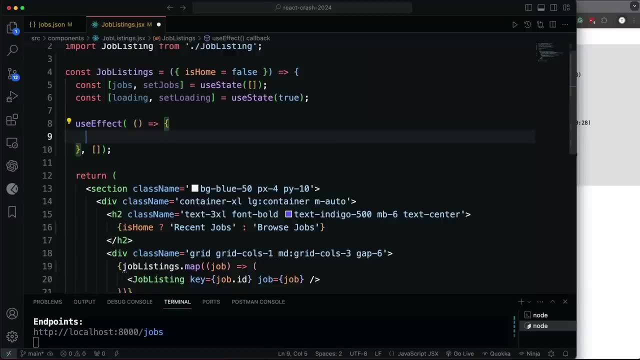 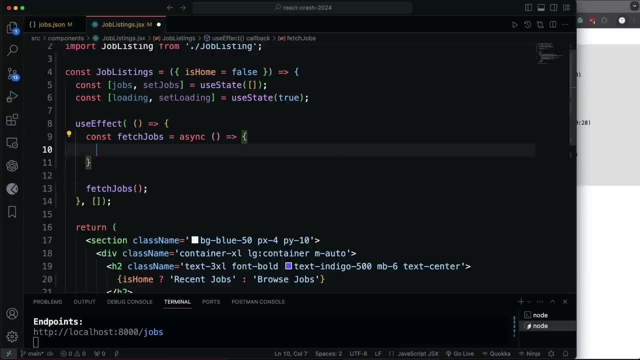 what we need to do is create a separate funk async function inside of here. So let's say: const- fetch jobs, set that to a sink, And then we do our fetching and then just make sure you call it So right, here we'll say fetch jobs. So in here I'm going to do const res, set that to a. 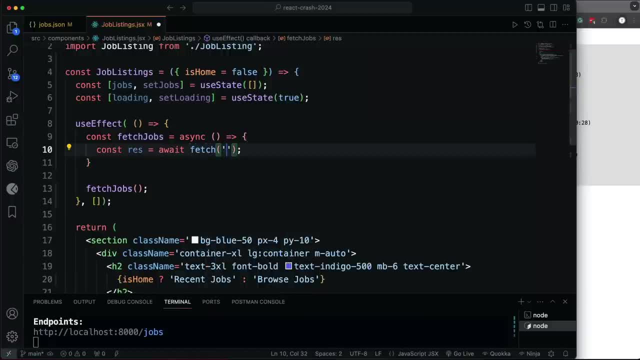 wait, fetch, And we're going to pass in here, let's say, HTTP, And then our back end, which is local host, local host, and I'll show you how we can add a proxy after, so we don't have to always. 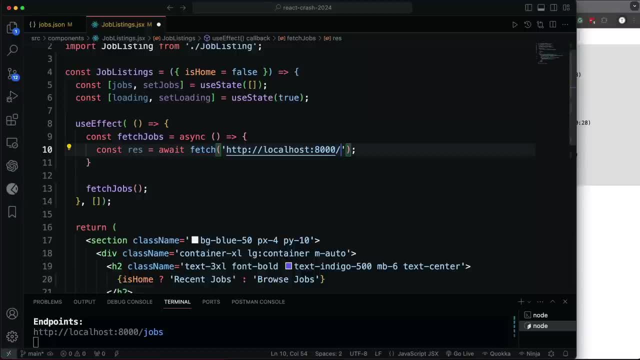 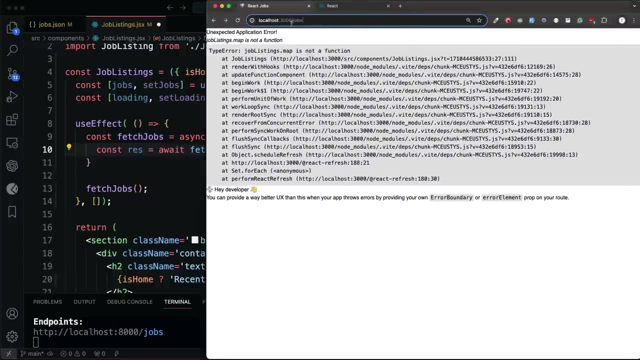 put in this local host 8000.. But for now we'll just add that And let's do slash jobs, right, because that's what we saw in the browser. So if I were to do local host 8000 jobs, that's our data. 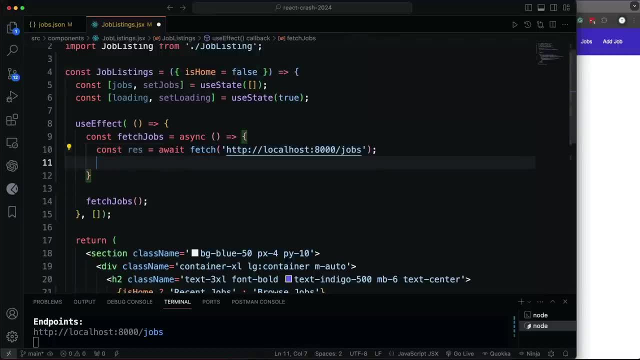 So that's what I'm getting here. And then let's do const data, set that to a wait resjson, And that should give us our data, And what we want to do is set jobs. we're setting this, this part of our state, to the data that's returned. Now I mean, we don't have to, but I'd like to put 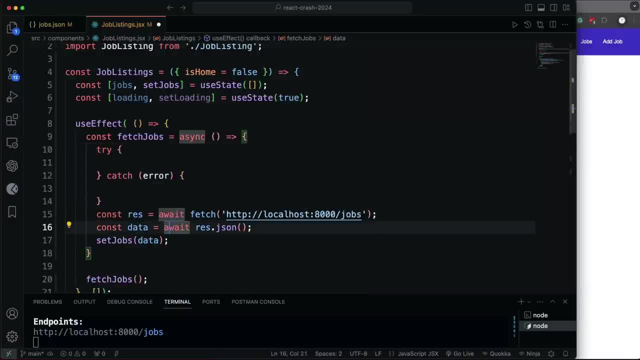 this in a try catch. So let's do that, And we'll take these, these three lines here and move them into the try And then in the catch. in the catch I'm just going to do console log for now And say error. 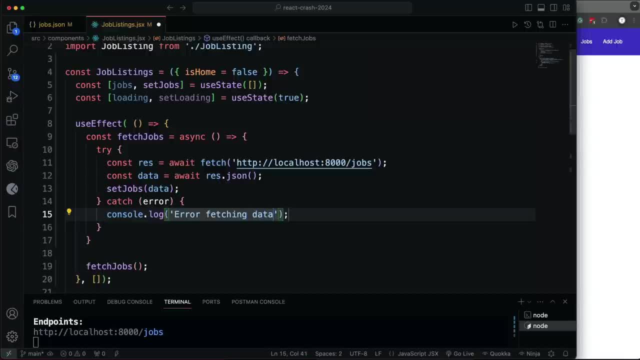 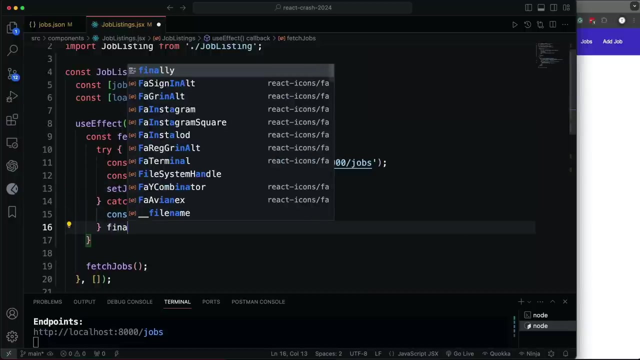 fetching data And we'll also pass in error. Now we want to set loading to false, whether it's successful or not, So I could put set loading false here and in here, But since we have a try catch, we can just add a finally, because whatever we put in here will run either. 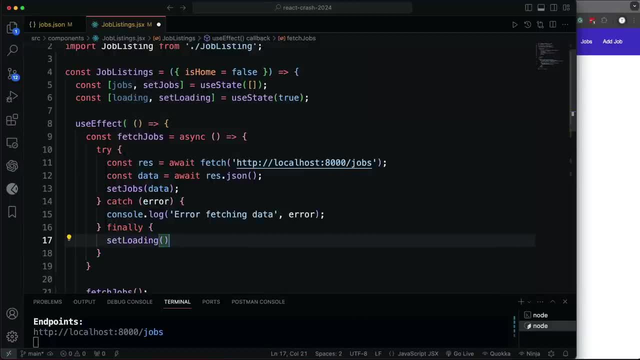 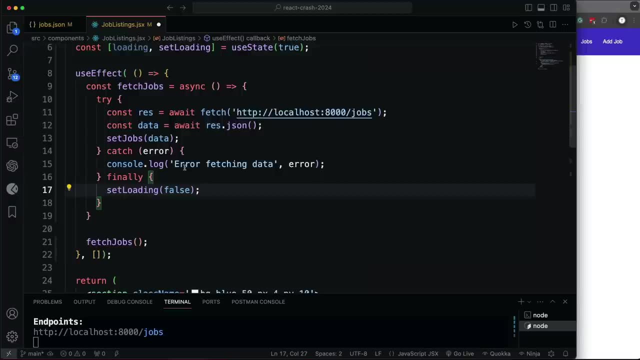 way, whether it fails or not. So that's where we want to put our set loading and set that to false. All right, and then, yeah, so that should work And it's going to put it into the jobs And. 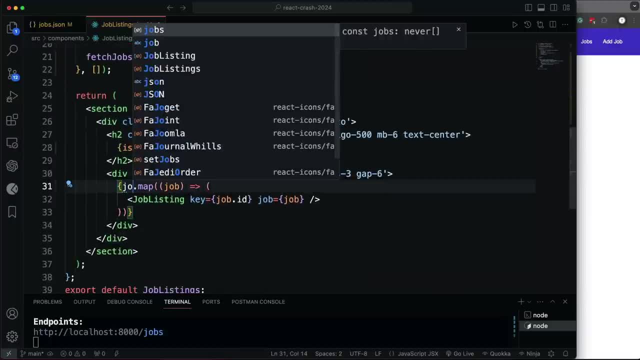 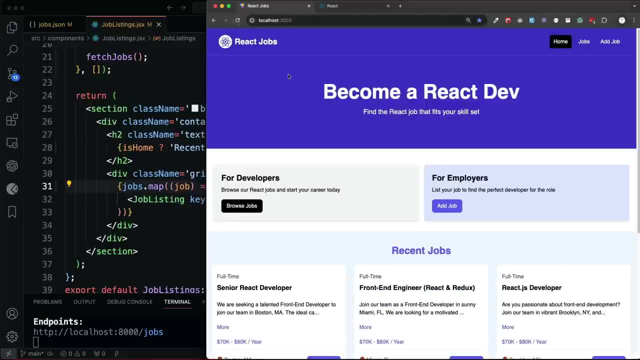 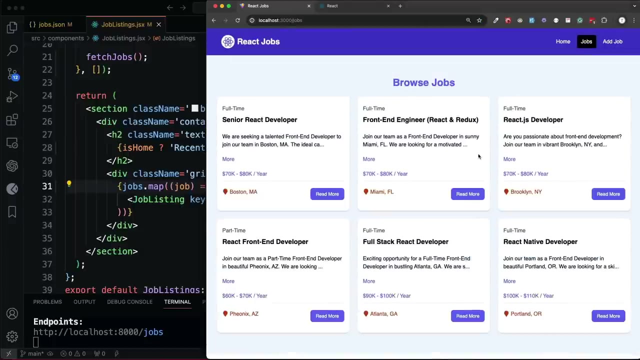 then down here let's change job listings back to jobs, So we'll save that. And then let's go, let's see home. And now you can see we have six again, which is fine, we'll hit, we'll handle that. If we go to the jobs page, there we go. So these are coming from our API. Now we're. 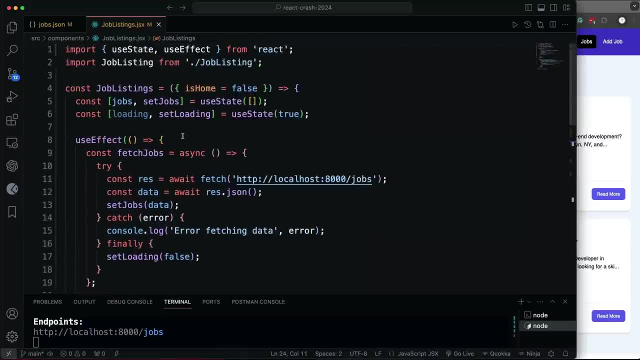 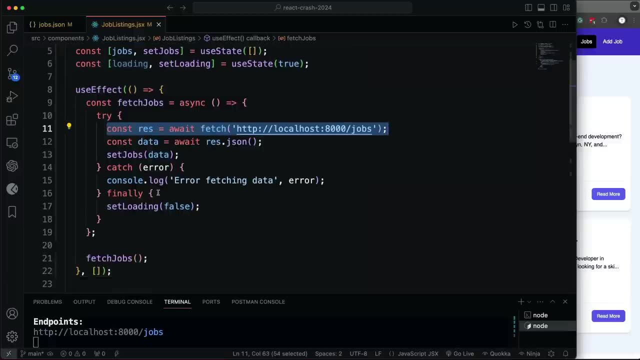 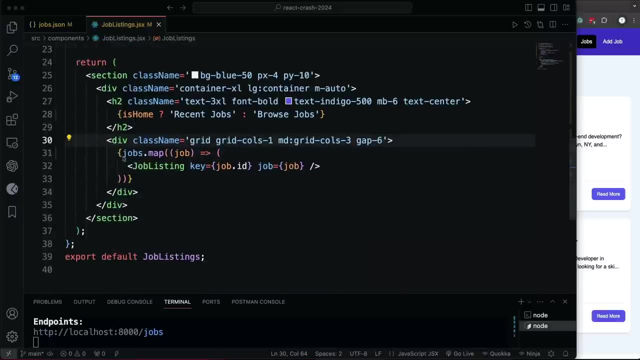 not just bringing in the file and using the data, where we're fetching from the, the back end, and putting it into, putting it into the, the job state. Now let's use this loading value And come down here where we're creating the list with the, with the map. I'm going to go right above that And 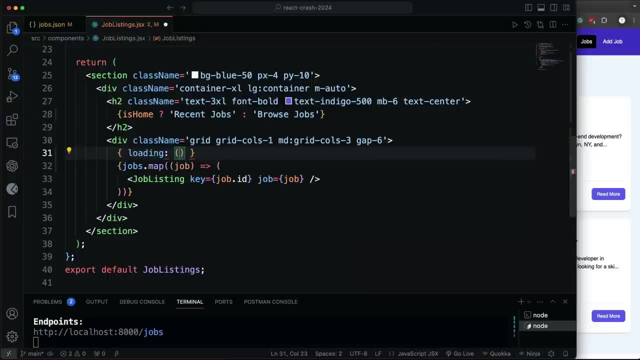 let's say, if loading, then we'll show. for now we'll just do, we'll just put an h2. And we'll say loading. but ultimately I want to show a spinner And then else then let's show, we'll just have a fragment And then I'm. 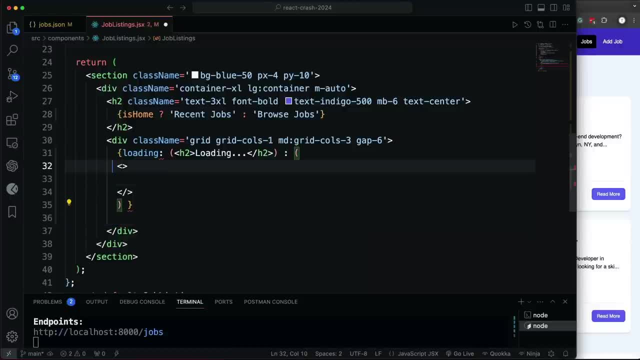 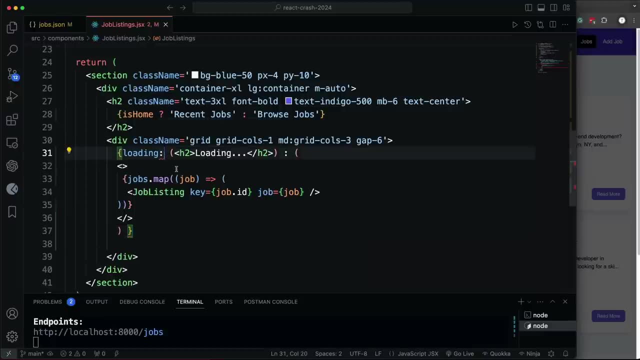 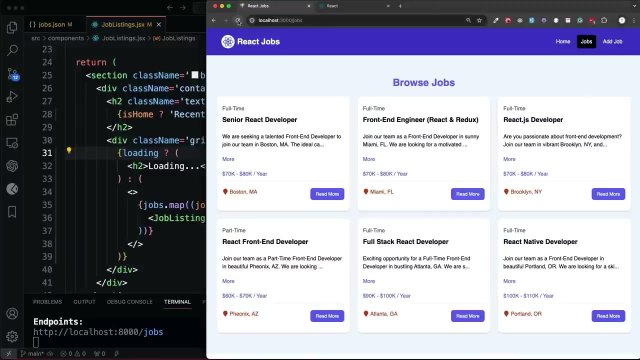 going to put this right here, this job list, into that fragment. What did I do here loading? I'm sorry that should be a question mark. There we go. So now when I reload, you can see it flashes loading on the screen real quick. So 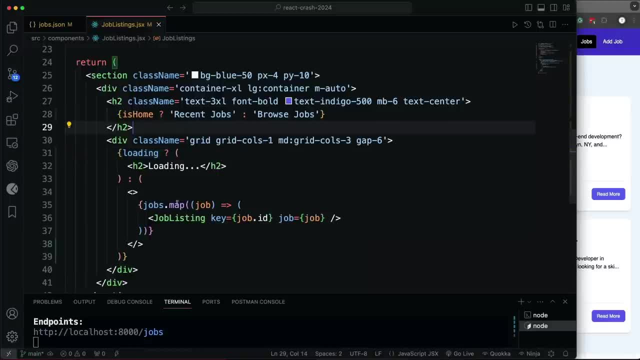 that's. that's when we're actually fetching the data. Now I want to use a spinner. So there's a package we can use, called react spinners, That allows us to to easily show a spinner. you could just throw an image in there, But I'm just going to use 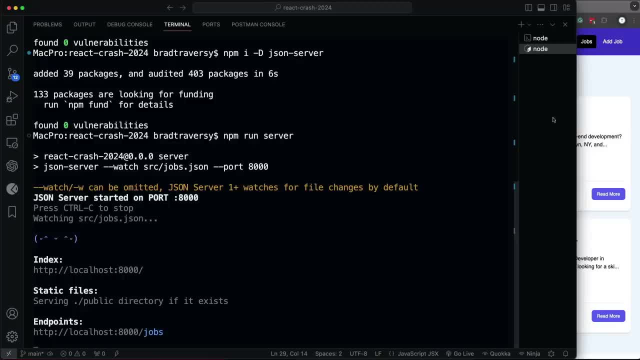 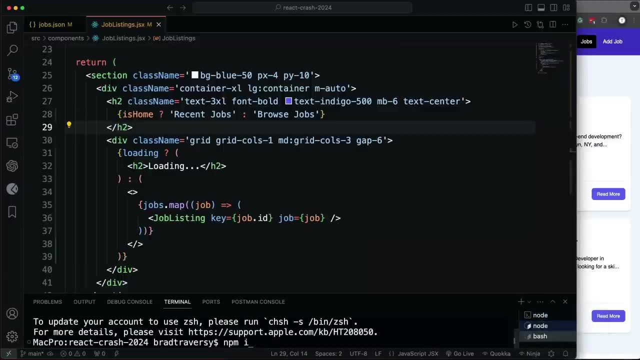 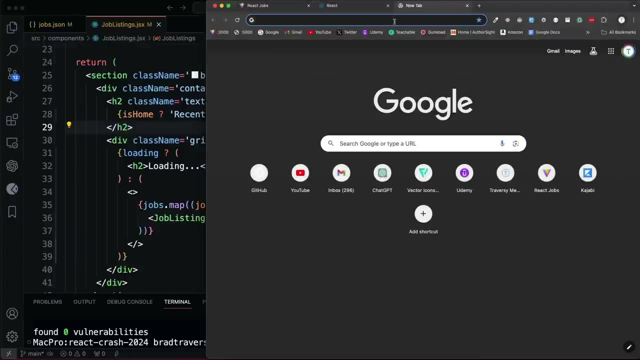 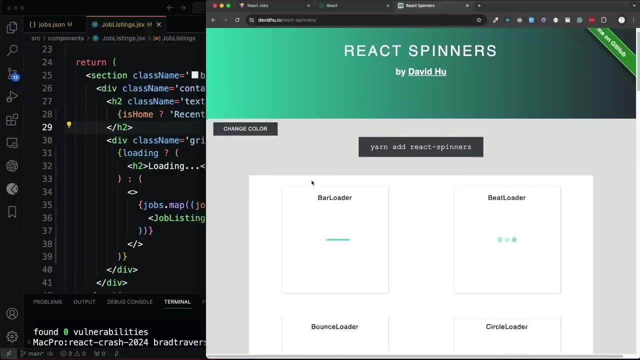 this. So I'm going to open a new terminal because both of these are running, oops, running the back end in the front end. so let's say: npm, install react dash spinners. and let me just show you this real quick. let's see react spinners. yeah, so you can show. like all these things, i want the github page. 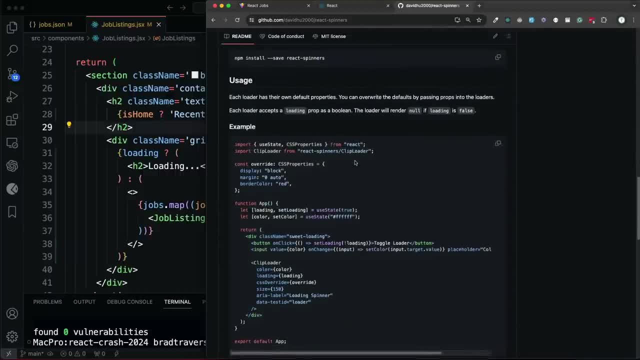 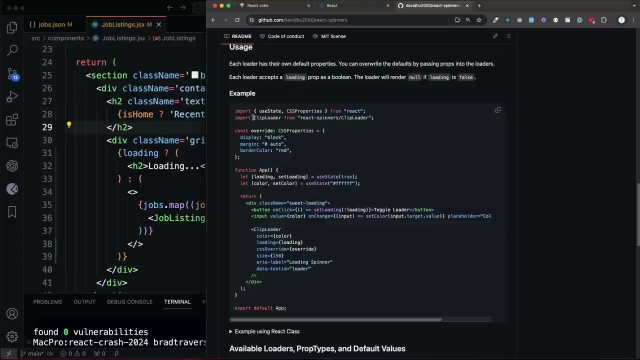 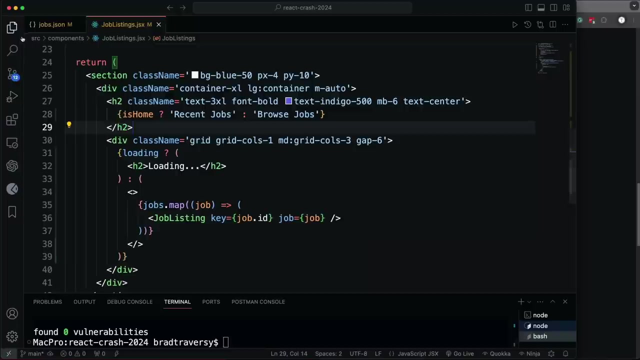 okay, so the way that we use it is like this: we can- uh, let's see, so we can bring. we can use the clip loader- so apparently there's different loaders we're going to use- just use the clip loader and then put it in like this: um yeah, let's uh, let's create a new component. let's call it. 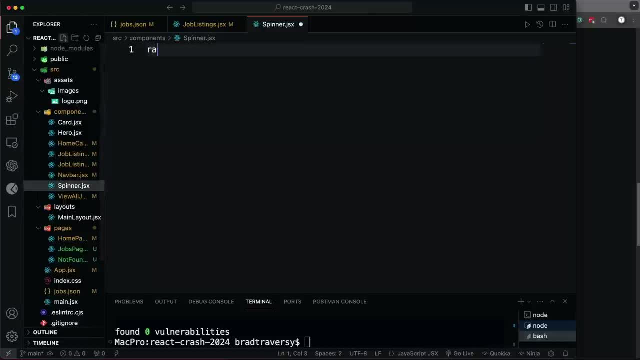 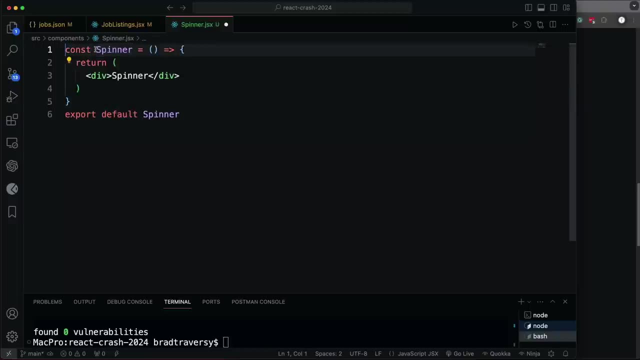 spinnerjs x, r, a, f, c, e. so you can see, literally everything is a component or can be a component. so in this component let's import clip- uh, what is it? clip loader and that's going to be from react spinners, clip loader. so we want to bring that in and then spinner is going to take in the loading state as 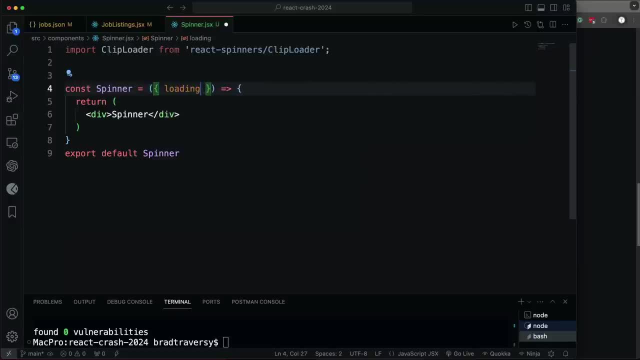 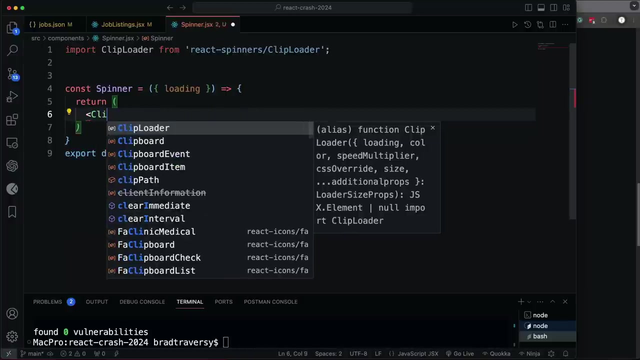 a prop. so let's destructure and add in loading, and then we're going to return the clip loader component. so here let's say clip loader, and this is going to be a self-closing. well, yeah, this is going to be a self-closing component. so let's say clip loader, like that, and then it's going to take in. 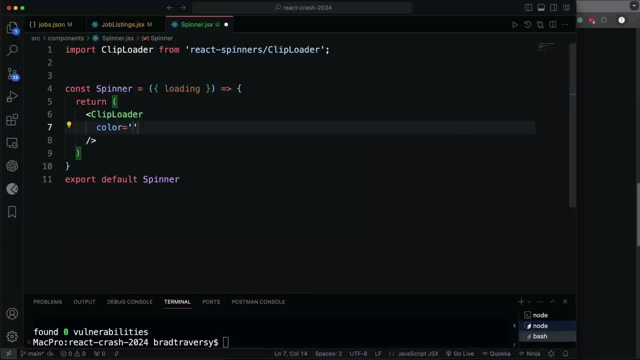 some arguments here, some props. so for the color, let's do hexadecimal four, three, three, eight, c, a and let's do loading, which is going to be set to the loading prop that's passed in. and then we're going to add a css override, because we want to just add a couple custom styles to. 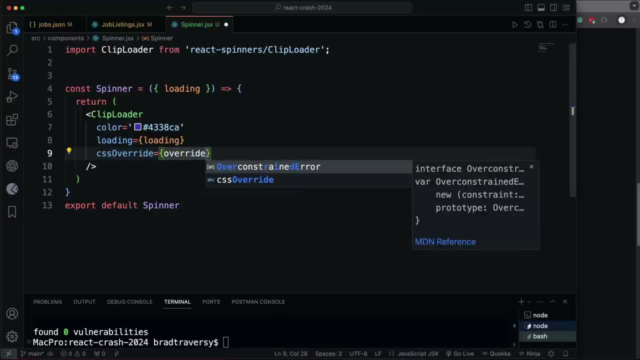 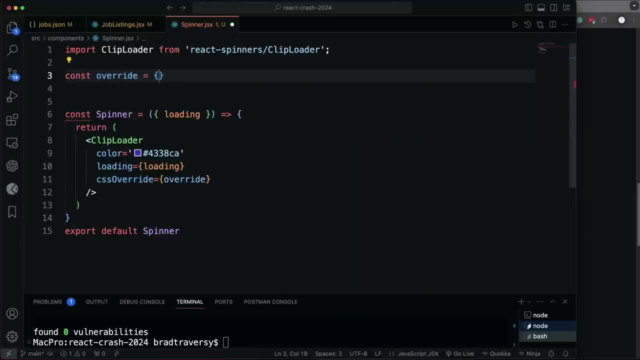 center it. so let's set that to a variable called override, and what we'll do is come up here and create const override. just like i showed you before, we can put styles in a variable. so all i want to do is add a display of block. uh, put a comma here and then a margin. let's say we'll do 100 pixels top and bottom and auto left. 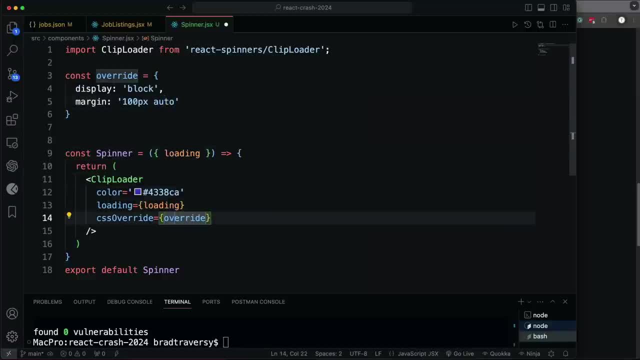 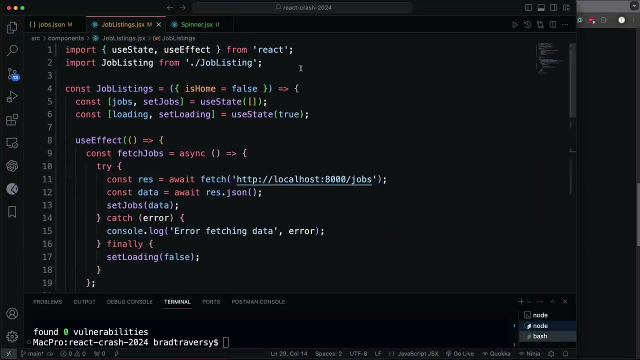 and right, so that'll put it in the middle, and then we're adding that to the css override prop. for the size, we'll set that to 150 and yeah, that should be good. so let's save that now in our job listings. we're going to bring that component in. 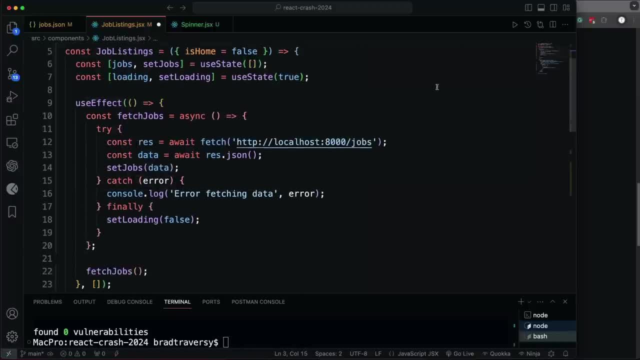 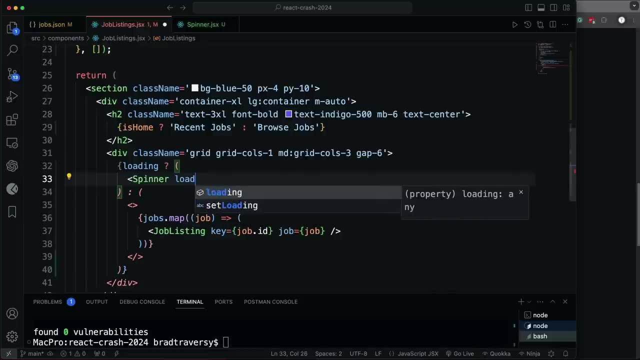 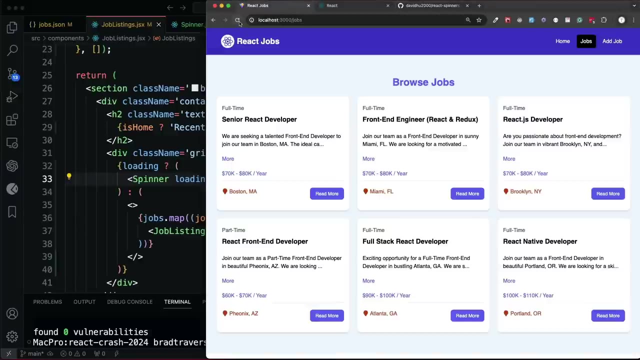 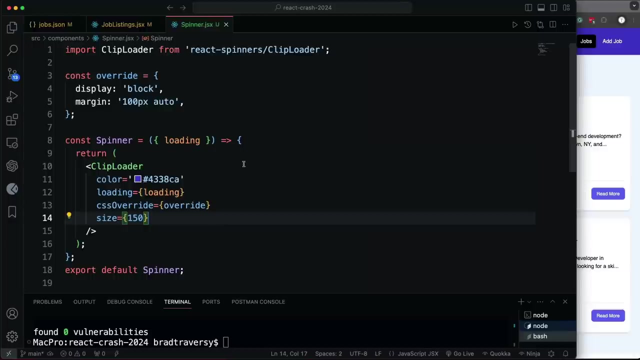 so import our spinner and we can come down here where we have this loading and just replace that with the spinner component and then pass in our loading state. so let's take a look at that. if i reload, okay, you can see the spinner real quick. it's not in the middle, though i'm not sure why. 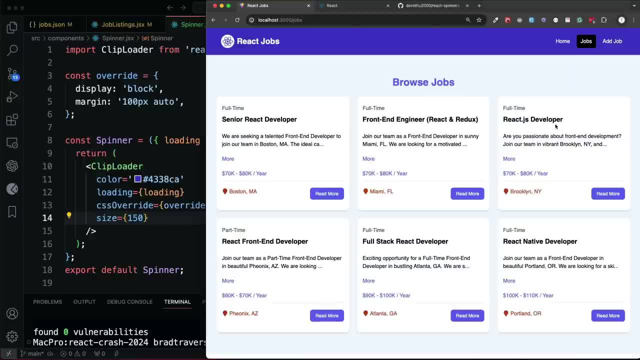 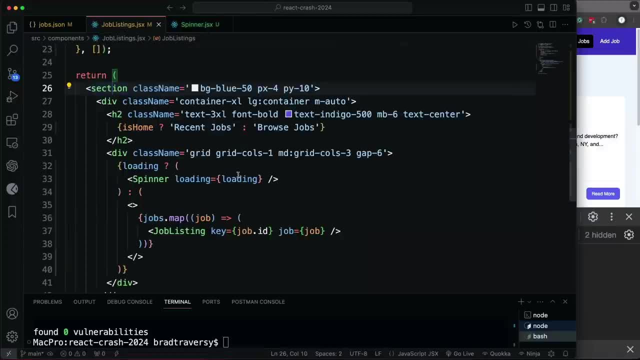 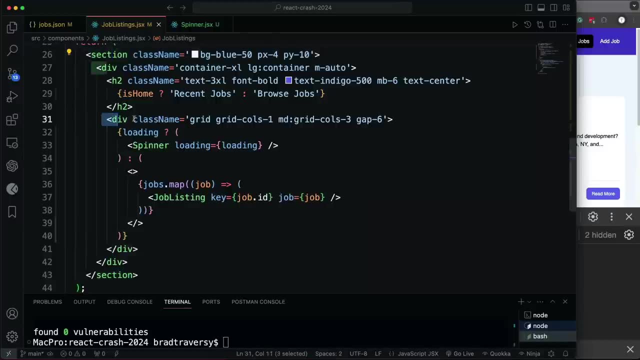 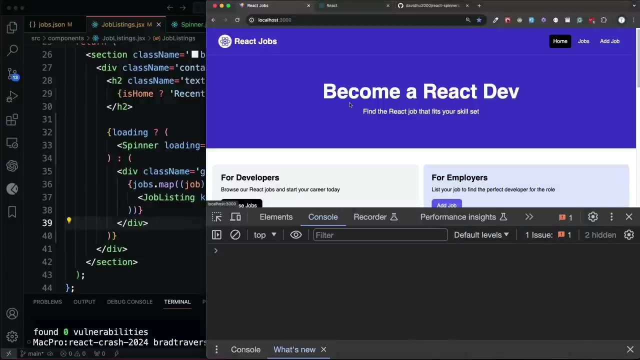 because we have, we have our override. uh, i should. yeah, it should be in the middle. oh, we have it in the grid, that's why. okay, so we should probably put this div inside. yeah, let's do that, we'll put that here, and then this ending div put that here. so now, there we go. so now it's in the middle and it should do. 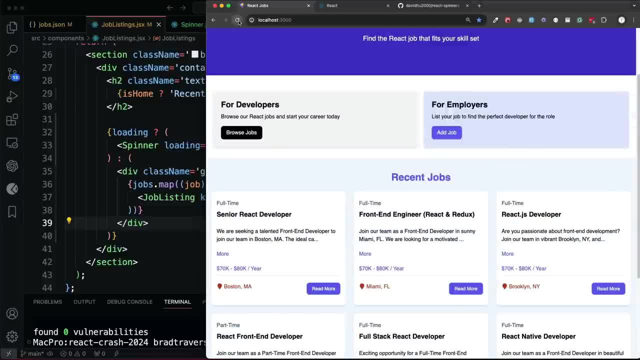 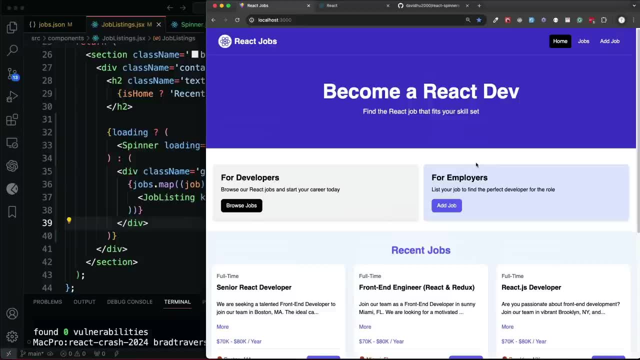 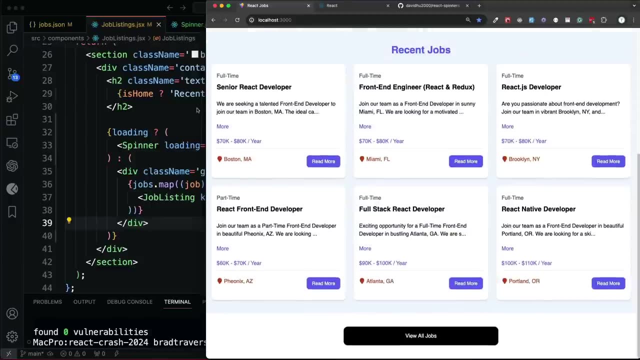 the same thing on the home page because, remember, it's the same component. yep, all right, and now you can use that spinner wherever you fetch data and you want to show it. so let's take care of the the home page. having, uh, having all six? we don't want to do that, we only want to show three. so what we? 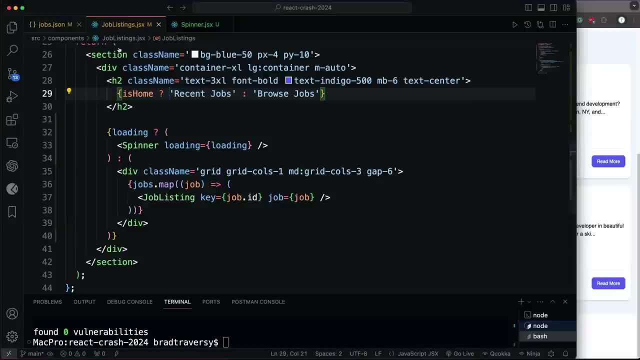 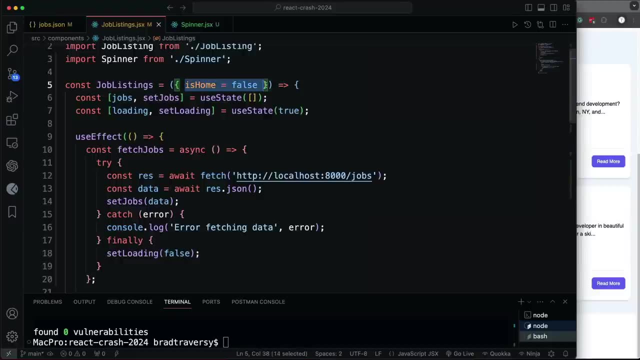 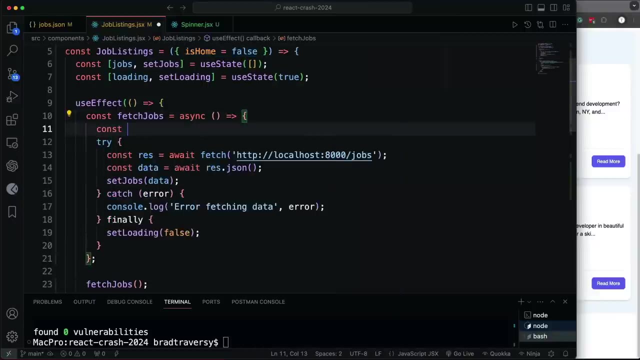 could do is. there's so many different ways we could handle this. but what i'm going to do is come up to the fetch jobs. so we have is home being passed in, so let's utilize that. so in the fetch jobs let's do const ape. and let me just show you that you can add on to this with json server this. 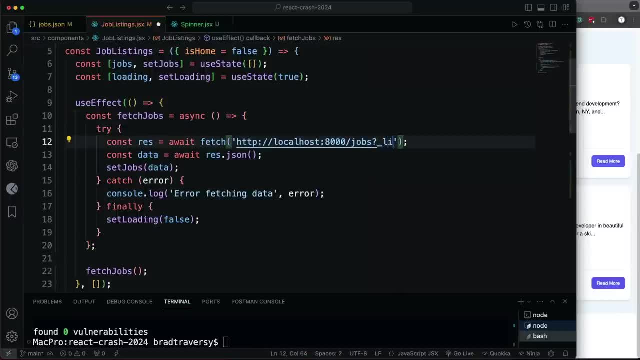 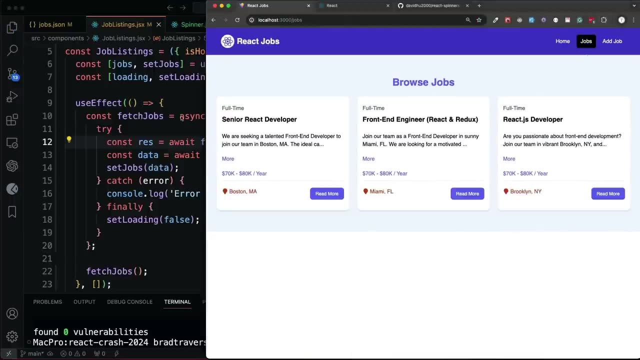 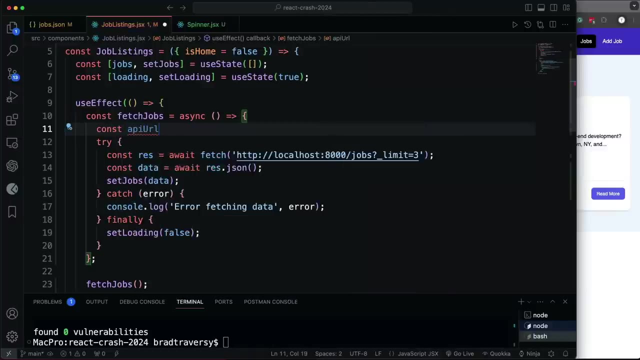 is another cool feature you can do question mark. underscore. limit equals three and if i save that now, it's only showing three. however, the jobs page is also showing three. so what we're going to do is, first of all, let's say api url and we're gonna set that and say if is home, right. so if is home is passed in. 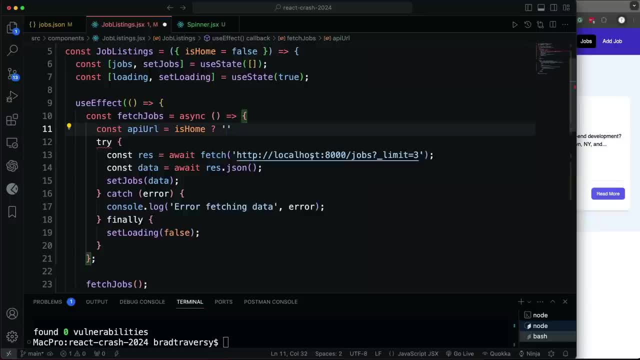 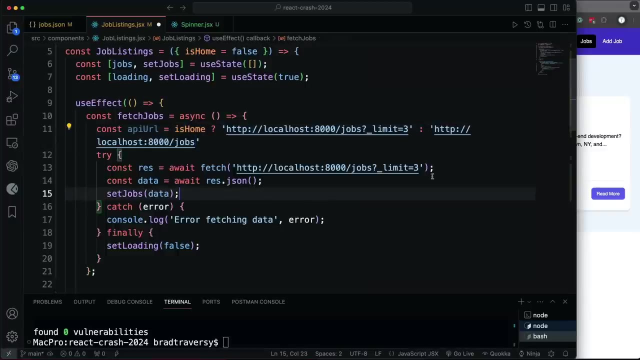 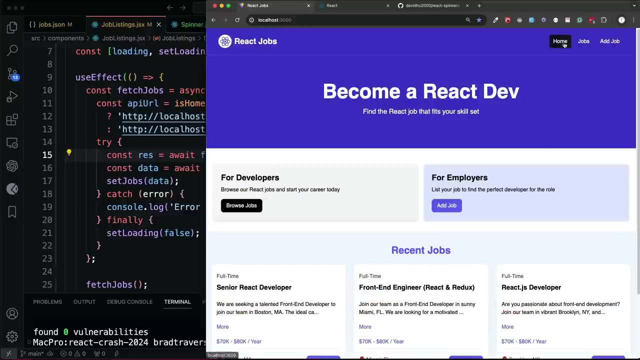 if that's true, then we want the ap. you want the url to be this because we want three. else then we want it to be this, without the limit, okay, and then we can simply replace this fetch with the api url. so now we have six on the jobs page and we have three on the home page. 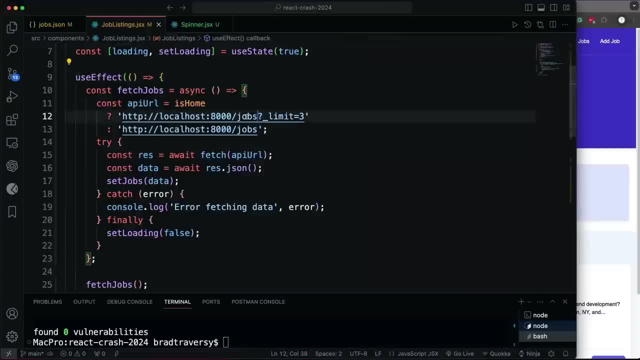 cool. so now i'm going to show you how to add a proxy so that you don't have to add this, because if we, if we deploy this project, it's no longer going to be at localhost 8000, so we need to create a proxy now. if you've ever used create react app, then 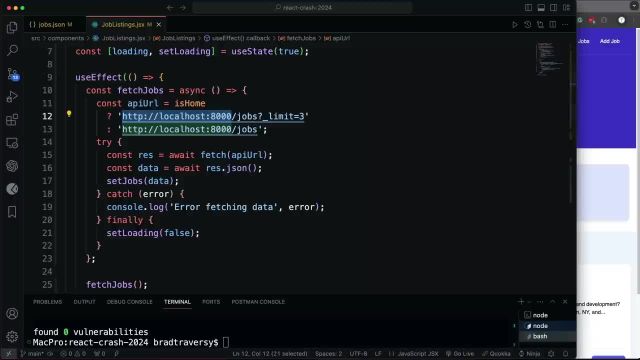 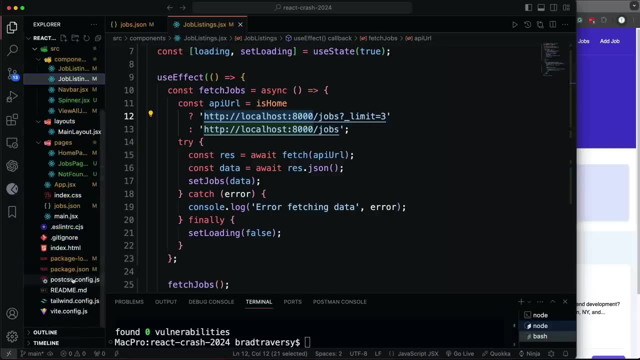 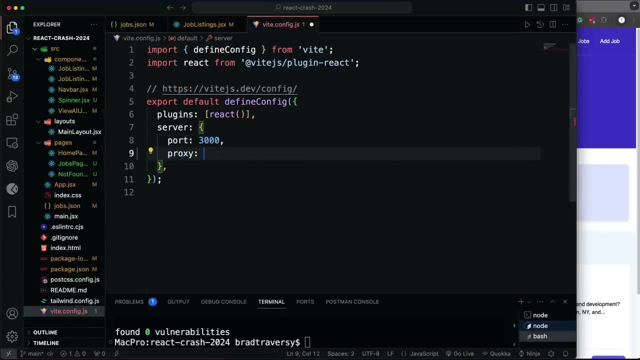 you know that you do that within your packagejson. with veet it's a little different. we do that within the config file. so let's go to veet, veet, config and in the server object, under the port, we're going to add a proxy and basically we're going to say if it's, if it is prefixed with slash api. 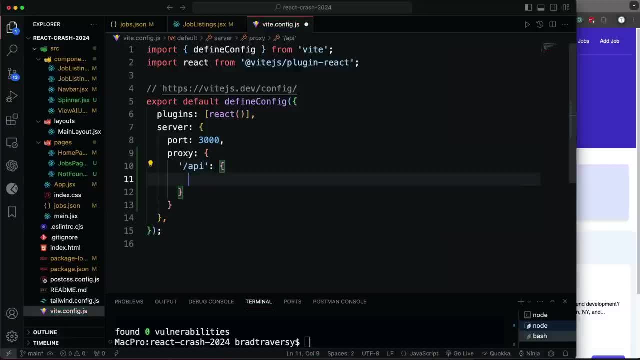 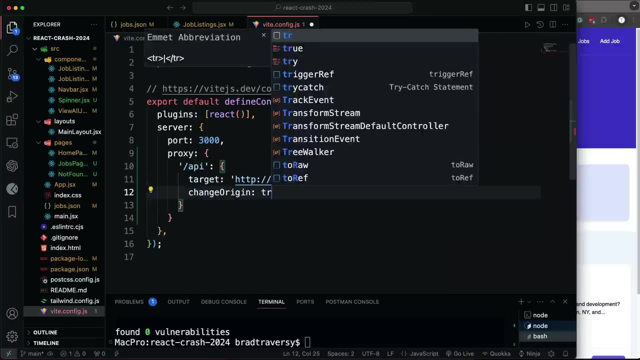 then we want to use this. so we're going to set that to an object with a target, and that target is going to be http, localhost, port 8000 or whatever port you use for json server. we're going to add, change origin and set that to true, and then we're going to do a rewrite and set that to. that takes in a function. 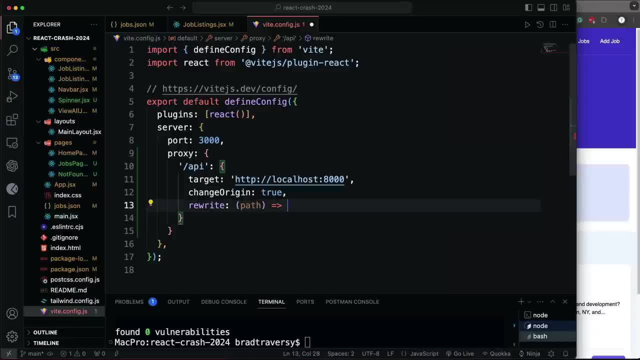 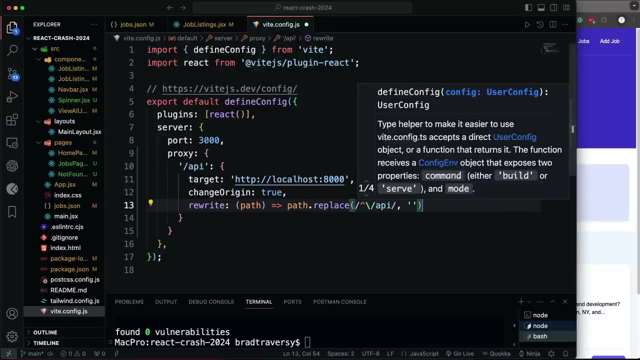 with a path and we're going to then just use, replace and pass in an expression for slash api. so it's going to be double forward slash and then a caret backslash, backslash, forward slash api, like that, and replace that with nothing. all right, so that way, if we do, 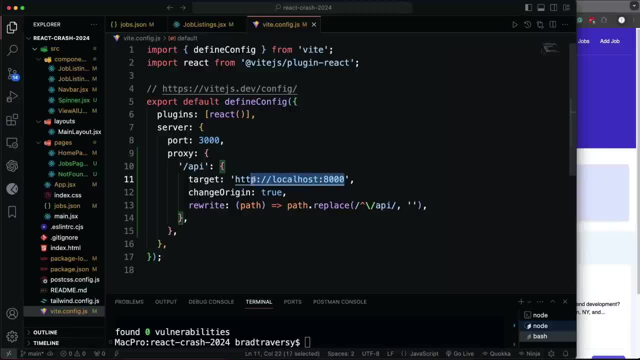 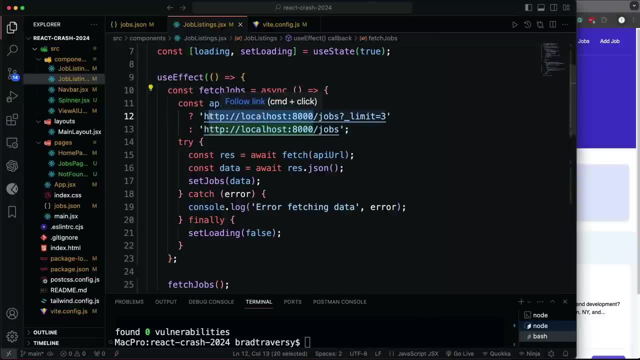 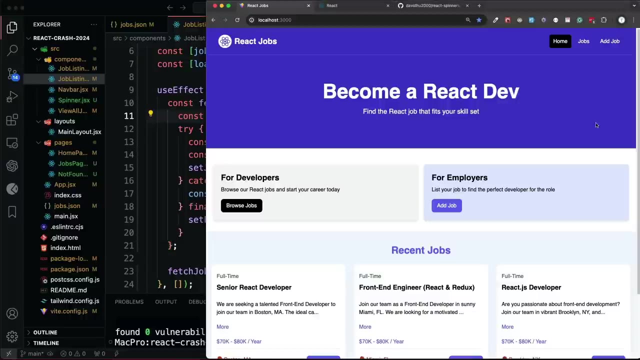 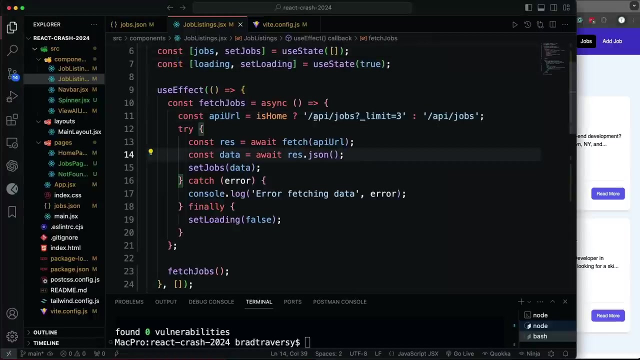 slash api, slash jobs. it's really going to hit localhost slash jobs, so let's try that out. we'll come over here and then let's change this, this and this to just slash api, like that, and let's reload. hua, i think that should do it like this. i think this is pretty good. so here we go. 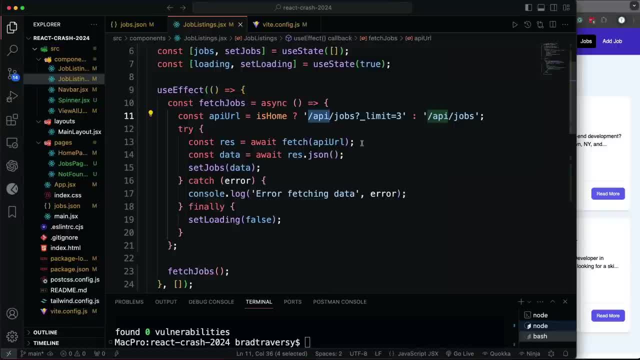 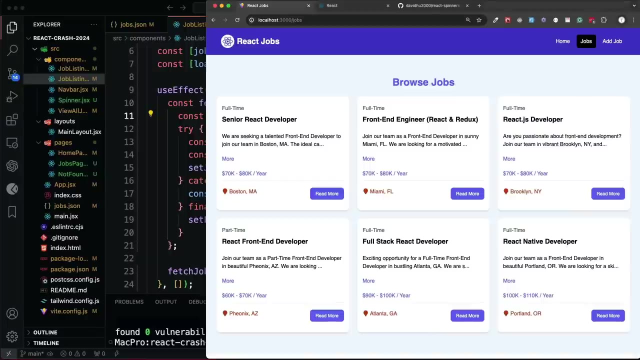 and it's hard to get this app covered. it's all the way up and colour back to cover it. so i'll set it here and that should do it here. so if you, if i'm приложable to this app, um, then coul we if we change this up here. 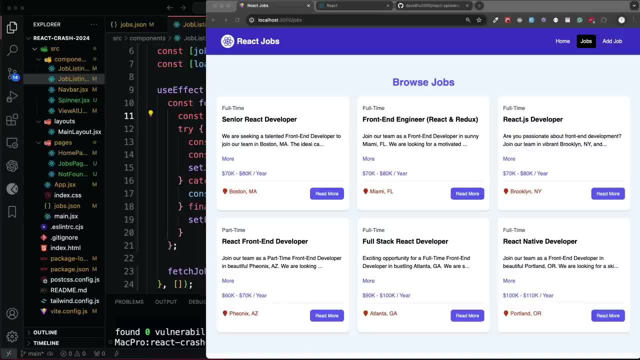 if we change apps up at all depends as you do this fetch data, So you're probably going to run into those. There is something called React Suspense which is included with React and it allows you to do a render while fetching What we're doing here. 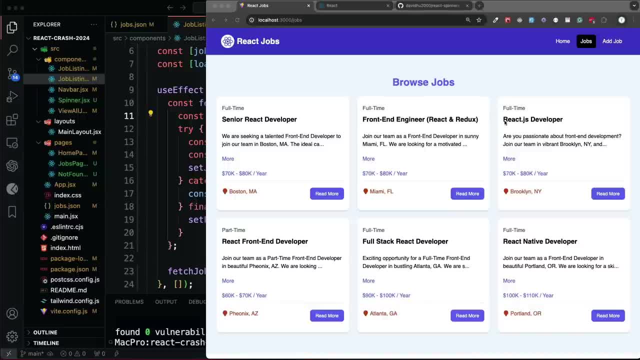 is fetch on render because when it renders it has a side effect of fetching the data. But Suspense will allow you to render while fetching and you basically provide a fallback UI such as a spinner or a loading text. whatever You pass that in as a prop or as an attribute. 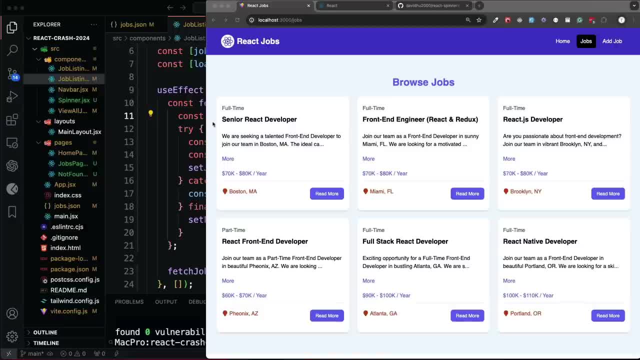 Now, I'm not going to do that in this video. I think it's kind of beyond the scope. I do have an older Suspense tutorial from when it first came out, or you can just check the documentation. What else? There's also something called React Query, which is a third-party library. There's 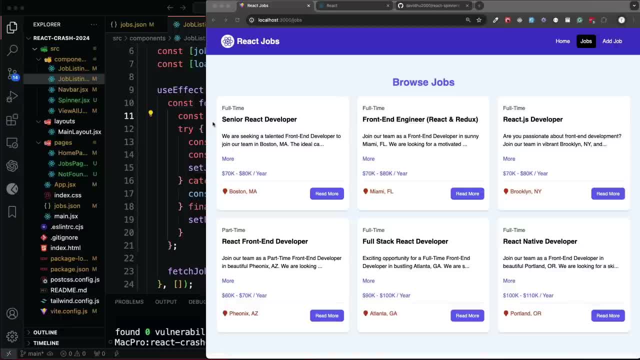 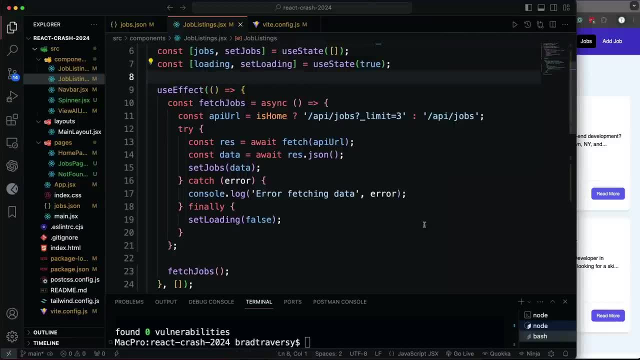 one called SWR as well, and those make data fetching a little easier than this. So that's something you might want to check out as well, But this is like the base way of fetching from a client-side component, And then also with React 19,, you have the new use hook. 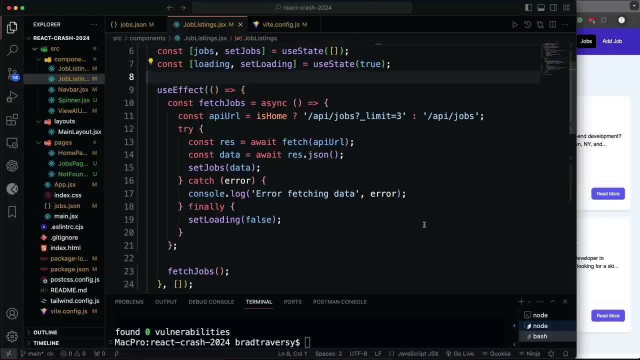 which you can also look into as well. In fact, that React 19 video I did, I gave you some examples with that. So that's the thing with React is there's so many different ways to do the same exact thing And some people will say that's wrong. you know, do it this way. 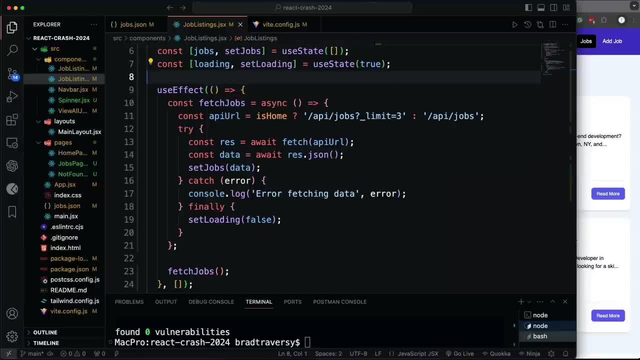 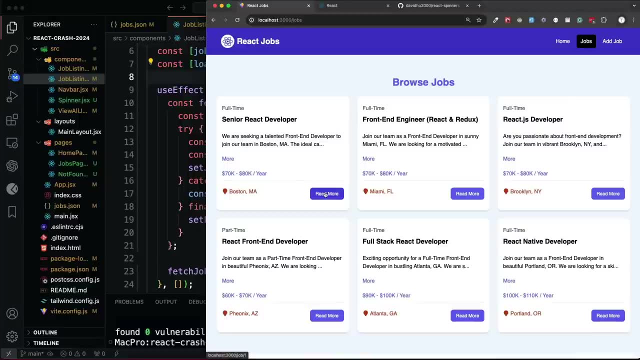 another person will say that that's wrong, So you just need to kind of do what works for you. All right, so now we can start to work on the single page, right This, right here, Job slash, and then the ID And the way that we're going to get this data is going to be a little different. 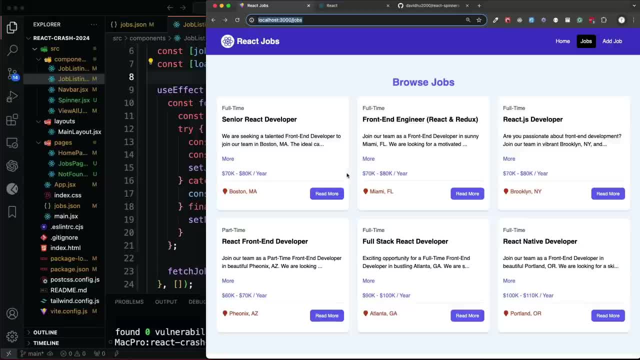 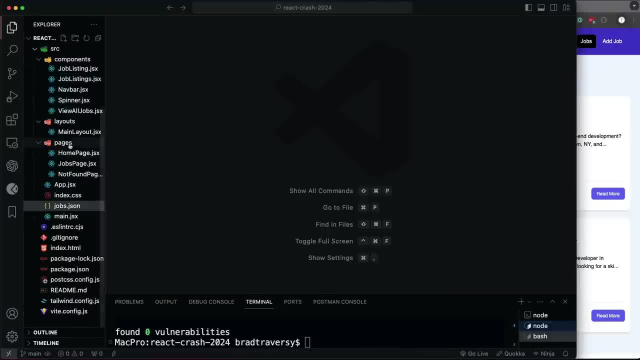 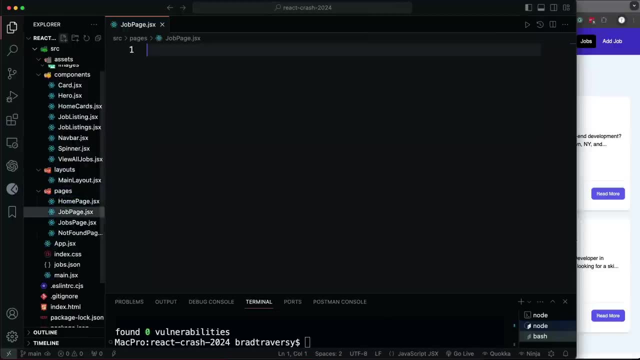 We're going to use a data loader from React Router, which is actually pretty cool, But we first have to create the actual page for the single job. So let's close all that up and then under pages let's create, let's say, job page singular, and then jsx rafce save that and then 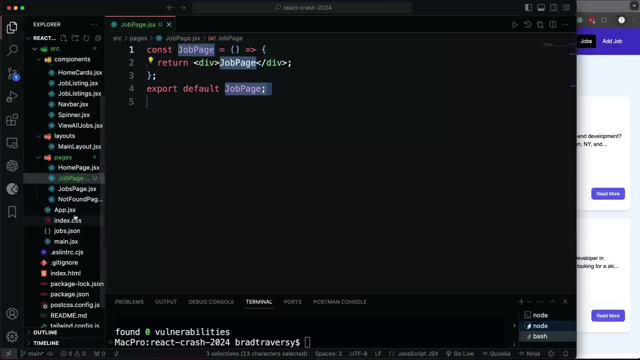 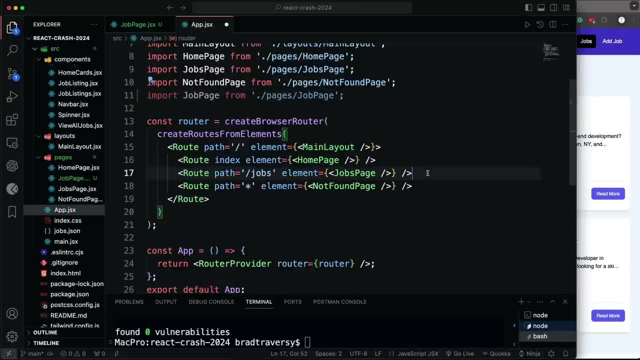 before we add anything here, let's create the route. so we're going to go to our app jsx, we're going to bring in the job page and then we want, we want to add the route so that if we go to job slash and then any id, that it loads this, this page. so i'm going to copy this down and let's do job page. 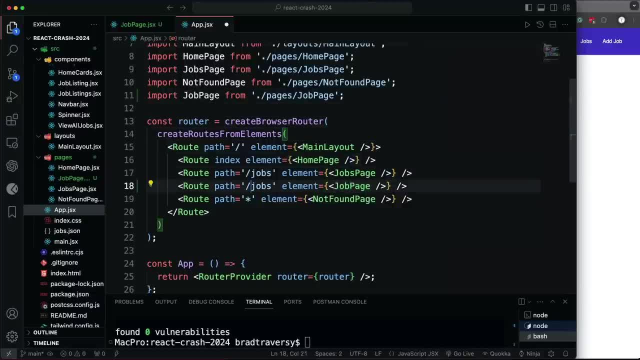 make sure you import it. and then for the, the path we're going to do job. well, actually, you know what? let's do jobs. i like to kind of keep these the same, even though it's a single job. i think i'm going to keep jobs. but you could, you could do what you. 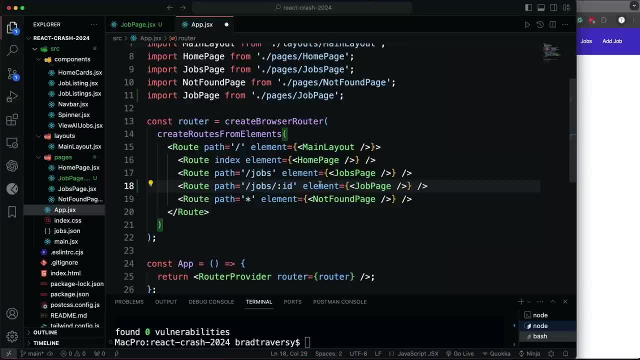 want and then we're going to do colon id. now the colon represents it basically signifies that this is dynamic. so it's not a literal id. the letters id that you're passing in, it's a, it's a symbol or variable. for whatever the id is all right, so let's save that. 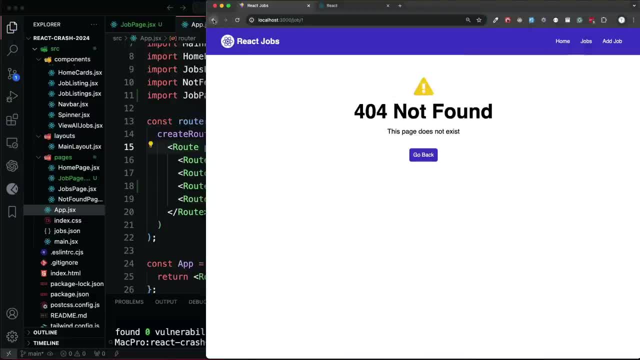 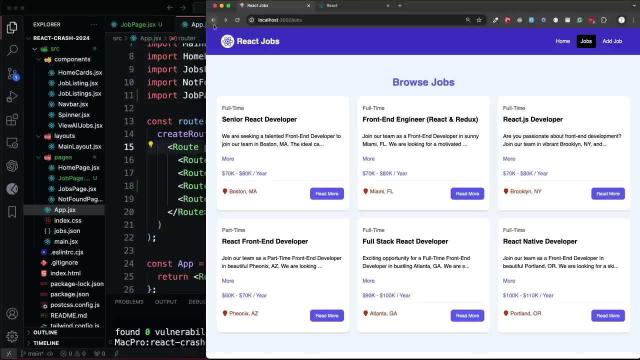 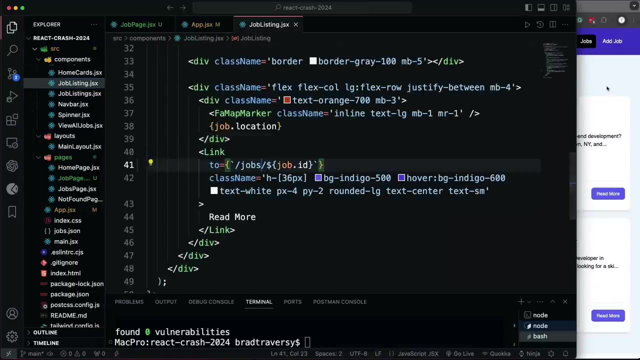 and then if we go back here and reload or let's just, let's see why isn't that working? so slash, oh, because i have job id, so let's change the, the link in the job listing component. so job listing, i'm going to say jobs, slash id. so now click it and there we go. so now we're seeing the job page and it doesn't matter. 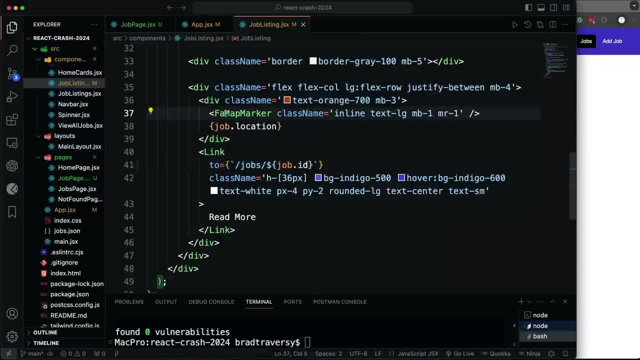 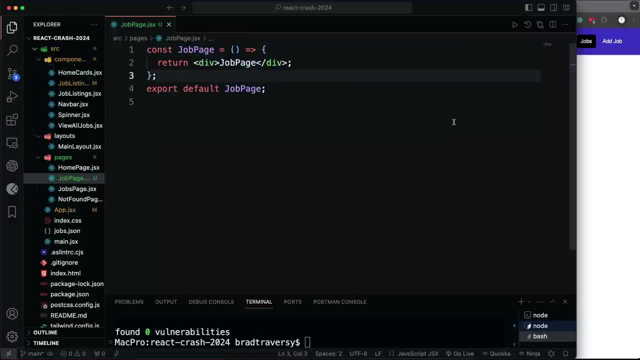 what the id is. here we're still. we're still loading that page. now, let's close up job listing, close up app. and again, there's so many ways to fetch data and we could do the same exact thing we did in the job listings component, but we're still loading that page. so let's close up job. 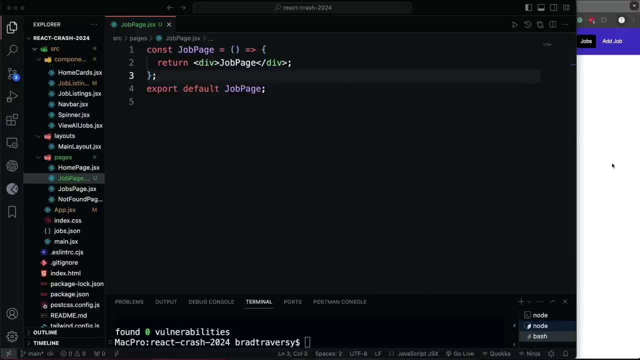 listing component, we can use a use effect so that, when this page loads, uh, we get the job. now what i want to do is use a data loader from react router. so this is going to work a little bit different than um, than we did with the job listings. now, a data loader we basically create. 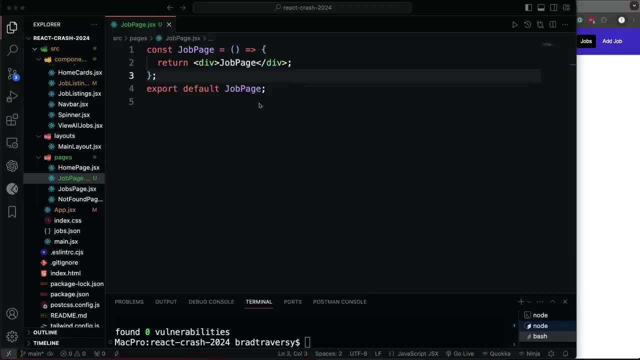 a function in this file and then we can export it from this file and then use that function in in other ways. so let's close up job listing component and then we're going to close up job listing component. we're going to do the same thing with the job listing function, but if i stay, 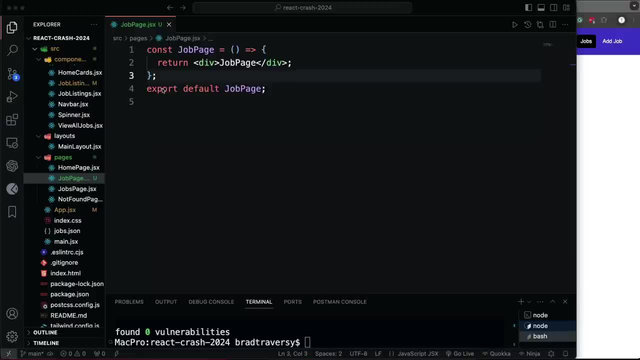 in the configuration document that shows up. i set it up and then, if i skip it, it will be a one time task. so in this case now i'm going to insert in a function called extrapolation, so every time i paste it onto my job listing unit property. if you did that before, we're going to 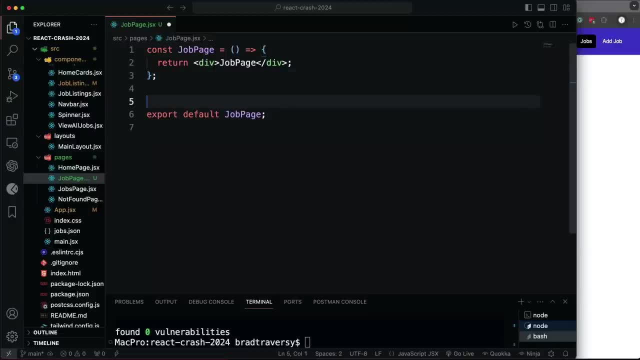 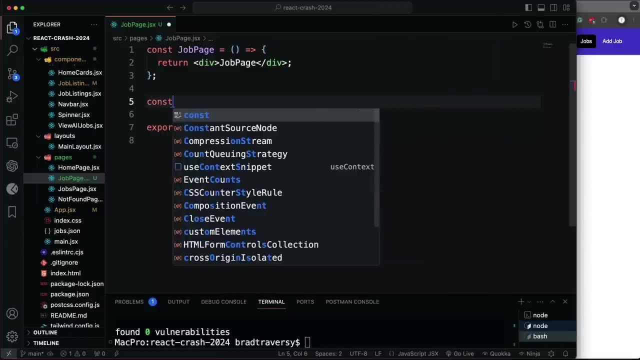 be showed that beginning page, inevitably, that it will be put in a post when it β? s or when it comes out. we're going to put an arrow up there and just put the arrow up there, and we're going to try to specify, kind of: allow it to be made whisky, sip it up, vpn edit, and then we're going. 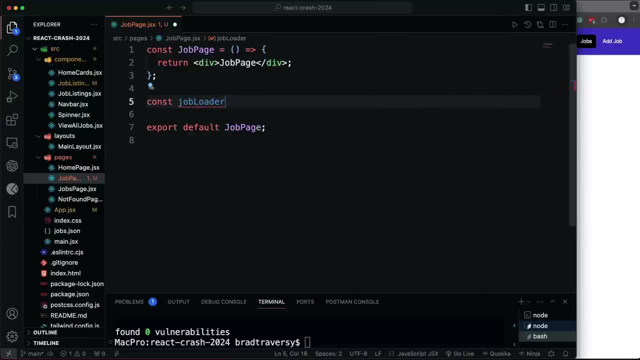 to go in here and we're going to through it and we're going to cut off and do это horse button wear. see that i filled this out. it looks kind of strange, but guys, i can job loader right, and then we're going to set this to async and it's going to take in actually. 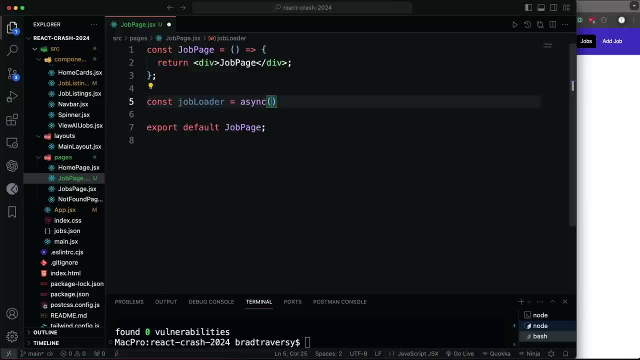 we'll- yeah, we get a pass in params, because that's how we're going to get the ID. You know what? I'm going to show you how to do it with use effect first, because I don't feel, I don't feel confident enough that I, that I showed you enough fetching with use effect. 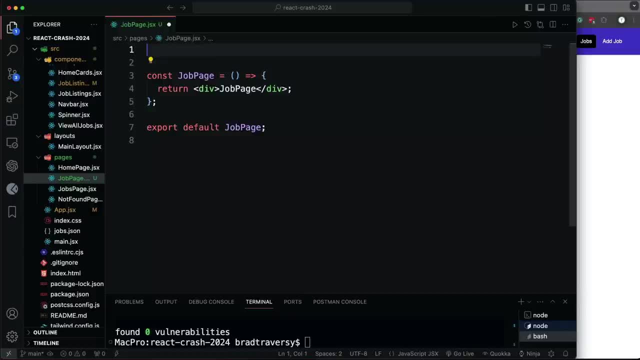 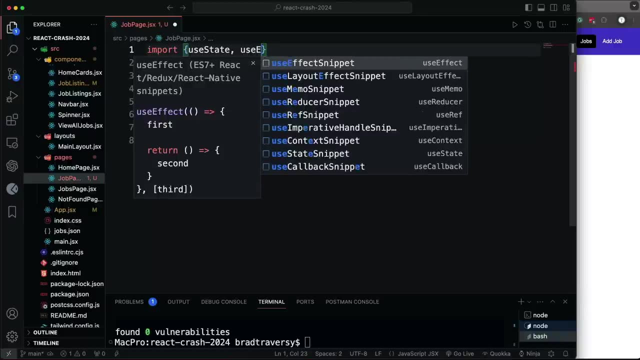 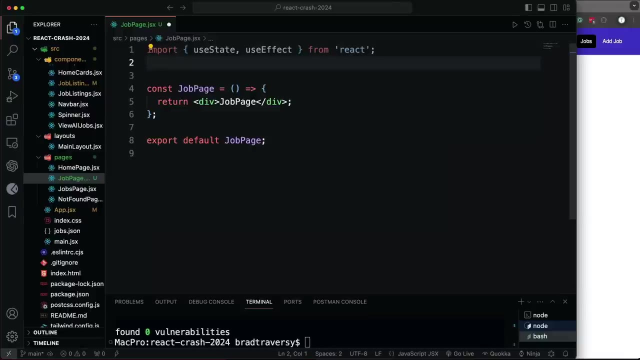 so let's, let's do that first, and then we'll change it up and I'll show you how to use a data loader. so I'm going to import use state and use effect from react and let's see we'll. 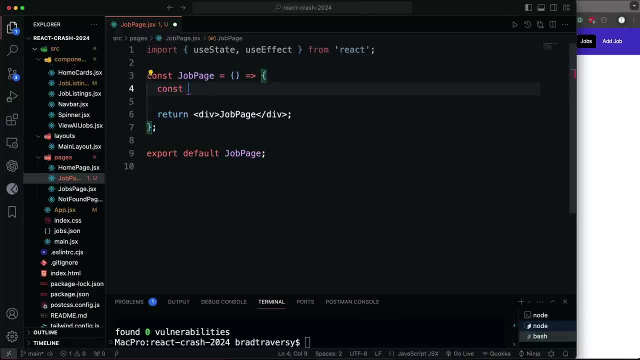 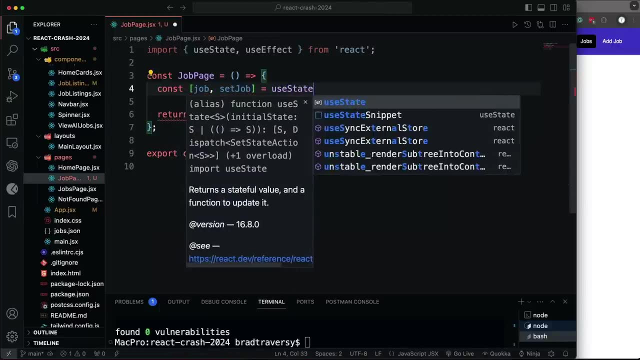 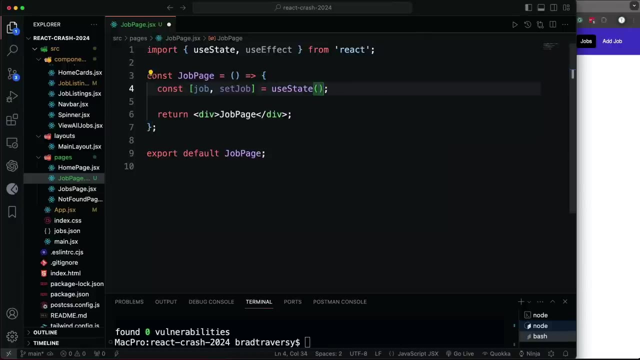 we'll add the job to the state. so let's say const and just job, and then set job all right, and then we'll set that to use state. and then as far as, as far as the default, we'll just do, we'll just, we'll just do null for the 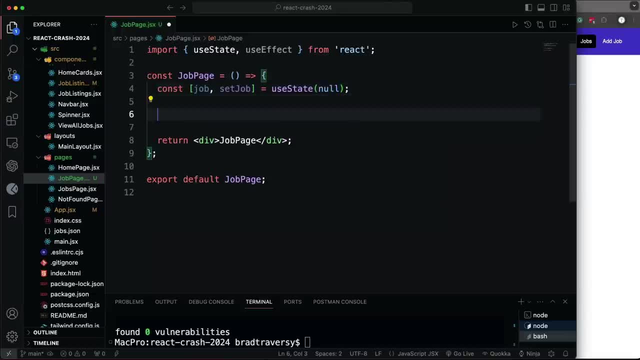 default and then we'll have our use effect and the use effect again takes in a function and dependency array and I'm going to create a function, just like we did in the how we you know when we got all the jobs. we're going to have this. this is going to be called. 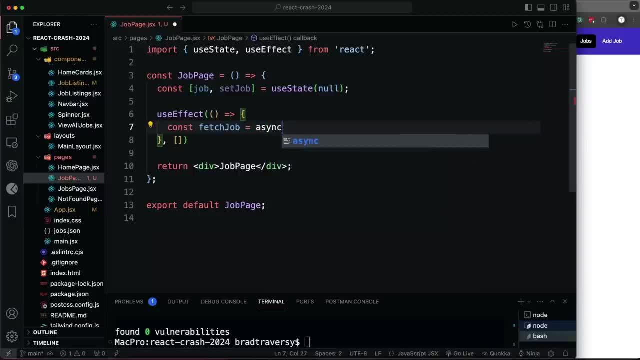 fetch job and this is going to be a sync- and then we want to call it down here. I like to do this first because I always forget to call it, and then in the fetch job, basically we can probably just copy what we did in the job listings, like this stuff here. 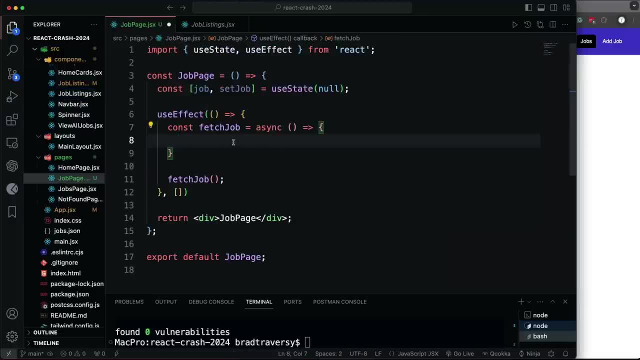 we'll just grab the try catch. I'm probably going to change this up after, but let's do HTTP. oh, we don't need HTTP anymore, we just do slash API, slash job. now we need the ID. so how do we get that? we can get that using the use params hook from react router DOM. 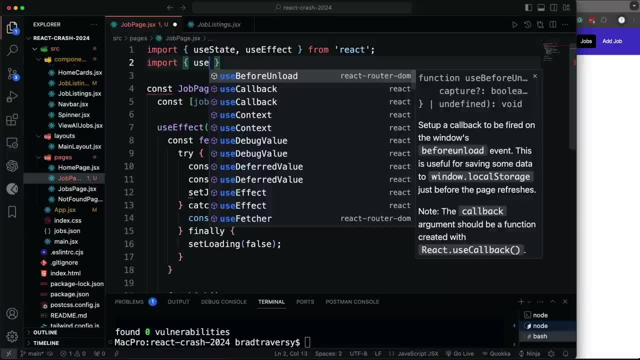 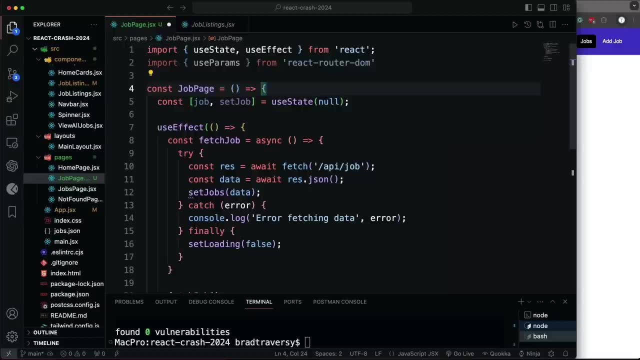 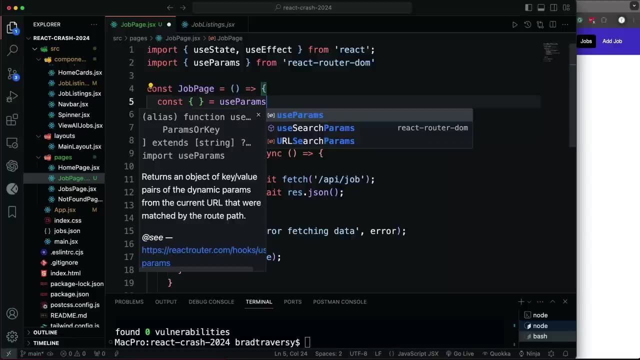 so let's say, import use params and that's going to be from react router DOM, and then the way that we do this is we can come, we can go right here at the top and we're going to destructure from use params and we want to destructure and get the ID. 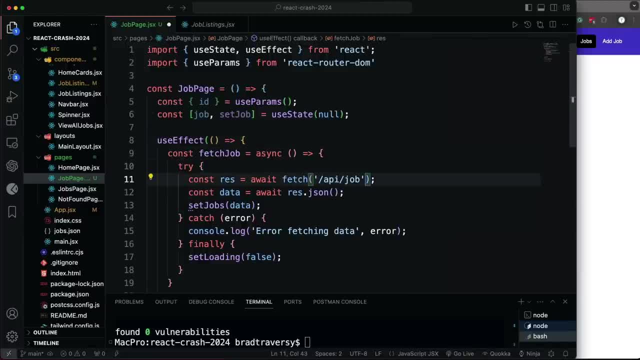 okay, so that should give me the ID. and then in here let's replace these quotes with backticks and we'll say: API slash, job slash, and then the ID. okay, then we get the data. and then, instead of set jobs, we're going to do set job data. and yeah, I think. 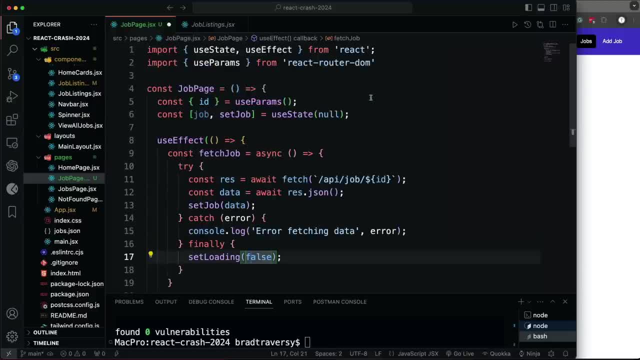 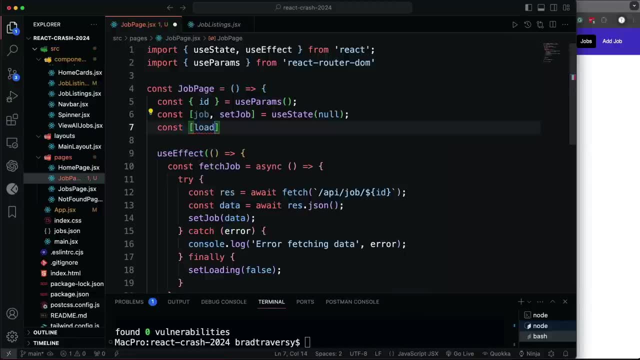 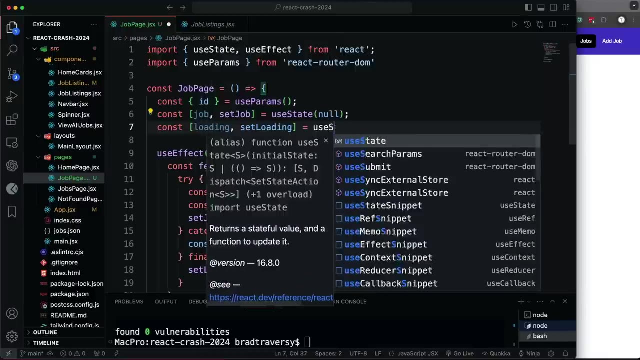 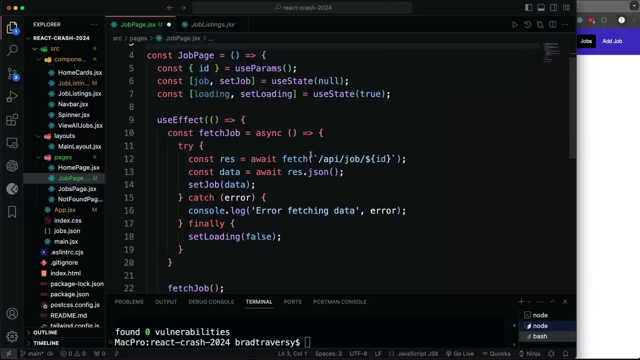 that's fine. yeah, I think that's good. oh, the loading state. we didn't do that, so we want to do loading. set loading. that's going to be true by default. okay, and let's see what else. 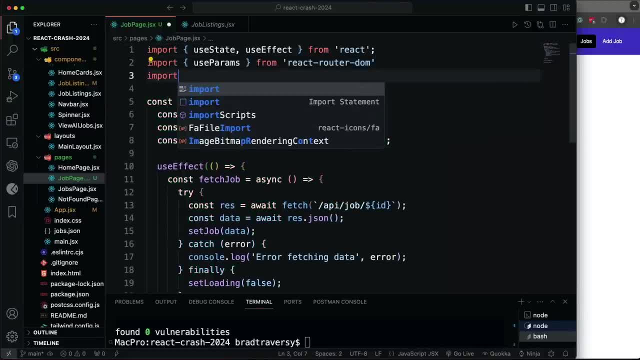 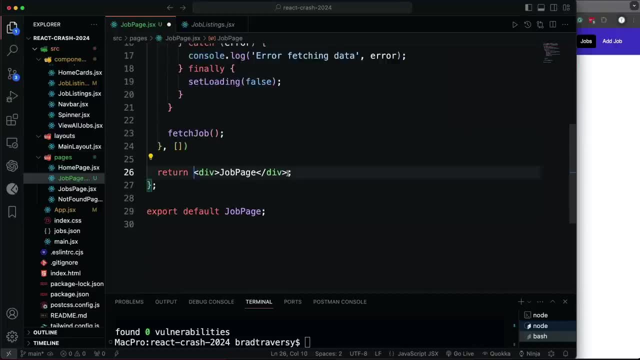 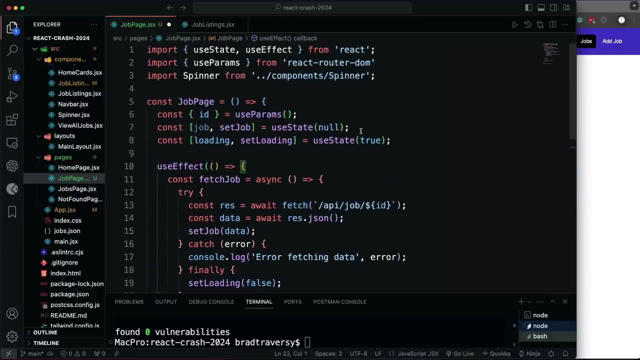 let's bring in the spinner component and then for the return, let's do return. if loading, then show the spinner else, okay, Yeah, else then we'll just put in H1 for now and just say job. And I want to make sure we get the job data. 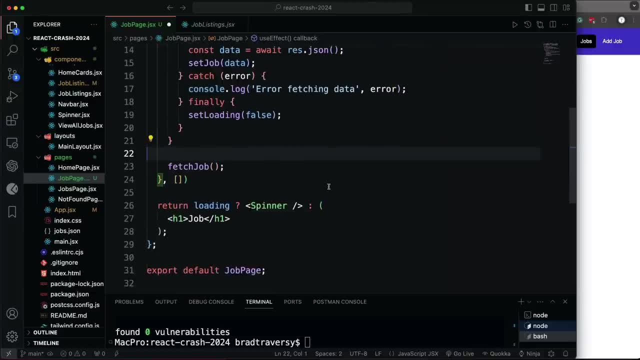 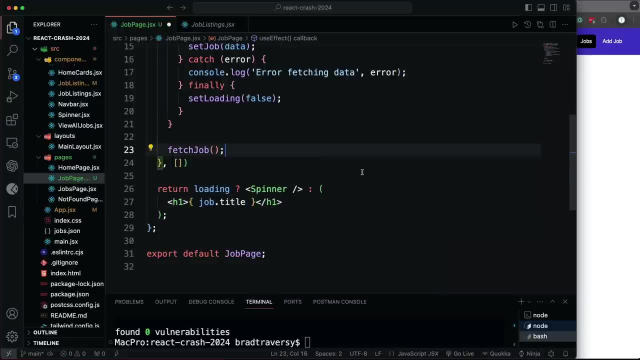 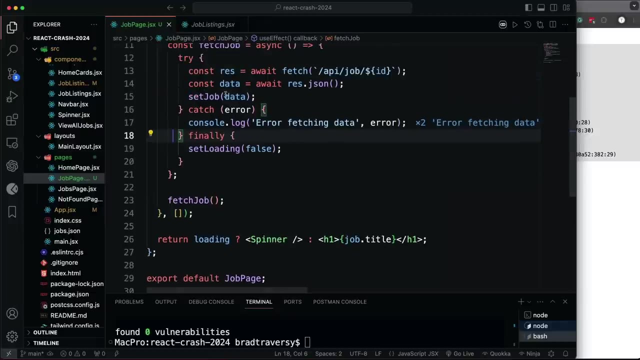 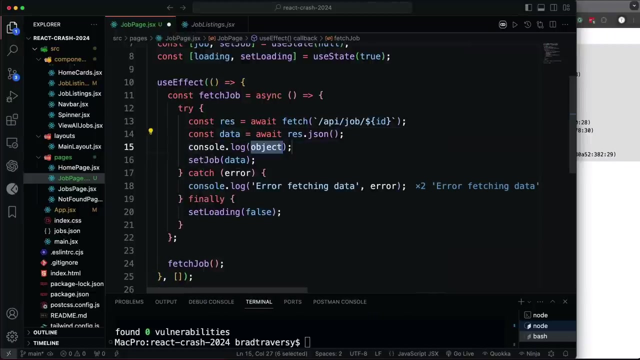 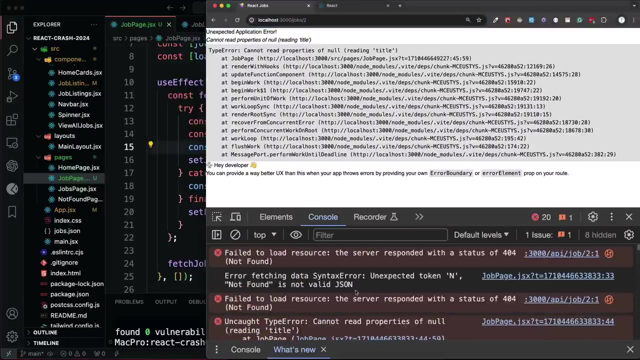 so why don't we put in this H1 jobtitle Cannot read property: no, So we're setting the job to the data. Let's see. Let's do a console log of data. Responded with a status of 404.. 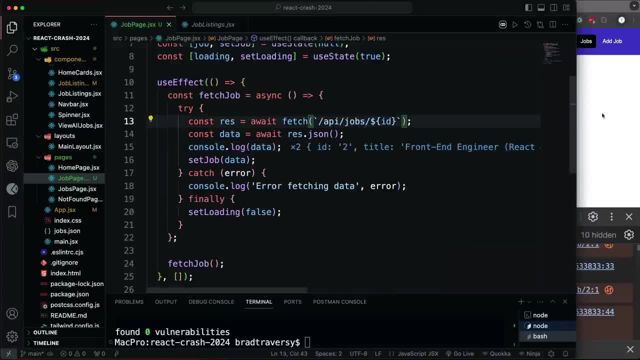 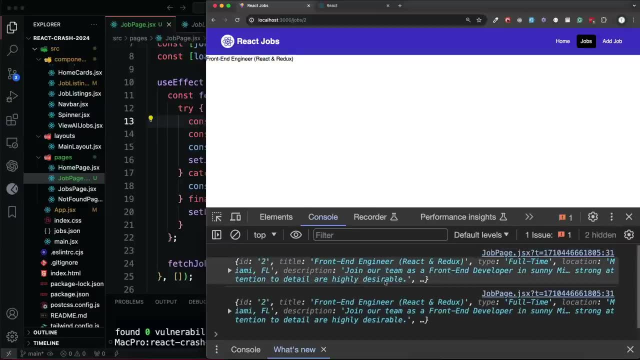 Oh, I think it's jobs. Yeah, There we go. So we're seeing the title and we're seeing it in the, the whole thing in the console. So just to kind of reiterate what's going on here, the component loads. 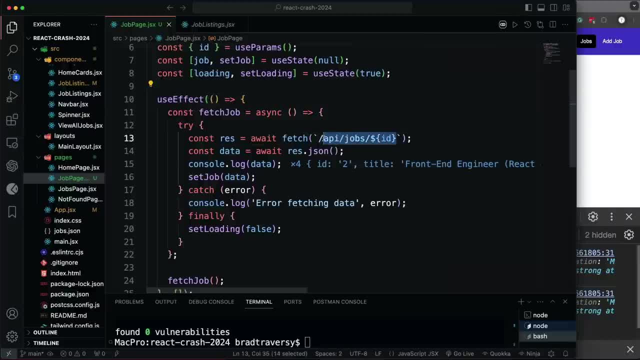 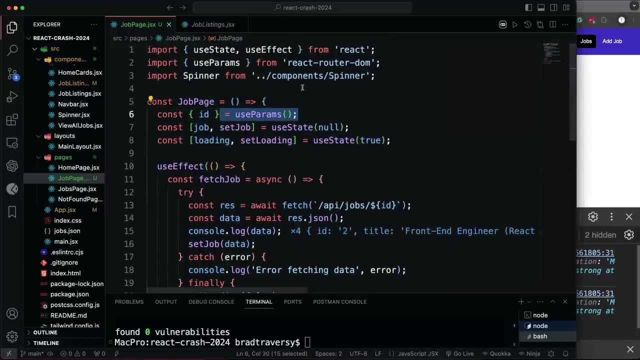 it has a side effect where we fetch the data from this, from API jobs and whatever the ID is in the URL, and we're getting that because of the use params hook from React Router DOM And then, once we get the data, we're setting it to the state. 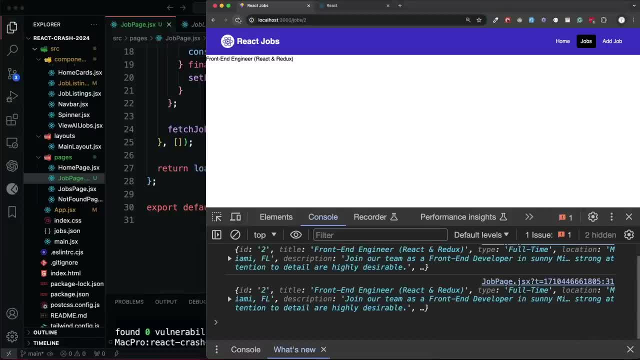 Down here we're saying if it's loading, show the spinner. So if I reload, you can see the spinner real quick. And then, once it's loaded, it shows an H1 with the with the title which is this right here? 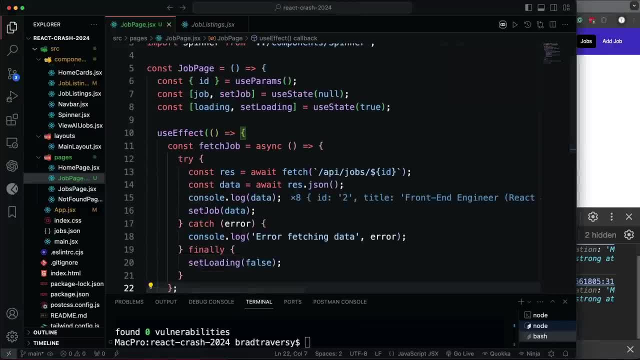 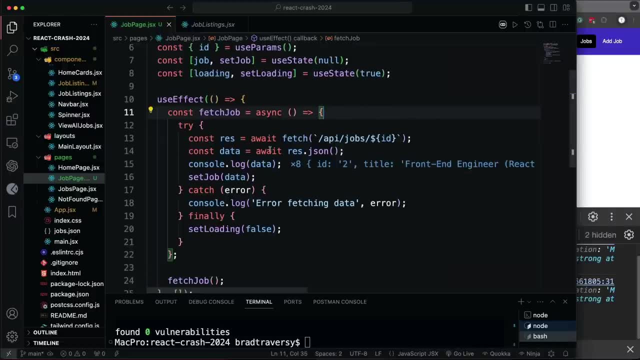 Okay, So that's how we can get the data just using use effect. Now I'm going to show you another way to do this, using React Router's data loaders, And we can do this without having to do the use effect, And we can also export the. 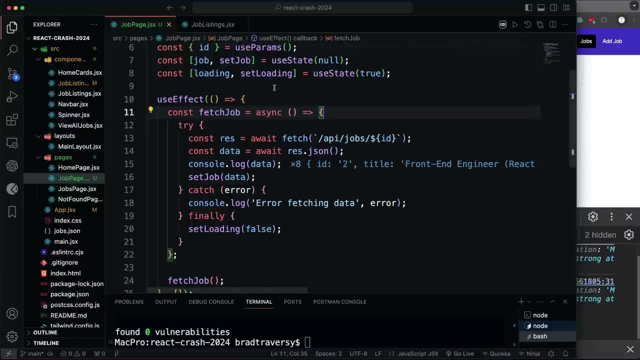 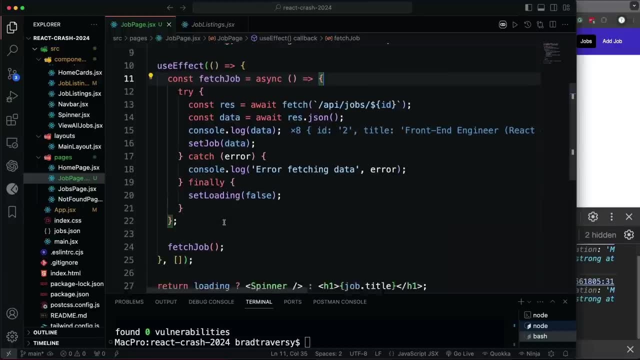 the data as well from this component, so we can use it elsewhere And we will use it elsewhere. We're going to use it in the edit page, because in the edit page we do the same thing- We have to fetch the job. So I'm going to get rid of this. 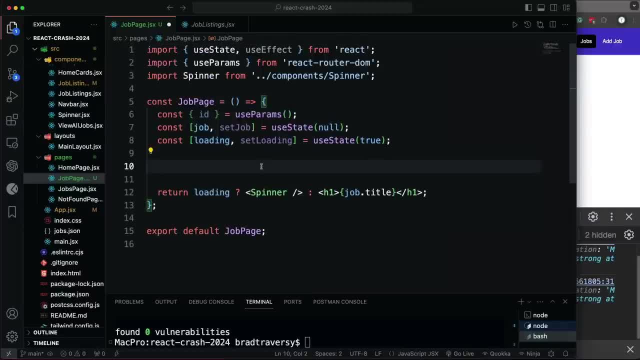 If you want to just kind of comment it out so you still have it, you can do that, but I'm going to get rid of that. I'm also going to get rid of the two states and I'm even going to get rid of the use state and use effect. 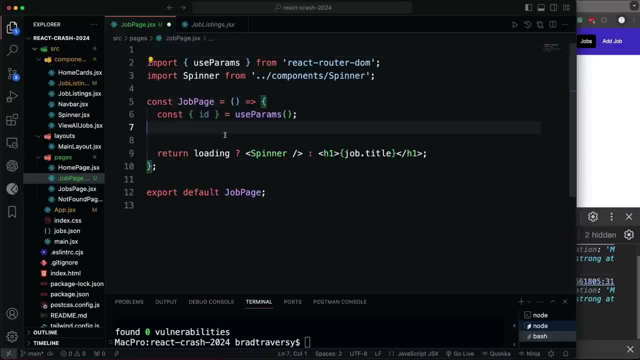 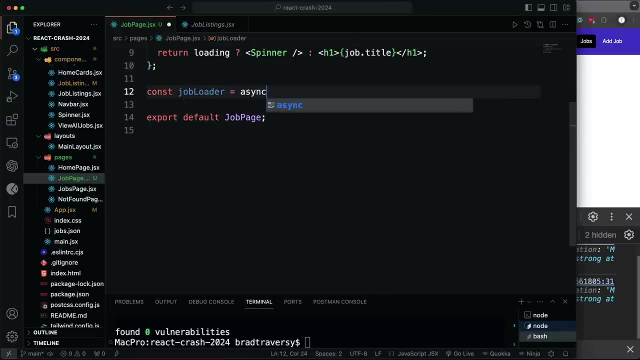 I'm still going to get the params because I do need the ID still And, yeah, we'll keep that as well. But what we can do is go under the function, above the export, and let's say, cons job loader, And remember this is a. 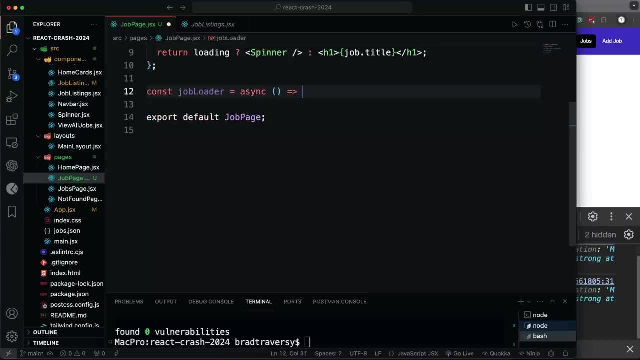 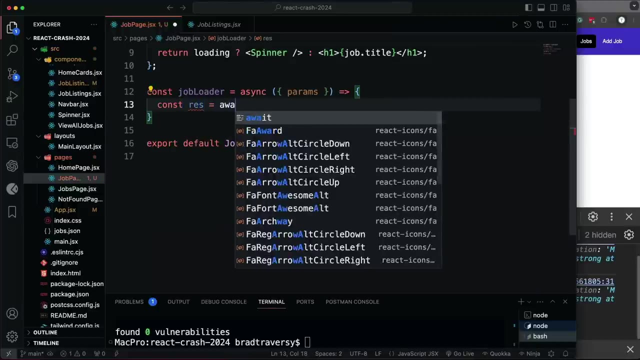 this is a feature of react router, not react itself. So let's set that and we're going to pass in an object with params, Okay, And then in the job loader. this is where we're going to make our request. So let's say res equals a weight. 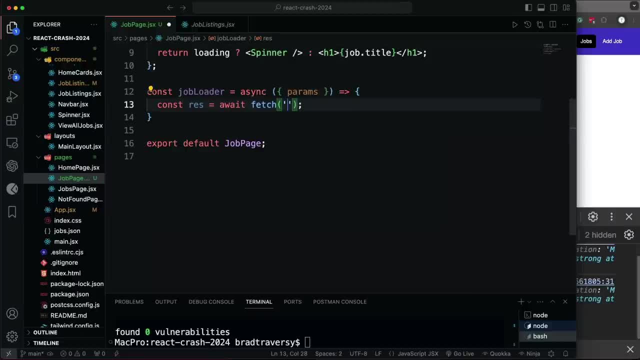 a weight fetch and it's going to be. let's see, let's use back ticks here and then slash, Slash API jobs and the ID we should be able to get from that params dot ID. Then we'll say cons data, set that to a weight and then res dot Jason. 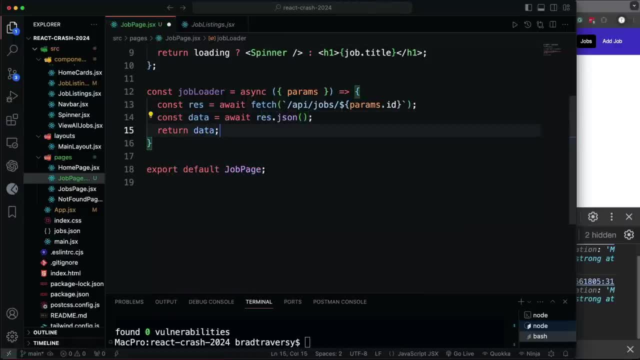 And then we're simply going to return the data from this function. Okay, So a loader is just going to return the data. Now we want to export it. but we also want to still export um job page as defined As default. 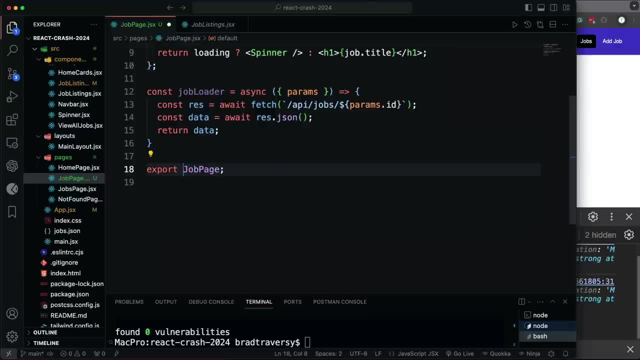 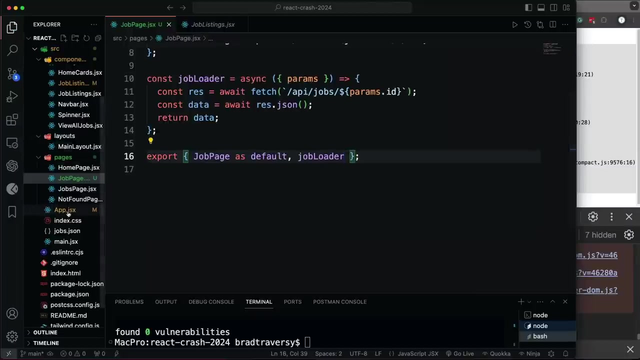 So what we can do is say export. we can do this, wrap this, oops, wrap this in curly braces and say job page as default, and then have a comma and also export the job loader. Now what we can do is go into the app for a app, JSX, where we're embedding the job page and where we imported. 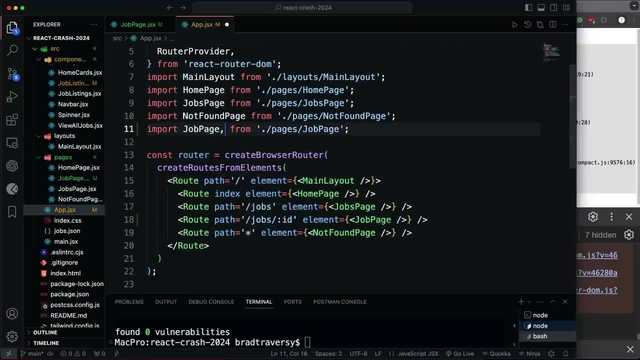 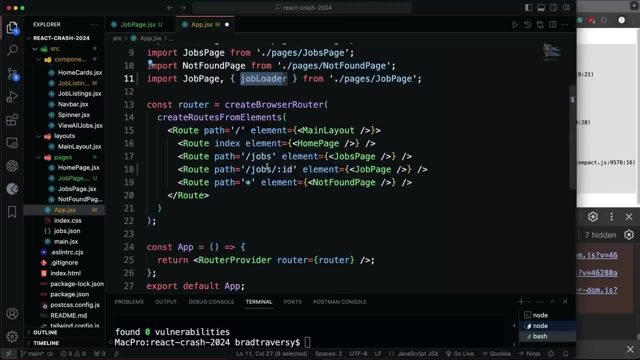 Imported job page. that's default, So no curly braces around that. but then we can also go like this job loader, cause we exported that as well. So now we have access to this job loader and with react router we can go down to where we have the route for job page. 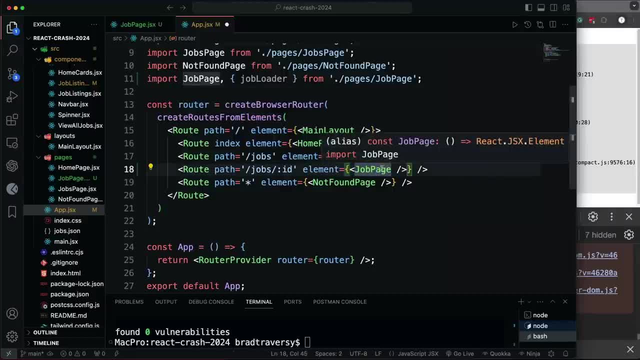 So we're going to put this in the route, not the, not the job page um component itself, but in the route. So I'll go after element and then say, look, I'm going to import this, I'm going to loader and set that to job loader, like that. 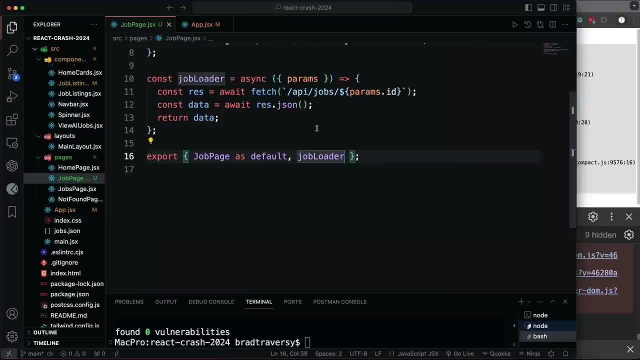 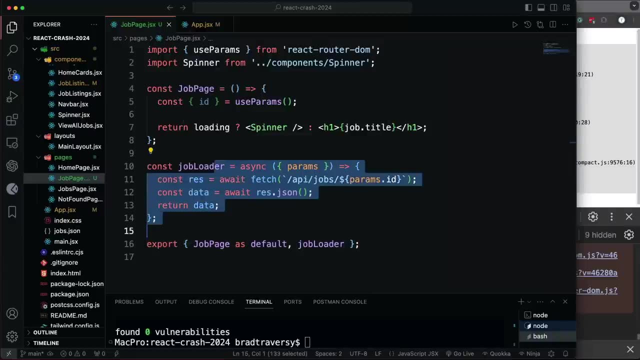 All right. So now we're passing in a loader. Now the way that we access this loader from in here, from in our component, So we're exporting it from you know from this function, and then we're passing it in to the route. 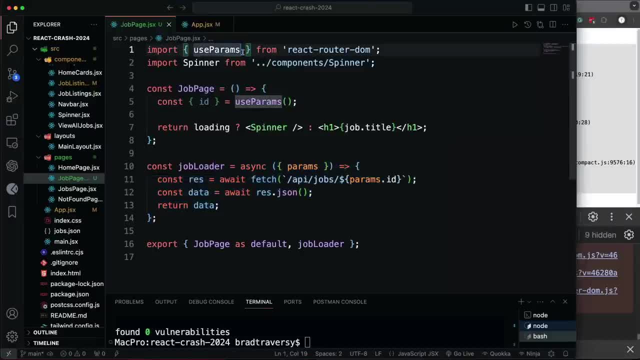 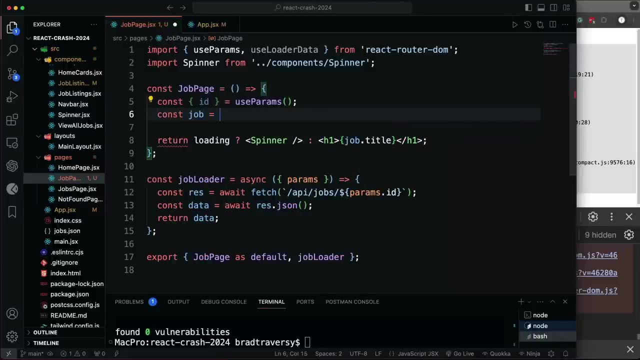 So the way that we can access that is with the use data load: use loader data hook, So use loader data and that's going to be from react router Dom, And then all we have to do is simply say: const job set that to use loader data like that. 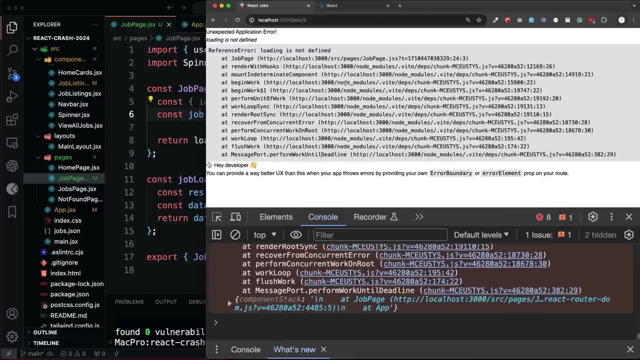 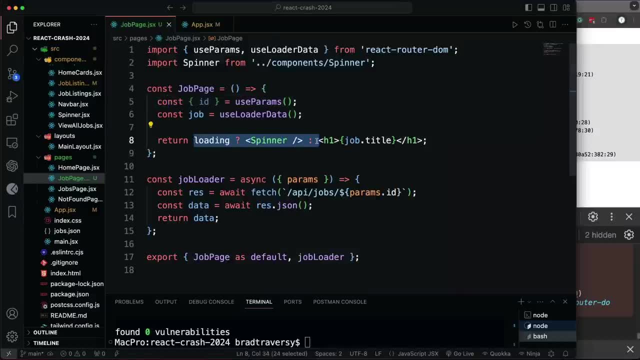 And then I'm going to save. let's come back over here. Let's see, Loading is not defined, so we're not using loading anymore. So I'm just going to return the H one and there we go. So you can see we're actually getting the data. 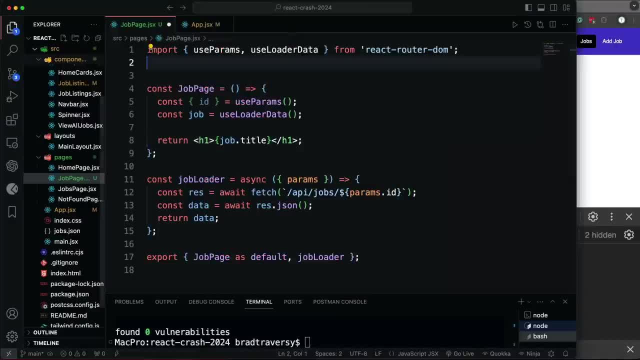 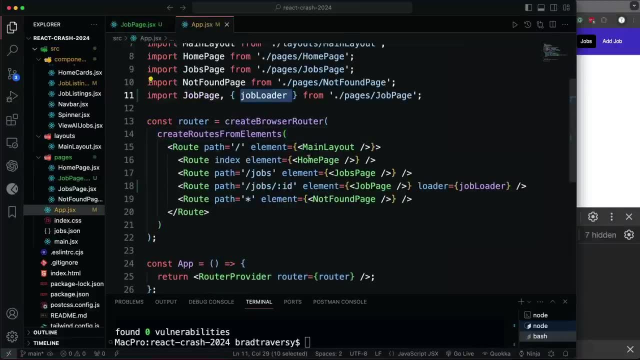 but this time it's actually coming in through that Loader. we don't need the spinner either. So we cleared up this file quite a bit And in addition to that, this job loader, we can pass into other components as well and use that to get a job by its ID. 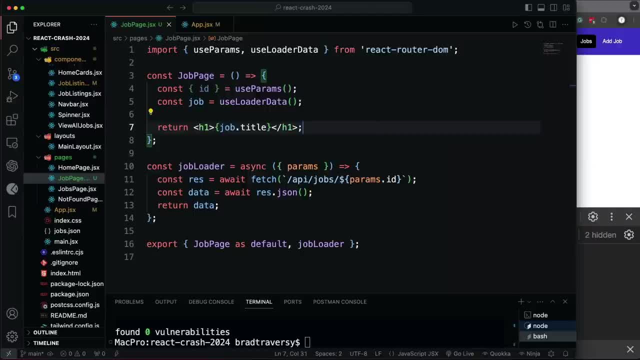 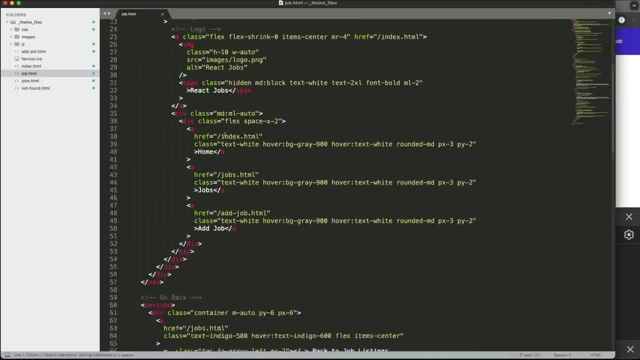 Now let's finish up this page. So I'm going to go to my theme And it's going to be the job dot html file And there's there's quite a bit here. So let's see, we have this section with the go back button and then this section. 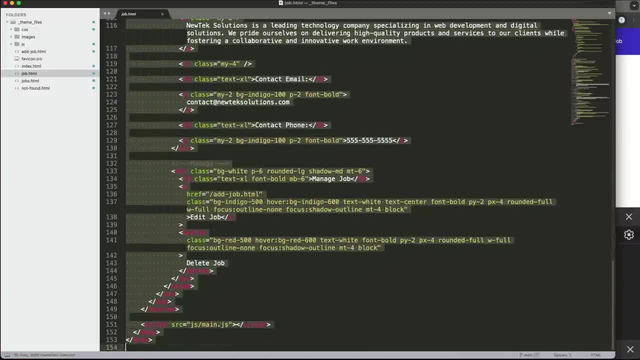 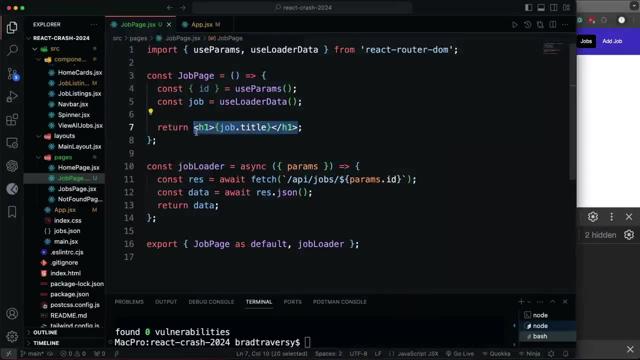 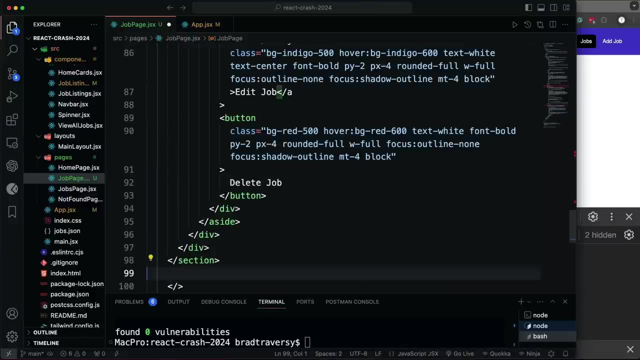 So I'm going to grab both of these sections. Okay, We're going to grab both of those, and then we want to return here. We're going to return a fragment with both of those sections, And then let's not forget to change all the classes to class. 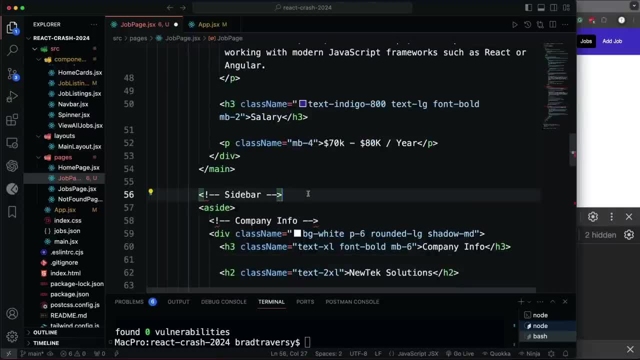 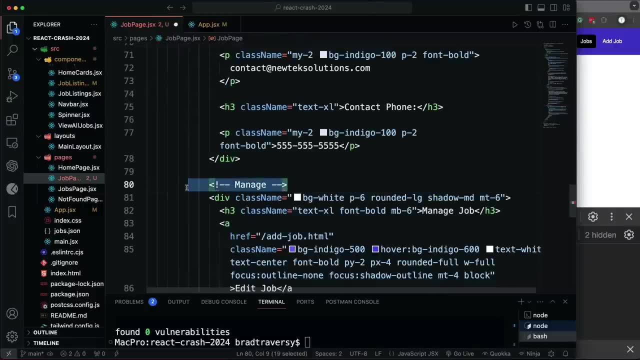 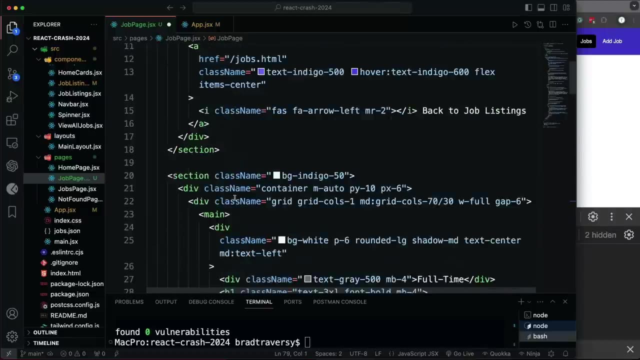 So we're going to go to class name and then any comments like sidebar right here. comment that out and get rid of that. Get rid of that, And is that it? I think so, So let's save All right. So now we just have just hard coded data. 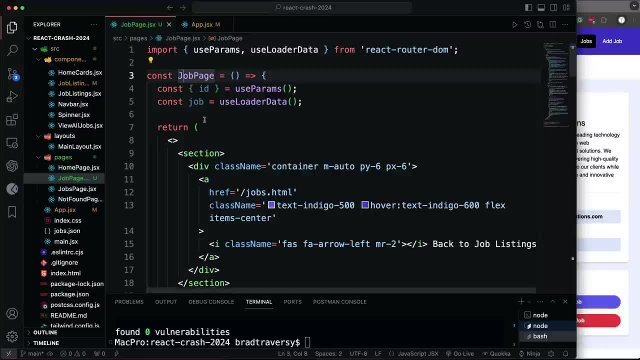 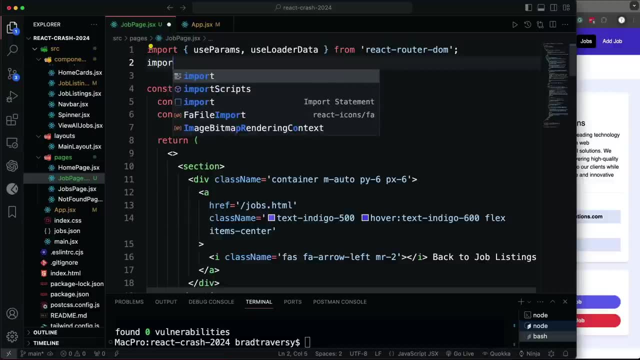 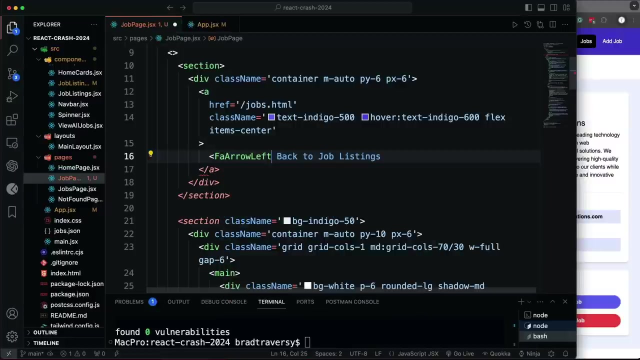 right, So we need to replace this with dynamic data. Also, we have an icon right here For the, the F a arrow left. So let's bring that in from say F a arrow left, and we're going to replace this with F a arrow left, and let's add a class name. 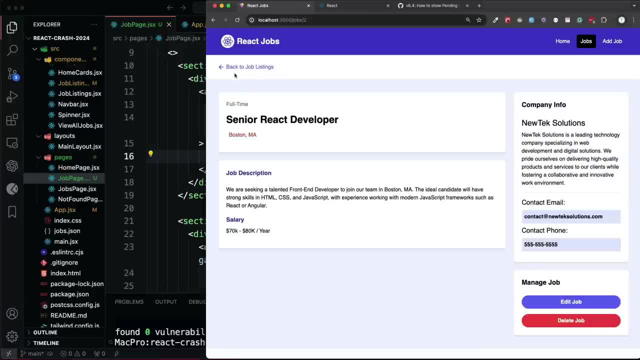 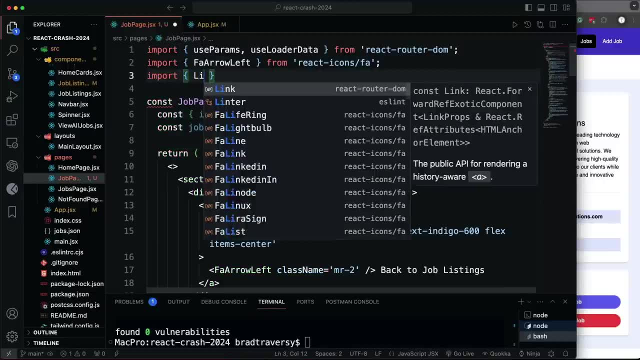 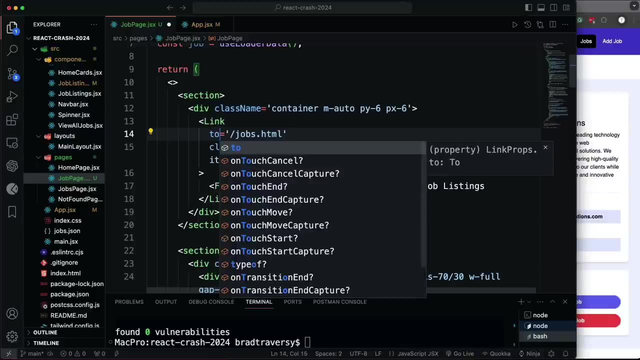 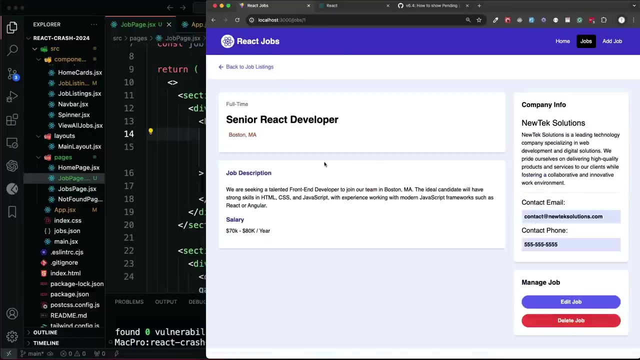 We're going to do margin right to and now we have our arrow And then, as far as the link, we need to bring in link and change that to link, change this to two and change this to just slash jobs. So now the back button should work good. 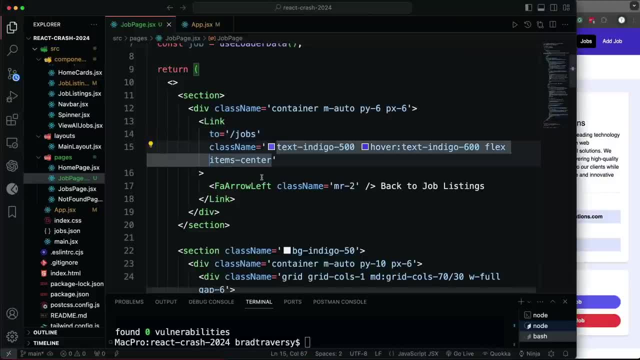 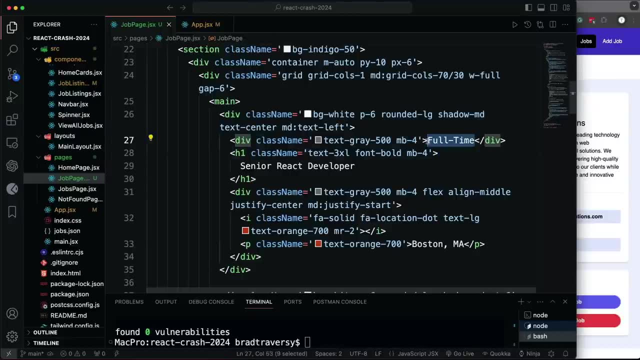 but notice they're all senior react developer, no matter what, because they're hard coded, but we have access to this job object so we can simply replace everything. So like right here, full time. let's change that to job dot type rights. change that. this is going to be the job dot title. 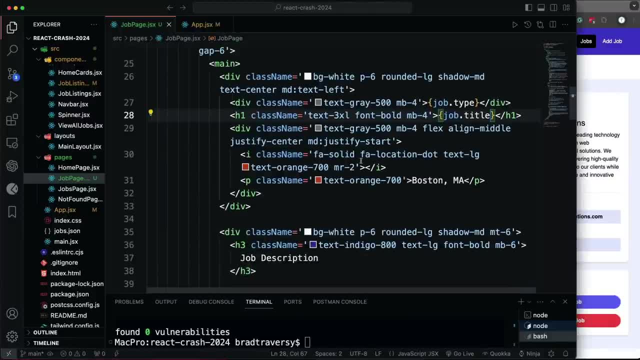 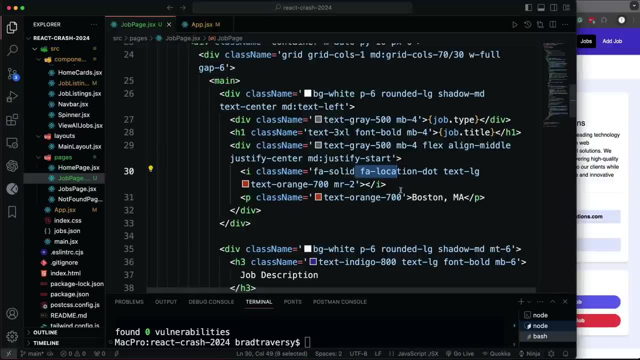 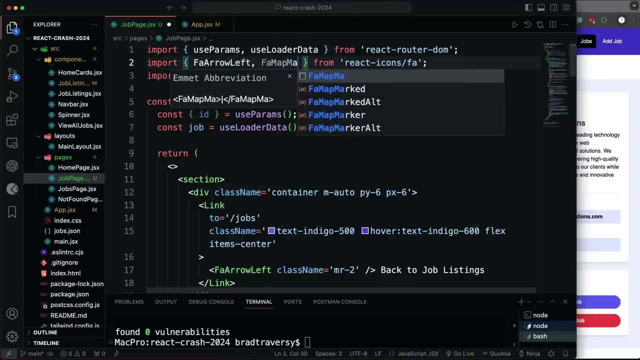 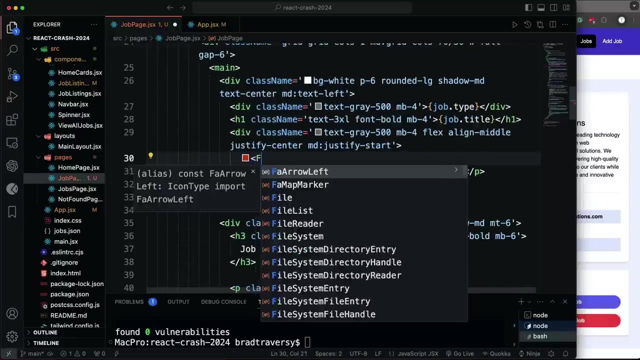 Okay, now we get front-end engineer. We do have another icon here, which I believe we're going to use, the map marker For that. Yeah, let's, let's bring in F a map Marker and let's replace this F a map and see what that looks like. 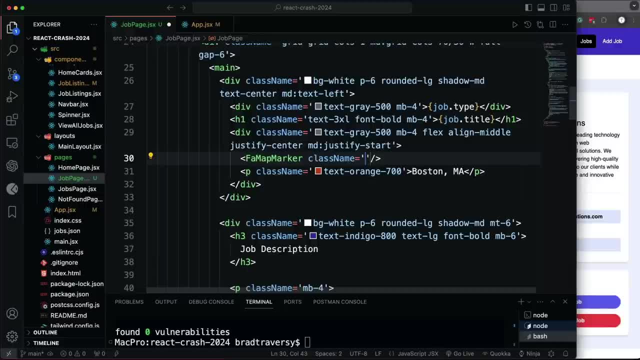 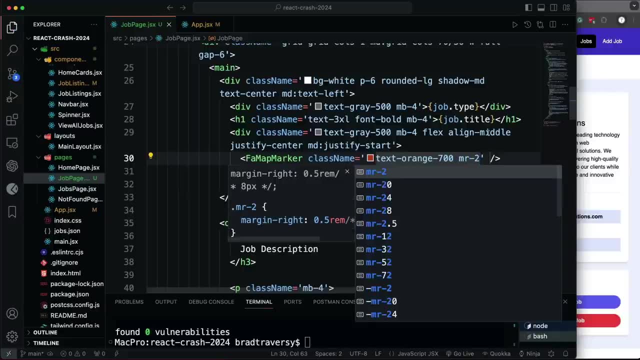 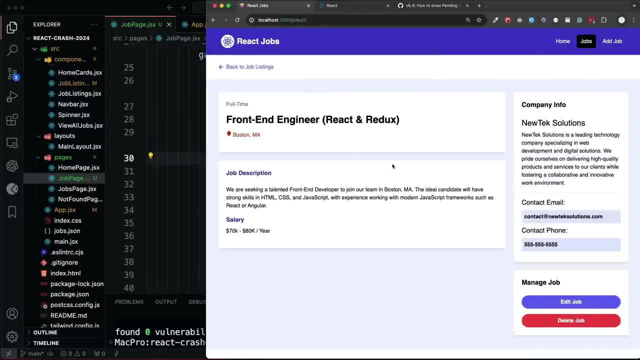 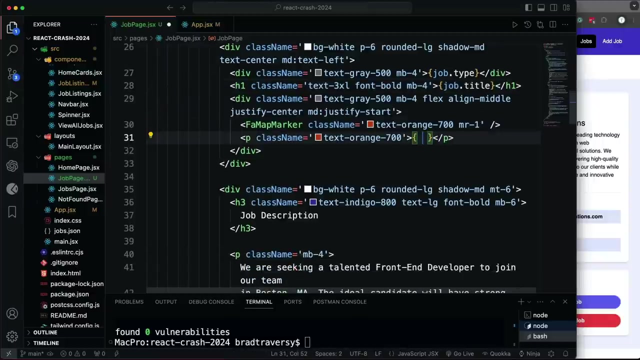 Yeah, so we want to give that, Let's say, class name text, dash orange, dash 700, and margin right to our margin, right one, Maybe. Yeah, that's good enough. Okay, so underneath that, this Boston mass, we're going to change that to job dot location. 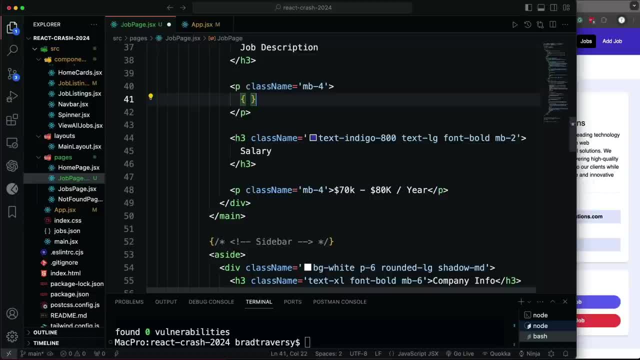 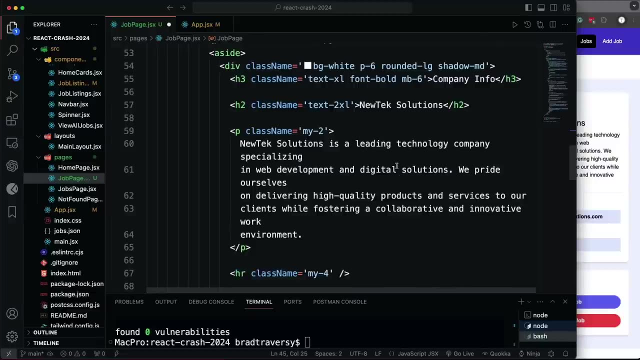 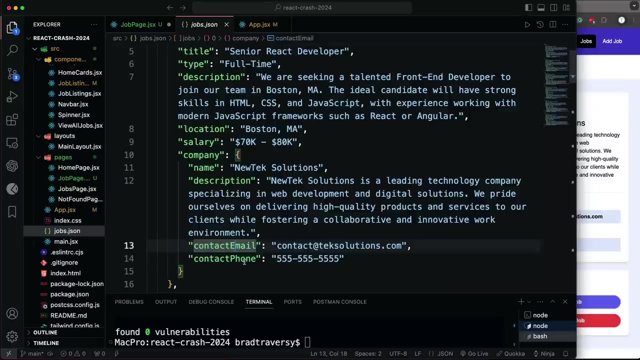 We have the description job dot description salary. So this right here we're going to replace that job dot salary. Now in the sidebar we have the company info And if we look at the data we have a company object with name, description, contact, email and contact phone. 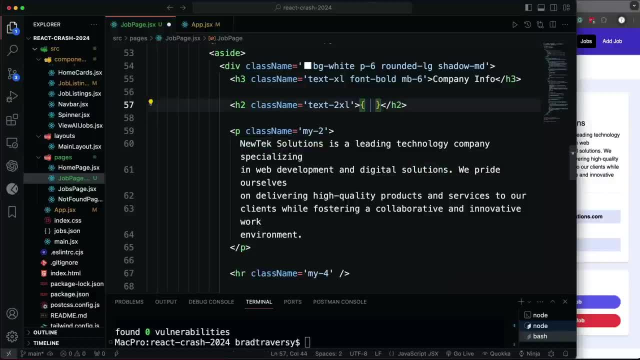 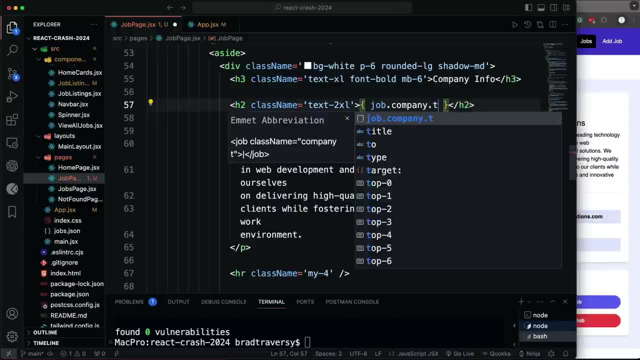 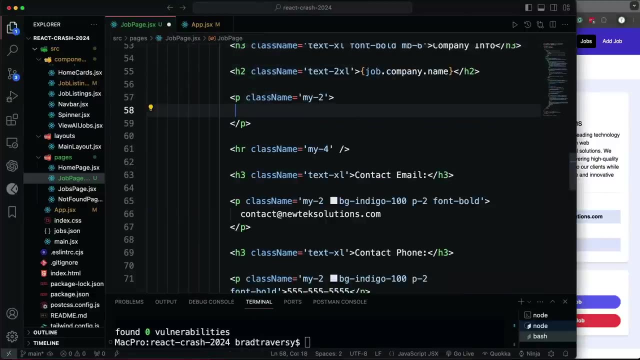 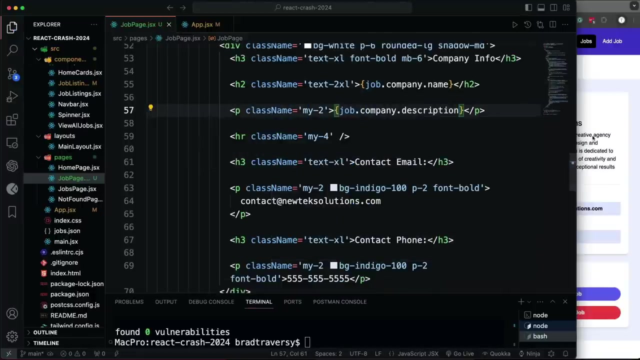 So for the name it's going to be job dot company Dot Tight, was it name? Yeah, so we get the name, then we get the company description. So that's going to be job Company dot description And then we get the contact email. 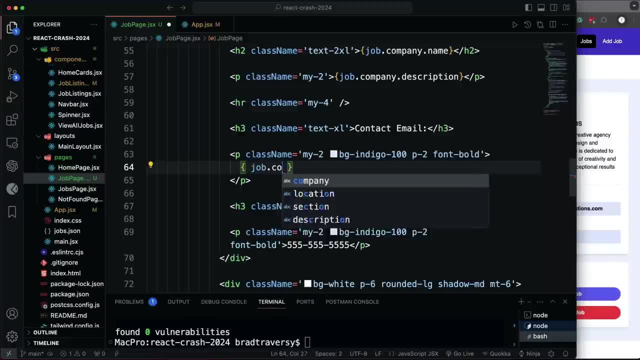 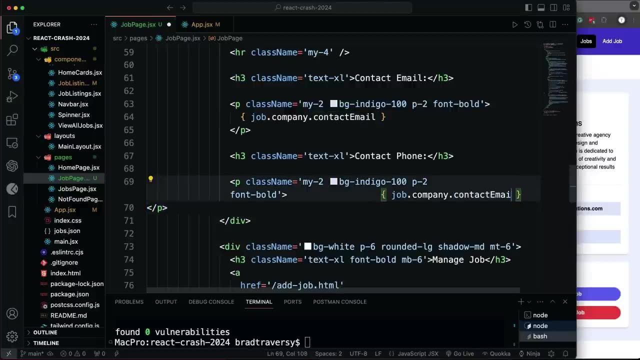 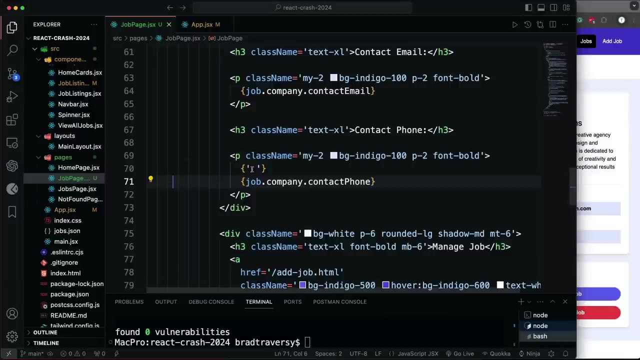 So this right here is going to be job dot, company dot contact email. And then we have the phone. So that's going to be job company contact phone. All right, so all that stuff Is now coming from our back end. And then what do we have down here? 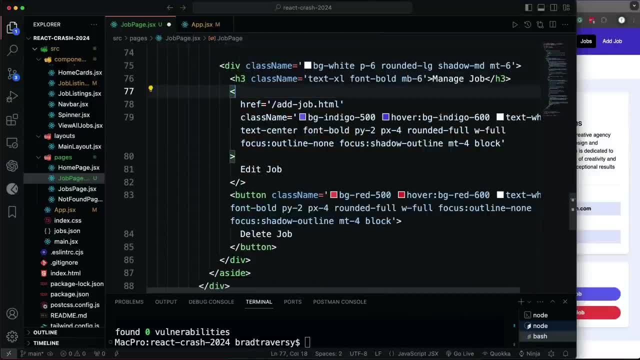 We have the edit and delete, So the edit is a link, So let's change that to link, Let's change this to two And then, as far as the link itself, let's make this dynamic with some back ticks, because we want this to go to slash, jobs, slash, edit, slash and then the job dot ID. 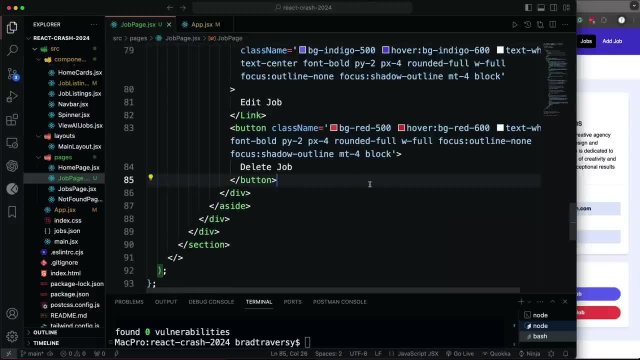 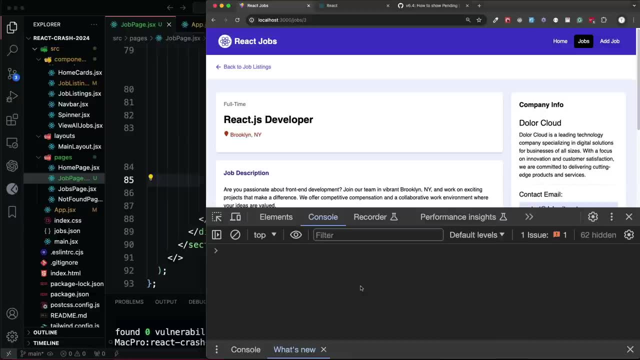 And we'll handle that later in the button. We'll just leave that as is for now And there we go. So now, whatever we click on, we can see the actual data, and let's make sure we're not getting any Errors. 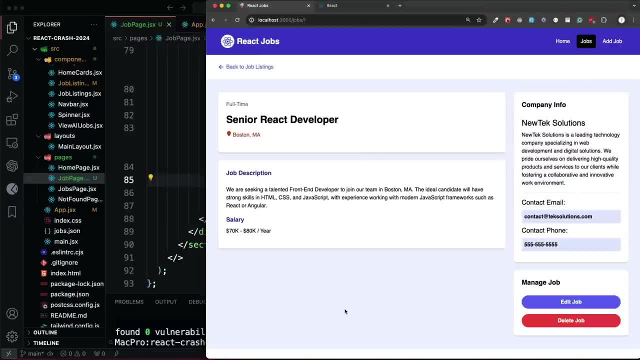 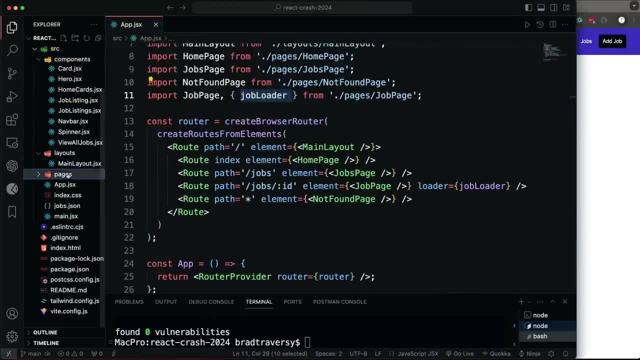 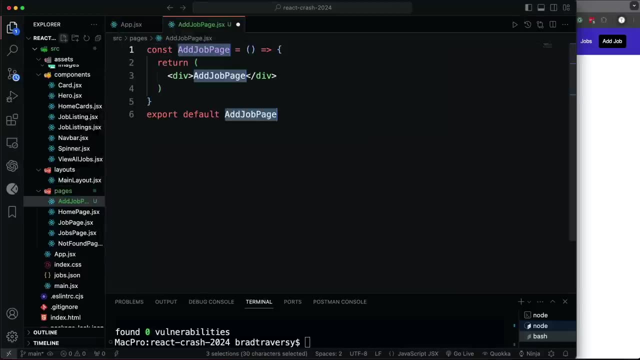 Cool. So we now have our single pages. So now we're going to do the, the ad job page, which right now doesn't exist. So let's create the page. So under pages we'll say add job Page And let's add the route. 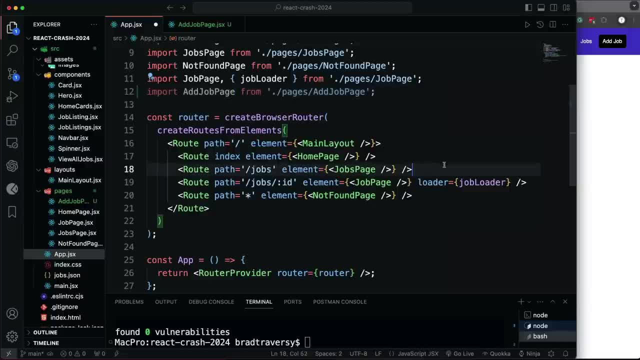 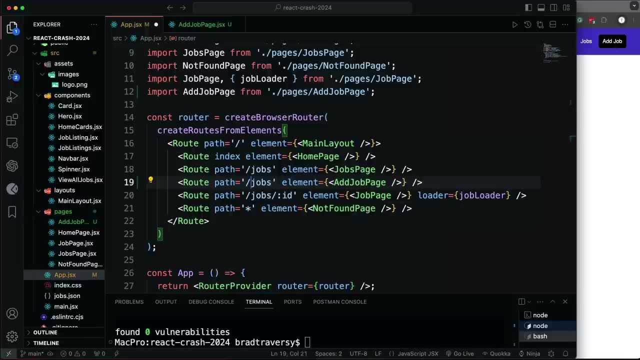 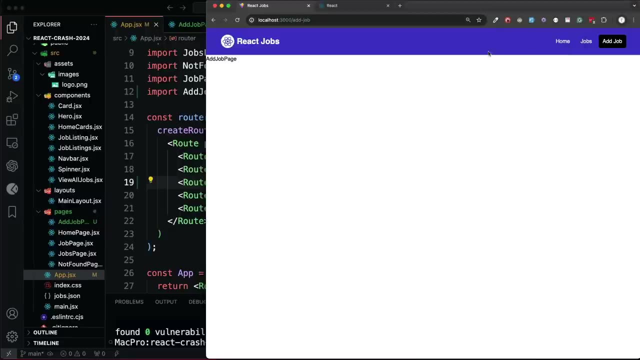 So we want to import ad job page and then we're going to put this- I'll just copy this down: Change this to add job page And then the path is going to be: Add dash job. Okay, so now, if you click on add job, 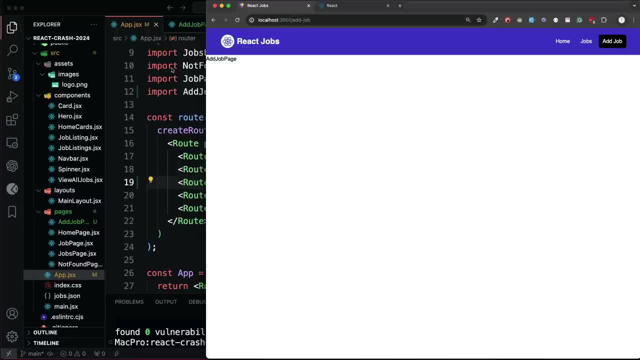 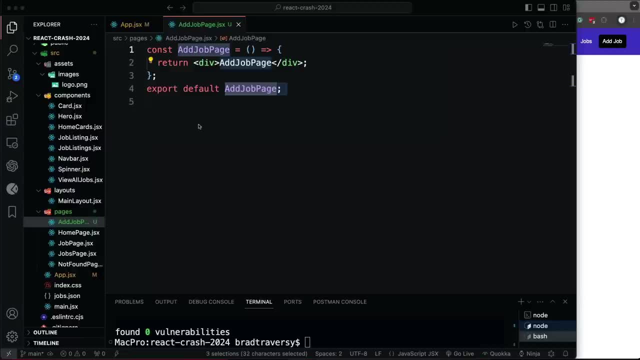 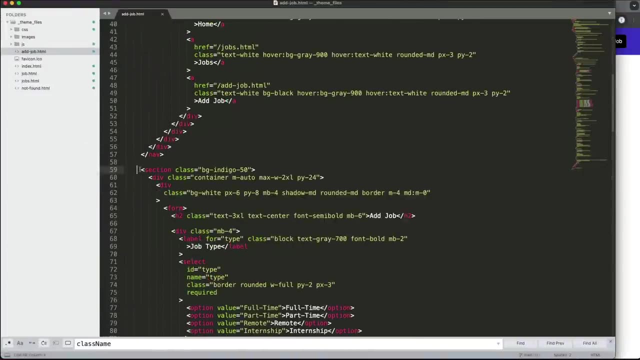 you should see that also. this button here should also go To the ad job page. All right, Now we need to get the form. So let's go to the theme file. So this is ad job dot HTML, And what we're going to do is get the whole section right here that has the form in it. 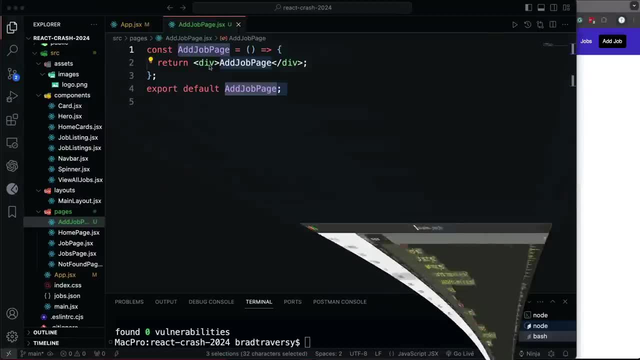 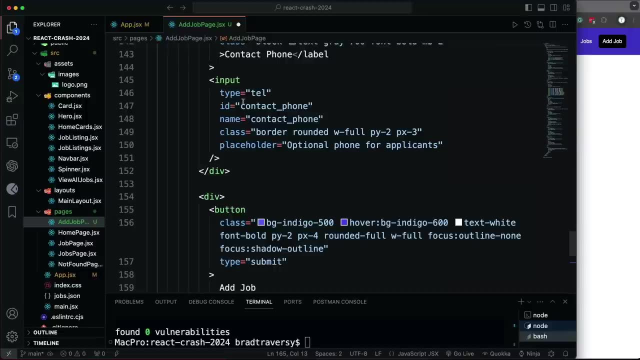 So just grab this entire thing And let's paste this in the return. So right here we're going to have parentheses and then paste that in. Now we have to change all the instances of class. So command shift L class name. 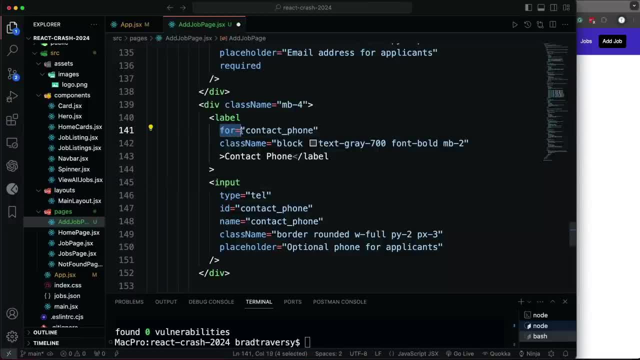 Also, these have labels with the four attribute, which isn't allowed in JSX. We need to change it to HTML four. So I'm going to select the four equal, not just four, because I'm sure there's other things in here that have for. 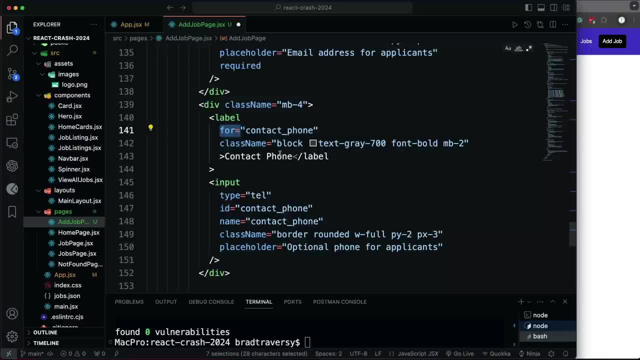 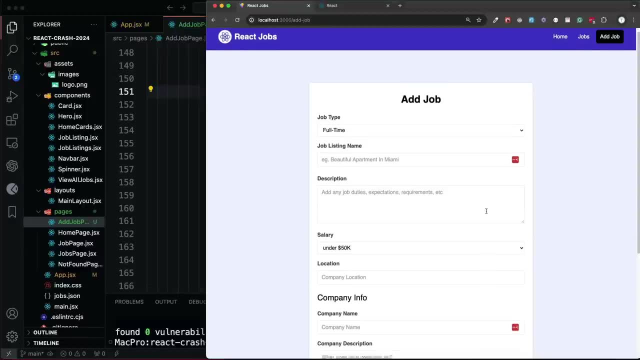 So select the equal sign as well, Select all of them, and then change it to HTML. Uppercase are four. I mean uppercase F for save it, And now we have our form. Now there's many ways To work with forms. 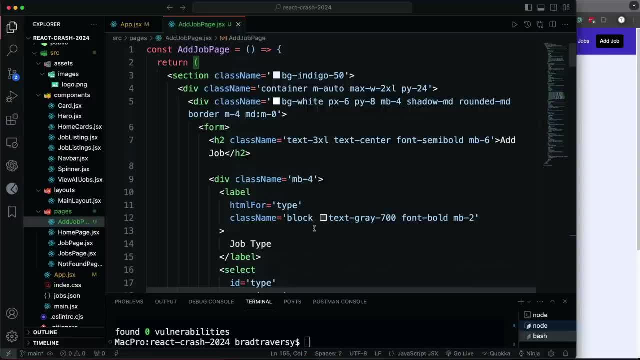 There's other libraries like formic. There's a lot of things you can do. You can use refs, but the, I'd say, the common way, the core way of doing it, is adding a piece of state for every field in your form. 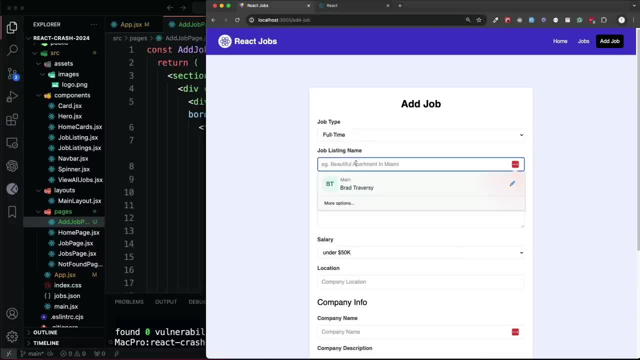 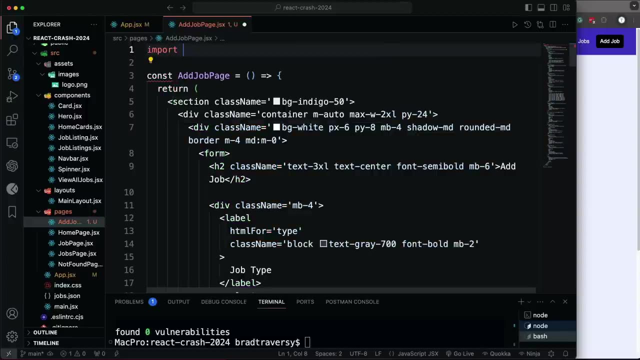 Okay, because these change and then when you, when you change it, when you type in it or you select, you change the state of that item. Okay, so what we're going to do is bring in add state. You, sorry, use state, add state. 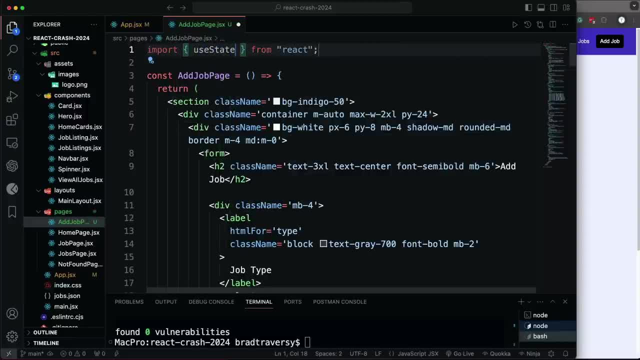 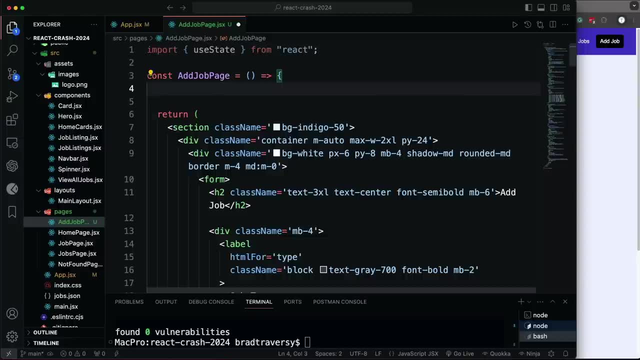 So let's import use state And then we want to create a state item for each field. Now, there's different ways you can do this. You could have just a single object in your state and have all the fields in that object, or you can do a separate piece of state for every field. 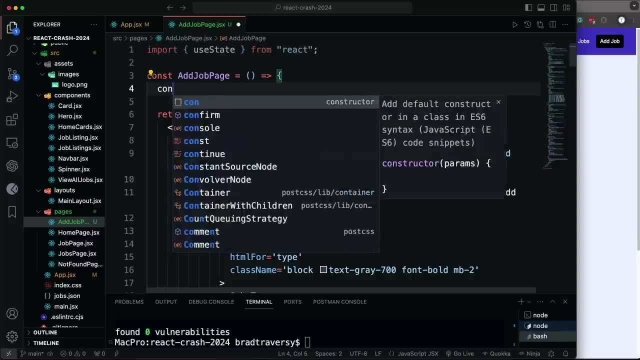 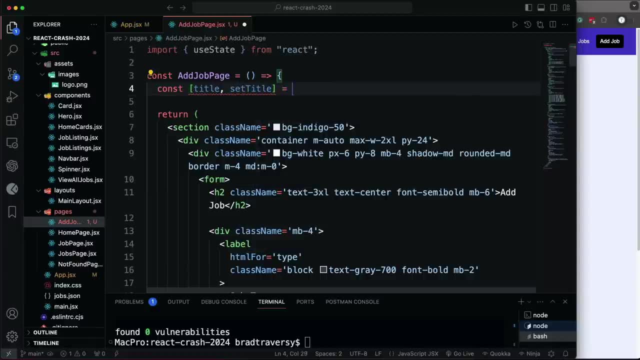 which is what I'm going to do, just to keep it simple. So let's say, once we know we have a title, so title, and then set title to change it, and set that to use state, And then in here is going to be the defaults, and most of these, actually all these- are just going to be empty strings as default. 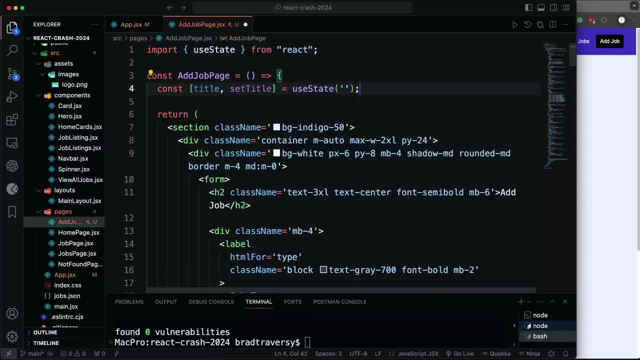 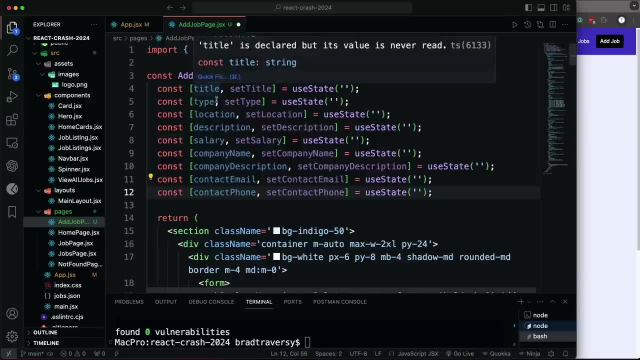 Now I'm going to just copy this down. Actually, you know what, I'm going to paste the rest of these in and then you can just copy them. Okay, so we have title, type, location description, salary, company name, company description. 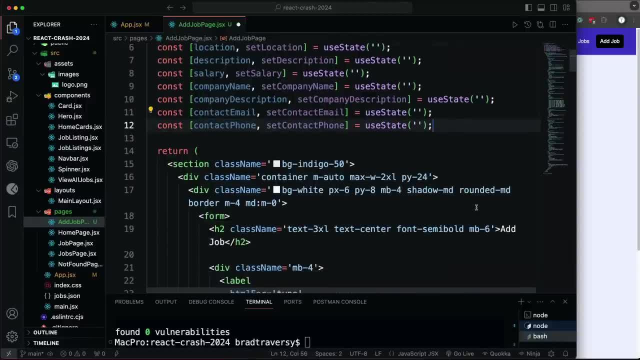 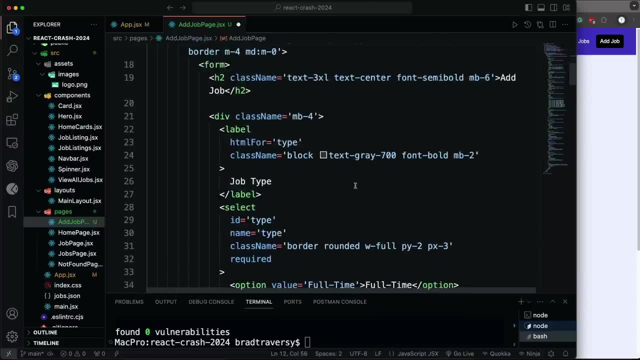 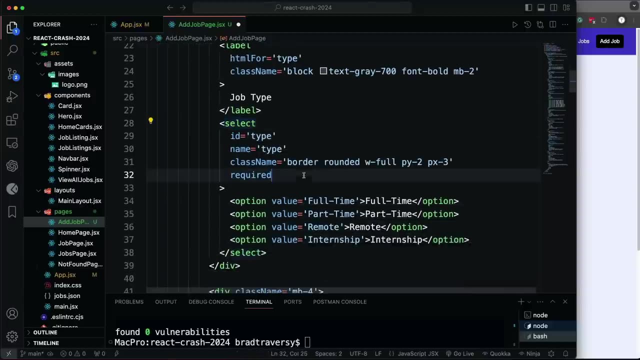 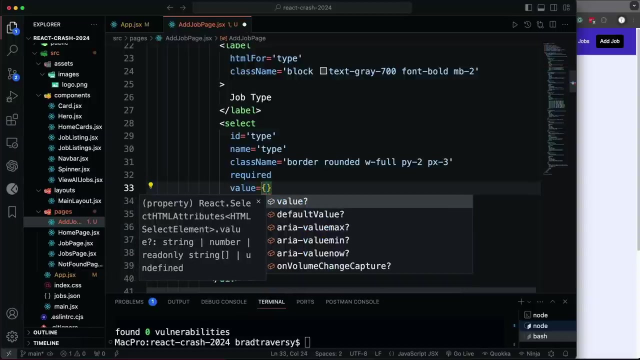 contact email and contact phone, All right. so those that, those are all the state, and what we need to do now is add on each input. So let's see: The first one is the select. It's the type, So this select right here, and what we want to do is add a value and set that value to that piece of state. 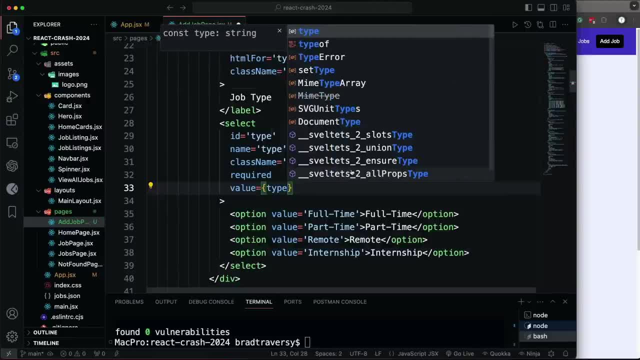 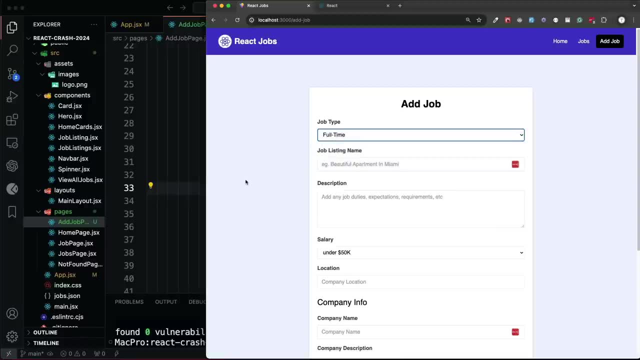 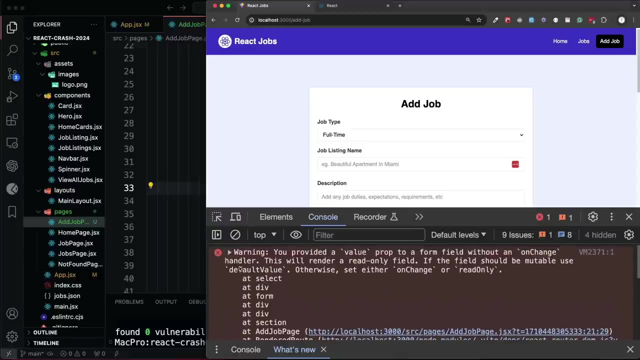 which in our case is called Type. Okay, so if I save that and I come over here and I try to change it, notice it doesn't work. It doesn't do anything. And if I look at the console, it's going to tell me I provided a value prop to a form field without an on change handler. 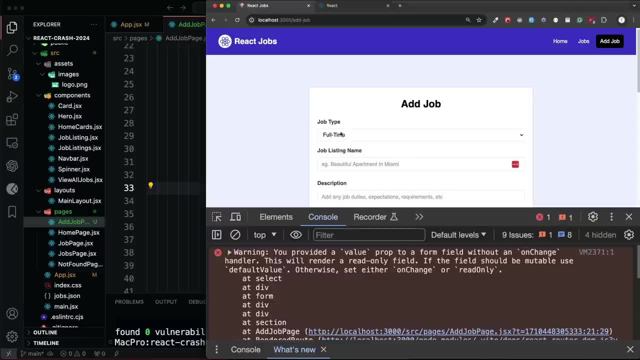 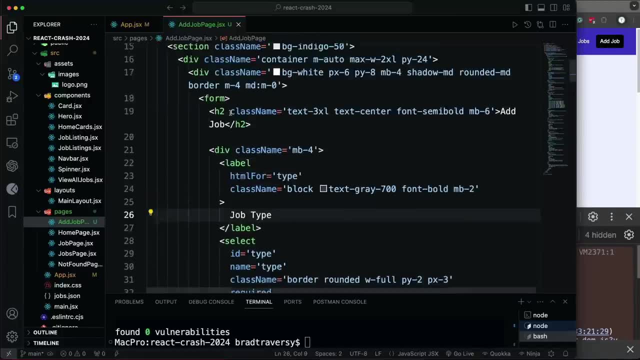 So basically, when you add a piece of state to or you connect a piece of state to an input, you have to add an on change because when you change it that state has to update and has to call this Set type or set, whatever the field is. 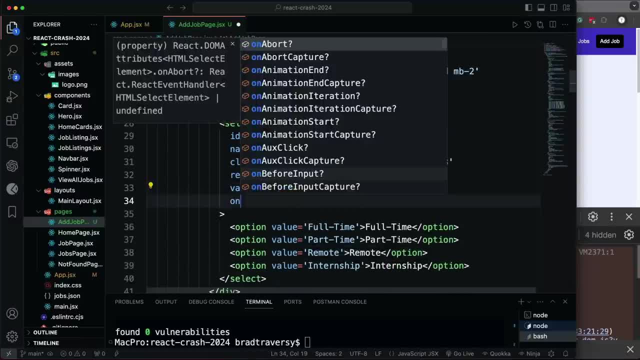 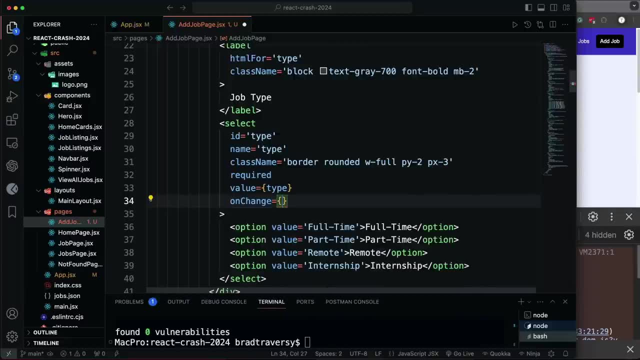 So what we can do is under the value We're going to say on change. So, just like any other event on click or whatever you just add it, camel case, And what we'll do is set a function and this can take in an event param. 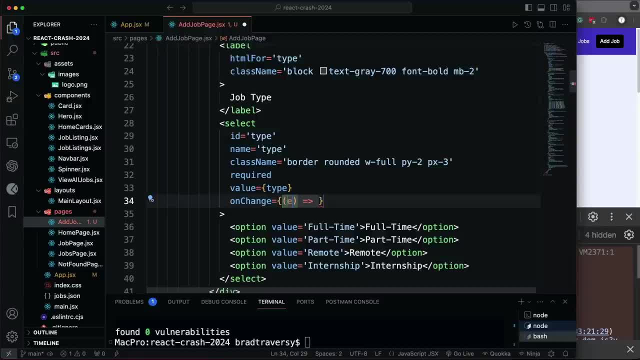 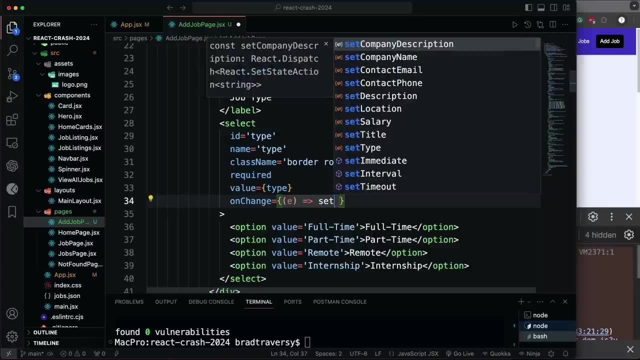 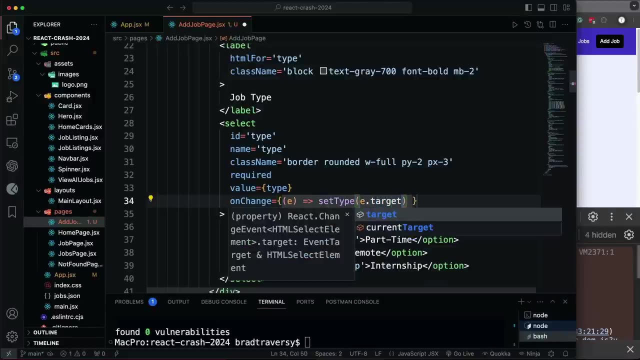 Okay, Now this parameter has on it a target dot value and that's going to be whatever is selected or typed in the field. So what we can do is then say so else we want to set the type And we want to set it to E dot, target dot value, because this is going to be whatever I select and I'm going to set the state to that. 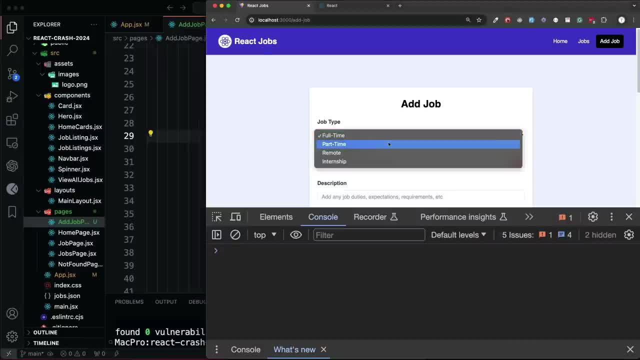 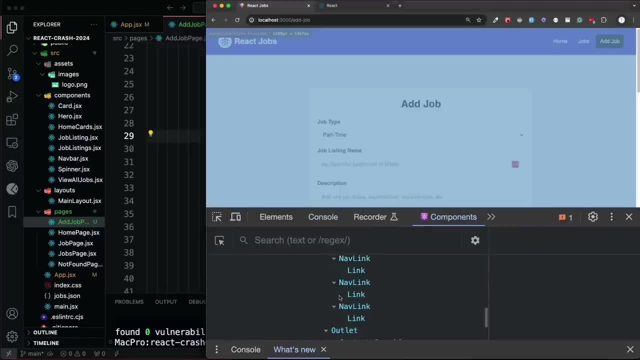 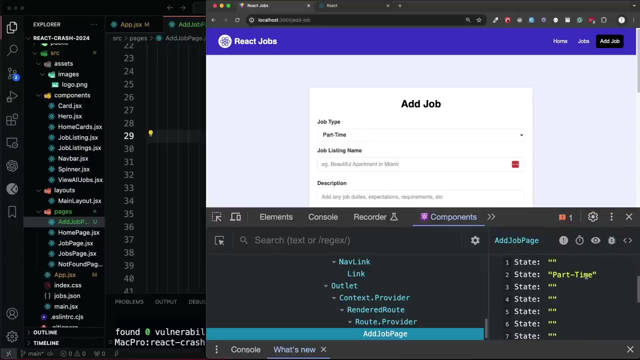 So now if I save that reload and I click on part-time, now it works. And if we look in our components, in the dev tools- Now we have a bunch of stuff here- We look at the add- Add job page And we look in the state where it says part time. 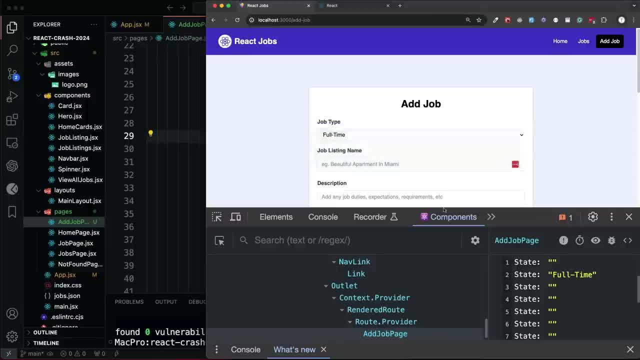 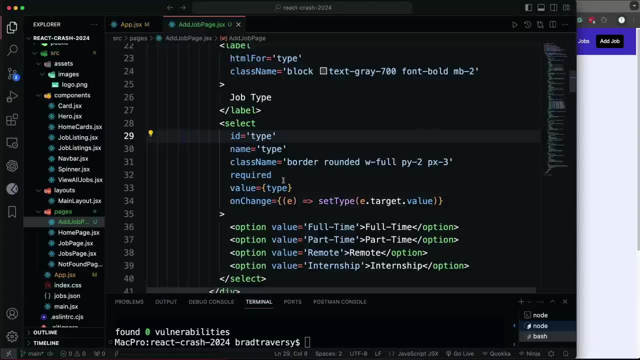 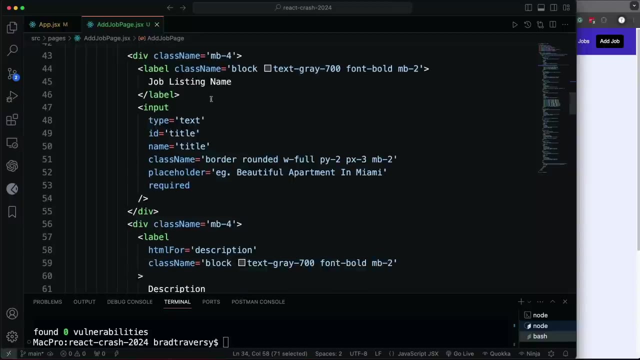 If I change that to full time, you'll see that the state updates. OK, So now this input is part of the component state, So we need to do that for all the inputs. So let's actually copy the value and the on change here and go to the next one, which is the title. 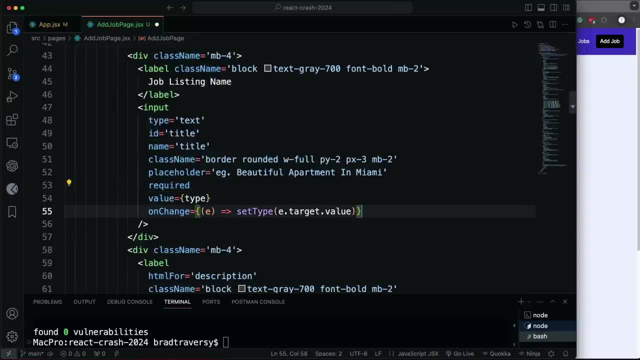 I know this says name, but it's the field, this title, So we're going to paste that in and then change that And that To title OK, And make sure that you this is upper case. If, if you selected both and change them at the same time, then this is probably going to be lower case. 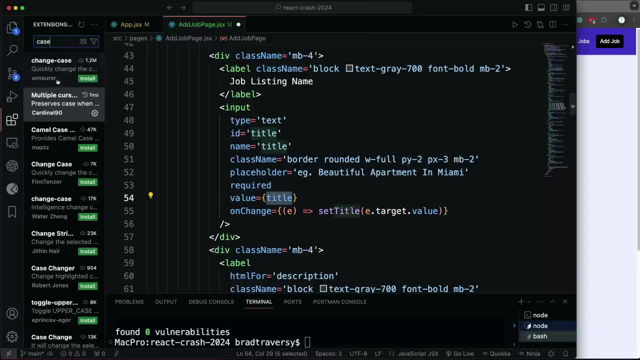 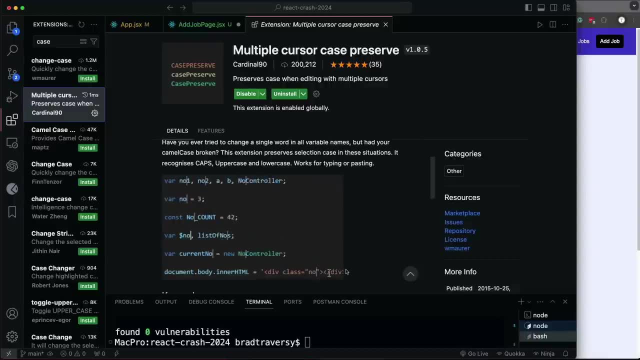 So you can manually change it to upper case, or what I would recommend is using this multiple case preserve extension And it'll basically just preserve your case if you're changing a bunch of stuff at once. So it comes in handy, It's? it's a small extension. 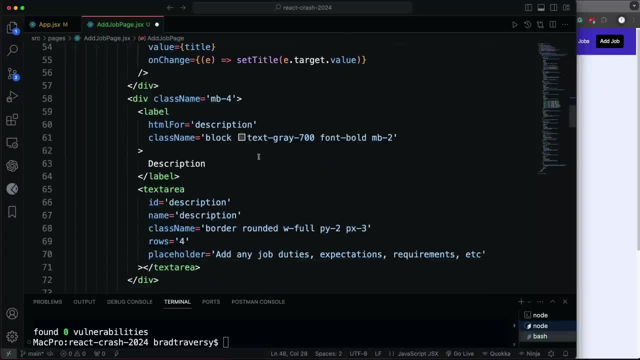 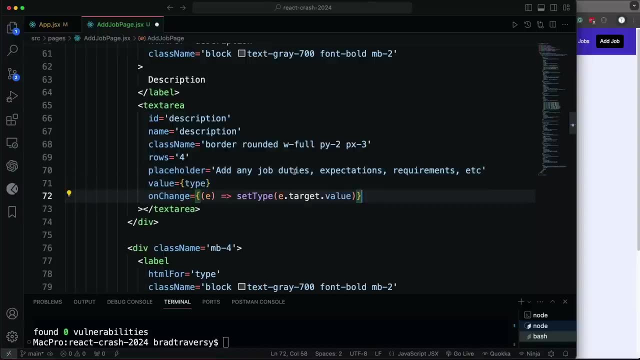 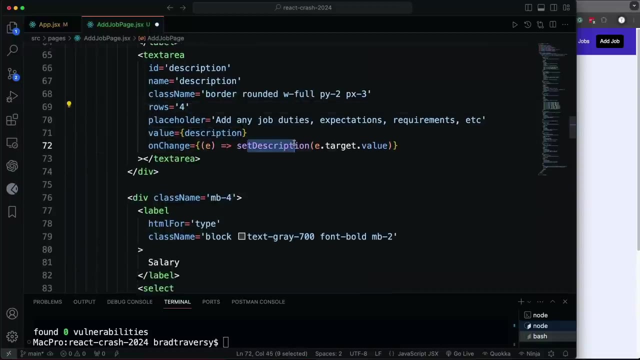 Pretty unknown, But it's very Useful. All right, So now description: that's the placeholder, the placeholder That's the text area, And we're going to go ahead and just change that and that to description. OK, So it's just setting that description state to whatever I type in. on change every time I type in anything: salary. 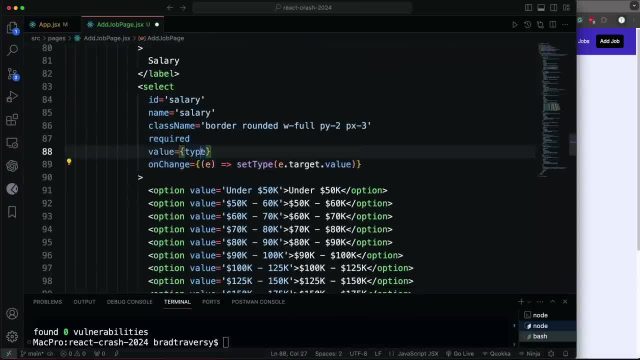 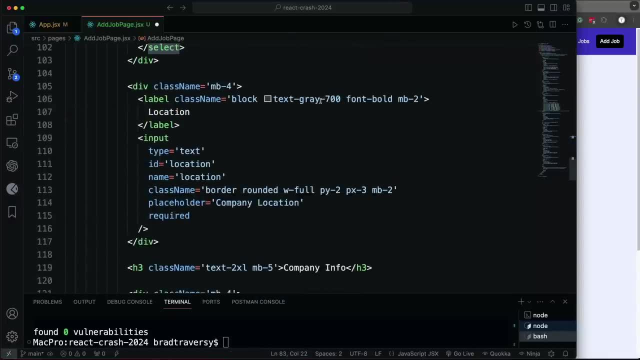 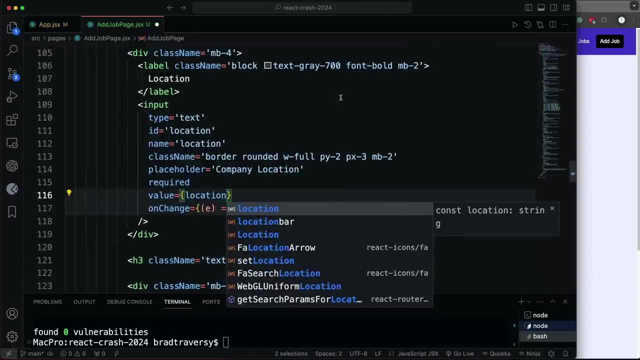 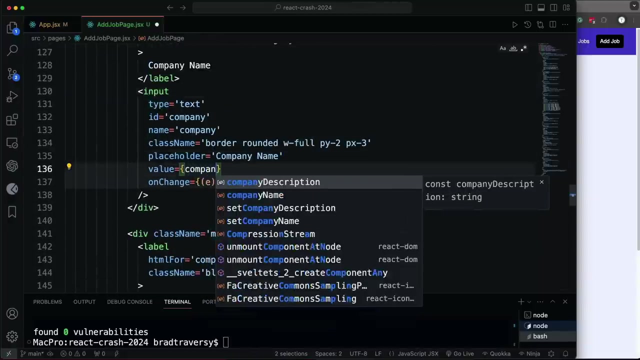 Let's see, this is another select, So let's paste that in and change that and that to salary. OK, Then we have location. So we're going to do this: this location Name, Change that Company Name And set company name. 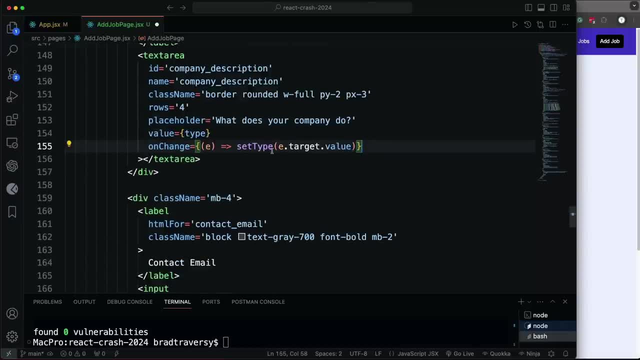 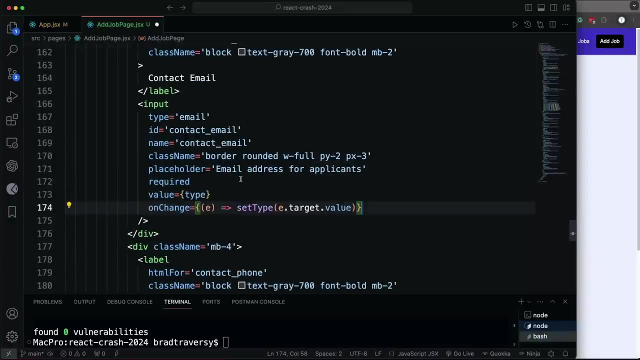 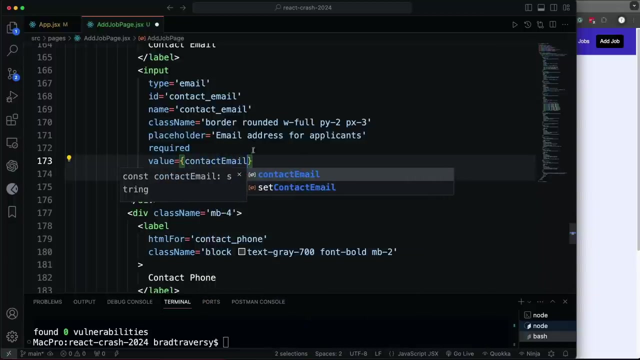 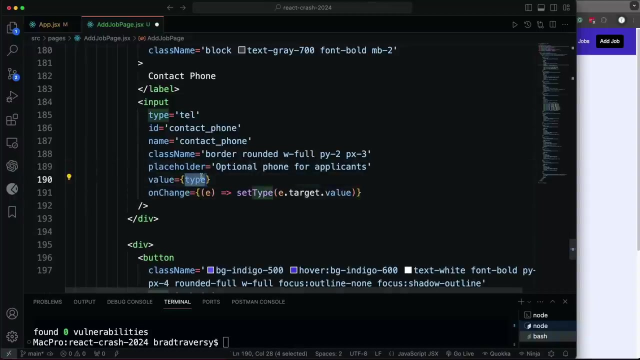 Then we have the description, So The. So this is company description. Oops, it should be set Company description. Then we have the contact email. Again, make sure you're changing this to not just the value. And then for the phone: 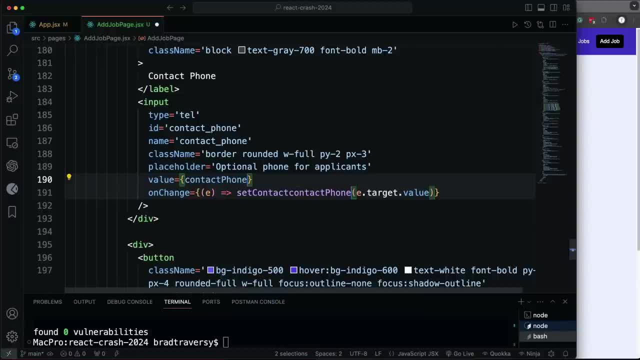 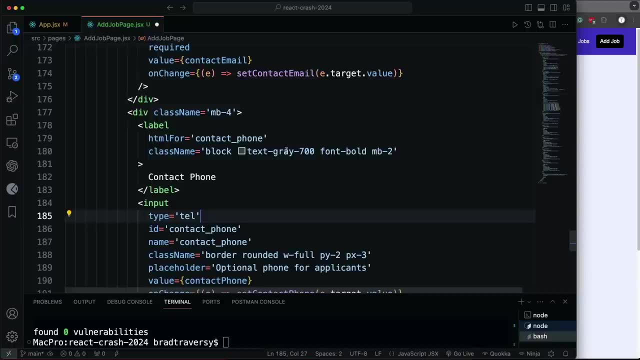 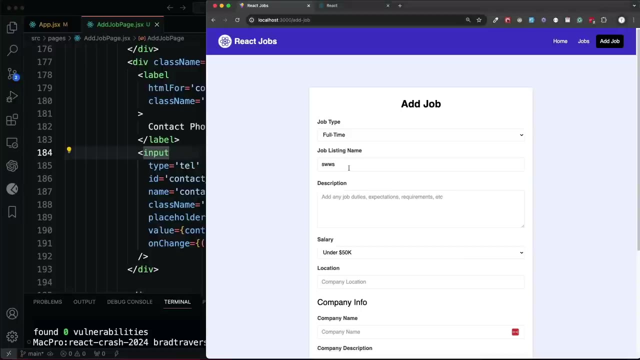 Contact Contact. Contact Contact Phone. Oops, Yeah, I would just double check. Double check all those, Alright, So I think that that should do it. as far as adding the state for each of these, You should be able to, you know, change these up. type in here. 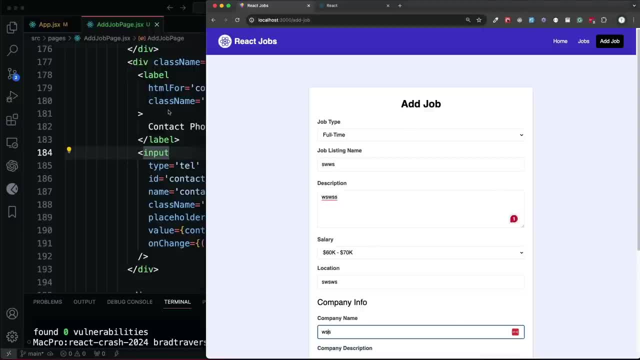 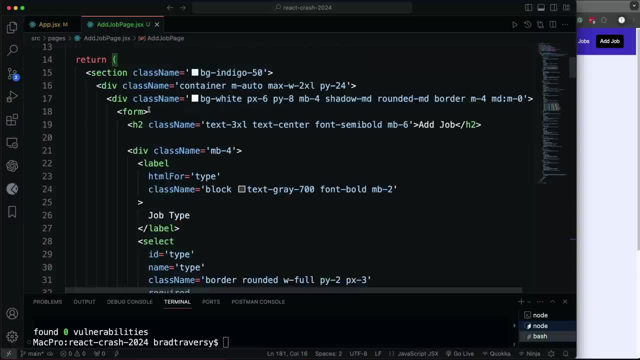 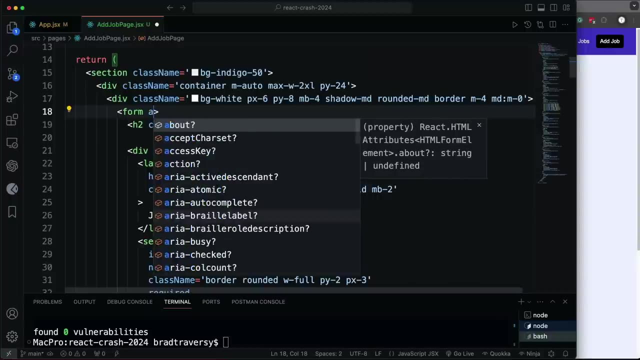 And it's changing the state of, you know, those fields. Now to the form tag. Now they just react. 19 is going to have something called actions, where you can actually put an action, set that to a function. That's a brand new way of doing it in react 19. 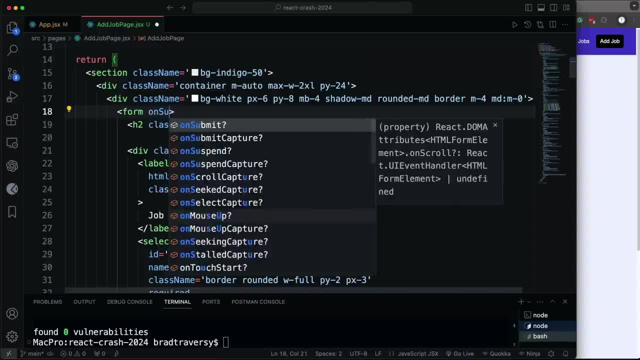 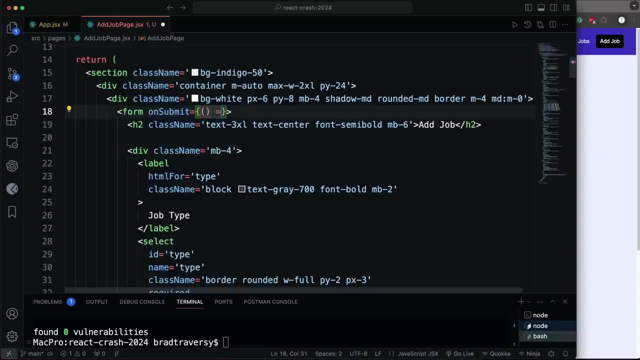 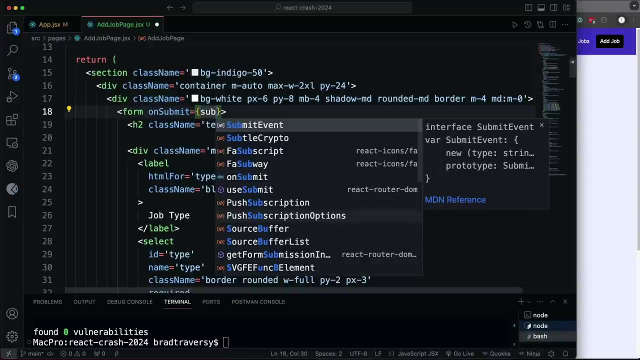 that isn't even released yet. So we're going to stick to just adding an on submit and set that to now. up to this point, when we have events, we've been putting the function directly in here, but we can set it to a function that we create. So let's say we want it to be called, we'll call it. 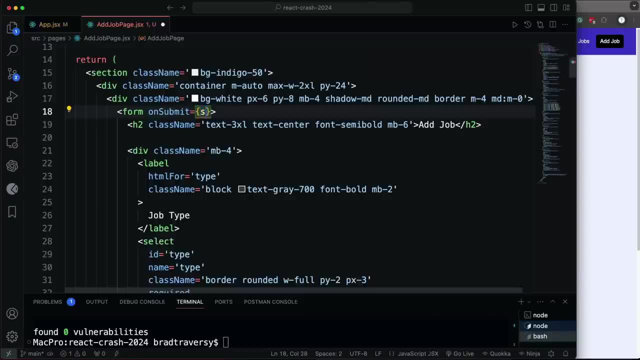 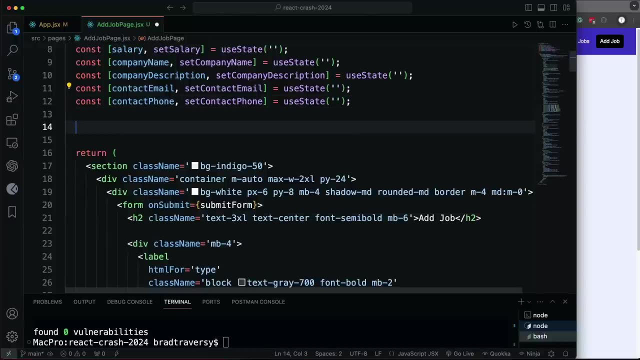 on submit. No, let's call it submit form And then we can create that function up here. I'm going to go above the return cons submit form And I like arrow functions. you don't have to do this. you can use a regular function if you want, And that's going to be the function that we're going to. 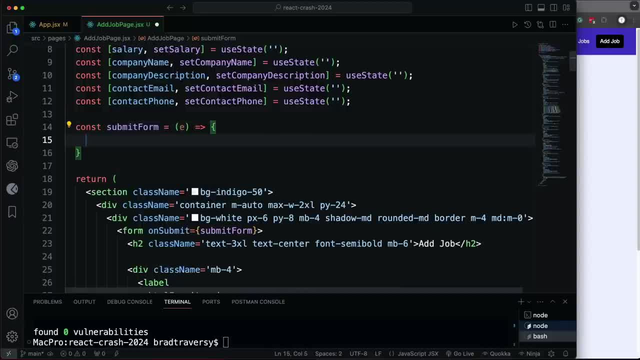 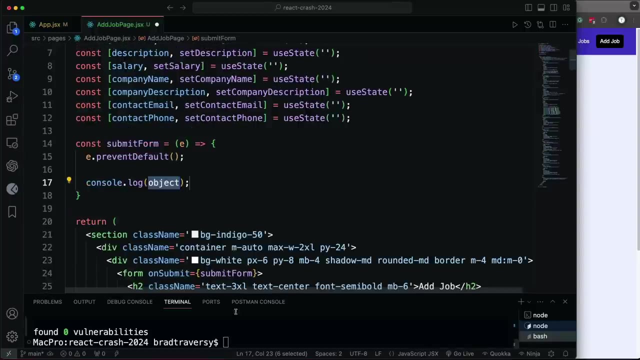 take in an event parameter because we want to stop the default behavior. So we can do E dot, and this is just like with vanilla JavaScript. So prevent default, And then let's do a console log And we should have access to all the state right, because they're all connected to those fields. So 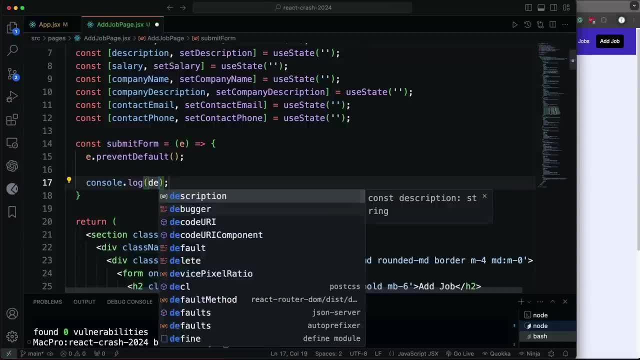 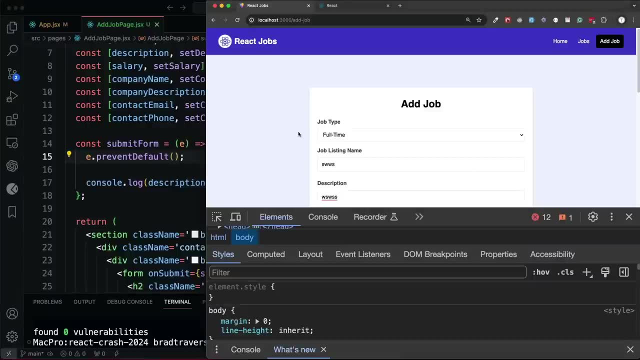 for instance, if I put in, let's say, description, a console log description, right, come over here, let's open up the console And just make sure, okay, and I'm just going to put something in the description and I'm going to. 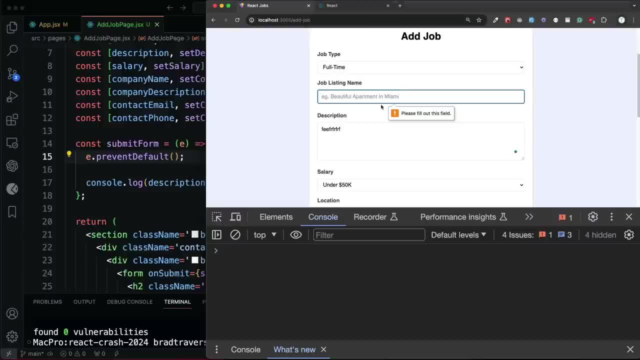 submit the form. Alright, so we do have some required fields. Let's see, is that it? Oh, this is required to. Okay, so now I submitted and what I had in the description right here is now logging. So we know. that the form is hooked up to the description. So let's go ahead and do that, And then let's go ahead and do that, And then let's go ahead and do that. So let's go ahead and do that, And then let's go ahead. 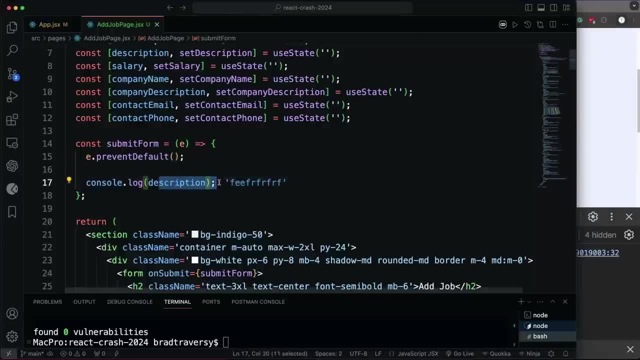 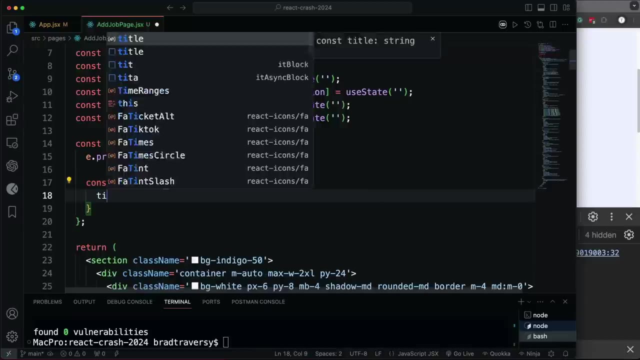 to this event, the submit handler, And we know that we can access at least the description field. So let's construct an object from the form fields that we want to submit to our API. So I'm going to say: const, new job, set that to an object And we want to set the title. And since I'm setting 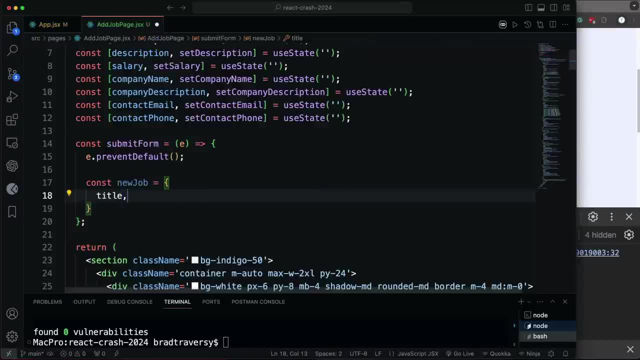 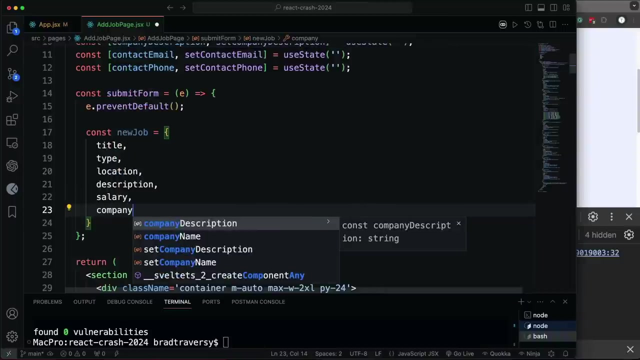 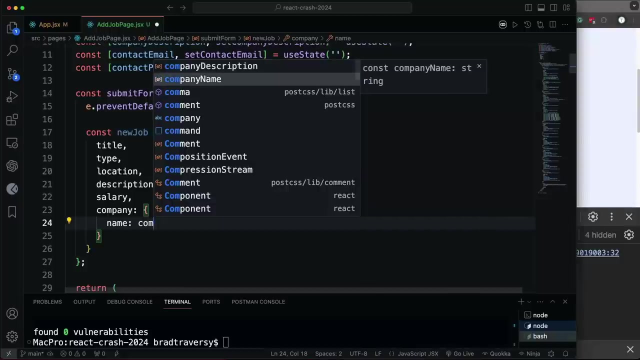 title to title like this, we don't need the second one, we can just simply do that. type: location description. We have the salary. Now this is where- because we need this to match up with the way our API is structured. So now we're going to have our company object And let's set name to the company name And let's set the. 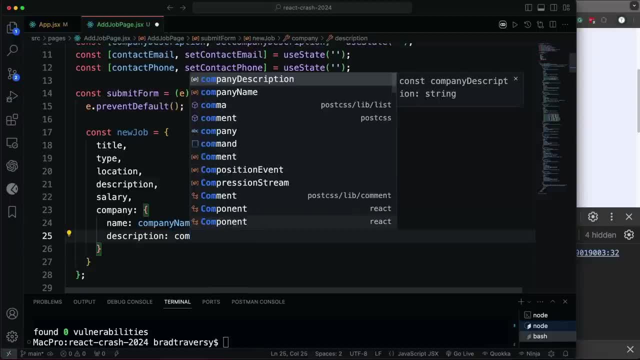 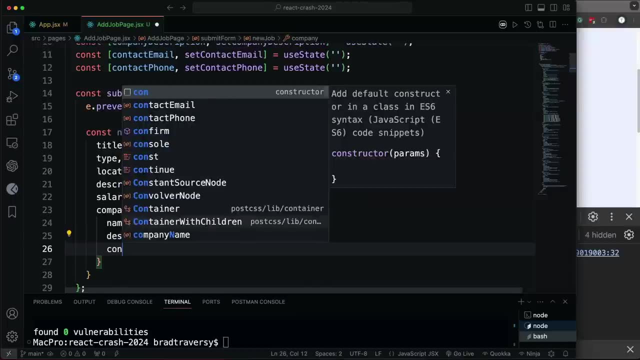 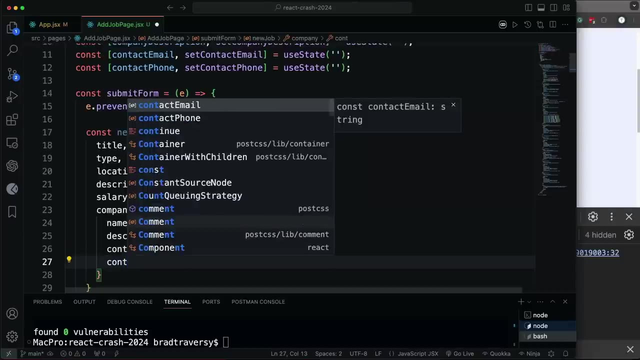 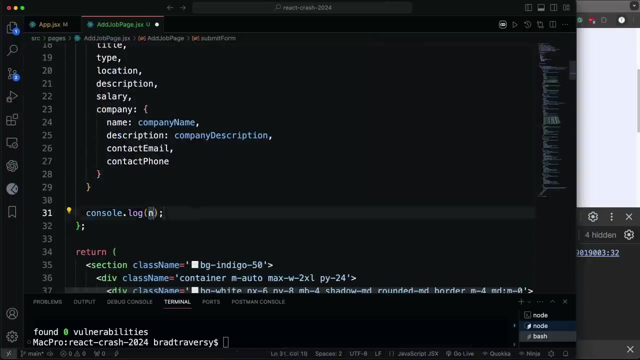 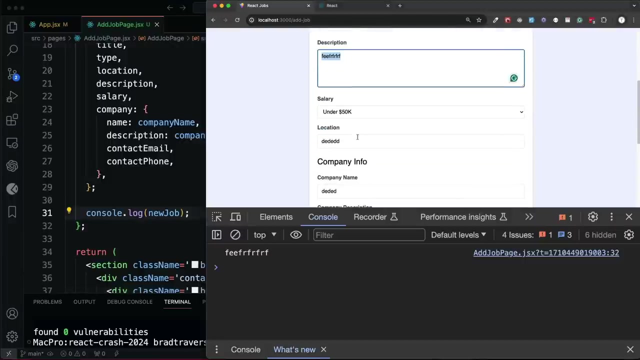 description to the company description, Company description. And then we have what else? contact email, And that's. it's called the same thing, So we can keep it like that. And then contact phone, Alright, and then let's just console log this new job, just to make sure new job, And let's see, I'm just gonna just make sure you fill. 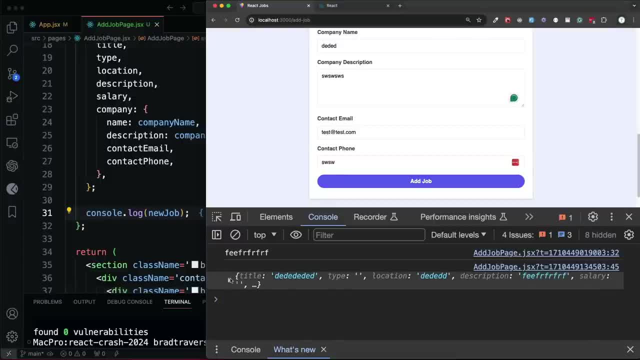 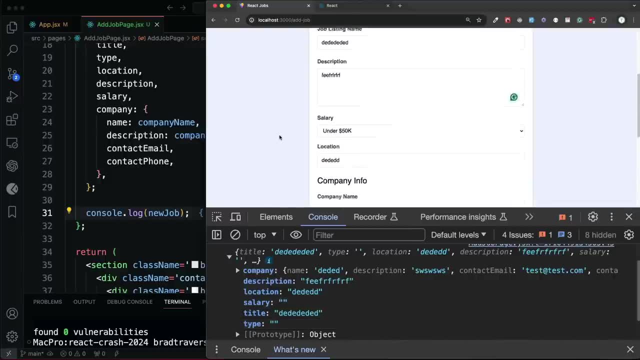 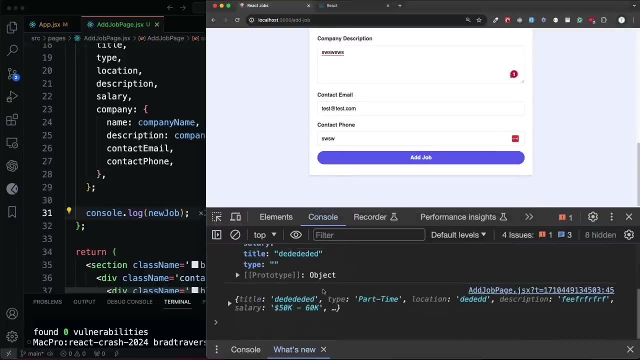 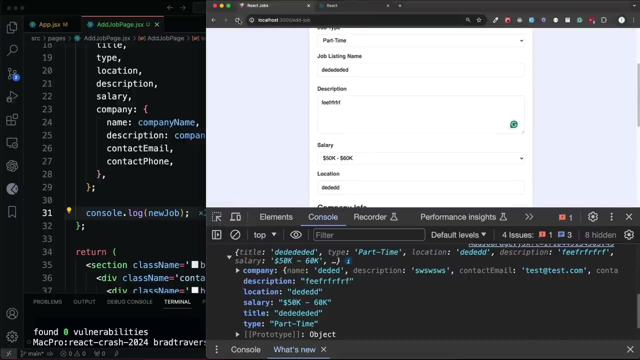 out every field So we can just make sure we submit. if we look in the console looks like salary and type, which are the two select lists. looks like those aren't showing up. okay, now it did salary type, alright, so that did. I just want to make sure. if I don't, if I leave. 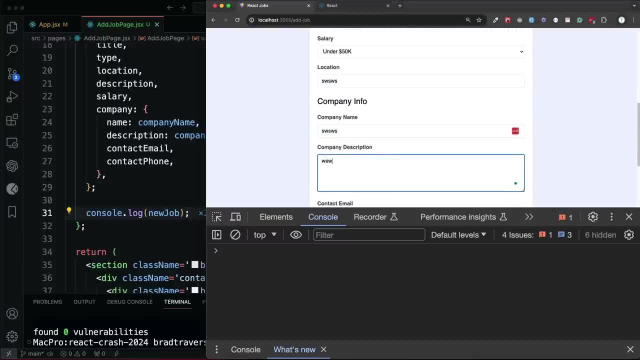 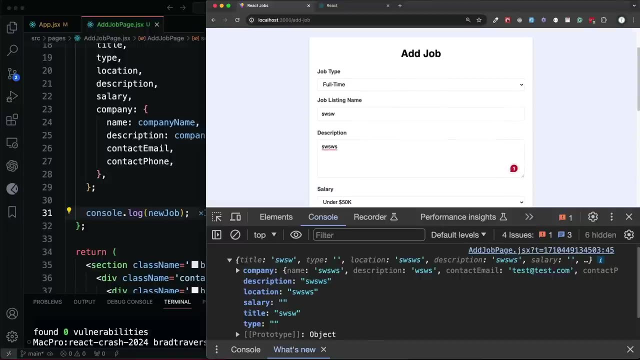 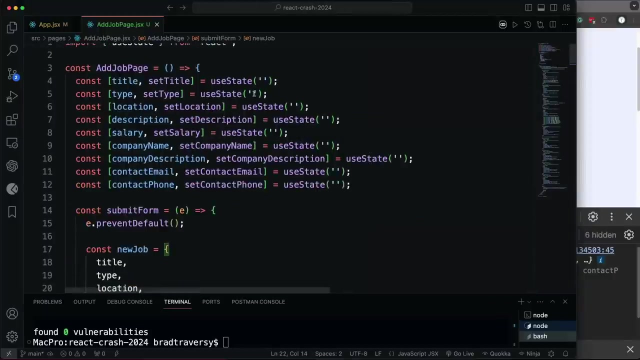 the defaults for salary. those should, those should show the default values, which they're not. they're blank, all right, so you know what we can do is set the defaults for those, since they're select lists for the type. for instance, let's say under what's the default? if we look at the 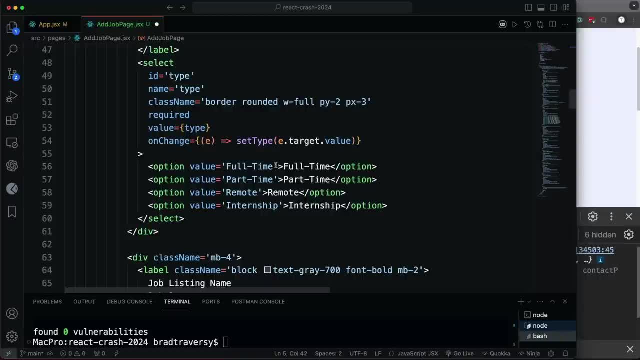 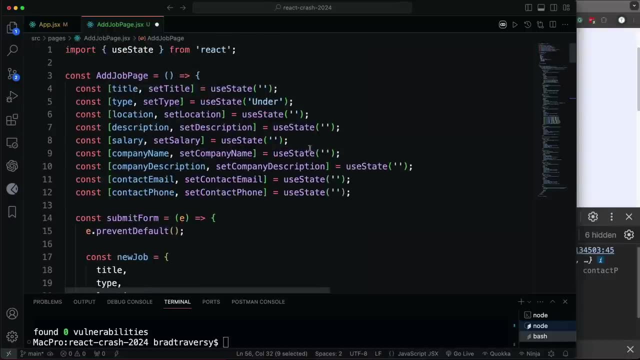 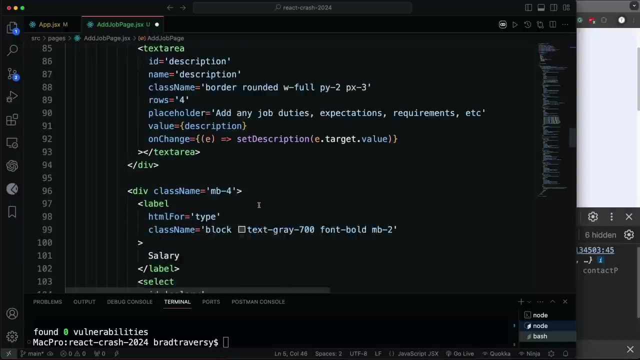 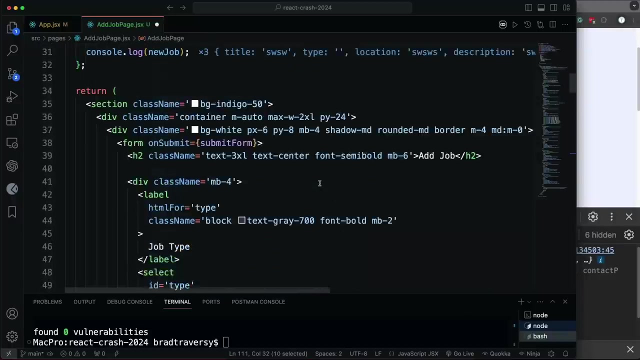 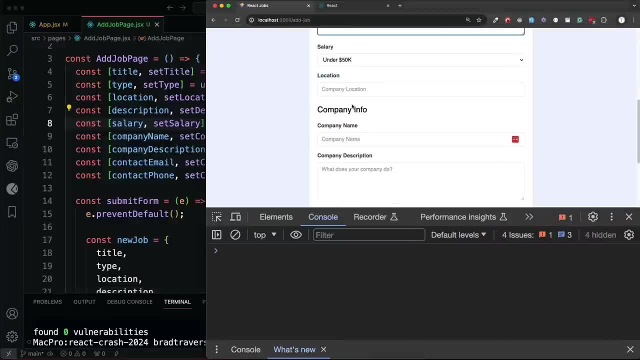 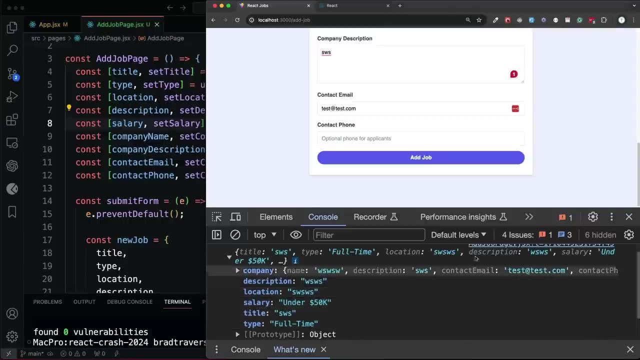 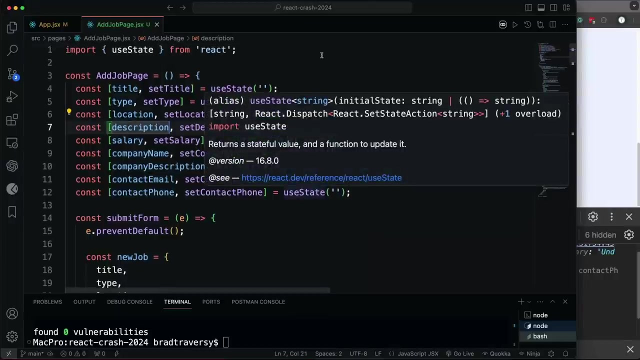 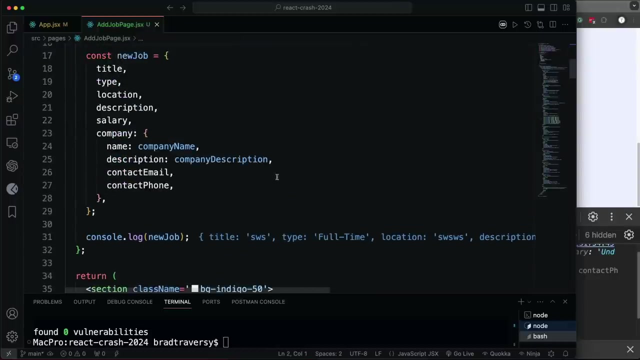 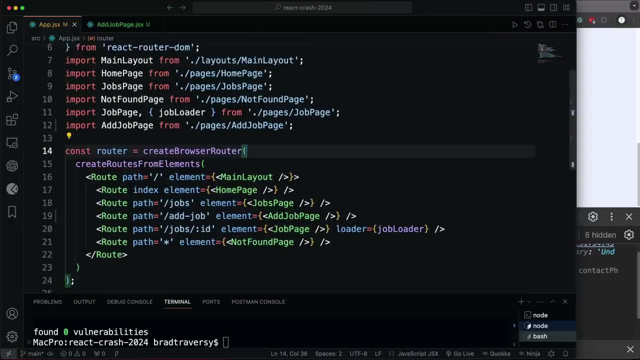 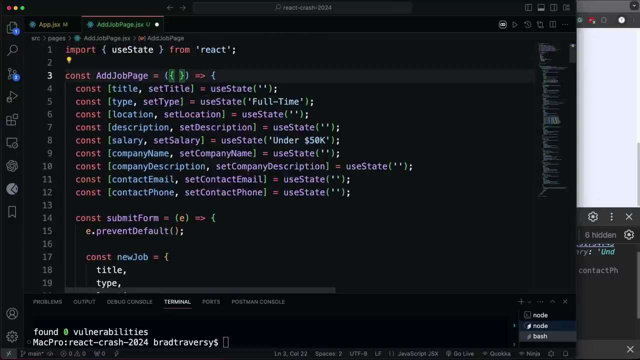 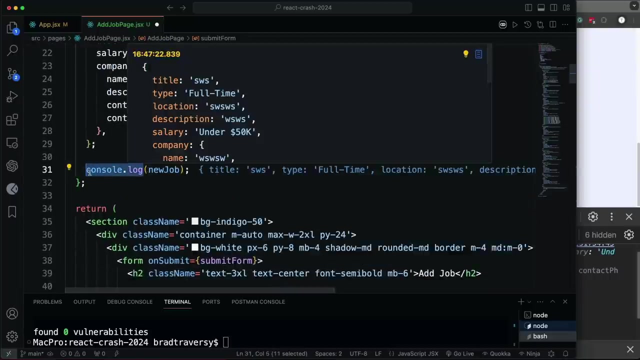 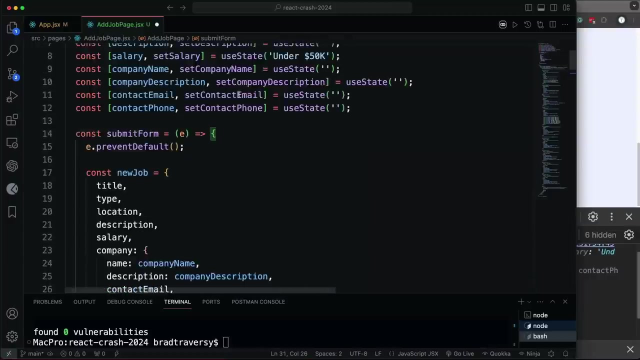 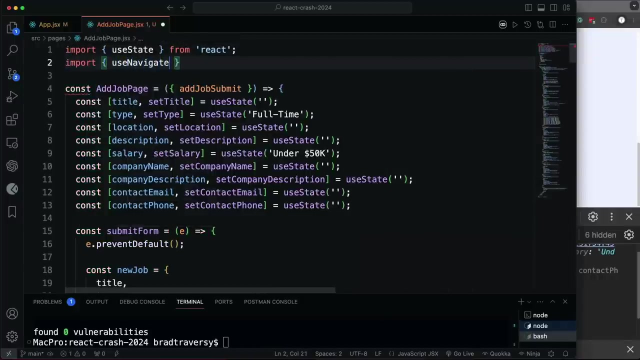 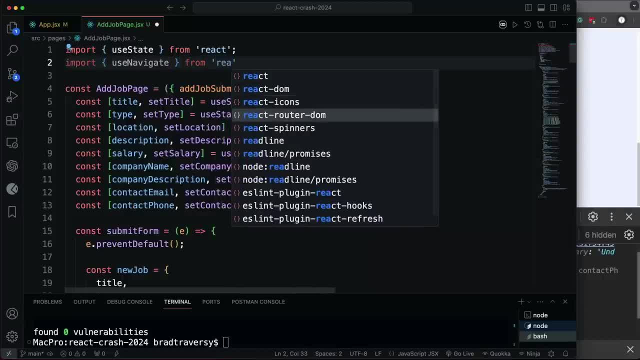 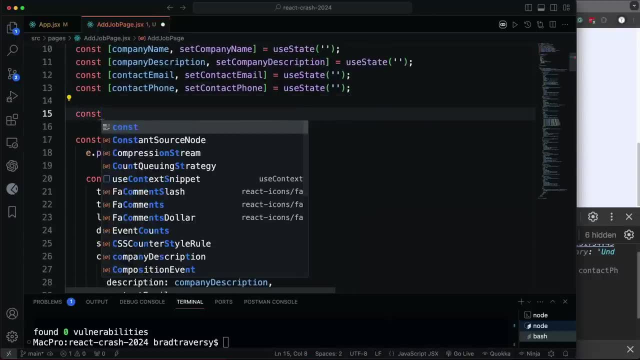 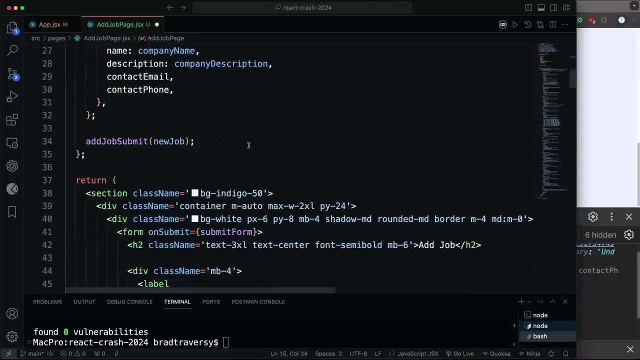 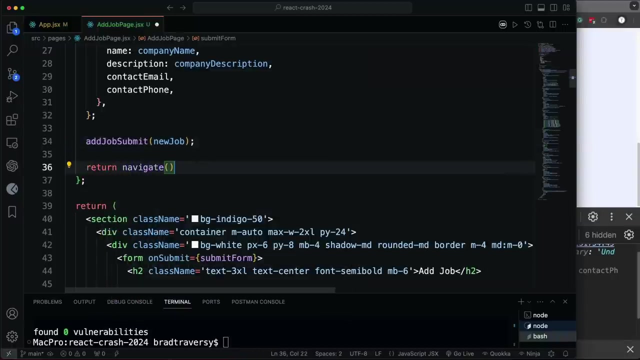 And that's going to be from React Router DOM. Now, to use this, we need to first initialize it. So I'm going to go right here below the state and just say: const navigate, Set that to use navigate. And then, after we submit, I'm just going to simply return navigate and then, where we wanted this to redirect, which is going to be slash jobs. 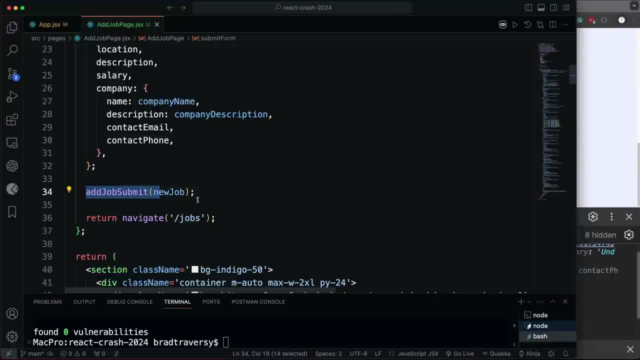 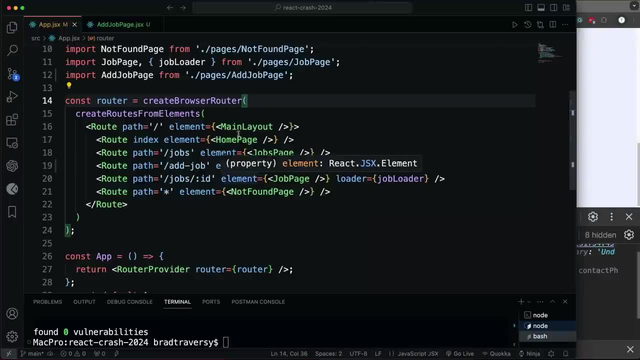 Okay, so this add job submit, this is being passed in now as a prop. So in our app let's go to the component which is the add job page And let's say add job submit, And what we'll do is set this to a function called add job. 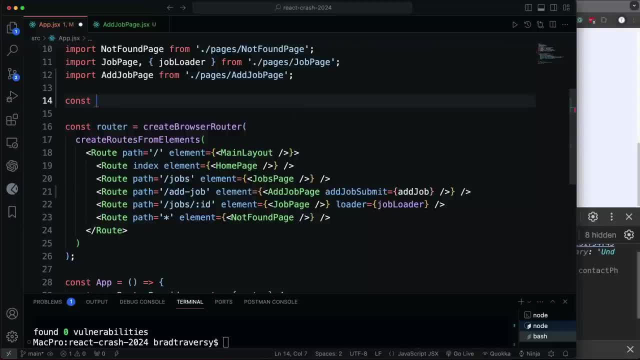 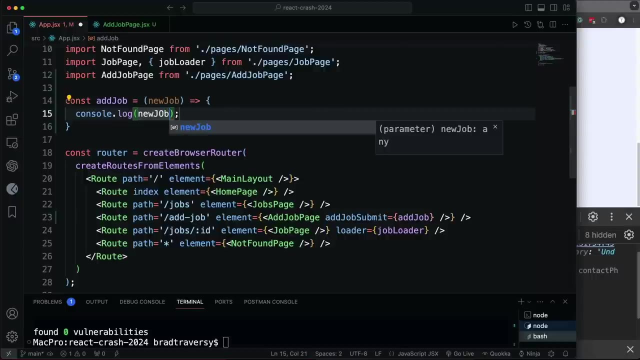 And then we can create that here. So we'll say const add job Okay, and that's going to take In the new job And just to make sure this is working, we'll do a console log of new job, All right. 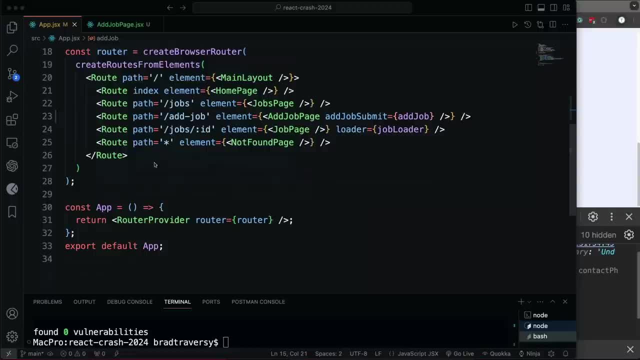 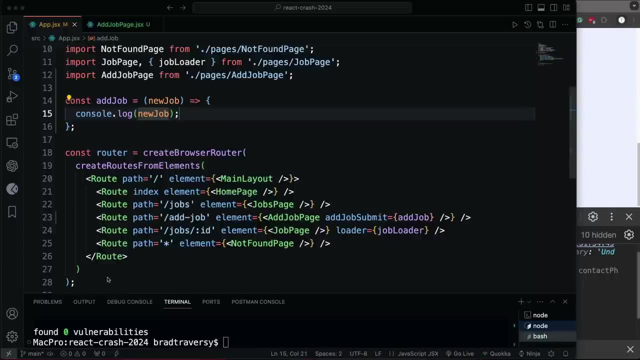 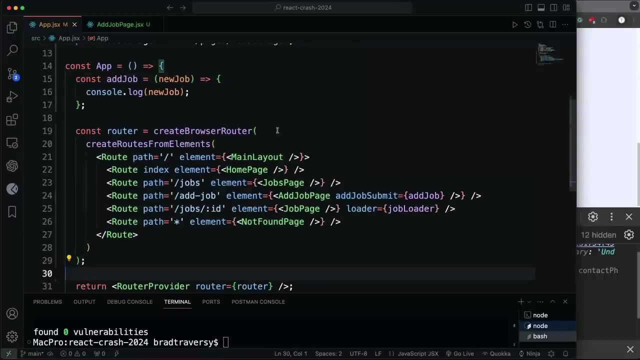 Actually, you know what This should be in the app component, And I'm going to move the router into that as well. Yeah, let's do that. Let's move this stuff Into the app component. I meant to put that in here to begin with. 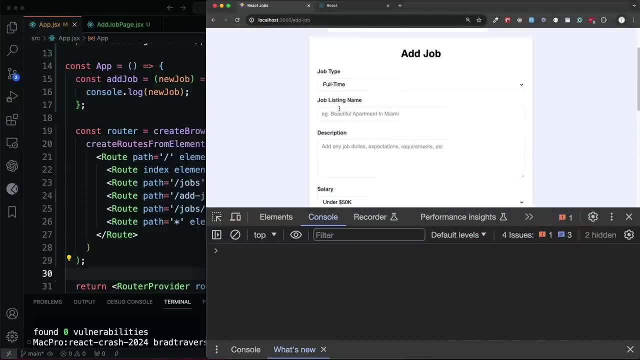 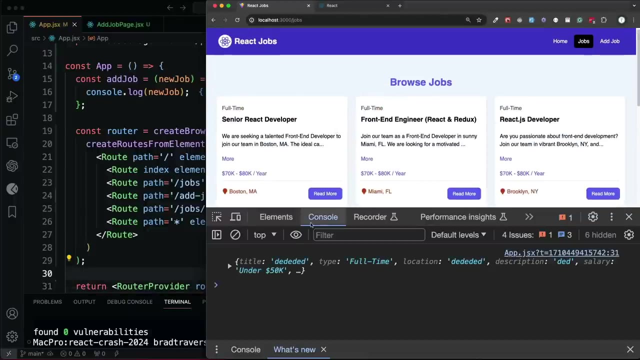 Okay, so that should still work. Now let's fill out this form again. Pain in the ass form. All right, so if I submit it, it redirected to the jobs page and it showed it in the console, So that means that it's calling this right. 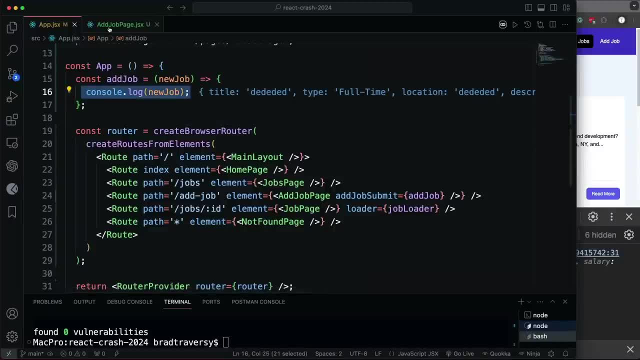 You can even see it in my editor Using console Ninja, And then it redirected us because of this. So if you want to call a function in a parent component, you can do that. You just pass it down like this, right? So I passed in this add job. 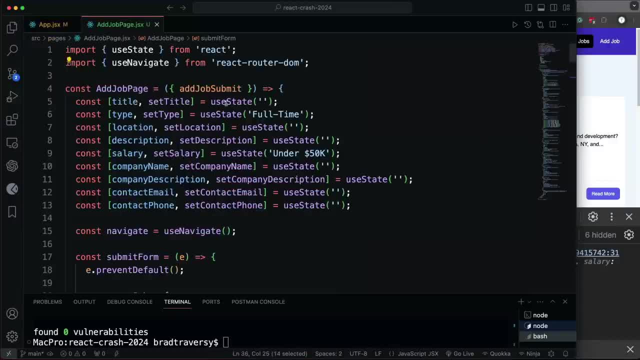 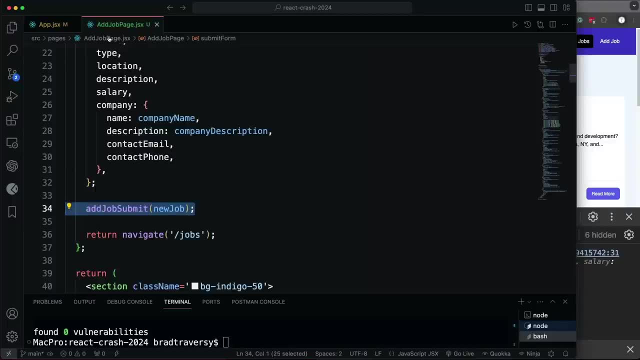 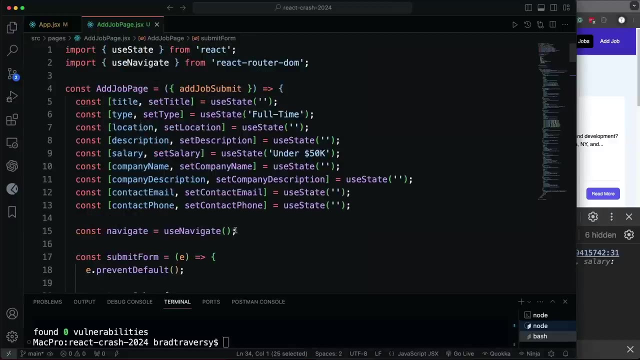 I pass that in as a value to add job submit. And then in this page I caught add job submit and I called it right here. So I mean that kind of confused me when I was learning this, because it's just a little weird to know. 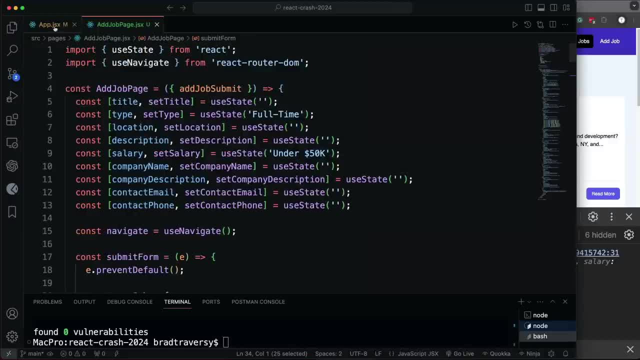 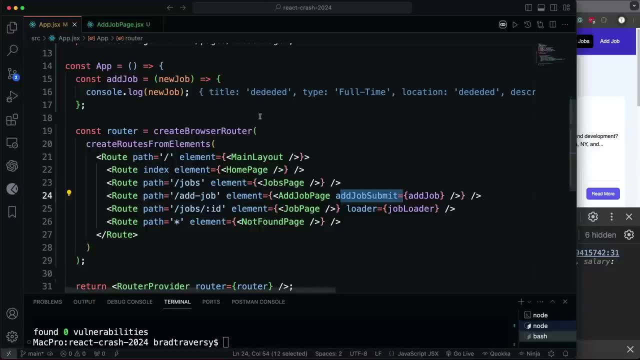 Am I passing this up? Am I passing it down? Like it's a little confusing, At least it was to me. But just know, you can pass in a function and you can call that function and whatever you put here, So add job, for instance, is going to get fired off whenever you fire this off in this component or this page. 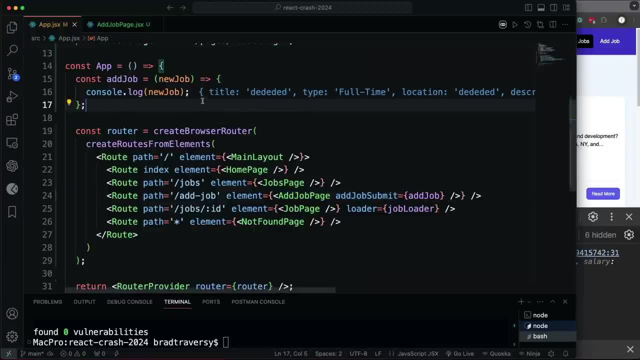 So Now that we've done that, we should be able to to make the request and actually add the job. So let's get rid of the console log and let's say, cons res, set that to a weight, a weight fetch, which means we have to make this asynchronous. 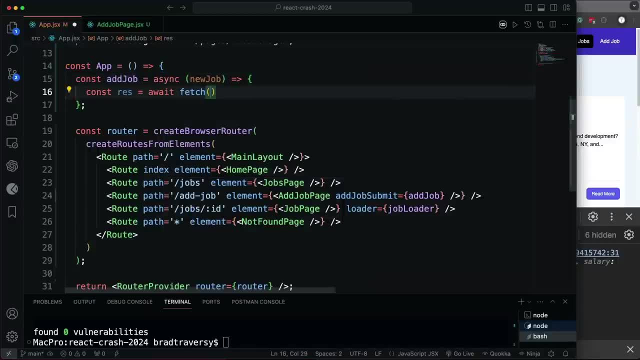 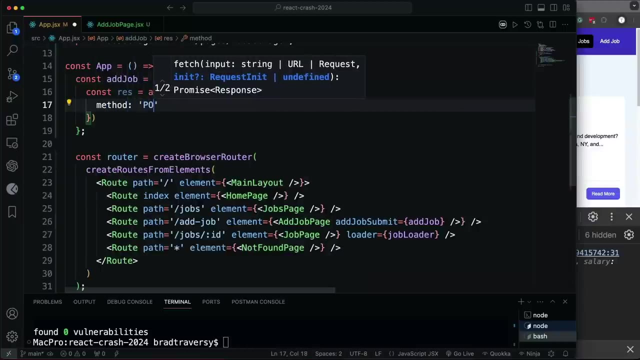 So a sync, And then we're going to fetch, let's say, slash API, slash jobs, But this is going to be a post request, So we need to pass in a second Object and set the method to post, OK, And then we also want to set the headers. 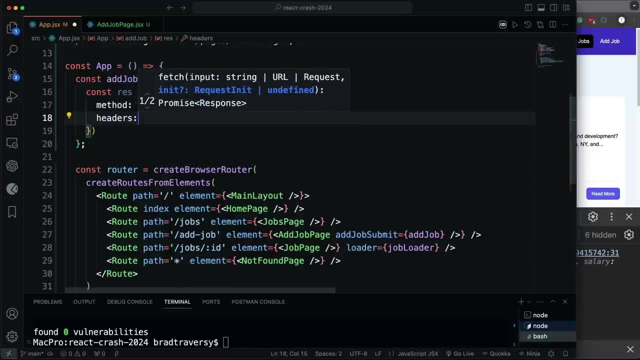 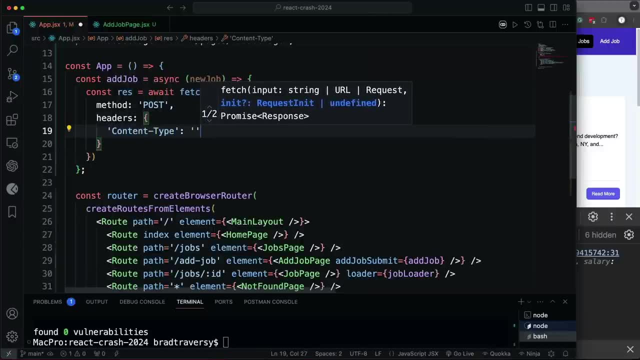 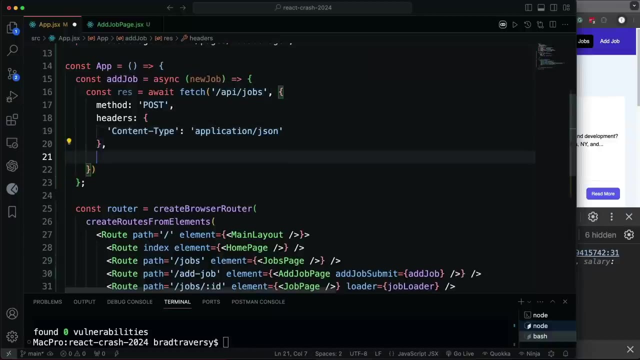 Oops Headers And that's going to be an object And we want to specify the content type. So content dash type, which is going to be application slash, Jason, And then the data itself is going to go under the headers in the 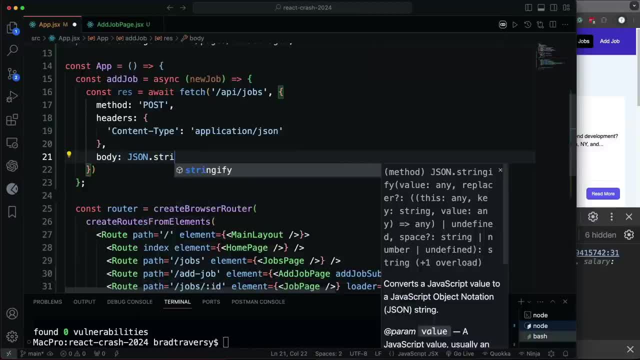 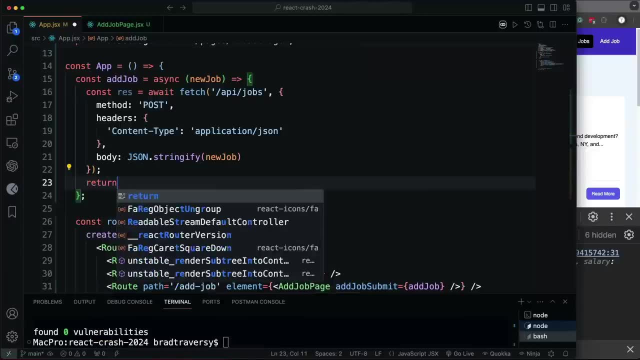 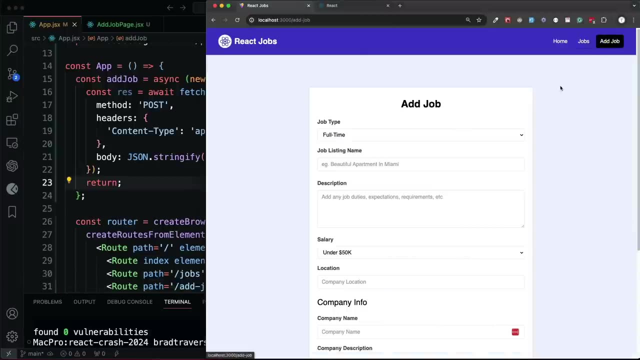 Body. We're going to wrap it in Jason dot string of fi And pass in that new job And then after that we'll just return. So let's save that and then Let's come over here, Go to add job. 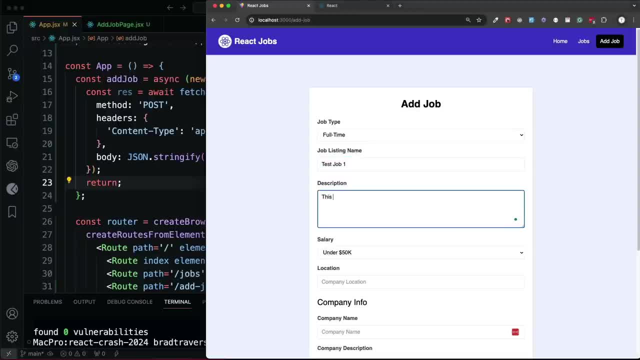 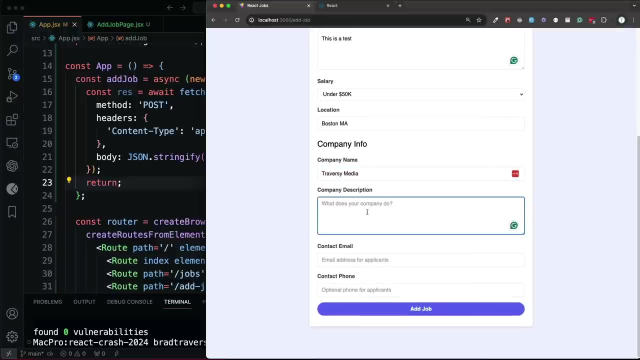 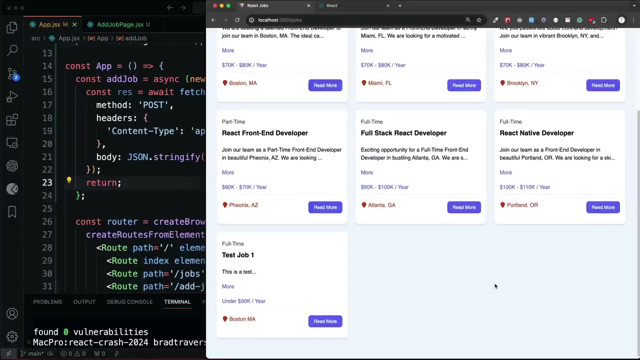 We'll just say: test job one: This is a test Test. Job One: This is a test Test One. Test Test Company name: This is an awesome company, All right. So we're going to go ahead and click add job and it redirect us to the job page and we have our new job. 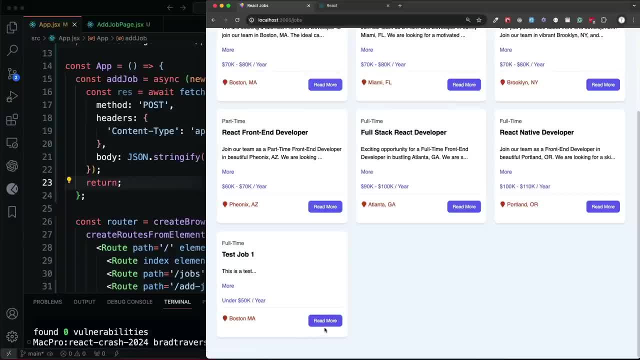 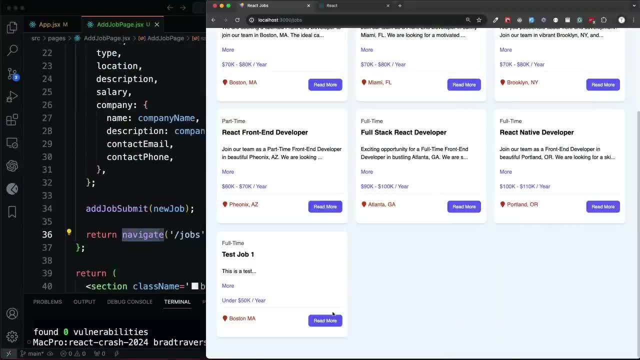 All right. So it made the post request And we just returned from this function. but we redirected in this one to jobs And if I click read more, it takes me to the single page for that new job. So now let's do the delete. 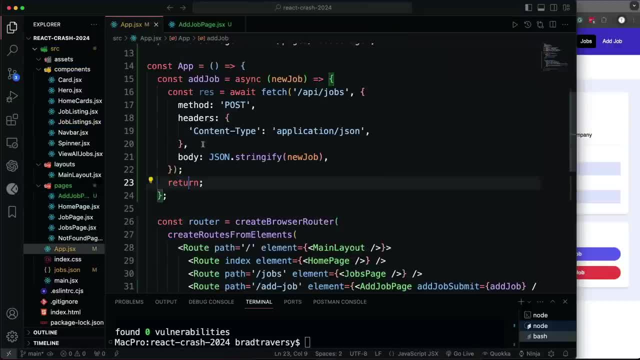 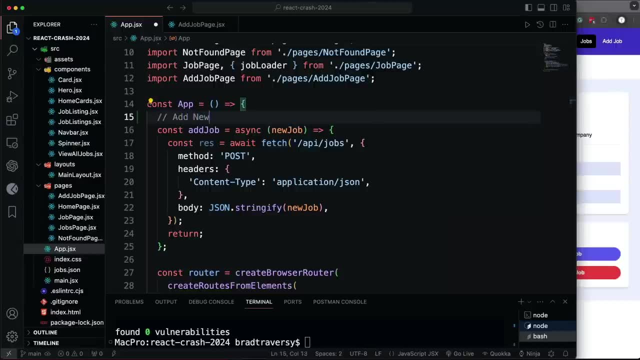 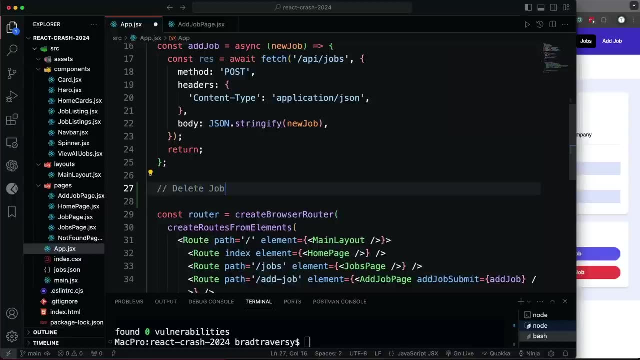 So I want to be able to click this delete button And again I want the actual request function to be in the main app component. So let's put a comment here, We'll say add new job And then underneath that add, let's say delete job. 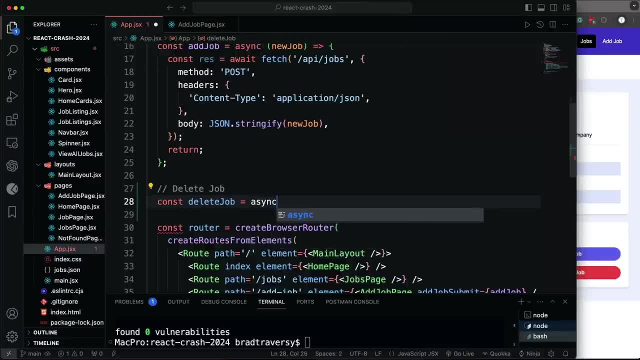 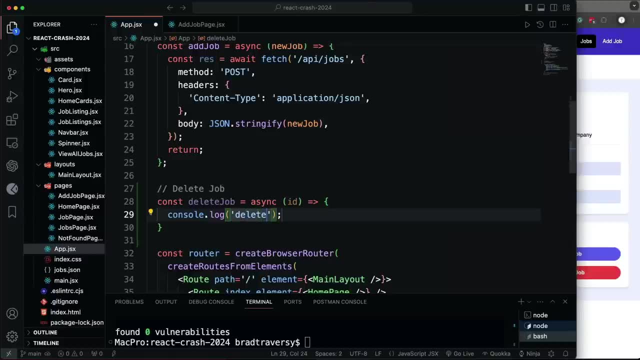 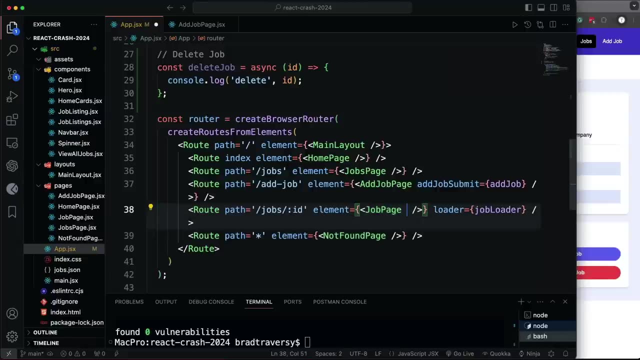 Call this delete job And it's going to be a sync. It's going to take in an ID because we need to know which one to delete And then for now we'll do a console log of delete and the ID And then that's going to get passed into the single job page right here as a prop. 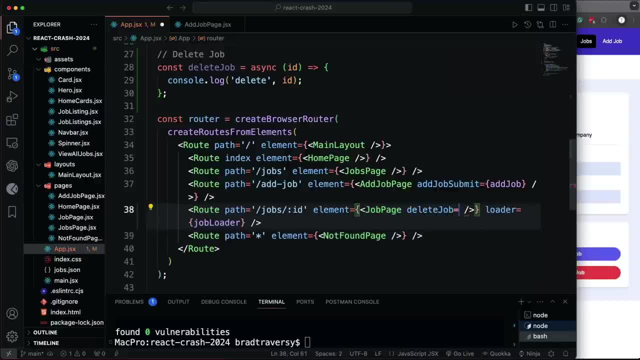 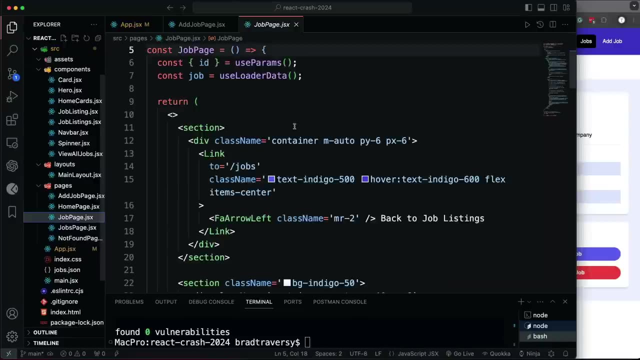 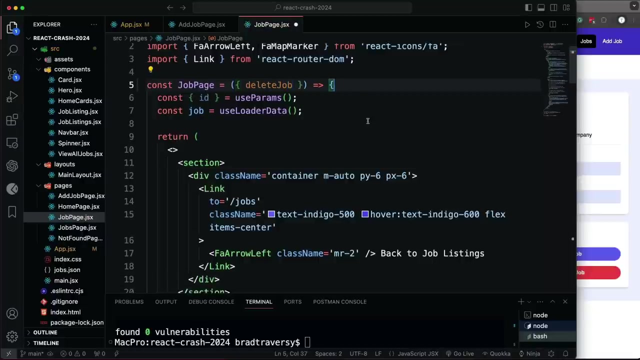 So we'll say delete job, Set that to, And then we can pass that in as a prop to the job page. So right here I'll say delete job, And then on the button, the bottom here, we have this button. 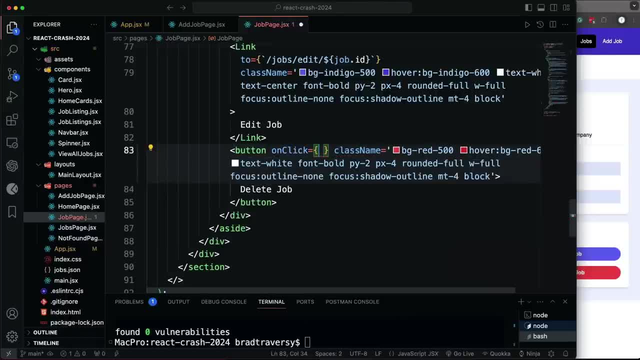 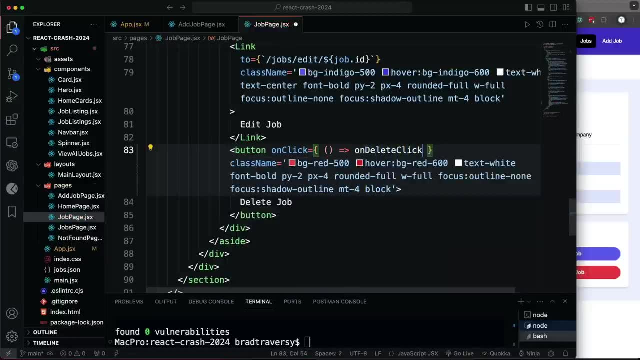 And let's say, on click, And we're going to set that to A function, And then we'll call another function called on delete click, And then pass in the jobid, Okay, And then this: on delete click, we're going to put that up here. 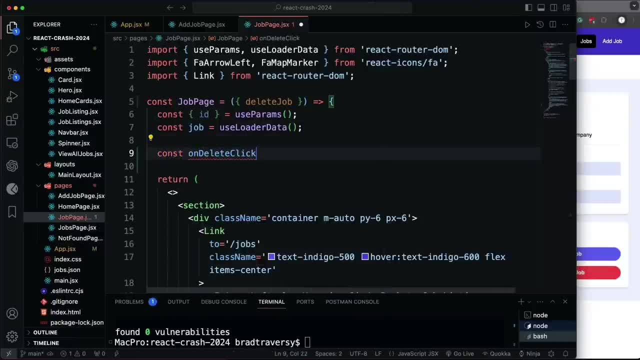 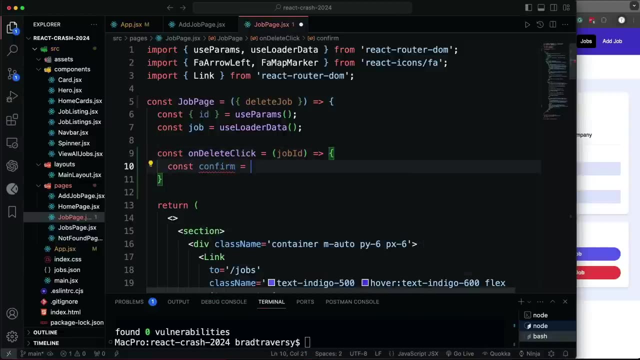 Const on delete, click And let's pass in. We get the job ID getting passed in here And I want to Confirmation since it's a delete. So I'll say const confirm. Set that to window dot confirm And we'll say: are you sure? 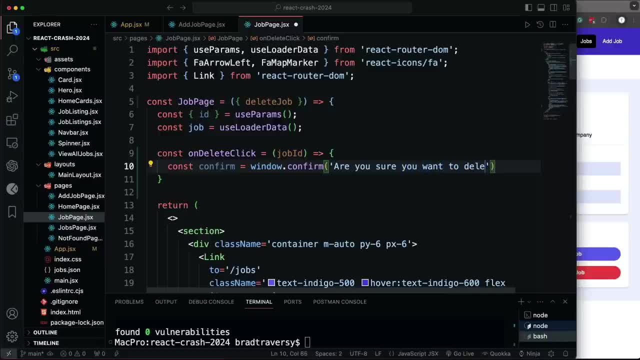 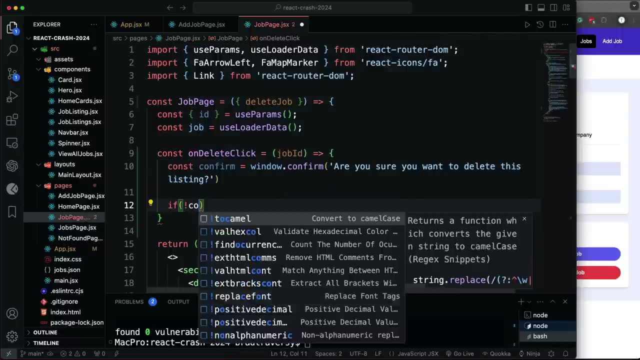 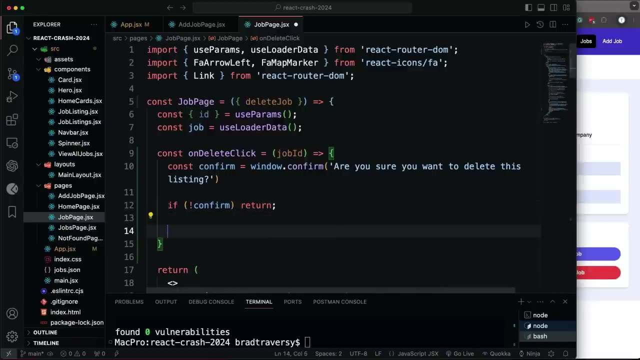 Are you sure you want to delete this listing? Okay, And then let's say, if not confirm, then we want to just return. If we don't, If we do confirm, then we're going to call that delete job that we passed in. 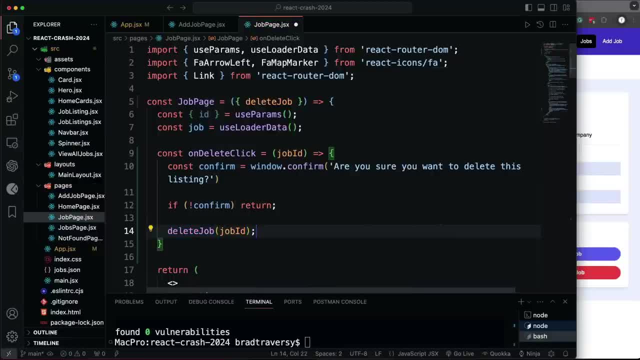 And we want to pass in the job ID. Okay, And then I'm going to redirect. So in order to do that, we have to bring in use navigate. So let's see That's going to come in from react router DOM. 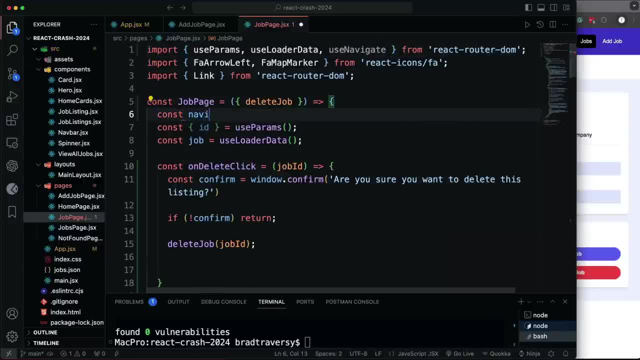 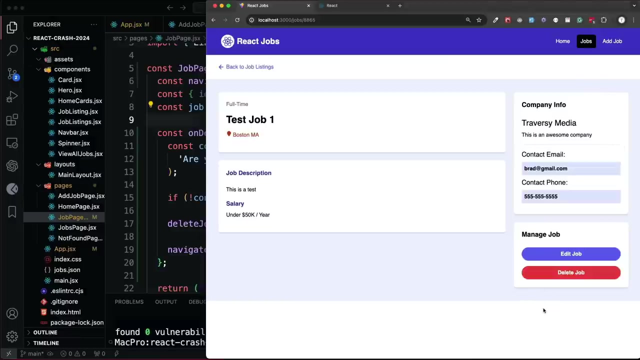 And then we have to initialize it, So const, And then we can just navigate to slash jobs. All right, Now let's just click on it And what should happen is it should redirect us and it should show the ID in the console. 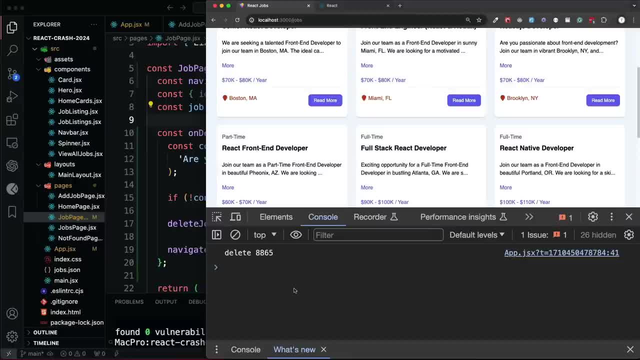 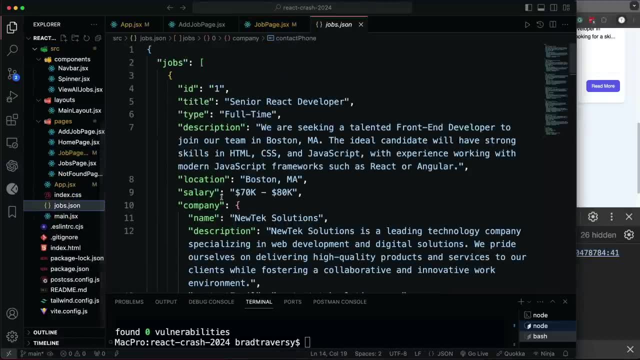 So click it, Say okay, Redirects And shows the ID. Is that the ID? Let's see Jobs JSON. So it should have added my test to the file. Yeah, right here. So that is the ID for the test job. 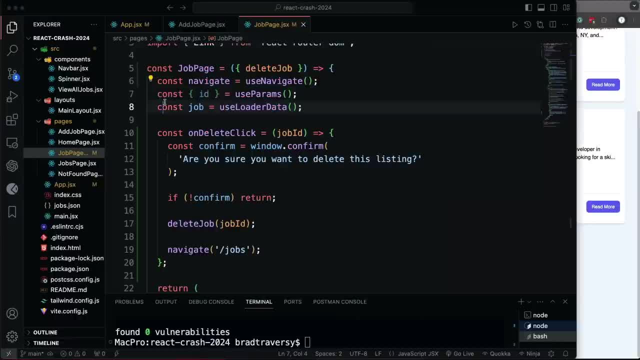 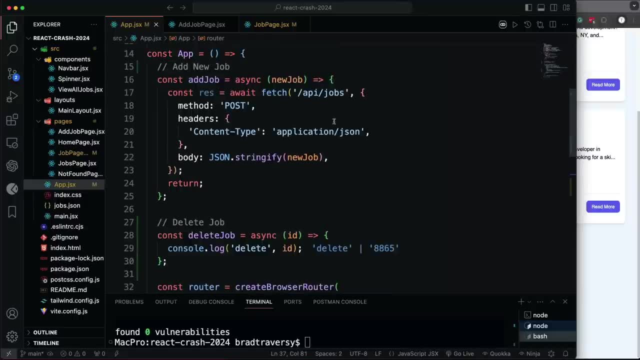 Good. So now we want to make the actual request to the API. So that's going to go right here. So we'll have all of our requests in. you know, nice and neat in this file. Now this is for a small application. 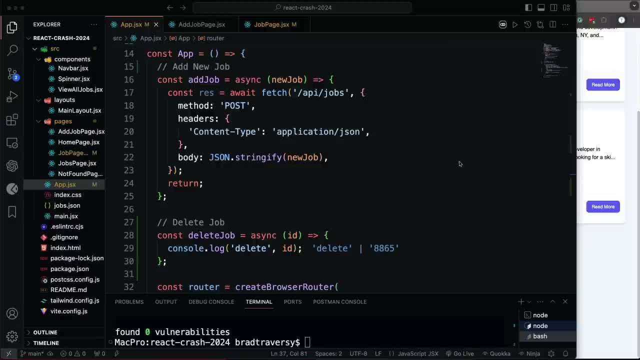 You could use content, The context API, which you know you would have it, oh, in a context file. you could use Redux or some other state manager, but this is such a small application We don't need that. So I'm going to just grab this from the add job and then put that here. 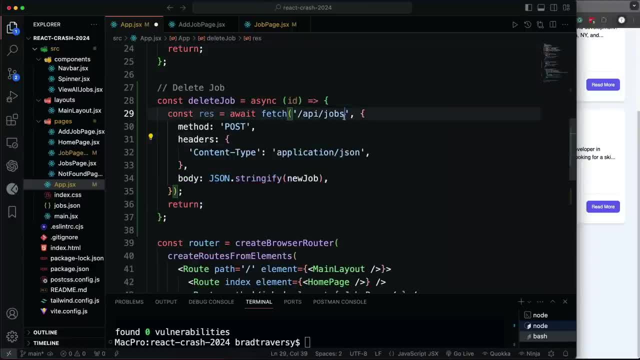 Okay, We're going to fetch API jobs. Now we have the ID coming in, So let's make this. make these back ticks and say Slash, and then the ID method is going to be delete. Okay, Headers, Get rid of that. 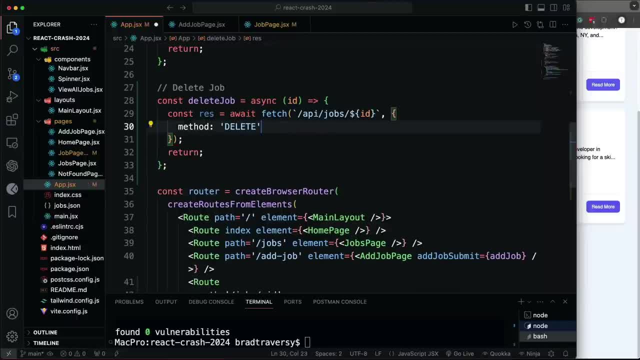 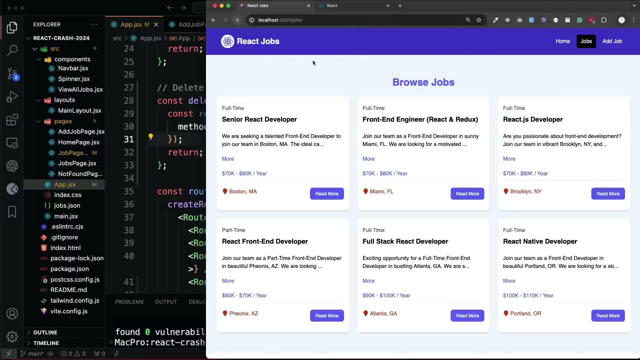 And get rid of the body. And yeah, I mean that should do it. Let's try that. So, to test job one: delete, Are you sure? Okay, And now it's gone. If I reload, it's gone. 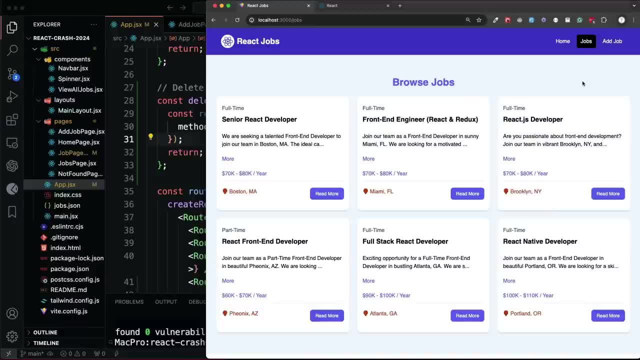 And it should be gone from that JSON file as well, And again you would be working with an actual back end. So that leaves us with the edit. Now, before we get to that, I want- even though it redirected us, I wanted to show some proof that we deleted the job. 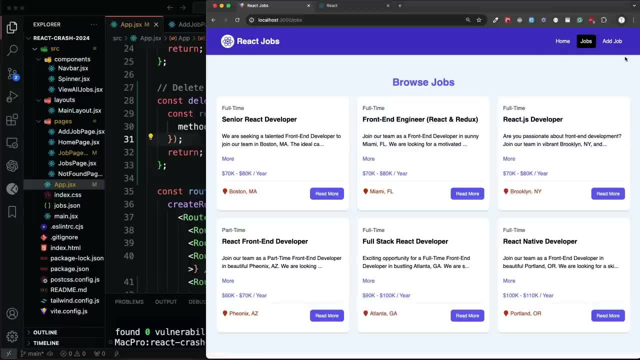 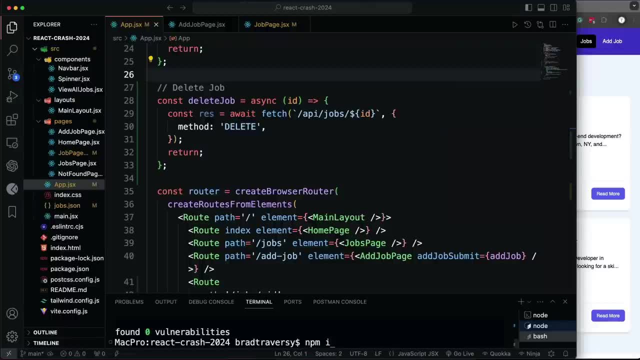 So we're going to use a package called React Toastify which will show a little toast notification Wherever we want. I want to put it, So let's install that. I know this is not you know this is a separate package, but it's something that you'll commonly- you'll probably commonly- use. 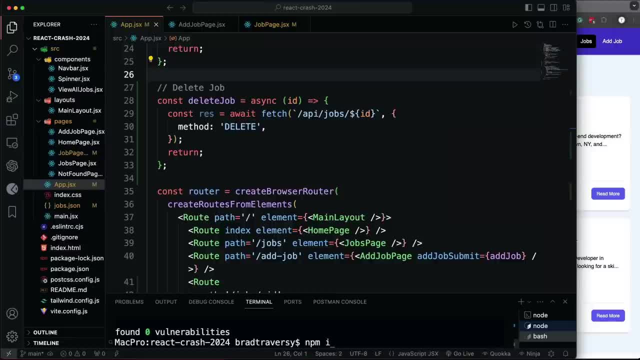 I use it all the time: React icons, React Toastify, React Spinner- These are things that I use in just about every project. So let's say React dash Toastify. Now, we have to set this up. We need to have 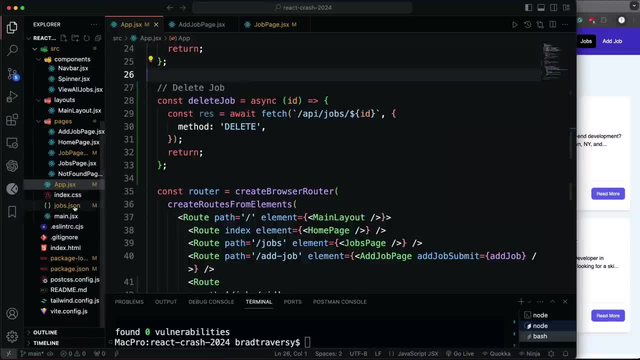 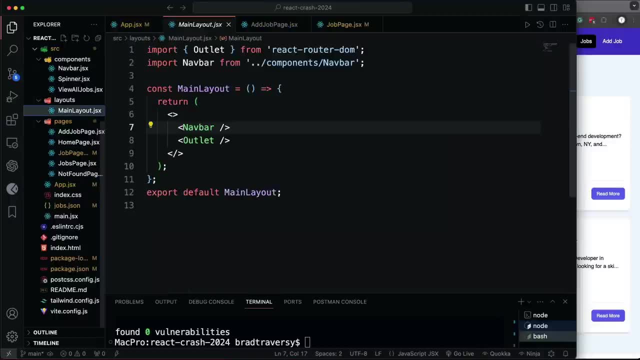 Um, Let's see In our layout is where we want to put this, so that we're a, so we have a, basically like a wrapper for the layout to output. So if we go to our main layout, we're going to import from here. 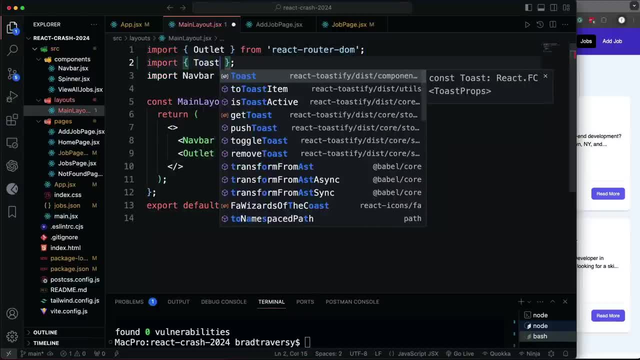 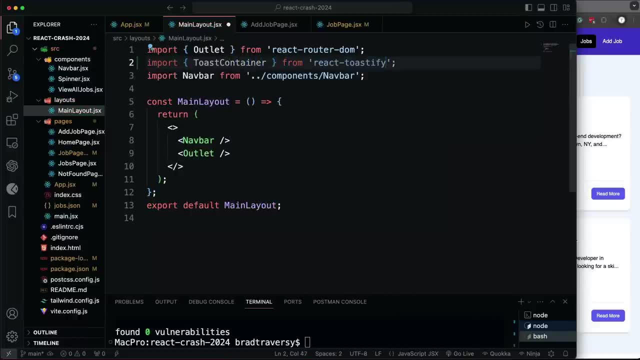 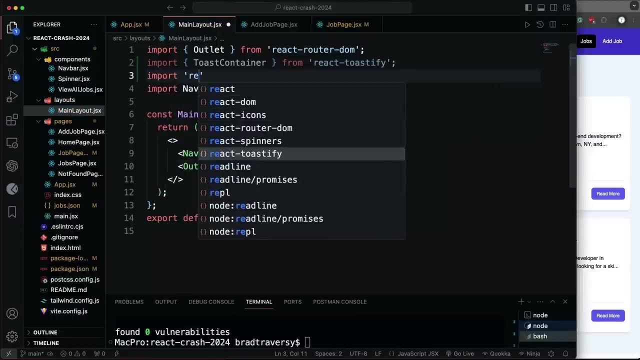 We're going to import the toast container, So toast container that's going to be from React Toastify, and then there's also a CSS file that we need to import, So that's going to be React Toastify, and then slash dist. slash- React Toastify dot CSS, like that: 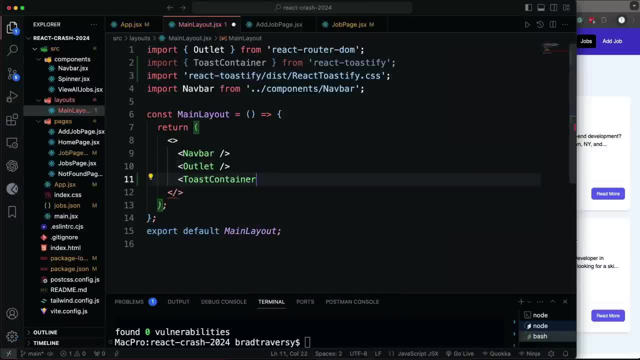 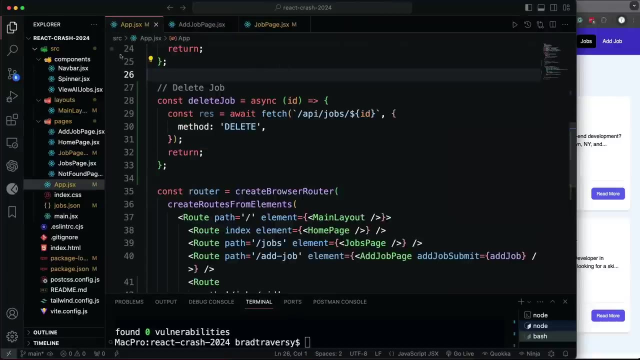 And in the container. you can pretty much put that anywhere. It's positioned absolute, so it'll. it should be up in the corner, but you can change the positioning with attributes or props if you want. But let's save that Now. what we can do is when we delete. 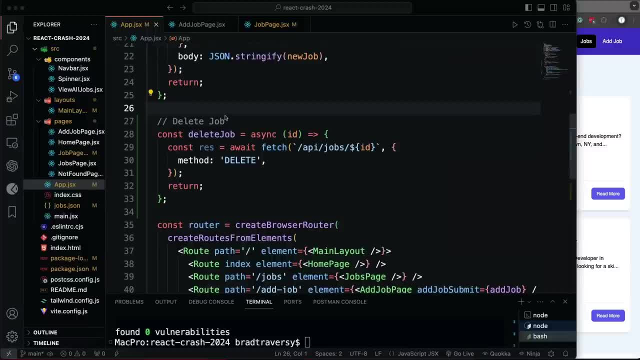 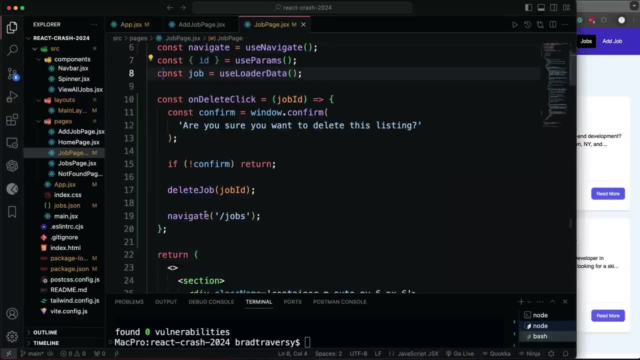 Let's see where should we put this. We're going to put this in. We could do it here, But I think I'm going to put it in the job page right before we redirect. So wherever you want to use a toast, you simply import. 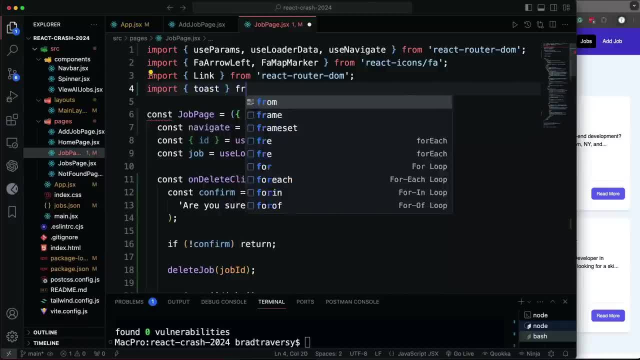 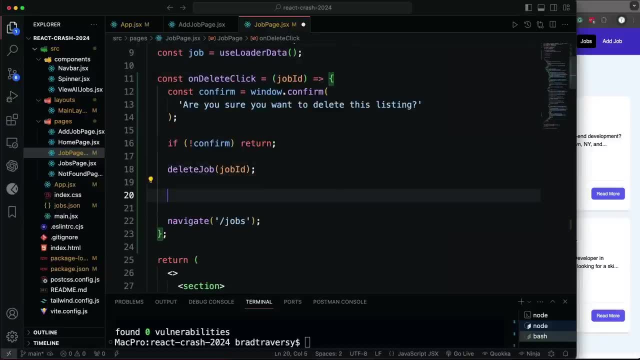 Toast From React Toastify and then, where we want to call it, Let's go right after we delete and say toast dot success. So you can do success or error and let's say job Deleted Successfully, All right, So now let's try it again. 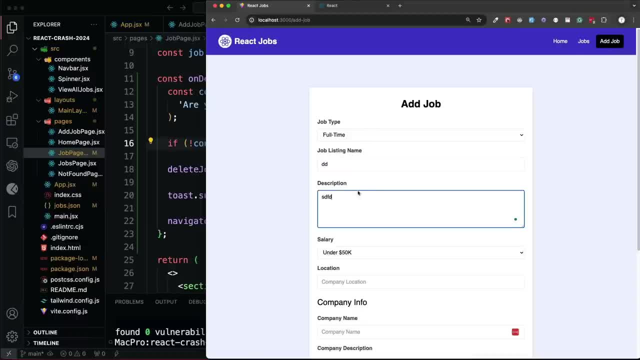 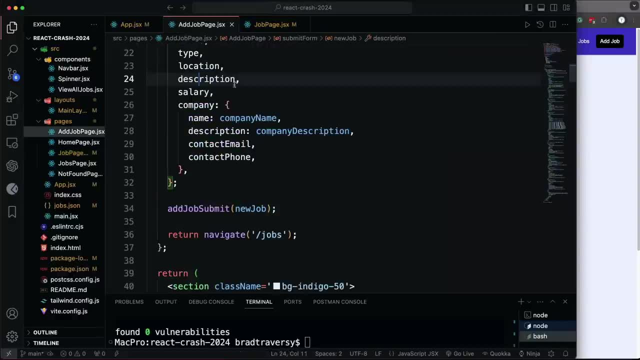 I'm not going to delete any of these, I'm just going to create another dummy job. Actually, before we do that, let's do a toast where we we added as well, So we'll import this into the ad page. And then, right before we redirect here, let's say: 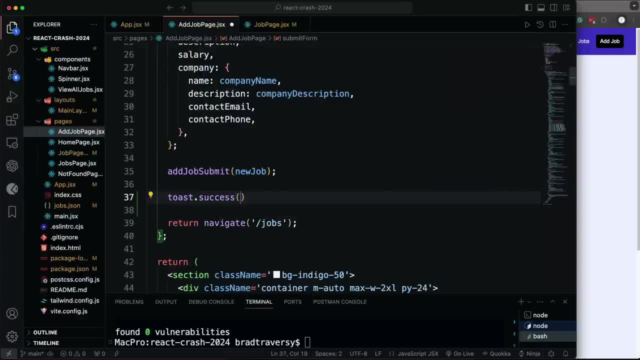 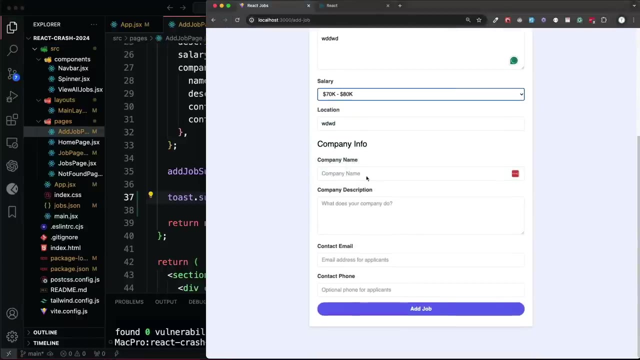 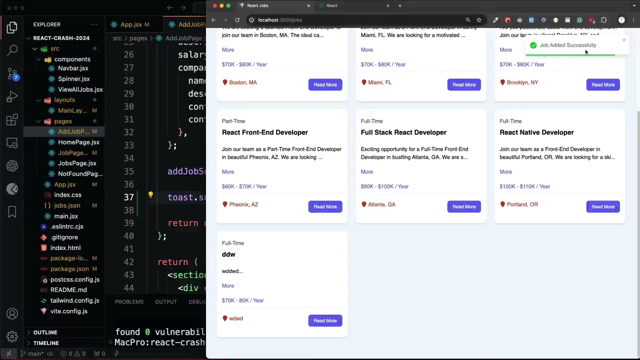 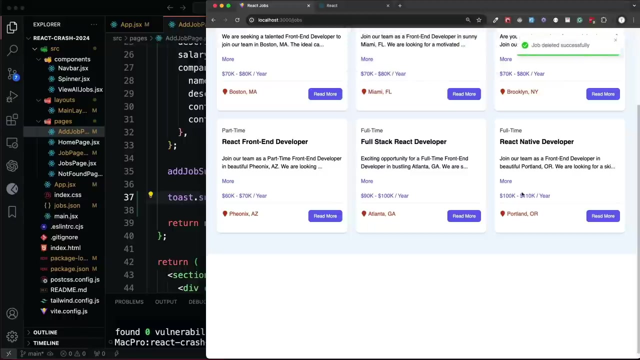 Toast dot Success And we'll say: job added Successfully. Okay, So now Let's just put whatever, just some junk in here, Add There, we go, Job added successfully. And then if I delete it, Job deleted successfully. 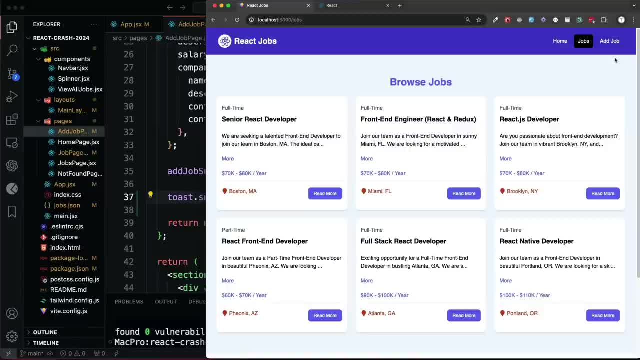 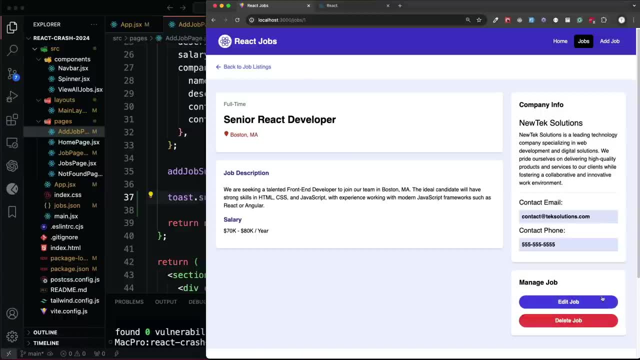 And you can do toast dot error if you wanted to show an error for some reason. All right, cool. So now we're going to do the the edit. Okay, we have this edit job button. Let's create the edit job page. 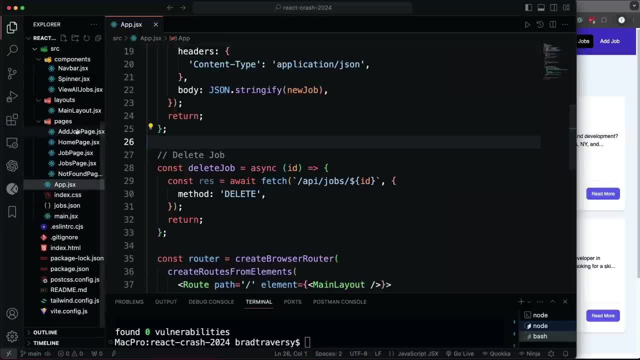 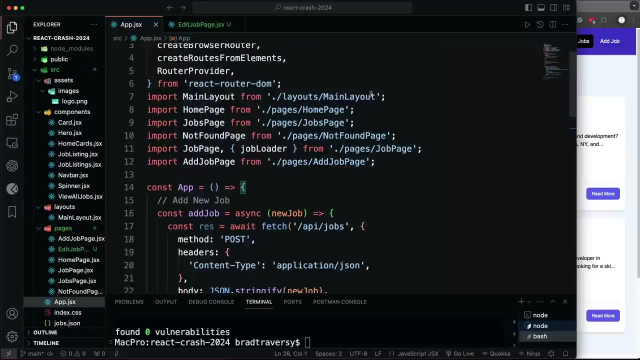 You can close this stuff up. Leave the app JSX open and in pages Let's say edit job page And then let's add the route. So in our app JSX Let's import Edit job page And let's see we're gonna. 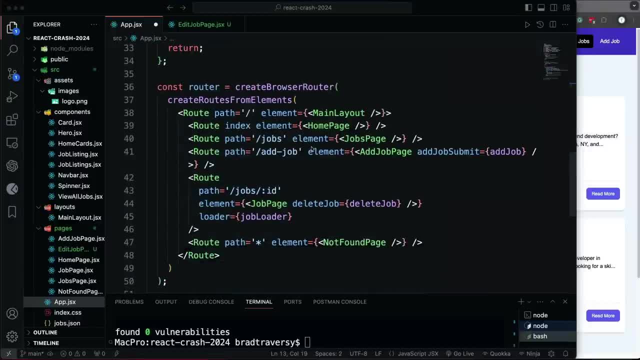 Add this. So with the edit page, I'm actually going to use the job loader, because in order to edit, we have to fetch the data right And we already have this job loader right. We have to do that loader, so we might as well use that. So I'm actually going to copy this route for the job. 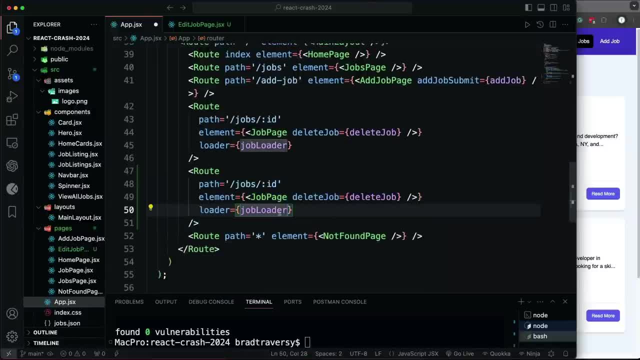 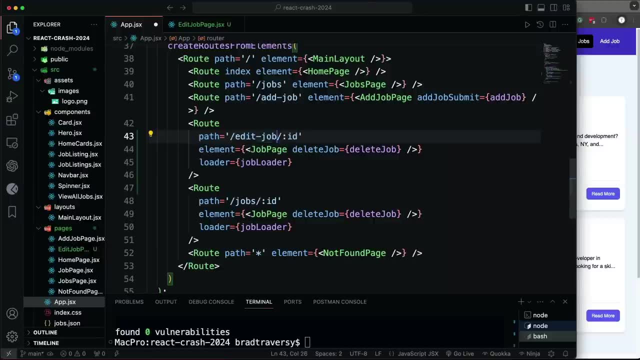 page. Copy that down. I'm going to change the route. Let's do this one here. We're going to change it to edit dash job and then slash and then the ID, and change this to edit job page and we can get rid of this delete job and, just like we did with the job page, we're going to 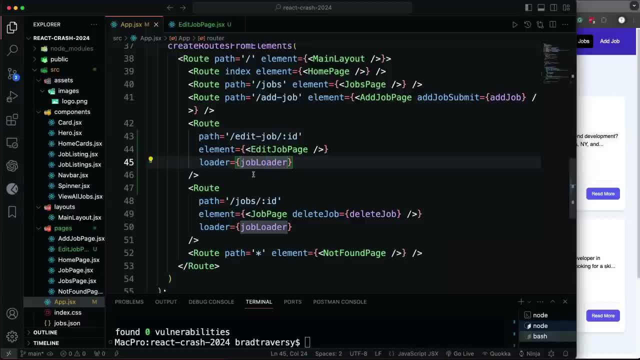 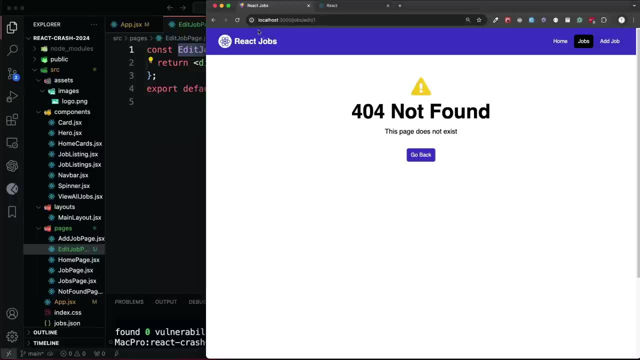 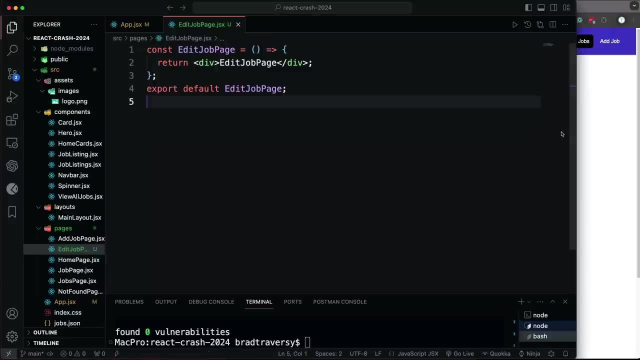 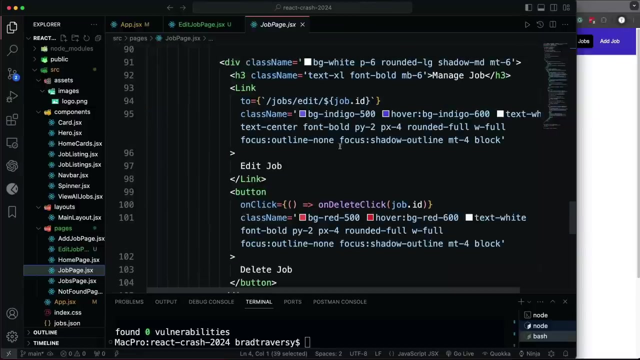 pass in the job loader. that'll give us access to the data, So let's save that Now. if we click on the edit button, it should take us wait a minute. that goes to job slash edit. I'm actually going to change that. So in the job page where we have the edit button, I'm going to change that. 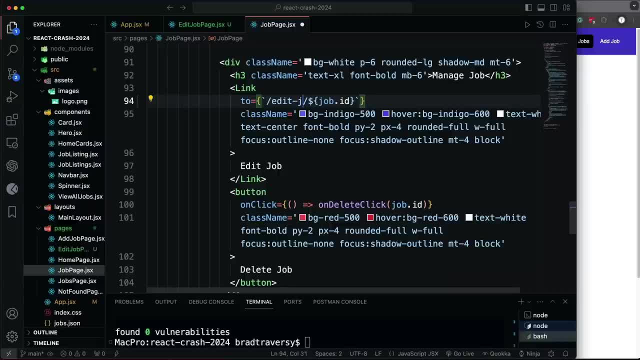 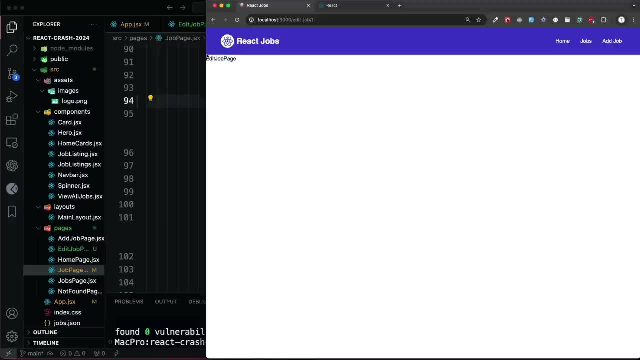 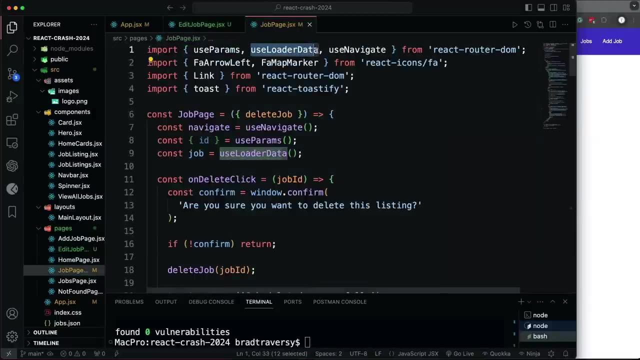 to edit dash dot job and then the ID. So edit, There we go. So now we're seeing the page And since we passed that loader and we can do the same thing that we did in the job page, We can bring in use loader data. 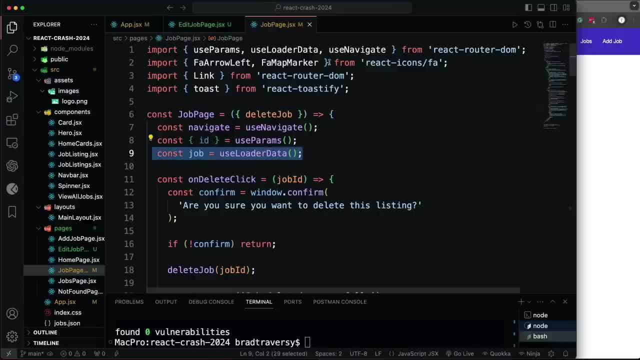 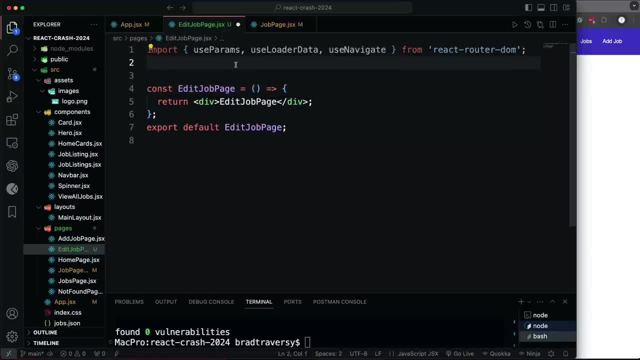 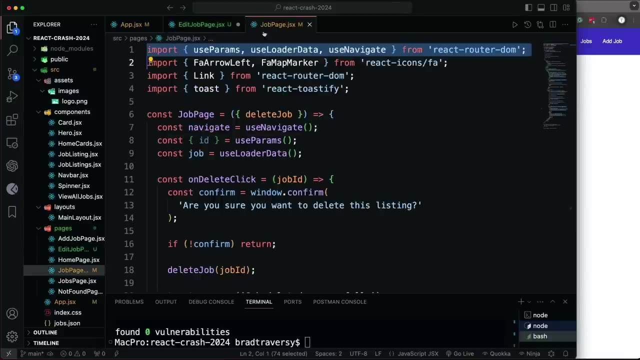 and then simply do this and we should have access to the job for that page. So I'm going to grab that and let's see: Do we need this stuff? Yeah, we'll just leave it for now, And then let's do this. So use loader data And go like that, And then I'm just 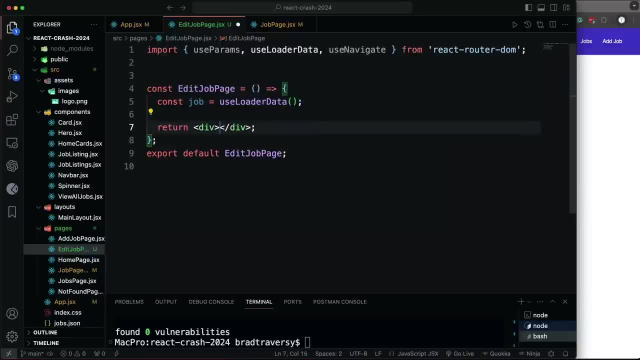 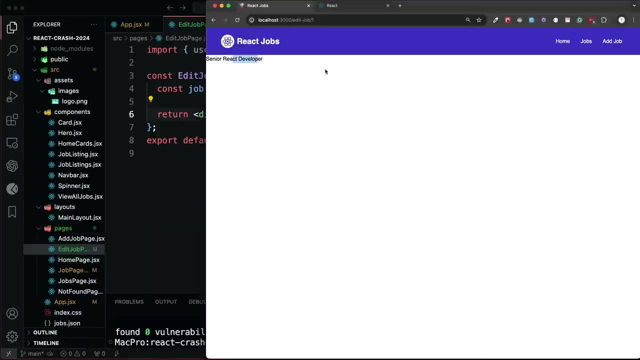 going to do. actually, what I'll do is output here and we should be able to get the job dot title. So let's go back and there we go, So we're getting the data for whatever job we're trying to edit. So ReactJS. 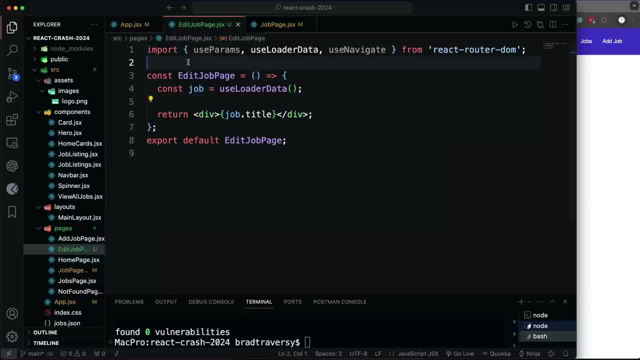 developer: Click on edit job. ReactJS developer. So I think that the data loader feature in React router is really cool for stuff like this. Now we need the form and we need to fill the form with existing data, So why don't we copy the entire? add form. So add job page. Let's grab the entire. 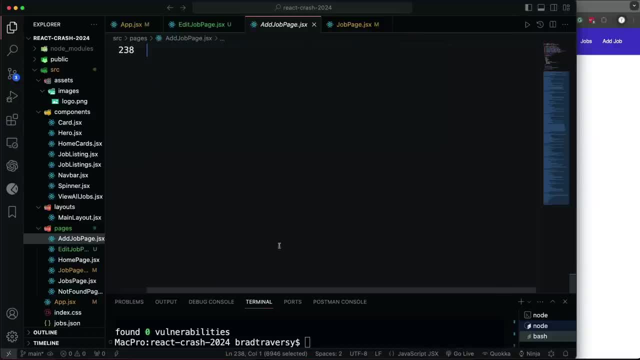 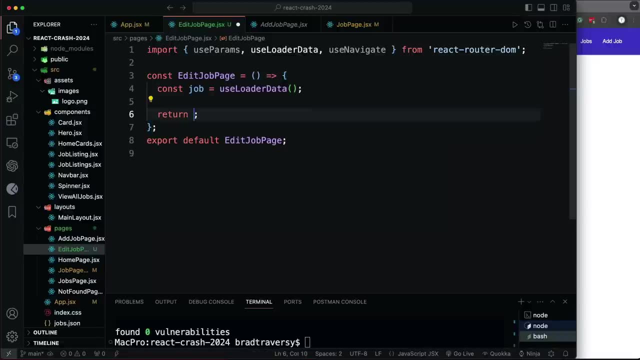 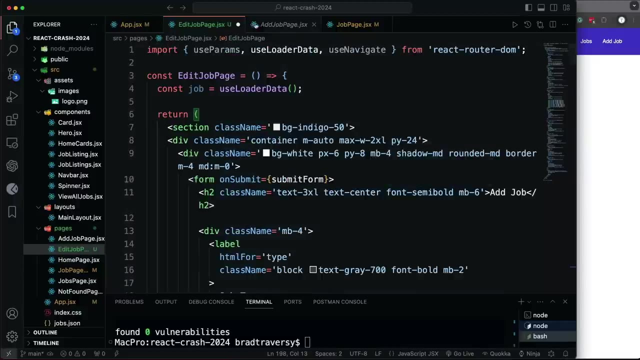 section. Okay, so we're going to grab that and then go to the edit job page And then let's return in parentheses, Paste that in, and we're going to do the same thing where we have the state, So we can also copy this, all this stuff, right here and put that in. Put that right here. 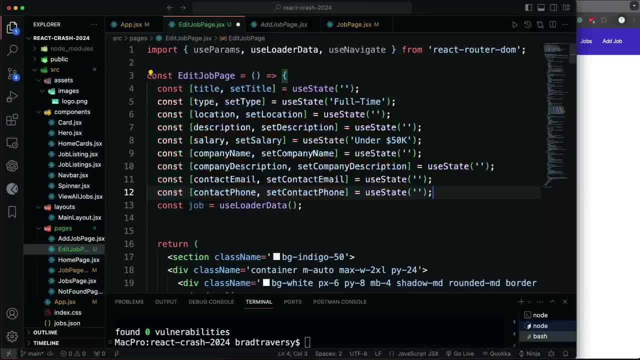 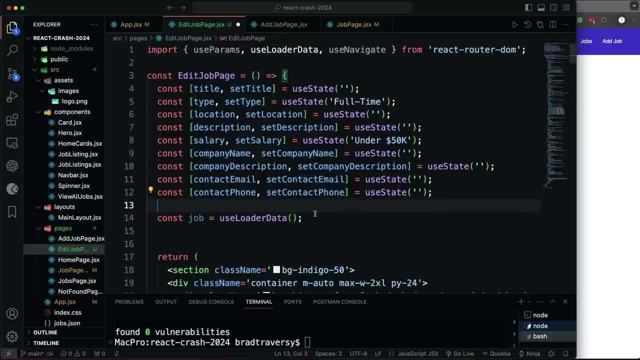 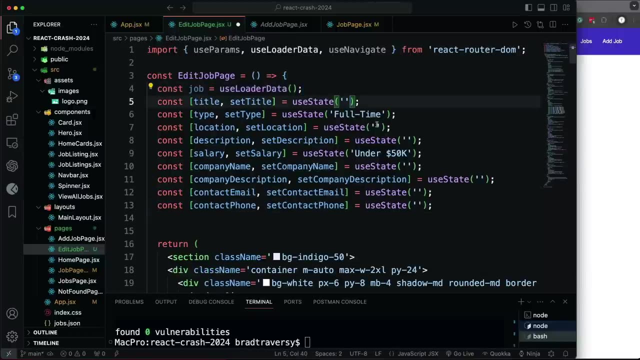 Actually, let's, let's post it in here, the state above that, all right, and then what we can do is put the default- actually no, we want this above the state because I want to add the defaults from this job. so, for instance, the title, let's say job dot title. so for the type, let's 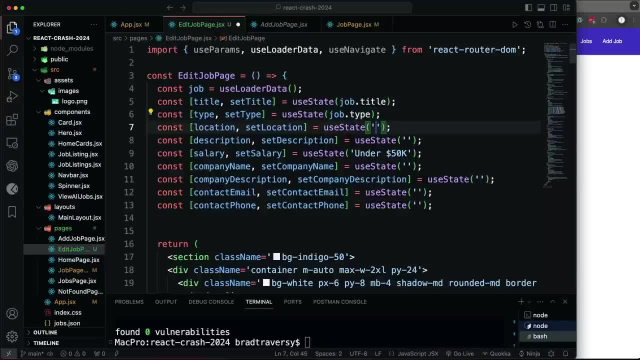 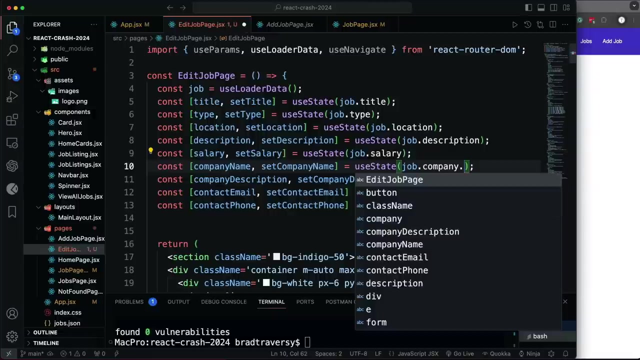 say job dot type, and this will fill, this will add the fields in the form, add the data in the form. so job dot location. this is going to be job dot description, job dot salary, job dot, and this will be company dot. is it company? yeah, I think. 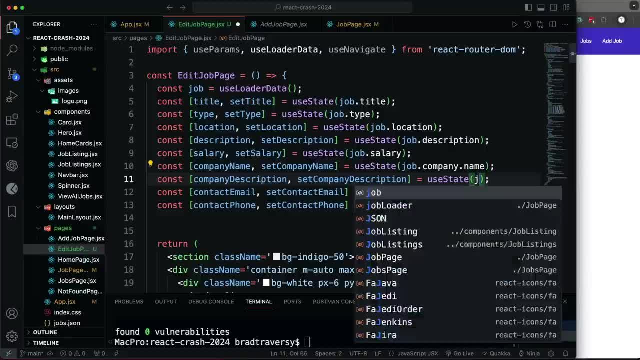 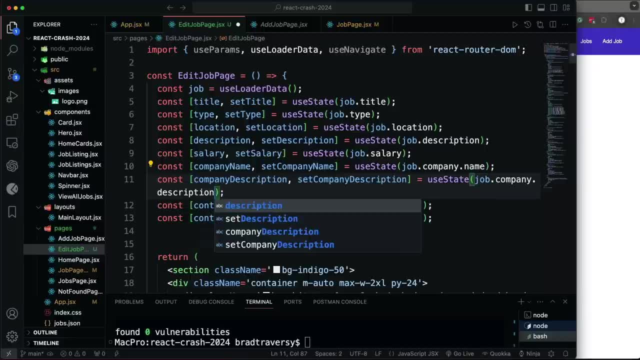 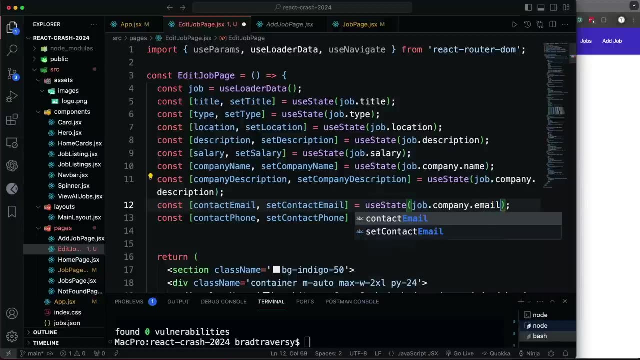 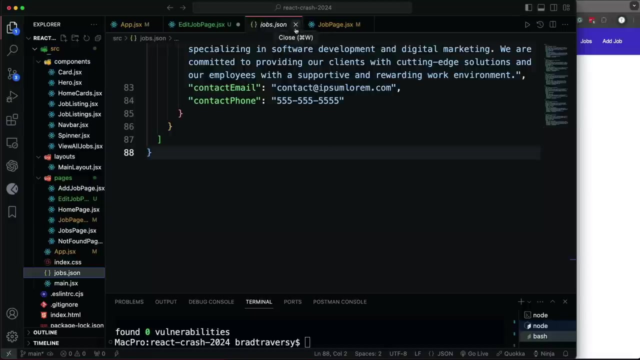 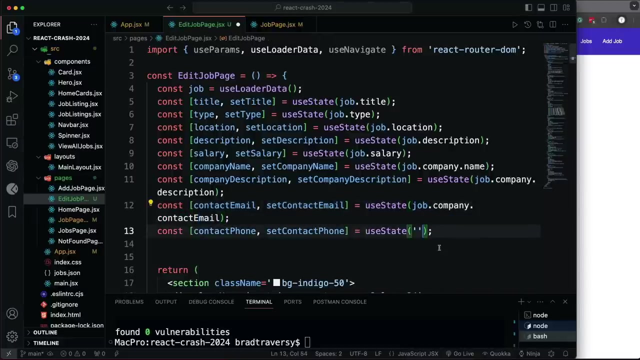 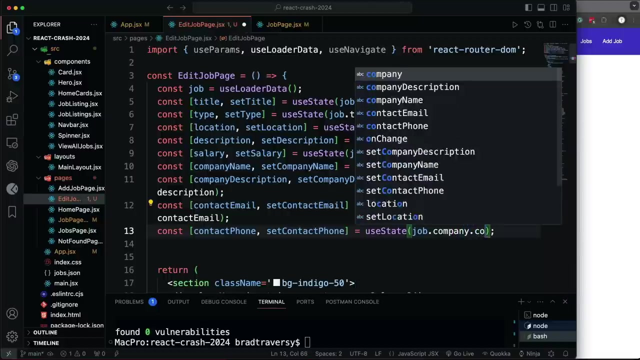 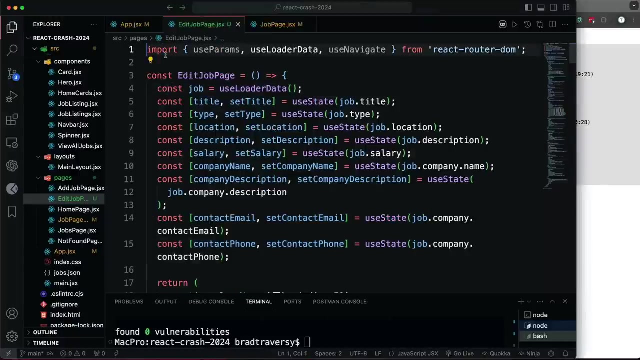 it's name: company name and then job: company dot description, company dot email. let me just double check. I think it's contact: yeah, contact email and contact phone: job, co. company dot contact phone. all right, so if I save that we get use stays not defined, so we do have to bring in you. 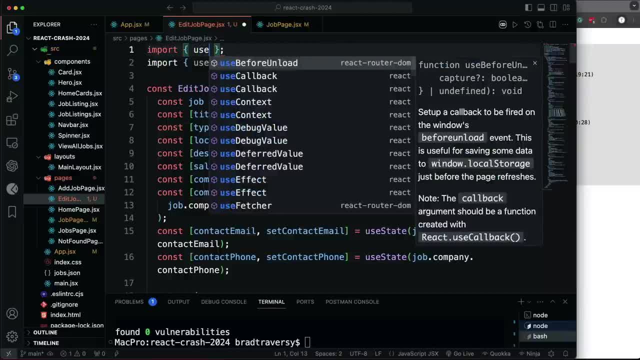 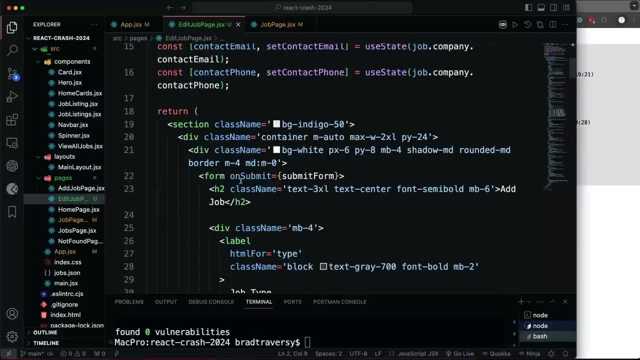 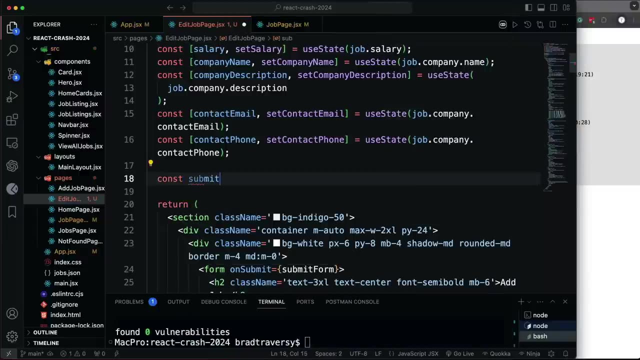 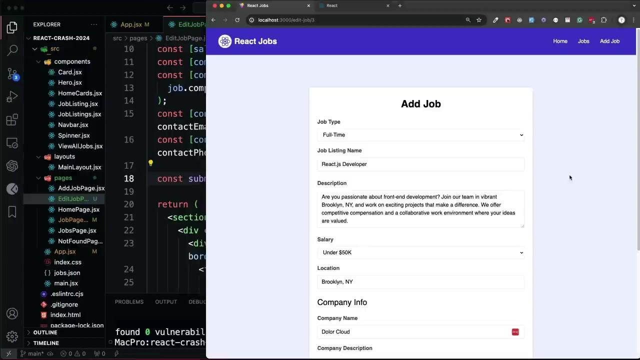 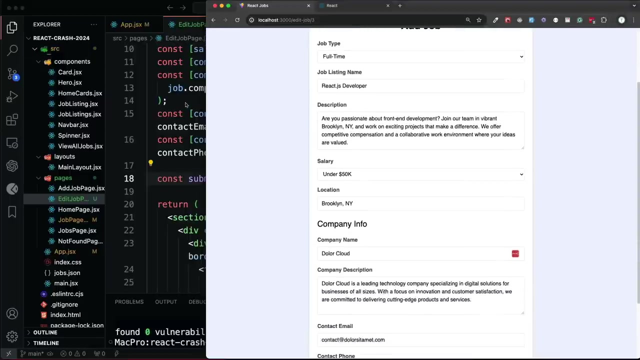 state submit form is not define, so the form has this on it. this submit form functions, so we just need to create that, say submit. I don't have to put anything in it just yet. just create the function And now you can see. the form is actually populated with the right data, which is exactly what. 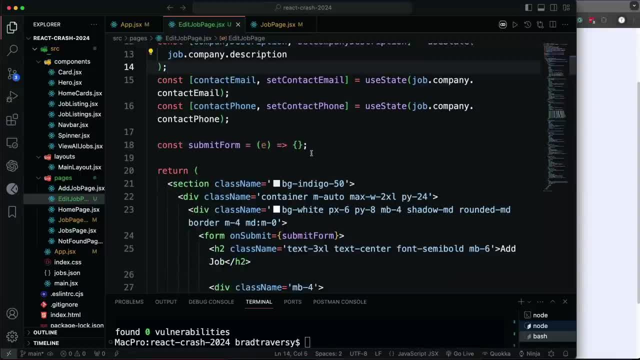 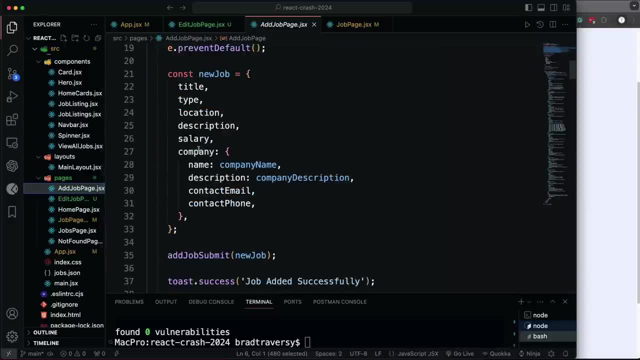 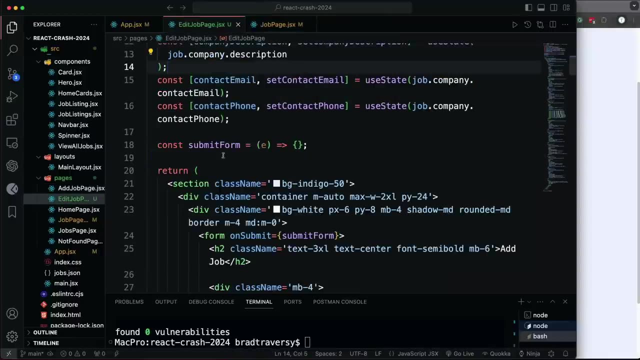 we want Now the submit form. we might as well copy it from the ad, because we're going to do the same thing and construct a new job. So let's just grab- yeah, we'll just grab- this whole thing And then, in the edit submit form, paste that in. 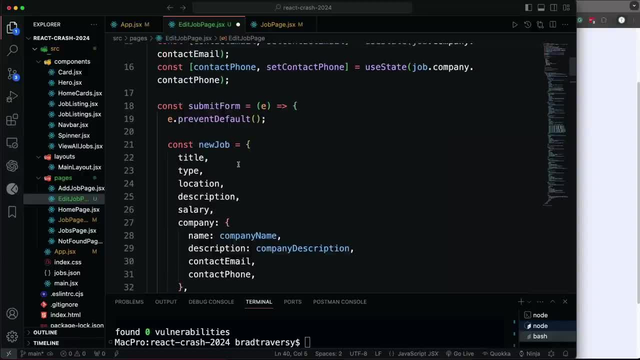 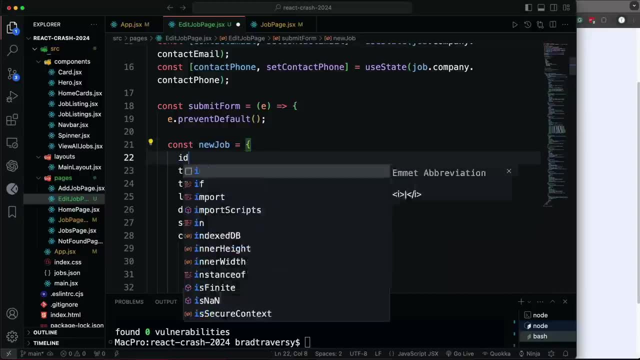 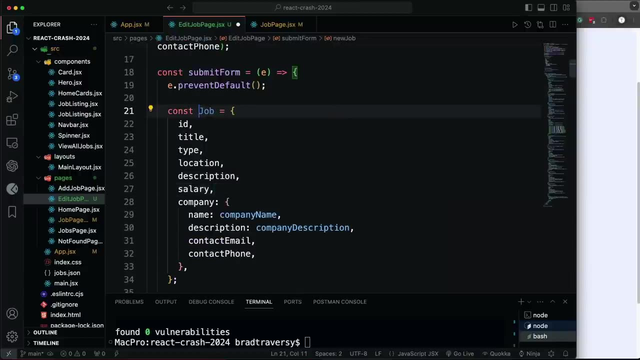 Now, one difference here is going to be: we're going to pass along the ID because we're going to need it when we make the request, So I'm just going to pass in ID right here And then, instead of- actually instead of new job, let's call this upload. 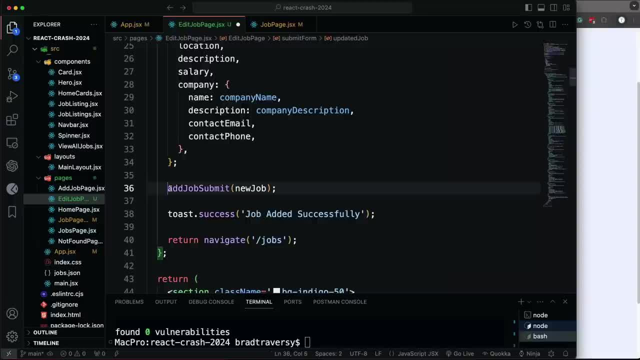 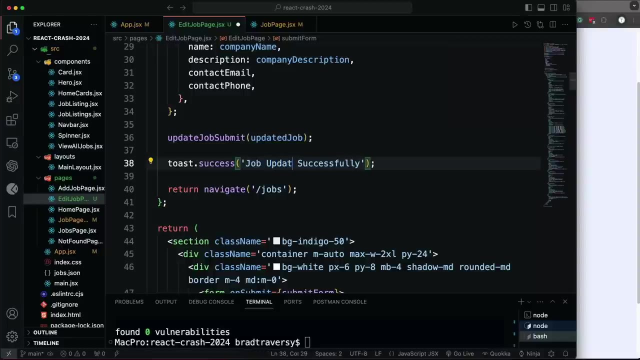 Updated job And then, instead of add job submit, let's say update job submit And pass in updated job, And then we'll do a toast. we'll say job updated successfully. But we do have to bring in toast, because I don't think- yeah, we didn't bring it in. 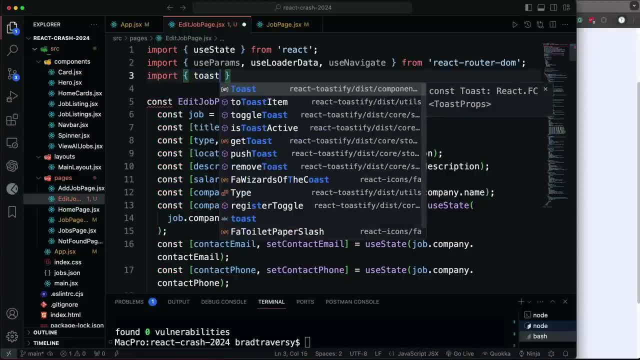 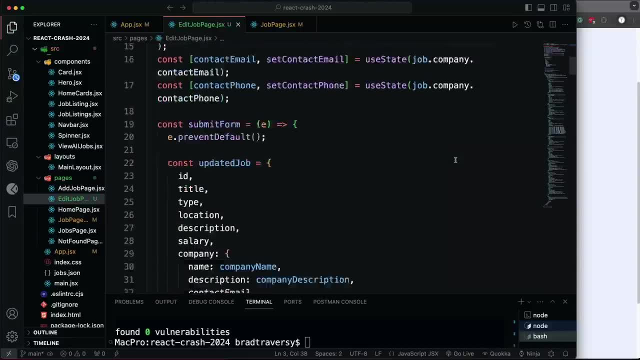 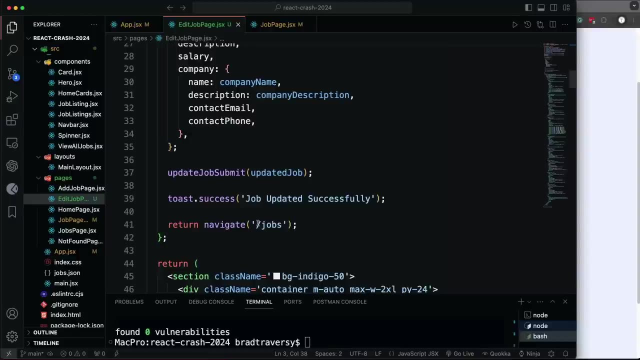 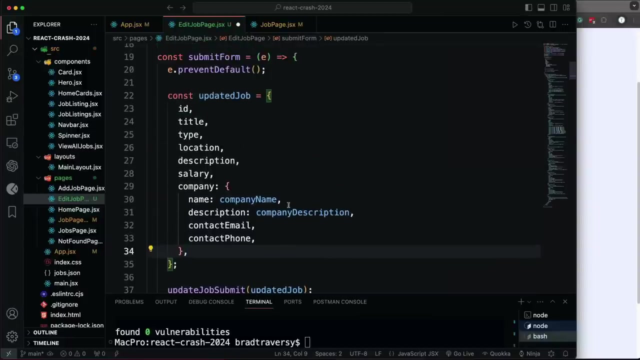 So import toast. Okay, Now this, this, actually, let's also redirect to the job page. So let's put in some backticks here and we'll say job, job, slash, and then the yeah, we just put the ID. 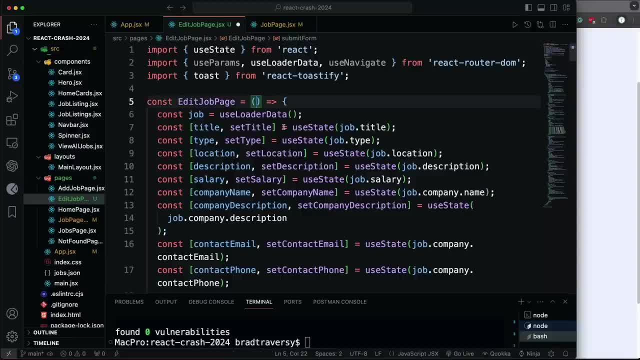 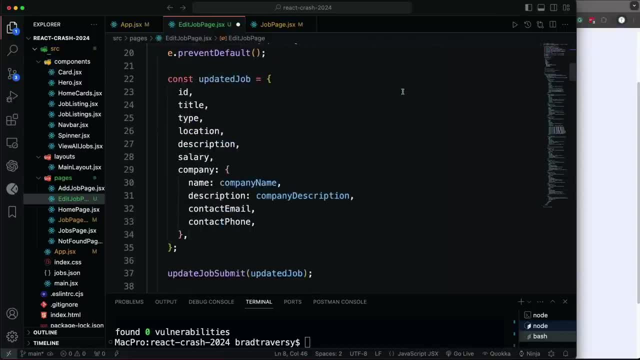 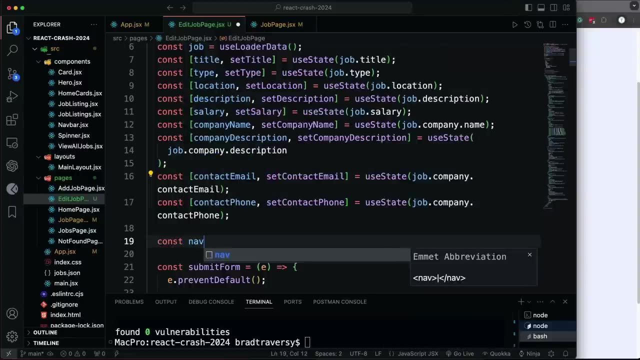 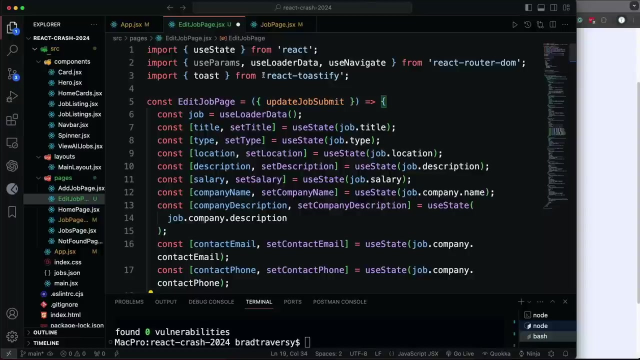 Now this right here: update job submit. We're going to pass in as a product Prop, So update job submit. Also, if we're going to navigate, we're using navigate here. that means we have to initialize, use navigate And yeah, I don't think we need. we don't need use params. 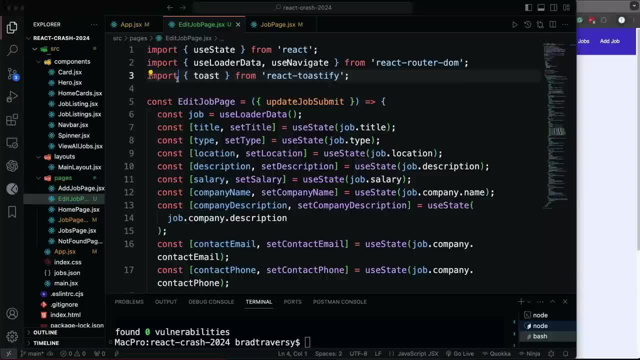 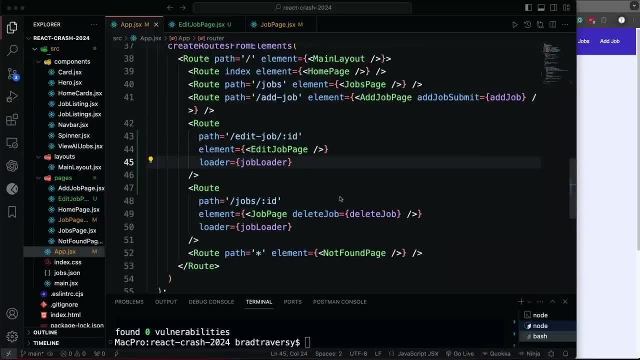 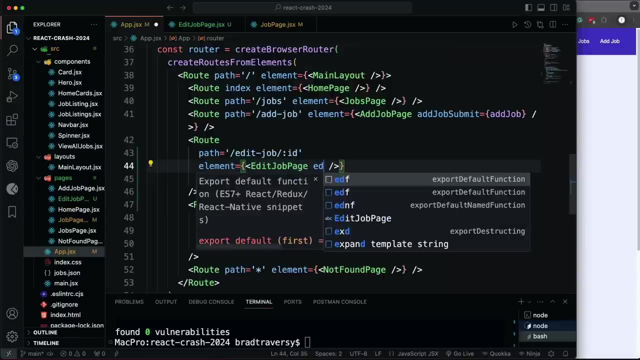 So that should be good. All right, Now this update job submit. let's go back to our app JS, because we need to basically catch that and then fire off a function in here. So where we have our edit job page, let's do update job submit. 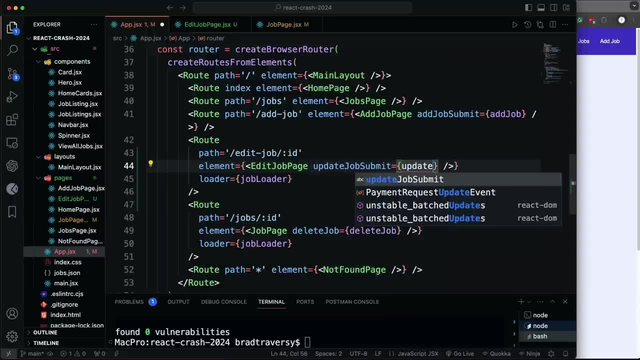 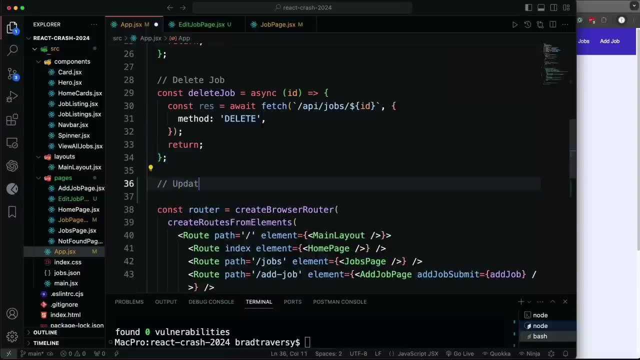 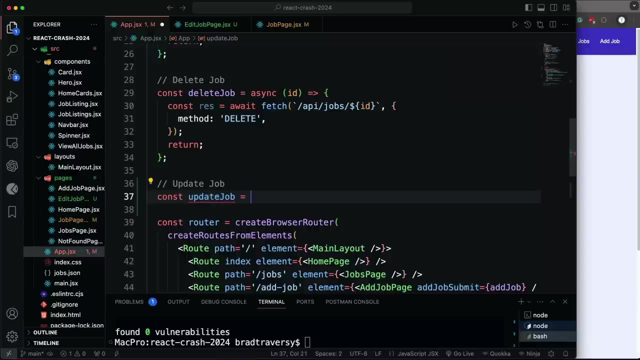 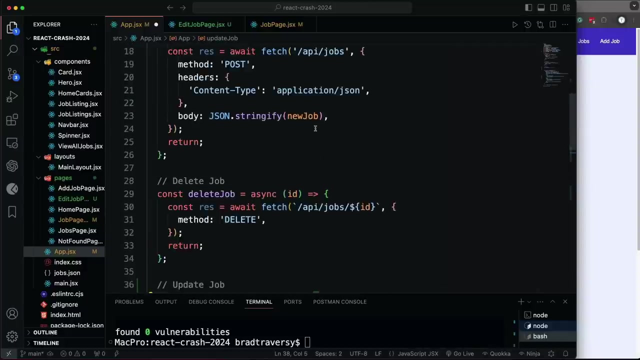 And we'll set that to a function called update job And then up here we'll create that. Okay, So, const update job. all right Now as far as what we're going to do here, I'm just going to copy this from the ad and: 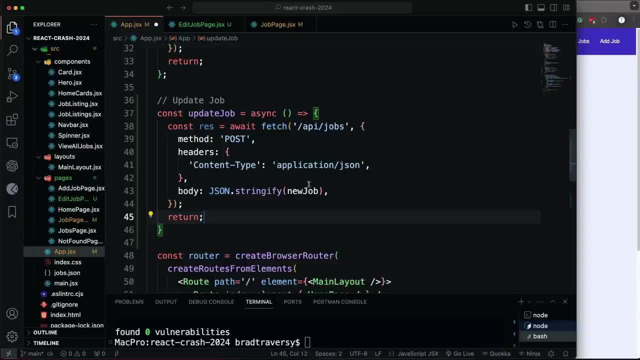 you could put these requests in a separate file if you want and some kind of service, but I'm just, I'm trying to keep things simple, Let's see. So this is going to be fetch And then, um, the job will come in here and then we'll change these to back ticks, because 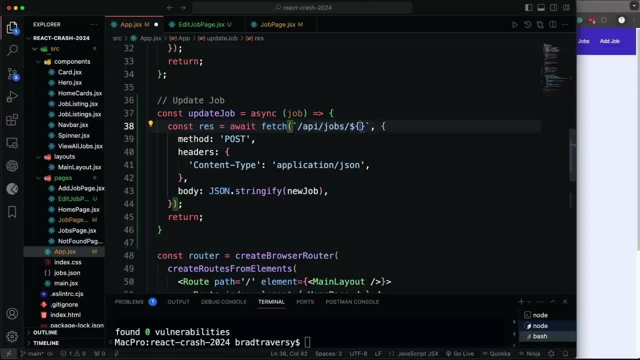 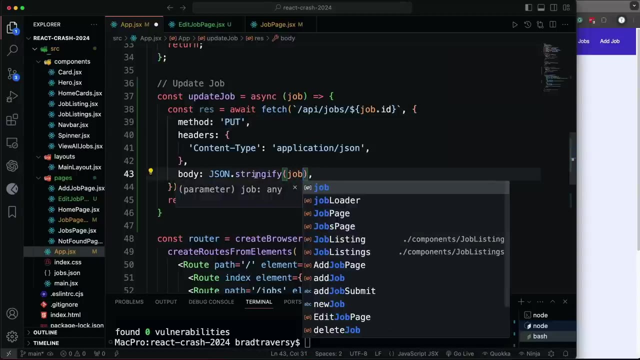 it's going to be jobs slash and then job dot ID. So that's why I added the ID in the other file. It's going to be a put request and let's see the body here is going to be job. Actually, We can call it. 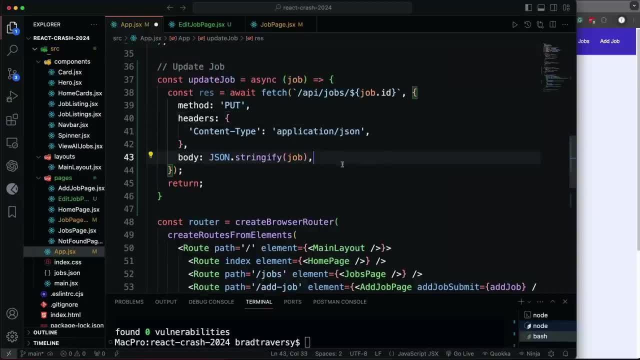 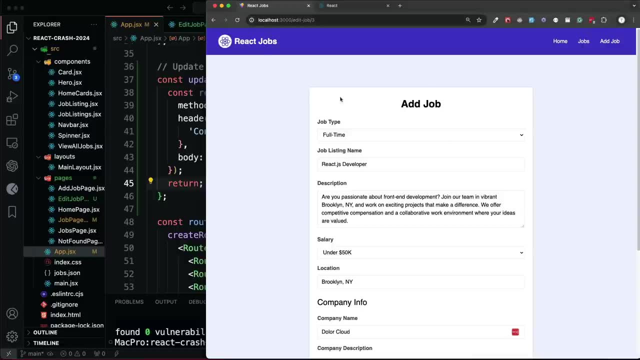 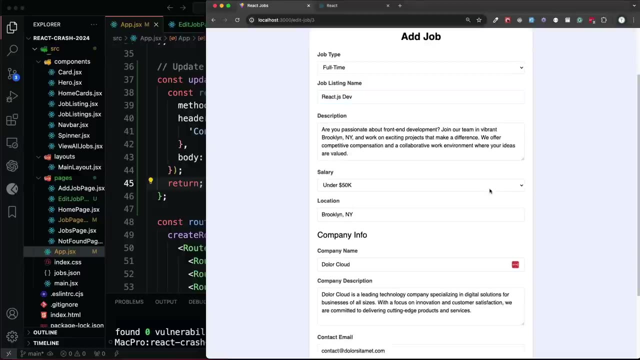 Actually we can call this: No, that's fine. Yeah, And then that should do it. Let's save that and let's try it out. So we have our react JS developer job. Let's change it to just react JS dev and we'll keep all the rest of the stuff. 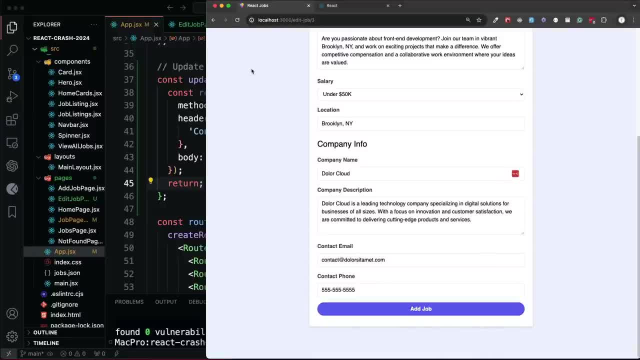 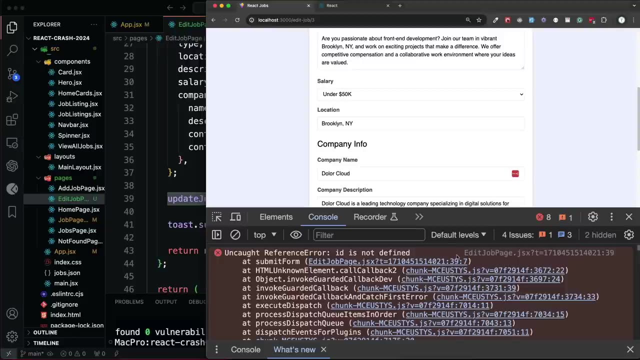 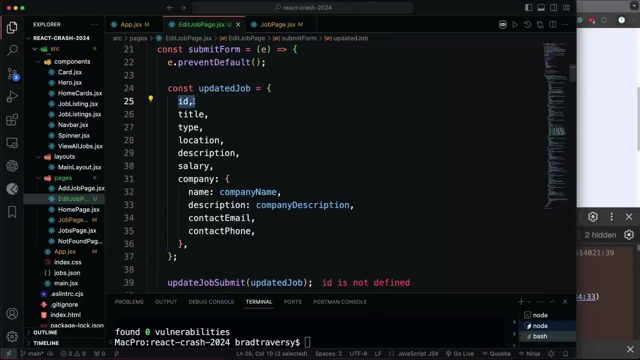 Add job. Uh, it's not submitting, Okay, Okay, Okay, Okay, Okay, Fine, Referenced ID is not defined. Oh, ID is not defined. Um, so this? So I guess, yeah, I guess we do need the use perams, cause we got to get the ID. 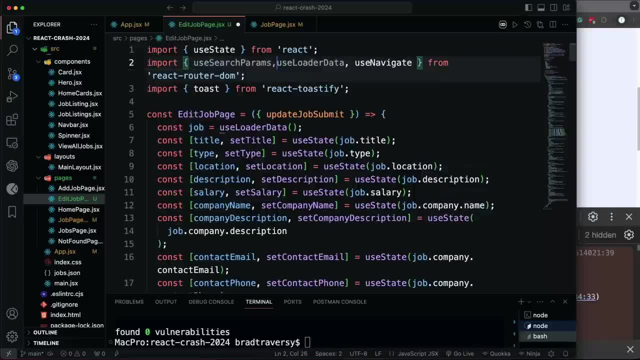 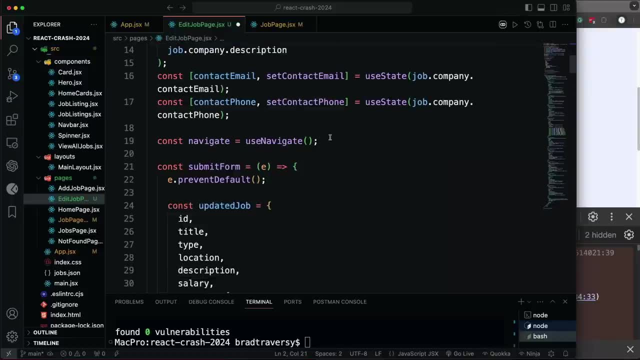 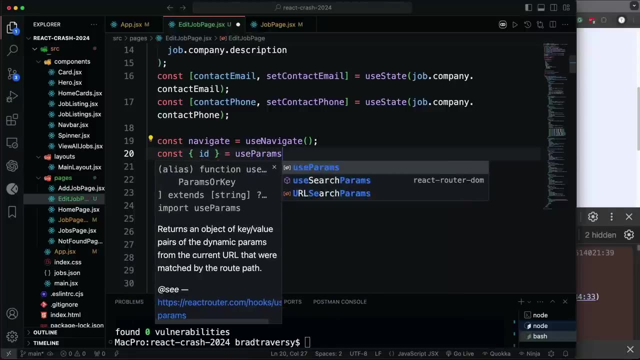 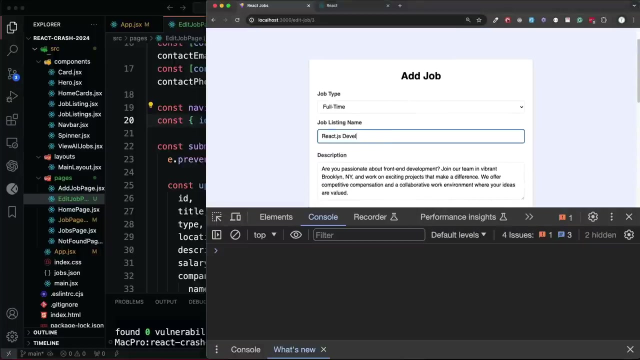 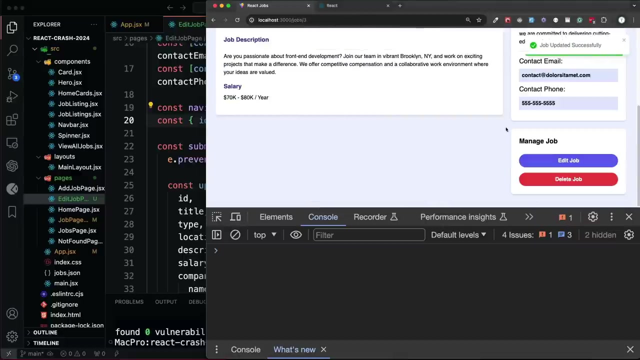 So from reactRouter dawn dawn, let's say: use params, Yeah, Yeah, Yeah, We can just go right here: const id: use params. okay, we'll try that. change that to react-dev. We'll change the text to this too. but let's submit job updated successfully and it changed. 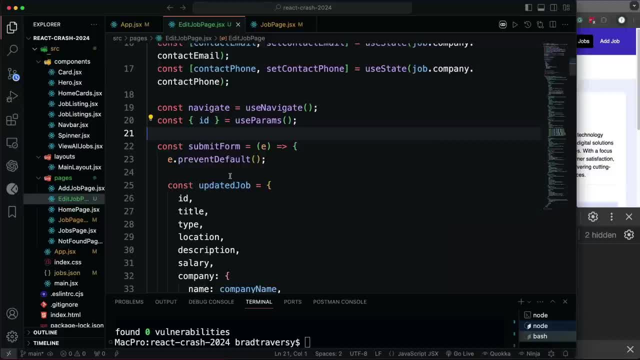 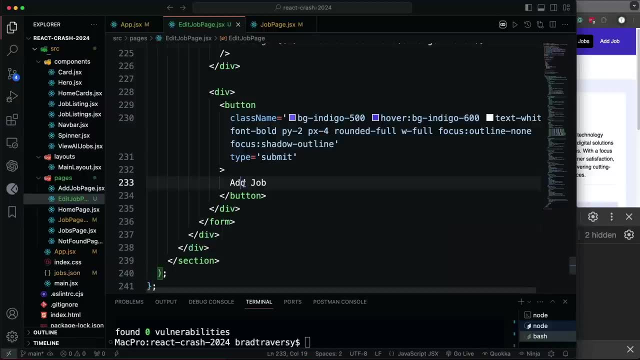 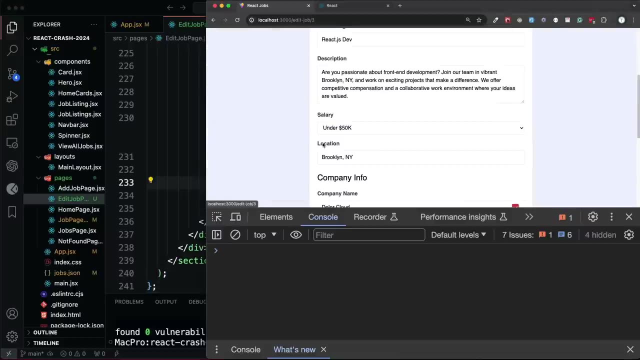 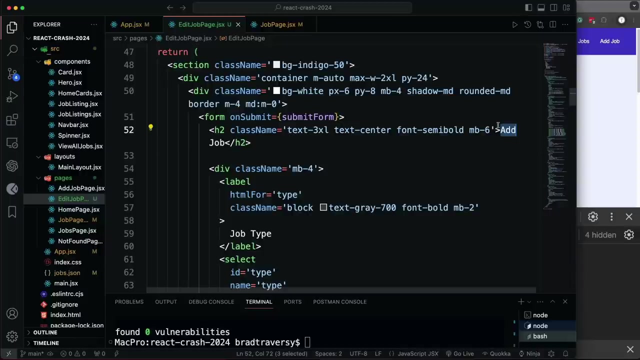 to react-js-dev and it redirects us to the page. Let's just change the button text. So right here, change that to update-job. Is there a heading too? Yeah, we'll change the heading because it says add-job. So, right here, update, All right. so we have a full CRUD. 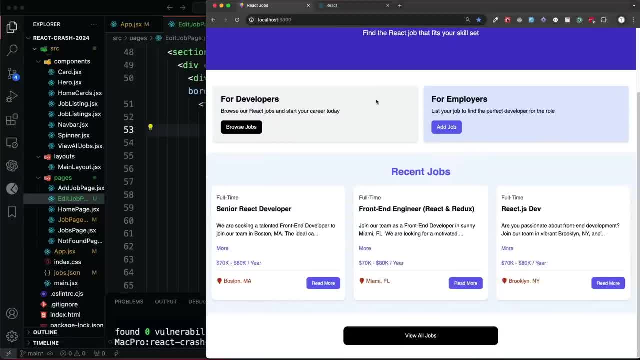 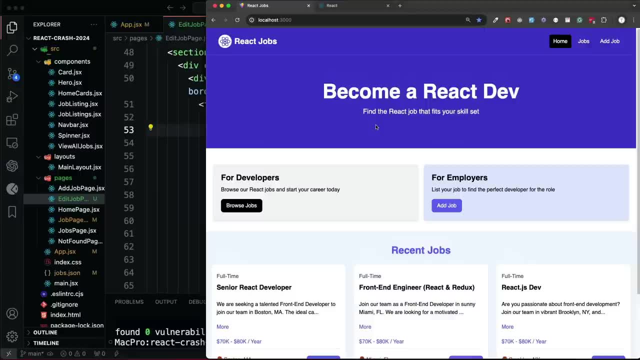 application. The only thing we're missing is authentication, but, like I said, that's beyond this tutorial. This went way longer than I initially planned and wanted, but we did a lot. You know, we learned about components, props, state, the react-router, data loaders. 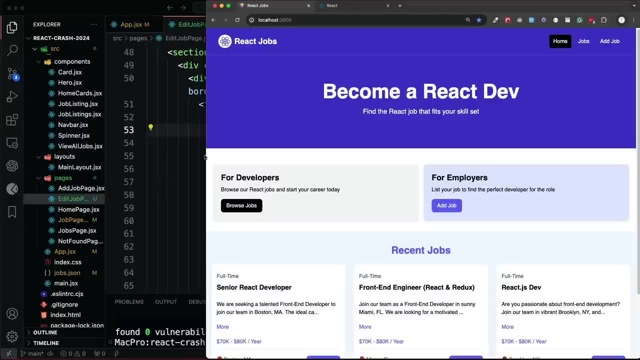 useEffect, useState, useParams, all those hooks with react-router-dom. So I think we touched on a lot and I think that you should have enough to create some simple projects on your own. Now, as far as deploying, what you would do is just run npm, run build, and that will give you. 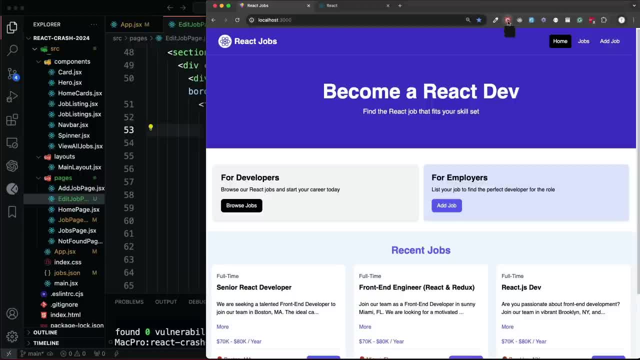 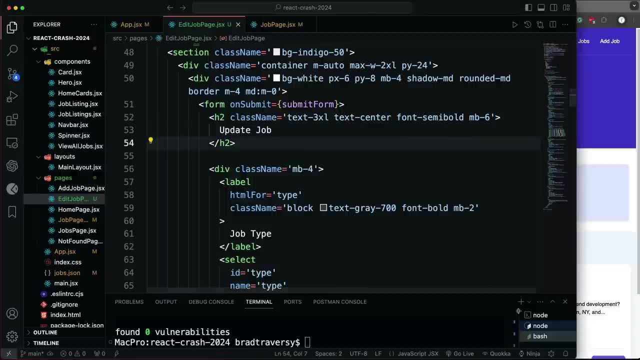 a production version of your site. You see how the react-dev tool's right here. it's orange and it says this page is using the development build of React because we're running the development server. So what I can do is stop the development server. 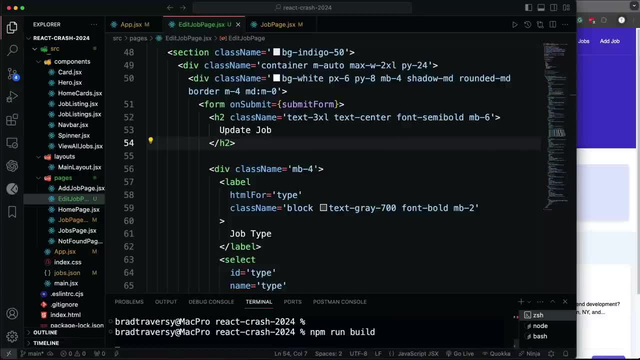 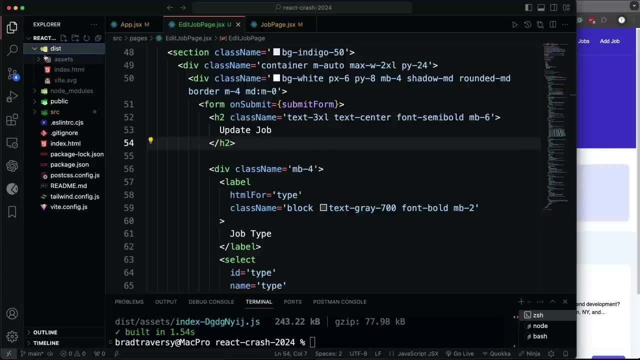 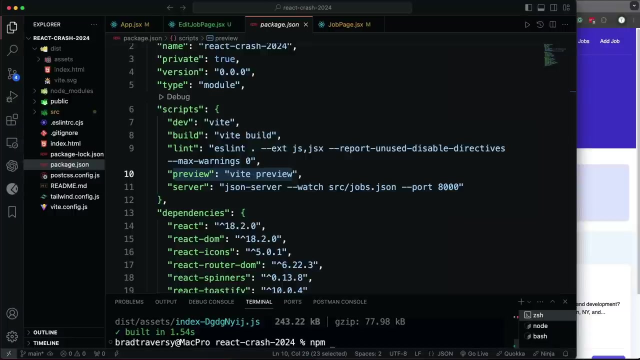 and I can do npm, run, build. What that'll do is create a new folder called dist and that dist is your production build. Okay, so I can run that with Vite. In the packagejson there's a preview, right, this preview, and that should run the development build. So let's say npm. 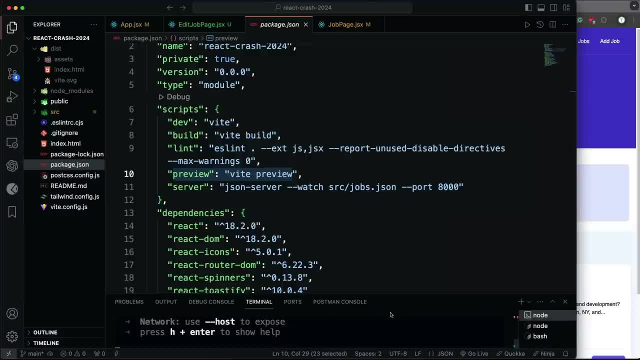 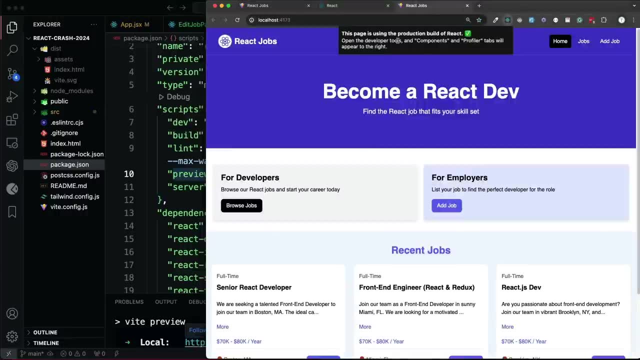 run preview And that's running on 4.1.7.3.. So now notice: this extension says this page is using the production build of React. Okay, so now this is what you would: deploy: this dist folder And you. 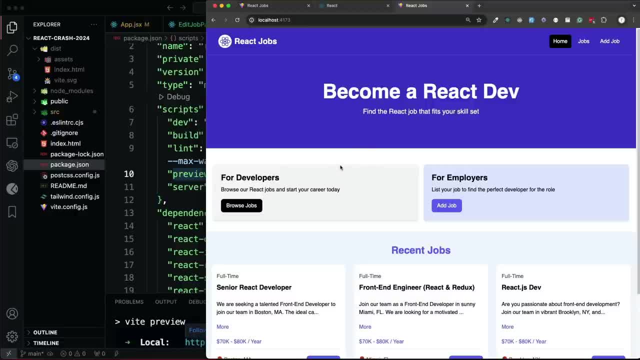 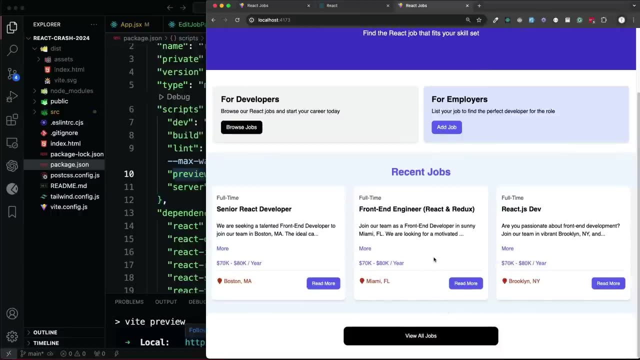 could basically deploy it anywhere. Now, if you do try to deploy this, it's not going to show the jobs because we're using a local server. we're using JSON server. If you actually want this to be a real project, then you're going to have to create an API with Express or something else. But 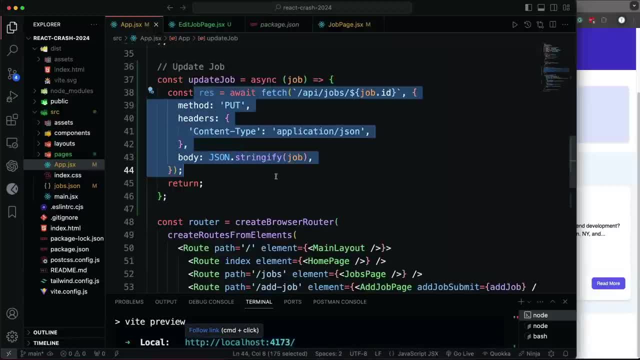 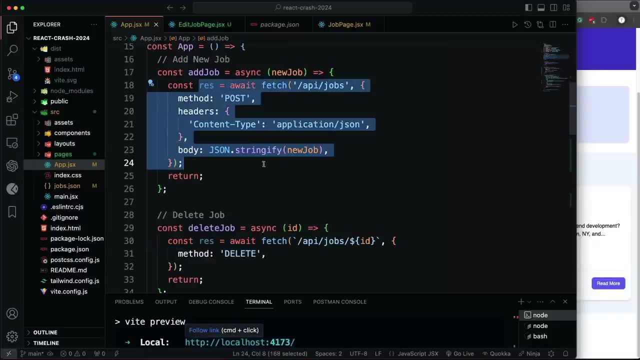 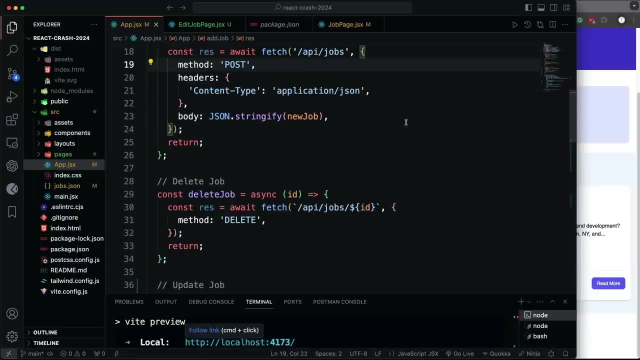 you're not going to really have to change anything as far as this stuff, Because this is going to be the same whether we're dealing with JSON server or you're dealing with a REST API with Express, Django, Laravel, just whatever. So, yeah, I mean, this is, this is a front end course, But I did want. 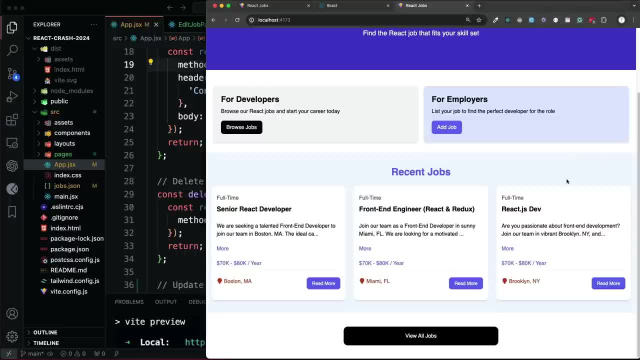 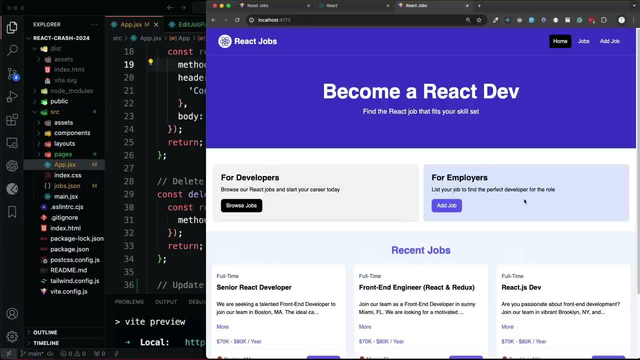 to give you some examples of using back end data, because that's what it's what you do in the real world. All right, guys. so hopefully you enjoyed this. I hope you learned something from it. Like I said, there's so many. 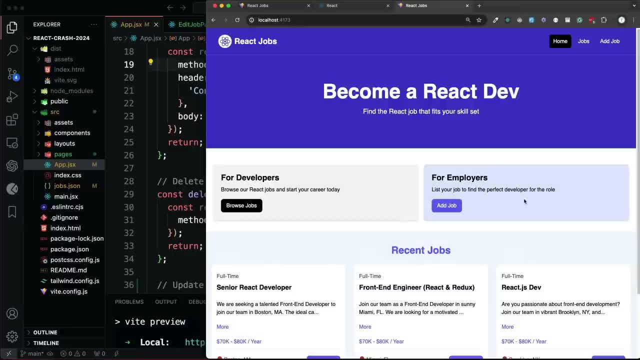 different ways in React to do everything. So if you saw some things the way that I did and you didn't like it, that's fine. You know everybody has their own way of doing things. And also keep in mind I try to do things as in the simplest way possible so that I can explain it and people can. 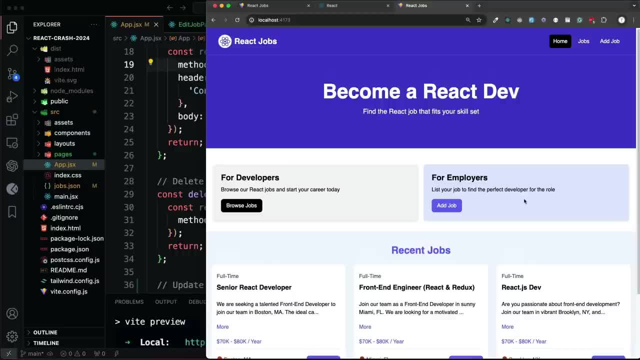 can learn it understand. But that's it, guys. Thank you so much for watching and I will see you next time.